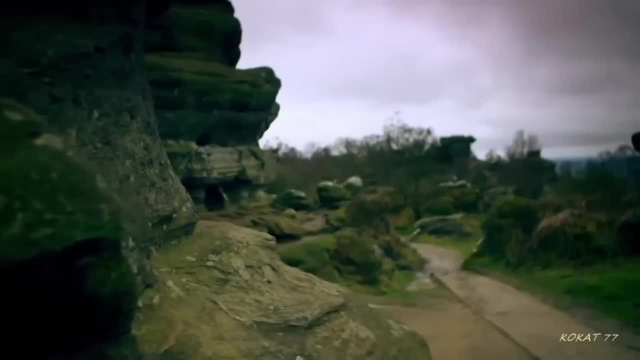 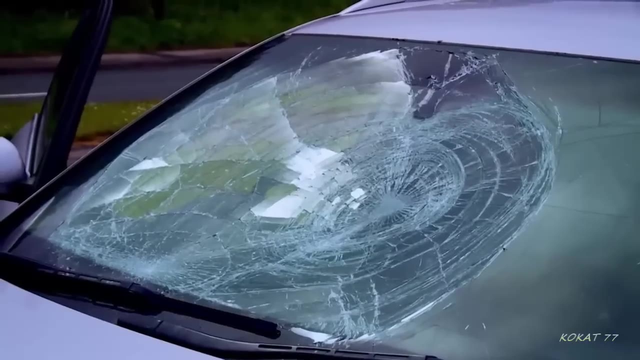 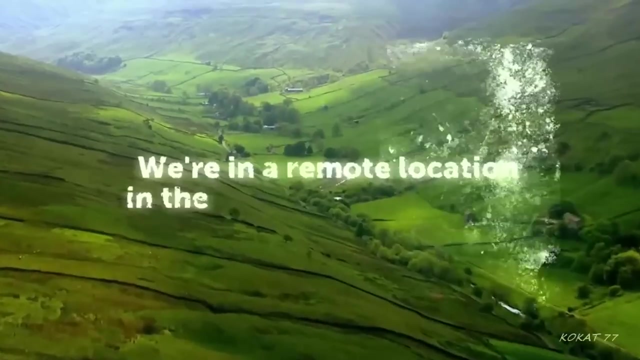 life is on the line. How far did he fall? About five metres. He's intubated and ventilated. You need some of Britain's most elite medics. Is there any serious bleeding? Yes, there is. yeah, Carb fill legs anything below my neck. We're in a remote location in the 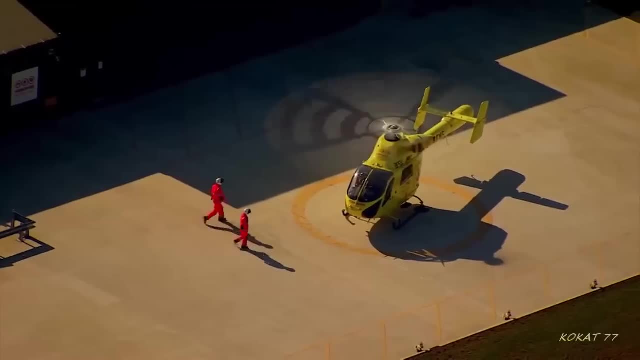 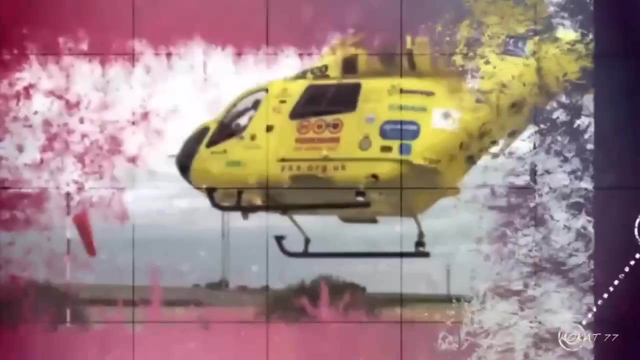 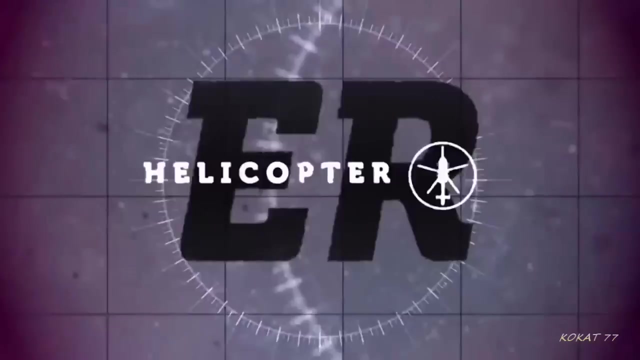 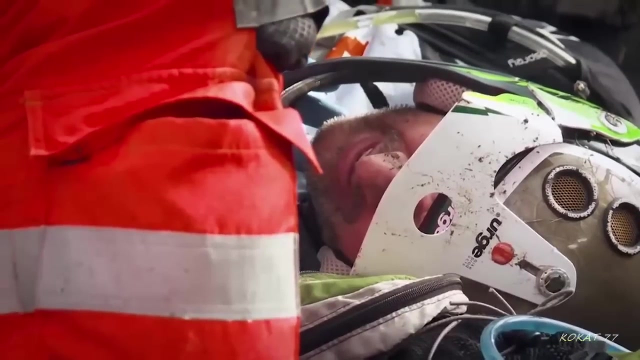 middle of the woodland There's broken a bike. The speed of the Yorkshire Air Ambulance can make the difference between life and death. Your discretion to take off. FedEx 99 listed Today: a mountain biker hits rocks head first. He's lost all sensation from the neck down. 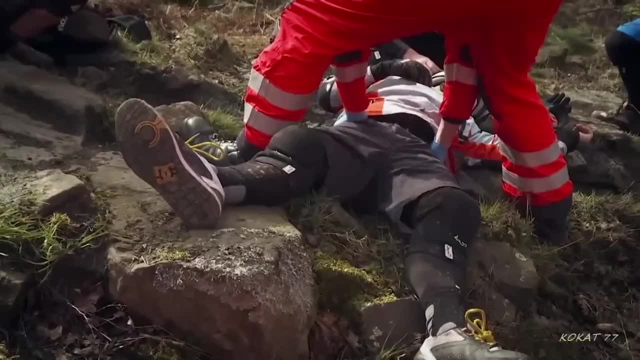 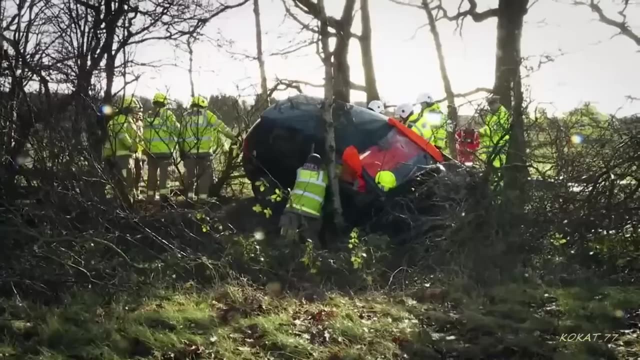 Felt like my head was just rolling down the hill. Yeah, Couldn't feel legs, anything. A driver and passenger are trapped in their car after it left the road and cartwheeled into trees, Come off the road at speed. Actually it's quite difficult. We've also got a ditch. 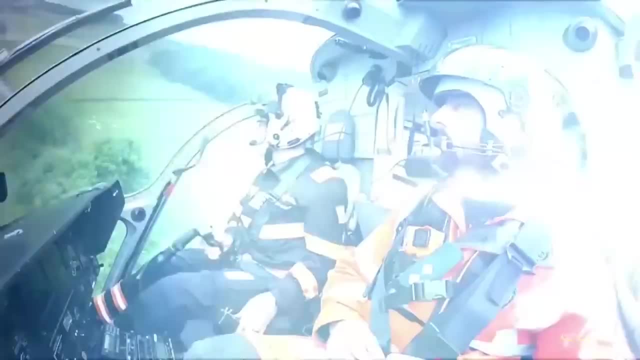 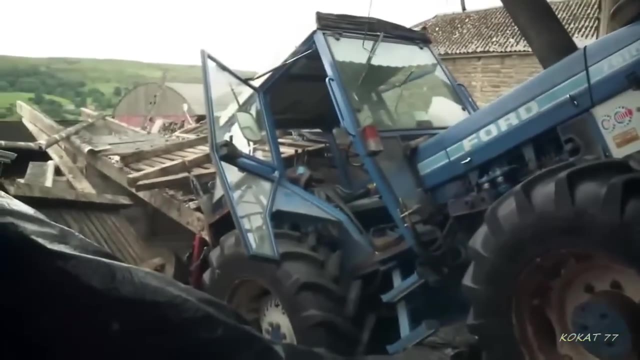 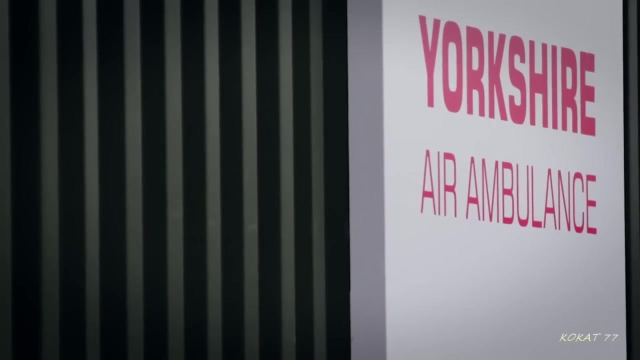 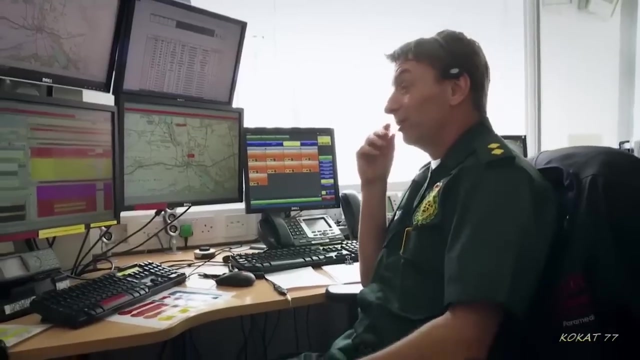 full of water. Nice, and still for me. my friend And the team fly into an isolation farm to rescue a tractor driver injured in a freak accident. This chap was with her. He thought she was dead. Hey, this is Tony. 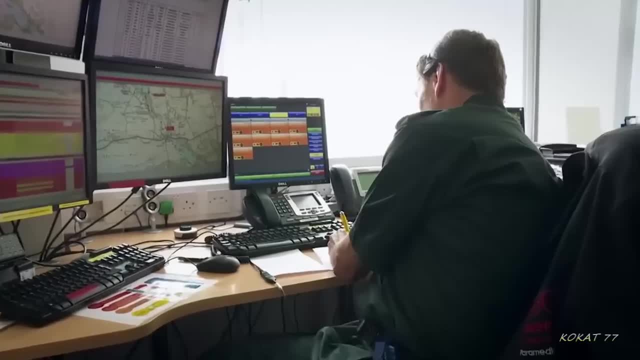 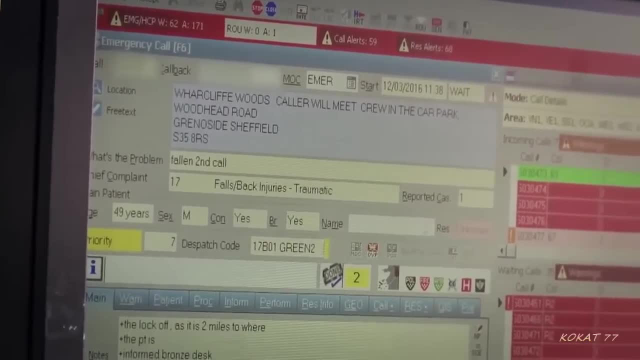 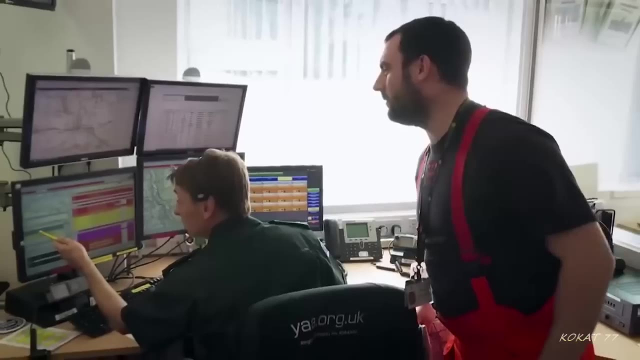 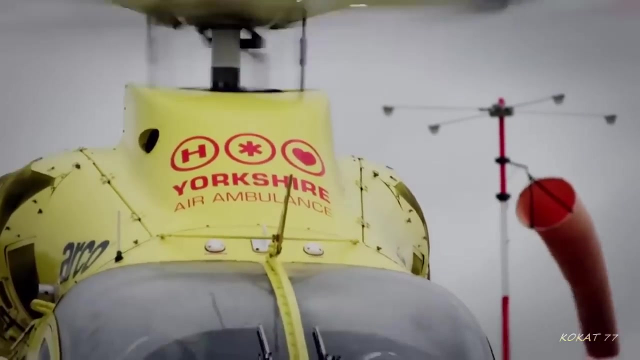 At Helimed headquarters. paramedic Tony Wilkes is on the phone to the ambulance service control room. There's an emergency in woodland on the edge of the Peak District. I haven't got a job. The rider is lying badly injured. Helimed 98 is off the ground. in less than a minute They'll be over the emergency scene. 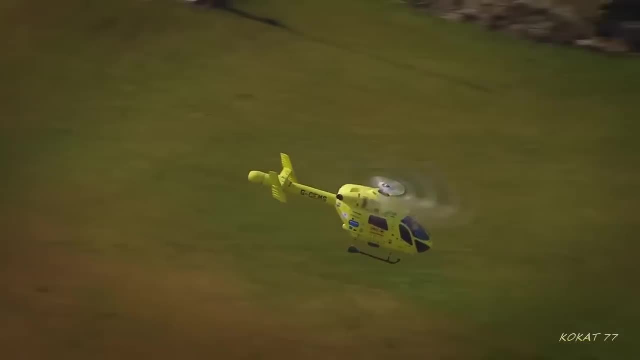 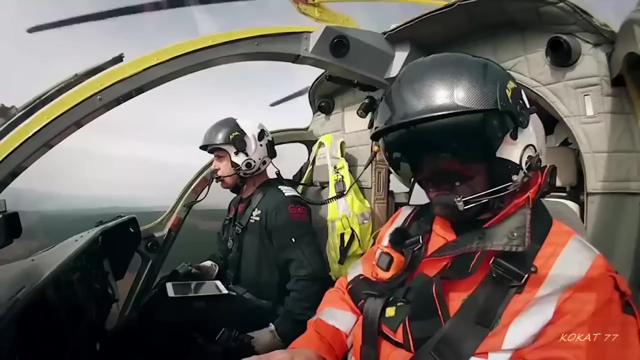 in ten. Tell me exactly what's happened. We're in a remote location in the middle of the woodland. The patient has fallen off the bike. They're complaining that they've broken their back and can't feel their arms in the way Eyes out. We're over here somewhere. 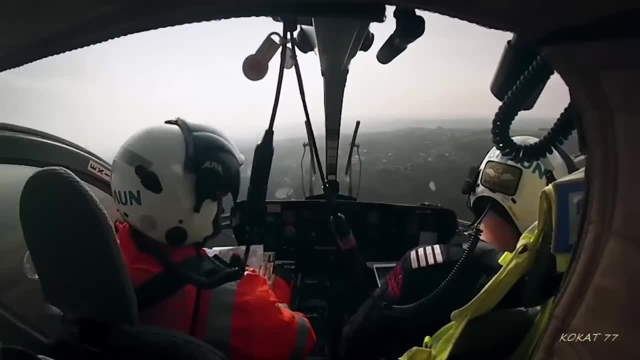 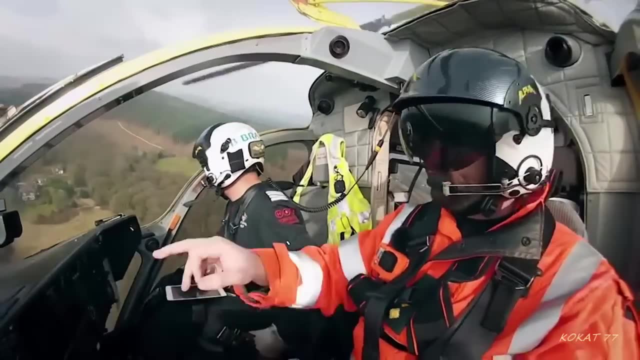 Yeah looking, Paramedic James Stubbley is navigating today. The patient is in luck. James is a mountain rescue leader with an encyclopaedic knowledge of the Peak District. This road is where they'll access with the RRV, the road that runs in between. 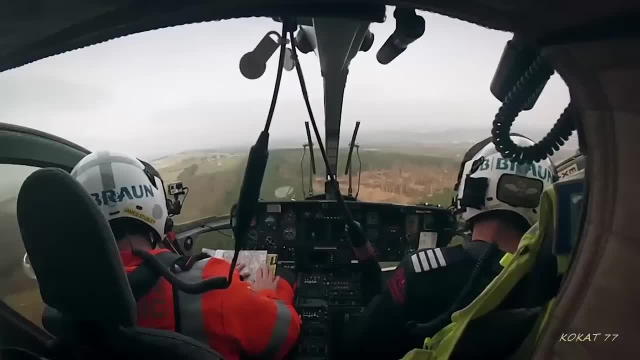 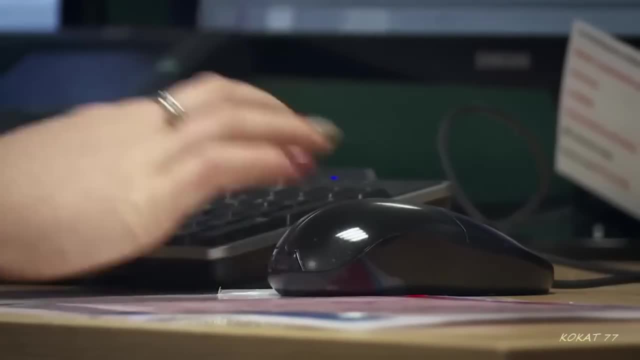 The RRV is just below us now. Yeah, All right. Do you know where that runs off? There's roads both sides of the road. That's the trouble. It's probably nearly two miles from the lock gate to where the patient is. 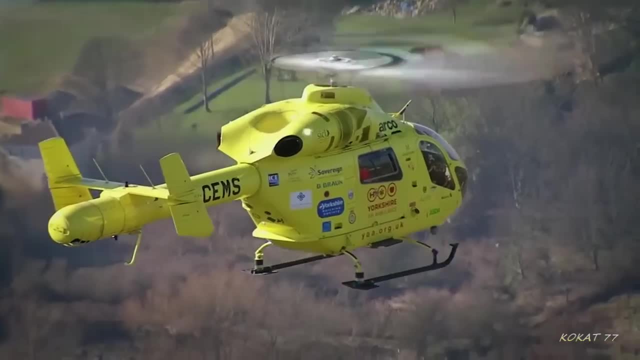 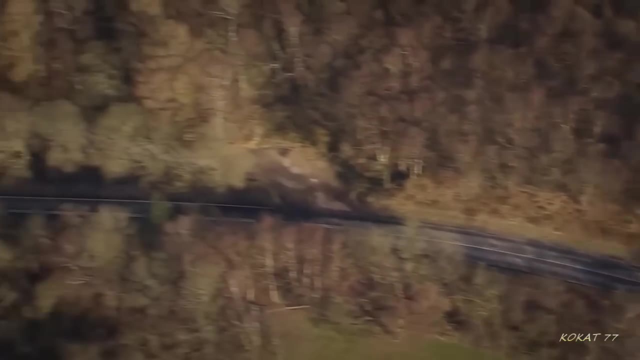 OK, So that's why I'm saying that we might need a fiber gate to cut the lock off. Right, OK, They're flying over one of Yorkshire's most popular and dangerous mountain biking sites, But on the far side, near the car park, there's a lot of downhill black runs. 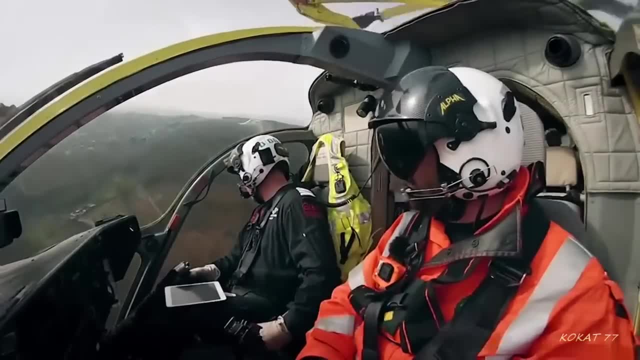 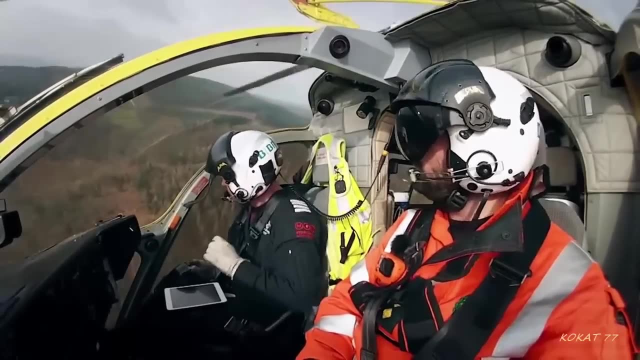 On the other side, On the other side where the car park was going out further out. yeah, I can't see out at all, But it's still not going to be easy to find the casualty. They only have vague directions from the 999 call to go on. 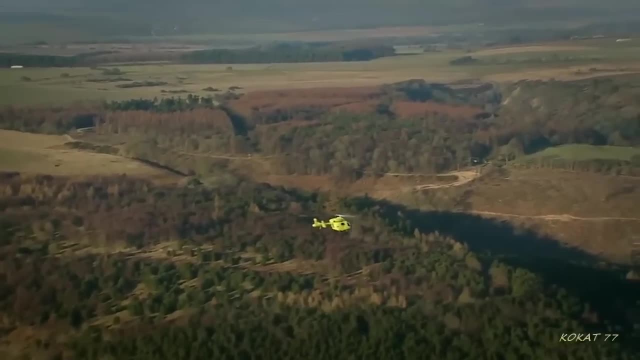 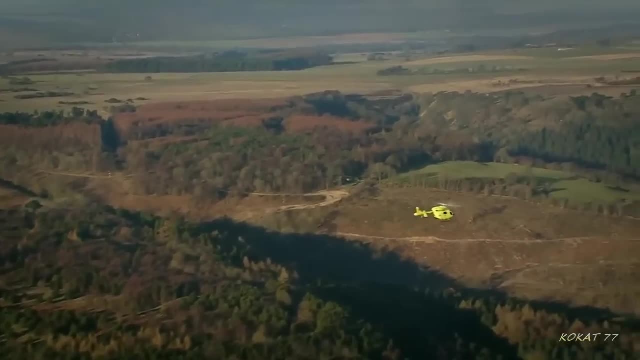 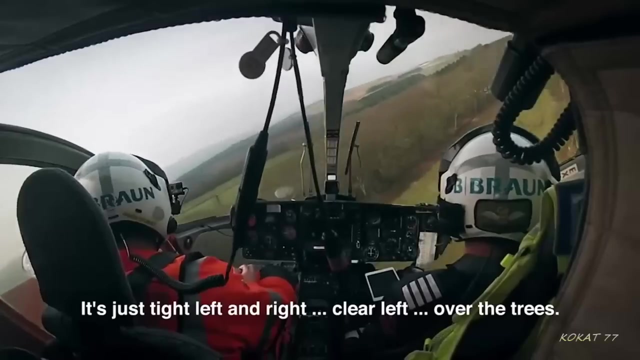 Yeah, Yeah, Yeah Yeah. Thousands of acres and the team has few clues to the scene of the accident. RRV's just pulling up the car park, so It is tight. left and right It's a lot of debris. 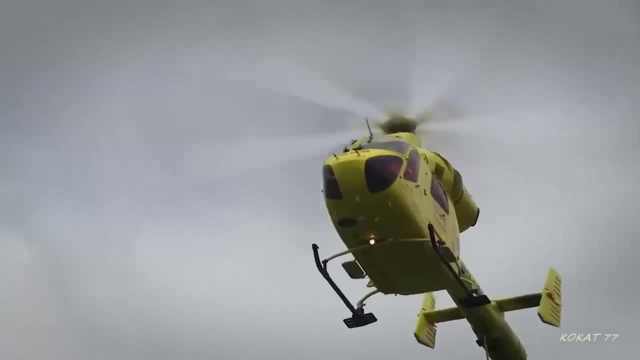 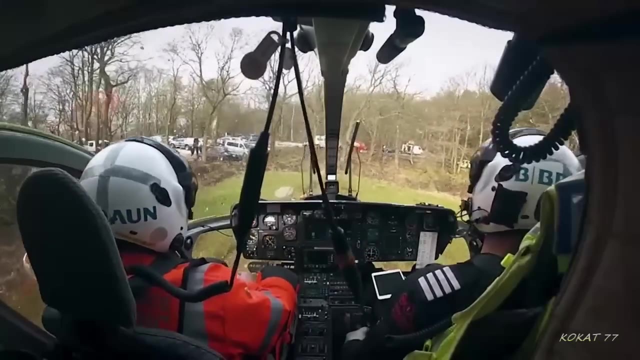 I'll say it, right, mate. It's very boggy in the foot, Pilot Gary's touching down, so paramedic Paul Holmes can ask other bikers if they have any clues. A bit more firmer there, mate. OK, take it out, Gary. 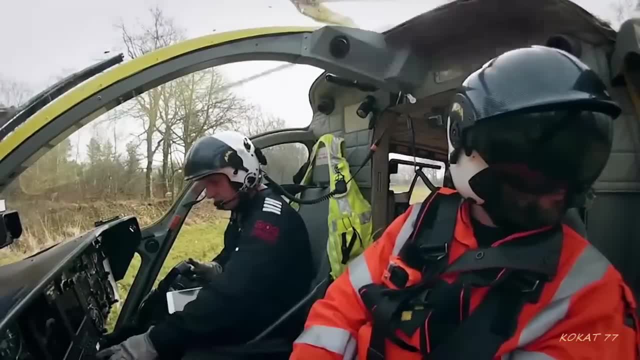 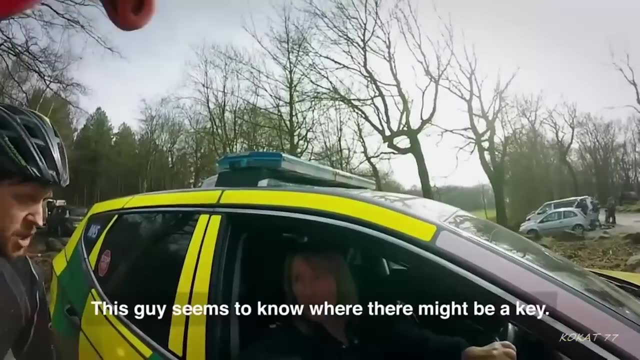 Yeah, I'm just going to go to idle. I'll wait here for a minute. Yeah, sound, There is a field, but then there's quite a high gate. All right, Oh, we'll sort that out. This guy seems to know where there might be a key. 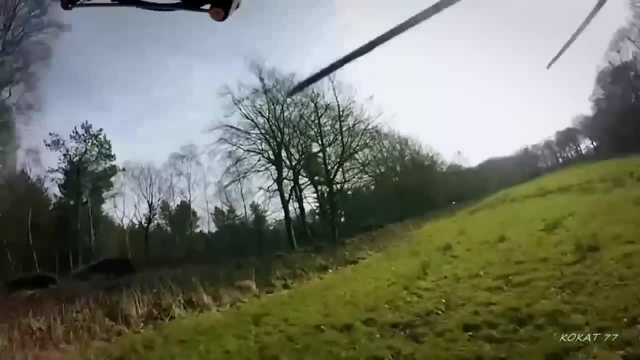 It seems the man's lying on a gated track deeper into the woods and, worryingly, he's showing signs of paralysis. Right, he's about a mile and a half down that track. There's a cyclist He's going to take. 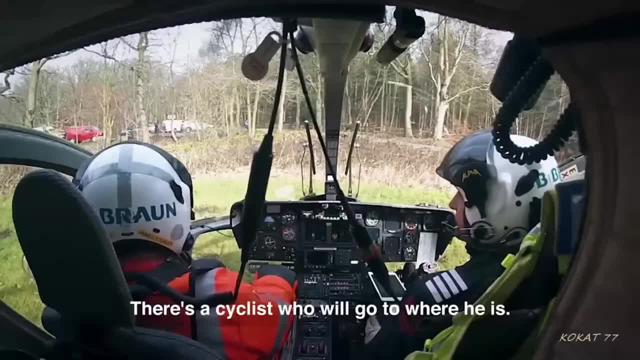 He's going to go down the track to where he is- The track on our left-hand side, Yeah- where the people are. OK mate, All right, we have no wind, so I'm just going to go straight, Yeah. 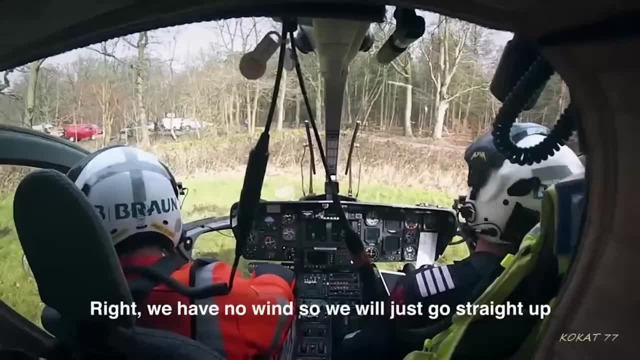 Yeah, Yeah, Yeah, Yeah. I'm going to go straight up, Turn round and straight up here. What's Bron's going to do? Is she going to go down? Yeah, she's going to go as far as she can to try and get a key for the gate. for where? 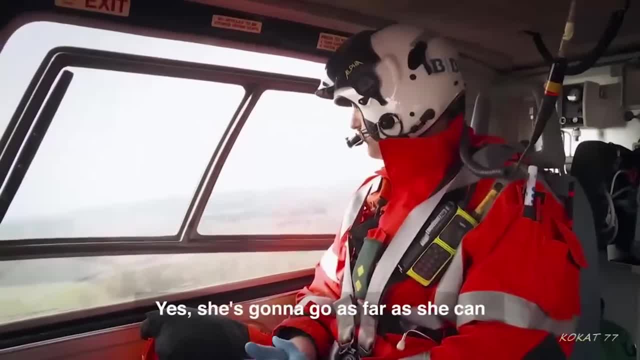 the patient is The key on Middlewood Station for it. I put it there myself Four years ago. I don't want to say I told you so, but Is that the cyclist there? Yeah, Yeah, Follow him. He'll take us to where he is then. 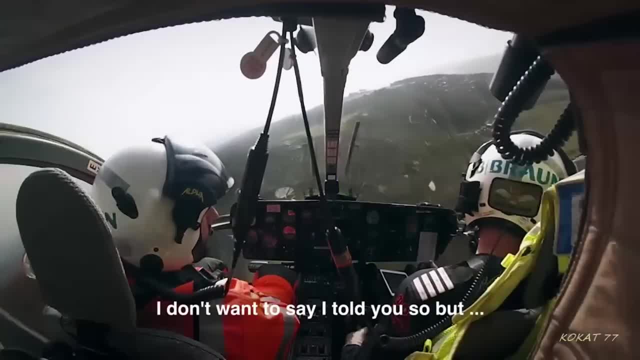 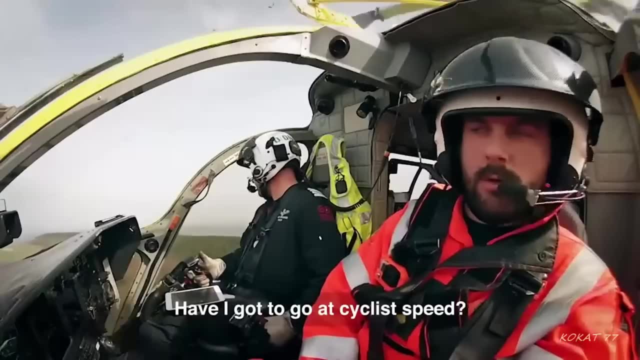 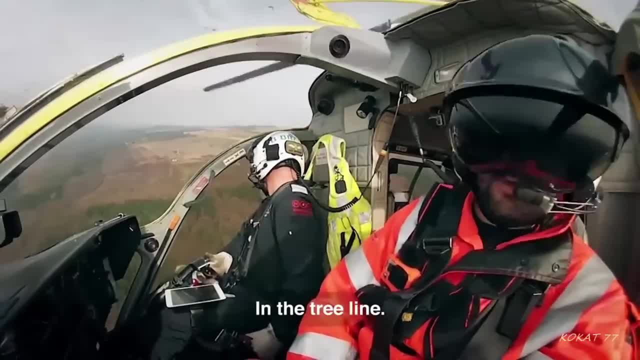 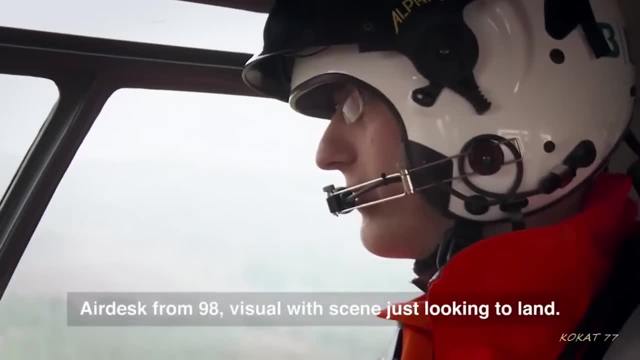 3 o'clock, Not seen In the tree line. He's got the wires. They're standing in the lower ground. the wires, Yeah, think of them, Ed. this is Kurt, from 9-8. Visual we're seeing. 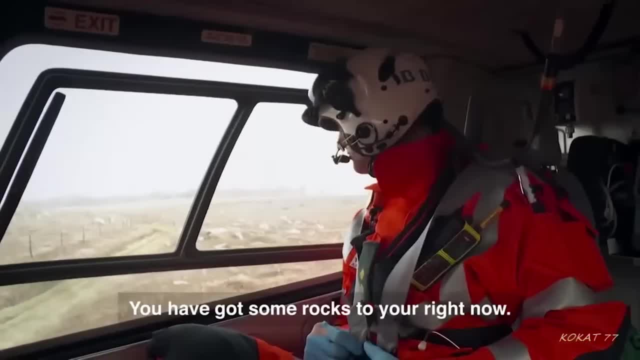 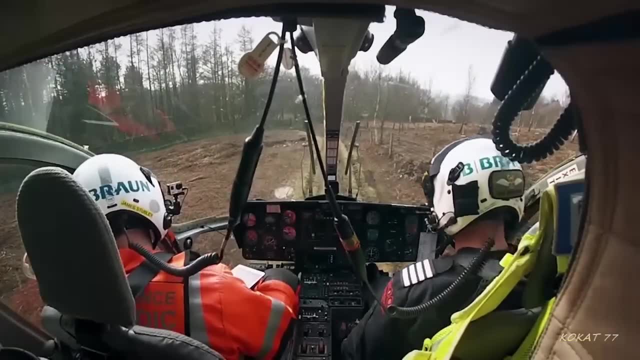 Just looking to land Right, not to land. there's a rock or something. You've got some rocks too, right? Yeah, Yeah, Yeah. Gary's touching down as close to the accident scene as he can From here on the team's on foot. 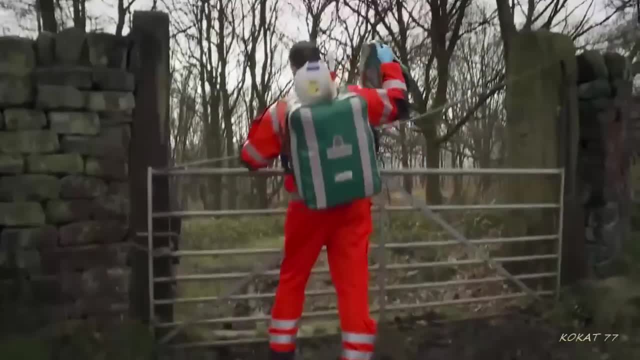 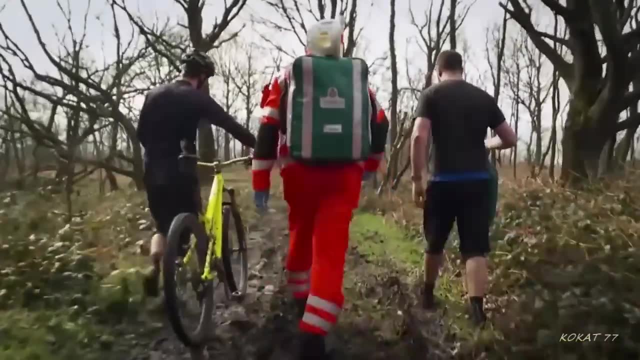 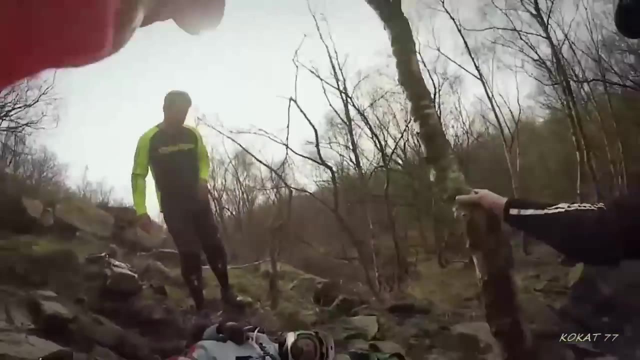 Hiya, you all right. Oh, this is the one where we need the key. Can I just give you that a second Mate Climb over at last. veteran mountain biker Rob Hobson is about to get the help he needs. What's his name, Rob Rob? hello, Rob. my name is Paul. 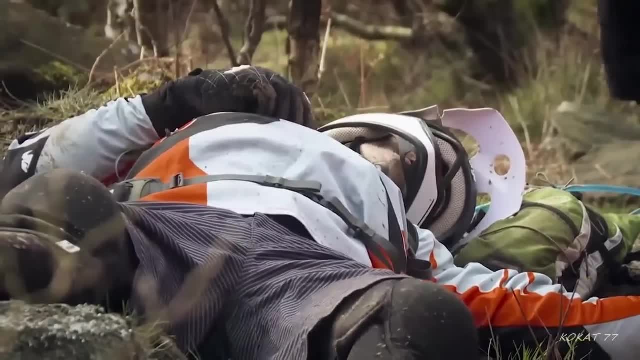 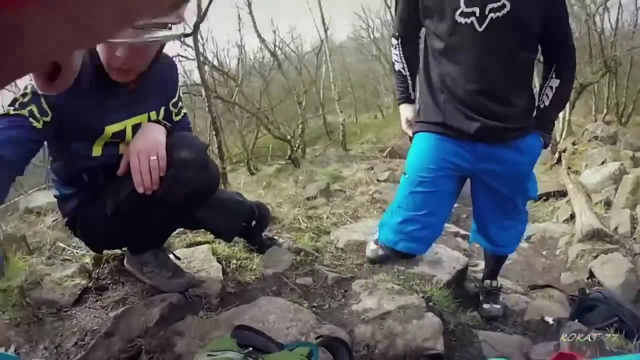 Okay, then it just gripped and then took me over the underbite. Right, okay, just went head first. It's a rock straight on the top of my head. It's impact is, in fact, a lot, right, yeah so, and as soon as I eat that. 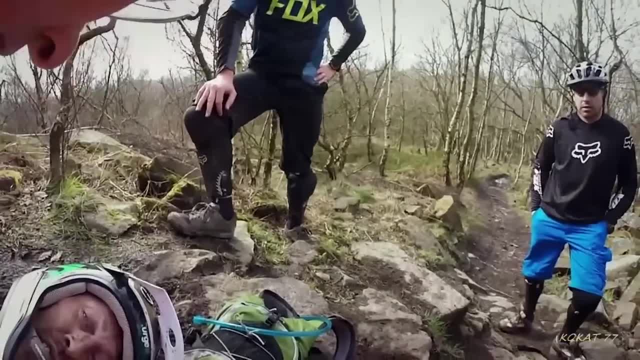 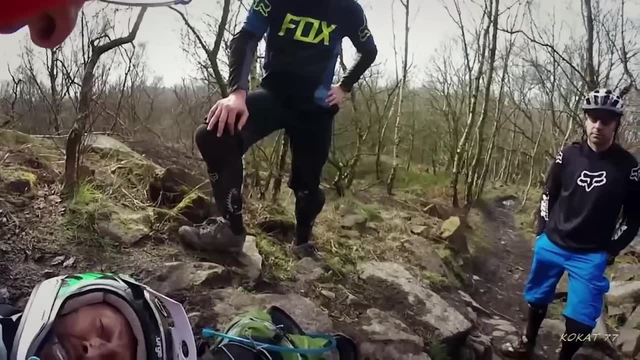 Literally my body went numb from the neck down right. okay, felt like my head was just rolling down the hill. yeah, come, Phil, legs Anything below my neck right, okay. and then now I've been laid here a bit obviously. look, I can wobble my feet, sure. 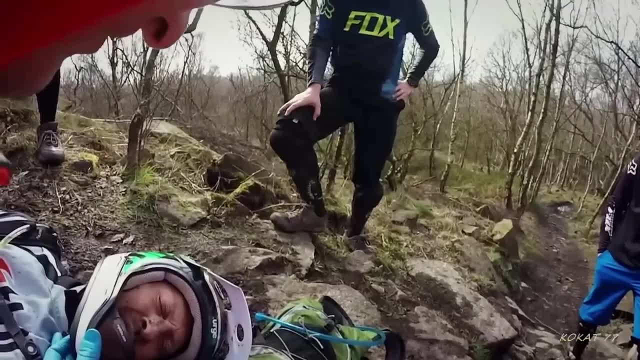 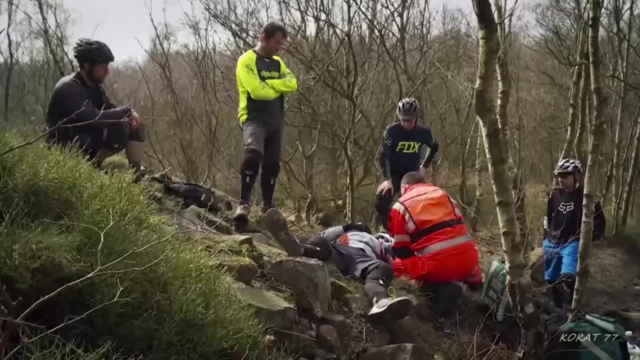 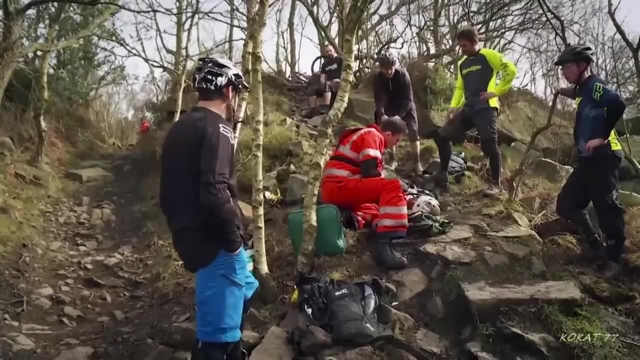 Yeah, and I can start to move them, but I've just got massive pins at burning pins and needles In, like me, shoulders across my chest, This arm right, so is it across the front more than your back, is it? yeah, These arms just feel dead, Rob. symptoms are very serious. 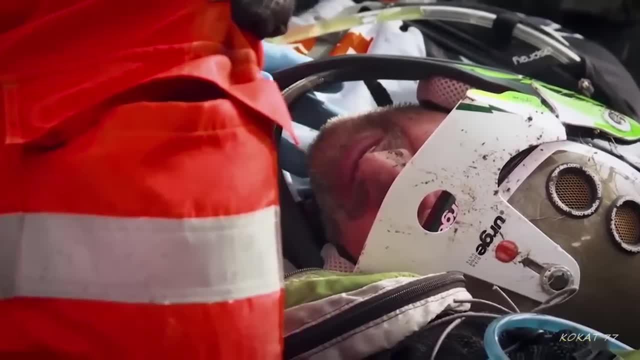 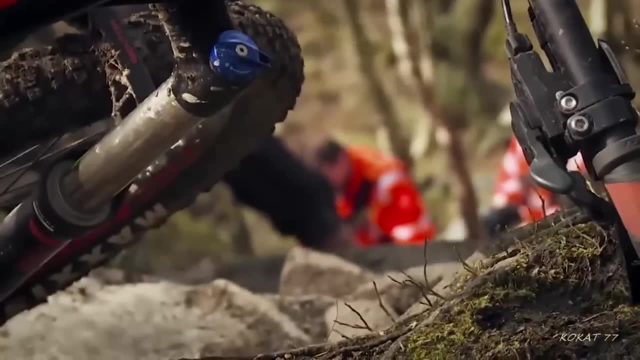 Pins and needles are a classic sign of a spinal cord injury. We'll get your helmet off in a few minutes, well, But I'll give you a quick assessment. mate, obviously your job is to make sure you don't move his head. one wrong movement could kill Their patient. Paul knows the impact could have caused other severe injuries. 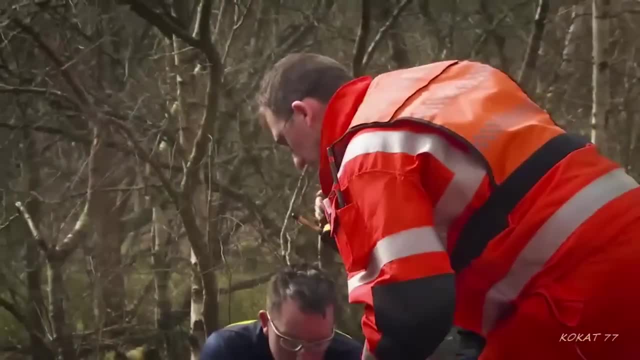 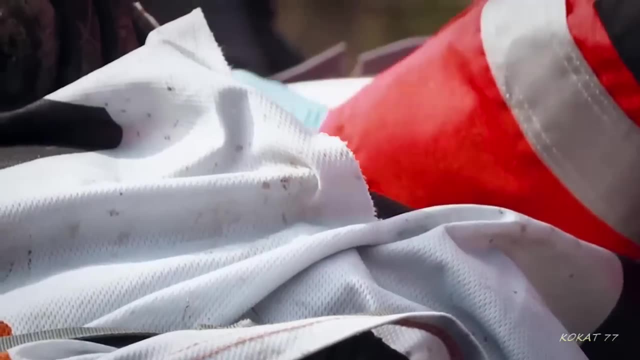 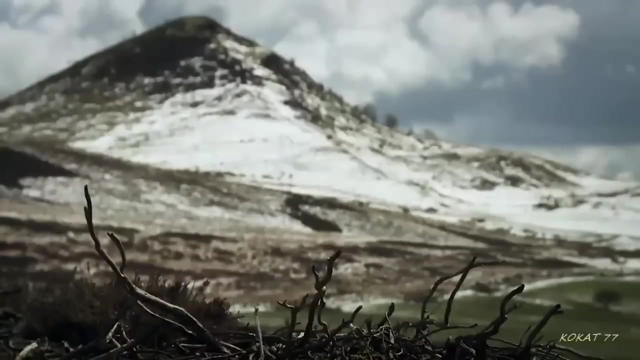 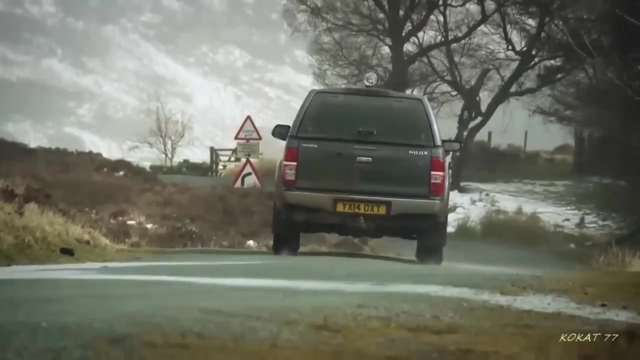 He wants to rule out other problems before dealing with Rob's spine- And the most critical stage in this rescue is about to begin- Paul must remove Rob's helmet and straighten his neck. It's a risky procedure but it's got to be done. It's an old joke, but the Yorkshire Dales really can experience four seasons in one week after a few days of sunshine. 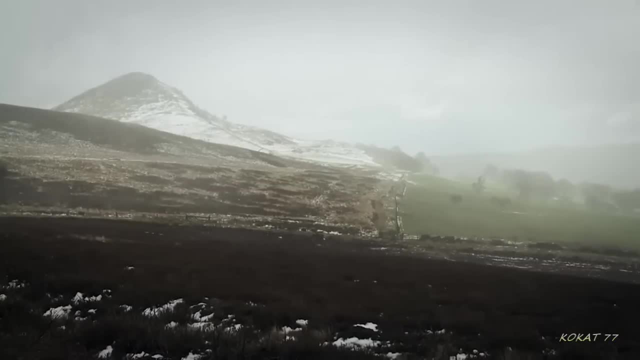 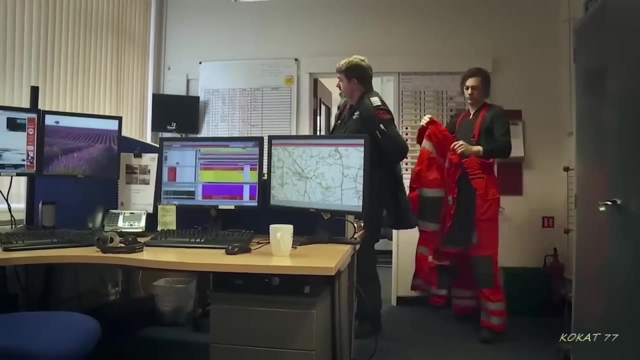 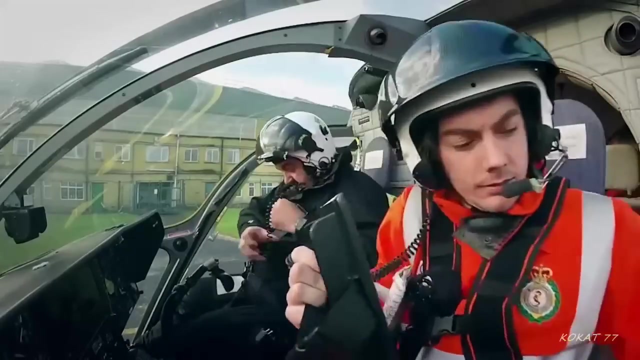 Snow and ice are causing treacherous conditions on the roads. What we got? I'll be back in a minute. Now there's a serious accident. The flight to the outskirts of Harrogate will take 15 minutes from their base in Topcliffe. Topcliffe traffic- can you make 9-1-Alpha engine mode? start down Harrogate. 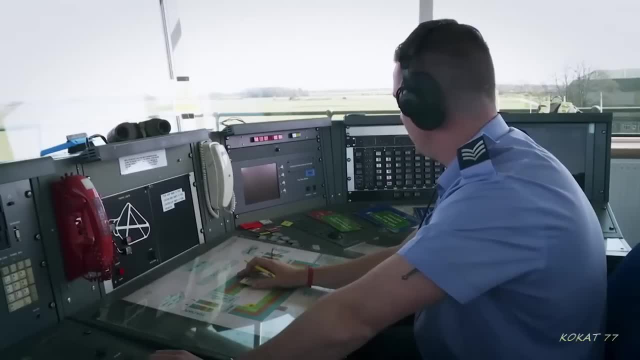 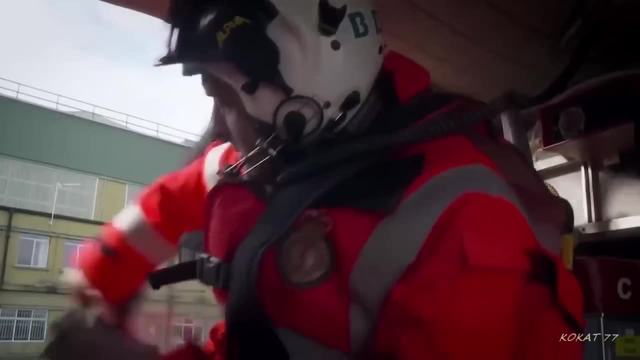 9-1-Alpha take off at your discretion. present position surface with a 2-0-0-1-1 cross on runway 7. Pete Rhodes is the lead paramedic today, with over 20 years experience. He's seen hundreds of car smashes and he knows accidents involving trees are among the most. 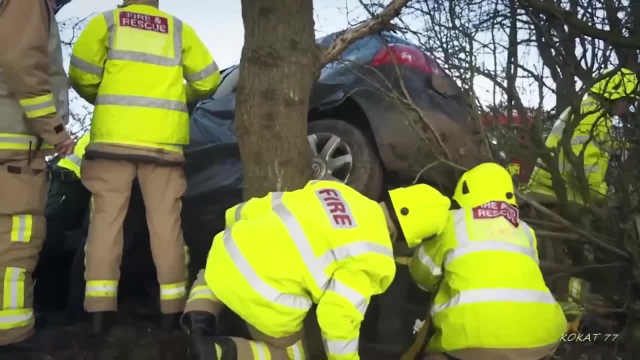 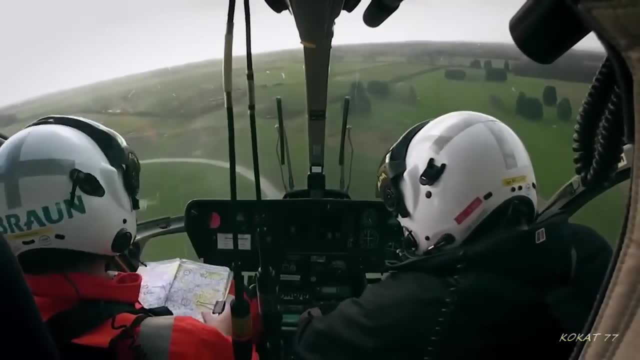 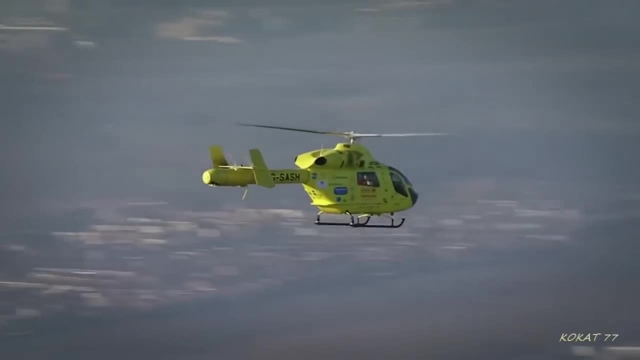 serious Crumple zones and airbags can do little to protect drivers or their passengers. More information is coming through from the emergency services already at the scene. With winds gusting to 40 miles an hour, It's going to be a bumpy ride for pilot Ian Musette, along with his navigator and paramedic Leon Baranowski. 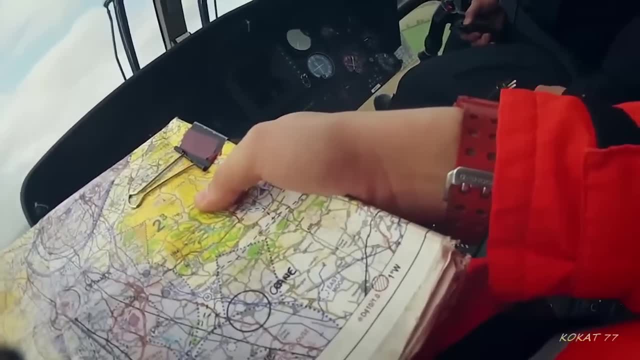 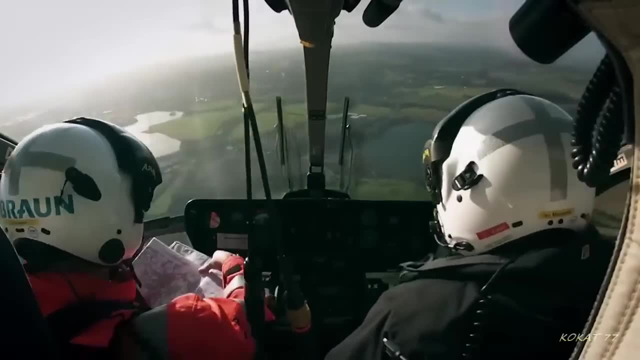 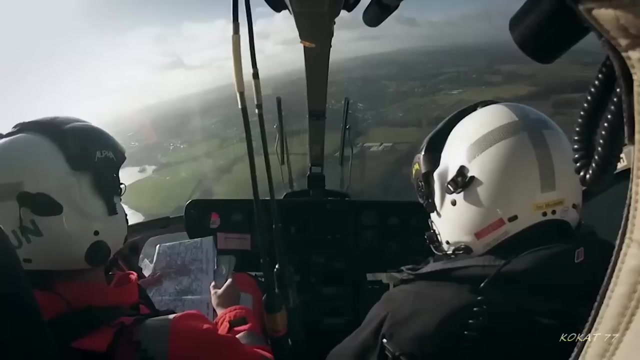 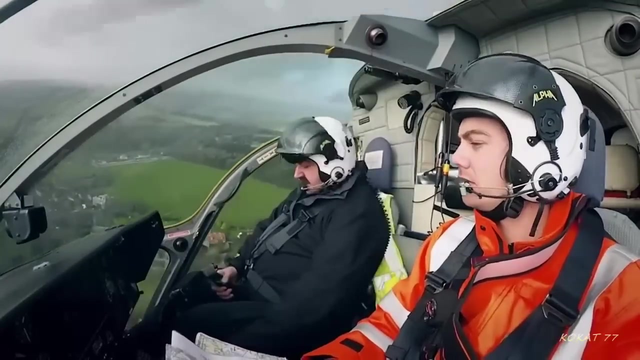 I'm trying to get the right amount of pebbly and we're flying a little bit out of balance. at the moment The aircraft is getting buffeted from side to side. Ian's working hard to keep it on an even keel. Landing can be the most difficult part of the flight. 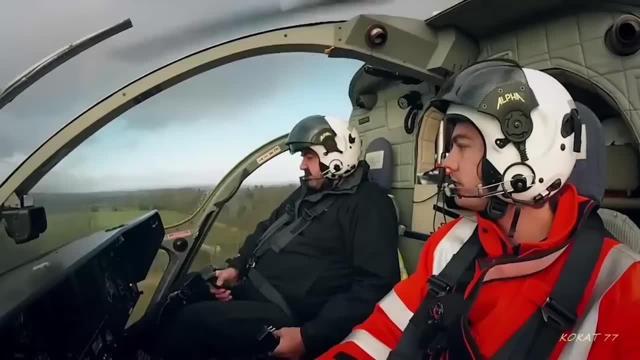 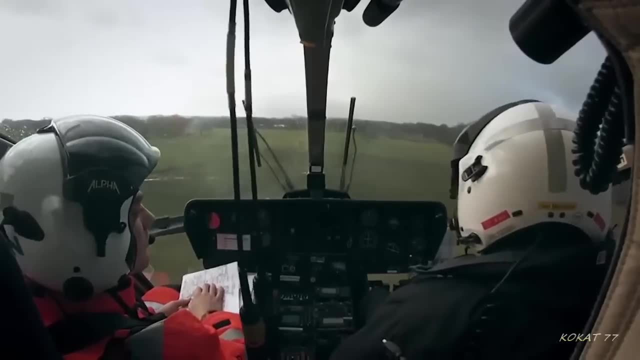 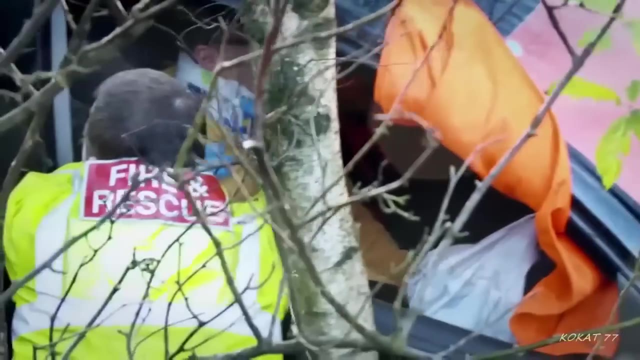 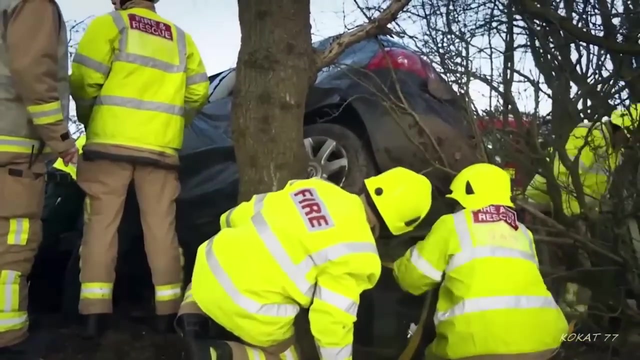 Even without high winds. as they approach the accident scene, extreme precision will be required to get the air ambulance down safely. The driver and passenger are injured and trapped, but with the car in such a precarious position, Firefighters must secure it before the patients can be taken out of the wreckage. 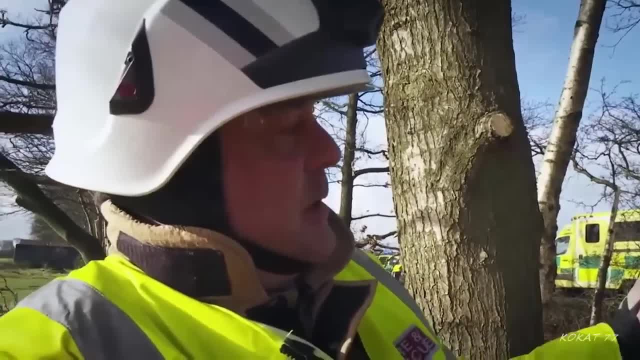 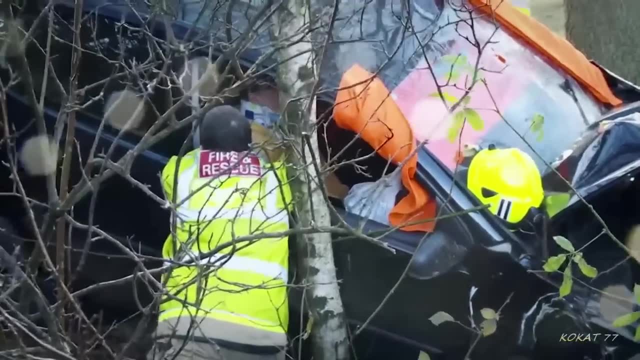 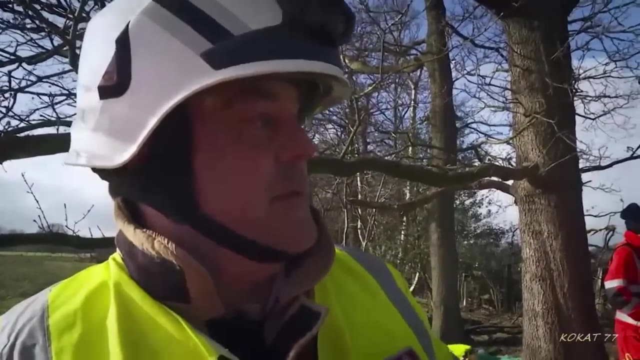 It's come off the road at speed and it's managed to trap itself between some Hedge row and trees and things, so access is quite difficult. We've also got a ditch full of water, So access is quite an issue at the moment. We've got plenty of personnel on site: crews from ambulance and from fire service. 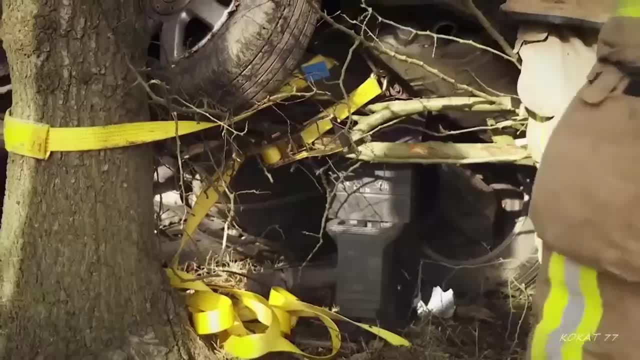 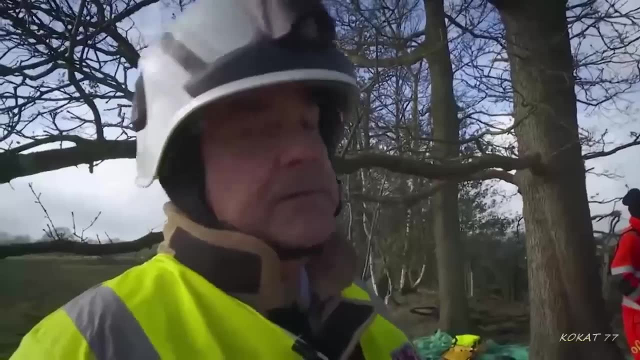 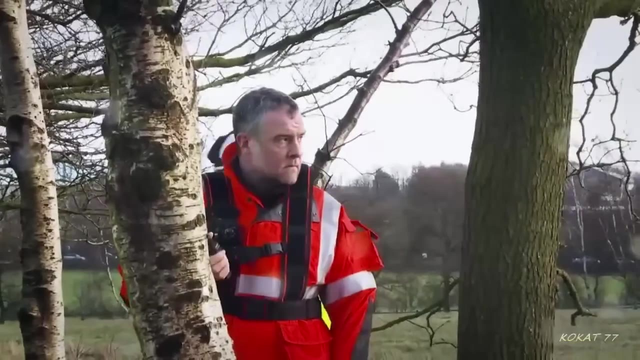 Making sure all the times that this vehicle is stable because it's a part in the air. So we we've also attached it to the trees that using some of our straps To maintain that stability for the casualty and also for the crew. safe With the car, secure the firefighters. priority is to get the passenger, who's called Natalia, safely out. 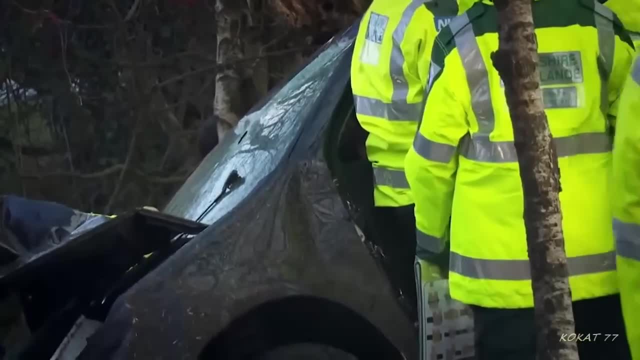 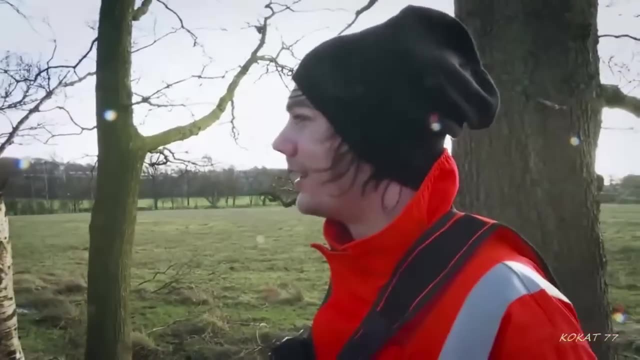 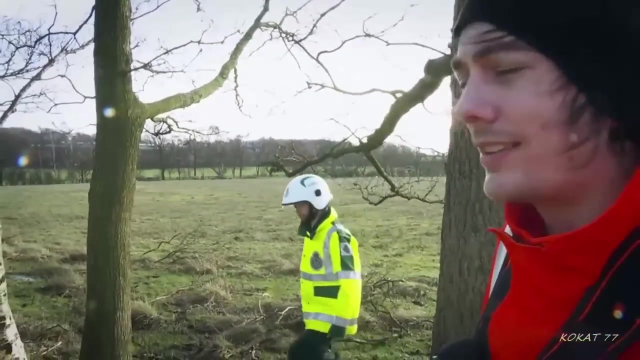 Pete suspects that both she and boyfriend Martin may have spinal injuries. this must be a delicate procedure. Looking at the what could have happened? car versus trees at you know 40 kmph, it looks like they've probably been relatively quite lucky, Both Natalia and Martin. 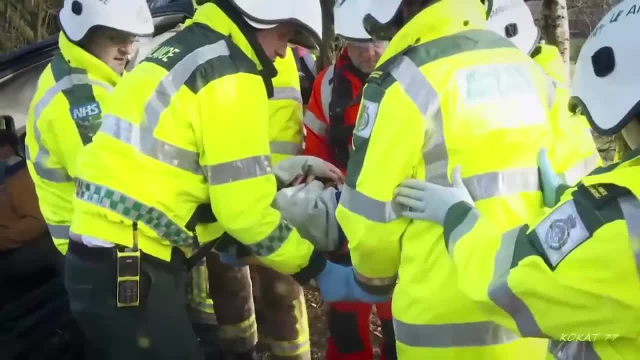 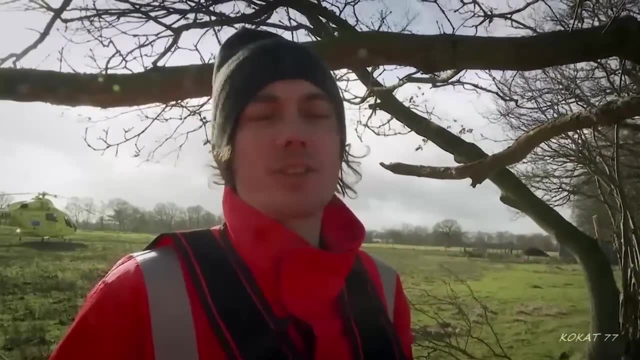 are Polish. English is a second language. Language difficulties can cause quite a few problems when you're trying to assess patients In trauma, though it's relatively easy, because you can usually see where the problem is, or at least find easily where the problem. 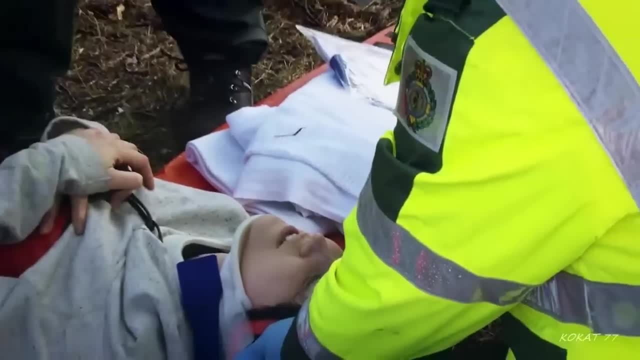 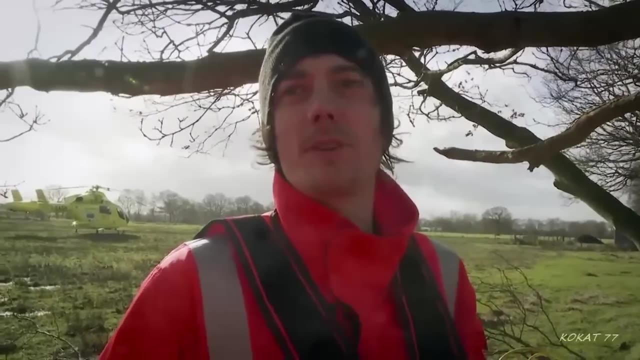 is In medical patients, it takes a little bit more. in terms of investigative questioning, then it's a lot harder to do. The ambulance service does have a set-up for that. We can use an interpreter through a language line, but the process of getting all of that in 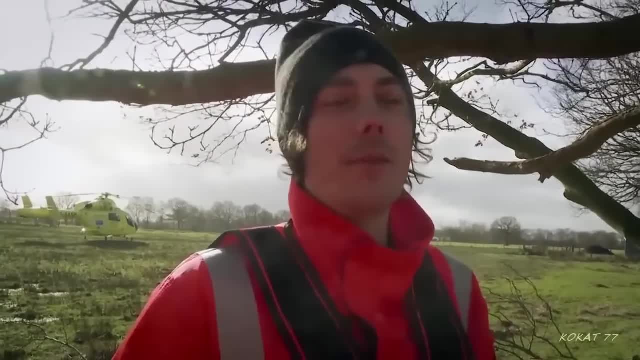 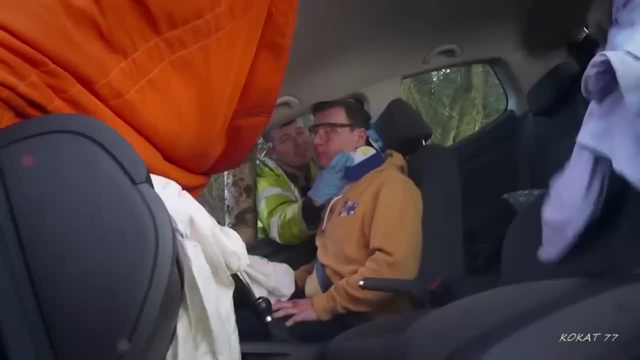 place whilst on scene can be quite lengthy at times. So usually we do our best and muddle on through and just go with the stock words and the stock hand signs. Stay still, Martin, Martin, Martin, Nice, and still for me, my friend, We've got a blanket coming over to keep. 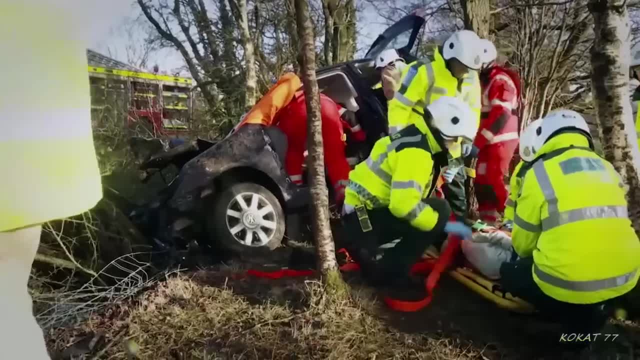 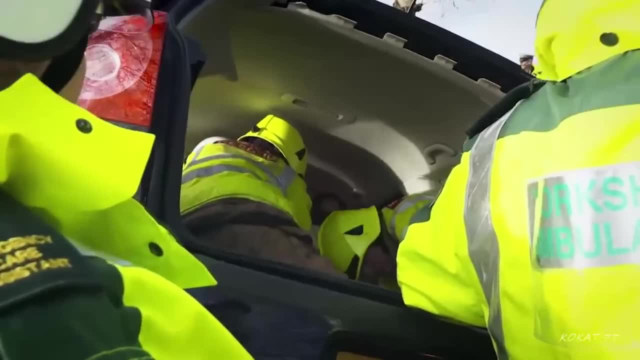 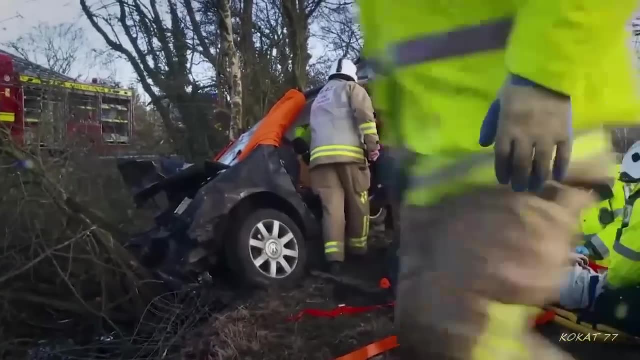 you warm now, Like Natalia, Martin needs to be brought out of the car horizontally to avoid damaging his spine. The high winds mean that, for once, both casualties will have a smoother ride. going to hospital by road. That seat will fall down with a pull-up. That boot's going to get unbolted. He will literally. 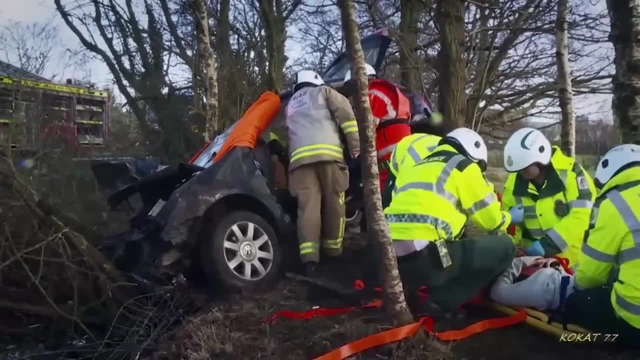 go straight out of there if you want him to. Everything is geared up. Look at the space of the back. If you're happy, we'll go with it. I'll just show you now. Hey, that's my big one, Big one. 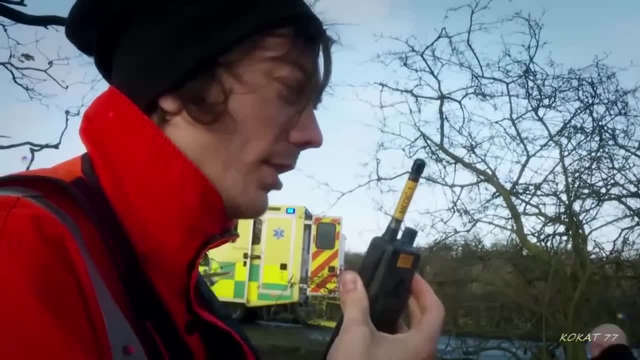 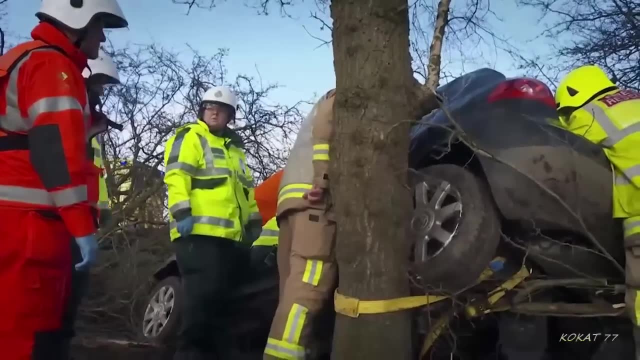 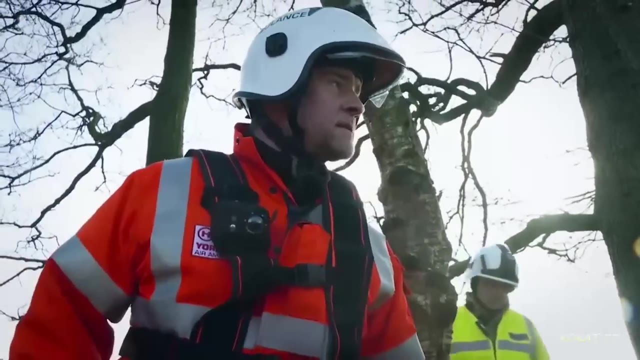 All patients are going to be going my road to Harrogate, so we're not going to be conveying anyone. As Natalia is taken to the ambulance, the tricky procedure of getting Martin onto a spinal stretcher is underway. Could you get us another extrication board, please, mate? It would be easier to slide. 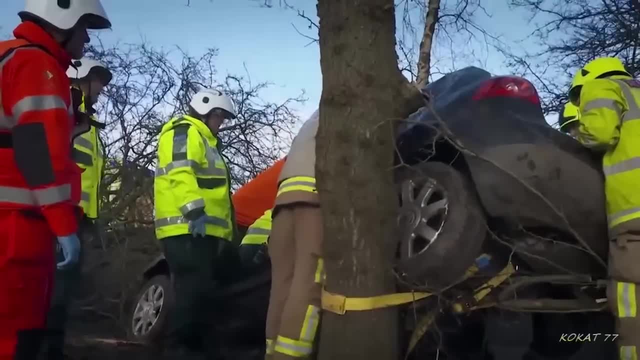 him out than that, If Pete's suspicions of a spinal injury are correct, one false move at this stage could leave the patient paralysed. You've got to trust us. Yeah, you've got to relax and trust us. We've practised this. 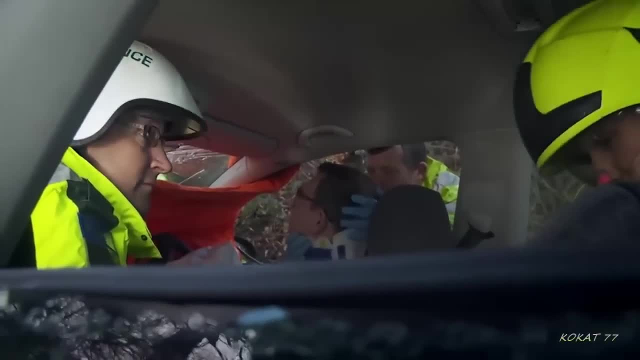 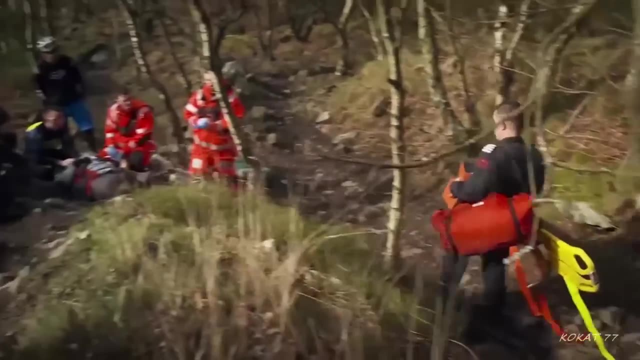 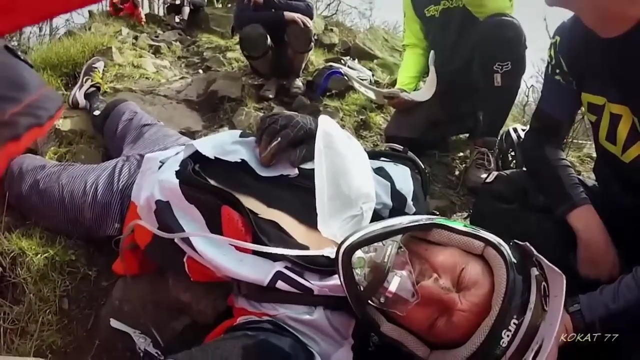 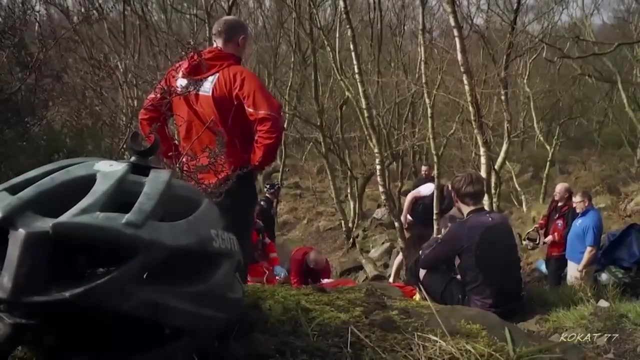 a lot OK. Deep in the woods on the edge of the Peak District, 49-year-old mountain biker Rob Hobson is lying critically injured. His neck is feared broken. I just heard quite a loud noise going down the slope. Yeah, I just went to see if he. 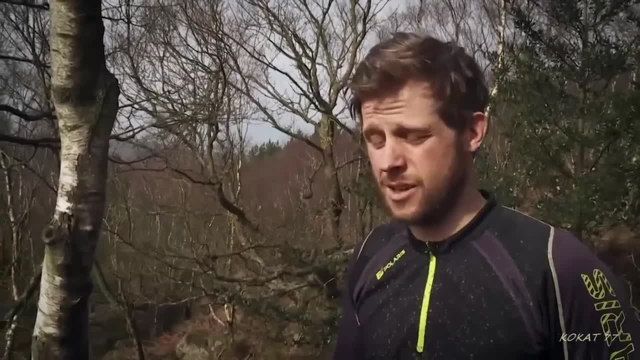 was OK and he was complaining that he kind of couldn't feel his arms and his legs. so obviously quite serious. so I just called the ambulance. Are you comfortable? as best as you can be, Because I don't want to move you, just because. 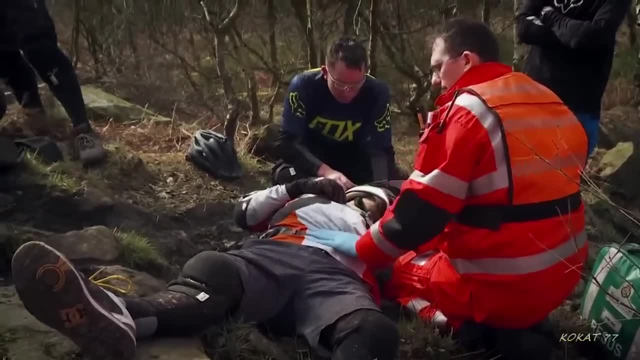 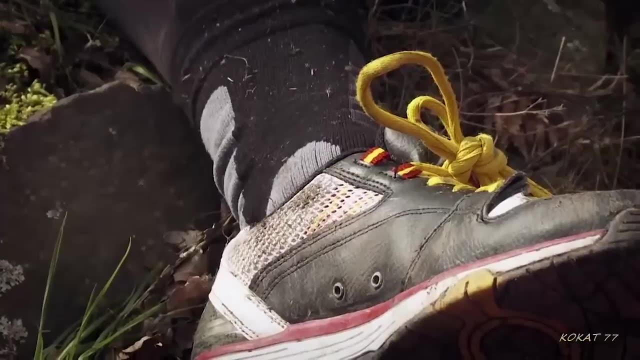 there's a rock just at the minute. There's no pain in your stomach, is there? He thought he couldn't feel his legs or anything like that, but we saw him moving his legs. We just tried to calm him down. really He kept sort of saying: it's bad, mate, it's. 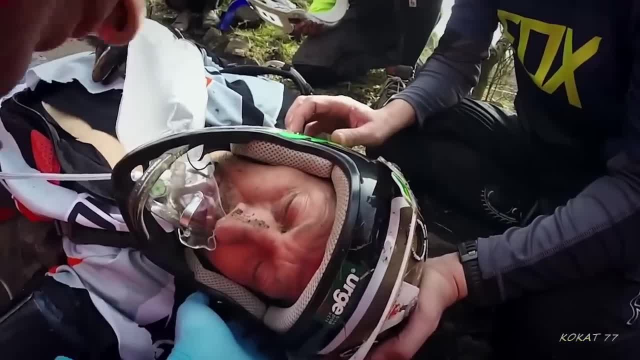 bad. It's a bit of a worry. In a few minutes, once we've just done your blood pressure, Rob, we're going to sort you out, mate. All right, how old are you? It was a consensus talk earlier on. 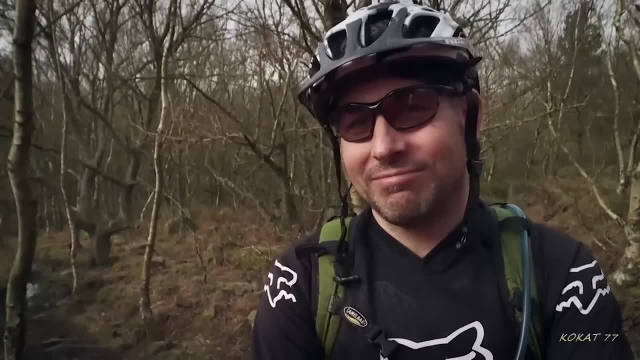 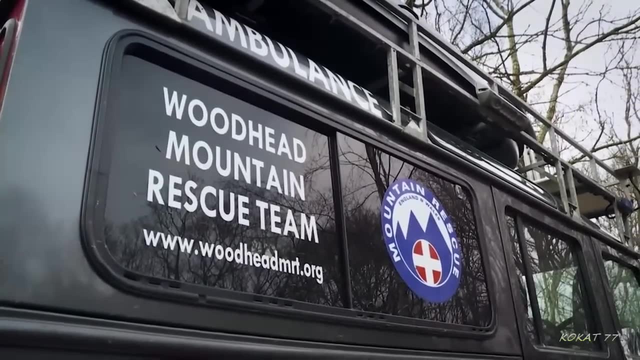 All right, We're not going to do anything too silly, and you know it happens. Paul and James are going to need help from Mountain Rescue to move their patient. MRT are about five minutes off. OK, yeah, yeah. 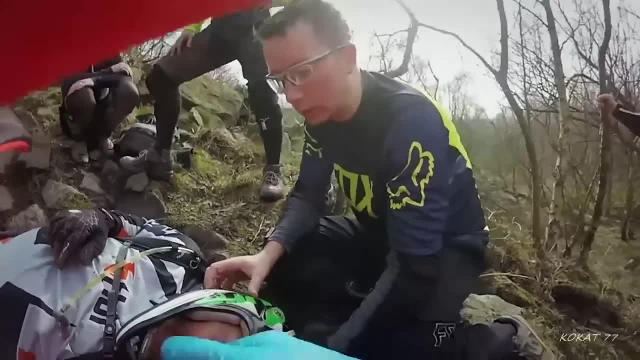 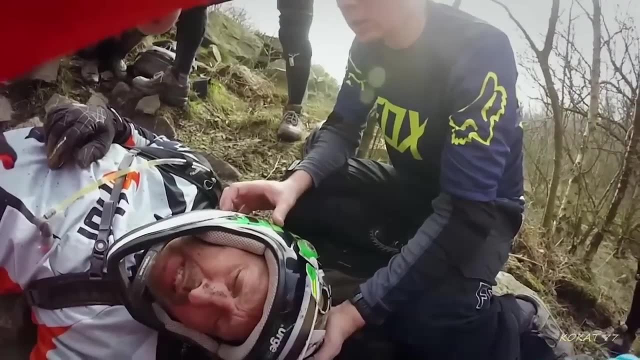 I'm just giving him a grip now. That's fine. What we're going to do then? obviously, because we don't know what's happened to your neck particularly, and because you've got this loss of sensation, numbness and what have. 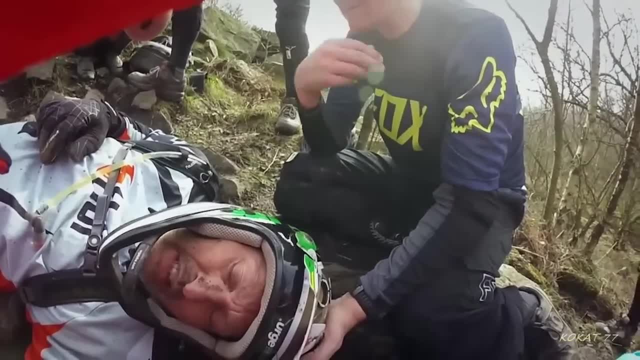 you. as you're probably already thinking, we're going to treat you for worst-case scenario. Yeah, I'll carry on physically and just give you a quick once-over. Just make sure we're not missing anything. Yeah, OK, mate. 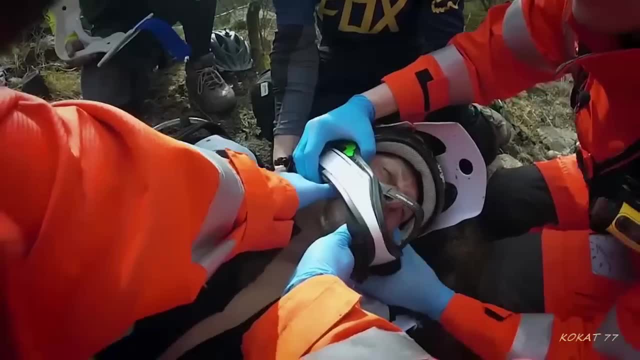 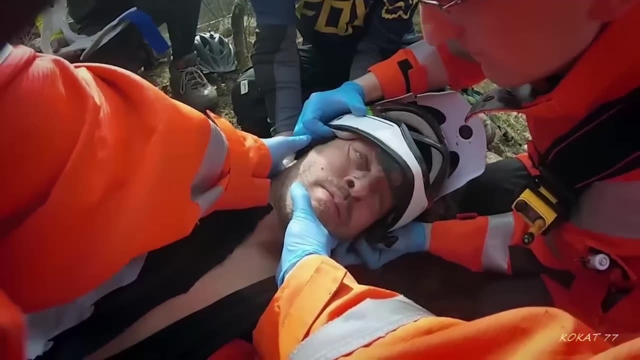 We don't want you to do anything, But if you get any pain, shout us. Yeah, Are you ready, mate? Paramedic Paul must now remove Rob's helmet. A mistake now could kill their patient. James is holding Rob's head rigid, but the next stage is even more critical. 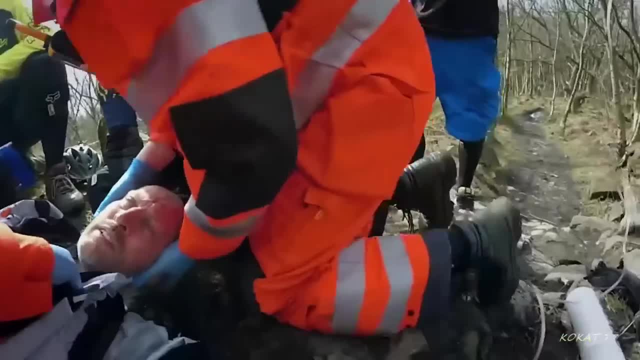 Right, Rob, We're going to have to straighten your neck slightly. There's no C-Span tenders. Which way? We're going to go to your, To your right. So you're looking to your right, So I'll do it. 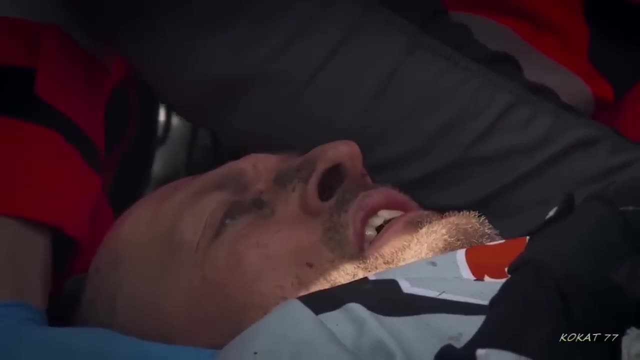 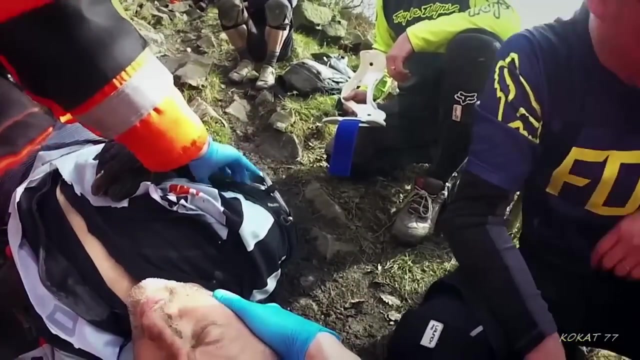 Look towards Al. Straightening Rob's neck is necessary but fraught with danger. Use your head, nice, and still You can let go now, mate. Thanks, Nice and slow. Can you move that right arm, boss? How's that? 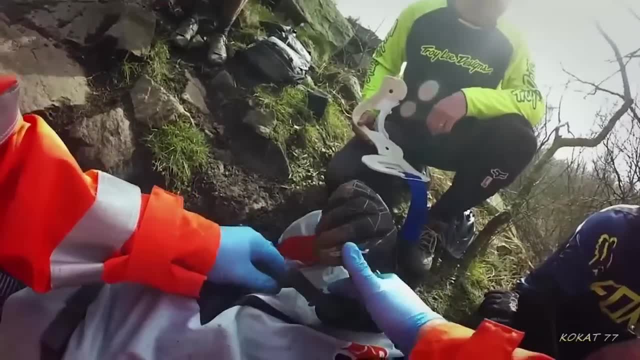 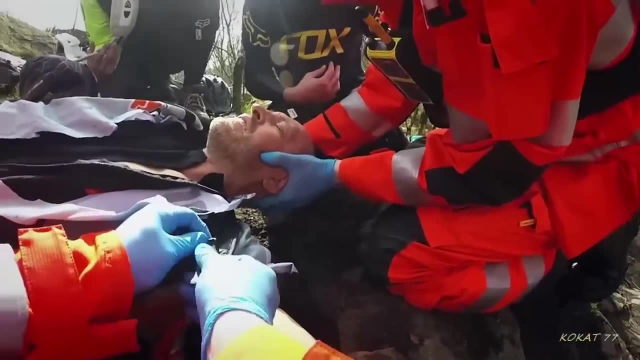 Limited movement. Oh, Rob's life is in the team's hands. Yeah, So you've still got no pain in your neck. No, Fantastic Slow. You're being nice and steady. You're doing really well there, Bob. I know it's uncomfortable, mate. 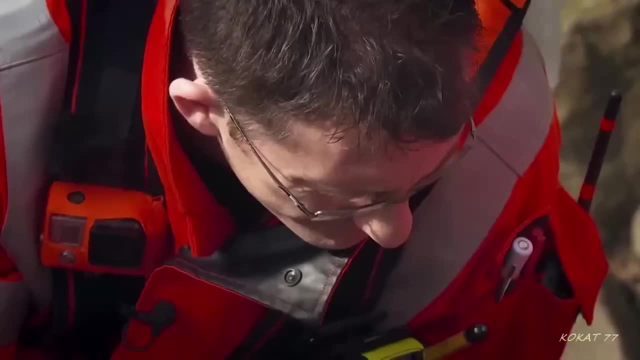 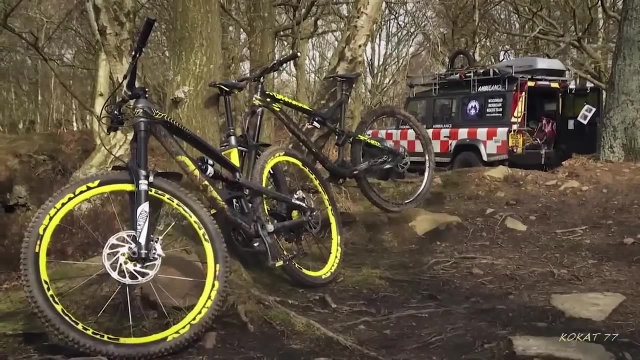 Yeah, All right, And I know it's quite scary. No, Last It's done. Now they can protect Rob's neck with a surgical collar. A mountain rescue team has arrived. How are you mate? You all right, Just going to be from your guys' point of view. 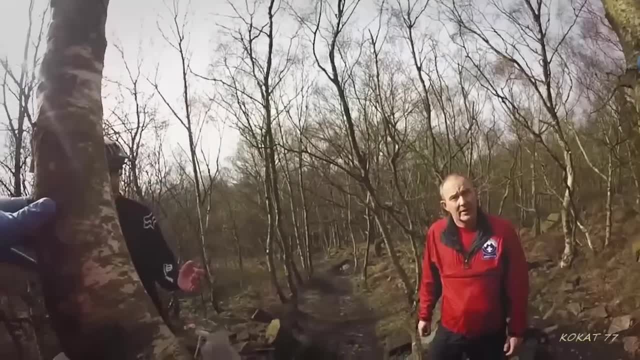 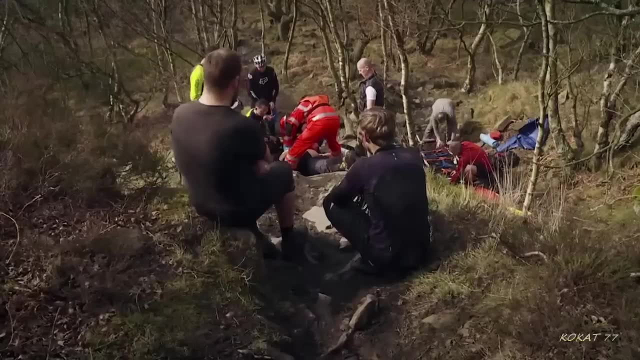 Some hands when we're transferring, but probably just a belt stretcher just to get him back up to aircraft. Right, We've got plenty of hands here, It's fine, But getting Rob to the chopper won't be easy. He's come off on a very steep track. 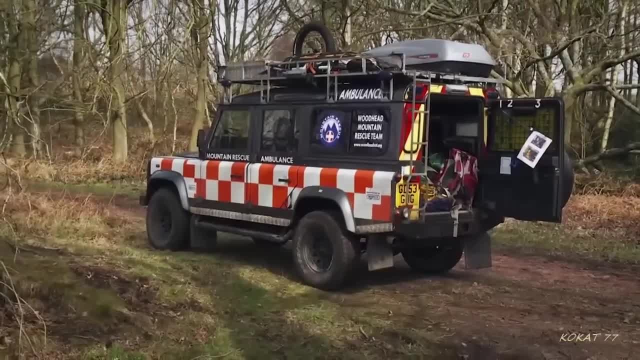 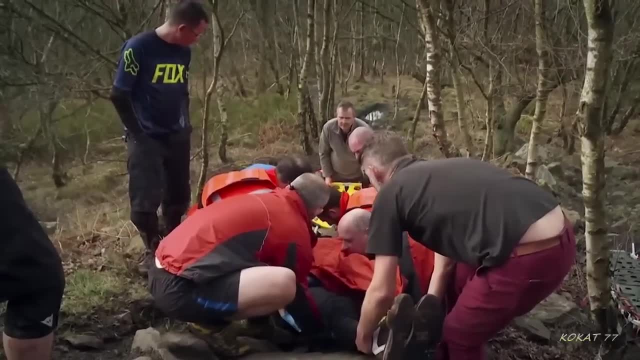 Mountain rescue are going to provide the manpower the team needs. If we're all set, This is going to be uncomfortable, Rob, Yeah, Ready to lift, Yeah, Ready And lift. That's good, That's all good And we're there. 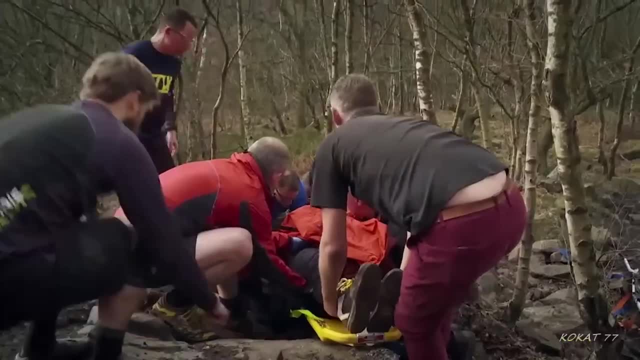 That's good enough, And there I call it: Ready to lower? Yeah And lower, We'll get your head up in a minute, boss, as well. No, no, We've just scooped him up now. Mountain rescue are just getting him out on one of their stretchers. 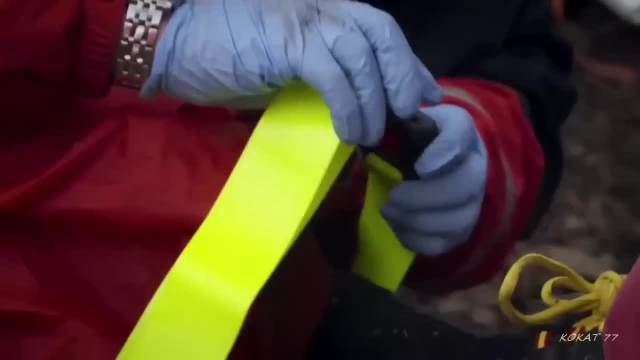 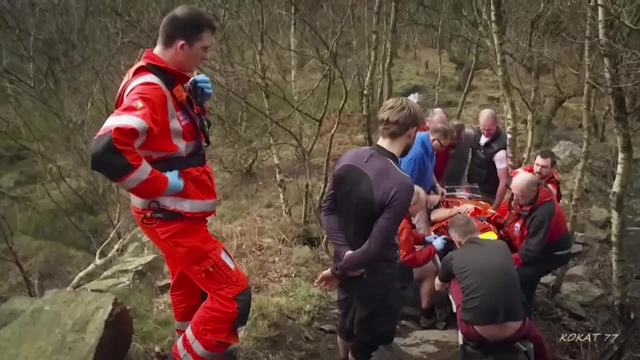 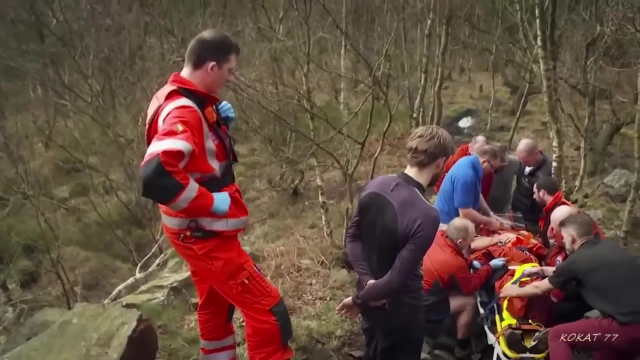 To be honest, we've got plenty of hands. actually, I'll leave the lock for the gate on it, but I'll not lock it So that they can access out of it. Yeah, That's great. Thanks, Leslie. Thanks for your help, Duke. 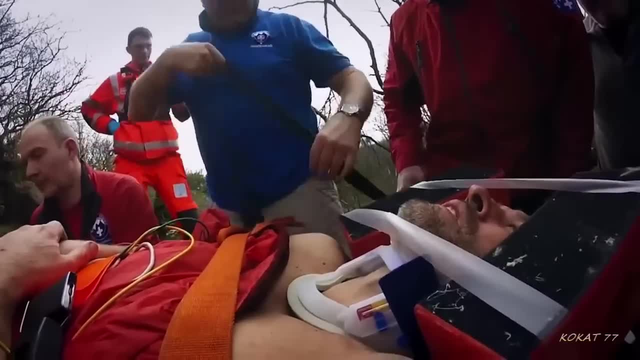 These guys are now going to carry up this track. We're going to get you to the aircraft, Then we're going to fly you to Sheffield, So it's only going to be the shortest flight on record, probably. Yeah, All right. 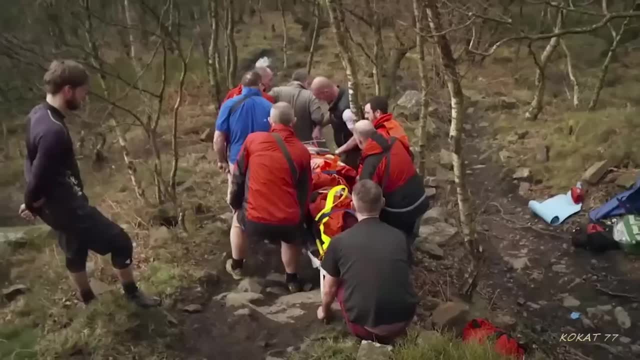 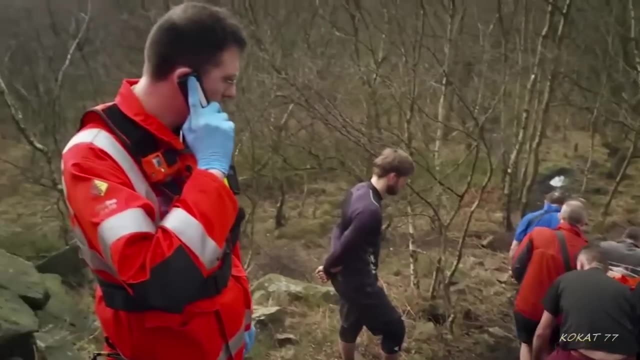 But we'll get you there smoothly at least. All right, mate, All right, It's helmet 98.. We've got a trauma call Feed up, please. It's less than two hours since Rob arrived in the woods on a day trip from his home in. 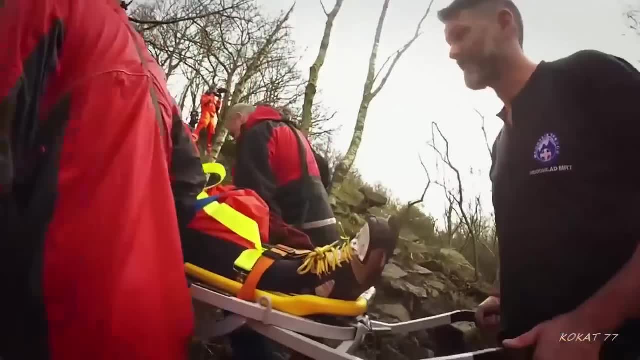 Lincoln. Now he's on his way to a lengthy stay in hospital. Yeah, Yeah, Yeah, Hi, It's Paul on the paramedics of the air ambulance Called a 49-year-old male. He's come down quite a distance along a rocky path on his bike. 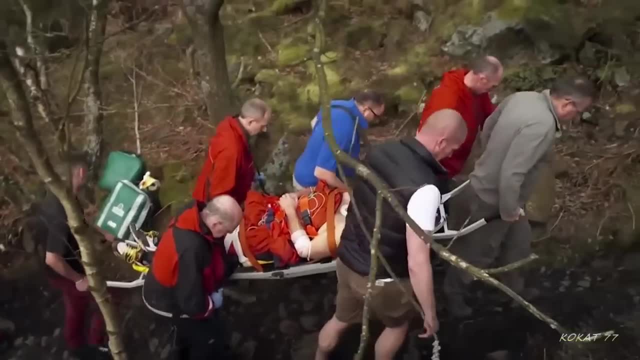 He's come over the handlebars and landed head first onto a rock. Even for the seasoned mountain rescue team, it's been a tricky operation. Well, it just demonstrates how difficult it is. Even though it's a short distance, it's quite difficult, especially with the underground. 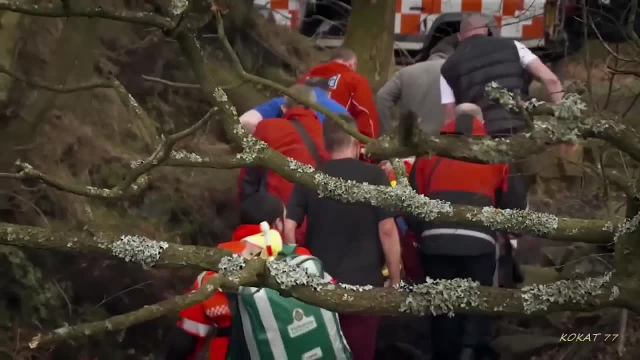 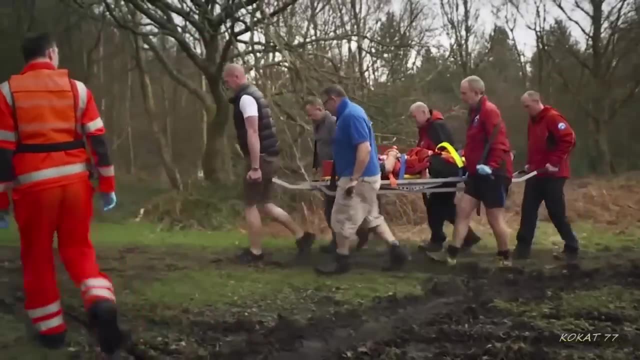 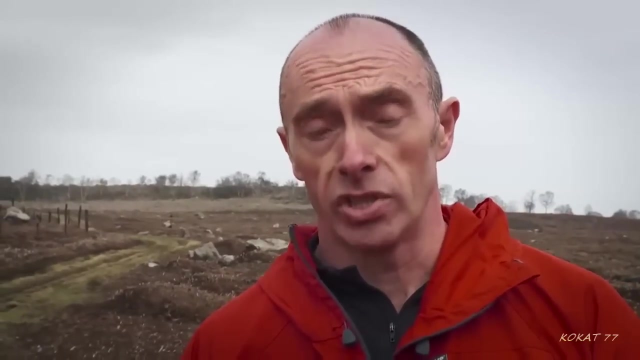 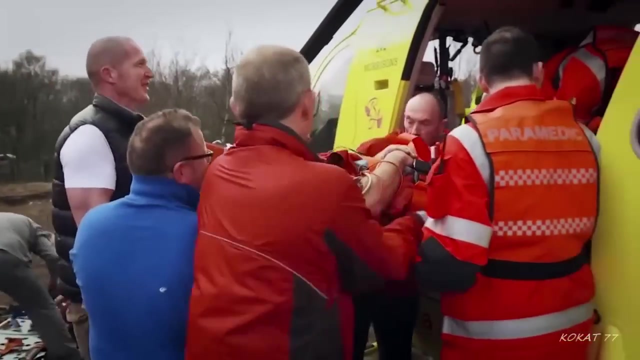 conditions and the kind of injury the chap had as well. I'd like to thank the crew and the team of the team for their support. Thank you, We need to go feet first. Accidents in Warncliffe Woods are common, but they're rarely this serious or this far off the beaten track. 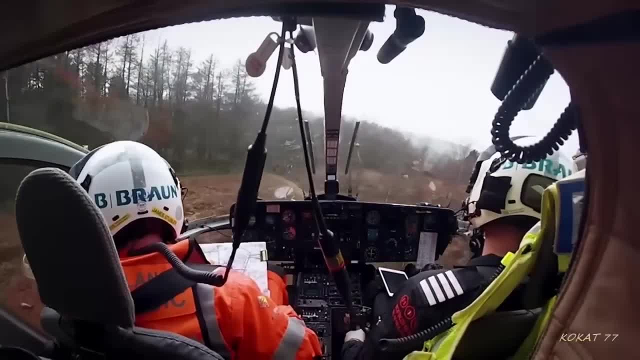 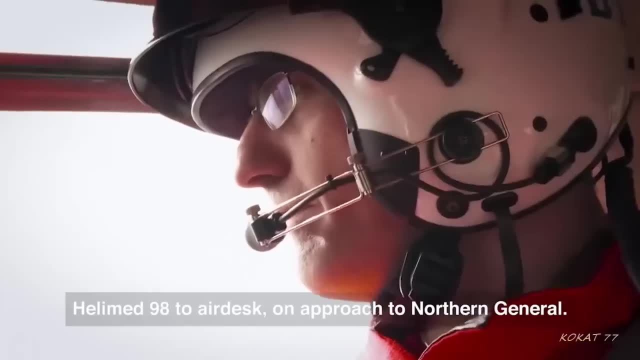 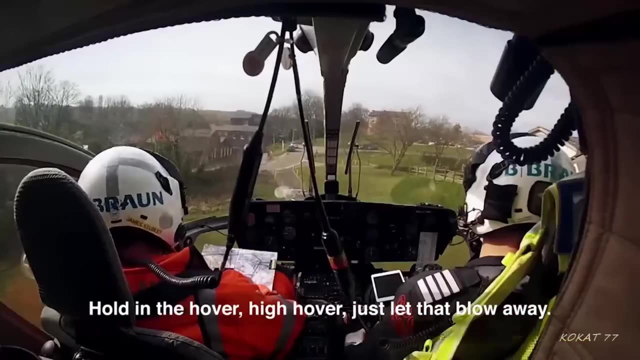 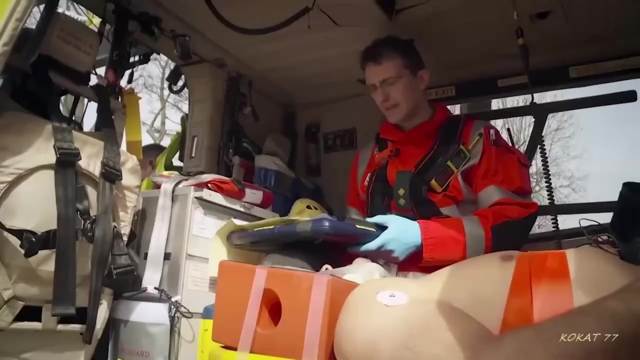 The team's flying rob direct to the Sheffield Northern General Hospital ten miles away. It's the regional trauma unit MN 982, NS Skirp on approach Northern General. Thank you, DC. How's that feeling? Is it coming back? 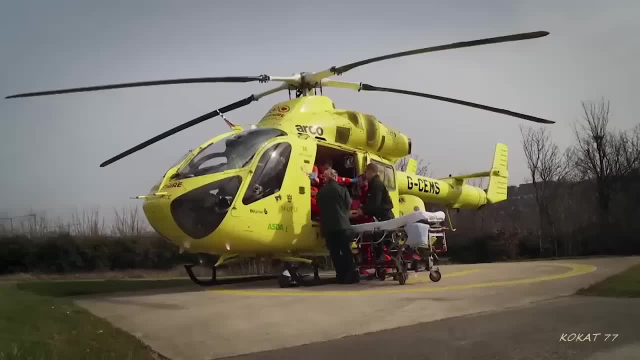 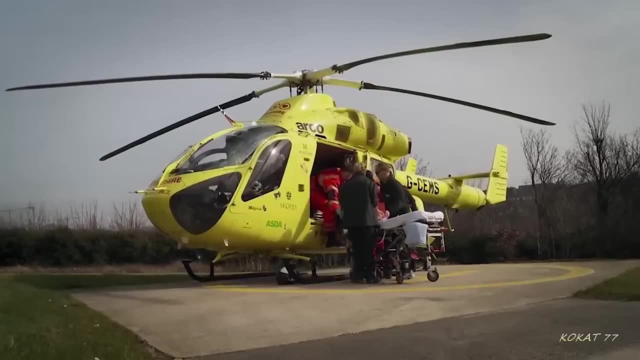 A little bit, but it just really burns in my elbows and shoulders. The team know the outlook for their patient could be bleak. Rob's about to undergo CT scans and X-rays to determine the extent of his spinal injury. It's quite a significant mechanism of injury. 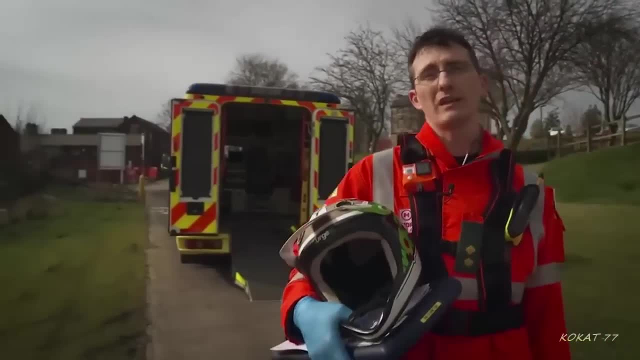 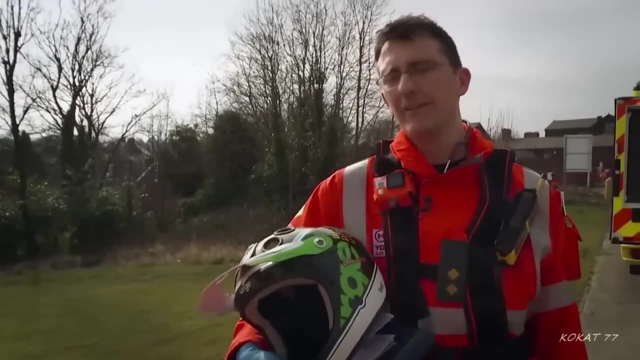 so it's ideal really for the hospital staff to be able to see what's happened on the external side so they can get an idea about what's happened internally. It's good to road traffic and generally it's quite good for them to take the helmet. 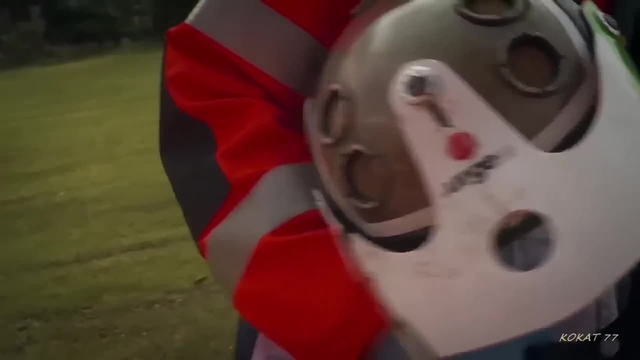 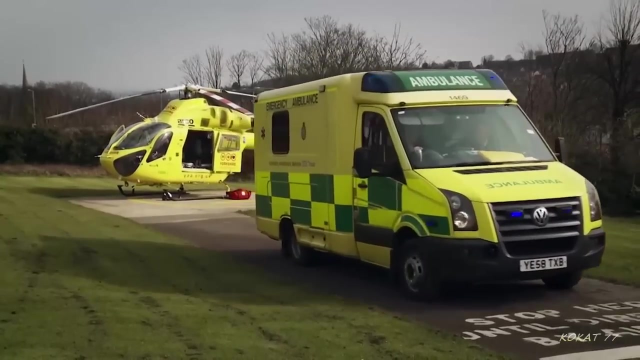 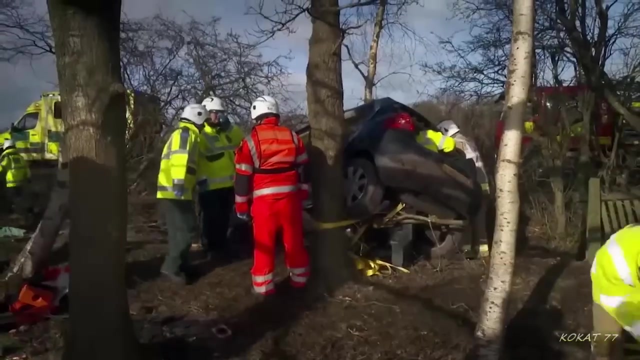 Although obviously, as you can see from the top of the helmet, there's not a lot of damage, it doesn't necessarily mean there hasn't been quite a big impact. The next few hours could change his life forever. On the outskirts of Harrogate, paramedic Pete and the fire crew 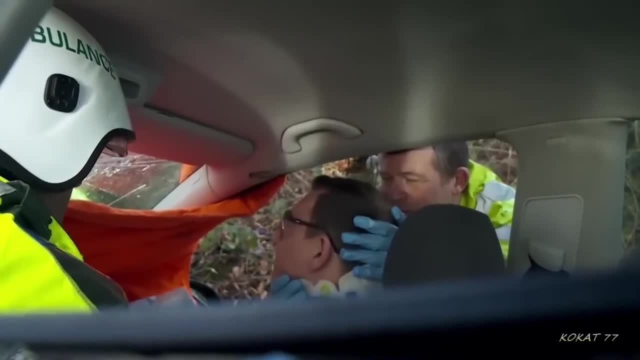 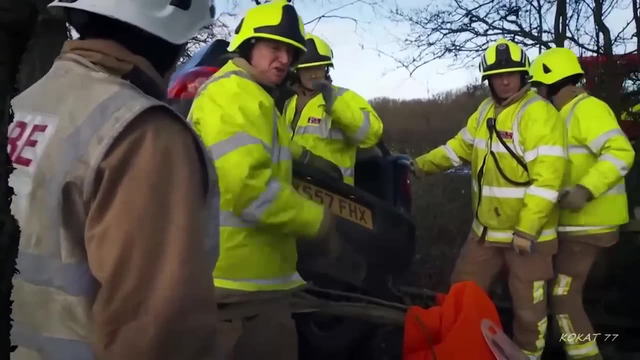 are attempting to safely extract an injured driver from his wrecked car. He left the road and ploughed into some trees. The team suspect a spinal injury. For your information, we're just going to take the back seats out now. All right, Martin. 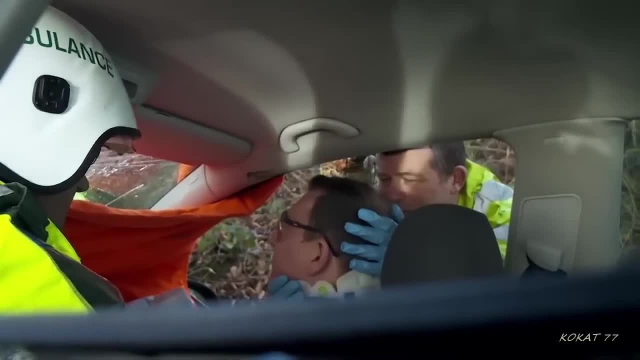 So there's going to be a little bit of noise and banging behind you, but it's all something that we have to do. OK, Fire up and talk Steve. Yeah, we'll be talking to him later. All right, Have a good day. 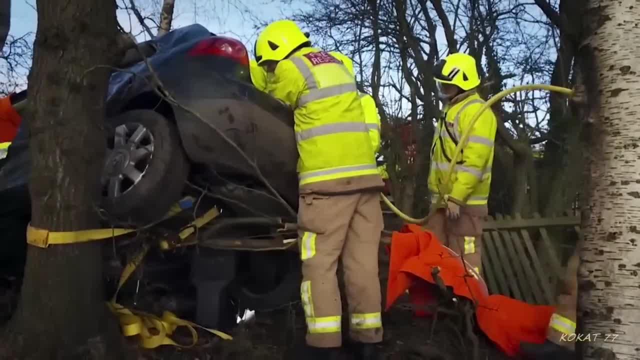 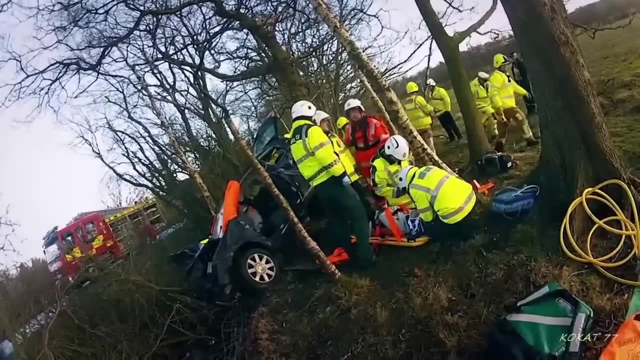 Have a good day. Have a good day. We must get him on a spinal board and bring him out horizontally to avoid further injury. But there's a tree wedged against his door, so the safest way out is backwards. We've removed the door from the passenger side. 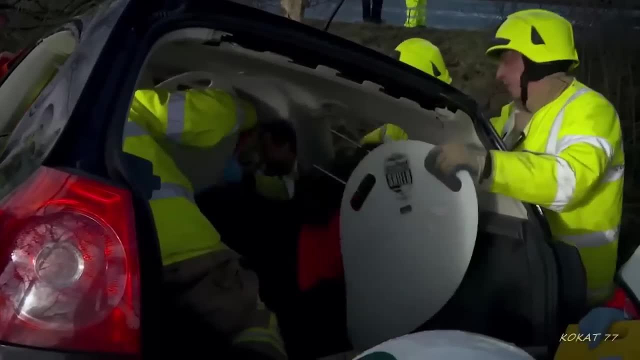 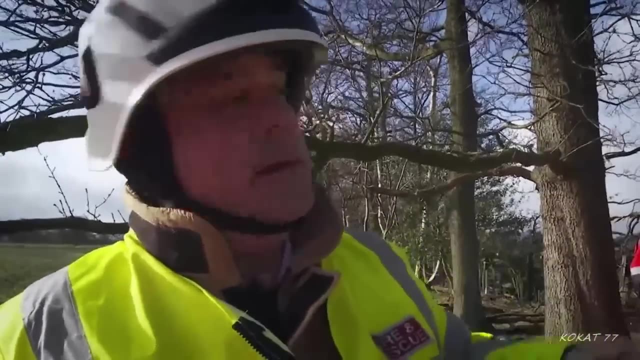 We've also removed the tailgate. What we're intending to do now is- now we've removed the back seats- is to lower the seat for the driver and then stretch the casualty out the back. OK, guys, you can lower it. 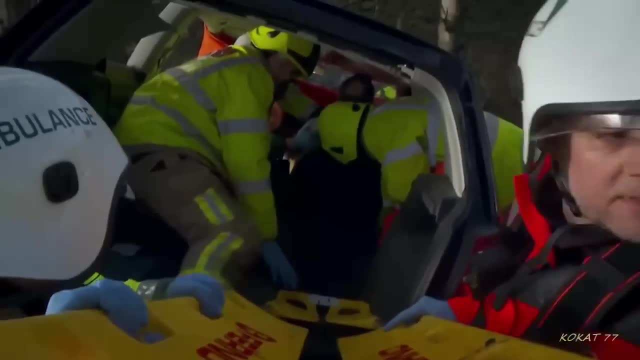 Can we get two of you guys just sort of at our shoulders to get the head in? We'll bring him down. Some of that's OK. Yeah, we're happy. This is going to be a delicate operation. The bridge is going to be quite awkward. 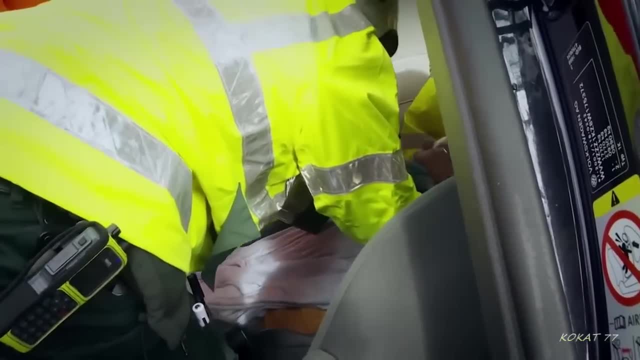 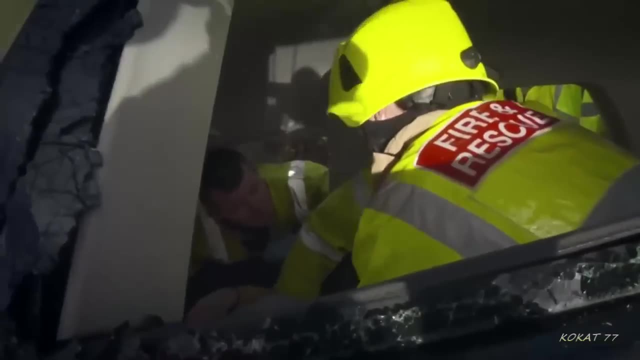 Yeah, See how far back they can get in. He's lying down now. I don't think his feet are in traps. That's it. Good man, Martin, You're doing really well Right. Leave, Martin, now we're friends. 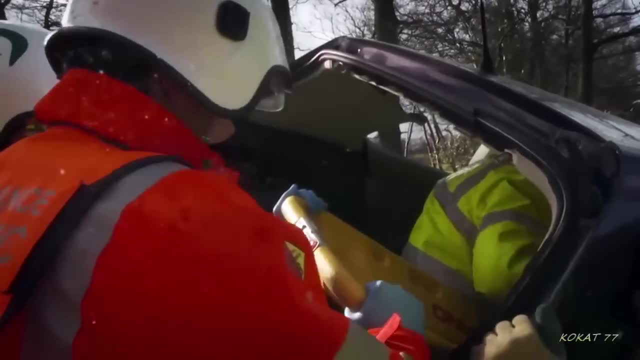 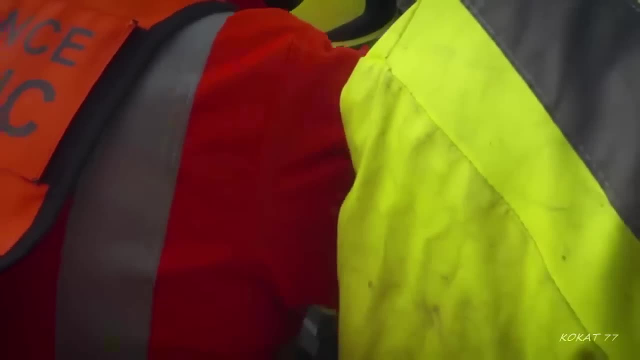 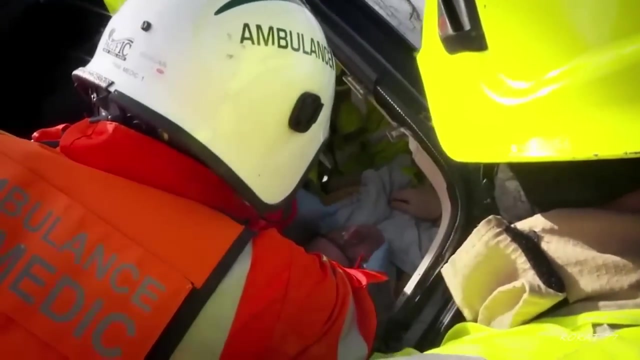 We're going to grab onto your legs. OK Yeah, One, two, three slide. Rest Same again: One slide. One, two, three slide. This procedure is slow and careful. Careful for good reason. If Martin has damaged his spine, any sudden jolts? 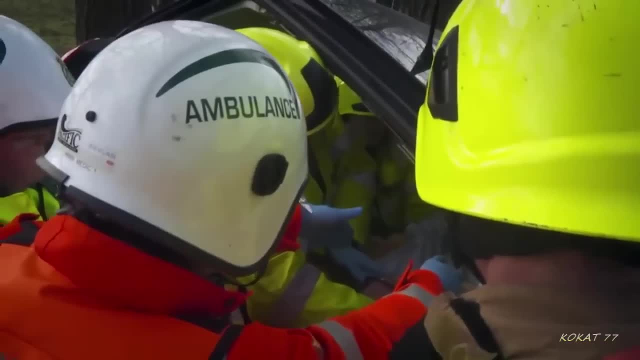 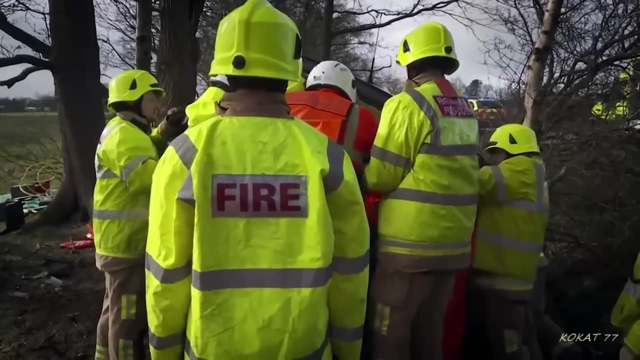 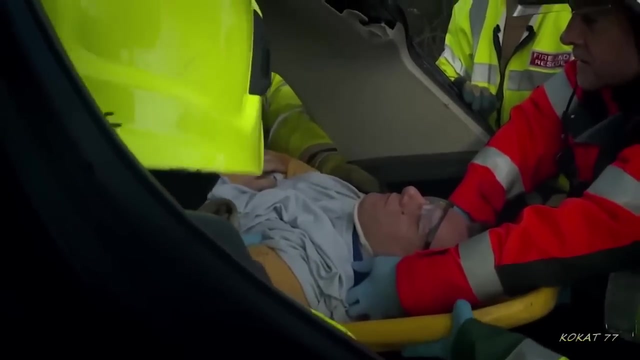 could cause permanent damage and paralysis. Rest there, It's right elbow, or just a jar of the plastic Going to carry on with slide, OK, One, two, three slide, OK, That's it. OK, One more, Everybody ready. 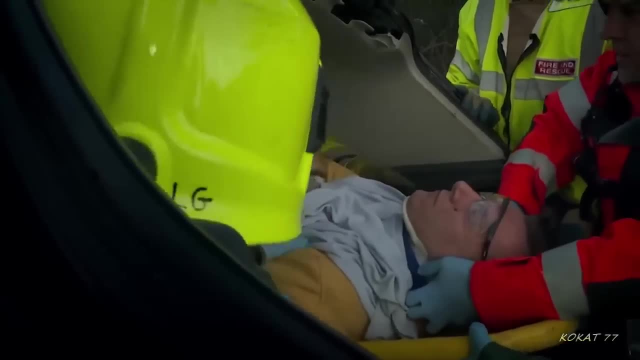 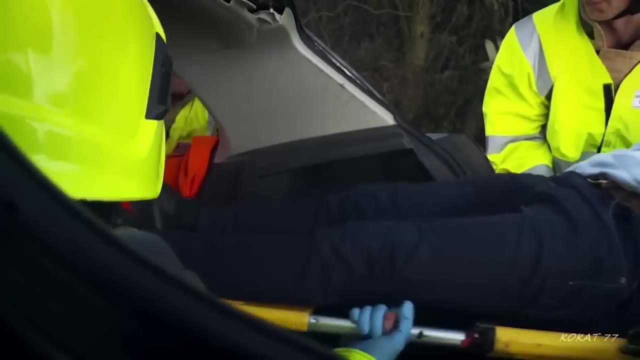 On slide One, two, three slide: Brilliant, OK, guys, thank you, There we go. That's it, I'll get in there. Somebody come and feed in there. Brilliant, Turn down, Perfect, OK, Nice and still. 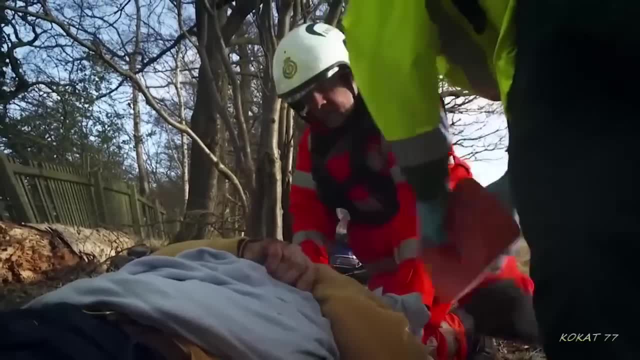 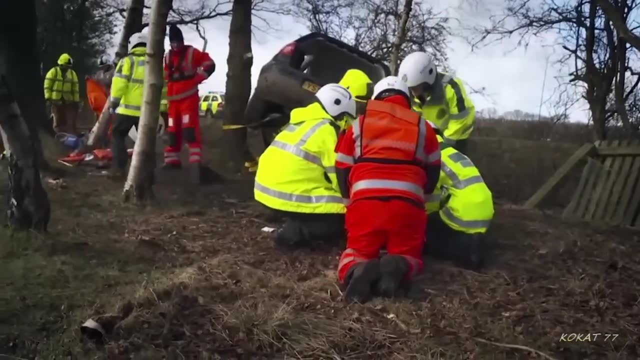 Lovely Okey-dokey, Get some blocks on you Just because you've had a bit of a do. you're not quite sure what's happened. Martin was traveling back from a weekend away in the lakes. Now he's facing possible surgery to his back or neck. 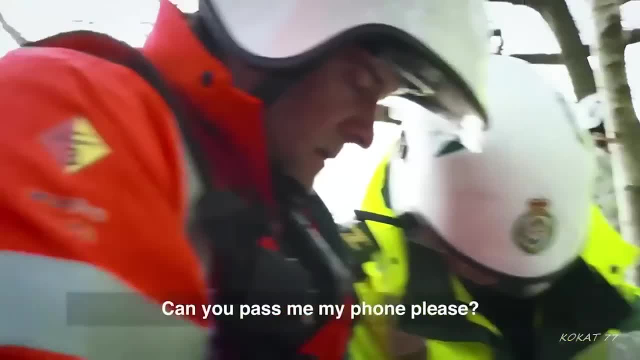 But his injuries aren't his only worries. Can you pass me my phone please? yeah, Your what? My phone? All right, we'll sort that in a minute. yeah, All right, We'll sort it out, Don't worry mate. 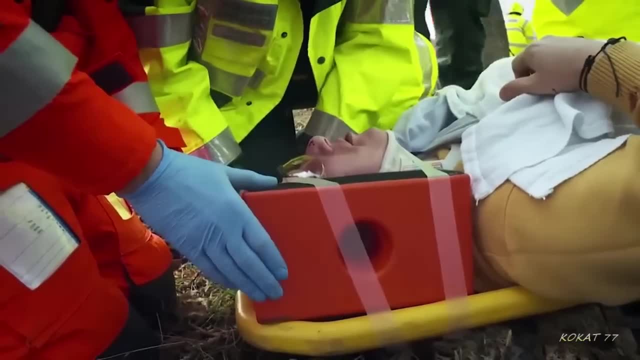 Just relax for now. Let's get you in the ambulance and we'll get everything sorted. Time of the flight. Right still, May I put it in my pocket? No, I'll sort it. I'll give it to you in the ambulance, OK. 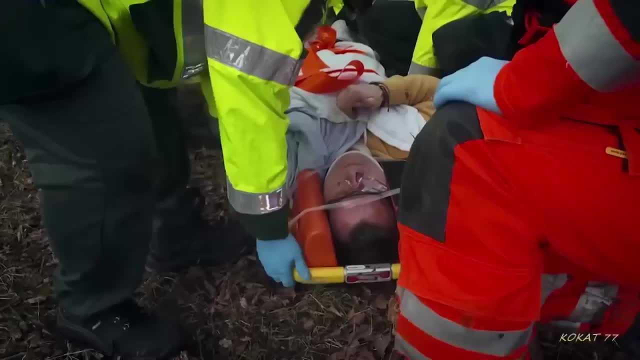 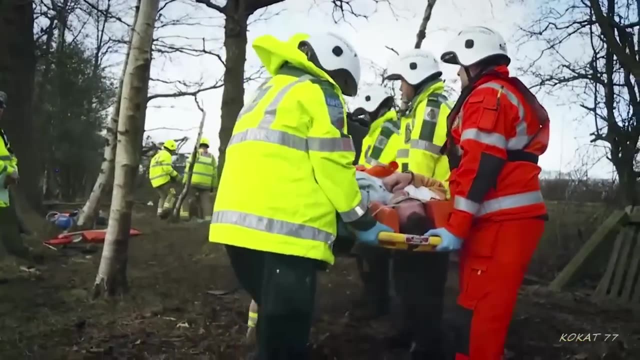 Don't worry, We're surrounded by coppers, mate, No one's going to nick it. Ready, steady, lift Marvelous No feet. first He'll be taken by land ambulance to join Natalia at the nearby Harrogate Hospital. 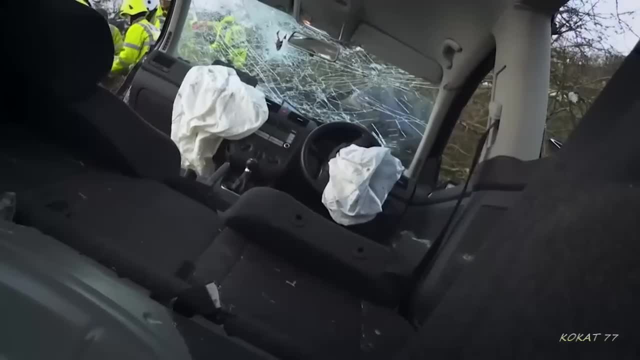 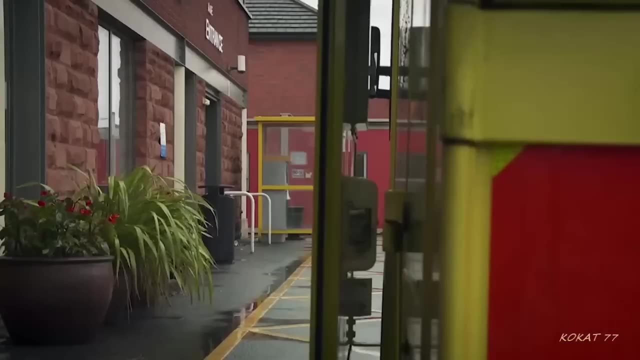 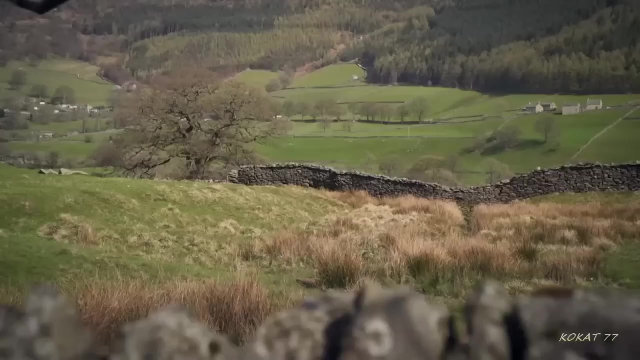 This might be a life-changing accident. It's a life-saving accident for both of them. Scans on their spines are already scheduled. The James Cook University Hospital in Middlesbrough covers some of the UK's most rugged countryside: the rolling moors and isolated dales of North Yorkshire. 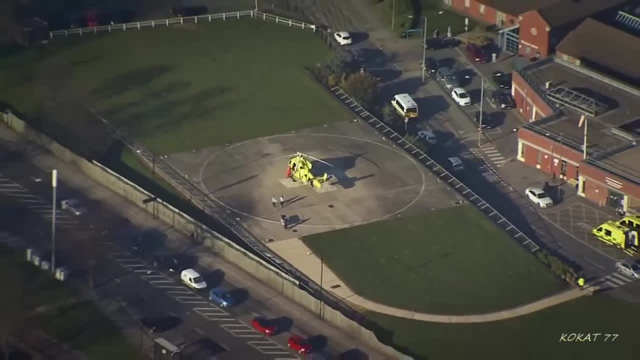 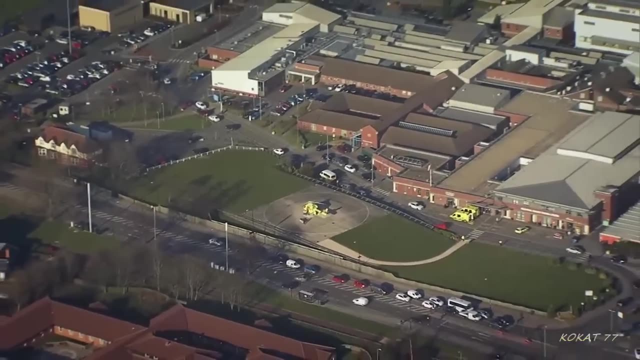 For many of its patients, it's an hour's drive or more from home, And today, on the helipad, paramedics James and Andy are going to show you what they've done. Yeah, the details are a bit sketchy, but it's somebody semi-conscious after a tractor. 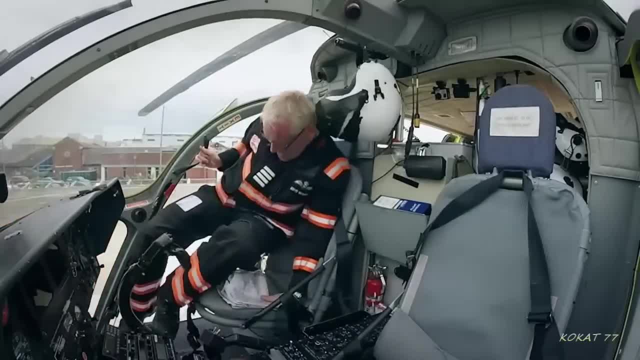 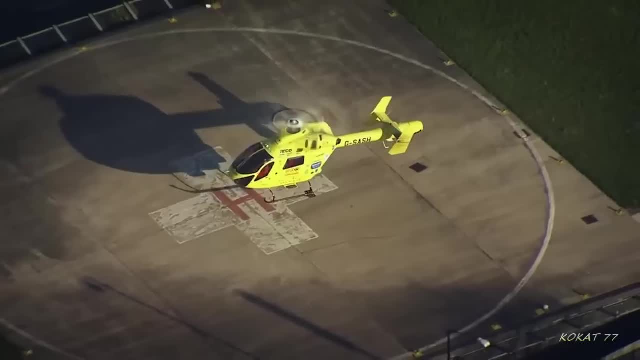 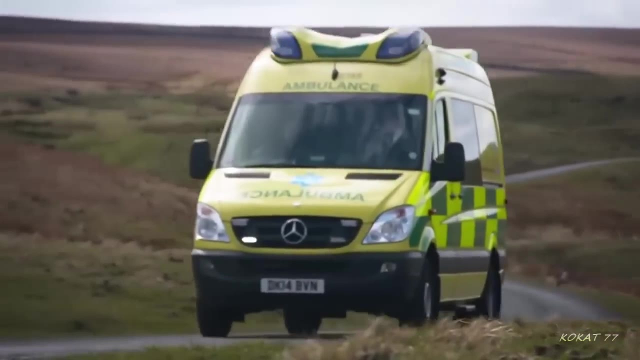 versus slurry pit accident. Slurry pit: Yeah, you're going to get it. What in the shit? The accidents happen just 20 miles away as the crow flies. Local paramedics are beating the chopper, but they're a 40-minute drive from Middlesbrough. 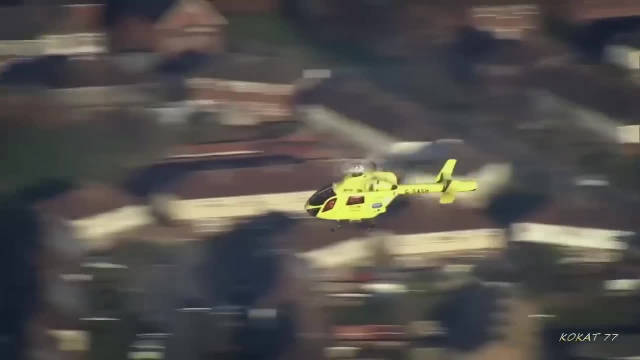 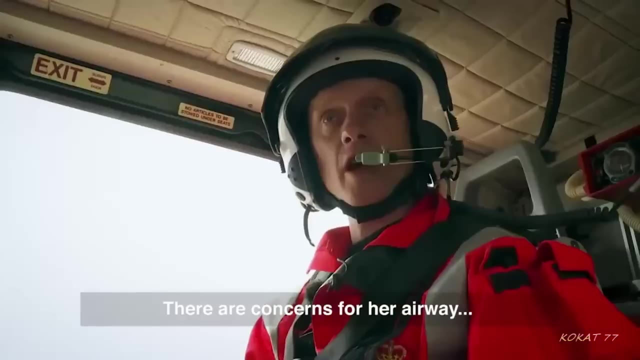 That's rotary topping. Oh yeah, We're in for that. to start with, Roger Pilot Steve Wardby will have his team at the isolated farm in 10 minutes. Sounds quite serious Concerns about airway. We're being semi-conscious. 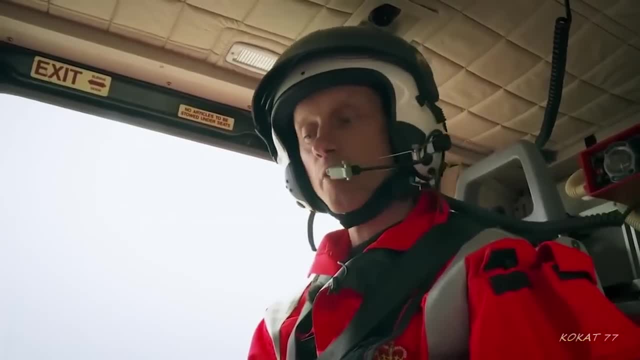 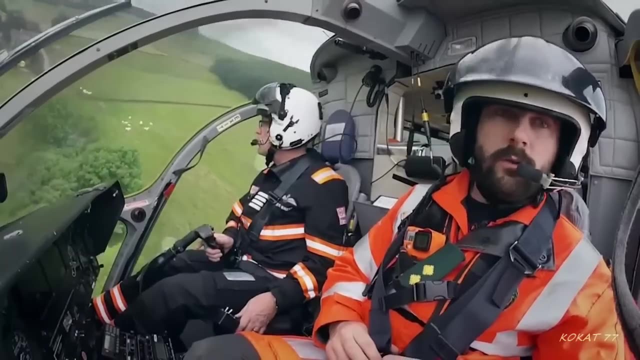 Just that's the first thought that goes through my mind. We'll see what we get there. Rosedale is a tiny community surrounded by the high hills of the North York Moors. No obvious wires by side. Thank you very much. A bit of a slope actually. 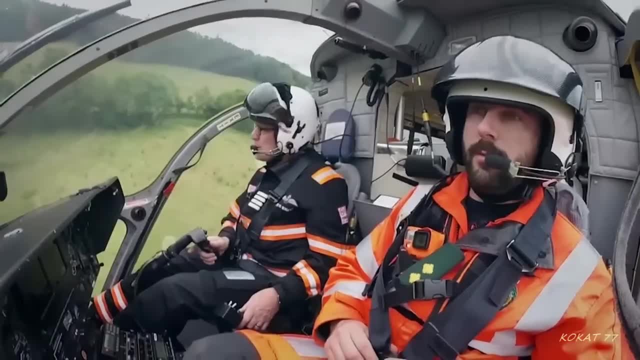 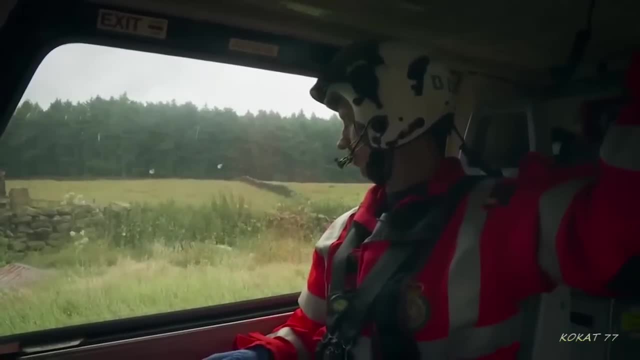 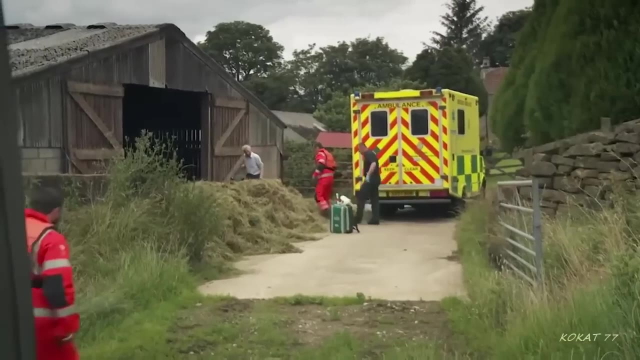 Unless you're right by the gate. No, we'll go right up there. Yeah, Got regular tin sheets there guys. Just watch that for me. Yep, Cheap 99 London. Claire Dring was driving a tractor when it careered backwards through the wall of a barn. 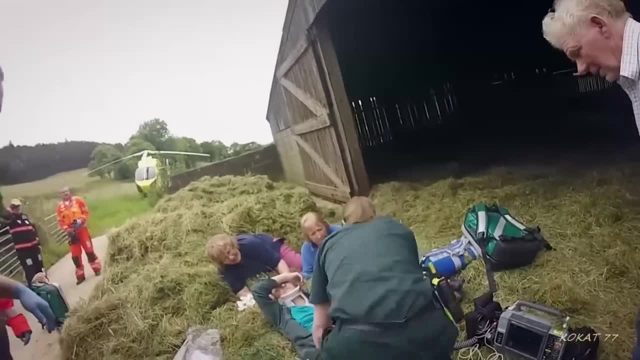 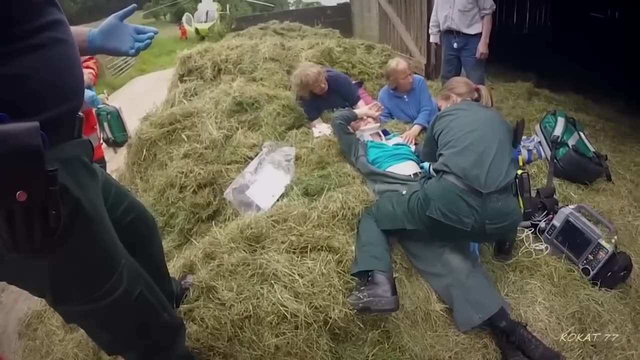 The cause of the accident isn't clear How we doing For some reason. we don't know whether there's been sort of an episode at the wheel or whatever. Yeah, But it's rolled backwards, It's gone through that road wall there which has destroyed it. 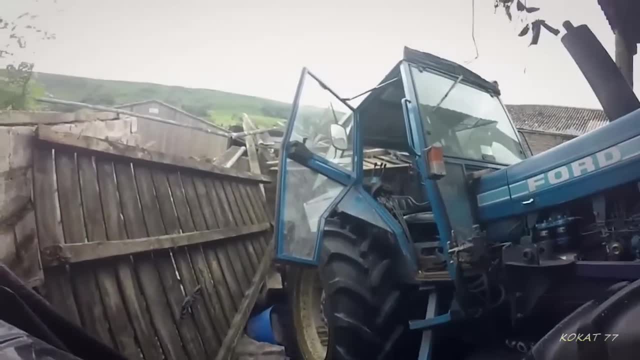 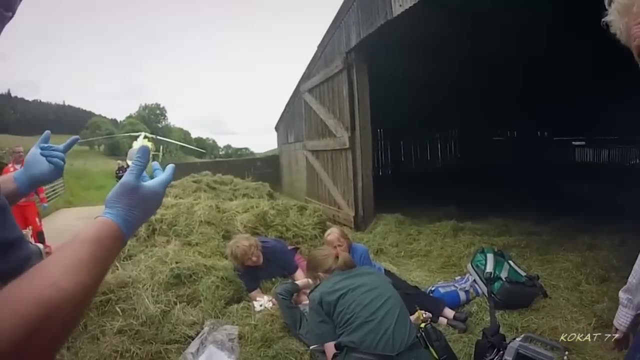 It's taken the end of the wall. The tractor came to a rest just feet from the slurry tank. There's the back of the cab- like a glass cab, Yeah, which was missing and it's possibly hit a head on some of the wood. 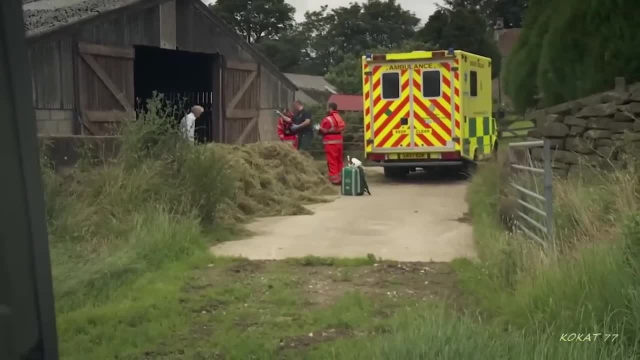 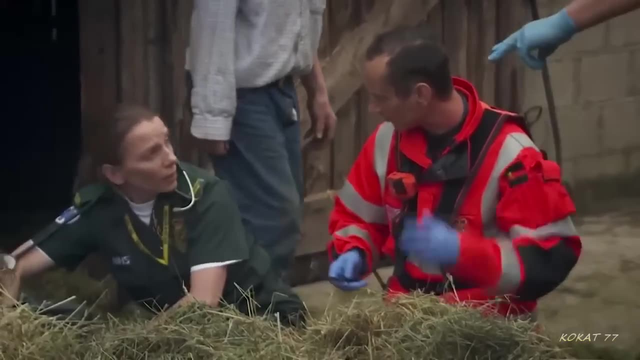 and the stone structure on the back of that. so we're thinking some kind of head injury. Claire is confused and lapsing in and out of consciousness. When you say head injury, are we on about with lower GCS or Agitation more than anything? 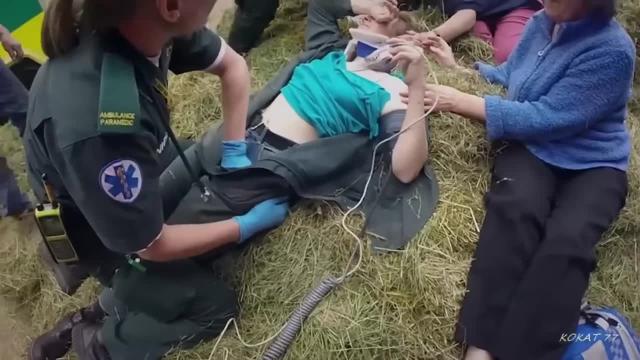 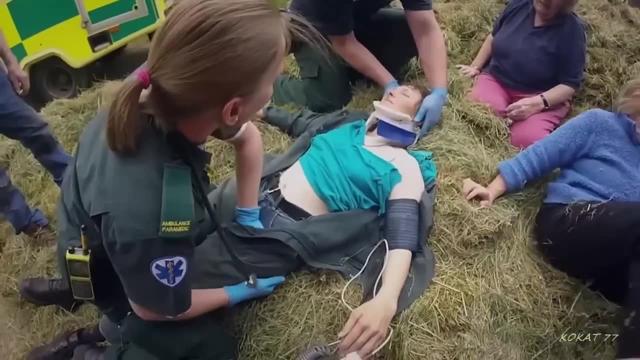 So probably about GCS 14, maybe At the moment. OK, Claire, nice to meet you, Claire, nice and still for me, Nice and still Tacky, ain't you? Her heart is racing. Paramedic Andy suspects Claire has a serious internal injury. 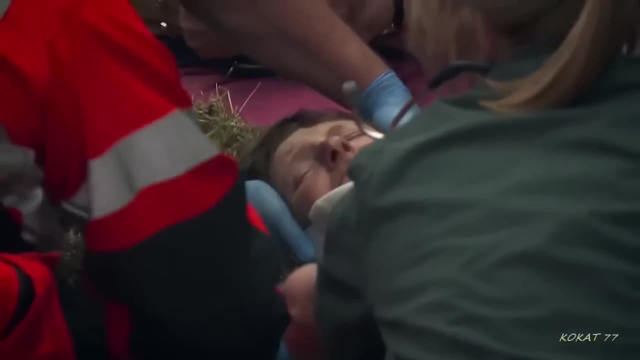 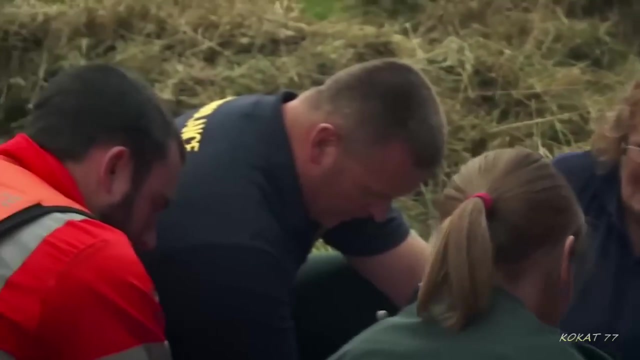 but it could also be caused by a head wound. I think it's the tacky from that. Yeah, Just going to bob a cannula in Nice and still, my love, You're doing great. How did she get up here then? 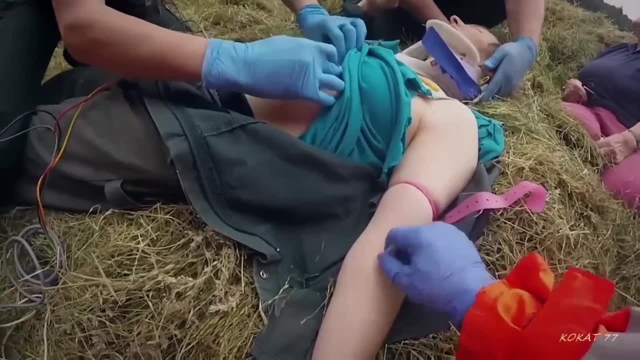 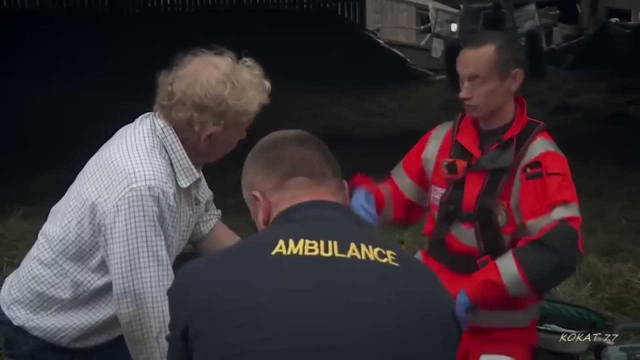 She got out. So she was unresponsive, probably had a bit of an LOC Very much so She was dead. So this chap was with her. He thought she was dead, so And out cold, Yeah. So she went in there just a little like that, looking pale or anything, or. 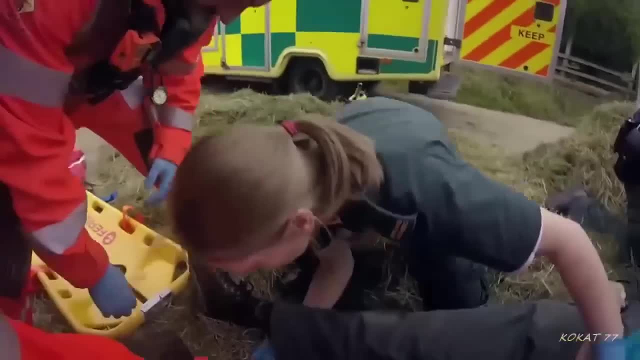 She's completely out. Like I say, she's mobilised up here, hasn't she? Do you know? when she got out then Did you help her out or did she just get out herself? No, I don't know. 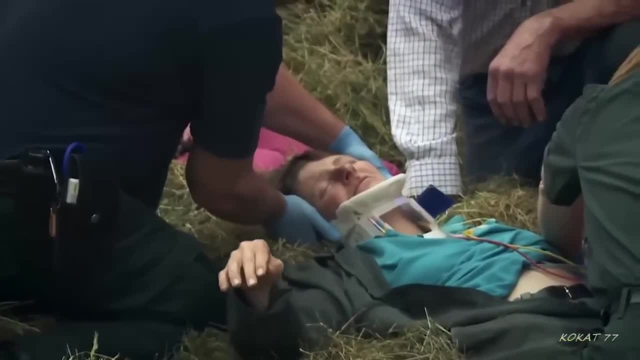 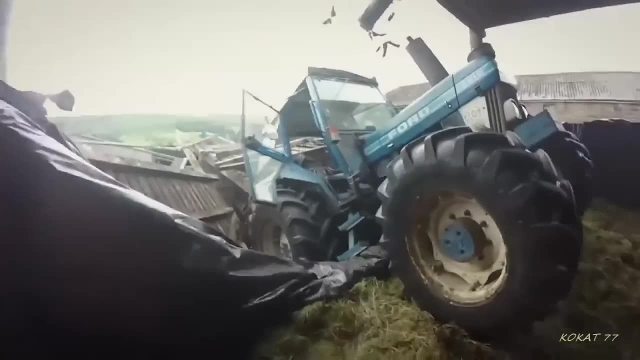 We were in a battle and you gave her in, Right? Do you want to have a look at it, mate? Yeah, The back of it's obviously out, but you can see where there's the wood and stone that look like they've come into the cab. 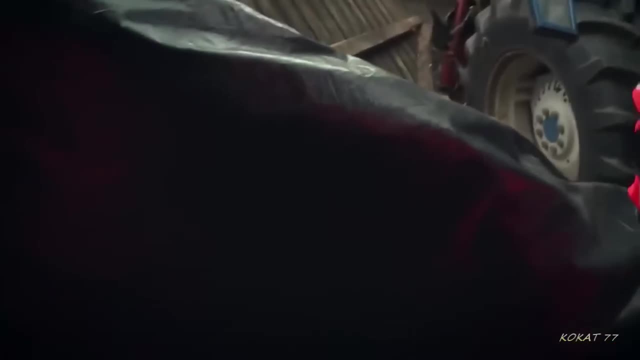 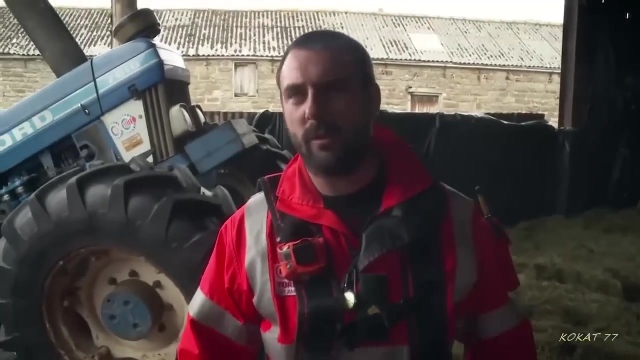 That wall there, the whole wall's gone back with it. Bizarre. I don't know whether or not she's just lost it and then that's it to knock back her head, but there's some confusion at the minute as to how long she may have been unconscious. 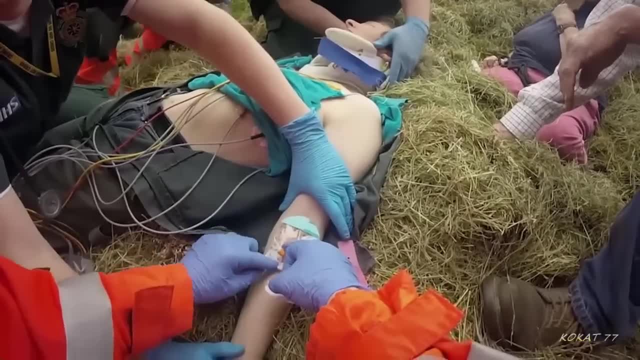 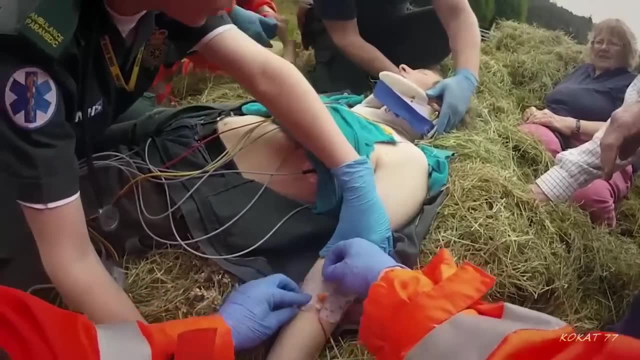 So we can only go on, really what we're looking after. She's not complaining of being in any pain, is she? No, not at all. No, No, no, Claire, can we just ask you yet again: have you got any pain anywhere? 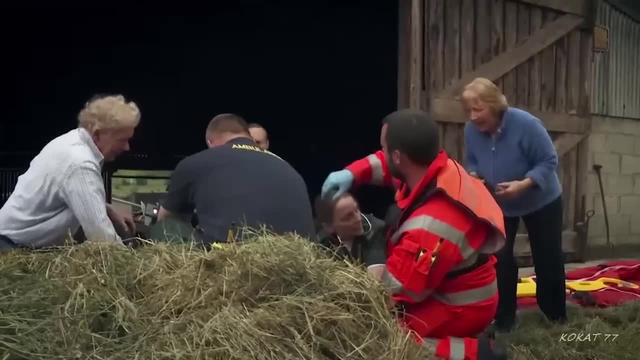 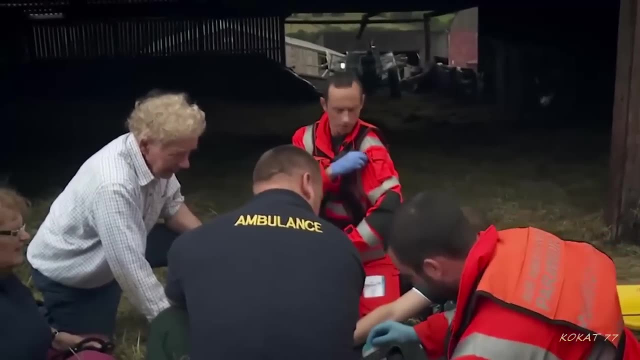 No, No pain. OK, Her confusion and lack of visible injury are making the assessment difficult. Yeah, mate, All of this is to make sure you keep well, OK, The only injury we can see is there's some bruising to the left side of her head. 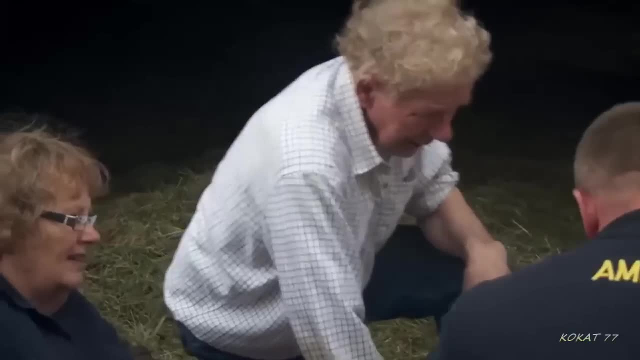 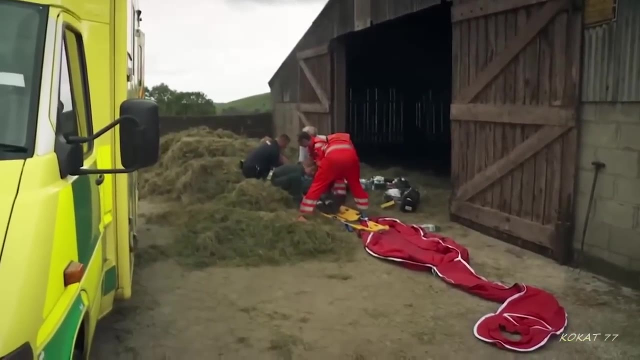 Left side this there isn't it Where my hand is Sort of temporal area, Yeah, Left temporal zygoma area, Just for one minute longer. It's a perplexing case. Bring her down, All right, Let us know when you're ready, mate. 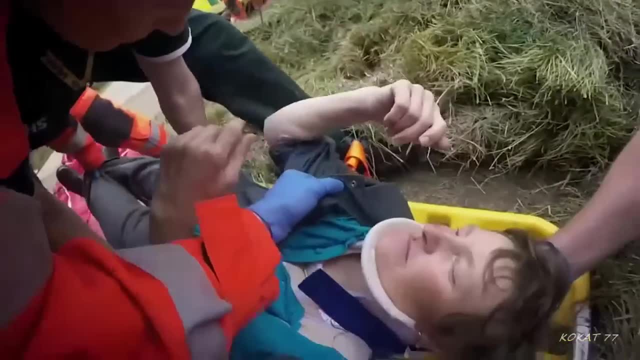 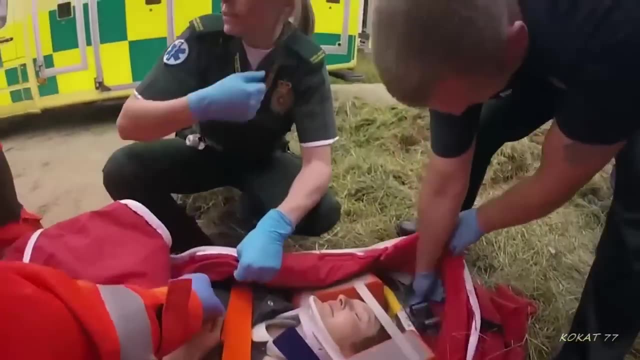 Just keep your arms in, All right. But there is a further clue. She constantly had this right-hand gaze over to this way. Weird innit. Her head is just to the right and her gaze has always been to the right. 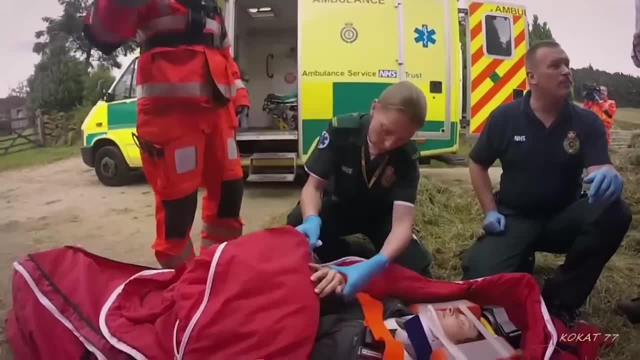 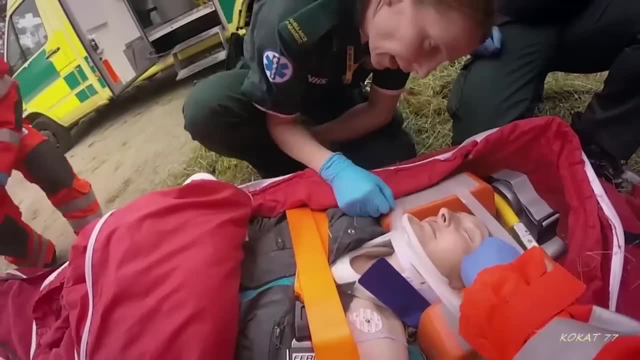 Right. Her constant glancing to the right could be a symptom of a brain injury. So we've got a bit round here, haven't we? A bit of a lump there. What is clear is that Claire urgently needs X-rays and brain scans at James Cook. 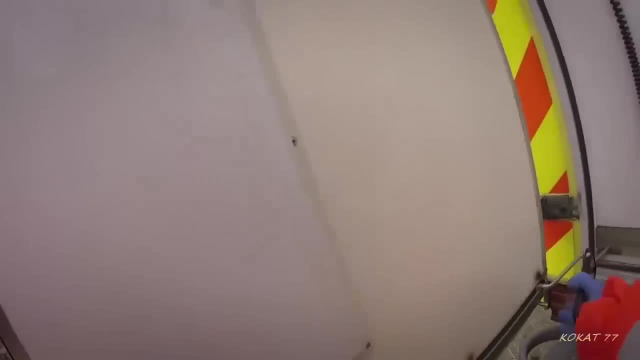 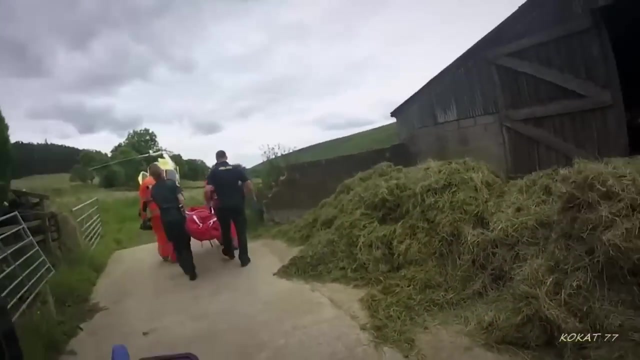 Helimed 99 is going to be heading back to Middlesbrough. You're doing a good job there, Excellent job. The air ambulance is always a welcome sight on the moors. It means the local medics can stay to deal with the next emergency. 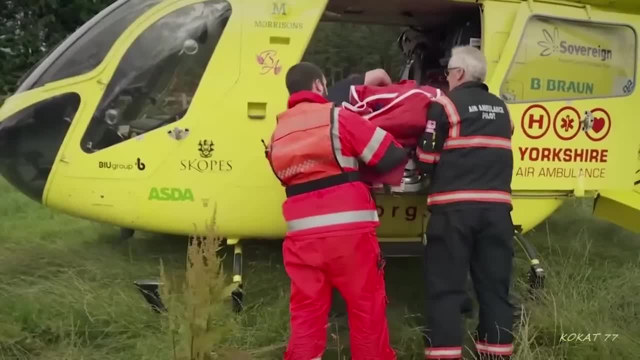 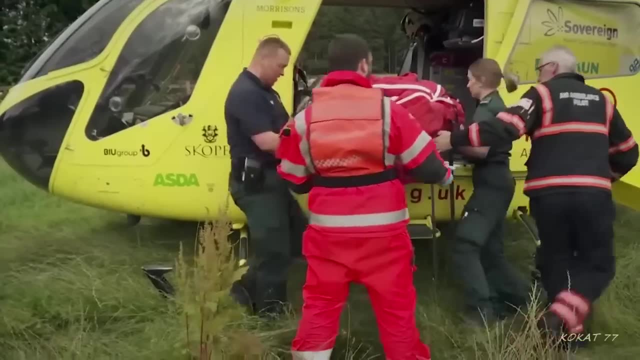 rather than wasting time on the long drive on poor roads to the trauma centre. Hiya, it's Andy on Helimed 99 again Now we're wondering whether she's had a bit of a do while she's been in the tractor. 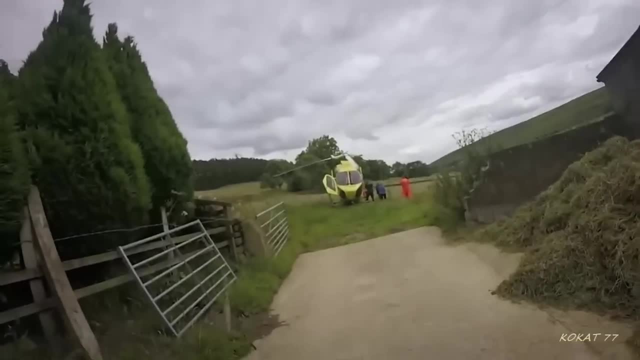 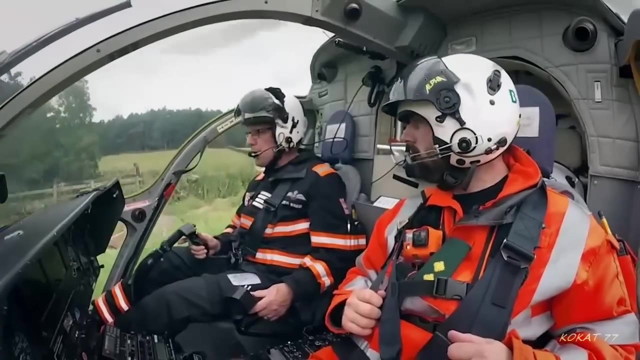 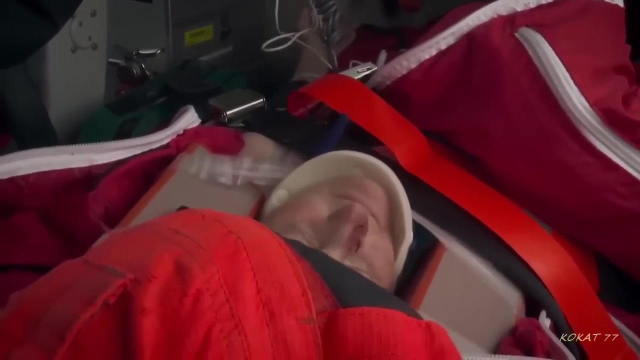 or she's got something going on post-incident, Probably about ten minutes. All right, bye, Bye. Paramedic Andy is hoping diagnostic tests will answer the many mysteries surrounding this case. She could have had a fit. She could have had some cardiac event. 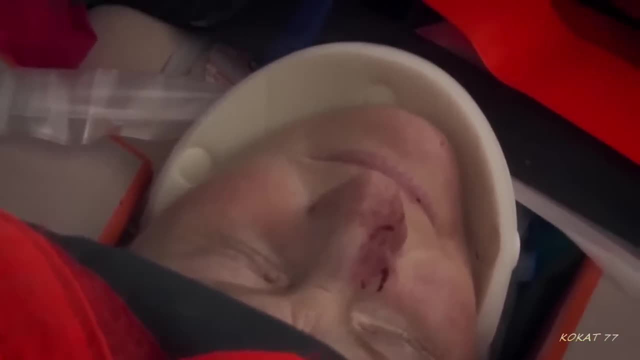 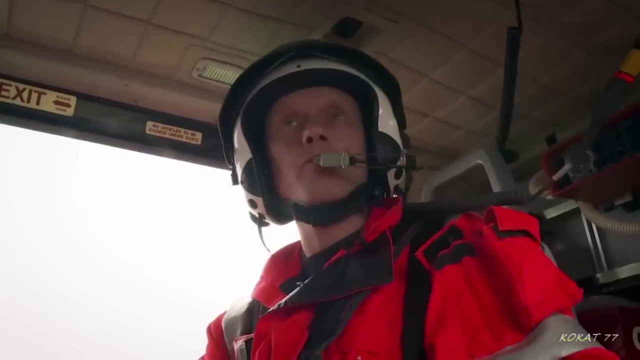 which has caused her to lose control, Or it could be a mechanical failure of the tractor. Got a fast pulse, which is a bit unusual. If she's had a fit, you could have a fast pulse. A bump to the edge, you could have a fast pulse. 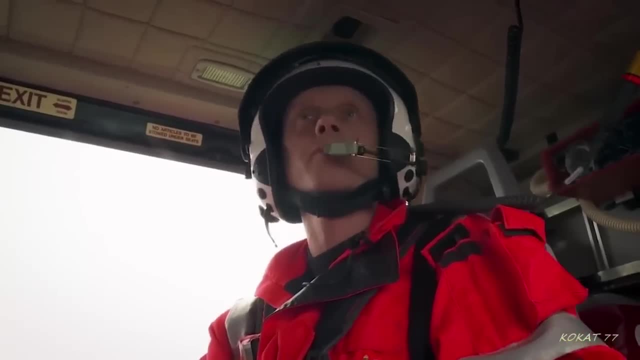 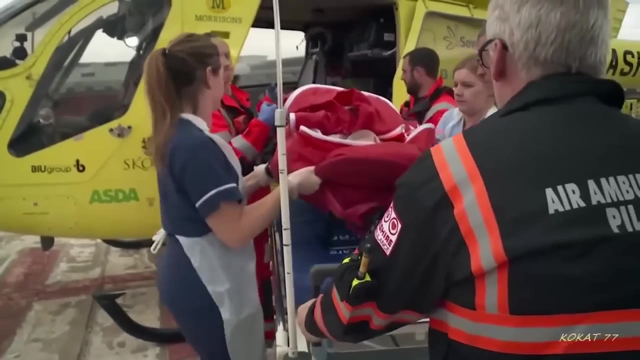 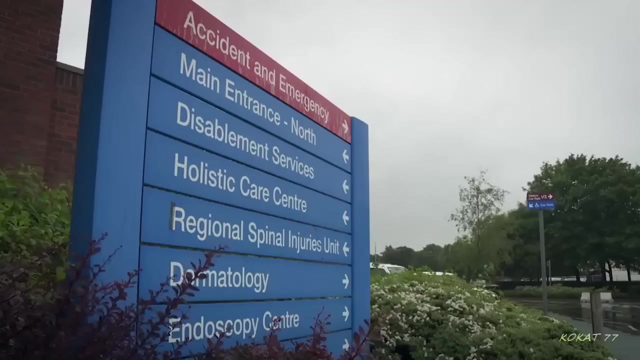 So something's not quite right. Claire is now minutes from intensive care, Ready, steady slide. She's x-rayed and a head injury is ruled out, But she has lacerated her liver. She undergoes surgery and after four days is fit to return to the country. 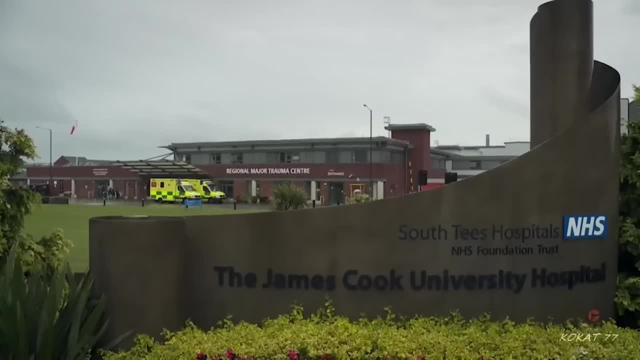 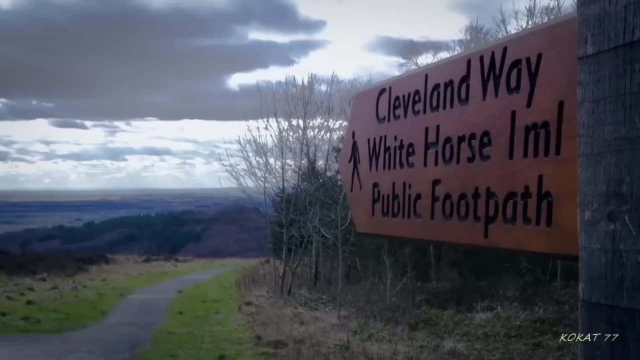 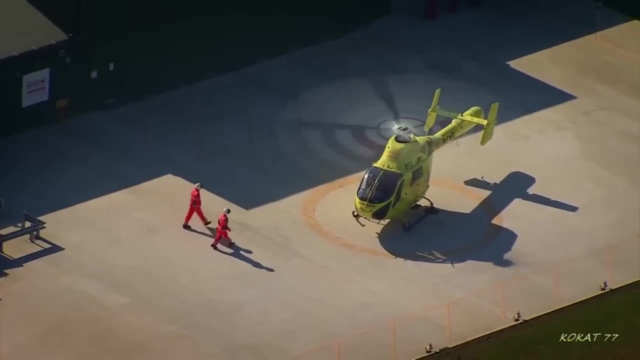 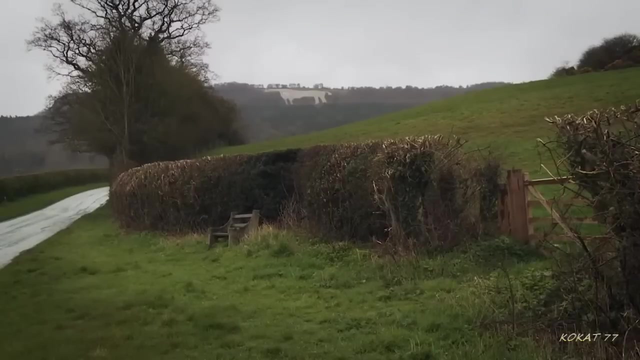 It's been a lucky escape. Hello ambulance service. It's a pressured breathing. It's midwinter in North Yorkshire and Helimed 9-8 is heading up to one of its most famous landmarks: a huge chalk horse carved into the side of the rugged North York moors. 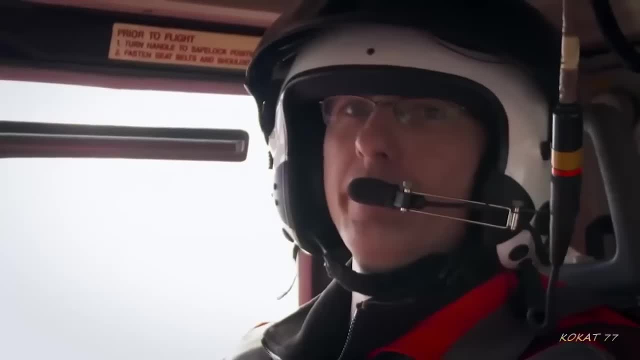 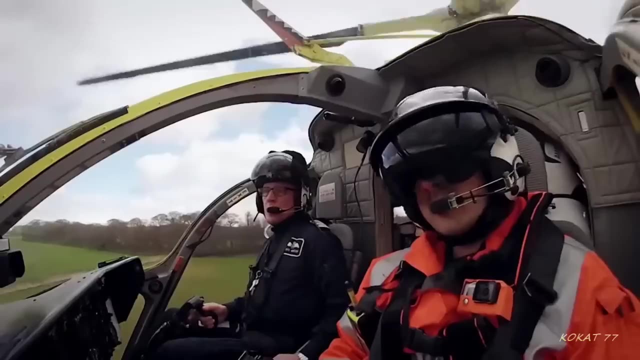 We're responding to a 67-year-old female who has fallen near the white horse in mid-North Yorkshire. We've got a crew responding to back us up, as well as Mountain Rescue. He went slightly from the left. The patient's life is in real danger. 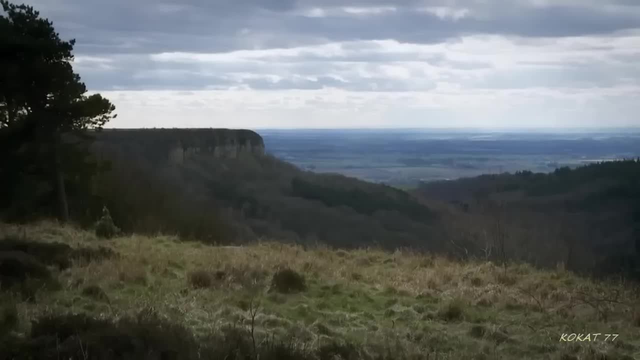 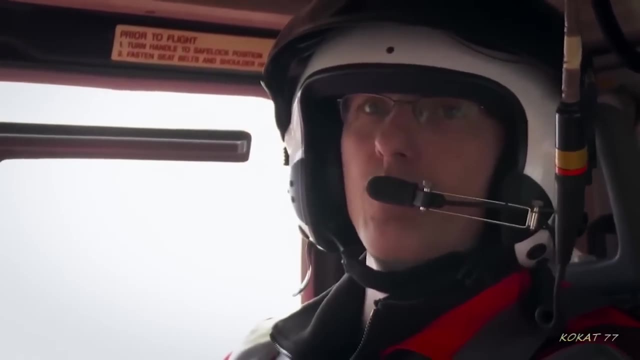 She's lying in sub-zero temperatures, unable to walk and a long way from a road, Knowing the area as we do. obviously, flying from top fifth, it is quite steep, so to try and get reasonable access to this lady it might be quite difficult. 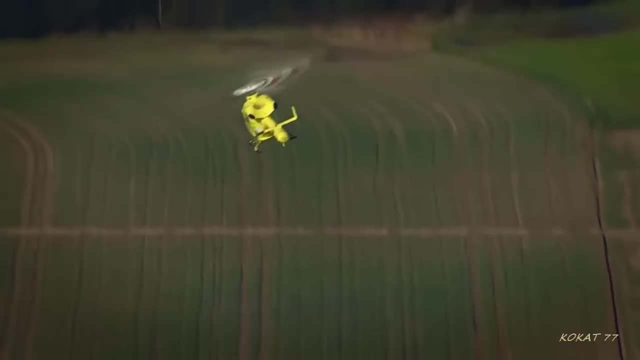 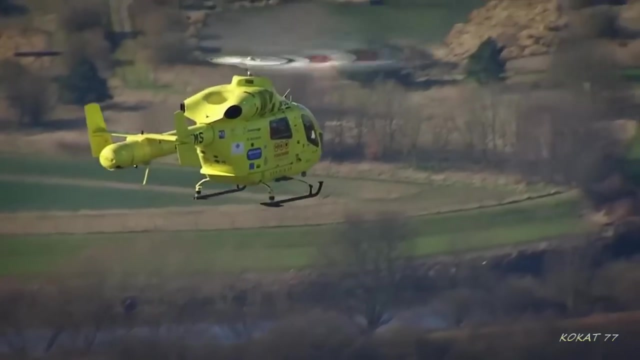 so it might be a bit of a trek down a hill up a hill, whichever we may find when we get there. Some of the white horses down south are really old, aren't they? They're kind of prehistoric, But I've got a feeling the one at South Bank is just like 50.. 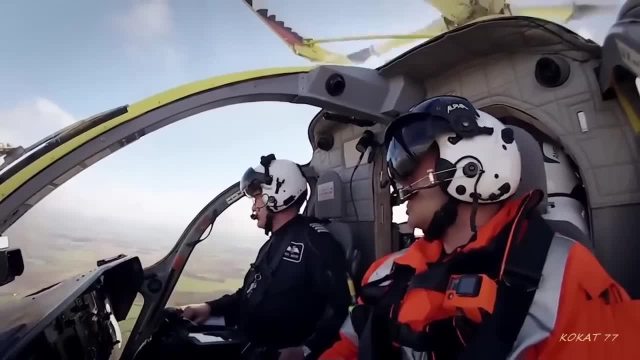 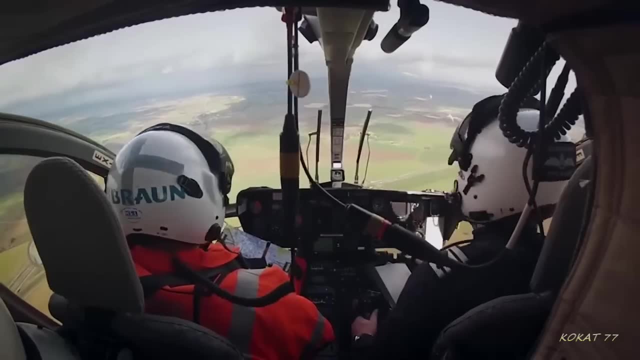 50,, 60 years ago, somebody decided it'd be cool if they had a white horse. It's just a bit of graffiti. that's what it is. Yeah, basically, yeah, We've got rain ahead, guys, For paramedics: Paul and Al. 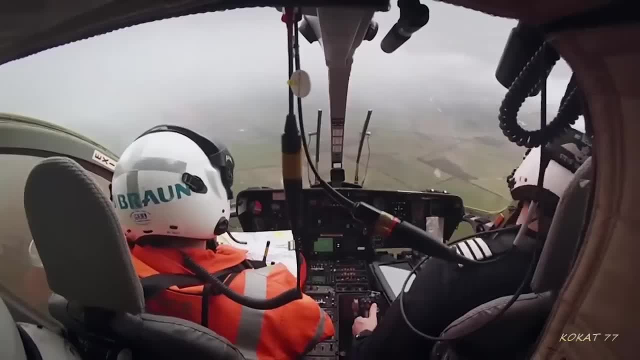 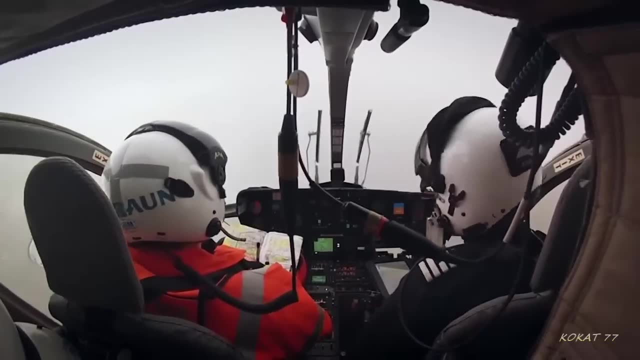 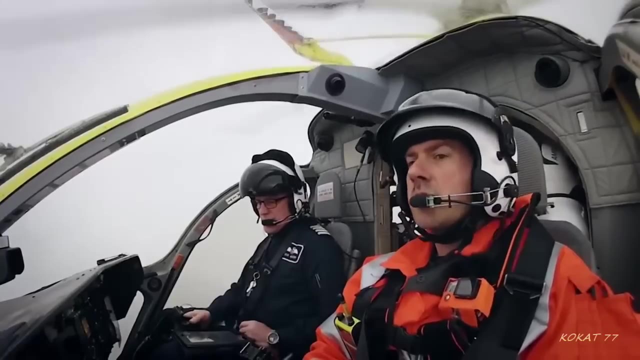 this is a routine mission made risky by the weather. Helimed 98's heading for a storm, I think ice forming on the Quite a bit, It's so cold. the rain is freezing on contact with the chopper. We'll come down. 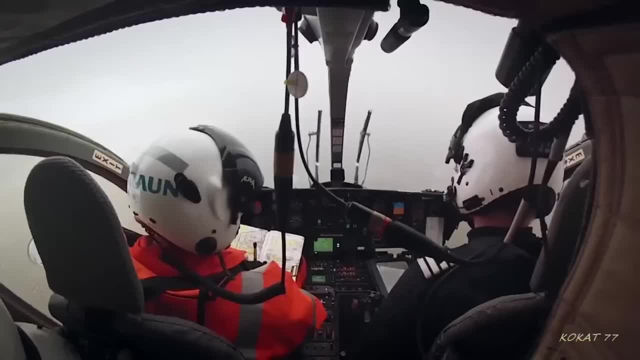 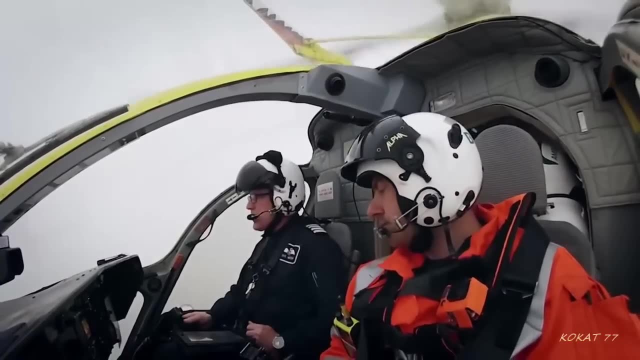 Outside air is plus one. If the ice is allowed to build up, its weight could cause Helimed 98 to crash. Pilot Steve must get out of the rain fast. We'll get ready to clear this. You can see the ground there now. 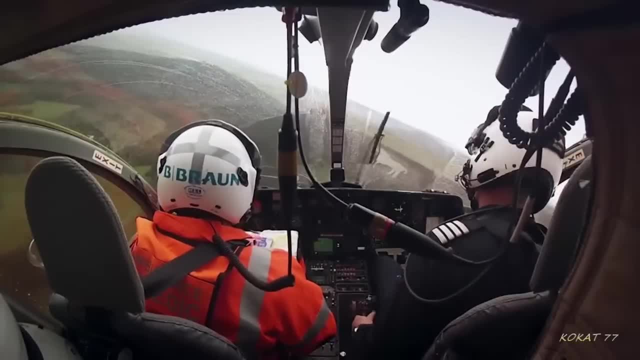 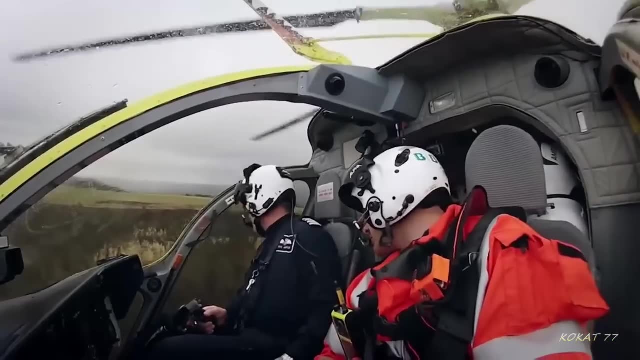 There we are. we're just about to come out now. It stops as soon as it's started, But the same freezing conditions are making this rescue even more urgent. There we are, casualty 2 o'clock Visual. yeah, We'll land on the top and 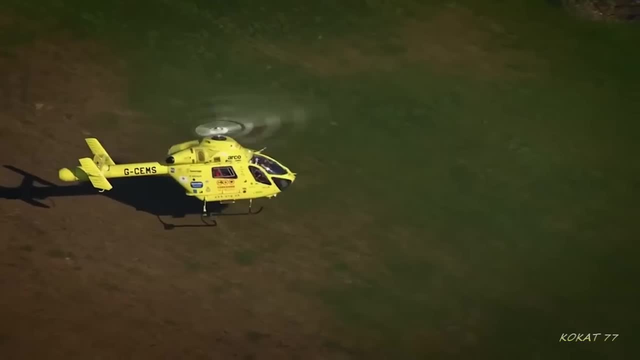 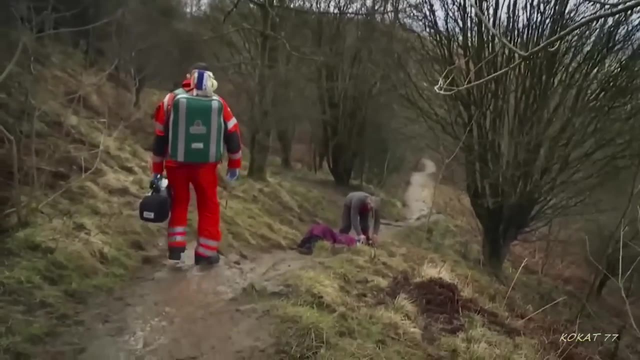 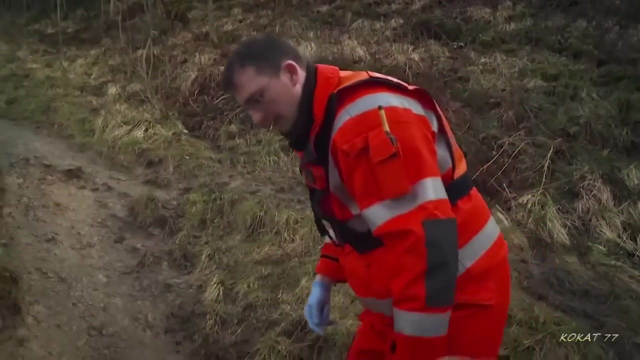 Yeah, yeah, Go down On the top and come down. How are we doing Mate 2, that's just arrived at patient side. now The team's patient is a veteran walker stranded on a treacherous footpath along the edge of the moors. 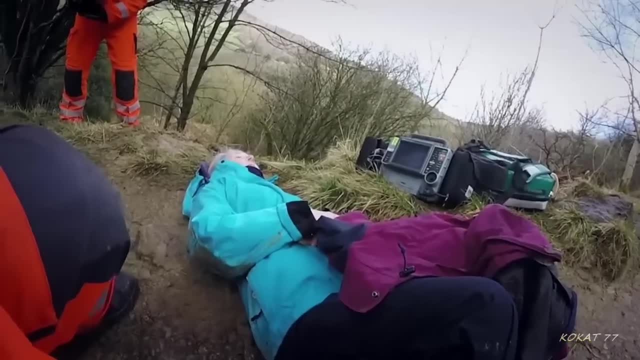 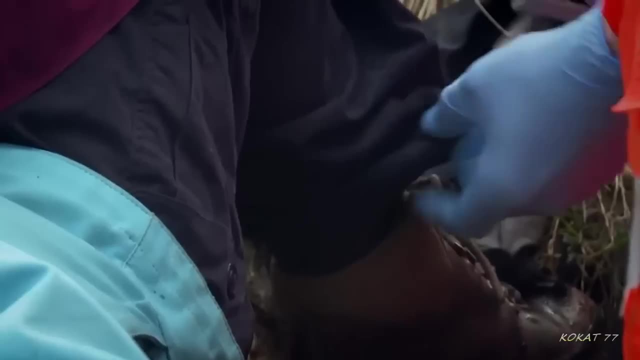 You know me fitting well. Yeah, So you've not been knocked out. can you remember everything that's happened to you? Yeah, Judith Moore is in agony and dangerously cold. We were coming up the bank. It was slippy so we were taking our time. 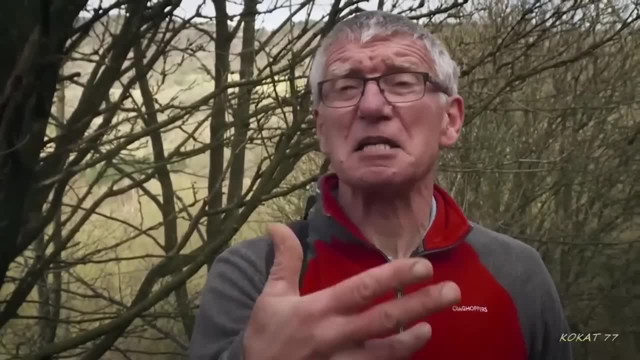 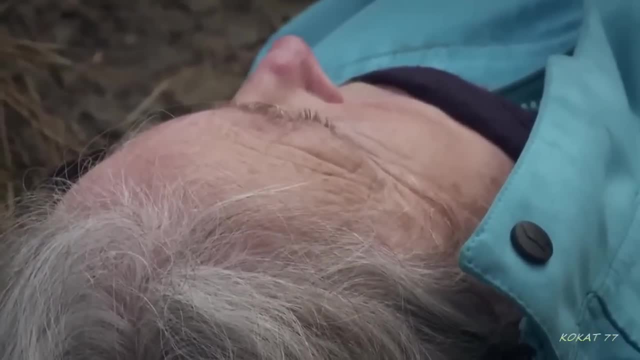 I was leading and I slipped and fell back onto my wife. She hit the ground with me and I must have fallen on her leg. Yeah, So your seat's more around your knee, is it? Yeah, It's like, Yeah, Yeah. 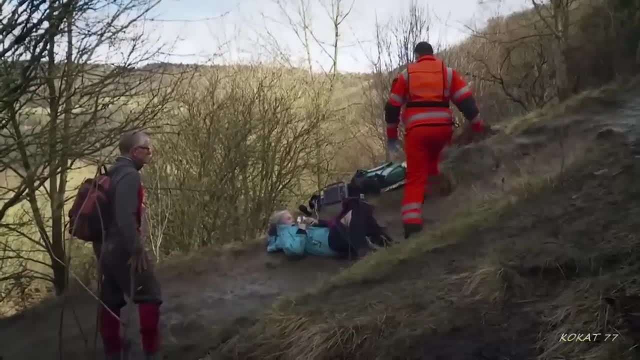 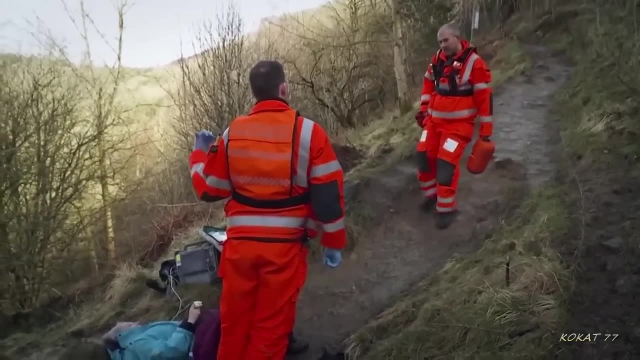 I wonder if you've dislocated your knee. Paramedic Paul diagnoses a broken leg and a dislocated knee. Judith's basically come over as her husband's fallen on top of her. Yeah, She's unable to move her knee as it is at the minute. 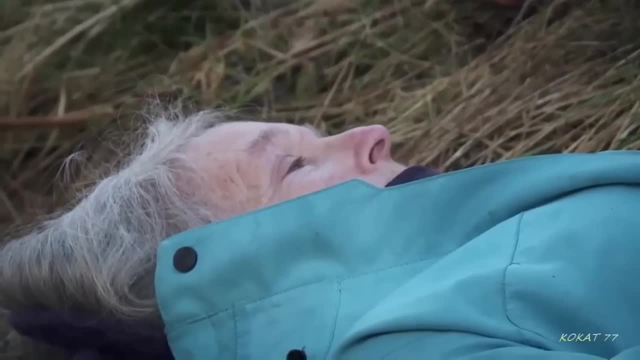 I'm wondering whether it's more dislocated than anything else. Right, She's really cold, so we could be doing something to keep her warmer. So if we- just If we- get the Flextalon on the path, Yeah, yeah. 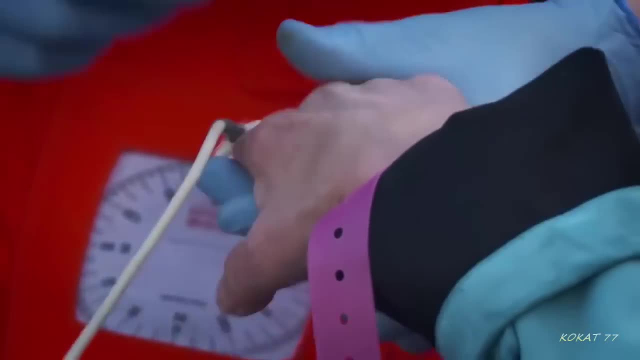 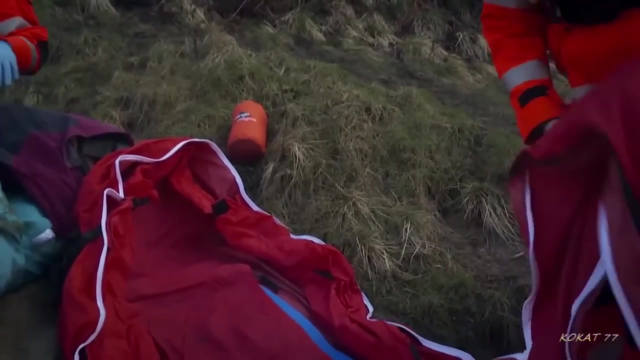 Just get her into it and then we'll get her sorted. How are you feeling? All right, Just cold. You're just cold. I know We've got a nice big, thick sleeping bag there for you to. Priority really is to insulate her, because the air temperature's probably only about. 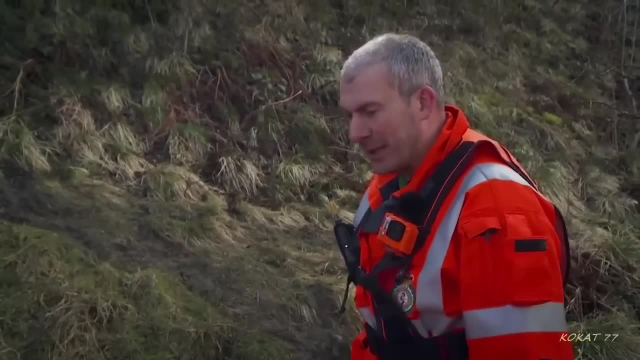 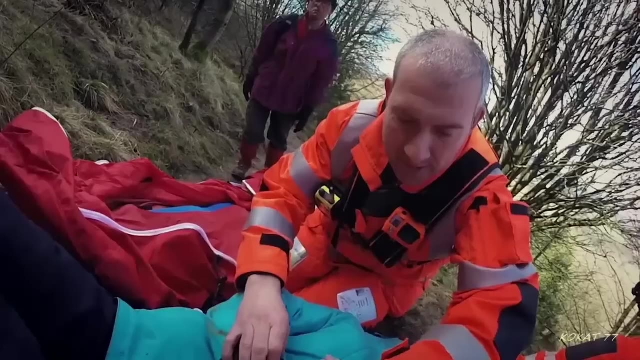 four or five degrees, And when you're laid in contact with the ground and not moving, you lose a lot of heat. so you get very cold quickly. That's what you like. Where are you from Hartlepool? Oh, they're all tough up there, aren't they? 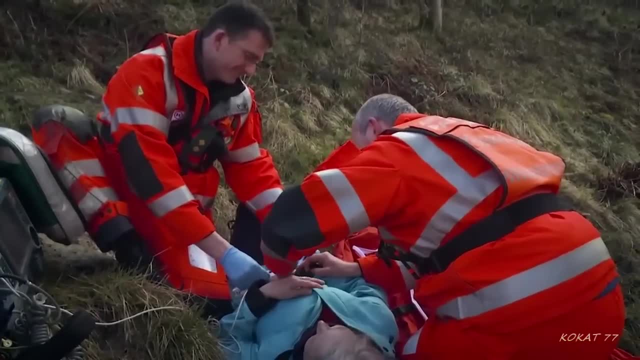 Yeah, Yeah, Yeah, Nice and silly sweetheart, Just try and twizzle around on your bum, Give me both your legs. Oh, oh, oh, oh, oh, oh, oh, Stop, stop, stop, stop, There we go. 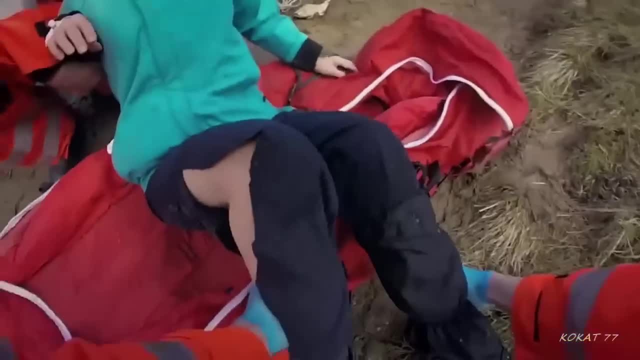 OK, Right, All we're going to do now is just turn you that way. Boom, That's perfect. Now just relax back. They're wrapping Judith in the Flextalon. It's a fur-lined bag designed to lock in heat. 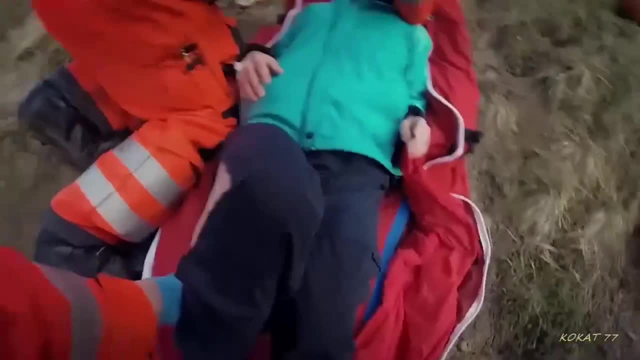 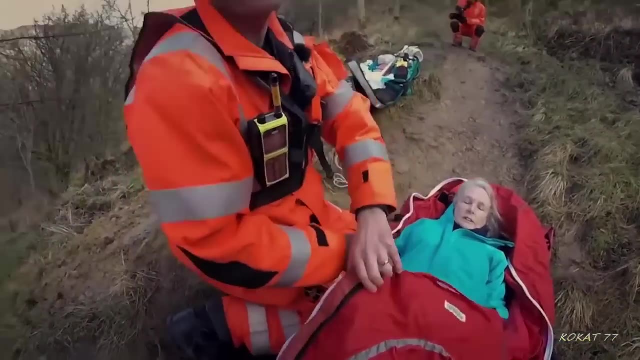 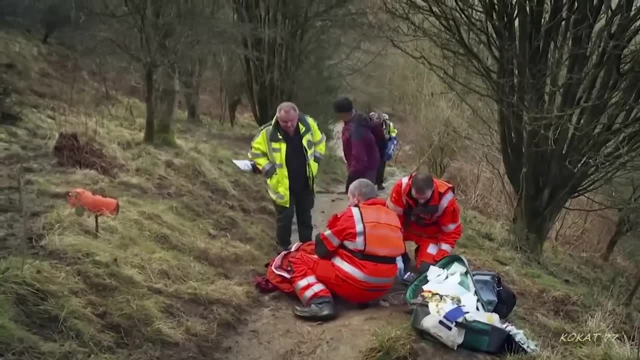 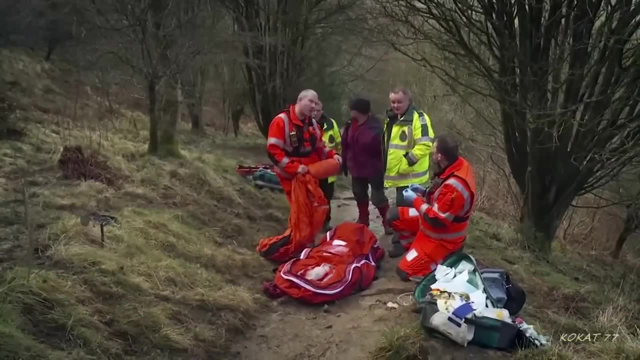 Yeah, Yeah, Yeah, Yeah Yeah, You're good, OK, Hello love, Hello love. This is my old pal here now The other boy's on the way down. But there are peanuts, But there aren't enough people to carry Judith up the slippery bank to the chopper safely. 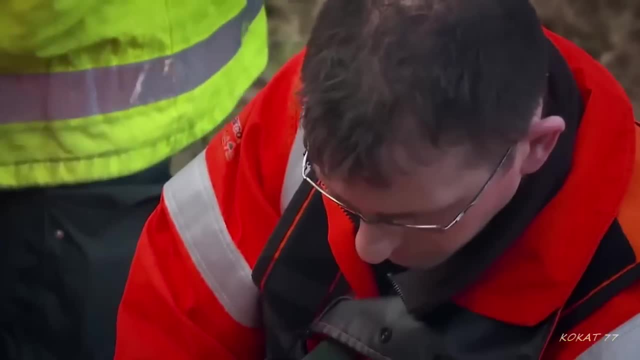 Uh well, they're left. Oh Well, they'll carry her up there. And thebec, How'd you carry her up there? MRT's on the way. MRT's on the way, so I've seen her on the way quer. 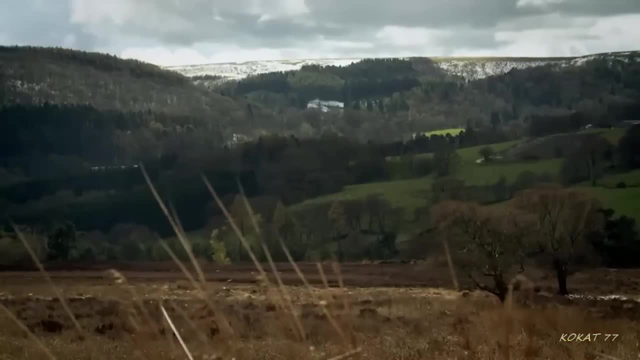 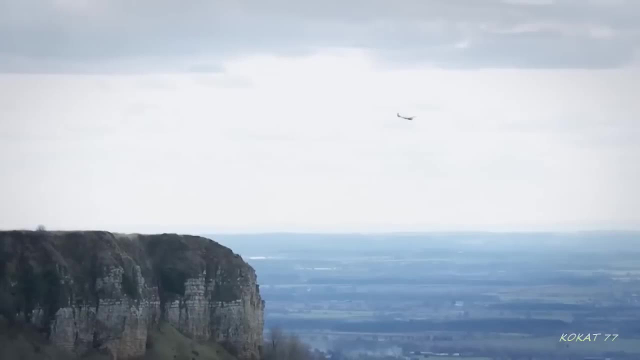 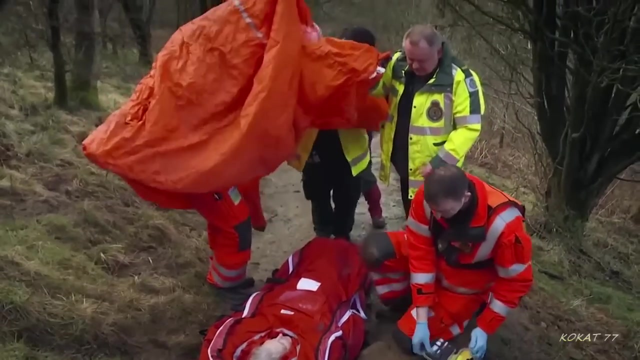 Yeah, They're going to need mountain rescue, but the weather's worsening and the temperatures are plummeting. High on the edge of the North York moors, walker Judith Moore desperately needs help. I'll come inside, Just sit on it now. 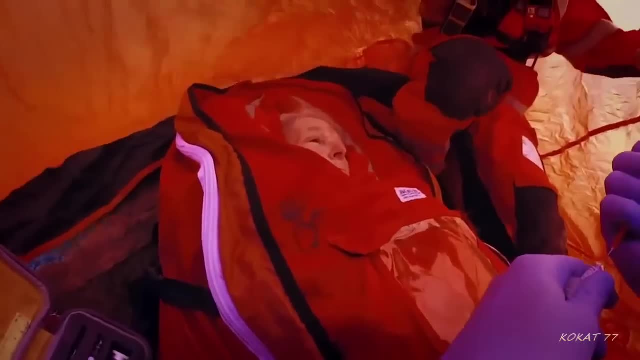 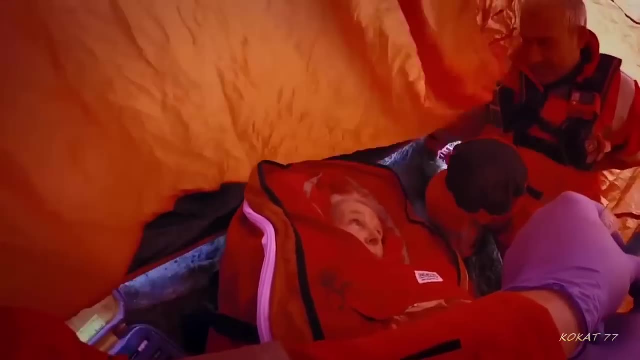 Just sit on a black. Find a black bit and sit on it. A mini tent will shield Judith from sub-zero temperatures. You'll literally be scorching. You'll not know why you're so cold in a minute. Surprising how quickly you warm up once you get inside the shelter. 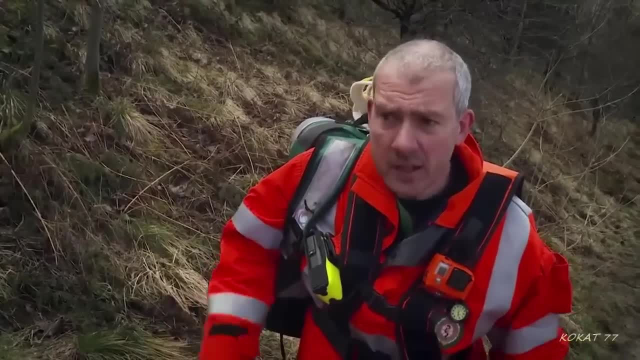 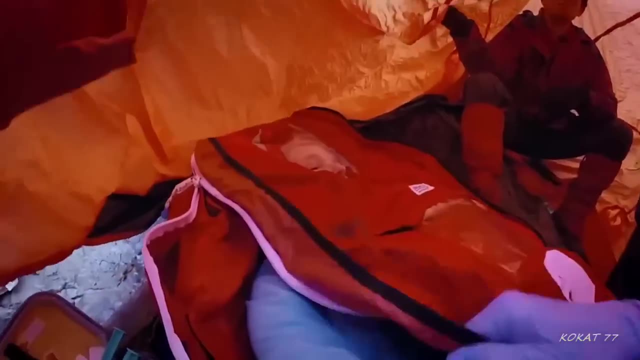 although it doesn't look to be much, It traps all the body heat from everybody in it, so the more people you can get in it, the warmer you get. Can I just lift your sleeve up, sweetheart? And it also protects you from any convection. 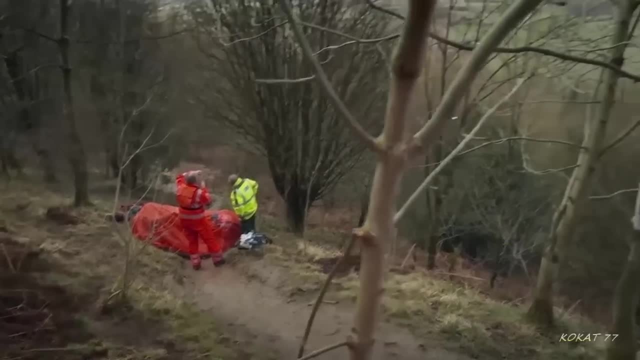 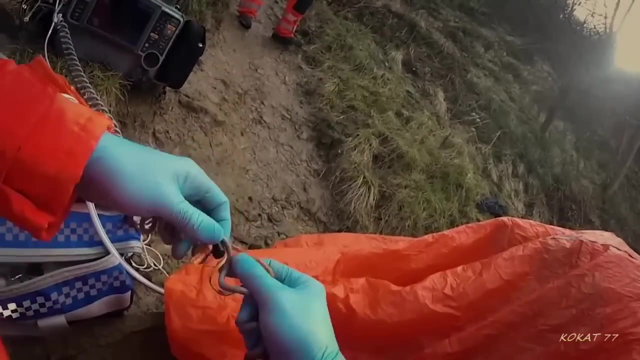 or losing heat to the surroundings. Paramedics Alan Peete are waiting for Mountain Rescue to help carry their patient to the chopper. Let's just flip this over so we can have a good look at what's going on. They're giving her powerful painkillers. 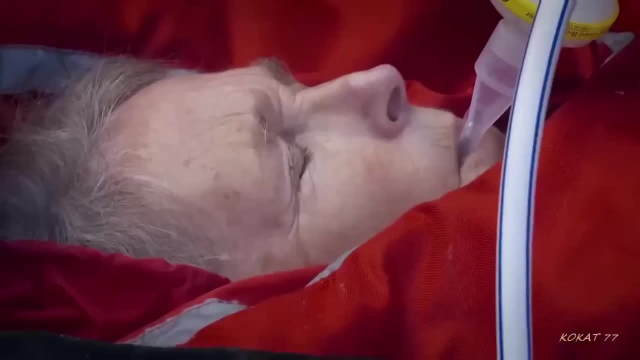 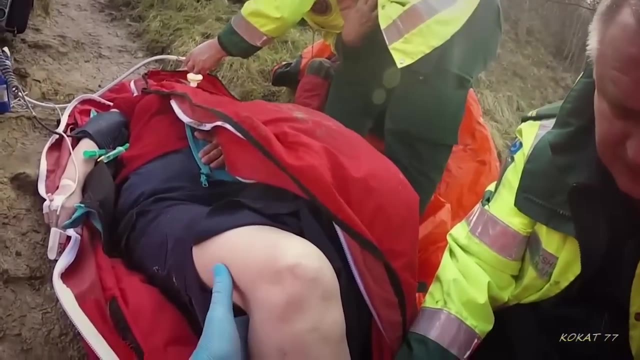 Her injury is agonising And they need to straighten her leg. Try and relax, sweetheart, as best as you can. Nice, long, deep breaths, love. That's it. Well done, Judith. Just try and keep your leg nice and relaxed. 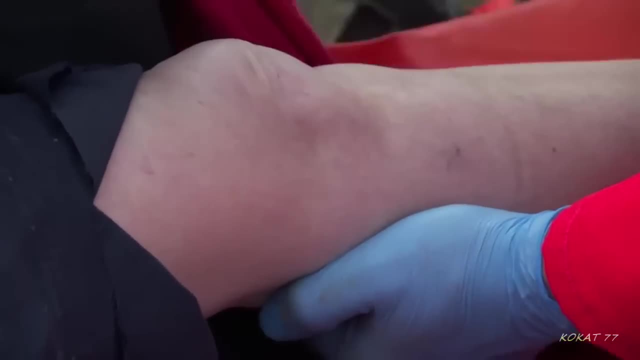 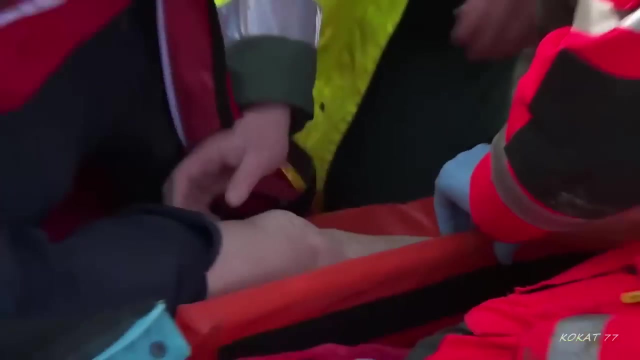 Well done, sweetheart. Nice deep breaths on that gas for me. The team's impressed by her courage. You happy there. Yeah, You've done that really well there. Judith, You're right, She's hard, She's hard. 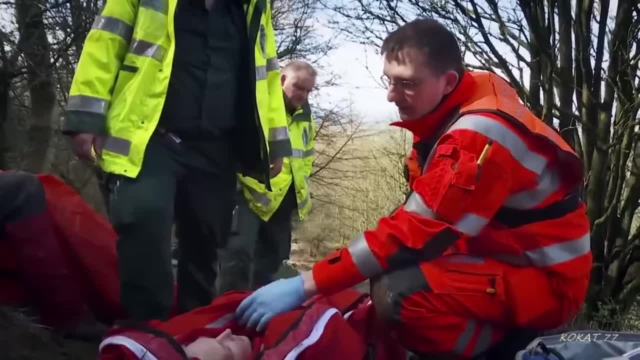 We've got Mountain Rescue coming out, OK, so they're going to put you on their stretcher to be able to get you up a lot easier than having to carry you. I think it's got a big wheel on it or something like that. 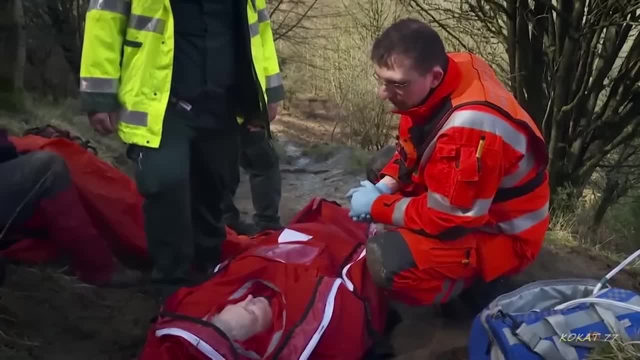 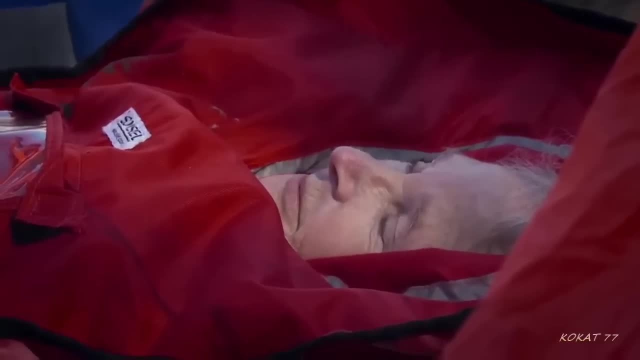 Will you wear an ambulance? Yes, love, We'll carry you up to the helicopter and we'll get you on board there. All right, though. At last Mountain Rescue have reached the scene. Hi there, Hey guys, you all right. 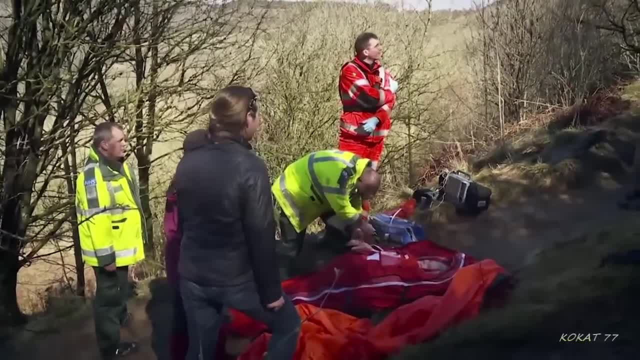 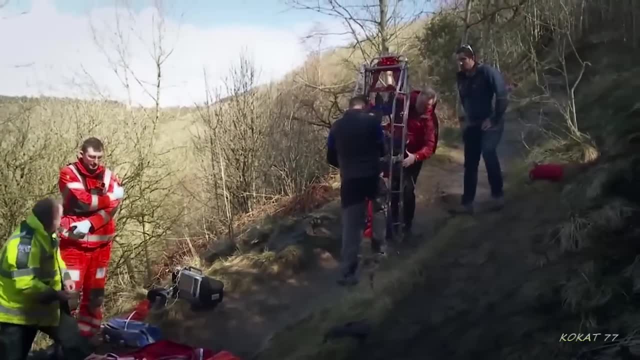 Thank you. Can I have these stretchers for you? This is Judith. Judith basically had a fall. Her husband's fell on top of her. She's then fallen down. I think it's a proximal tibia fracture. We'll probably wait on a few more just to lift. 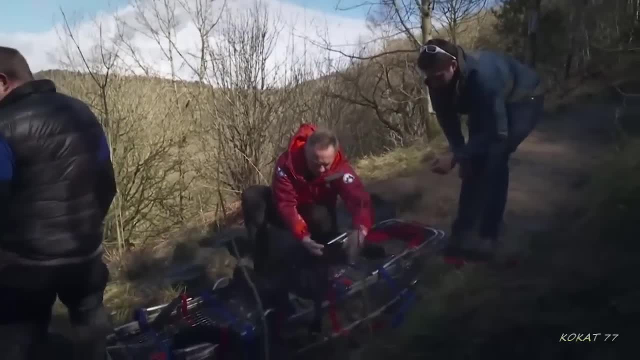 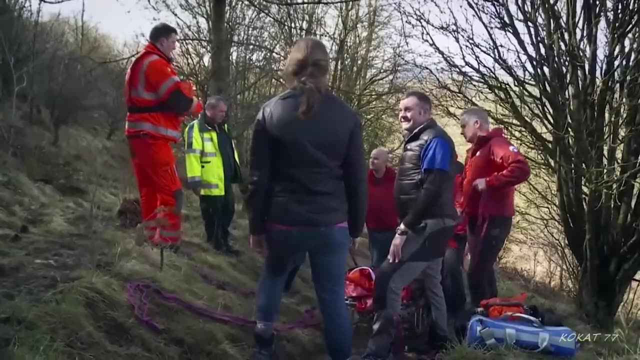 Slide the stretcher in down, clip up, load and go. That sounds good to me. You're the experts, But the ground is lethal. You all right, Yeah, yeah, good, You all right, John. Hey, Prepare to raise and raise. 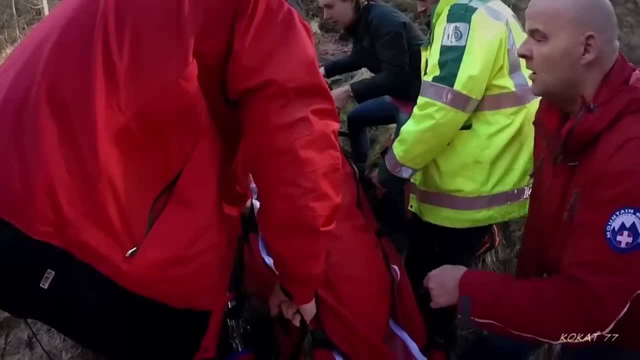 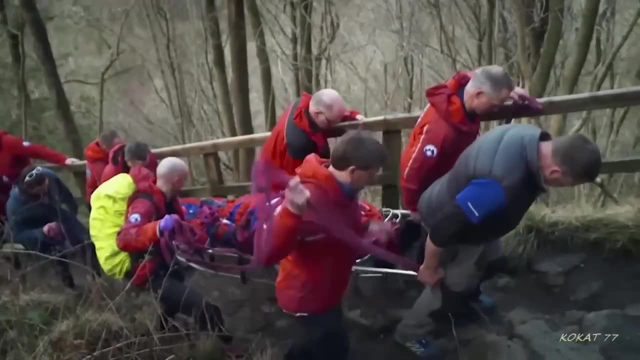 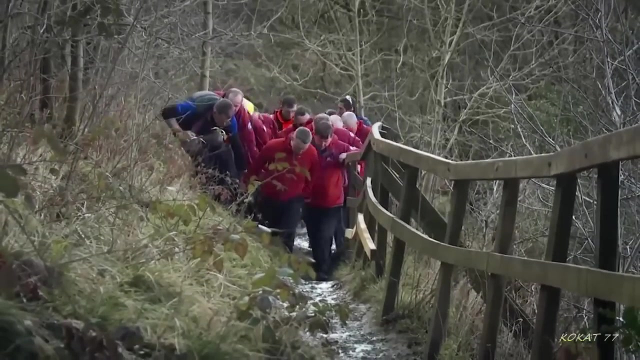 Well done Judith. Good lad, And better, lower and lower. They're going to use their specialist stretcher to carefully carry Judith 200 metres through the woods up to the chopper. The Helimed team can call on seven Mountain Rescue teams. 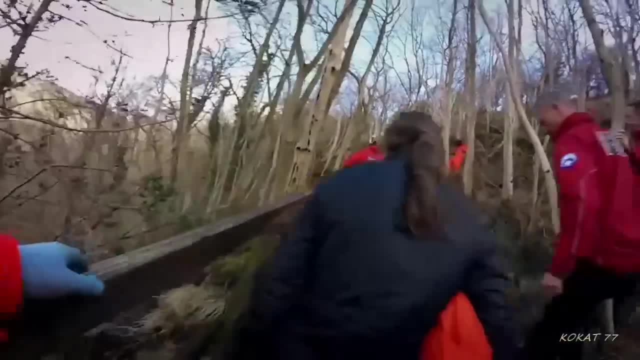 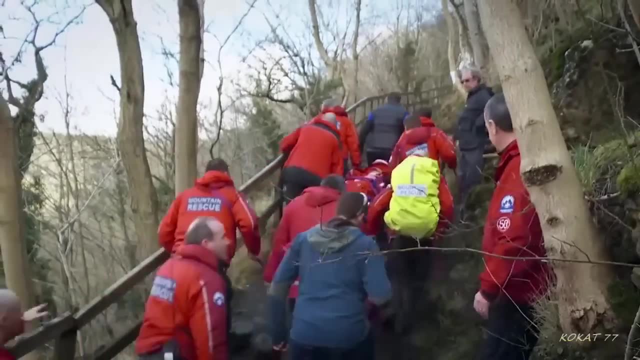 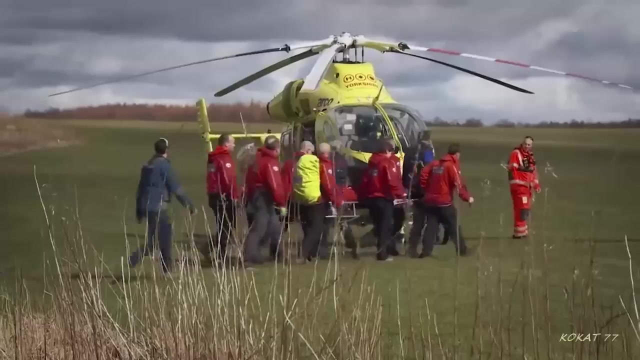 all volunteers who turn out from home or work Fade in on the sides. Without Mountain Rescue's help this would have been a risky journey And we get to see Sunshine Judith's reached safety OK tug and glider out at 2 o'clock. 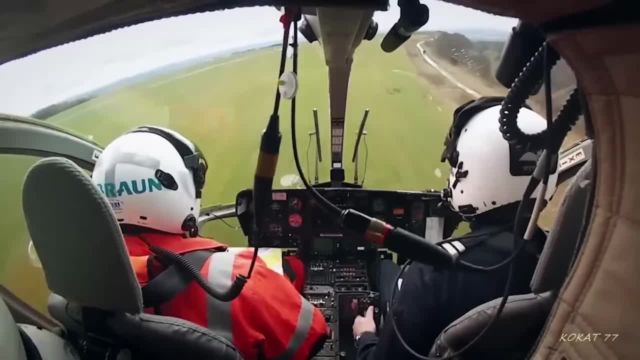 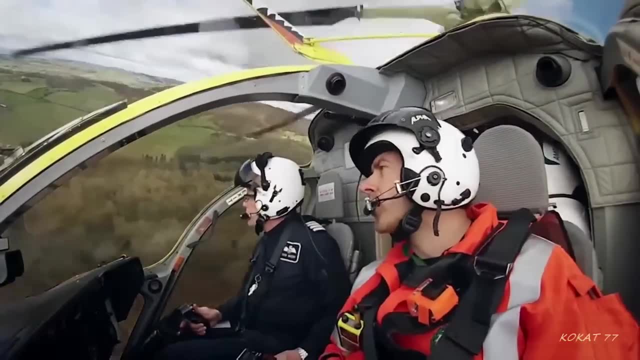 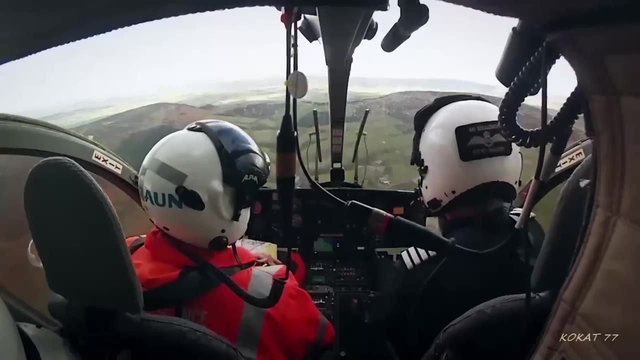 Back radio ahead of medical. And turning to the north Pilot Steve's anxious to get his patient to hospital before the weather turns again And it's still making its presence felt. Oh, some hailstone look. Oh big pieces. There's a lot of hailstone. 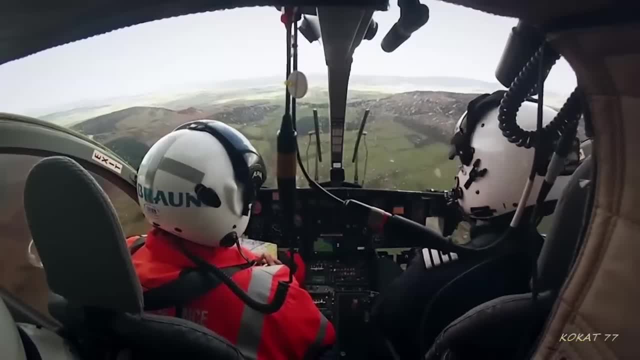 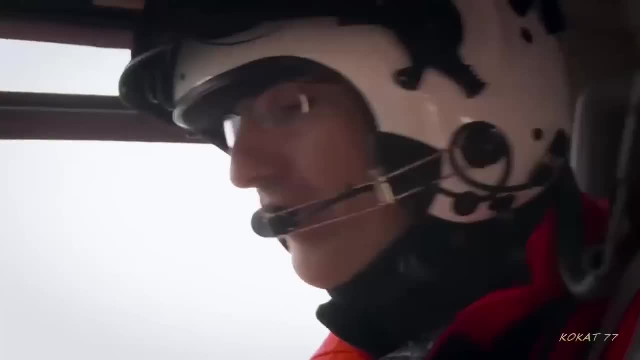 There's a lot. look, Wow, Won't be long, Judith. All right, though. Yeah, Helimed 98, Listerd routed, James Cook. They are heading north 20 miles to Middlesbrough. Surgeons are waiting to assess Judith's injury. 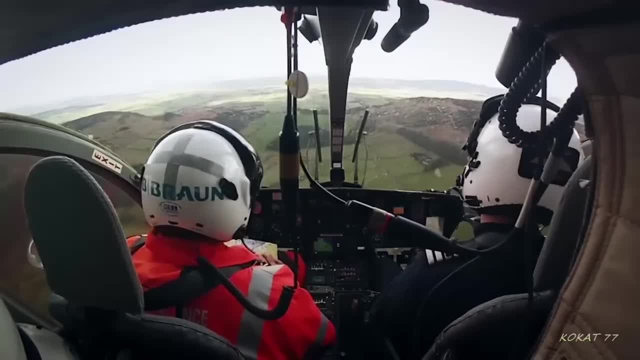 Helimed 98, send us wind, 260 degrees, 11.. Thank you, Judith's hill-walking days may be over. It's just a matter of time before she can get back to work. She's got to get back to work. 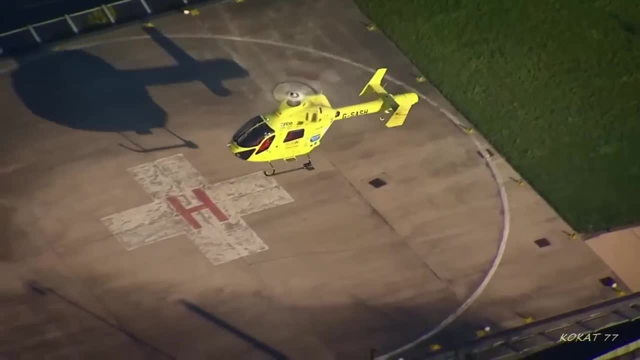 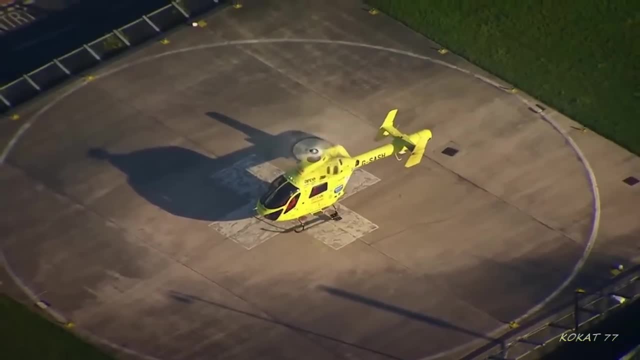 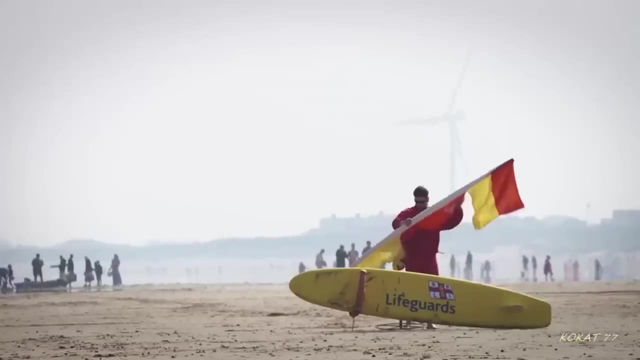 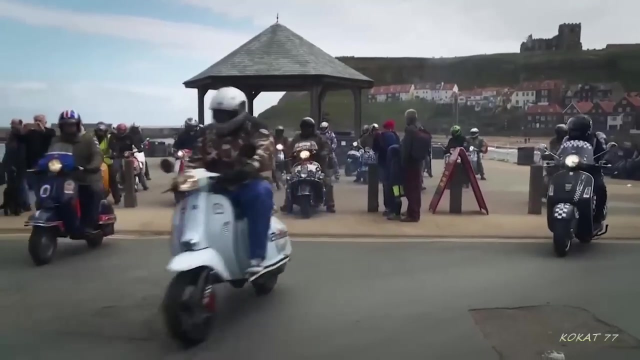 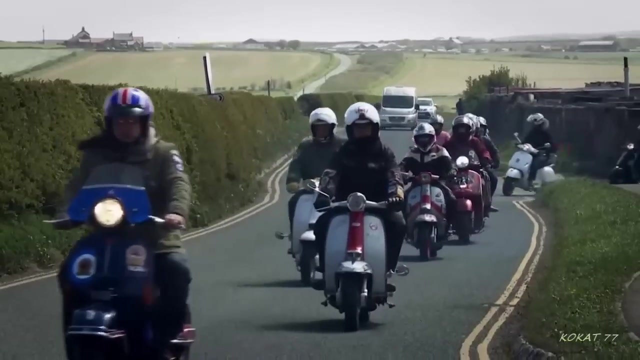 Judith's hill-walking days may be over. Yorkshire's heritage helps drive a tourism business worth £6 billion a year, But there's one group of visitors who do more than most to bring history to life For the born-again Mods, the scooter is still king of the road. 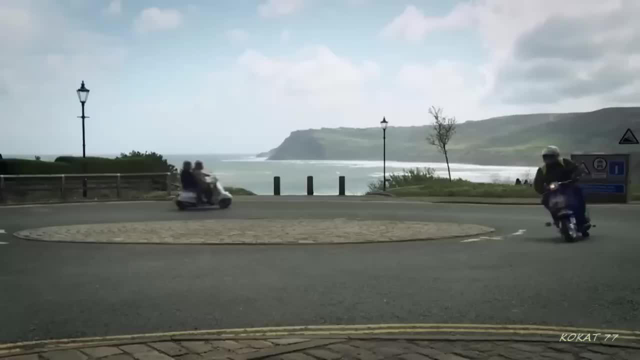 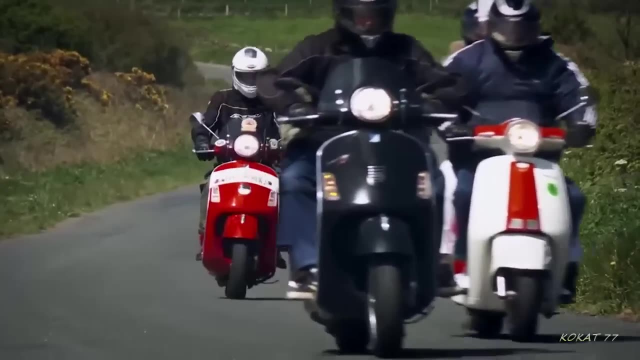 and parkers- the height of fashion. Vintage shirts change the world. It's hands for hundreds of pounds and a restored Lambretta can cost more than a car, But news has just come in to the Totcliffe base that a rider has come off in bad weather. 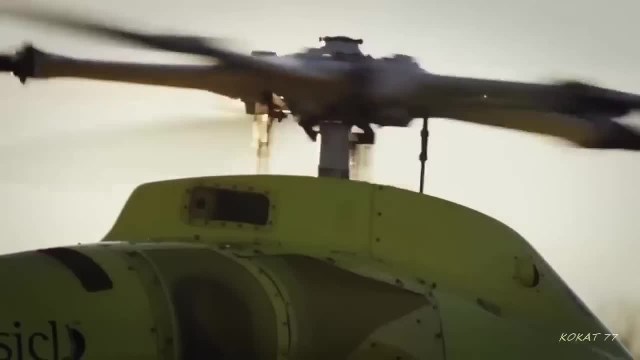 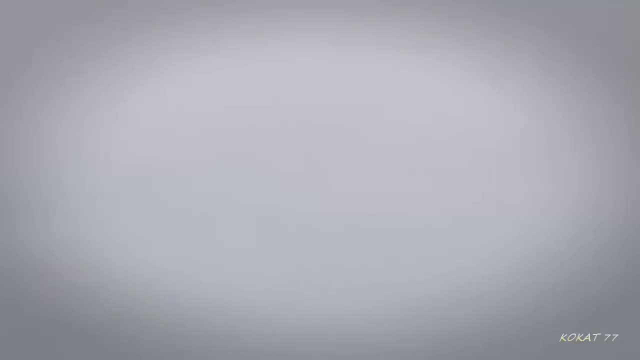 between York and Harrogate. Pilots Steve Wardby and paramedic Kit von Mikvits know that these cases can be serious. I've got rains at junction 47. That's all to affect it. Yeah thanks, I'm just going to go. 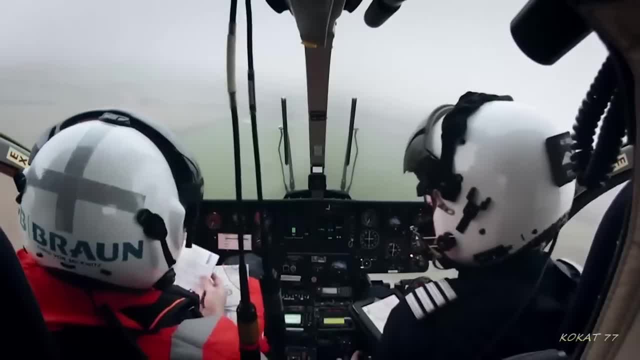 and see where he's left. Oh, DCA there at 11 o'clock. Ah yeah, roger. Oh yeah, he's on the bend. He's lost it on the bend Right. We'll come down onto that patch there. 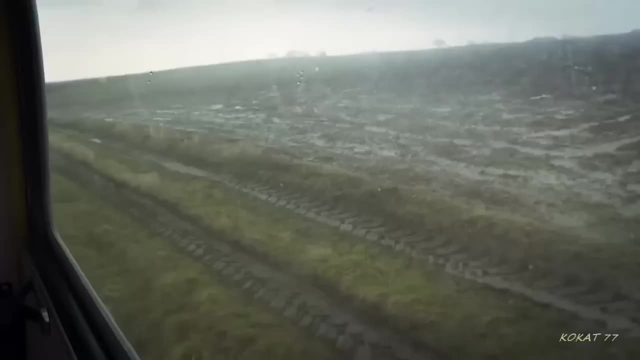 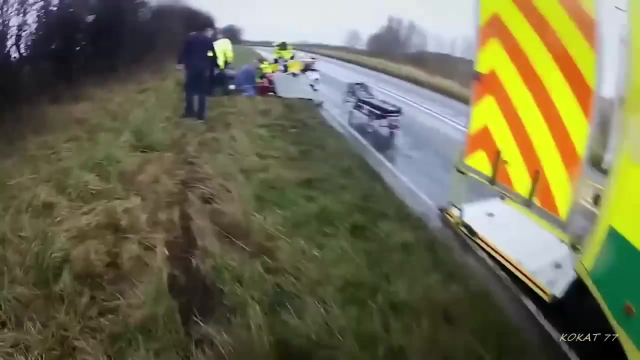 in the middle of 1 o'clock. Right, Thanks for that Puddle. There you go. Lead paramedic Paul is first out of the helicopter. He gets an update from local paramedics. Heyo guys, You all right. 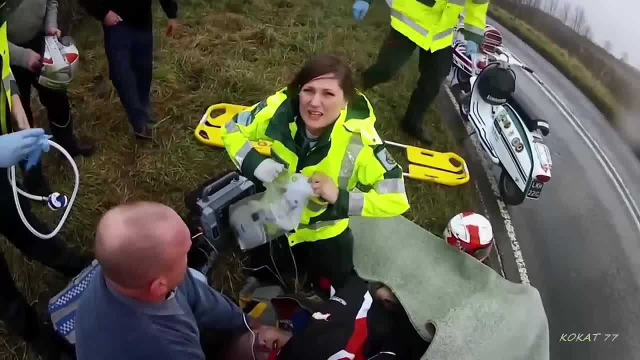 Hey mate, You all right. This is Steve. He's come off his bike. OK, I've got good air entry, I've got no radio, but I've got a carotid. Steve, where's it hurting mate. 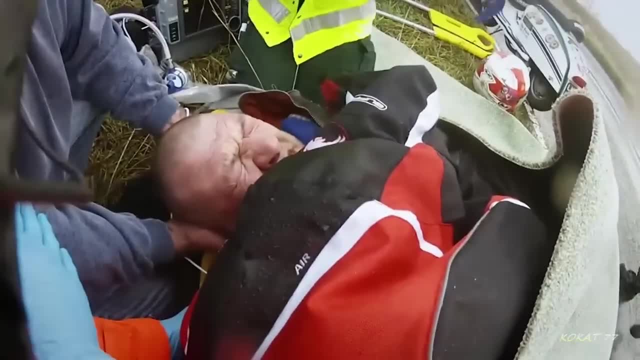 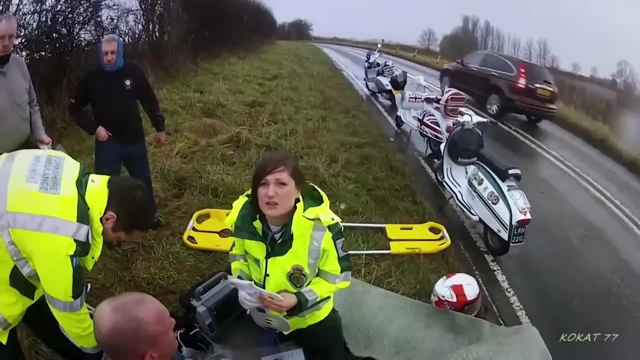 In my back, Right in your back, I mean absolute heaven. I can imagine mate. So what's that pain? now, on a scale of 0 to 10?, 10. 10? You can feel it crunching. You can feel it crunching, can you? 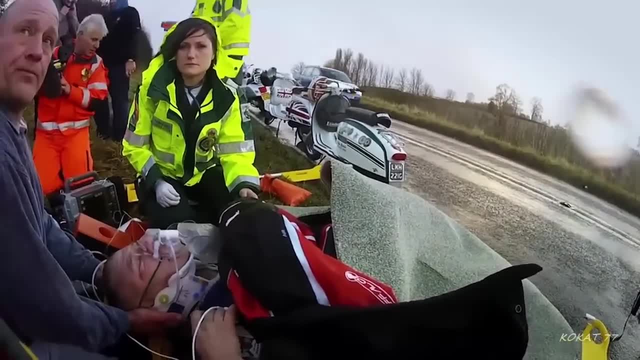 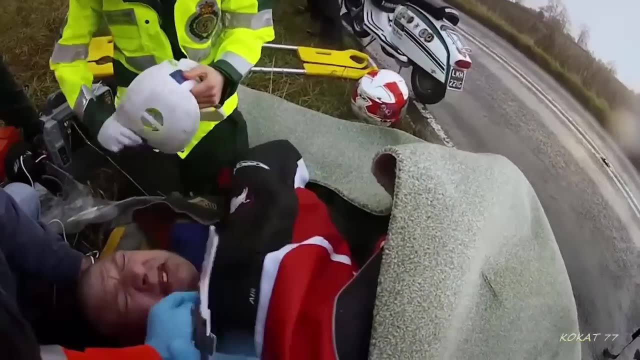 49-year-old Steve Campbell's description is graphic and worrying. His restored scooter is badly damaged, The weather is atrocious, There's mud on the road and he came off on the bend. He did have a bit of blood in his mouth. 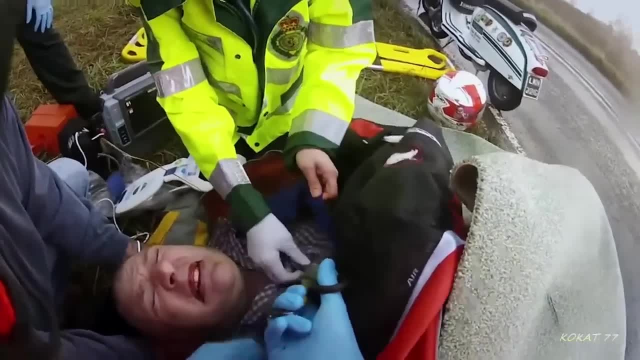 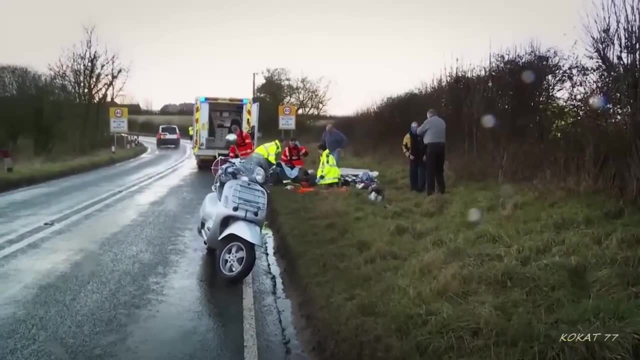 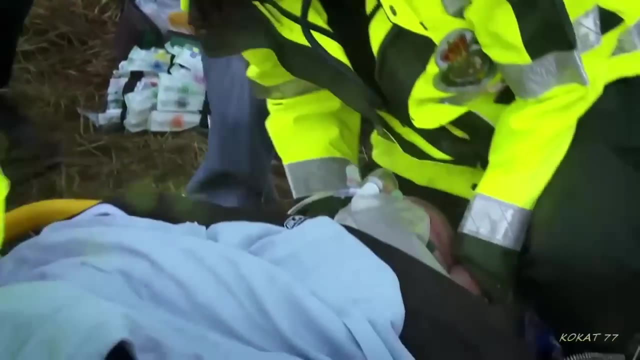 And he's got chewing gum, which I've removed. Oh, OK, No loss of consciousness or anything like that. No, it says no, Right, OK. Steve was on his way to a scooter rally when the accident happened. The crunching sensation in Steve's back is called crepitus. 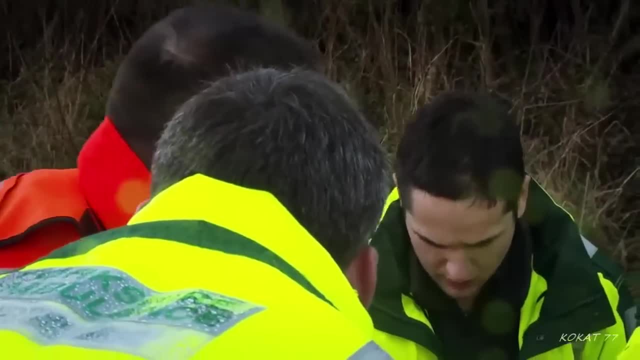 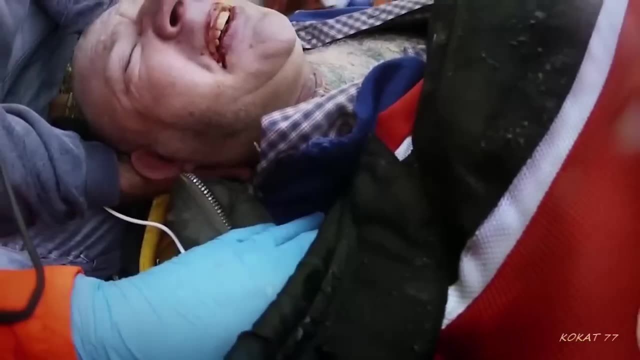 It could mean he's displaced the bones or cartilage in his spinal column. The team will have to be very careful when they move him. Steve, you know me fitting well. Eh, You know me fitting well, Yeah. Yeah, I think them stats are accurate, you know. 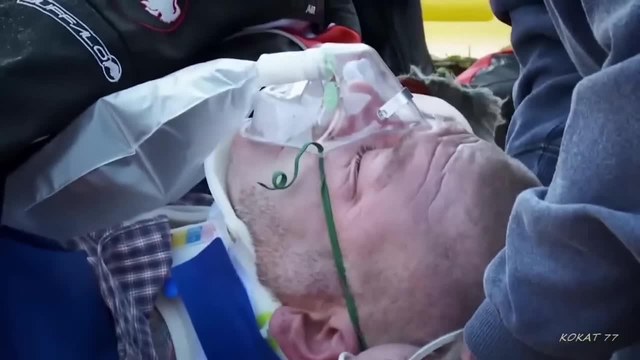 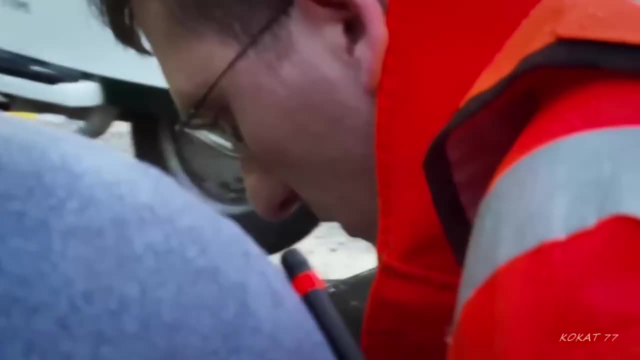 Looks a bit sad. obviously doesn't he. Stats are 84%. Where's that hurt? The amount of oxygen in his blood is low and his skin is blue. The cold isn't helping. They need to warm him up. I'm conscious he's going to become hypothermic soon if you're not careful. 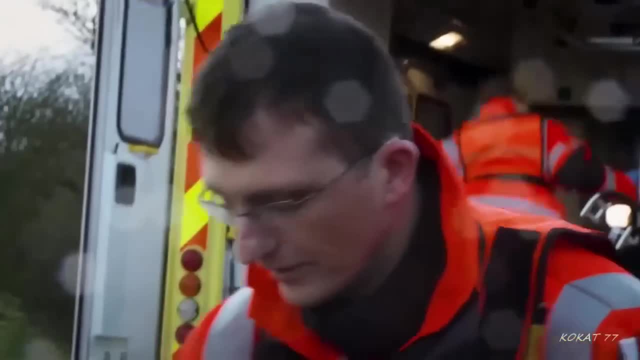 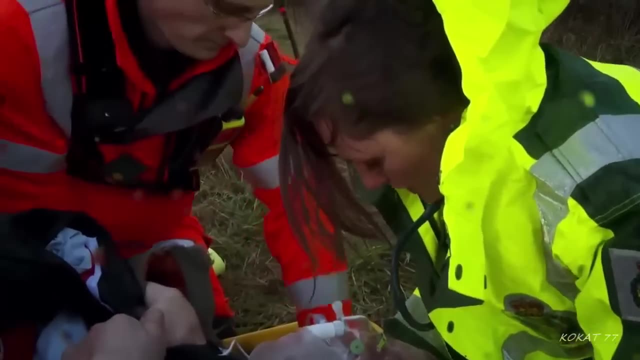 So we'll cannulate him in a backup wagon, Unless he's under a lot of pain as we start rolling him, then we'll just reassess him. All right, Steve, what we're doing is we're just going to be putting a scoop underneath your back. 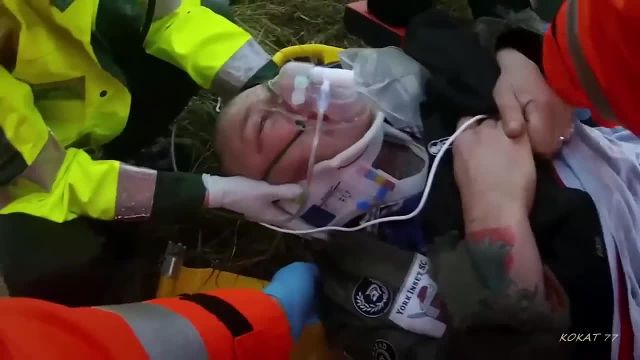 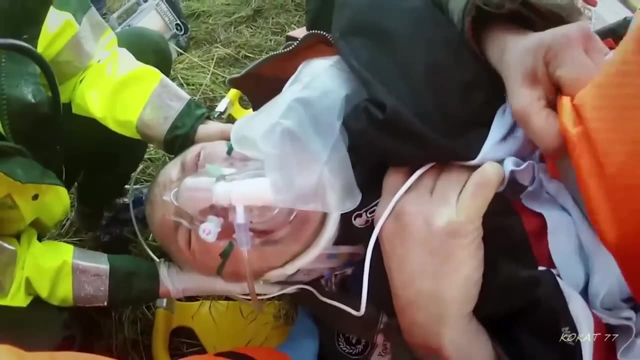 all right, This will be a roll and lift without pain relief. It's not going to be easy for patient. Steve, Ready Steady. No, All right, Steve, Well done. You're doing well, You're doing really well. 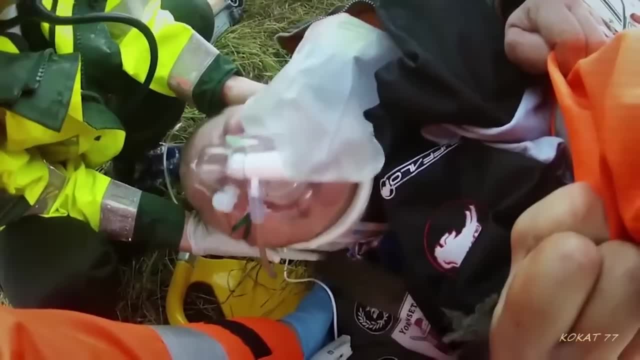 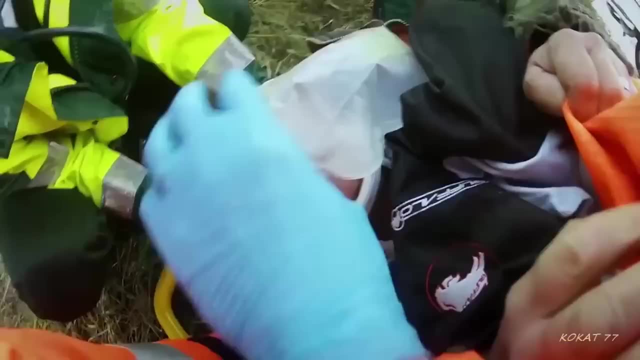 OK, No, It's just the board going under. It's just to get your. Just keep your head still for us. All right, OK, We're going to roll back. Well done, Steve. Steve, you're doing really really well. 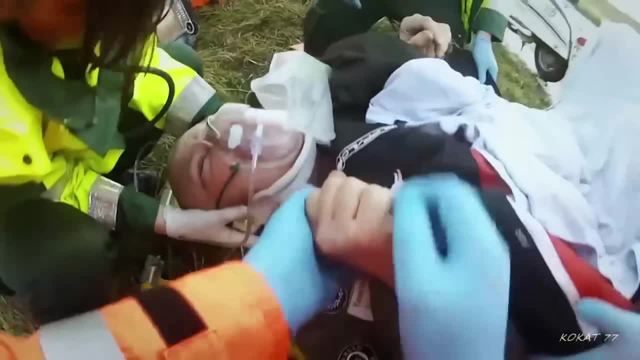 All right, You're doing really well. How are you doing, Steve? I'm painful. I bet it is mate, Just bear with us. The thing is, Kit, can you get some morphine drawn up? All right, One last one. 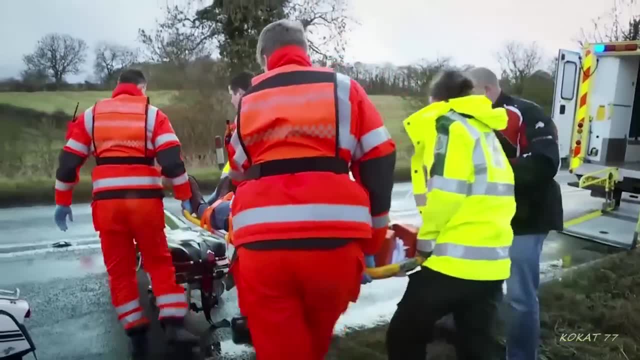 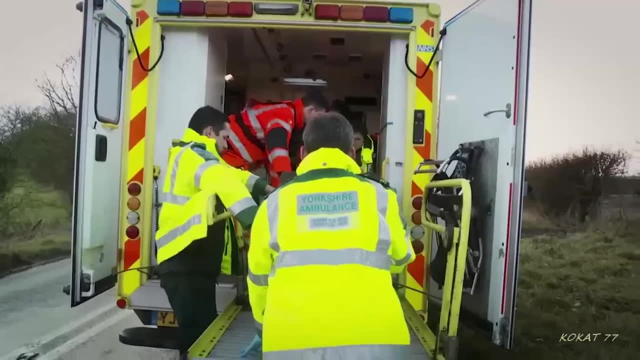 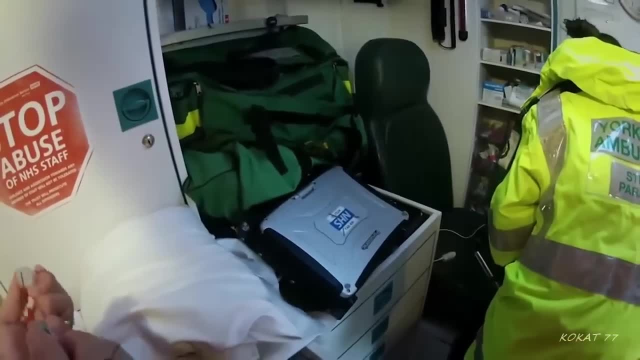 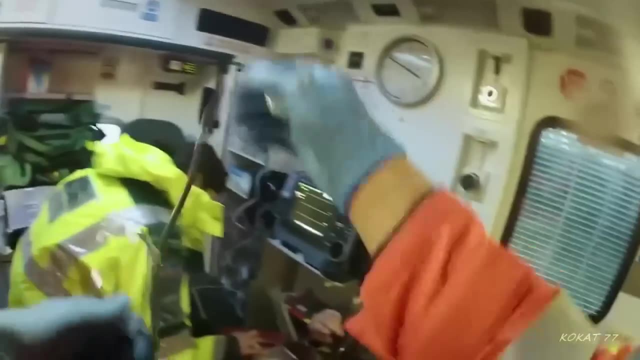 You. all right, He can now get the pain relief he badly needs. What's wrong? Where am I? You're on an ambulance. Ketamine is a powerful and effective drug, but it can leave the patient confused. All right, Steve. 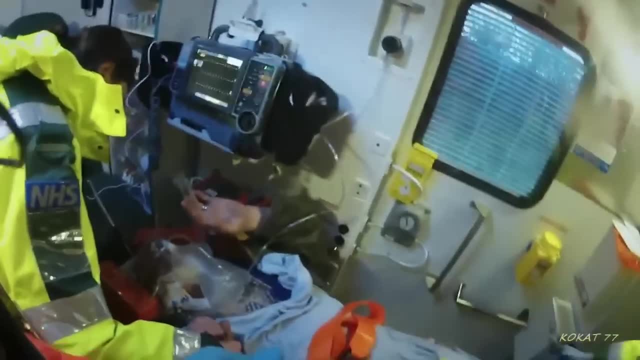 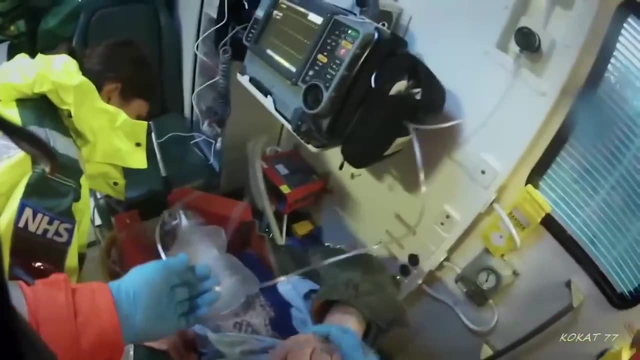 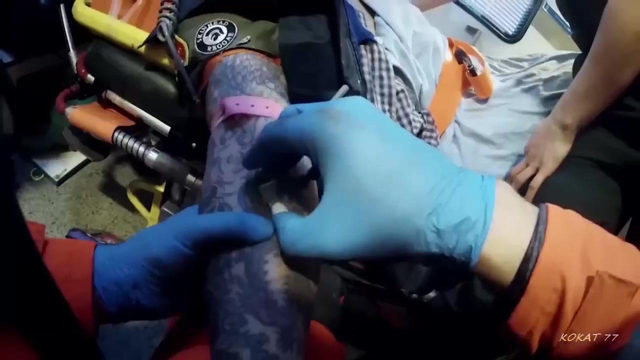 You all right. What's wrong? I'm scared, You feel scared. You're on an ambulance now and we're going to look after you. OK, He does feel some crepitus, some movement in his back, movement in his back. so obviously that's a big concern really, because if he has done, 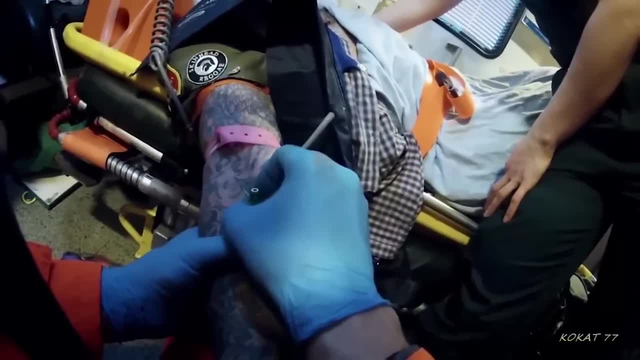 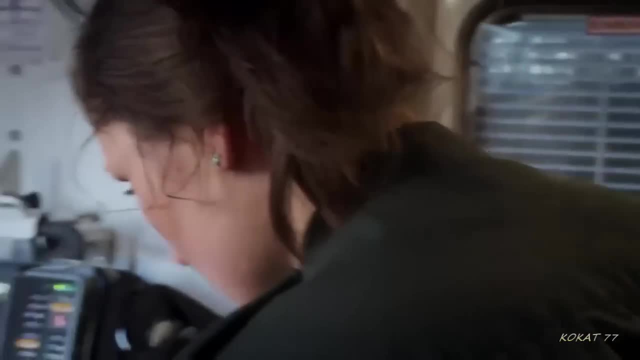 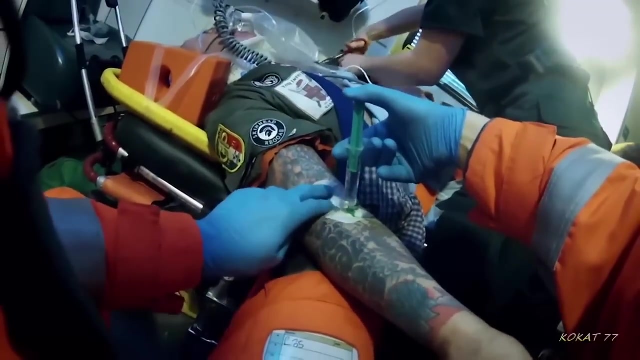 anything significant. the more we move him, the more damage it's going to do potentially. Right, Steve, I'm going to give you some morphine. Can you do me a favour? can you lean on this side? can you just cut that other sleeve off? No, not the jacket, Sorry, mate. Oh no, What's? 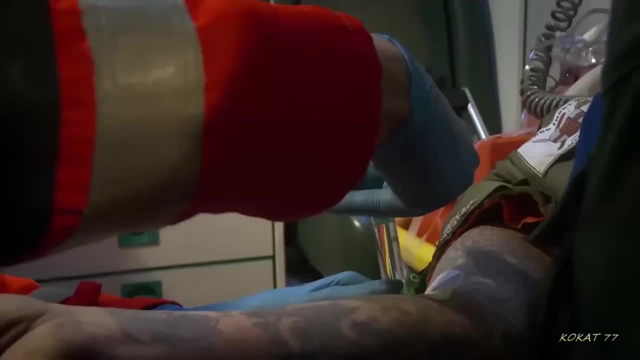 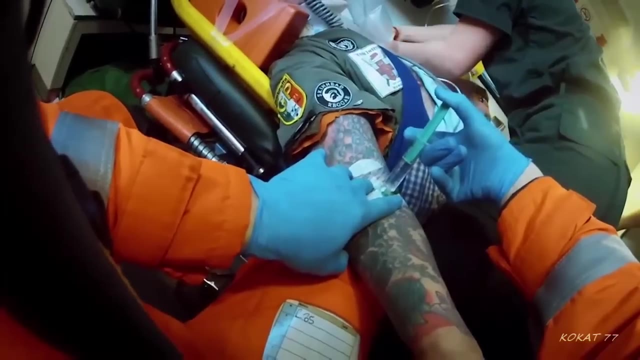 wrong. Did you get your back? No, my jacket. Why are you going to have to cut that off? I'm afraid we did mate. if we could have saved it, we would do, but that's the least of his worries at the minute. 40 year old that jacket, And you just sliced it up And I've just cut. 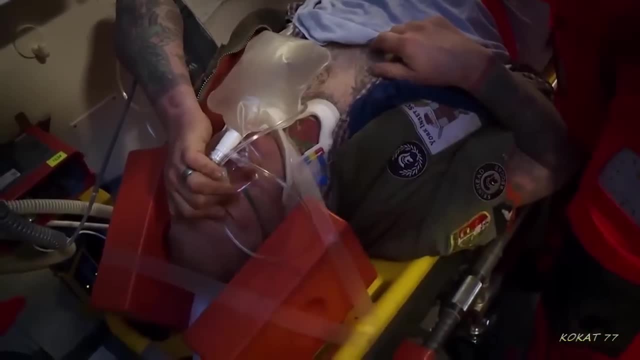 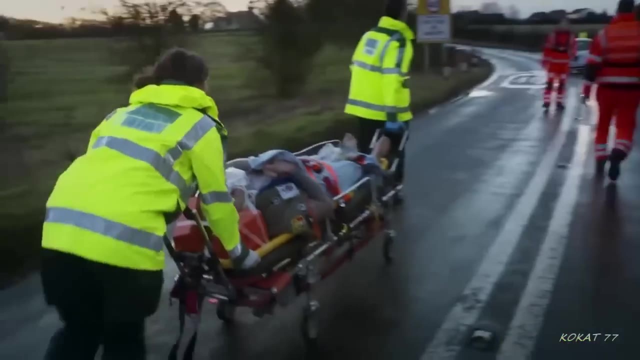 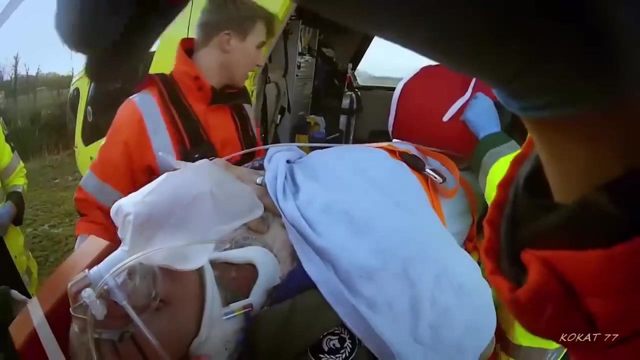 it off. I've ruined his day, If it wasn't ruined already. Steve's going to be flown to the Leeds General Infirmary. I need to go further on kit, I think. Has that done anything for your pain at all? No, it hasn't done anything for my pain at all. I'm going to have to go. to the Leeds General Infirmary. I need to go further on kit, I think. Has that done anything for your pain at all? No, it hasn't done anything for my pain at all. I'm going to have to go to the Leeds General Infirmary. I'm going to have to go further on kit, I think. Has that done anything? 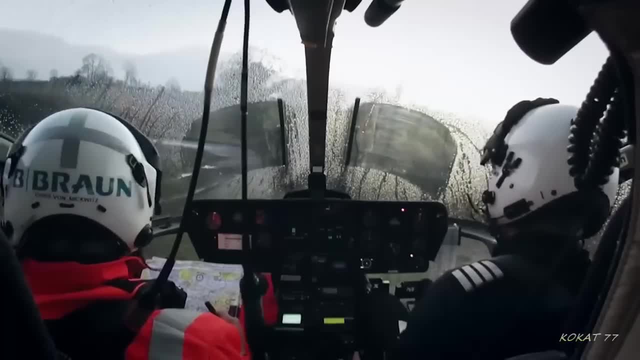 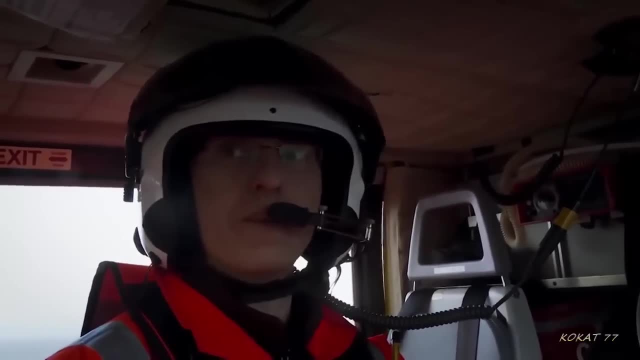 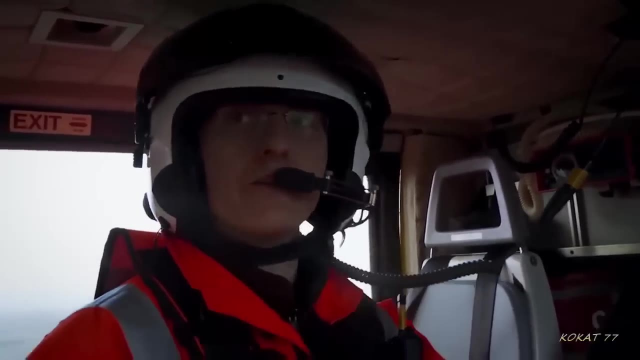 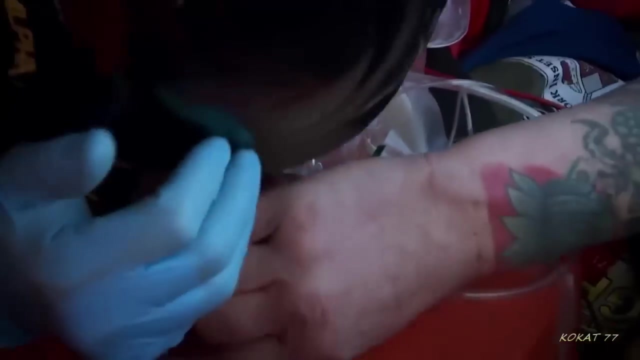 for your pain at all. No, it hasn't done anything for my pain at all. I'm going to have to go to the Leeds General Infirmary. I'm going to have to go through a full skin treatment. Here we go. 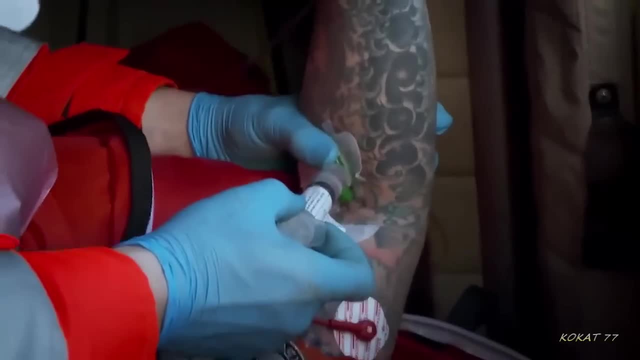 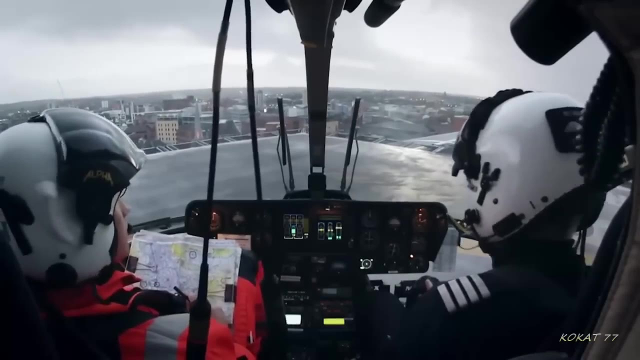 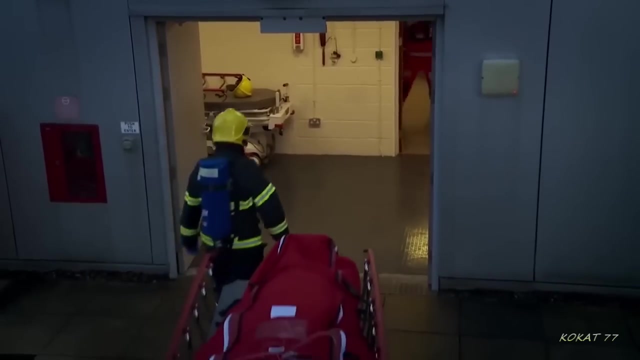 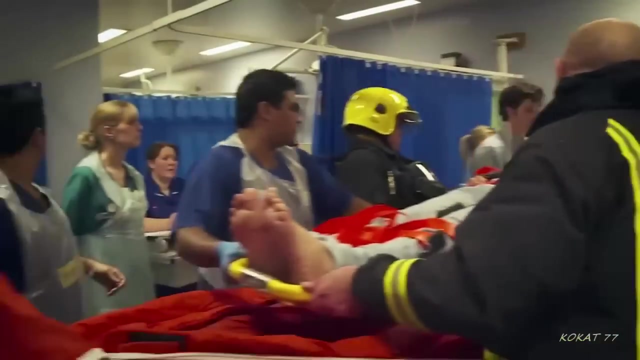 It's still in a lot of pain. It's blood so And it's not 900 LGI. Steve's taken straight to RESOS to be examined by a team of specialists. Scans reveal why he's in so much pain. 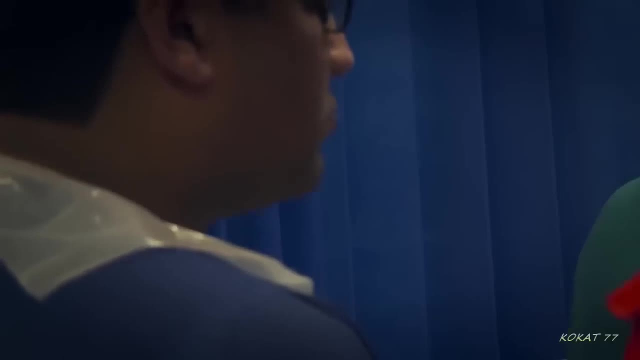 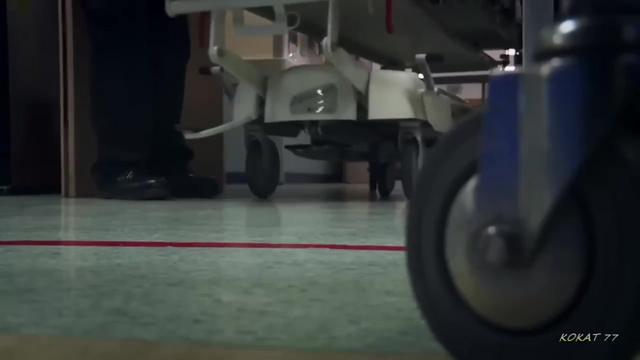 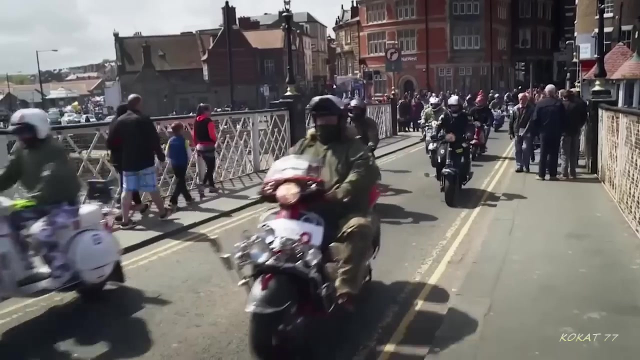 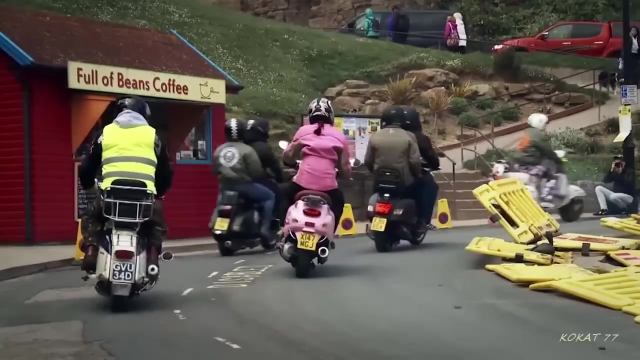 His back is broken in three places. Steve had major surgery to stabilise his spine, but serious complications meant he spent six weeks in hospital. He's now home and making a good recovery, but his scooter-riding days are behind him. Judith, the woman who slipped on ice near Sutton Bank. 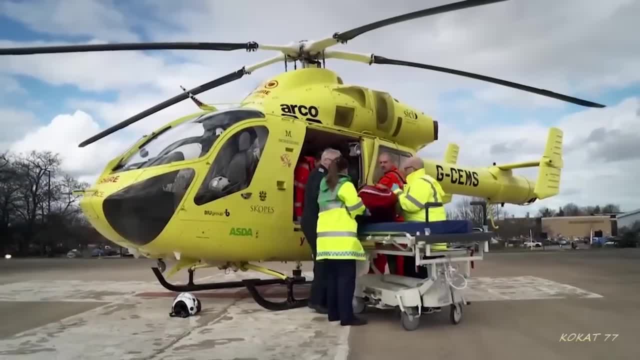 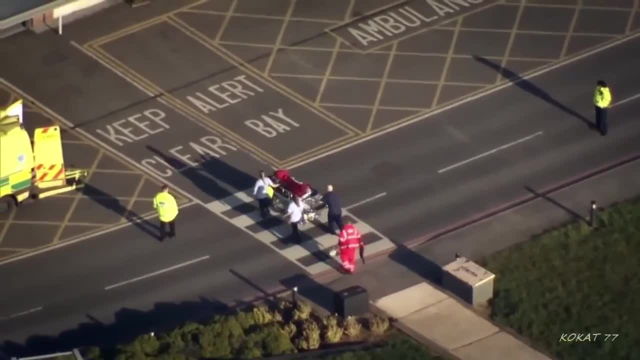 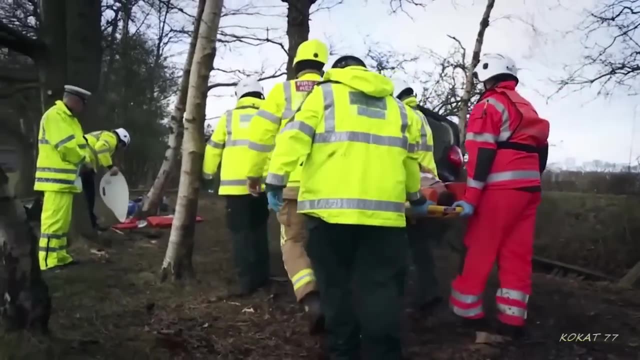 was taken for treatment. She had dislocated her knee and broken her leg. She was in plaster for six weeks and will need a replacement knee before she attempts any more. hiking. Martin, who embedded his car in trees, broke three ribs and fractured his wrist. 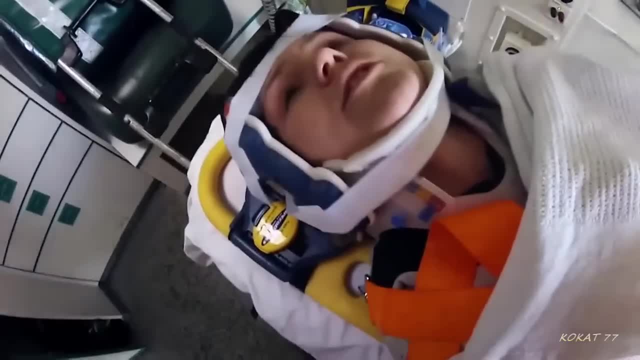 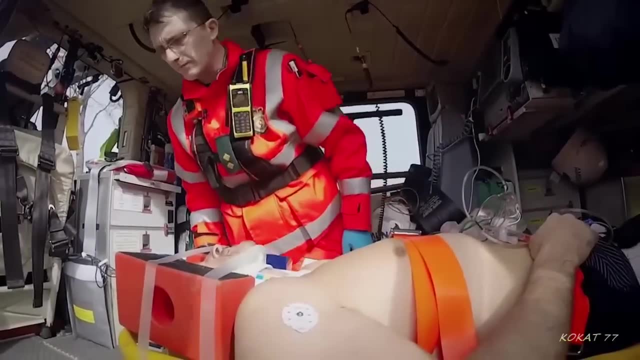 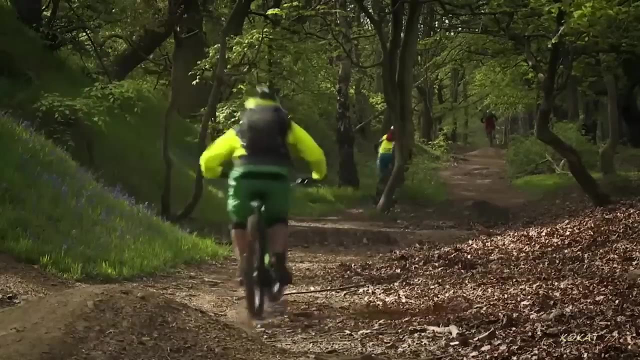 His girlfriend, Natalia, wasn't so lucky. She had to undergo surgery for a fractured neck, but is recovering well. As for mountain biker Rob, tests revealed he had also broken his leg. Three vertebrae are now bolted together, But he's determined to get back out into the woods. 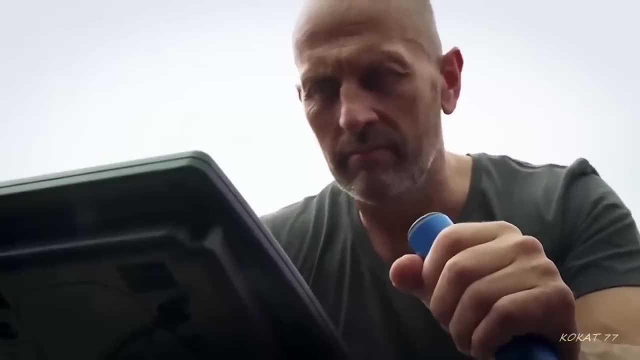 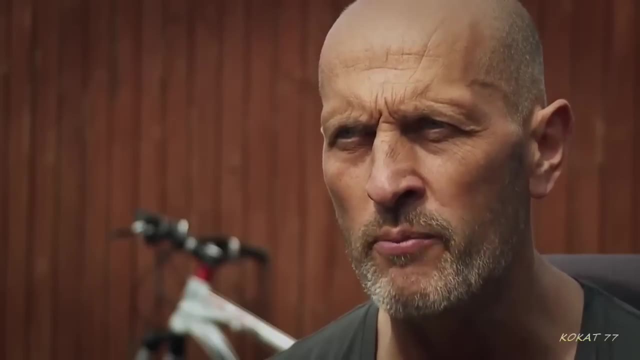 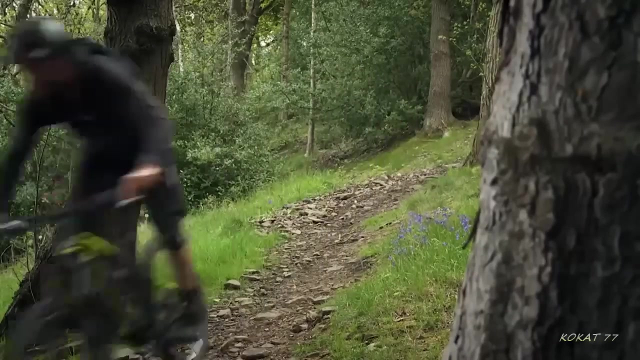 with his mountain biking mates. Only he's got a lot of recovery to do. first Ongoing I'm on physiotherapy to bring back my movement because I'd lost movement in my legs and strength in my arms. For the time being, the bike riding's out. 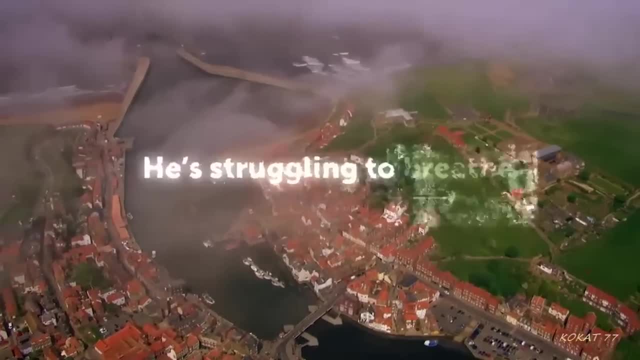 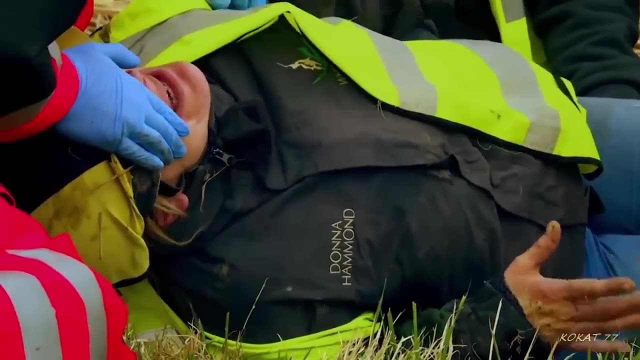 Perhaps it's got to. He's breathing. He's struggling to breathe, Very seriously injured In some of the UK's most remote places. Ow, ow, ow, I can't do this. Stay on the line and I'll tell you exactly what to do next. 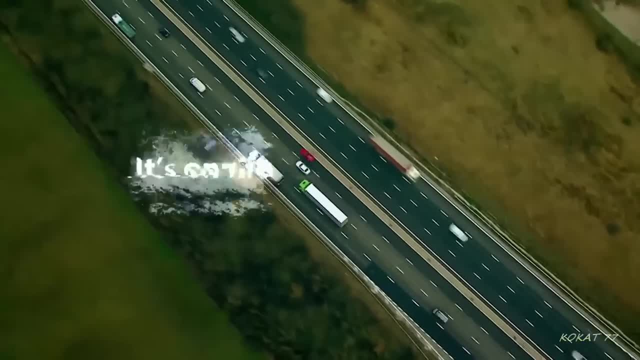 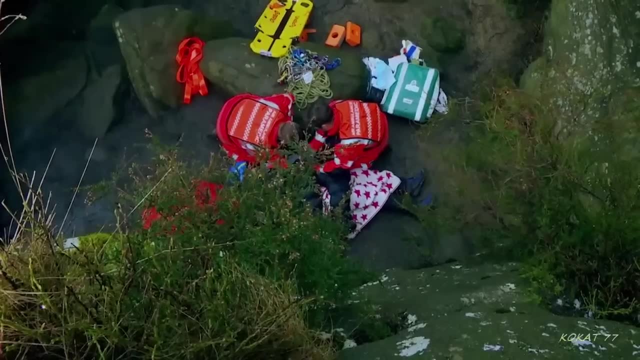 There's just been an accident on the M1 motorway. It's on fire and it's gone into the railway bridge. Your life is on the line. How far did he fall? About five metres. He's intubated and ventilated. 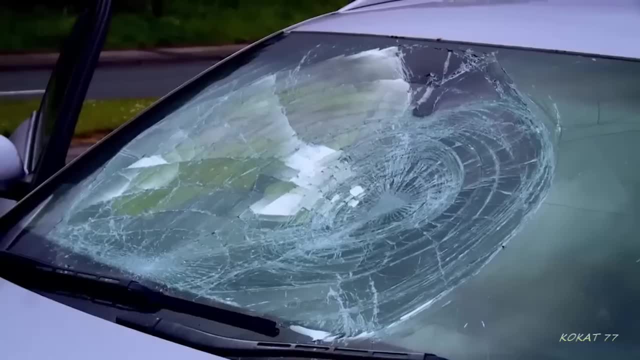 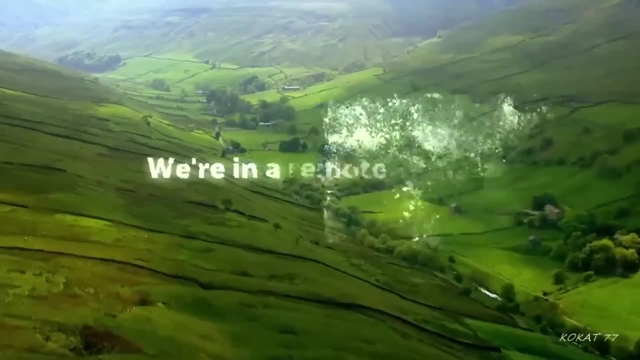 You need some of Britain's most elite medics. Is there any serious bleeding? Yes, there is. yeah, Calm- I can't feel legs anything below my neck. We're in a remote location in the middle of the woodland. 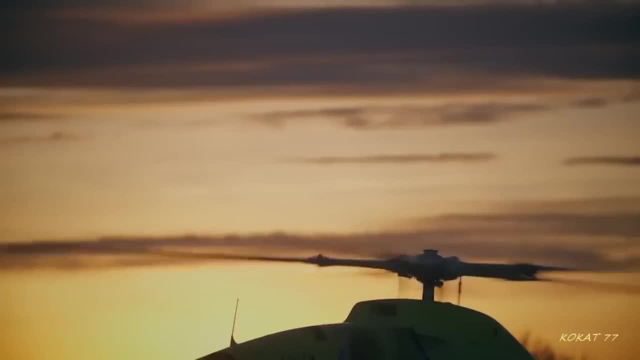 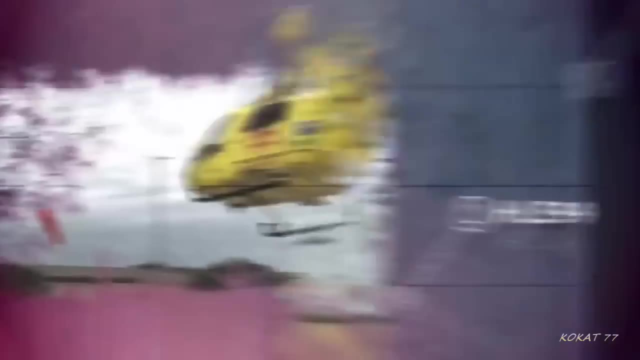 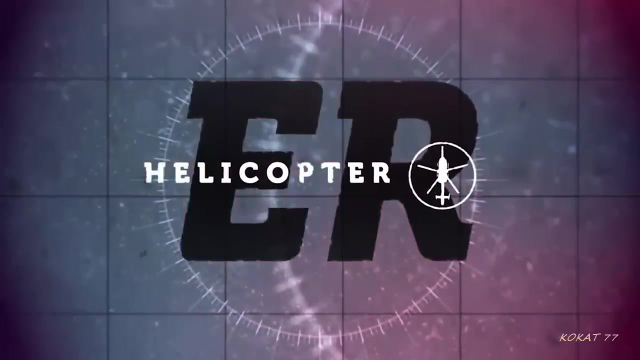 There's broken a bike. The speed of the Yorkshire Air Ambulance can make the difference between life and death. Your discretion to take off, Sir. there's no nine listed Today. there's a desperate fight to save a tractor driver trapped up to his neck in a lake. 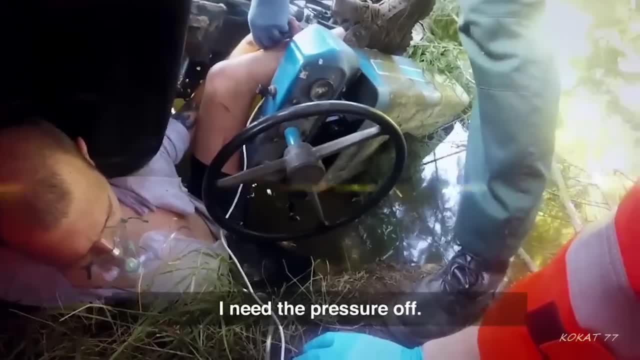 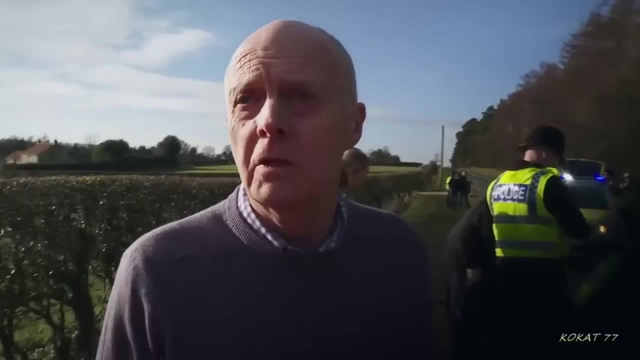 I'm sinking, It's pushing me forward And it cuts it off. The team's called to a badly injured biker who hit a 200-pound deer. He had no chance. He braked, came off and that was it. 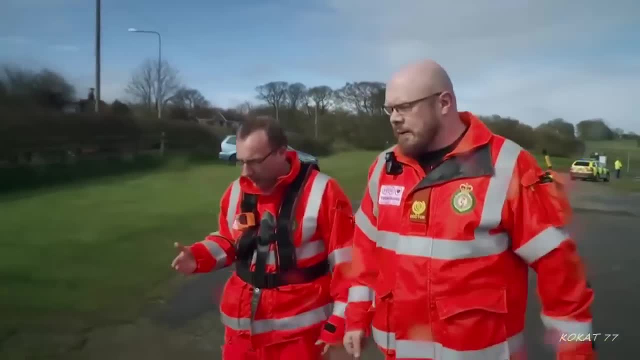 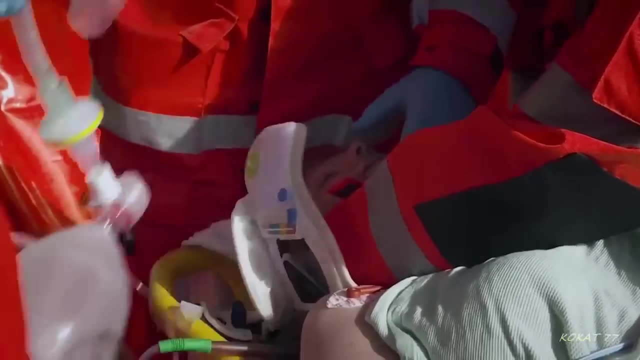 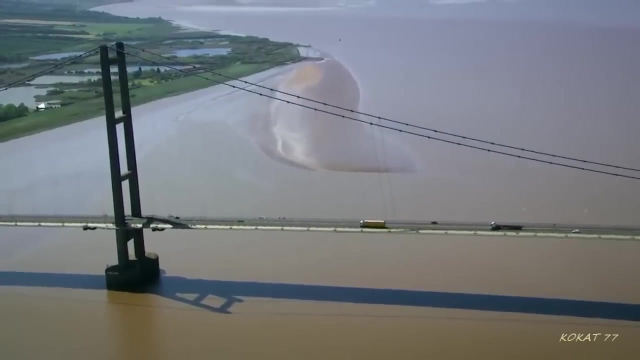 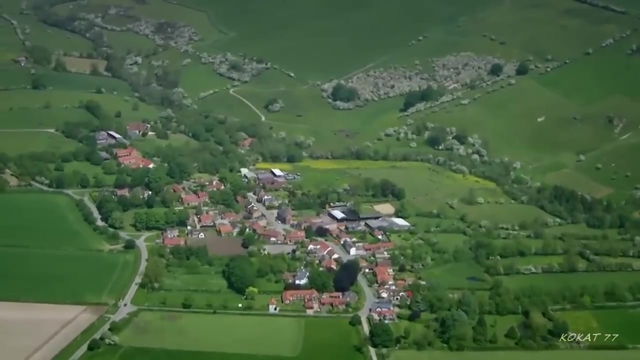 And flying doctor Andy is forced to anaesthetise a patient in the street. I'll give the drugs, I'll bag her gently during that time. OK, is everybody ready? Yeah, From a tiny hamlet on the Yorkshire coast, reports of a serious accident are coming in. 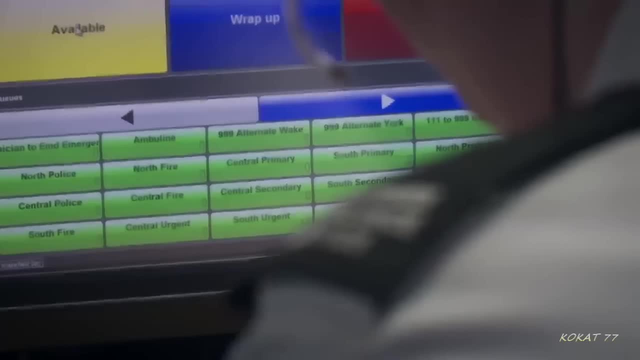 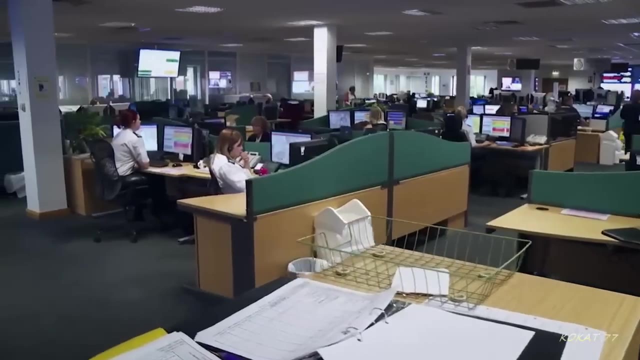 Ambulance is a patient breathing. 60 miles away in Wakefield. the man's life is in the hands of the 999 call takers at Yorkshire Ambulance Service Headquarters. He's stuck under a tractor in a corner. OK, tell me exactly what happened. 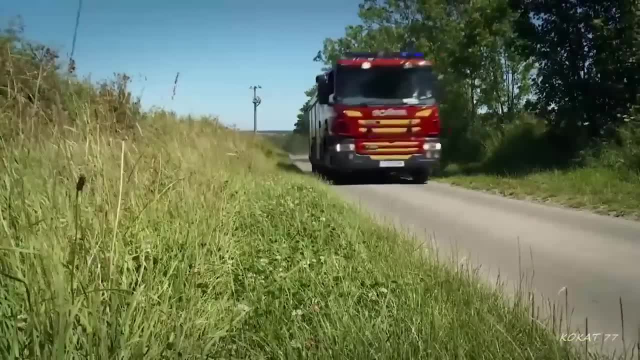 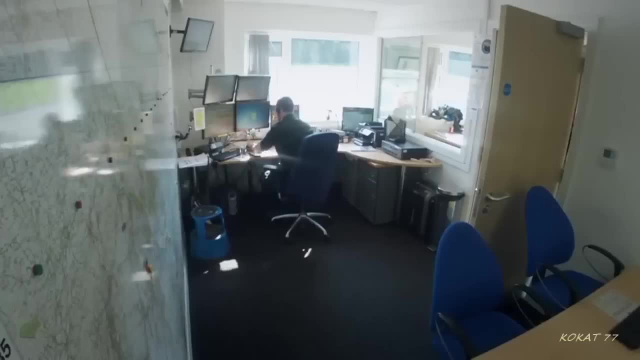 He's gone over a bridge and it fell off and he's stuck. WHISTLE BLOWS, WHISTLE BLOWS, WHISTLE BLOWS. Even before the caller has hung up, rescue will be on its way. Air ambulance dispatcher Jane Stubbley. 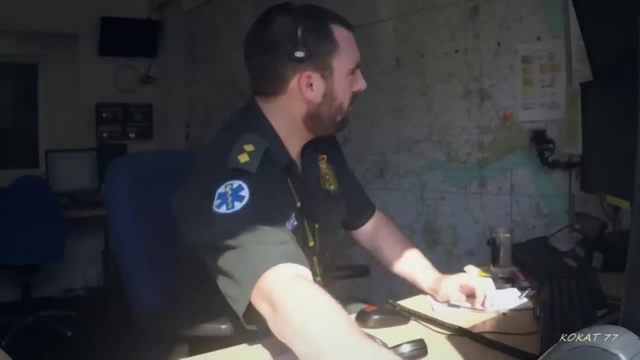 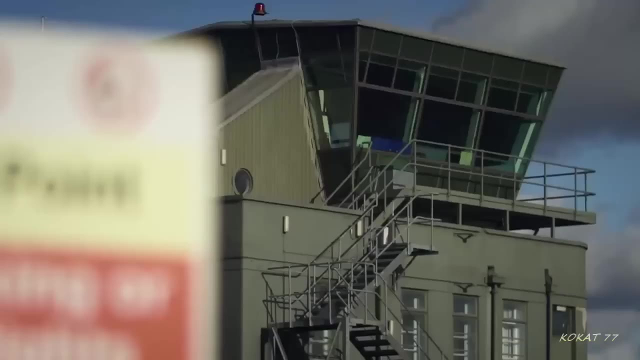 is listening in to the call. It's OK, sweetheart, We've got help on its way. WHISTLE, BLOWS, We've got spying here. We've got everybody on the way, Don't worry. Paramedic Tony Wilkes is being scrambled to the scene. 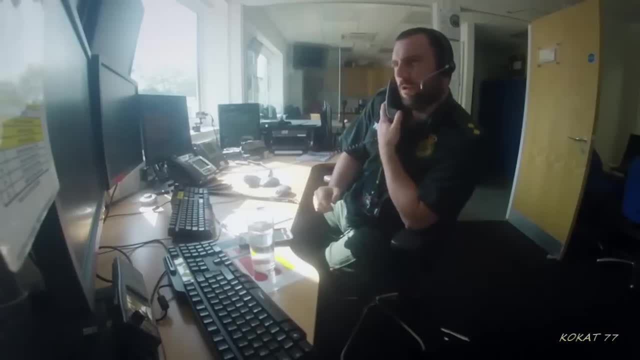 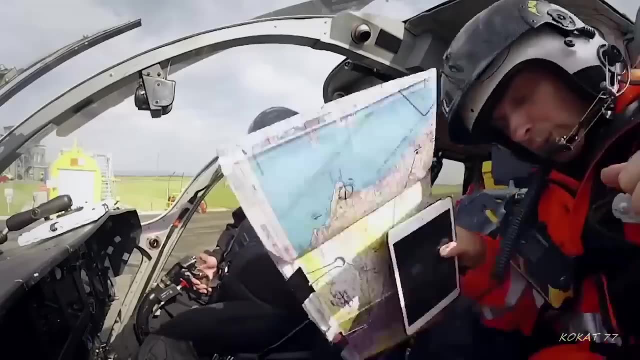 Top quick. it's time. Hang on, mate. Just watch Job 1845,. will you OK Start at a location We'll definitely go in because he's trapped underneath it. The details of the location are sketchy, but Helimad 99 is already on the way. 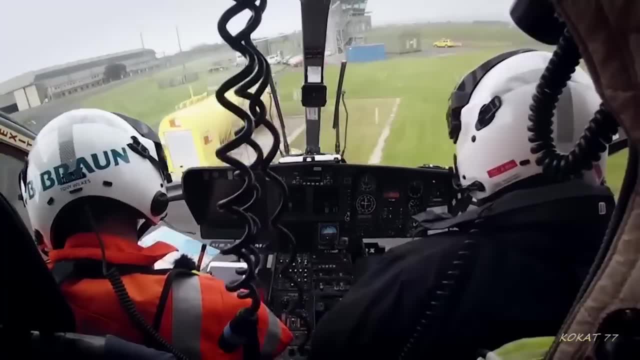 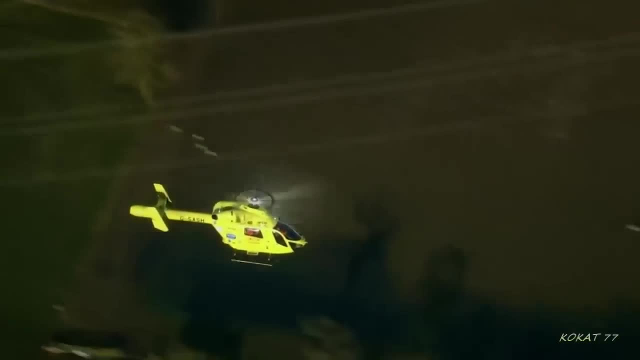 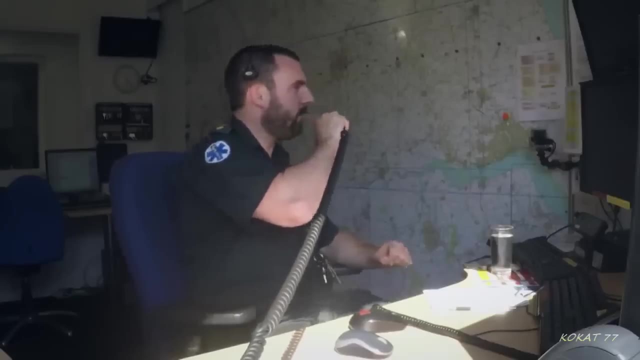 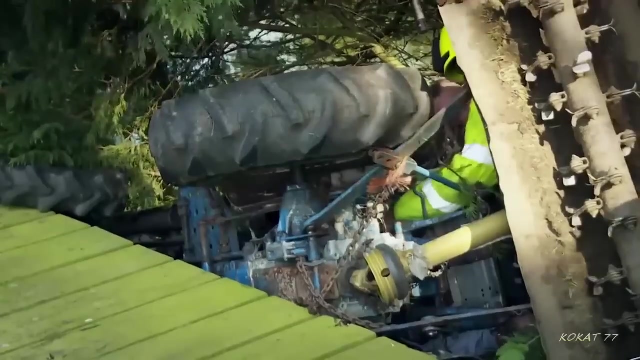 in just 15 minutes And they now know exactly where they're going. Tango Alpha 1905405.. 11855,. thanks for the mid-99.. The accident has happened on the banks of a fishing lake near the seaside town of Hornsea. 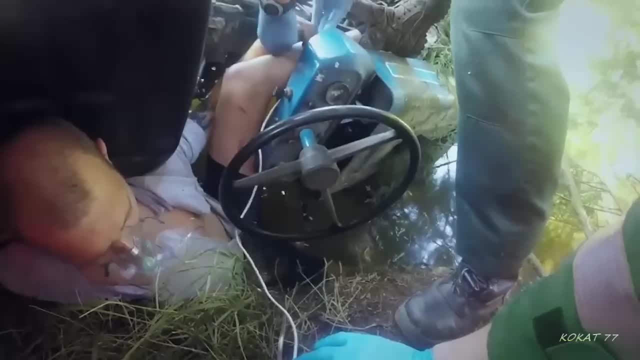 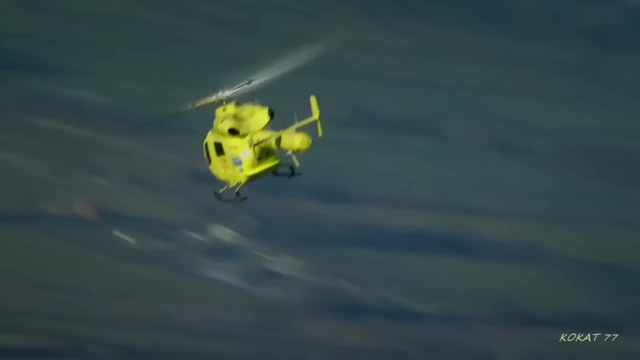 Local paramedics have now reached the man, but he's in a terrible predicament. Every second counts. The trapped man is in danger of drowning Once we get there. obviously, it's a case of actually trying to assess him while he's underneath the tractor. 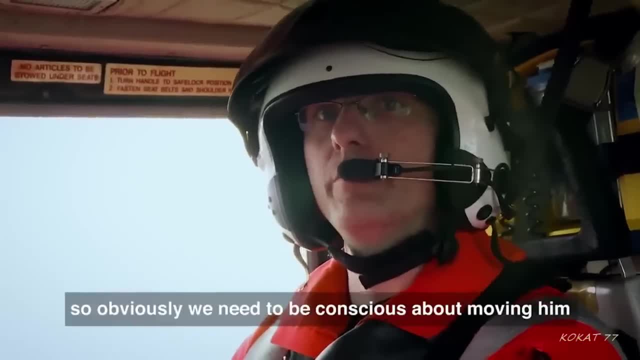 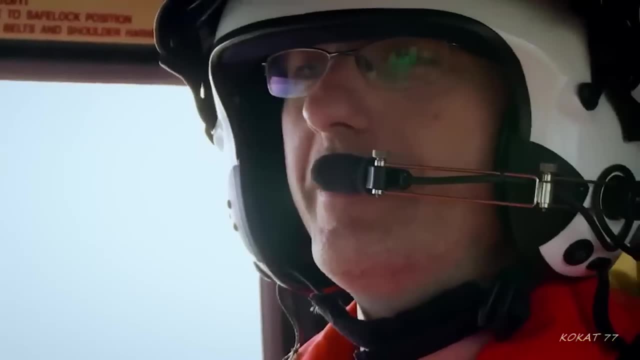 It's quite a heavy piece of kit, So we need to obviously be conscious about moving him, because he could have some significant major trauma. Yeah, Matt, they're sticking live jackets up. Paul, I know I was thinking that. Yeah, some water there at your 12 o'clock. 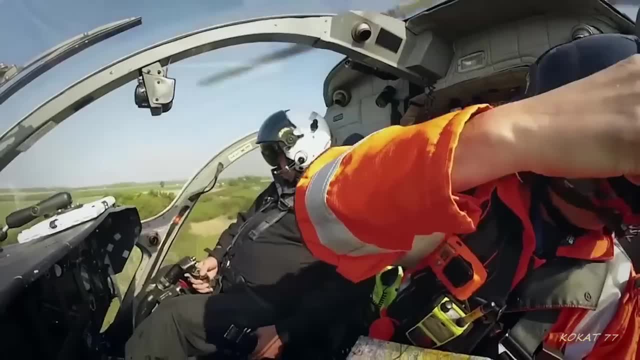 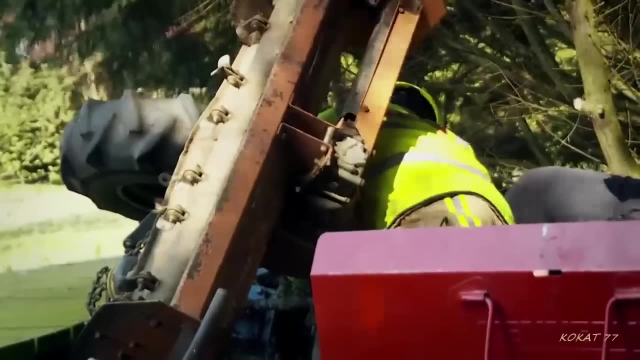 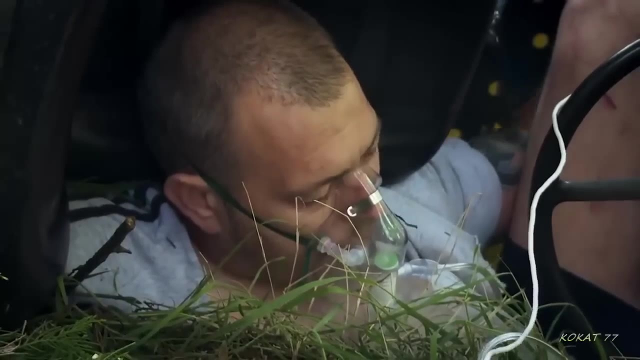 Yeah, that's from 99 over at sea. OK, clear, left 99 on the ground, Hey guys. Hey, are they all right? then Groundsman Sam Brockwell's mini-tractor plunged from the bridge, trapping him by the leg. 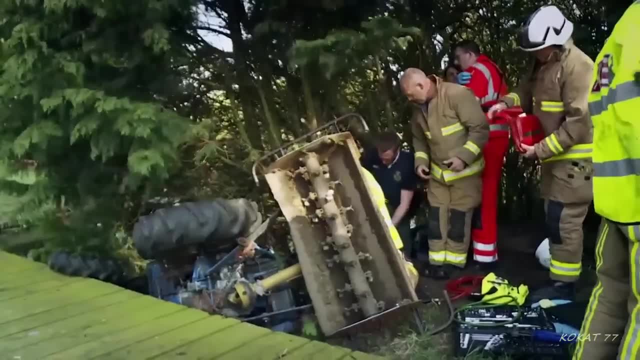 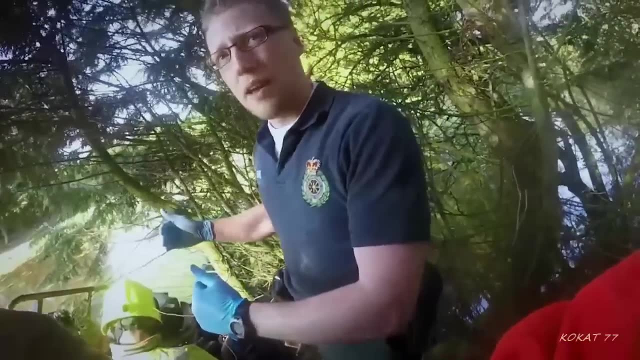 I've got a crew member trying to bring in a collar. All right, OK, I don't know what these guys are planning on doing. It's looking predominantly like it's the seat that's trapping him, but the seat seems to be supporting a lot of the weight. 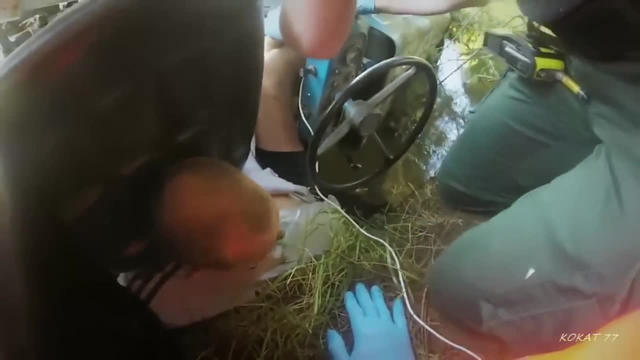 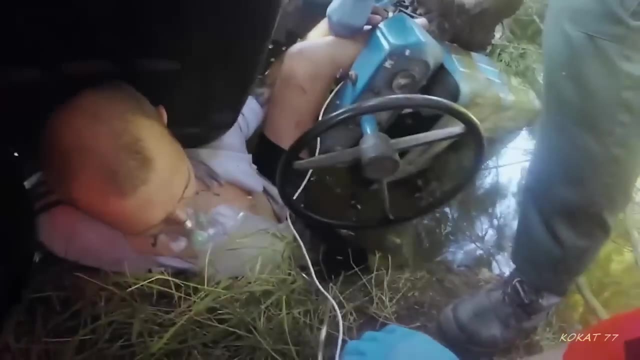 Only his head and shoulders are clear of the water and he's terrified. he's sinking deeper. Is his left leg right up in air, then Left leg's up there. It looks like it's quite an acute angle, doesn't it? 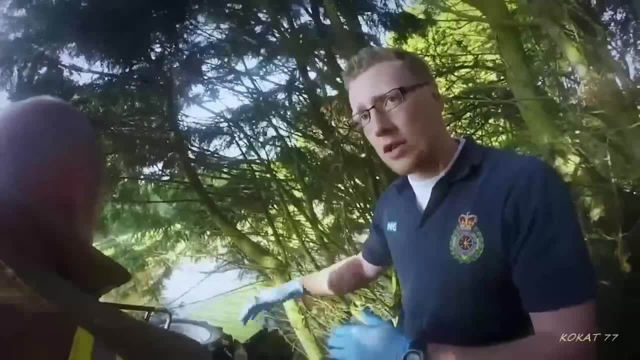 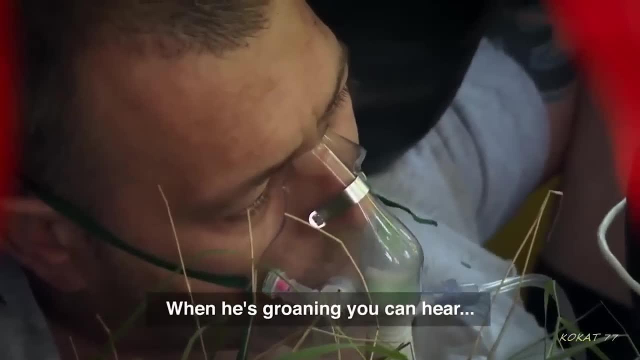 Yeah, yeah, yeah, Right leg he can move. That's not trapped at all. Right leg's quite free. That's under the water. Yeah, yeah, yeah, It looks like he may have a collapsed lung. When he's groaning, you can hear. 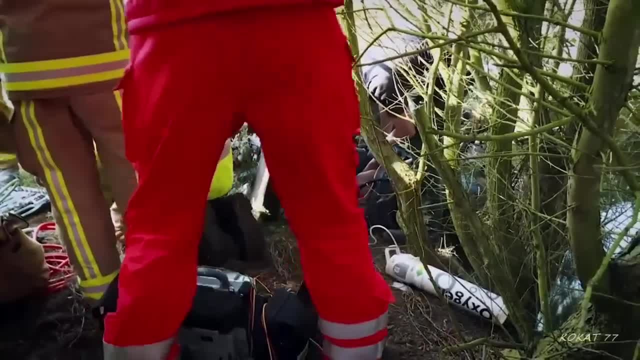 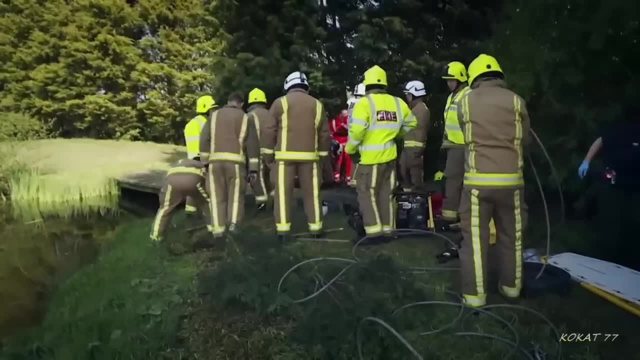 You can hear something. Yes, Right, OK, Possibly got some decreased air entering his right-hand side. Paramedic Paul knows Sam's life is on the line. If the tractor settles further, his patient will drown. Look, it's sinking. 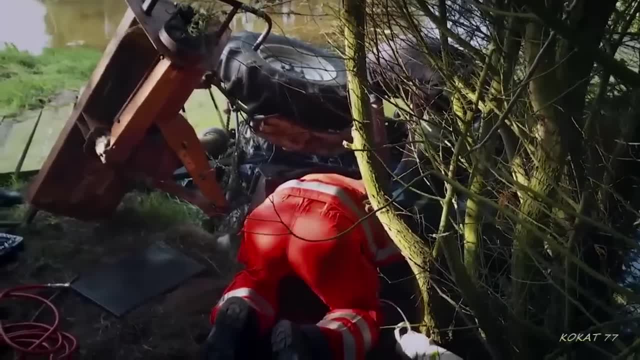 Right, listen, my name's Paul. I'm going to try and get you out as quick as we can. It's sinking, Pushing me further in. OK mate. He says he can feel the tractor pushing him further and further under water. 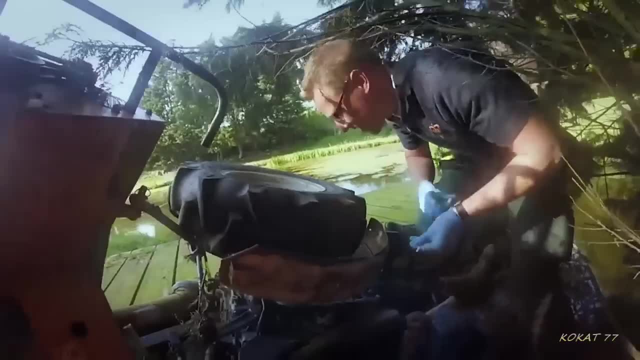 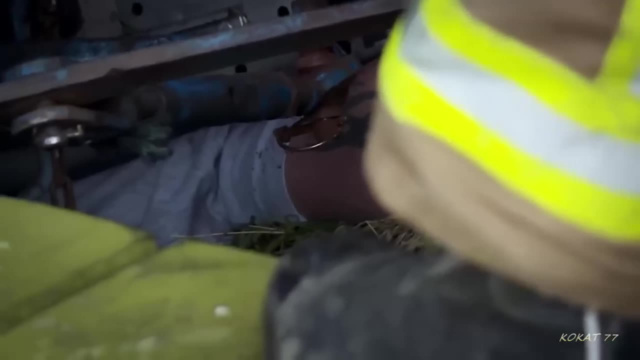 Just bear with me, I know it's a bit awkward. All he can do is give him painkiller drugs and wait for firefighters to work out how to lift the tractor without further injuring 32-year-old Sam. He's desperate to escape. I need the pressure off. 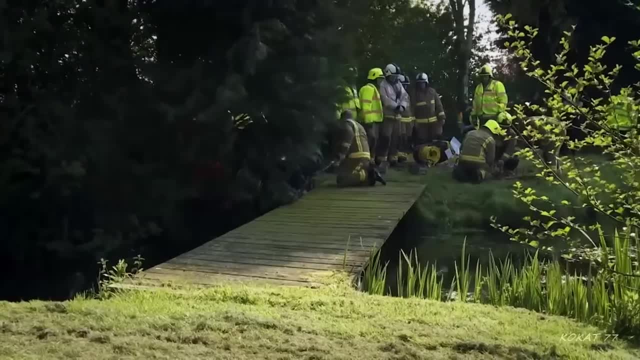 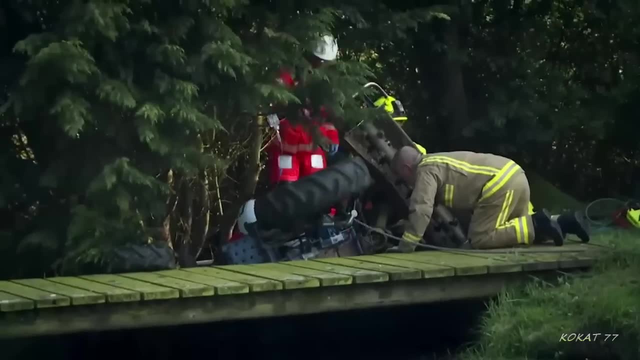 Listen, we've got to do this carefully, haven't we Nine-two? Do you know what I mean? We can't just rush. Lifting the tractor could crush Sam's leg further. They need to be careful and it could take time. 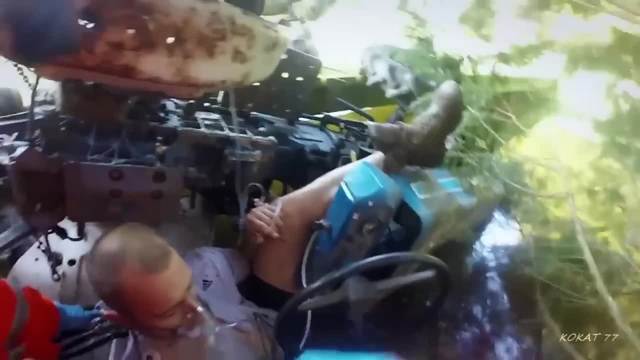 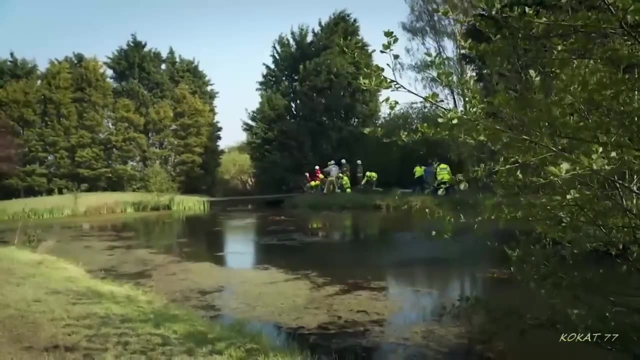 That's time Sam may not have, His temperature's falling and he's showing signs of losing consciousness. He's coming with it. Sam's going to get rid of it. He is going to get rid of it. I've already got it, Sam. 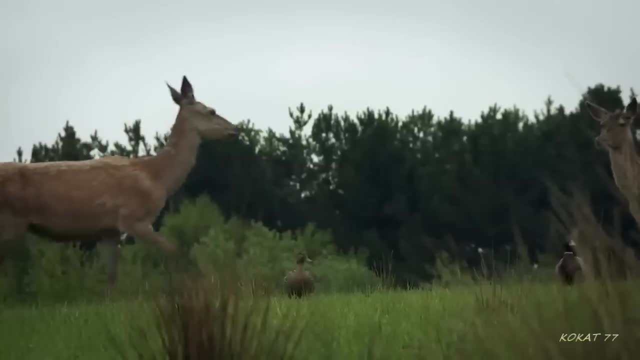 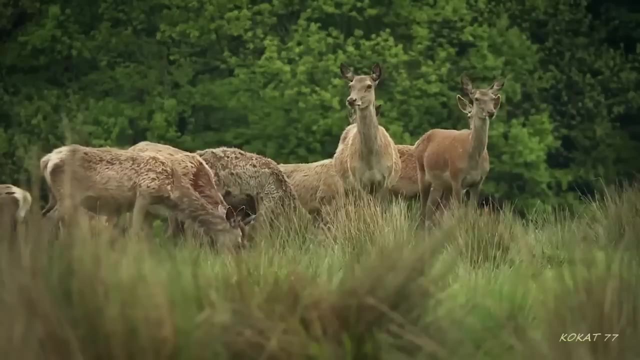 I'm going to go in that way and then he's going to come back in. We're going to take him down. You're right. Sam's going to be right. I can't expect him to get through here. He's going to be useless. 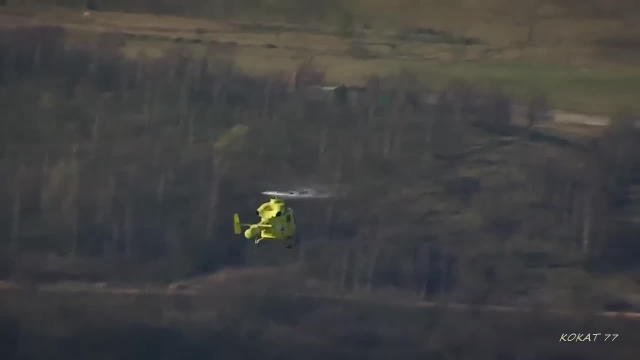 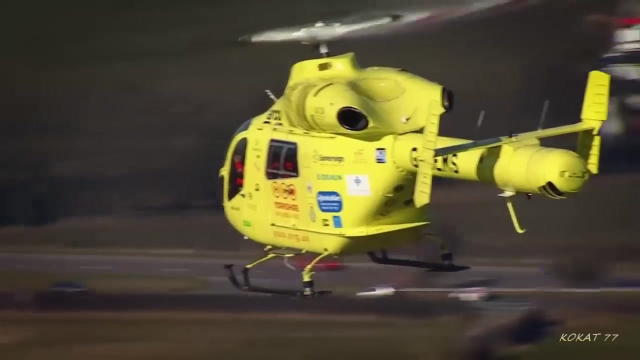 He's not going to be good. He's not going to be good. I'm going to get him down. Sam, That's better. Sam's got a lot more to do. You know, motorcyclist is hitting an animal on the road. 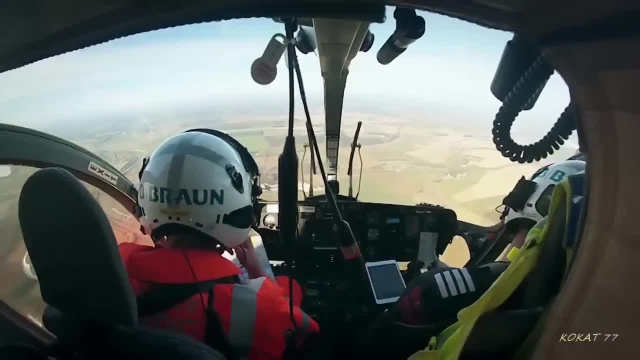 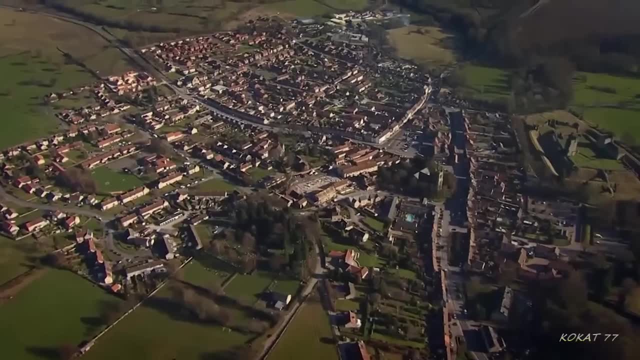 Motorcyclist is unconscious but breathing, Getting some more confirmation of what the injuries actually are? Yes, obviously, Noah, The team's heading for the market town of Helmsley. It's a mecca for bikers out enjoying the winding B Road north. 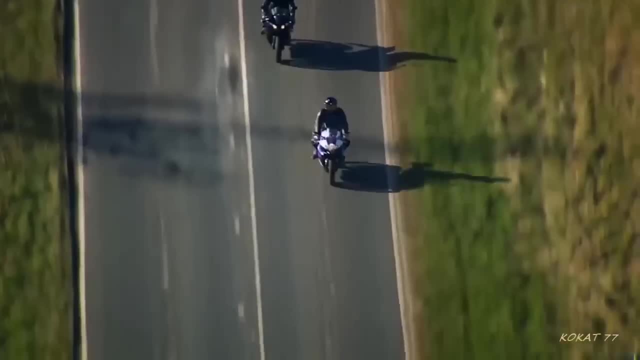 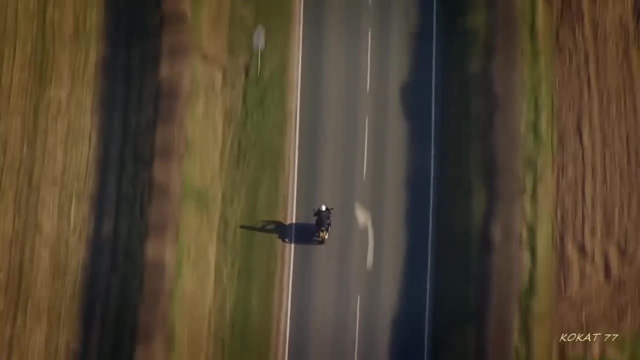 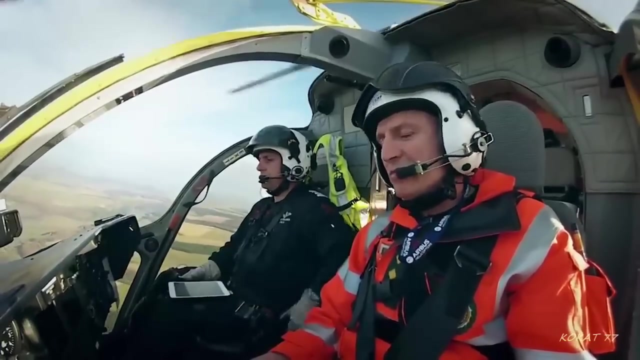 through scenic Billsdale to Middlesbrough. We've been to this road many times in the past. It's an area of open road in the countryside that quite often both cyclists and motorists alike use the race up and down. So I'm not saying that's the case with this patient. 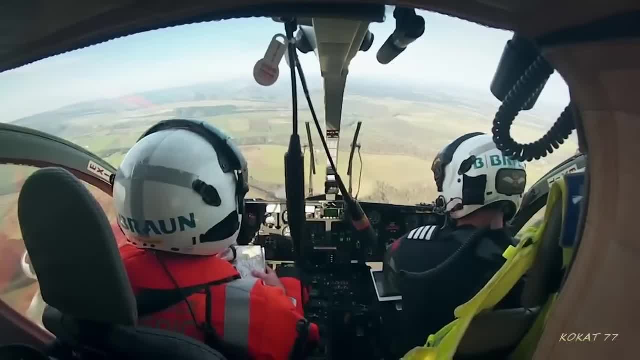 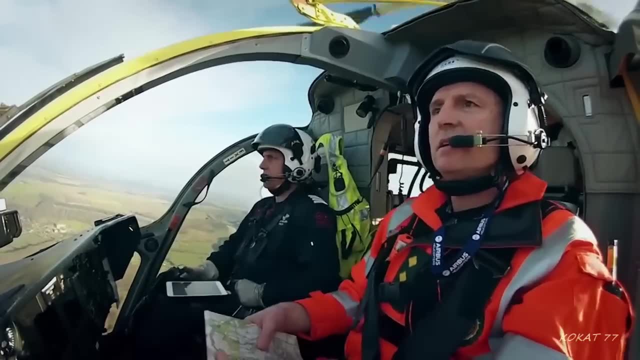 but we have attended quite frequently in the past- Got the road, Got that cut-out I was on about. You can see the road this side of the wood. You've got two or three port vehicles. That's got a visual, yeah. 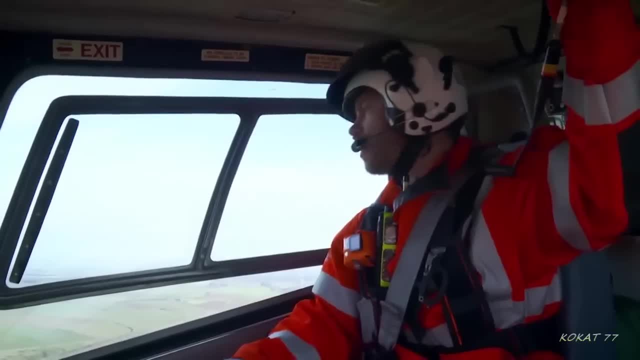 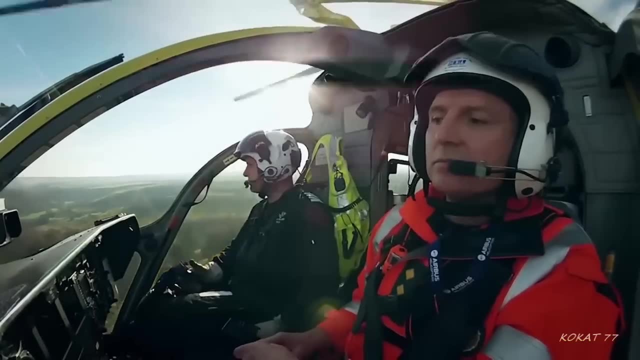 Coming back. man, You're right. Hi, that's from Helibet 98.. The visuals I've seen. I'm prepared to land over. Yeah, I'll go in front of that police car. I don't know if I'll fit. actually. 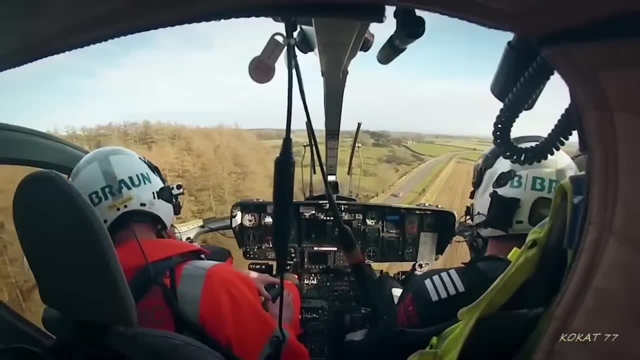 We'll go and have a look. If not, I'm going to put it in this little field below us. Pilot Gary is on final approach to a tight landing spot in the middle of the road. I can't win that field. There's green wires. 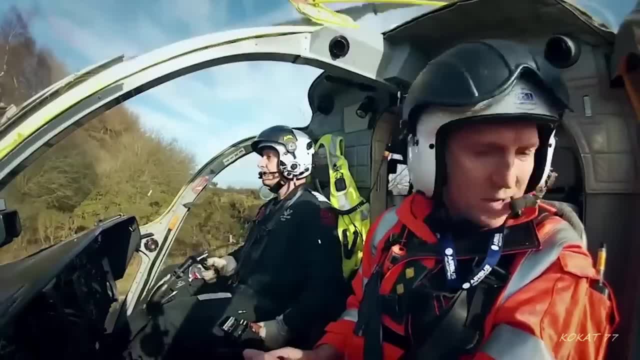 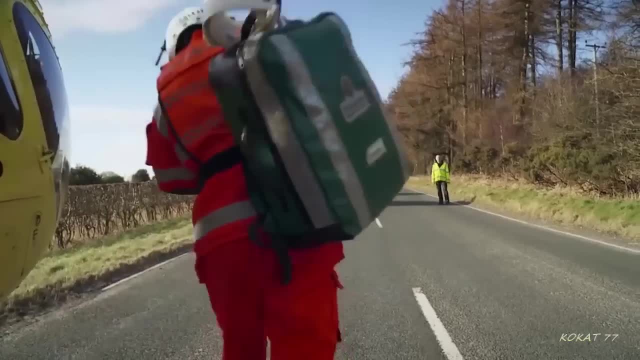 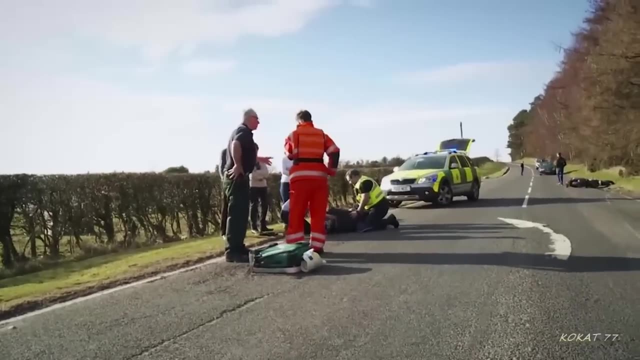 This red car's the first thing, Gary, Still good mine, Just this side. Thank you. There we go. All right, you got it A lot of pain. He's sort of posting his hip. whether he's got some confusion. head injury, hip pain. 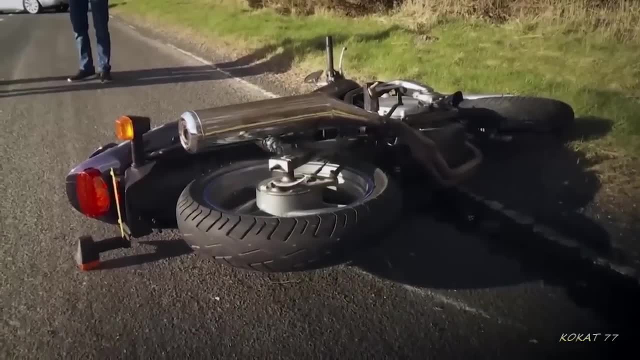 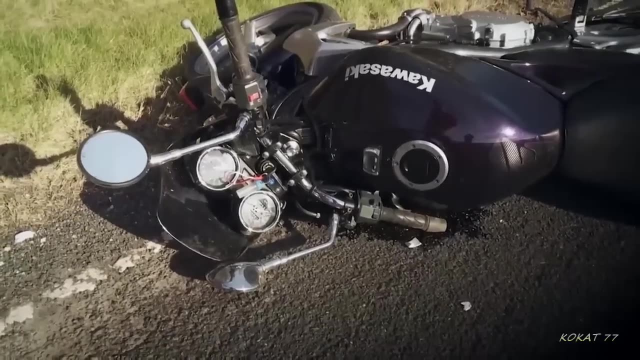 I'm not sure at the moment. The injured rider was thrown from his high-powered bike and slid more than 50 metres down the tarmac. He was wearing protective leathers, but he's still badly hurt. He's a good colour, He's fine. 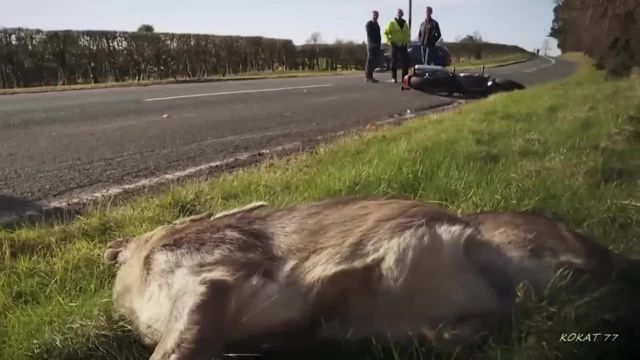 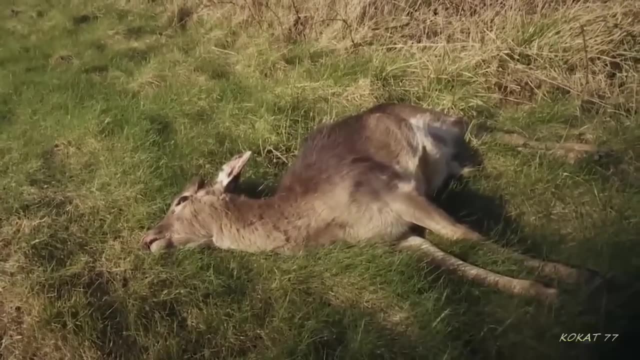 He's got a lot of pain. We'll get some oxygen on him. The other casualty of the crash wasn't so fortunate. A fully-grown deer crossing the road from nearby woods was killed instantly. It can't have been going very fast. 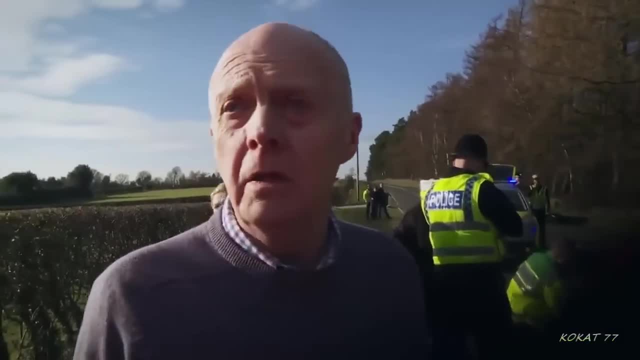 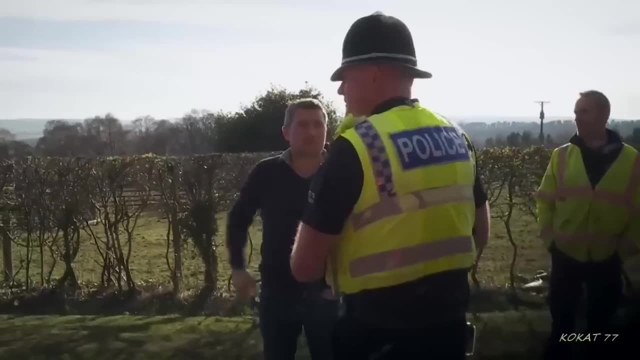 And he kept at this point and a fawn ran out of the field. He had no chance. He braked, came off and that was it. There's two dead deer in here in the last two days. Locals are used to accidents caused by reckless riding on this road. 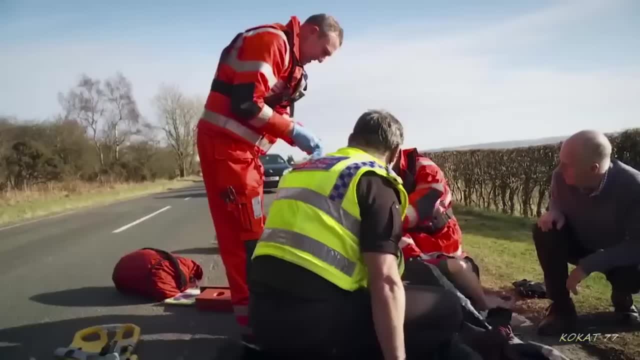 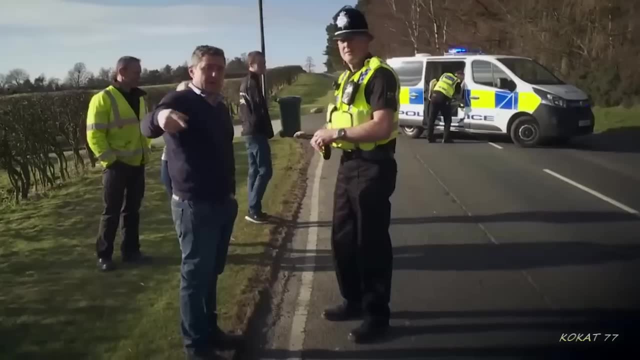 but this wasn't that sort of crash. Kenny Best, the 59-year-old biker, was riding sensibly. Kenny, just relax, fella, OK, Just don't move your head too much. for me He's like MotoGP here on a weekend. 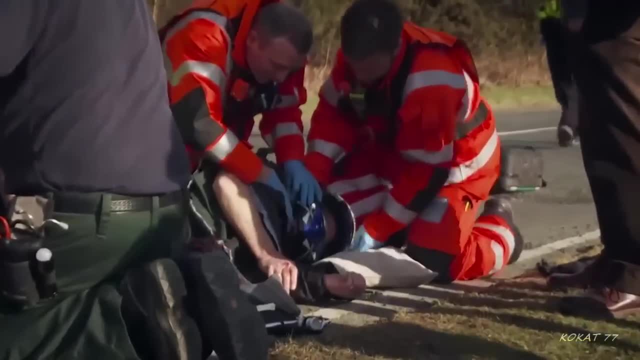 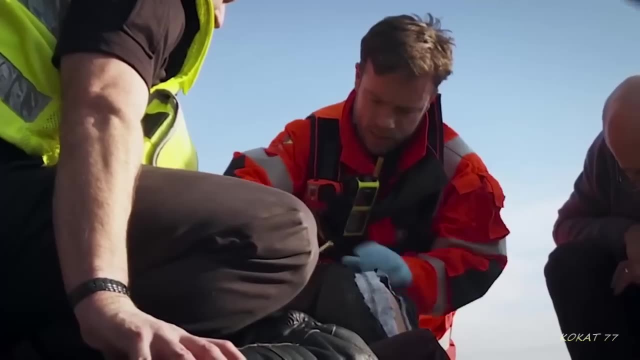 I never even heard him coming. Kenny, we're going to take your helmet off, fella. OK, Passers-by did the right thing, leaving the rider where he fell. Now paramedics Pete Vallance and Lee Greenwood must remove his helmet. 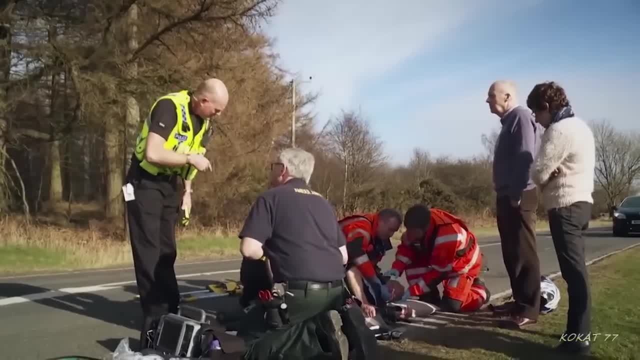 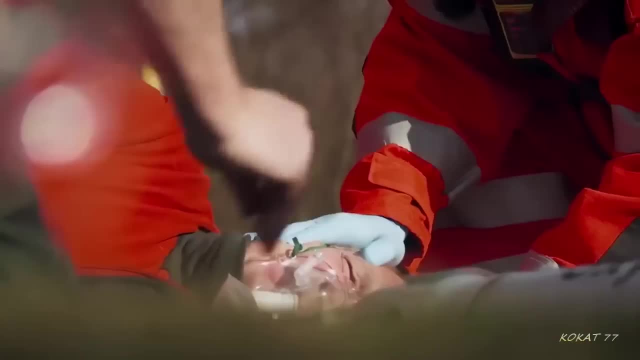 It's feared he may have injured his spine. There you are, Kenny, Let's keep you. Just relax, Kenny. OK, Kenny, Kenny, don't move, Don't just. Kenny's in severe pain. Lee is trying to make him more comfortable. 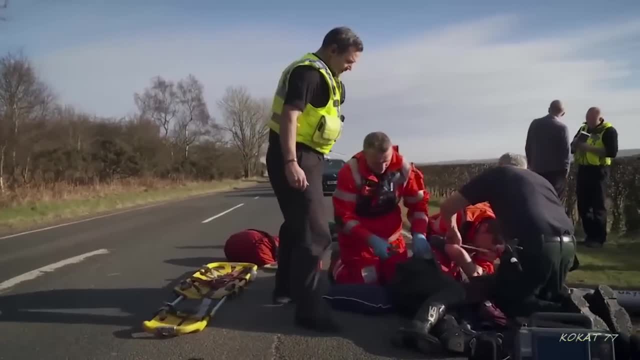 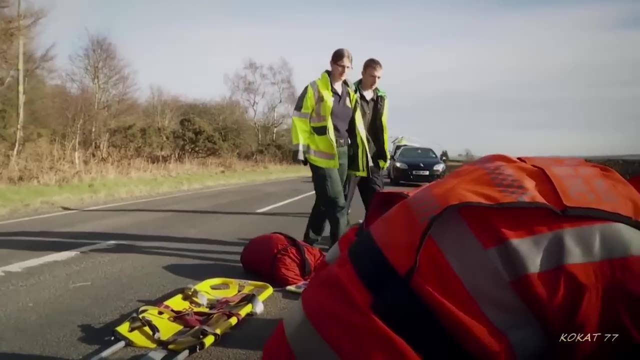 Is it pain in your pelvis Or in your back? Yeah, everywhere, Pain everywhere. Well, getting a package up and stuff, That's it. It looks like he's fractured his femur. The fear is he could be bleeding internally. 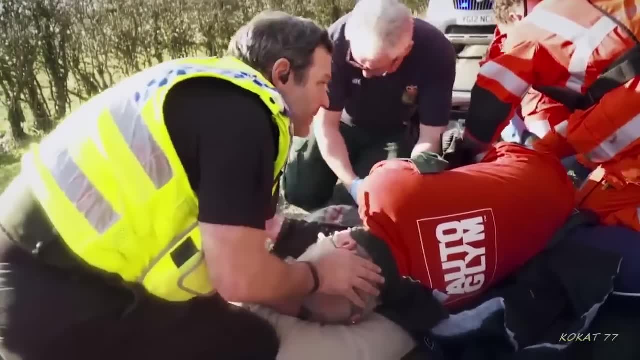 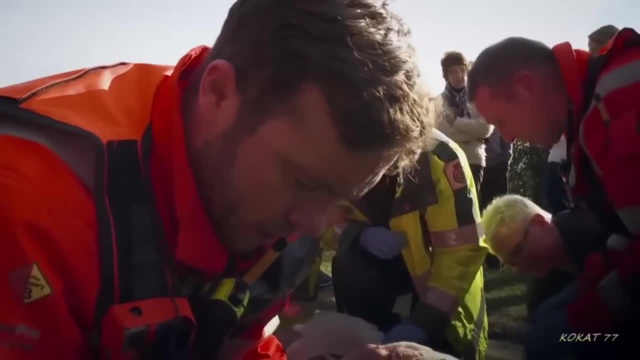 If so, this crash could kill him. Yeah, you can hear it. He's in quite considerable pain. It's quite difficult to assess him. It doesn't look like he's got anything obvious that we can see. I'm just complaining about the pain around his hip and pelvis. 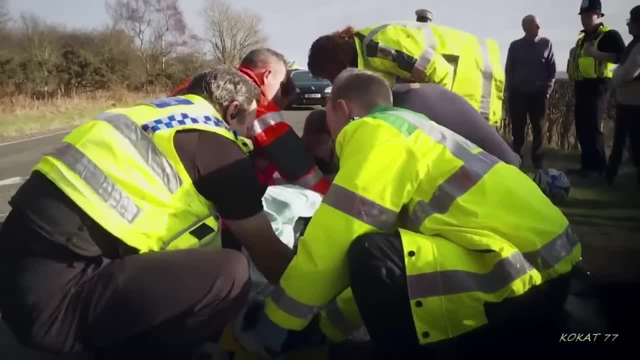 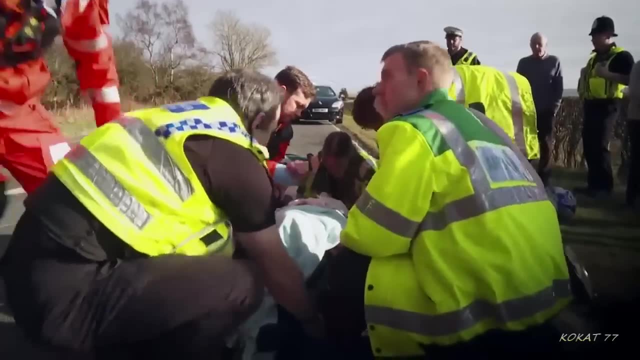 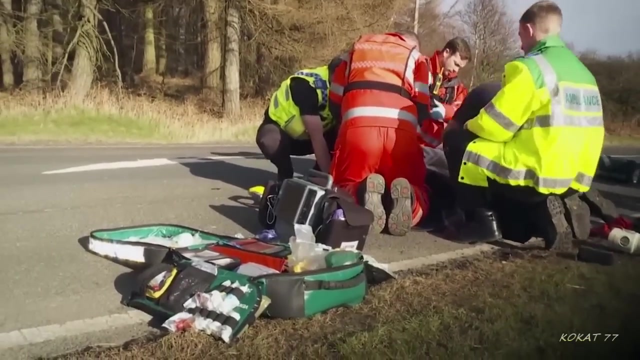 So we're going to get some anesthesia on board. They must use a splint to prevent broken bone fragments damaging internal organs. Kenny, just relax, Just relax, OK, Kenny's also been injected with TXA, a drug to prevent bleeding and encourage clotting. 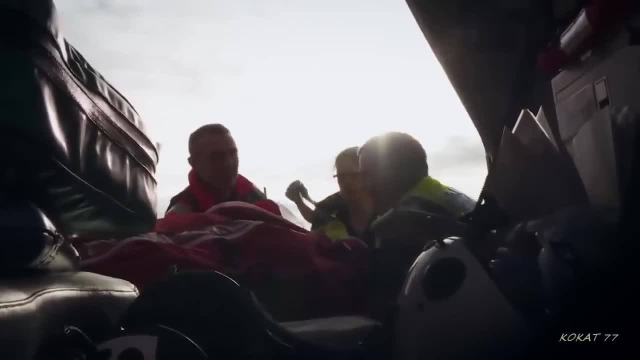 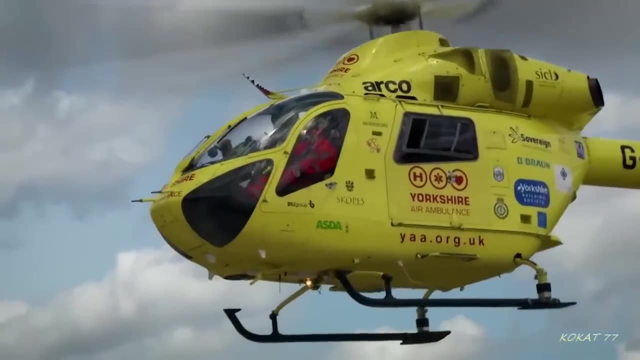 Push it out there and literally feed around. They're going to fly him direct to the Jameson James Cook Hospital in Middlesbrough. There was nothing he could do to avoid this crash, but its effects could have devastating consequences for him and his family. 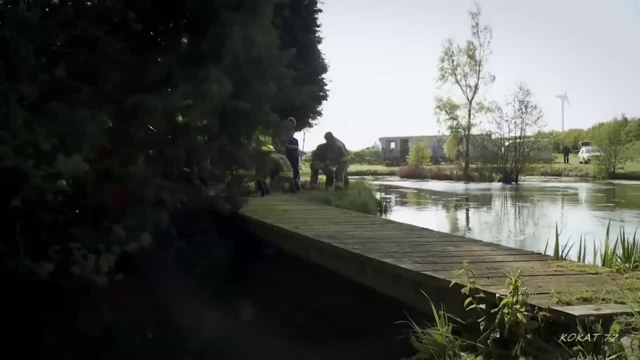 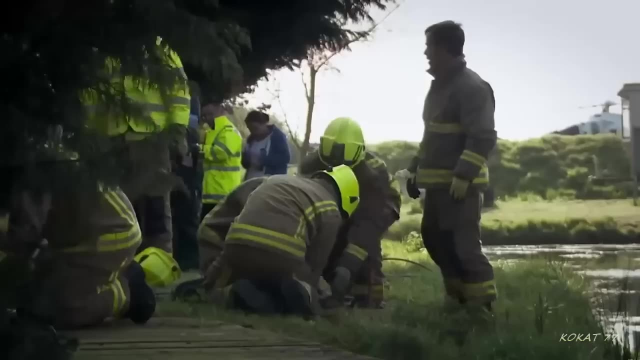 On the banks of a fishing lake on the Yorkshire coast. Sam Brockwell's life hangs in the balance, Trapped beneath his tractor. there are fears he could drown. Are we aware of the panic? I'm going to do the forebore to make that seat. get the seat out of the way. 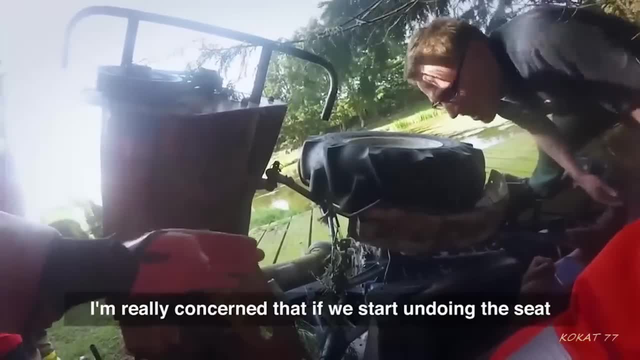 OK, Then we might be able to get him out after that, Right? OK, I'm really concerned that if we start on doing the seat, he's going to fall further this way. If that fails, we'll just literally start lifting it. 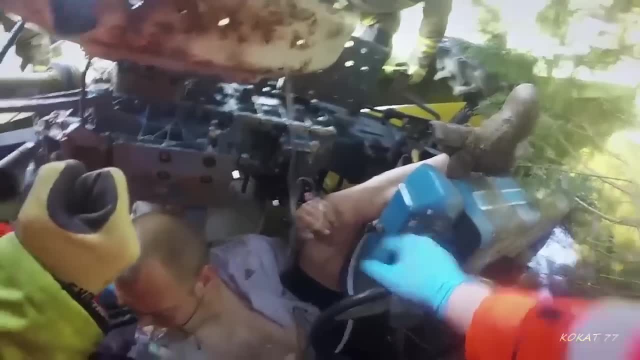 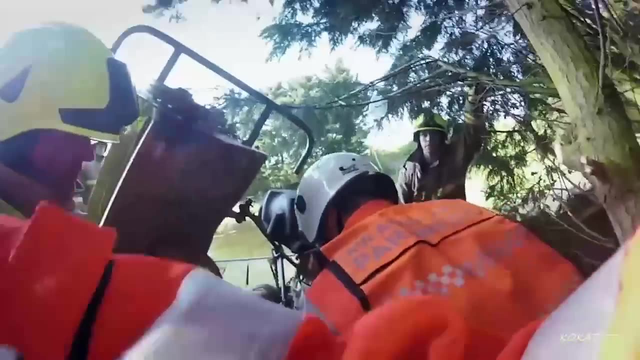 and we're going to have to just get him out. OK, Sam has a suspected broken shoulder and a collapsed lung, But paramedic Paul fears his patient's life could also be in danger from compartment syndrome, a lethal condition caused by toxins building up in trapped limbs. 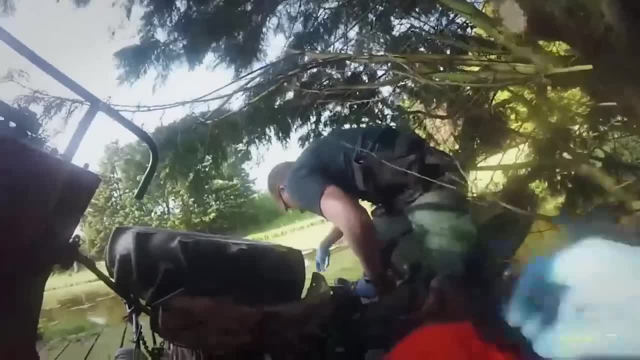 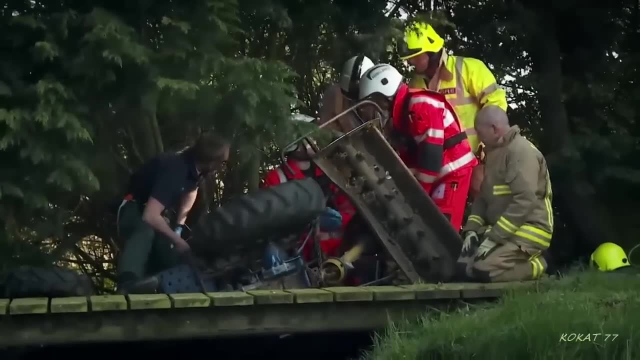 It can cause sudden cardiac arrest. Can you feel me touching you there, Sam Whoa? Can you feel that? Mm Yeah, OK, Yeah, sorry, Can you get us ECG Dawson? We'll put him on ECG, just in case he's throwing up some ectopics. 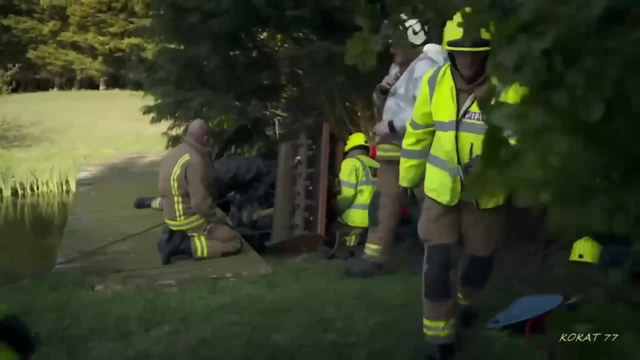 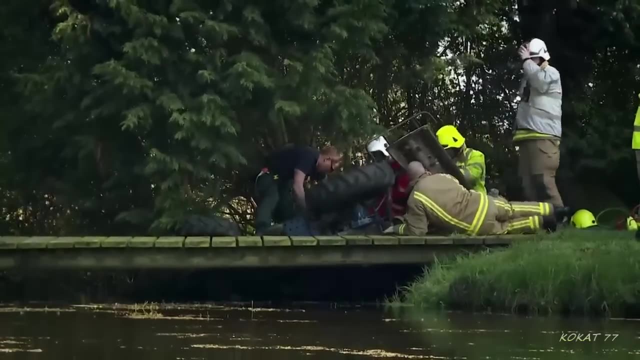 He's monitoring Sam's heart for spikes in the rhythm, ectopics that could be signs he's going to arrest. So you said last BP you were. We have got BP on him. Oh, haven't we? He can't get around to his arms. 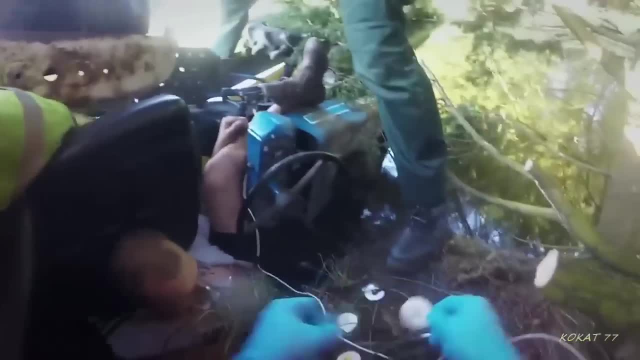 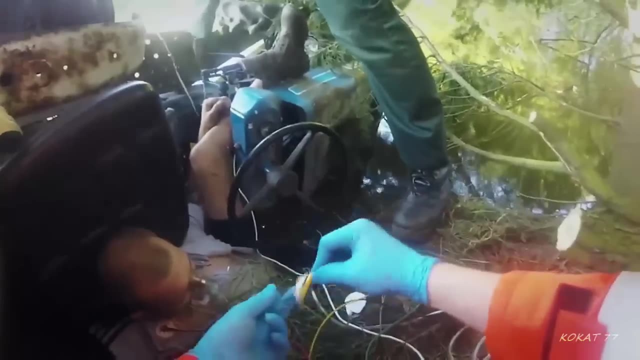 He can't move his arm, His pulse is growing weaker and his blood pressure is dropping. Let's just stick these on, Sam. Can you talk to me? How old are you? How old are you, Sam, 32. 32.. 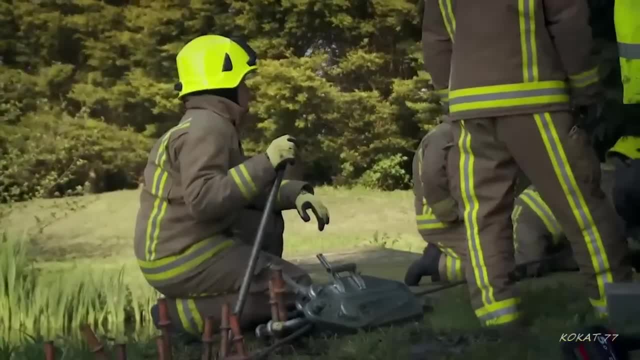 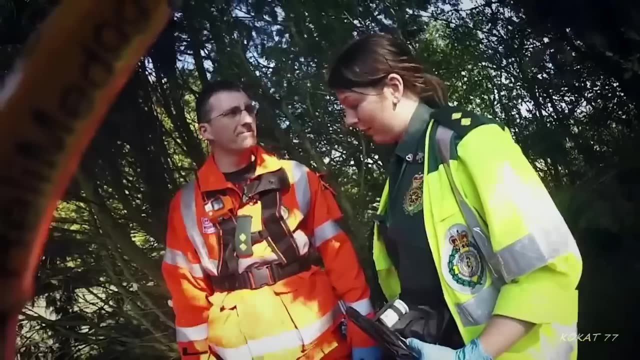 Where do you live? Hull, Hull, Yeah. Is there any pain in your tummy there? No, You've got there. OK, Give him some TXA. Yeah, All right, Because he looks quite trapped, so he could well have something. 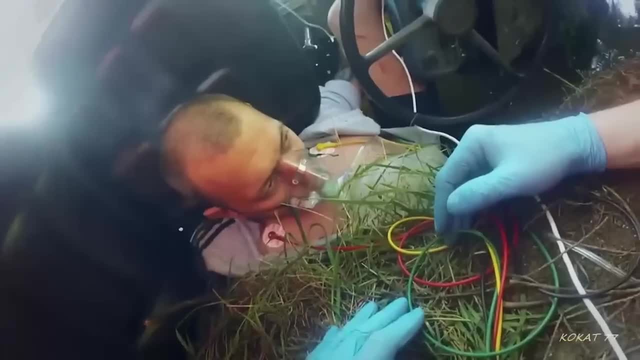 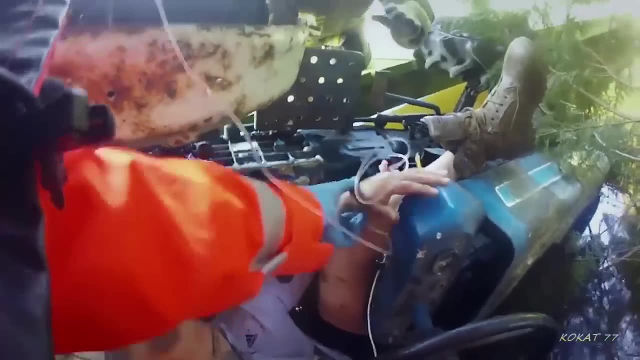 Yeah, absolutely. You know what I mean. So we'll give him some TXA as well. Oh, Paul wants his patient freed quickly. TXA will reduce any internal bleeding, Oh fuck's sake. All right, Sam, We'll get you out of this when we can mate. 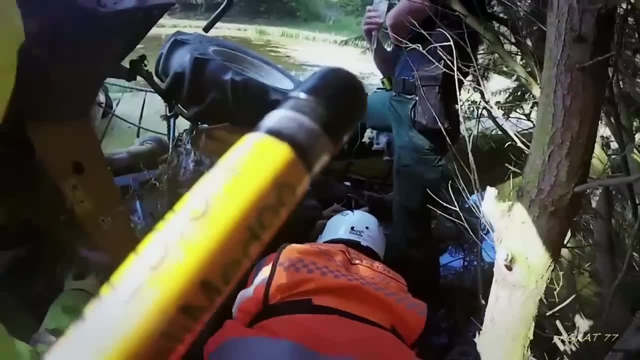 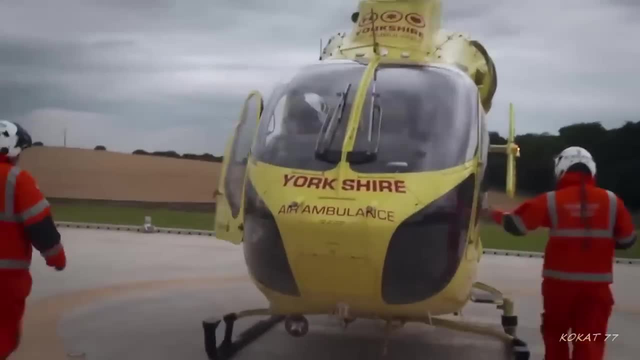 It's getting worse. What's getting worse? Just the weight. I know, mate, I know The team's so concerned about Sam's condition. the second chopper, Helimed 98, is being scrambled. It's bringing a trauma doctor to supervise his care. 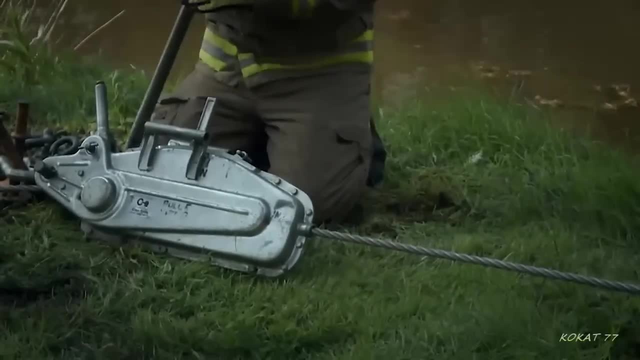 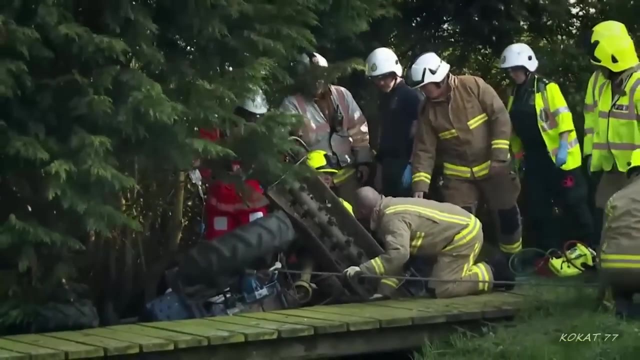 You'll be able to feel it moving as they're trying to tie things around it. OK, The second. they've taken the weight. we can get you out. All right. All Paul can do is reassure Sam as the firefighters get to work. 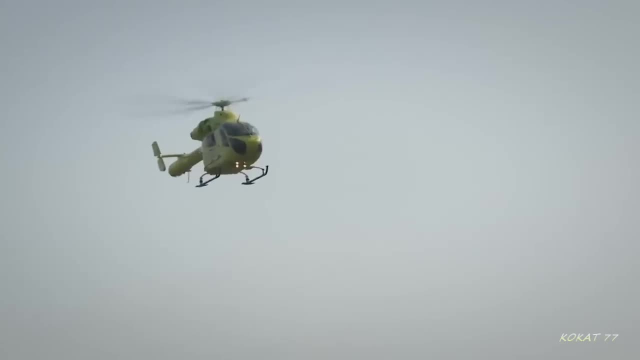 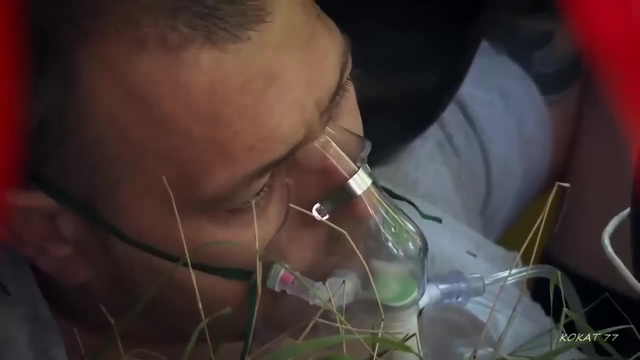 You're doing really well. Helimed 98 is arriving on the scene to join the rescue. Any pain in your shoulder? Yeah, A lot, I love a lot. Tell me, can you get some morphine drawn up as well, mate? 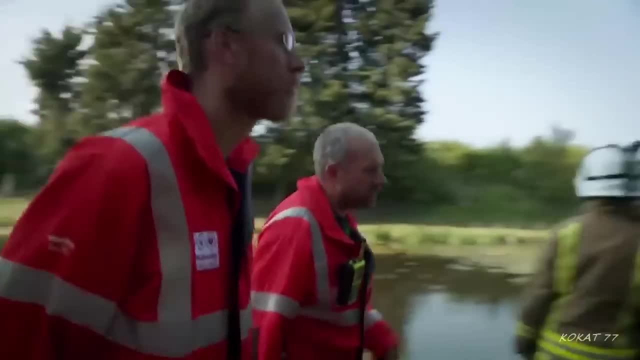 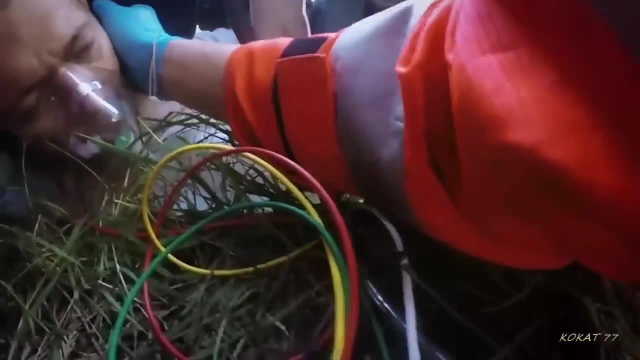 Dr Neil Sandbridge will be in charge of resuscitating Sam. if his heart stops, Just give us a shout. if you start throwing so many topics up, will you mate? If your heart starts getting a bit funny, all right, then obviously I'll give you something to stop it. 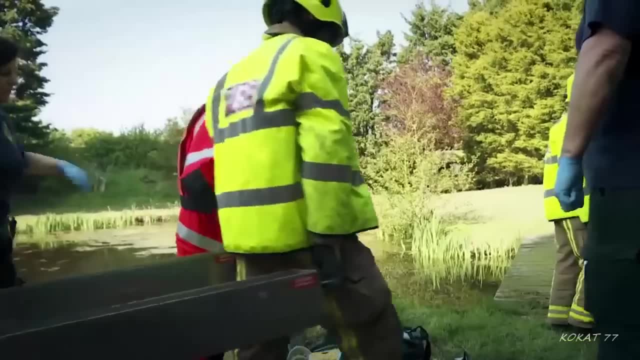 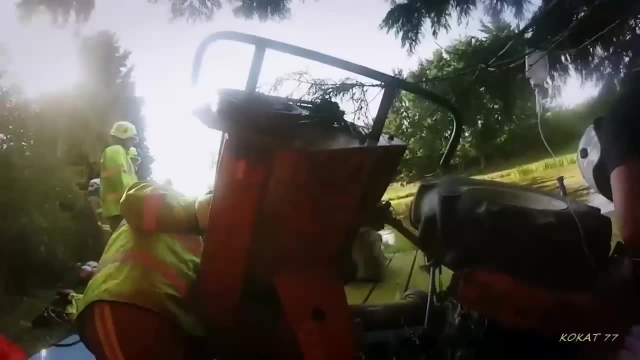 OK, You're doing really really well, mate. At last it's time to move the tractor. All right, We're going to start taking some of the weight, OK, And you'll start feeling a little bit better. Cables are now supporting its weight. 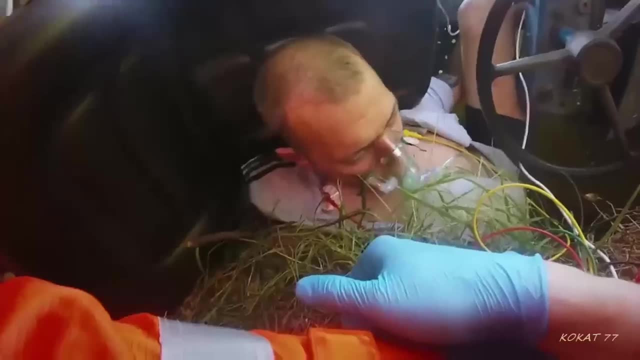 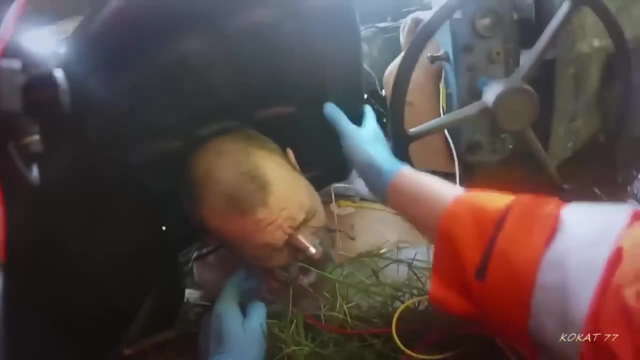 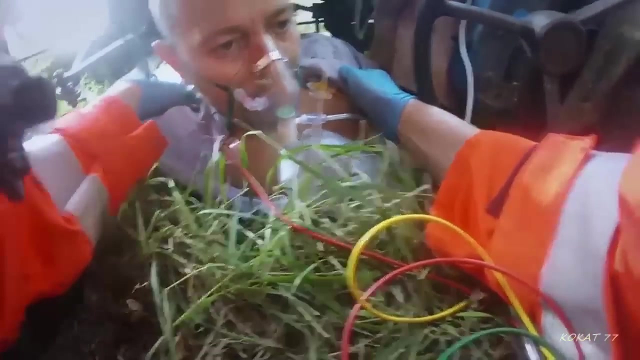 They'll first have to remove the driver's seat. Where's that? Where's that? Your shoulder? Your shoulder, It's feared Sam may be suffering from hypothermia. He's been submerged for an hour or more. All right, Well done, mate. 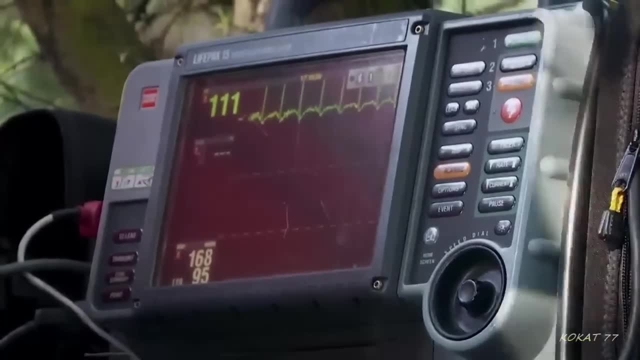 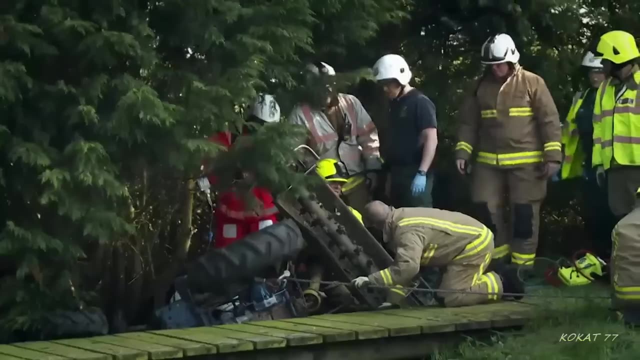 Good lad, Anything on his ECG? No, nothing yet. Good Yeah, we're going to have to be careful where you strop around his shoulder- If we can get around his waist- because he can put his foot down on the ground and he's just slipping. 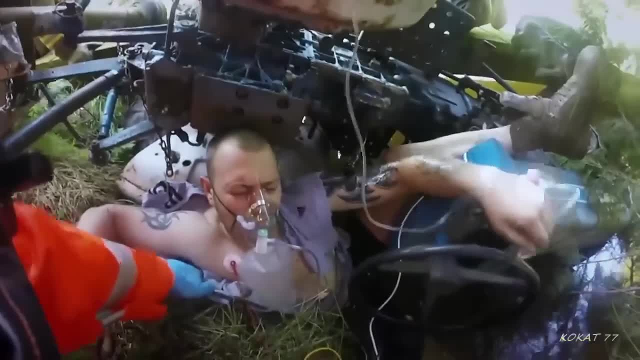 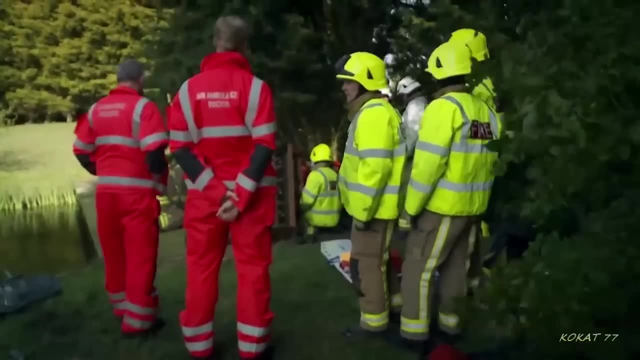 You can try and avoid getting something underneath there because of his shoulder. You know what I mean. Sam's got to help himself. Firefighters have created space for him to move his leg. Are you going to push up with your leg? Yeah, I'll try. 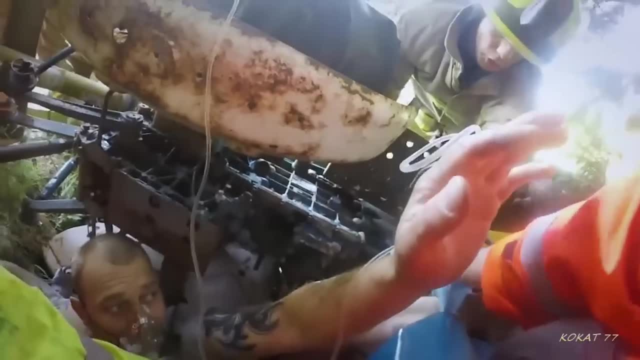 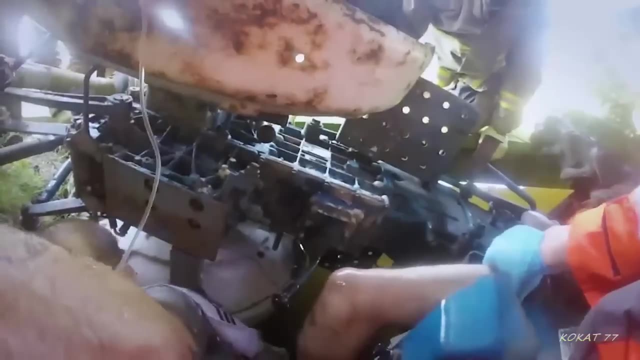 Can you move that leg? Yeah, Would you be better putting your leg further down? Wait, Hang on a minute. There's no pain there in your pelvis, is there No, Right? Can you move this leg? Hang on a sec. 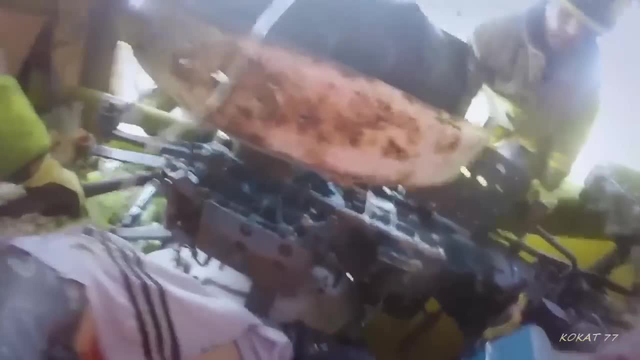 Oh, come on, mate, That's it. Come on, mate, That's it. Watch his shoulder. Just watch the tractor as well. All right, buddy, Come on, man, Watch his arm. Someone support his arm for me. 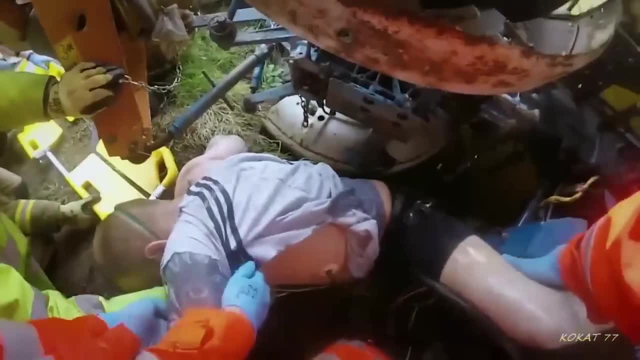 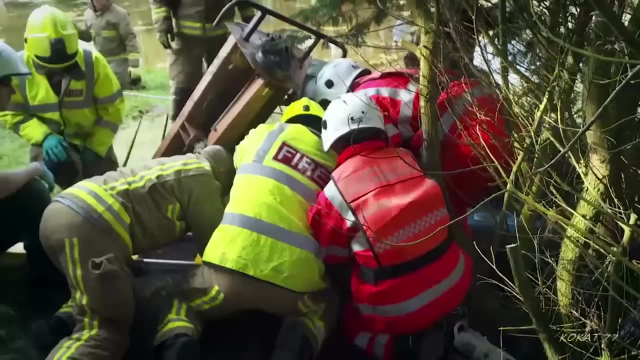 If you can, You're going to lift his knee over that stairwell. That's it. Oh, Watch his arm. All right, I've got that His arm. Oh, Oh, Just take the board back. One last push bud. 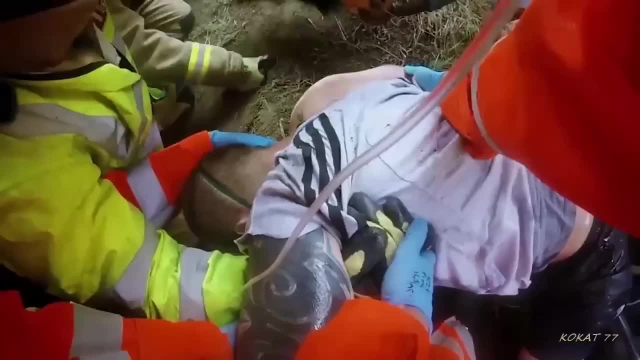 Can I see One last push? All right, Three, two, one go. Come on, mate. At last he's free. Now the focus is shifting to his injuries. Oh, Oh, We're going to have to get him off his bad arm. 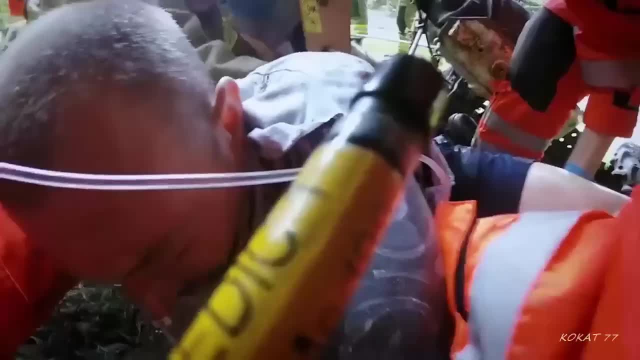 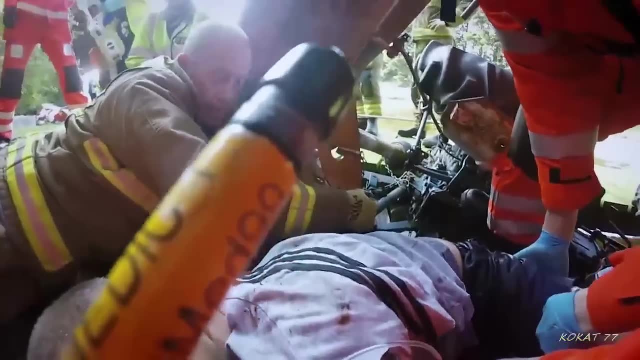 Oh Oh, And you have to keep your feet straight. Oh, Oh, Oh, Oh, Oh, Oh, Oh Yeah, I'll just come up this way. then on to his-. Yeah, Yeah, I'm just conscious about his shoulder as well. 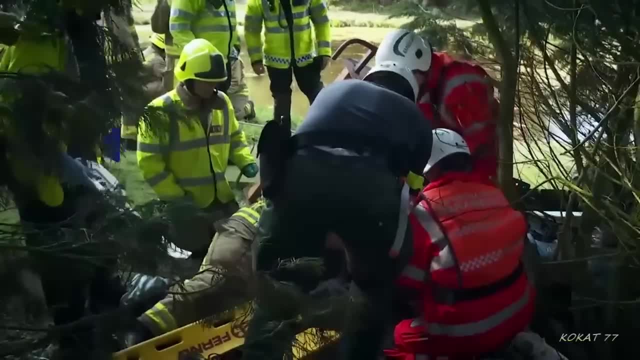 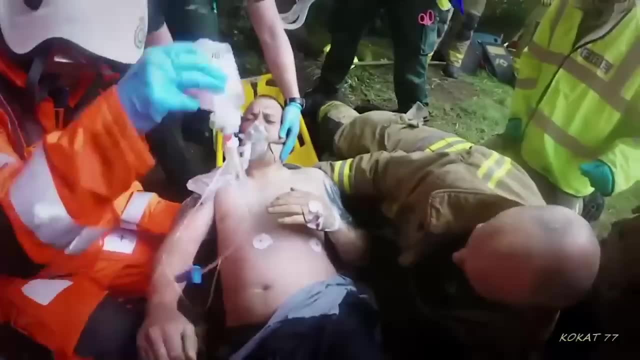 A little down. Oh, you fucking do this, Alex. can you just support his head for me as we go down, mate, please? Oh, Thank you. All right, Sam. That's it. That's it All right, mate. 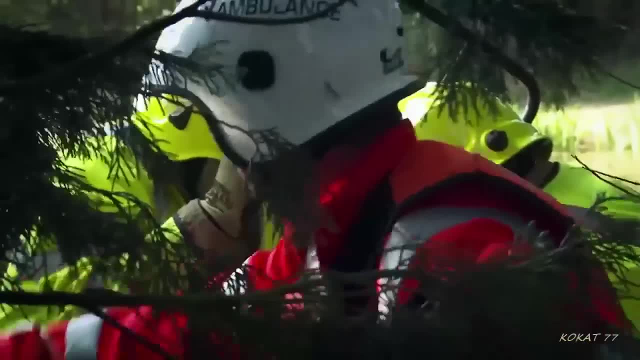 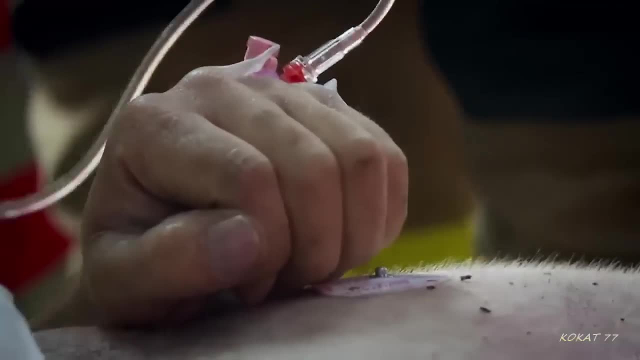 Oh, Fucking hell. There are fears he may have broken his pelvis, a potentially deadly injury that can cause fatal internal bleeding. but the cold is also a serious danger to him. Fancy, I can tie you up, Get on your blankets to wrap him up. 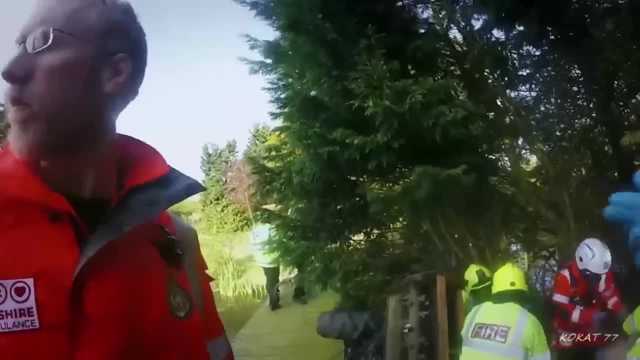 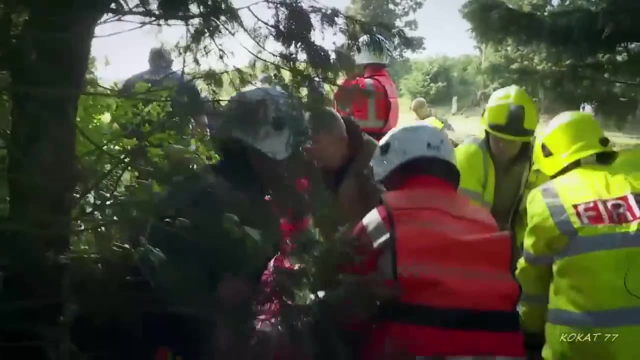 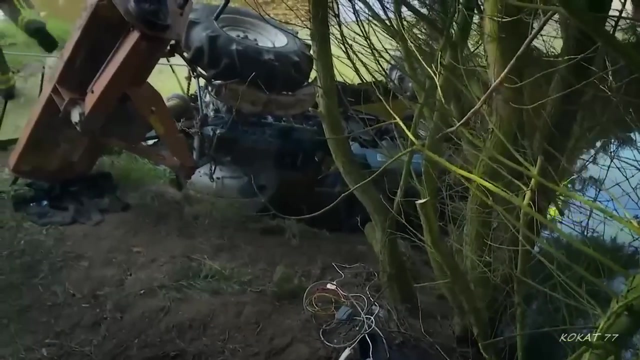 Get down, wrapped up and out of here. the race is on to get into hospital. it's 20 miles away in hull. try just lifting as it is. for the fire brigade it's been a very difficult rescue in an almost impossible location. the main challenge is really it's securing the tractor so we can actually manipulate. 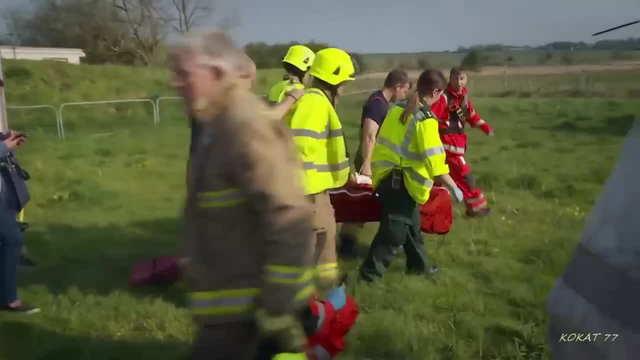 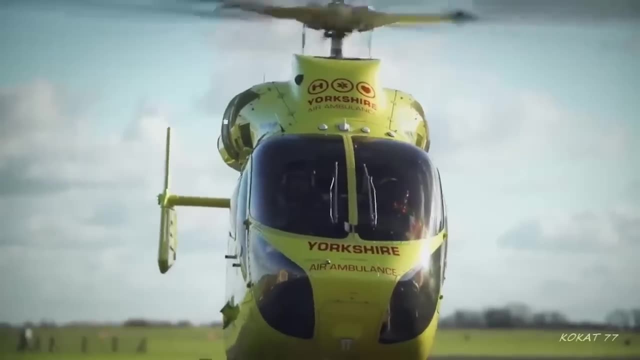 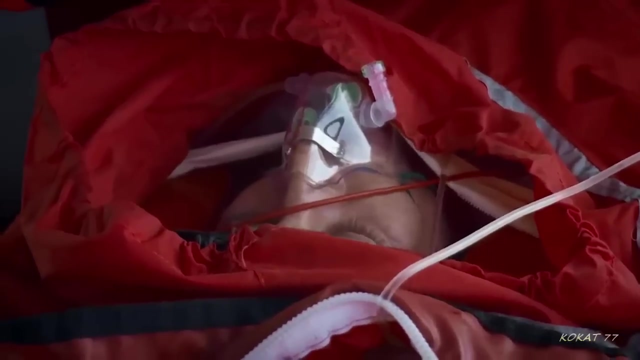 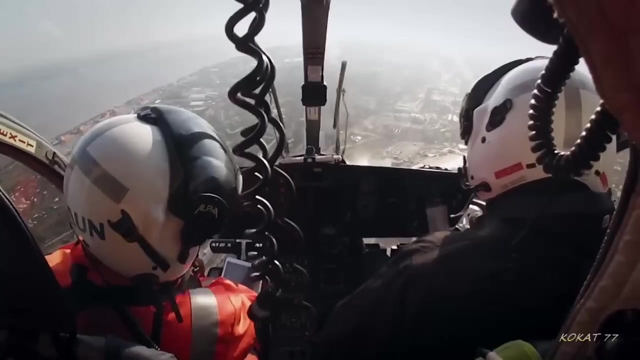 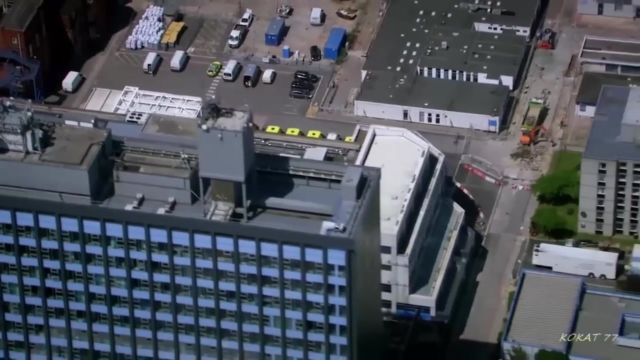 the casualty from under the tractor. it was a cold which was getting to the chat and obviously we need to extract some more from there quickly. an hour ago, sam was cutting the grass around the fishing pond. now he's on his way to a major trauma center. a full surgical team has been assembled to assess his condition. 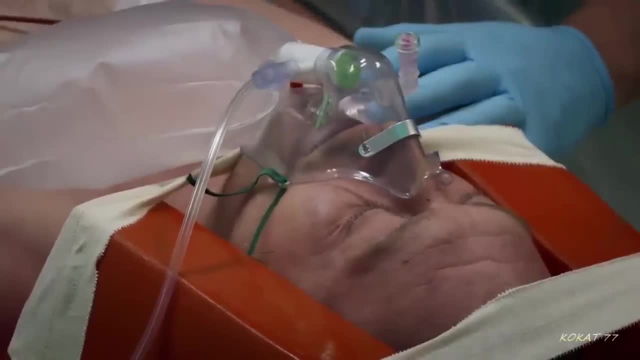 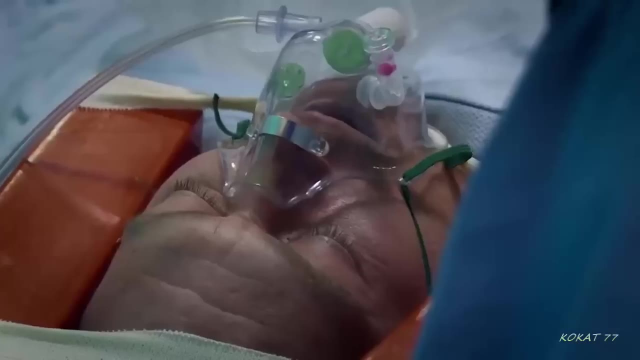 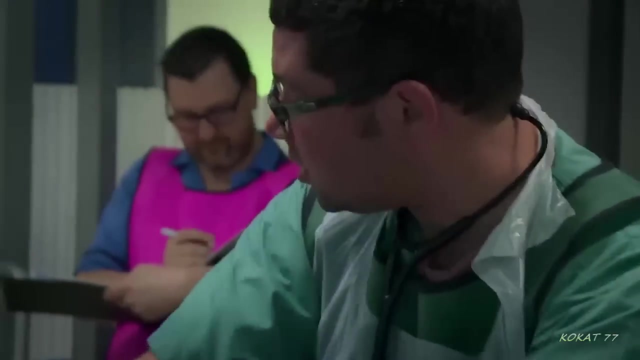 paul fears his patient may have many undetected injuries. his right arm was bent right back behind him. his leg was quite an acute angle so he could well have done a pelvic injury. it will be a few hours before the specialists know the extent of the damage. 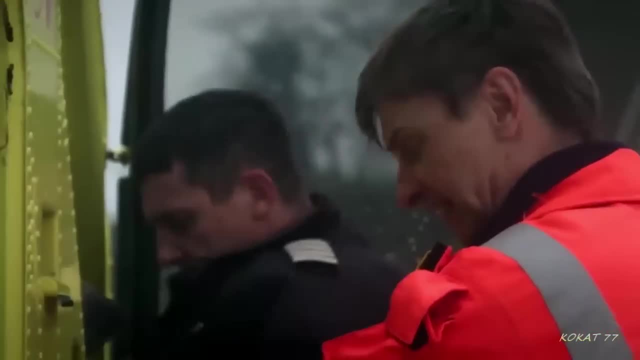 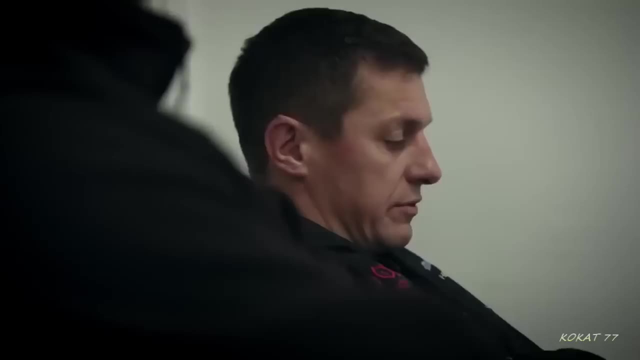 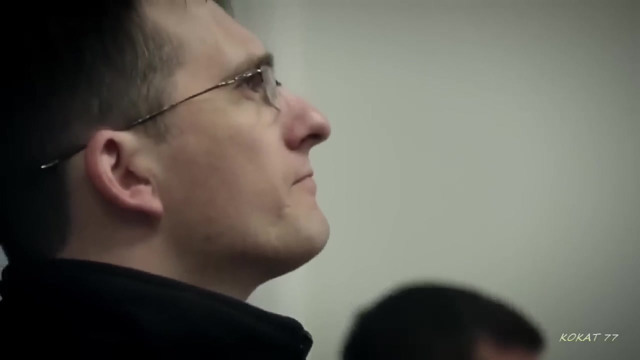 for the air ambulance team. the day's weather forecast can be a matter of life and death. at least a minute before. some of the winds: 40 knots, gusting, 24 all the lines. pilot gary brasher is briefing his crew. but windy, forecasting a few, four thousand all day and then again throughout the day. 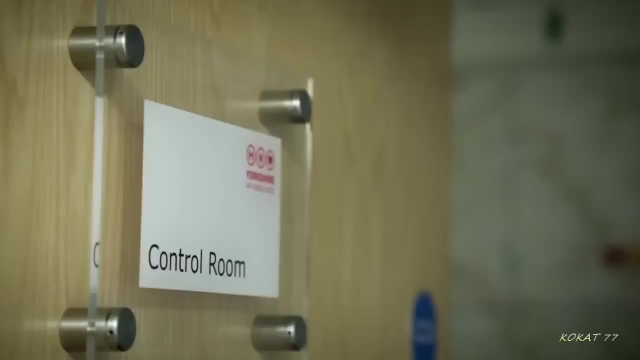 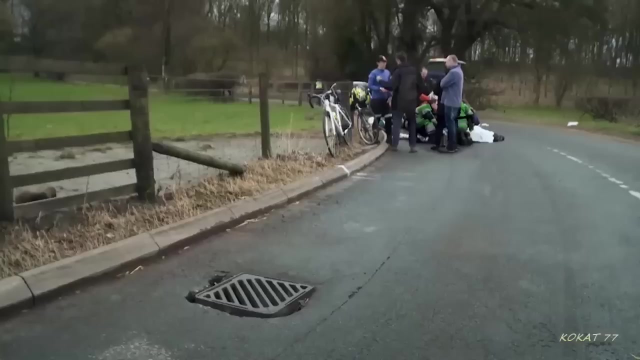 rainy event, heavy rain, and it's not long before the blustery weather becomes a factor in a very serious case. there's a patient breathing. patient's bleeding, but she's bleeding from her head. on a rural cycle route near rippen, a wet road was a factor in a crash. 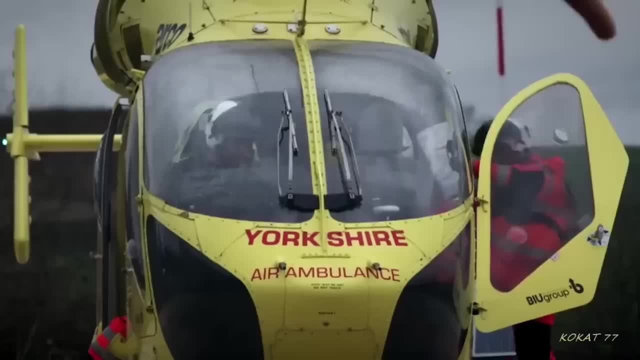 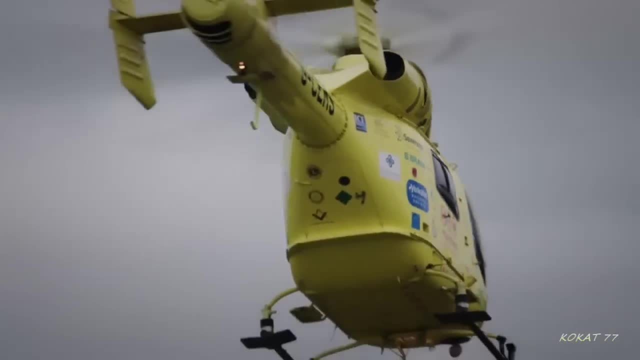 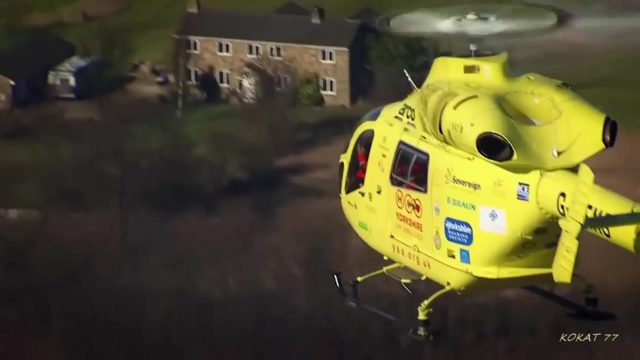 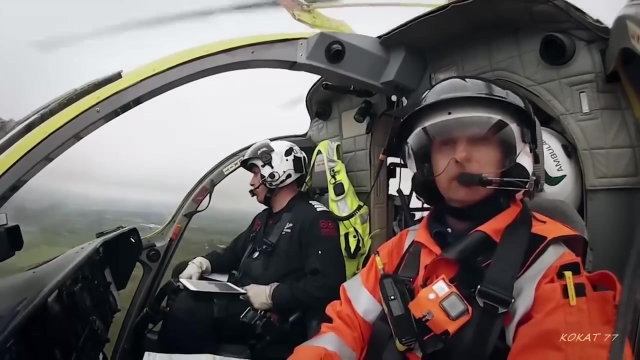 that's left a rider fighting for her life. she's coming. i'm assuming there's some form of Rose heads help. we're at the mercy of the callers. quite often when we get there it's not always as we've got time and energy, as we find it on the call. 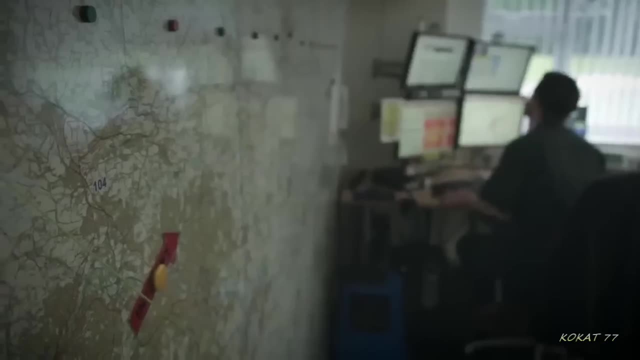 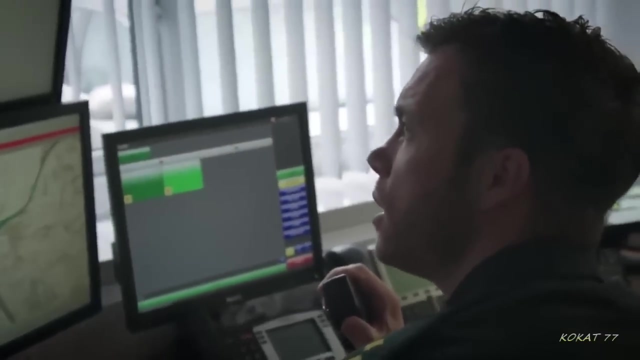 1198,. can we have a hospital breakdown when you've got a few minutes, please, please, Closer to the lead. yeah Yeah, I've got Harrogate at 12 nautical miles, LGI 23,, Northern General at 27 nautical miles over. 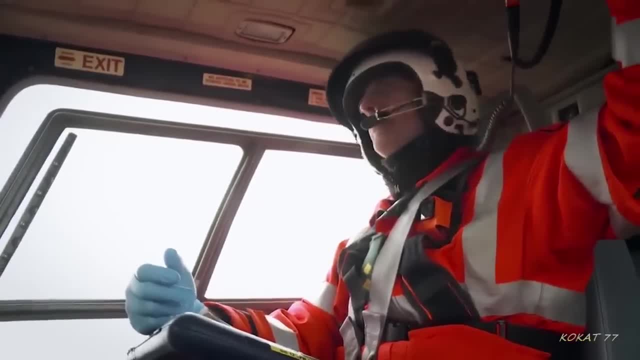 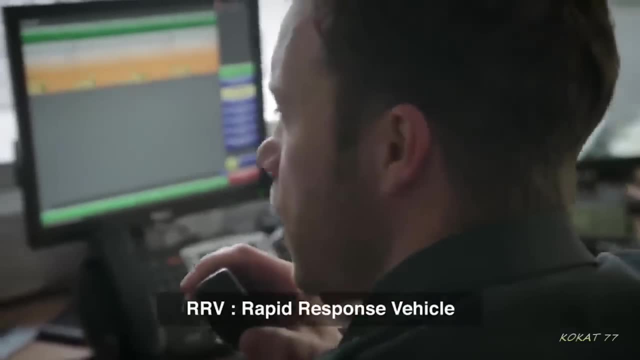 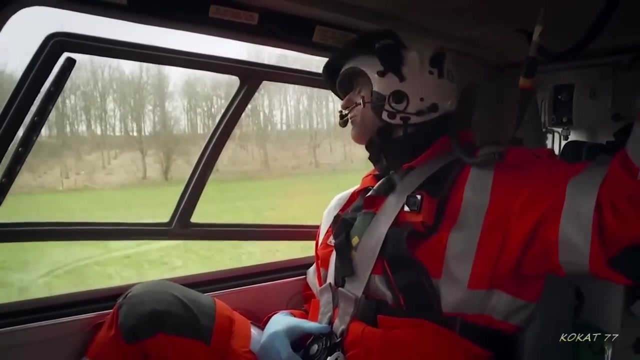 1198, Airdesk. we are one minute to the scene. Is anybody already on scene? Yeah, that's all received. There is an RRV keyed on scene over Clear left. I'll let your shutdown go, cos I'm going to have to do a bit of climbing, I think. 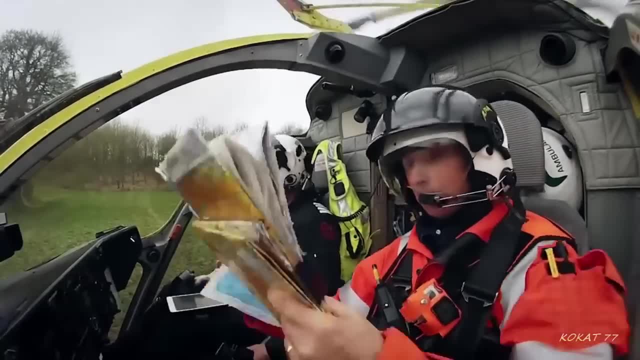 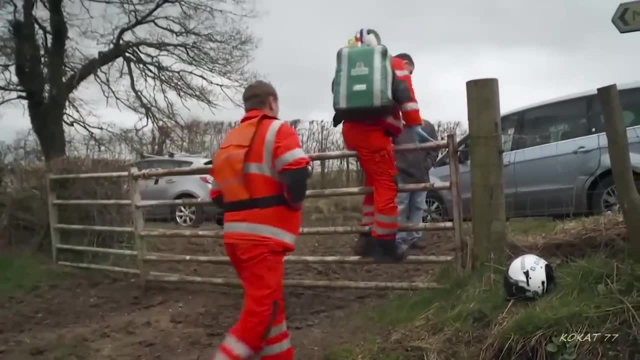 There's a gate mate on the left. Oh is there. OK, I'll get out now. then A 62-year-old cyclist has a severe head injury. Paramedics Tony Wilkes and Paul Holmes know cycle accidents can be very serious. 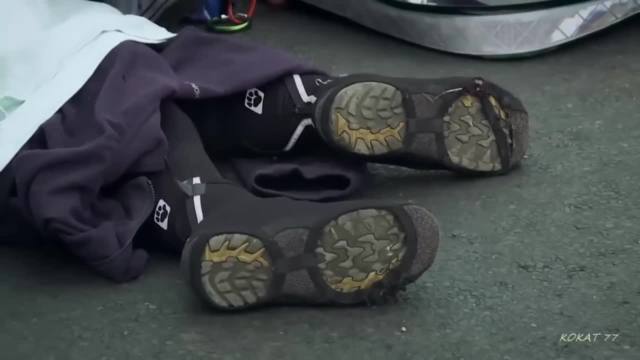 Hi, there, Hiya, How are you doing? She's come off the bike, rolled over Dotsie Dotsie behind her, saw her on the back, OK, But she's been semi-conscious since then. 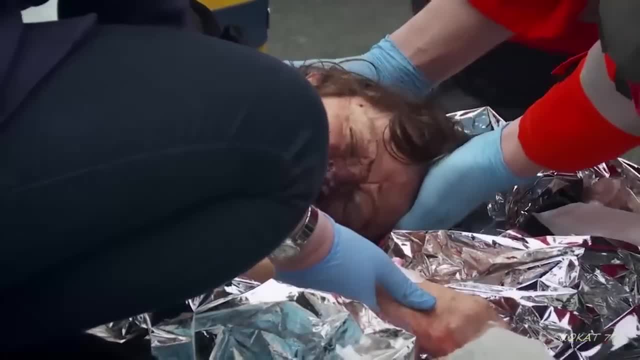 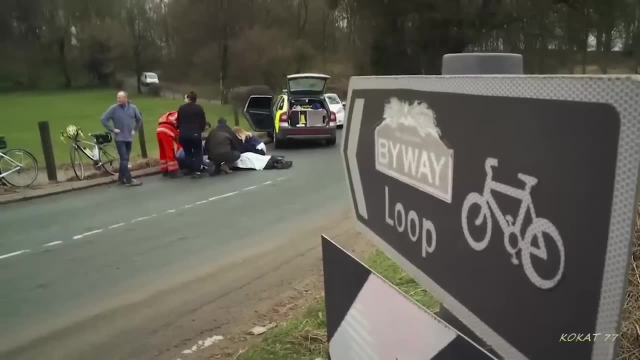 She's withdrawing the pain. Yeah, Karen Corham is critically injured. She was riding down a hill when she lost control after hitting this drainage grate. It seems to match the facial round, the jaw round the nose, left eye closed, right over. OK. 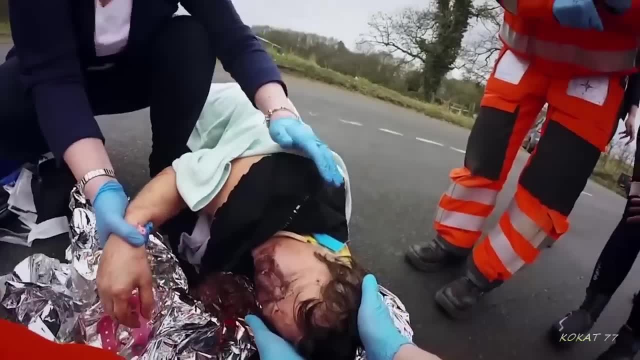 She's probably doing 15.. Did she have a helmet on? Yes, she did. We've taken it off. She's doing 15, 17 miles an hour. OK, yeah, yeah, Your verdict on injuries: Potentially life-threatening. 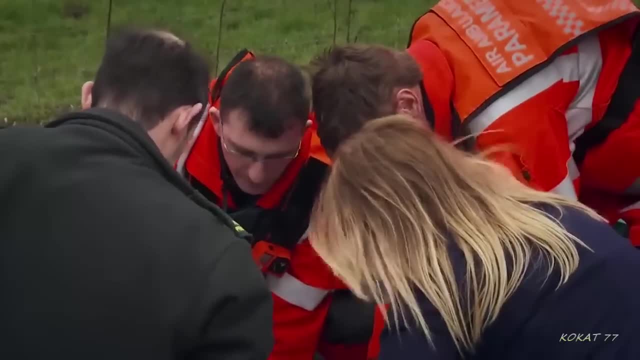 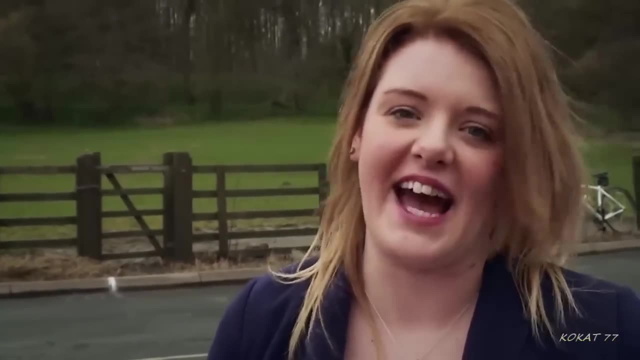 Right, Potentially OK. The accident was witnessed by a motorist. She's put her medical skills to good use- I'm a nurse- so we have to stop and help when we can. What happened when she landed on the floor? 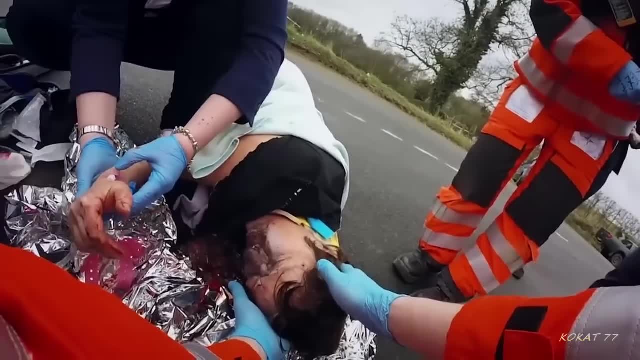 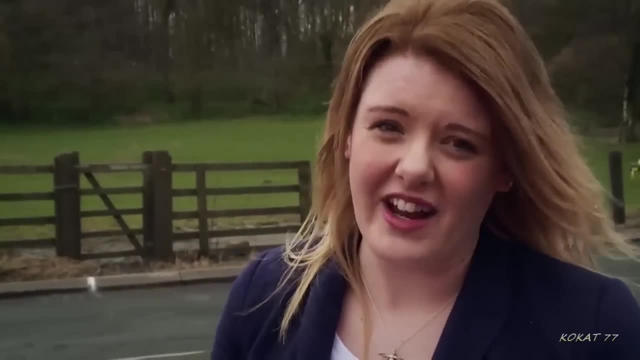 She landed on her back. The bike fell out from under her. I rolled her into the recovery cos she was bleeding quite a lot through the nose as well. Yeah, It was quite clear that she'd got quite a bad head injury. There was a lot of blood. 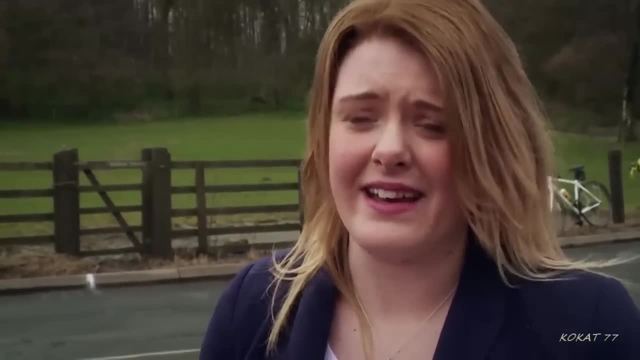 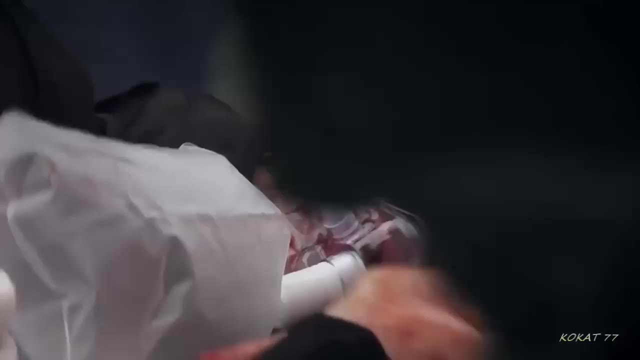 So just worked with the first responder really to just turn her over and get her airways clear. I take it all the blood's come from her head. has it Probably really come from her nose? Oh, from her nose. I couldn't have a look in her nose, OK. 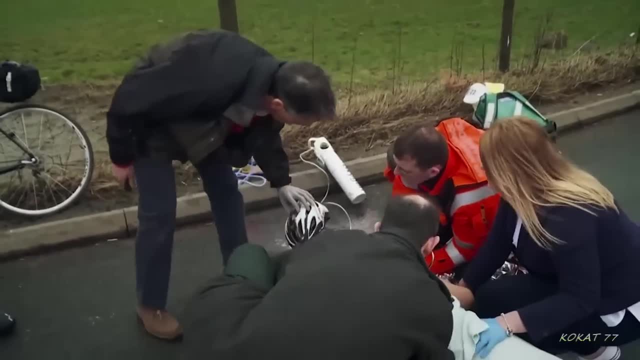 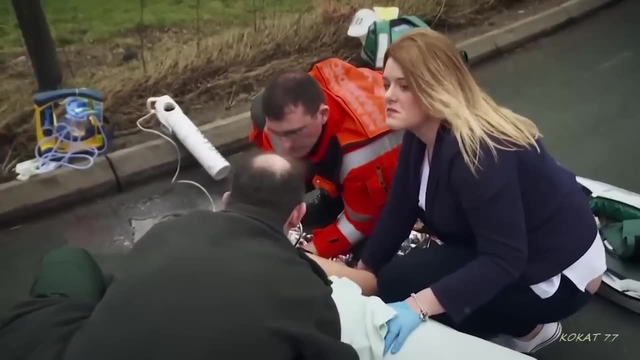 Is there much damage to her helmet? Where's her helmet? Her helmet did little to protect her face. No, there's no damage. where I took it off, I've been up and down her neck and her back and her pelvis again. 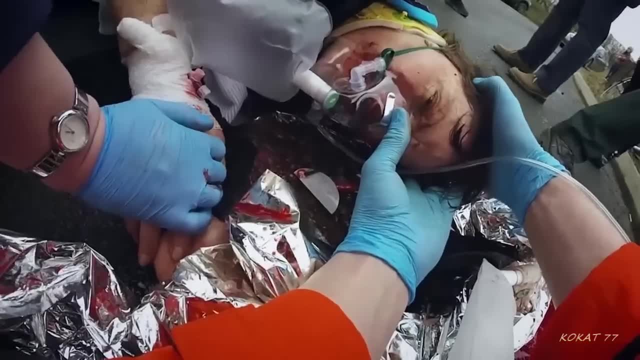 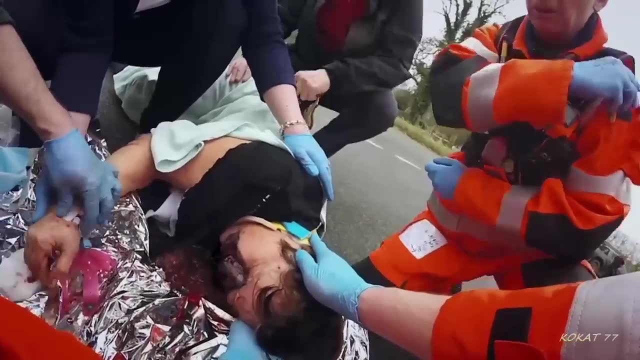 She's not clenched. OK, Karen, open your eyes. Just try and relax. All right, Can you talk to me? Well done, Do you get suction out of it? Oh, just for a minute, Can you use your suction mate? 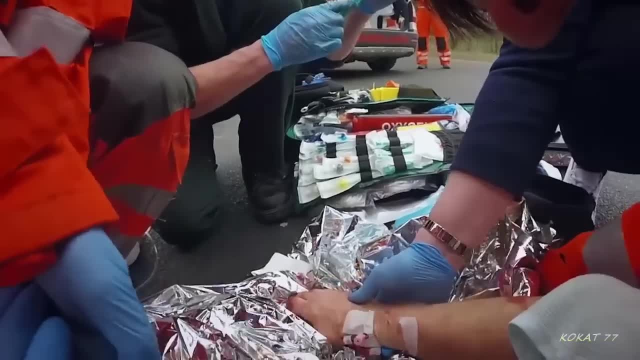 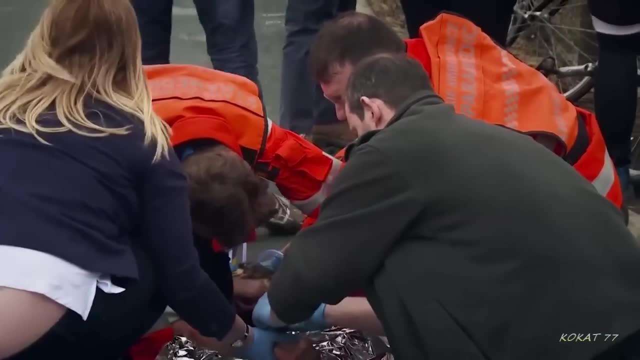 Karen's having difficulty breathing and she's not making much sense. Just reach your mouth, sweetheart. I'm just going to do a bit of suction. Karen desperately needs intensive care. Her husband has driven to the scene. Keep dancing still, sweetheart, just for a minute. 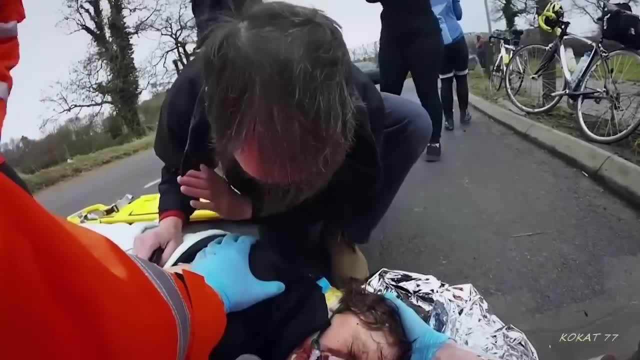 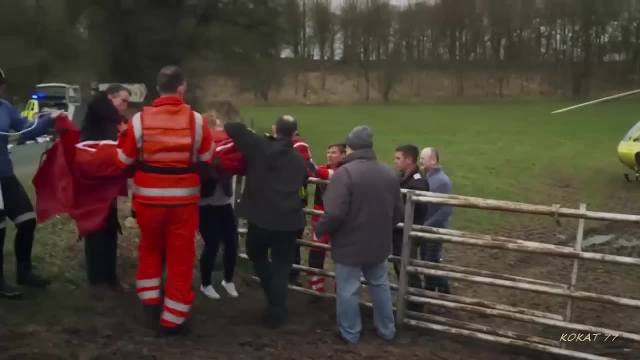 Still, my darling, still I'm going to roll you onto a stretcher. The team has alerted the trauma centre. 20 miles away at Leeds General Infirmary, Lift and slide it on top of the gate. Time is critical. The sooner she undergoes surgery. 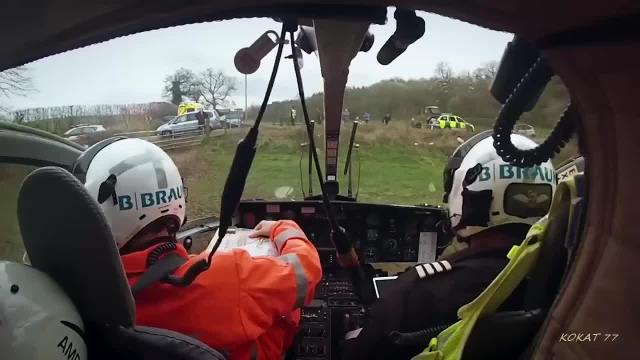 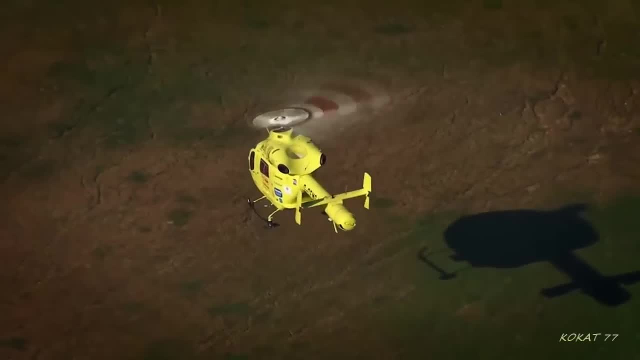 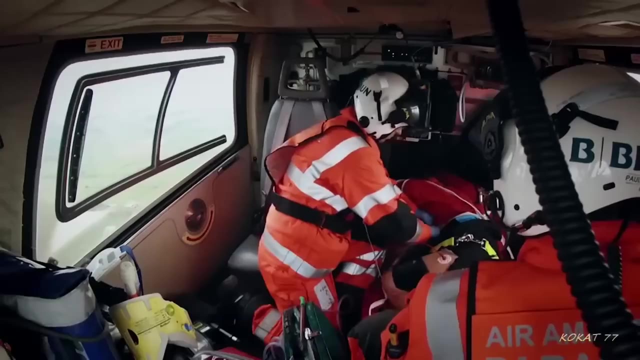 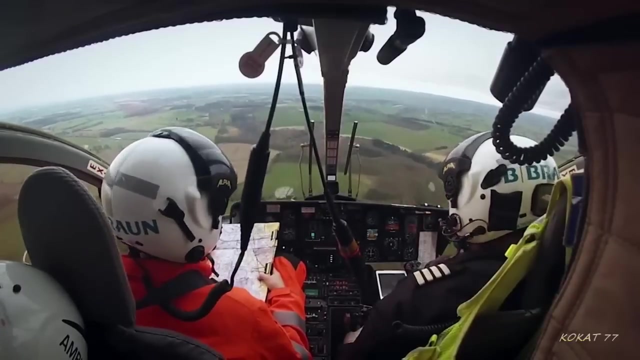 the better her chances of survival. We've just lifted the C routing LGI ETA approximately 10 to 15 minutes over. Both Paul and Tony have their work cut out keeping their patient alive. Her blood pressure is dropping. That horse is getting even slower. 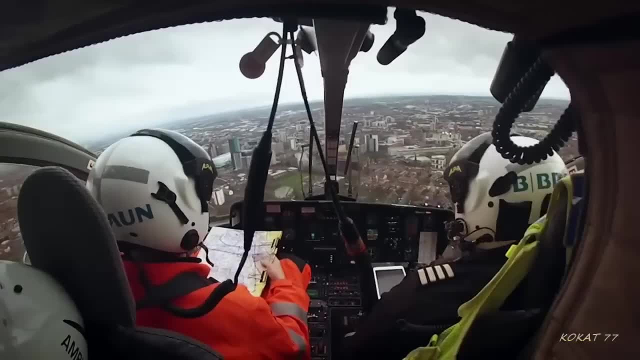 I think we're going to see you soon. That should be nothing. Hello, Ben 9-8.. Our person is letting down an LGI, Don't be a problem. actually, Desk 9-8.. Find also an LGI. 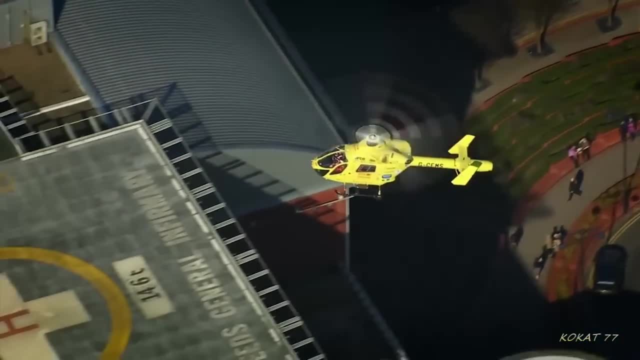 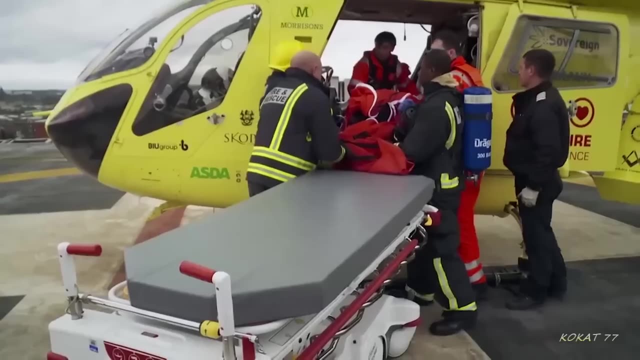 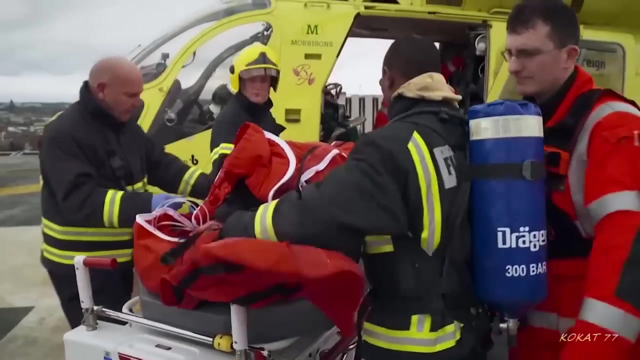 The rooftop landing pad is a welcome sight for the medics. Her life is now in the hands of the trauma team. This is Karen. She's in her 60s. She's a cyclist. Came off the roundabout at quite low speed. 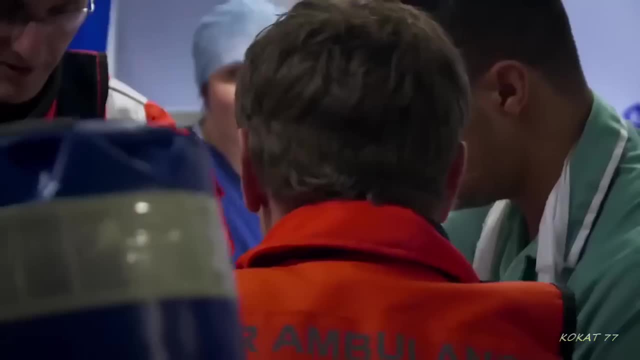 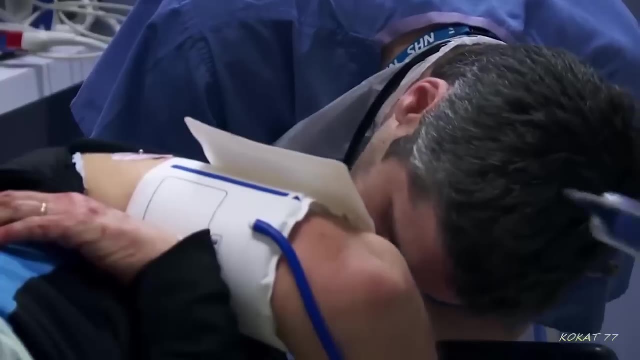 but she's gone face first. She did have a helmet on Face first. onto the ground, Reduced GCS immediately. When we first turned up there was a lot of blood coming from her nose and facial injuries. more than anything else, Neurosurgeons spot a bleed on her brain. 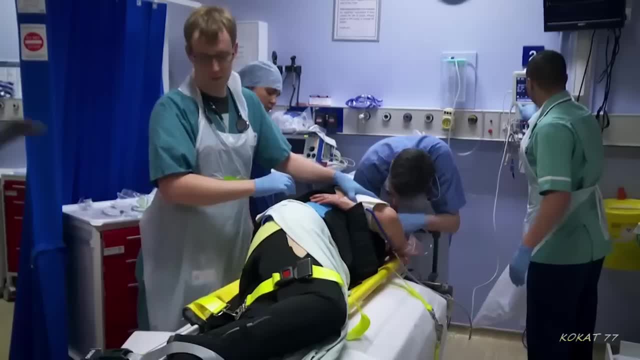 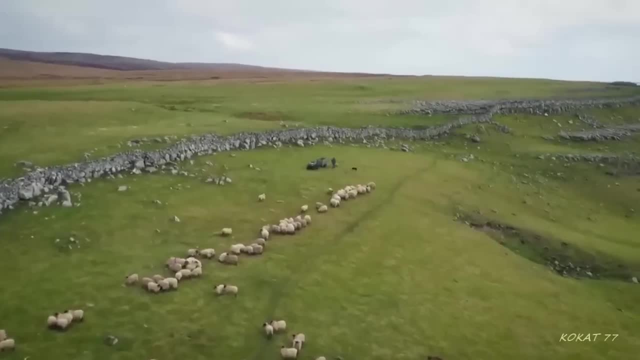 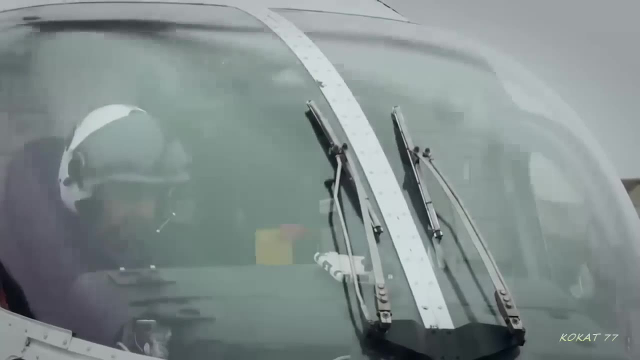 They operate immediately to reduce the pressure. Karen is fighting for her life. For Yorkshire farmers, the local air ambulance is a lifesaver and its crew everyday heroes. Hundreds owe their lives to these choppers and today another farmer's life is on the line. 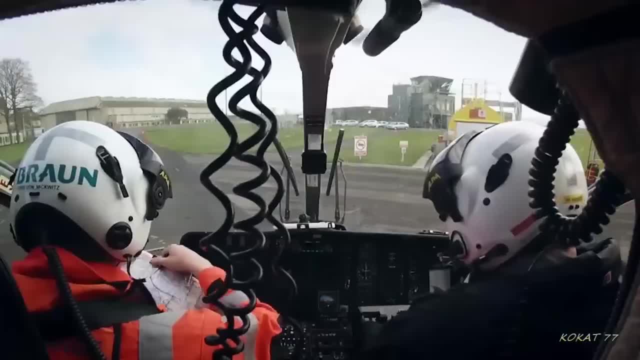 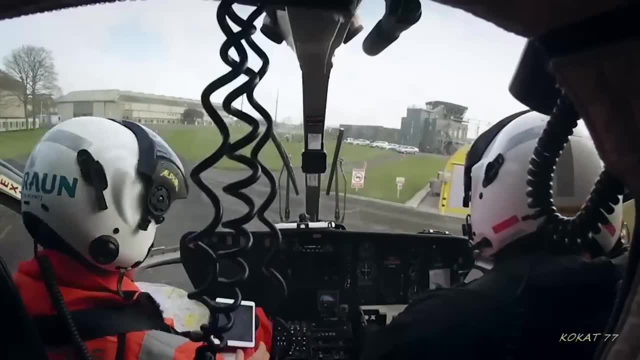 Top of the tower: Animate air 9-alpha Looking to lift outbound Cool Top of the tower. Take us your discretion: 7-10-1-0-6.. Not a field gate: 20-10-2-2.. 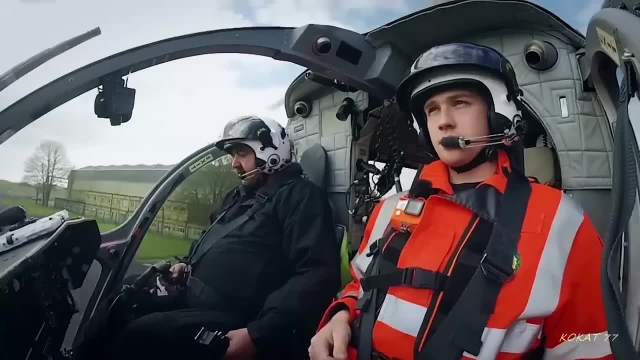 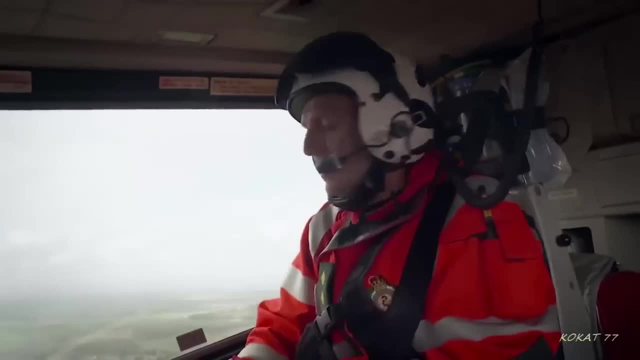 Paramedics, Pete Vallance and Kit von Migwitz are being scrambled to a farmyard accident near the town of Goole: A man attacked by bulls. Kit, what grid was it, please? It was yeah. Echo Yep 569.. 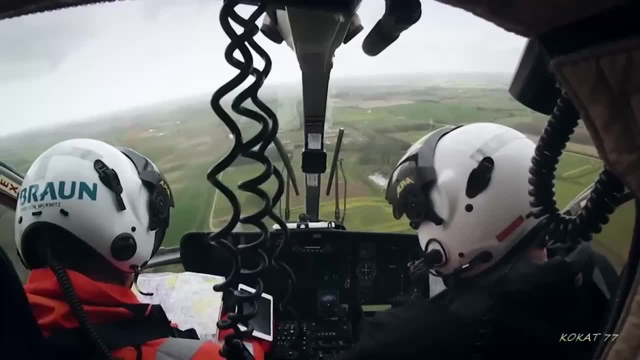 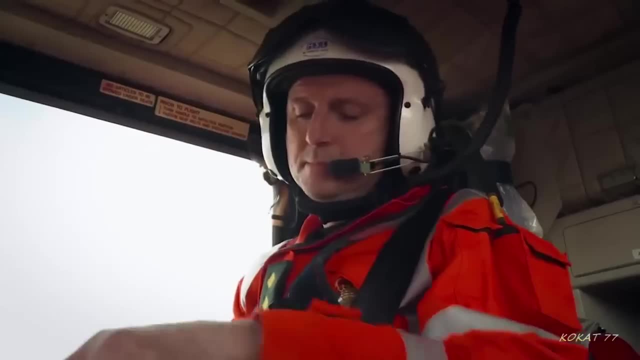 Field 47. And it is right next to Egborough Power Station. Thank you very much. 10-9-9, sir, Information is patient, now out of field And waiting in a silver car. RRV is just on scene. 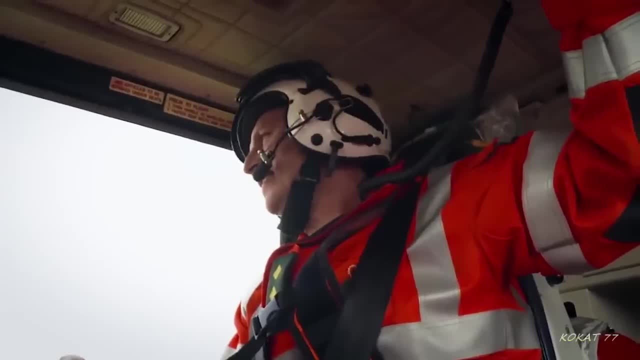 Over. Yeah, that's all received, Thanks. We get called to quite a lot of farming incidents. We've had a lot involving cattle and certainly bulls over the recent years. So farm workers, they know the risk of it. They're obviously working day in, day out with the cattle. 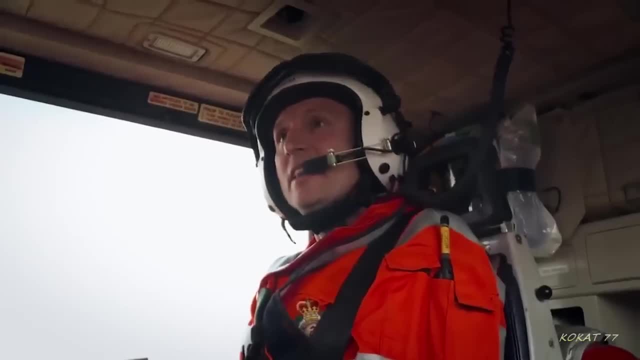 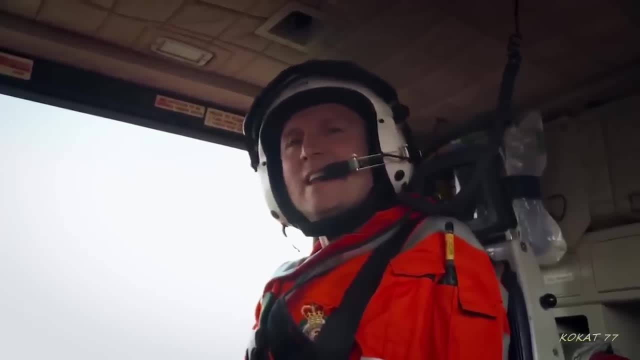 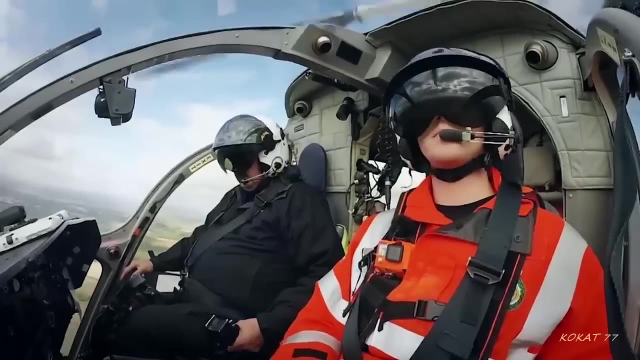 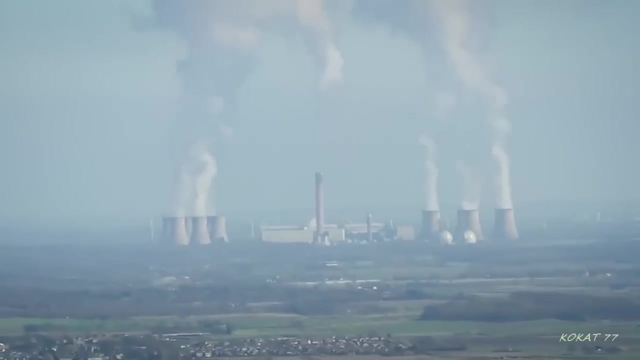 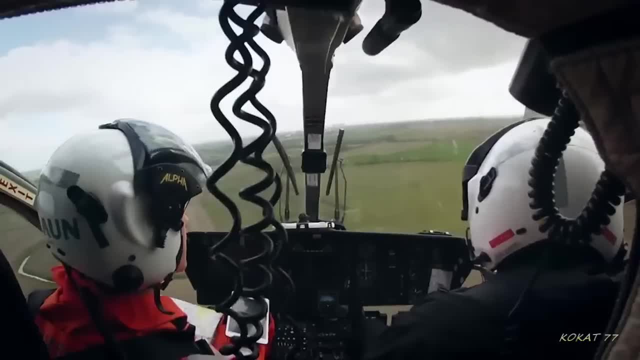 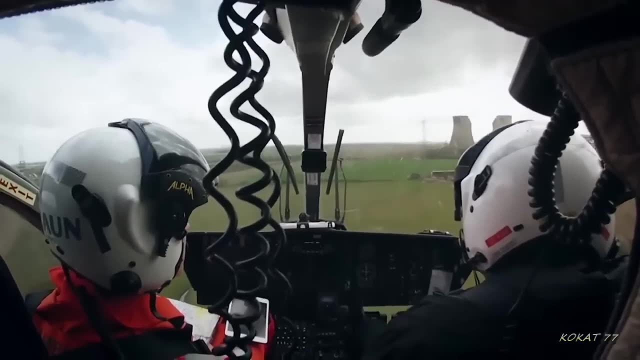 Pilot eon improve set must find a way through a network of high tension cables. Got the small wires to this side of the river, But there's another hazard on his mind. Where's the bull? Was it a shed? Was in a shed, yes. 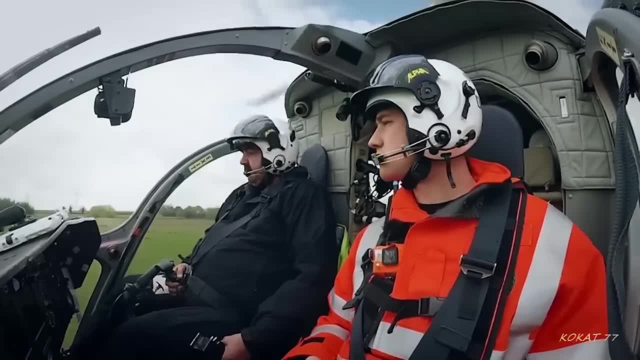 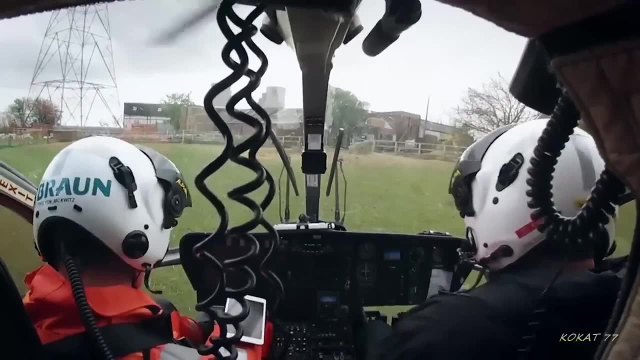 Race Rising ground to the front. Pete, you're waiting for me to stop. OK, I'll wait for you to stop this crew I'm seeing in there That is from 99, landed on city number. Local ambulance crews have reached the farmyard first. 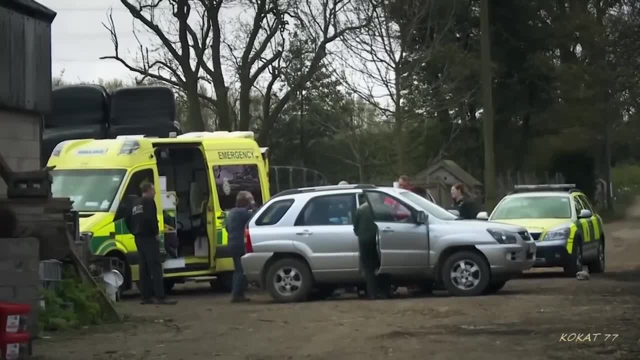 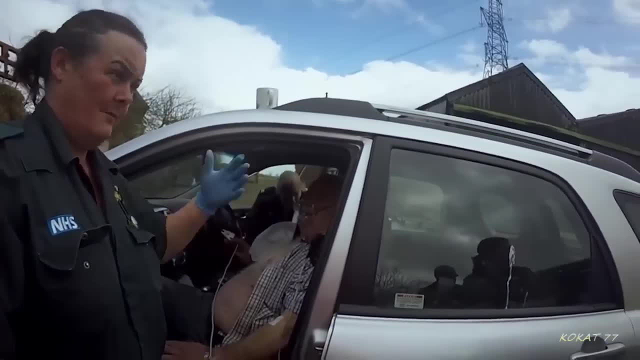 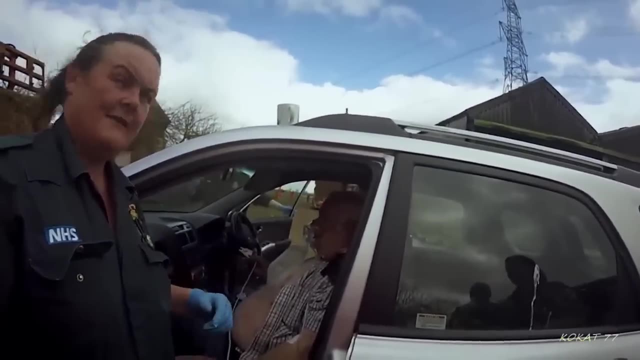 The bull picked him in his bum area to the floor and then it's proceeded to kick him in the chest And head, Headbutting- sorry Farmer. Tom Lancaster is lucky to be alive. His chest was crushed by an animal weighing close to half a tonne. 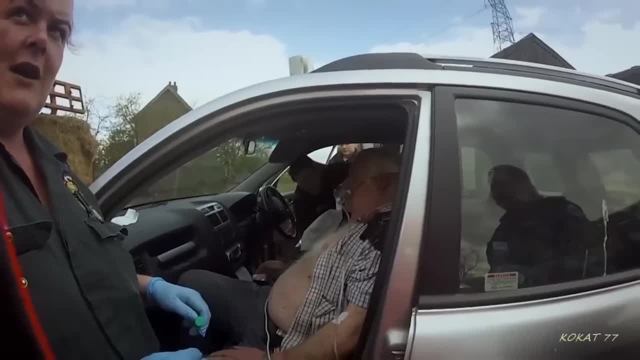 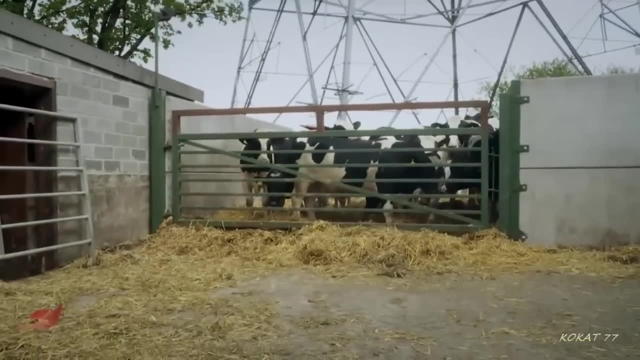 What's your score now out of ten? pain-wise, I've not asked him to be honest, but knowing him it'll be a little two because he's a hard-on farmer. Tom was feeding his herd of young bulls when he was knocked to the ground and trampled. 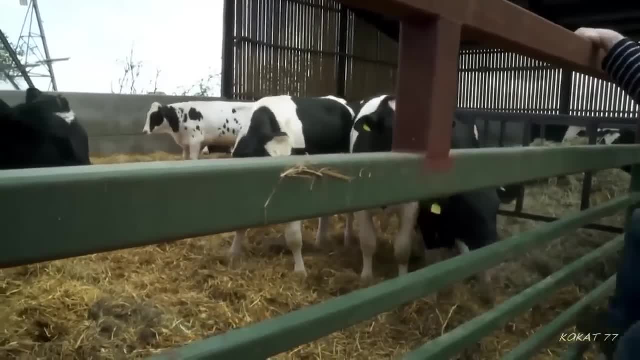 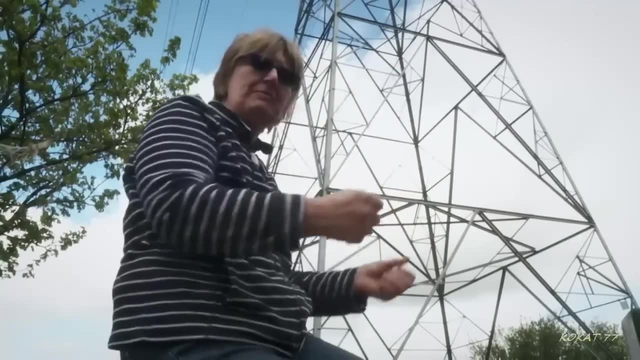 Neighbours found him bloodied and badly hurt. He was actually bent down, so he didn't see it. It hit him up the bum, Booted him up the bum And then, of course, it knocked. And it's been hitting him on this side. 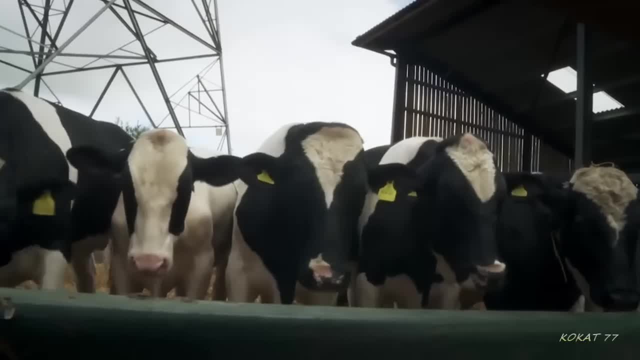 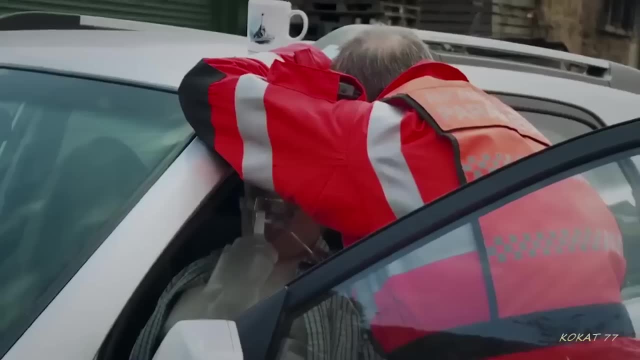 Not just once. apparently it's been hitting him a lot. Bulls are often bred for beef. They grow faster, but they're also more aggressive than cows. Is it normally bad-tempered, then, or have you just cut it on and off there? 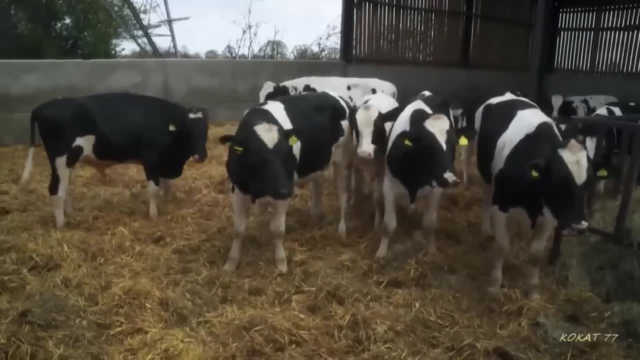 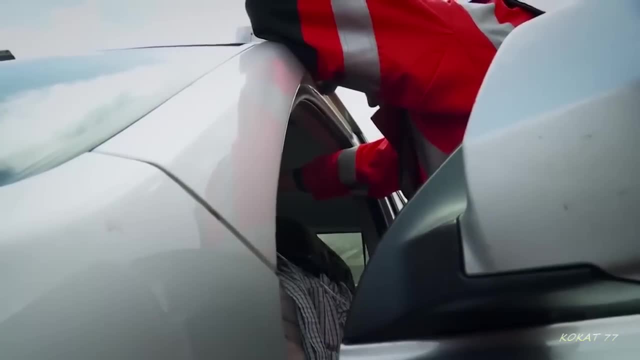 Cut it on and off. there Have you, So you can recall everything that happened. I can, yeah. And you got yourself up and walked out here. He knocked the phone out of me on three turns, Yeah. So you were in a bad mood then, yeah. 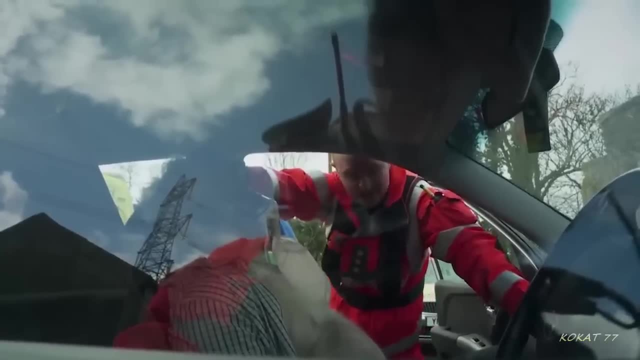 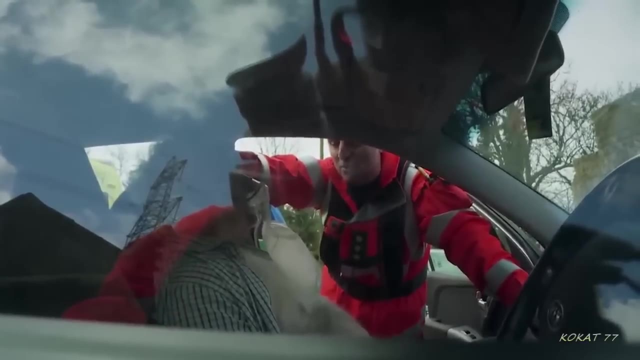 Yeah, So we'll get our trolley out, we'll put it at the side here and we'll ask you to step out, nice and steady, and then we'll just try and get you down and keep you as still as we can as we go round. 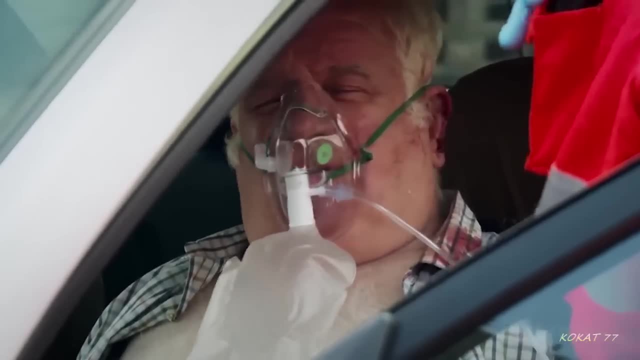 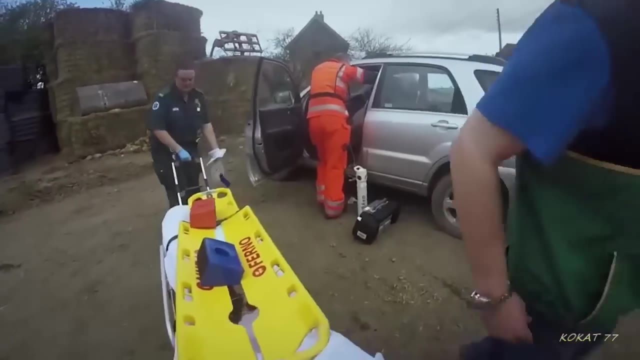 His farming neighbours are shocked by the attack. I've known Thomas for 22 years and I've never known him be hurt like this with cattle. He's worked with them all his life. you see, Pete fears Tom may have a neck injury. 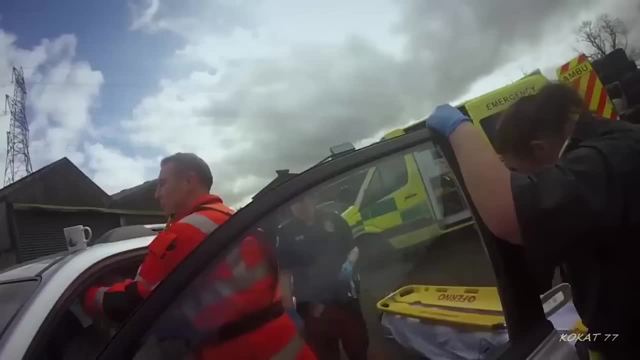 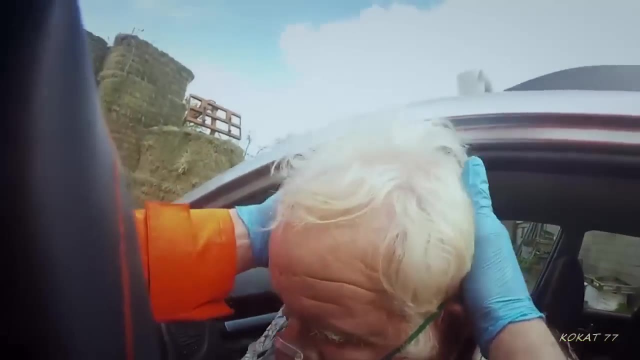 And he could be bleeding internally. Keep your head still. There's a bruise on the roof. Is that for the crew Right, bring this leg round and tuck the floor for me, that's it. Before we move. anyway, just stand a minute. 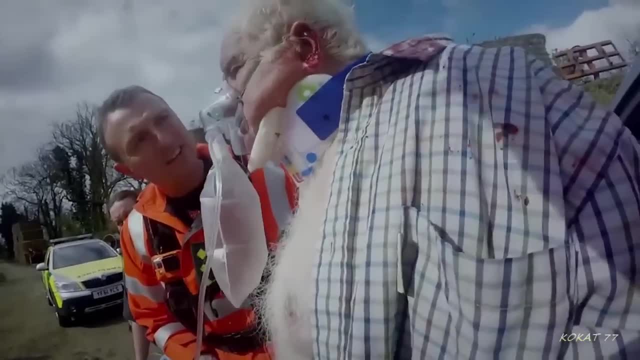 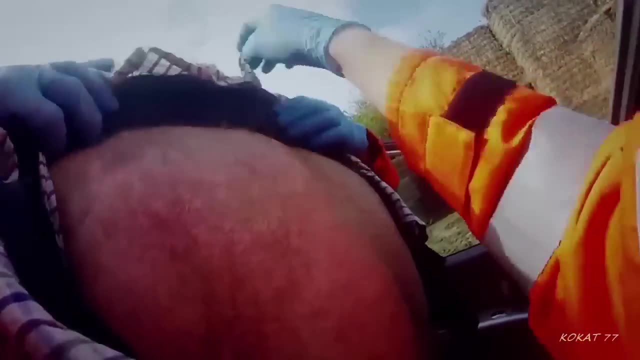 Okay, Where's that hurting? Can I have a quick look at your back? Is that okay? There are clear signs of the attack on his back, but no sign of bleeding. Big, big bruise left shoulder, left chest, Same on the right, just there. 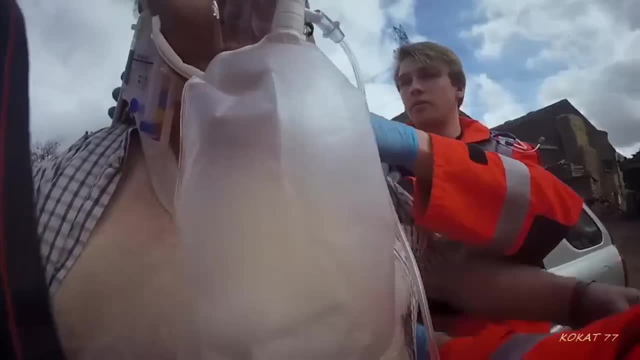 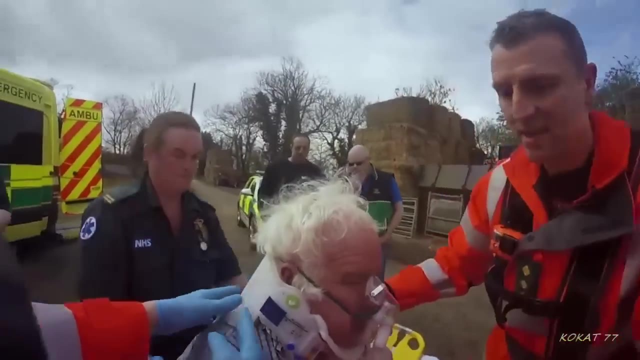 All right, come towards me, Thomas, and then turn round. okay, We'll just get you sat on edge. You might feel it tilt a bit because it's a rigid board. They're going to strap Tom to a spinal stretcher. 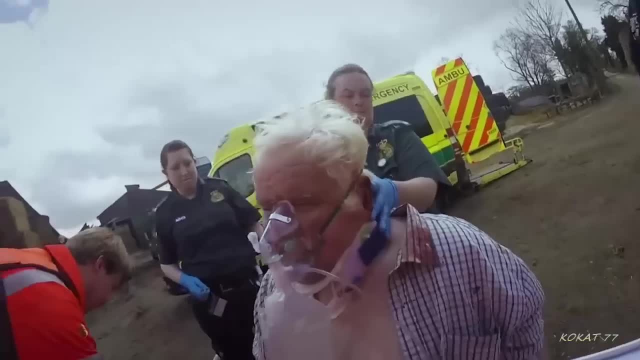 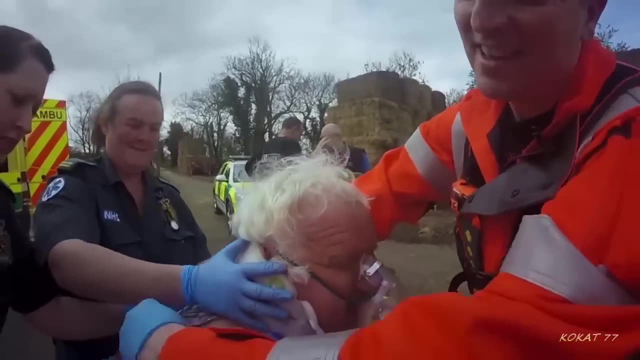 Happy there. yet All right, we want your feet down this end. It's not your best shirt, is it? It was, Oh, go on it'll, We might get it off then We've ruined his jumper. He wasn't happy about that. 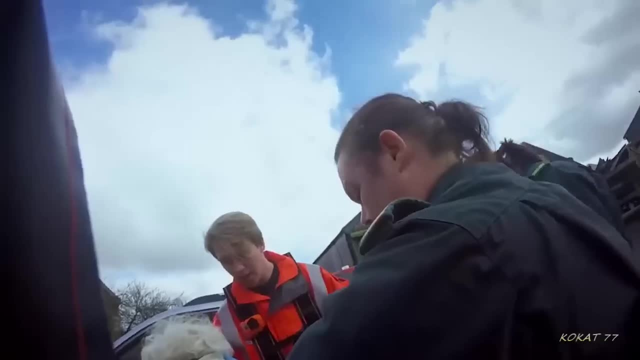 Keep your head still. Tom, Can I just help you, help spin you. If Pete helps you from behind, I'll help you with your legs here and we'll just do it all in one. okay, Are you ready? Super? 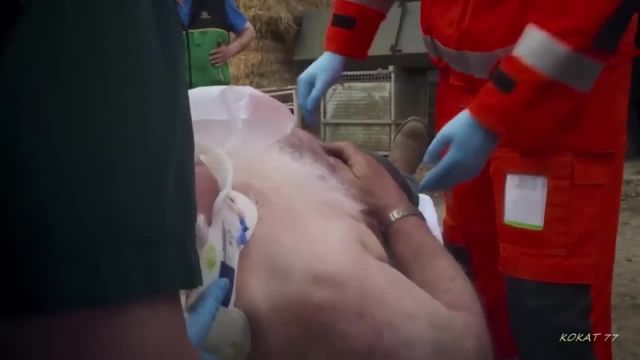 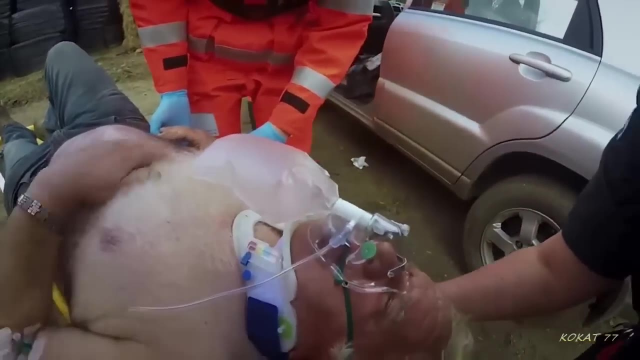 There we go A little blanket. Only now is Tom showing signs of pain. We can get a bit more pain relief, Is that still not? Oh no, I won't prop it up, You just pull it on there. All right, just bear with us one minute. 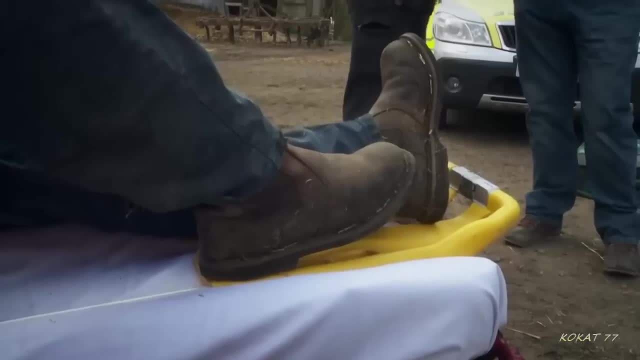 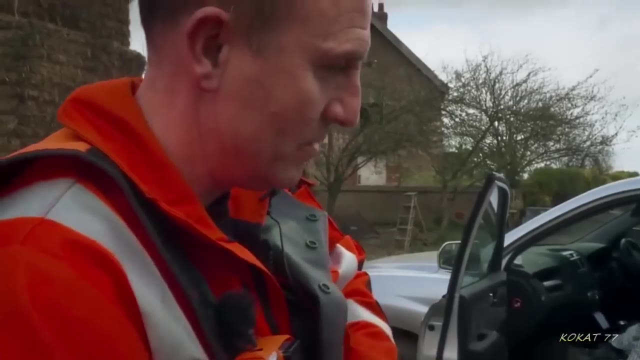 Let's get a bit more pain relief. Oh no, Let's get this morphine in. That's great stuff. We've got Thomas settled in a fashion. He's got what looks to be some rib fractures. He's got quite extensive bruising across his back as well. 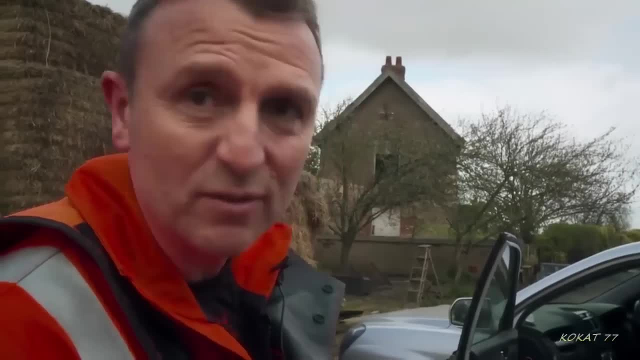 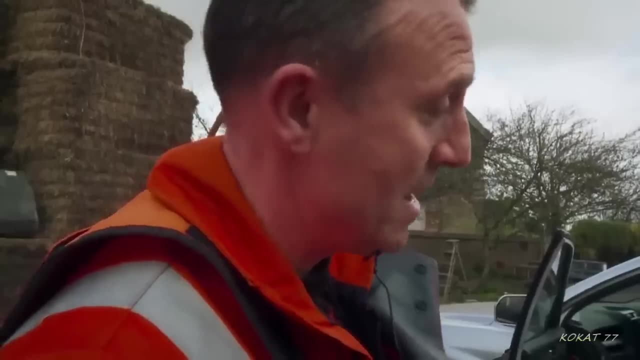 So we don't know if there's any other internal injury yet taken place. He's fully alert and his obs are good at the moment, but initially his oxygen saturations were low, hence him being on oxygen and taking precautions immobilising him. 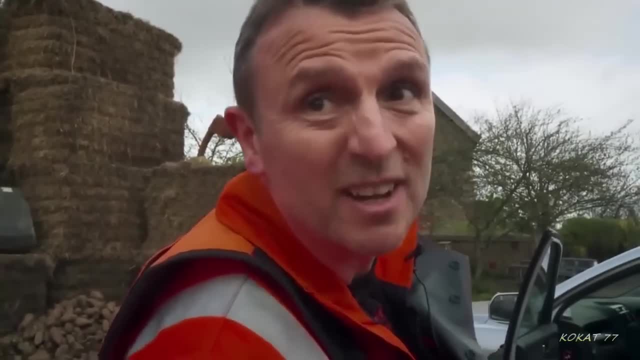 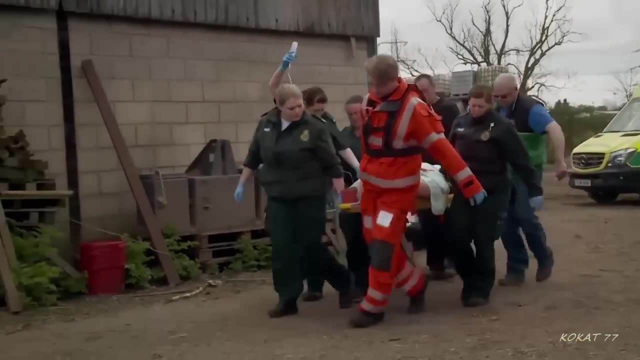 So it sounds like the bull's had two or three goes at him and caused what could be significant trauma. The team's flying Tom to the major trauma centre 20 miles away in Leeds, but their patient isn't keen. He absolutely hates it. 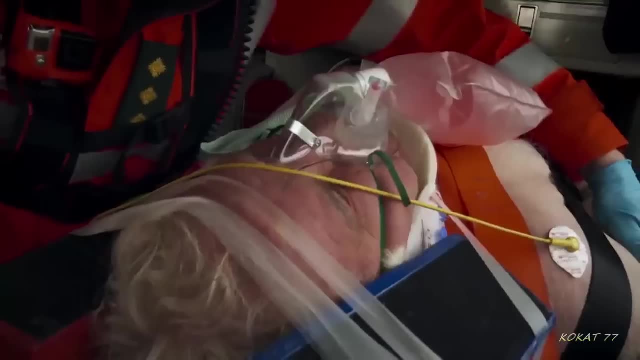 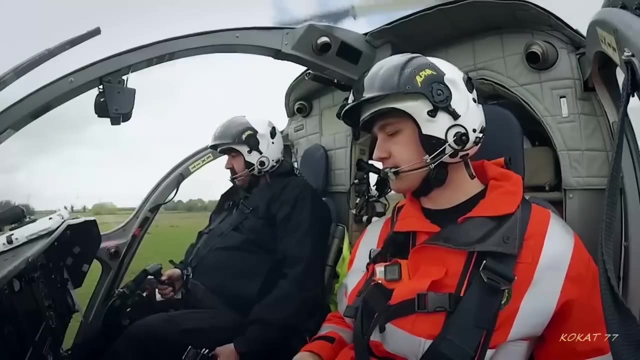 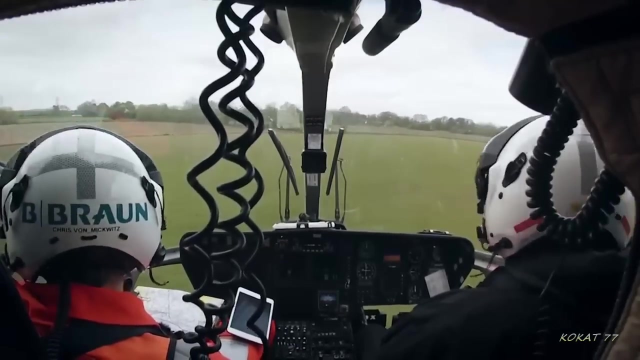 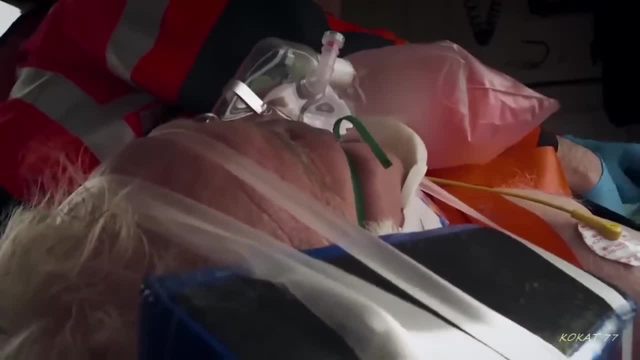 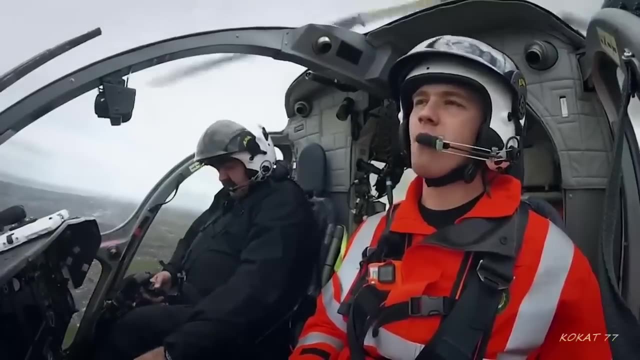 that might deteriorate later on. His breathing has now improved. NMN 99 Alpha. your new QNH is 1024.. 1024, thanks. NMN 99 Alpha. Tom is already booked in for scans and X-rays at Leeds General Infirmary. 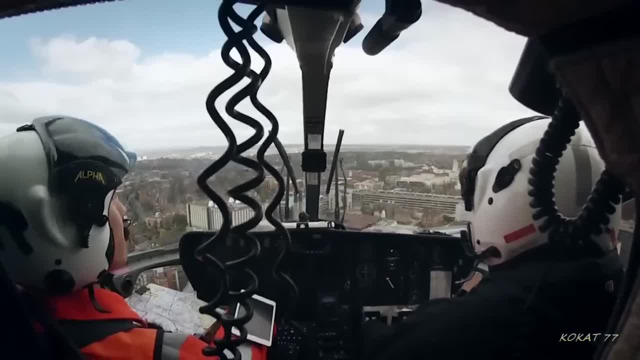 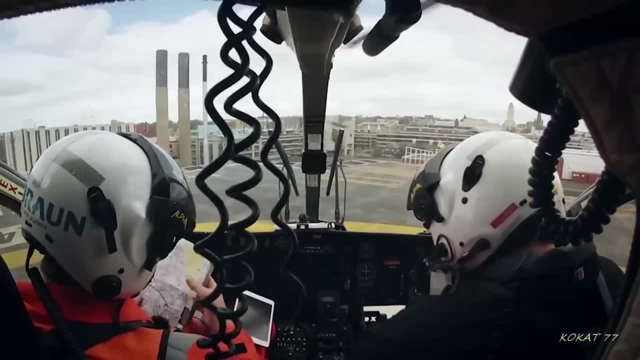 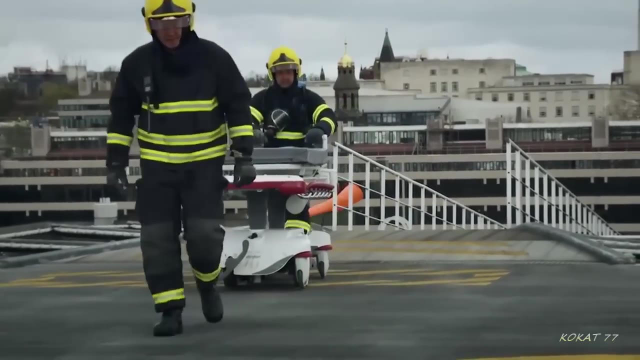 OK, 1024, that's 500 feet. That's good Coming on down. Here we go, Helmet on. It's taken just 10 minutes to fly him from Farmyard to the heart of Yorkshire's biggest city. Did your breathing feel any easier? 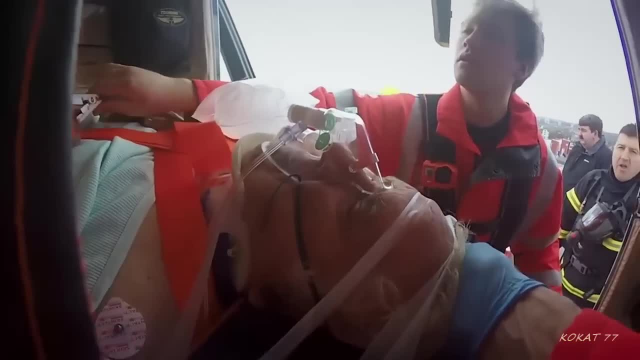 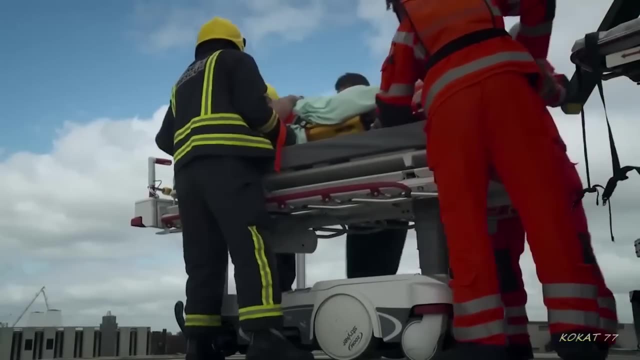 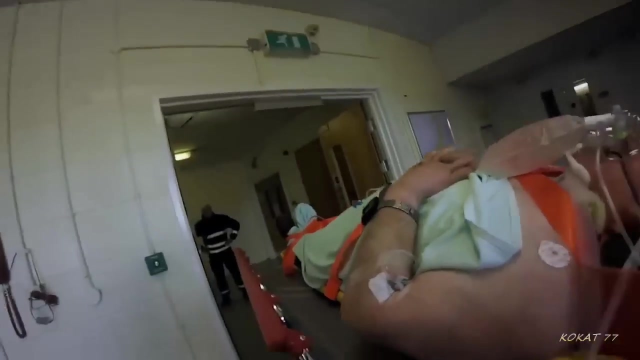 It feels a lot better, Does it? Apart from where your ear's bleeding, you've got no pain around your head at all. No, What did you think to your first flight then? It was all right. Your mates were saying, he'll never get in that. 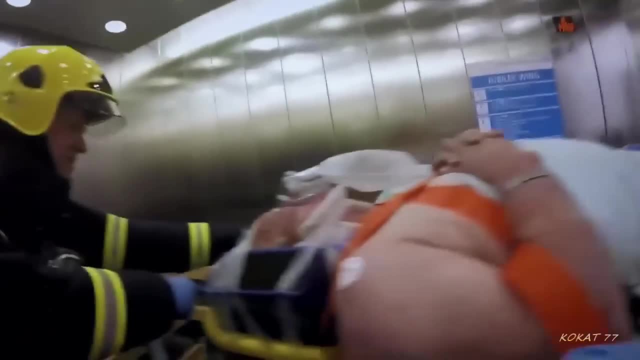 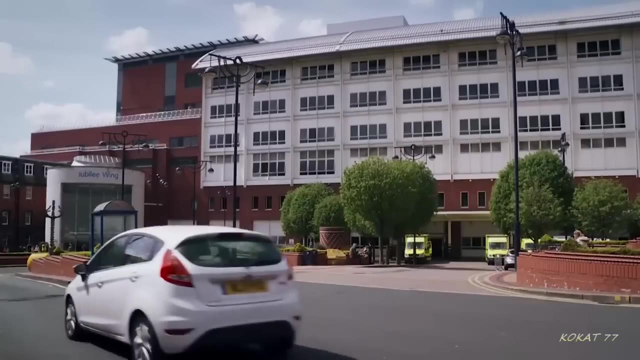 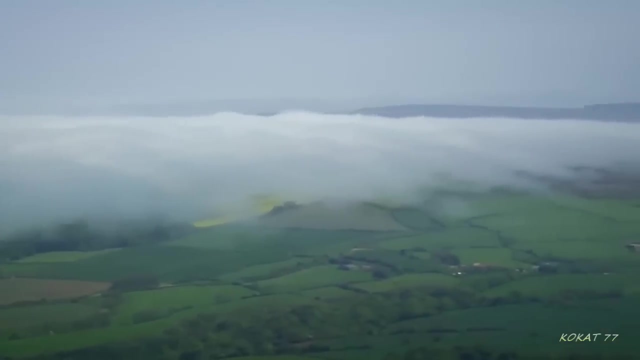 He don't like flying. I said the wrong thing, didn't he? I think it's a bit late now. All right, Even if the results are good, it could be some time before Tom is fit to return to his cattle. Helimag 99 is fighting through low cloud. 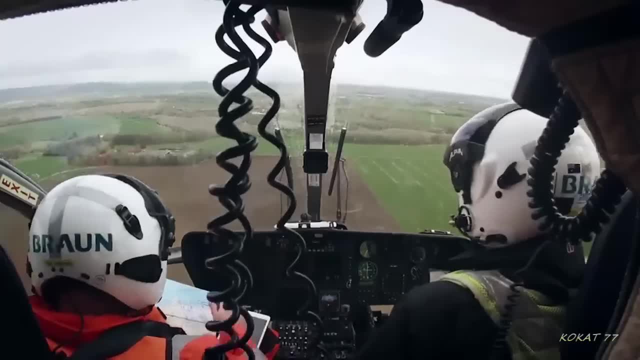 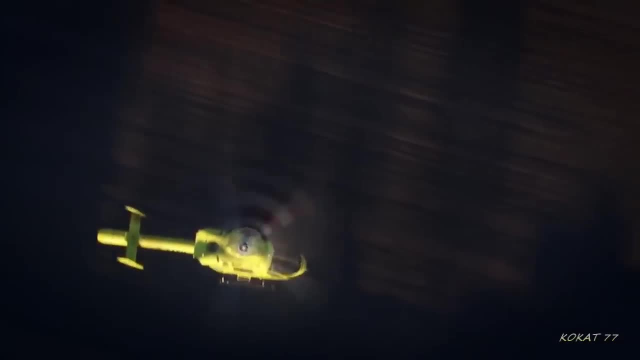 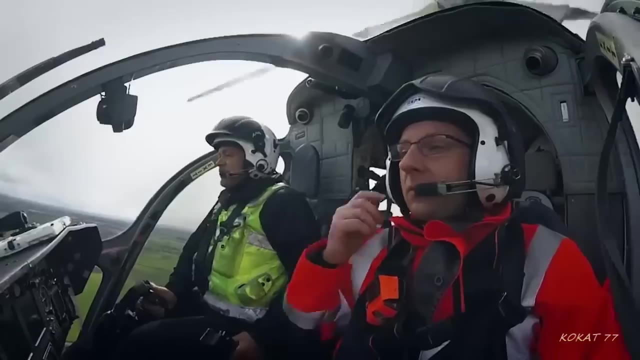 heading for the Yorkshire coast. A bit of weather on the way there, guys. Their mission is critical. A woman's life is at stake, Roger. Update from scene. The patient is GCS3. Over, OK, And the weather's clear. 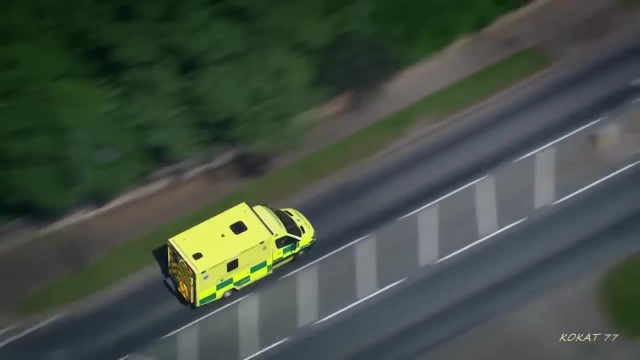 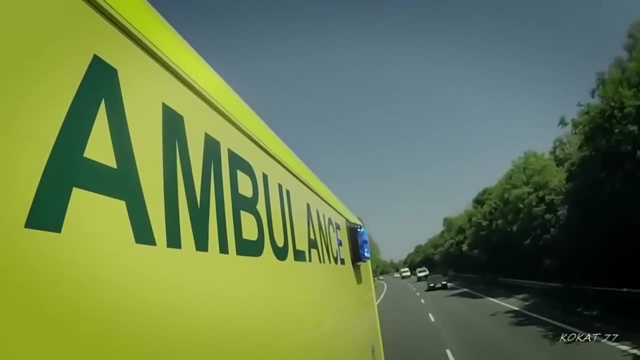 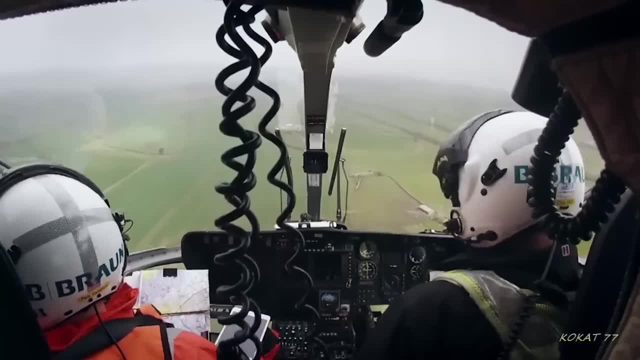 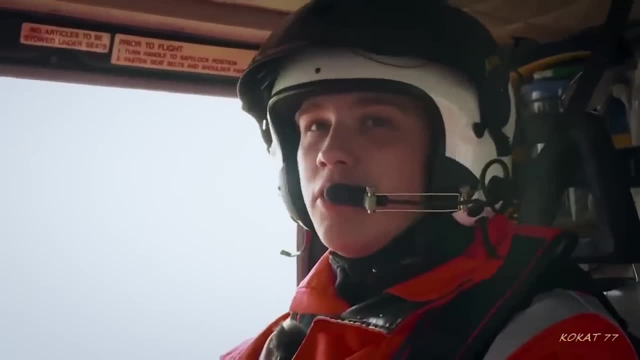 OK, OK, OK, OK, OK, OK. It's weirder than anyone I've ever seen a serious call at the moment. We've been told that lady's fallen off a ladder with a potential head injury. I know she's completely unconscious at the moment. 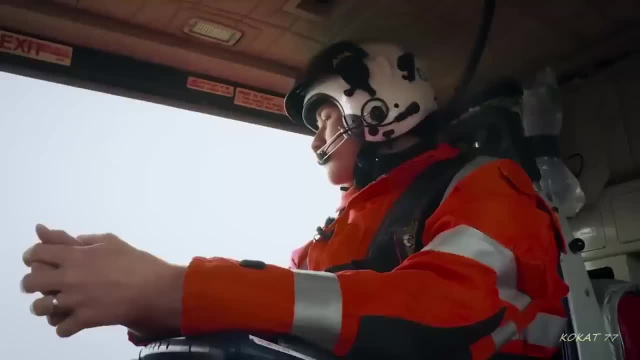 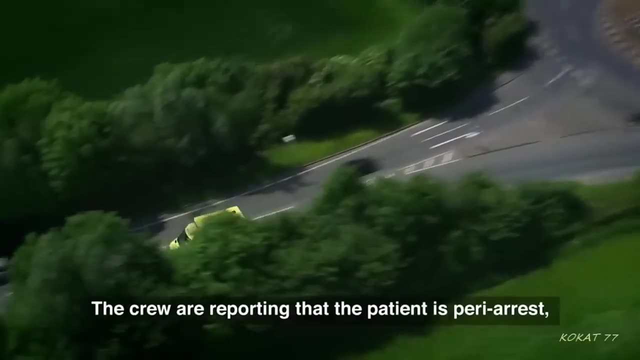 It's feared she has a brain haemorrhage. Paramedics John Baxter and Kit Von Mickvitz know Helimag 99 may be the woman's only hope of survival. The two were reporting that the patient is peri-arrest. Prior to that they were reporting that the patient was quite combative. 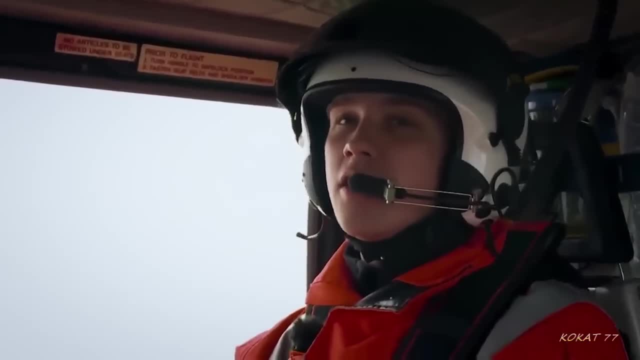 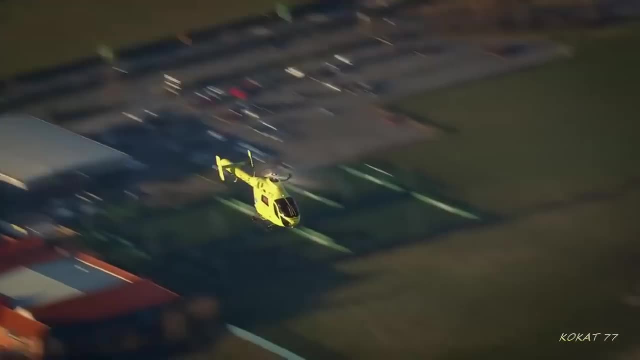 They're concerned that she is going to have a cardiac arrest or that her heart couldn't stop because her injuries are so severe. She could have the bleeding within her head or a different type of severe injury. We're making it seem as quickly as possible now. 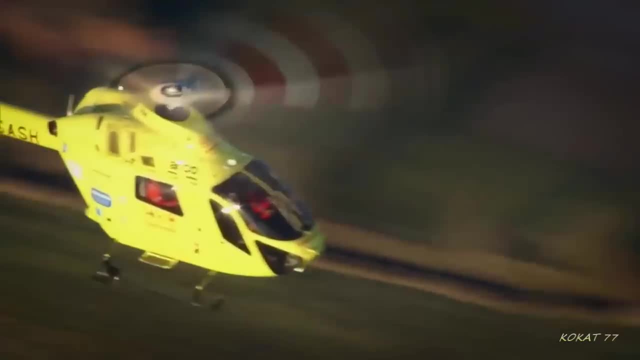 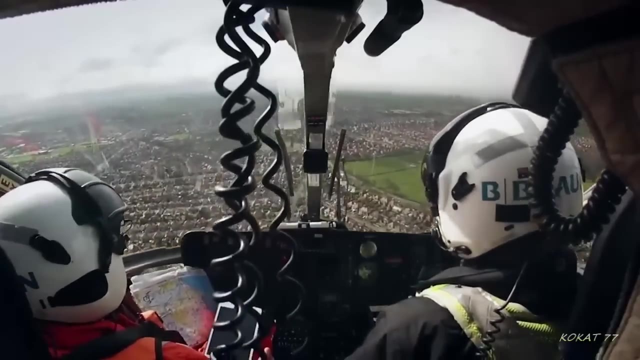 Time really is important. At least they're now through the low cloud. I think I've got Brindleton mate. Is that the road crew coming down past the trees? Is that them? Yeah, Yeah, that's them, yeah. 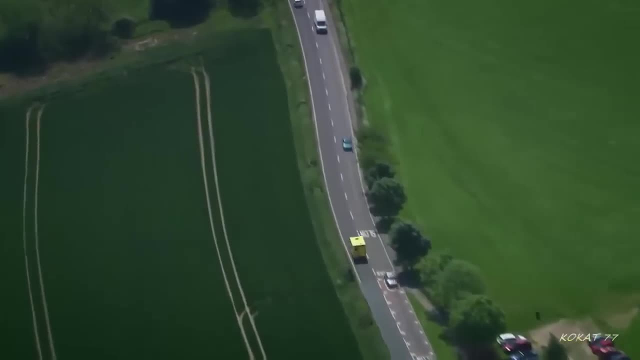 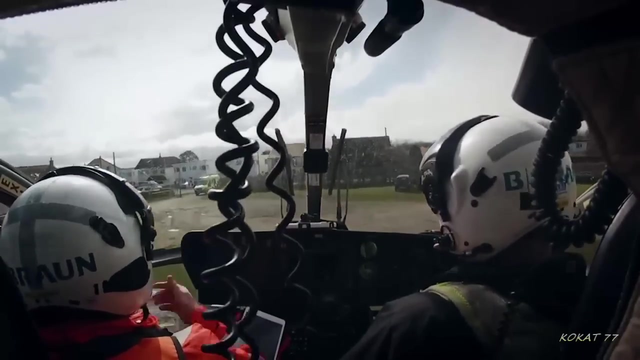 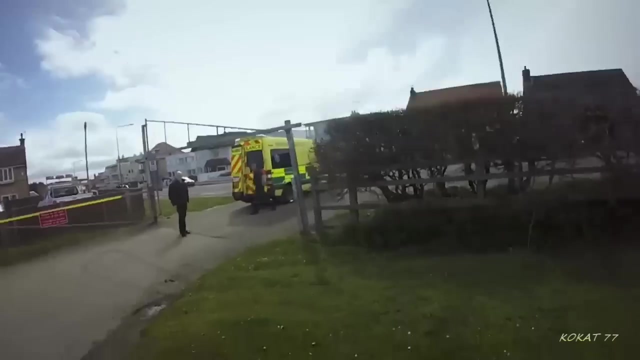 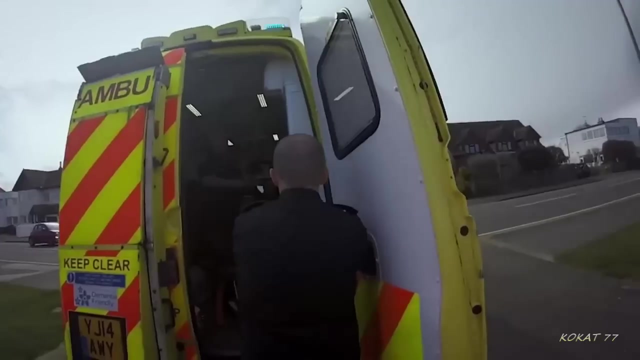 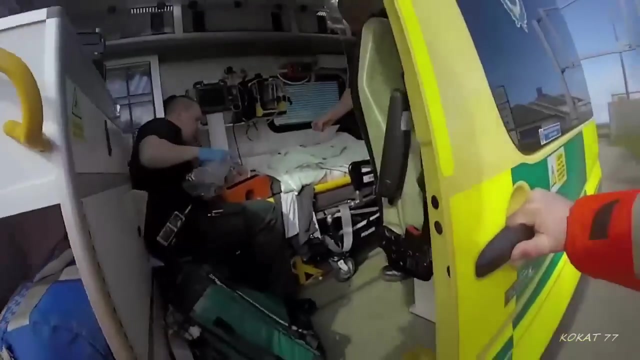 Got it. They're arriving at the same time as the ground crew who found her. Linda Parsonson went out to trim a hedge in her back garden. Minutes later, her husband found her lying unconscious. She's critically ill. Hiya, I'm Kit, one of the paramedics. 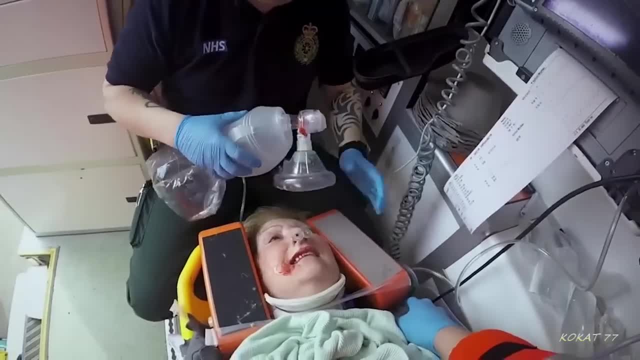 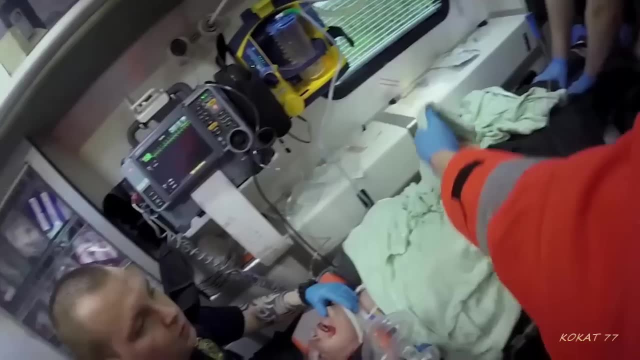 What's her name? What was it? Linda Linda's agitated It could be a sign of brain damage. Kill pose with a pinpoint Right. A little access in this hand, Lovely. So we've got another aircraft coming as well. 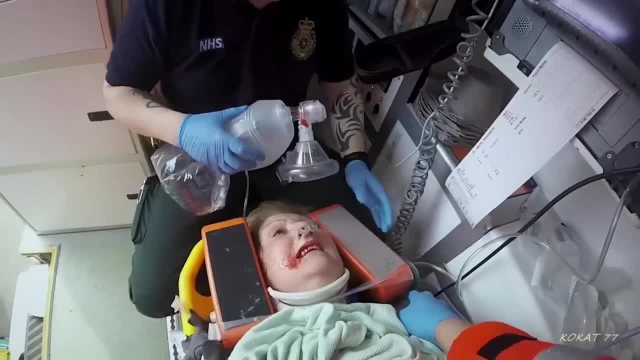 We're going to probably be putting her off to sleep with an anaesthetic- emergency anaesthetics. In the meantime, we'll just try and get her as comfortable as we can and see what we can do for her. OK, All right. 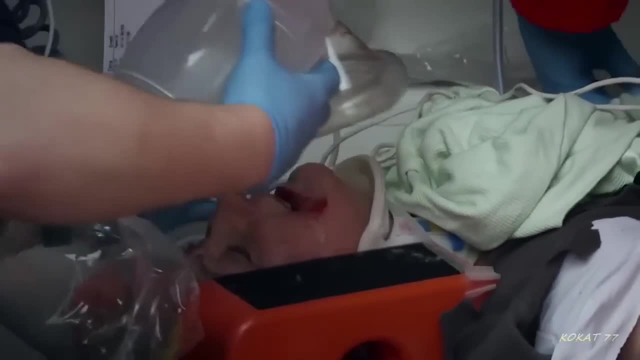 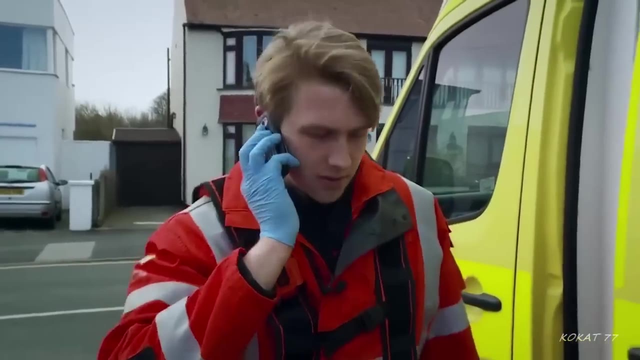 Kit wants to give Linda a powerful sedative. Ketamine will calm her down, But its use must be authorised by a senior ambulance service doctor. Hi, Steve, Sorry to bother you, It's Kit, one of the paramedics on Helimed 99.. 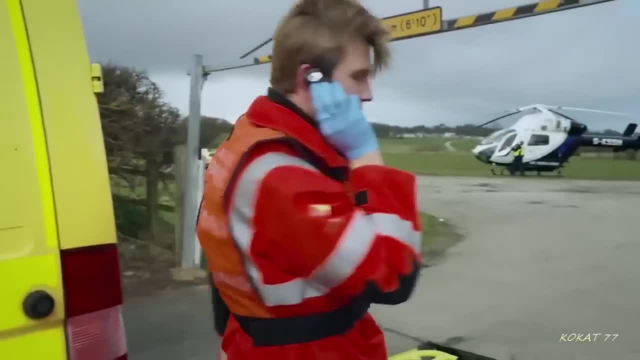 We just wonder if you're OK with us giving something just to settle her down and if you can get her sets up a little bit and stop her being so agitated. Fab, All right, Thanks very much for that. I'll speak to you later. 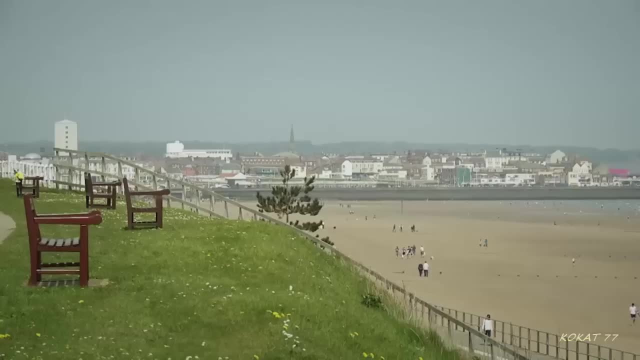 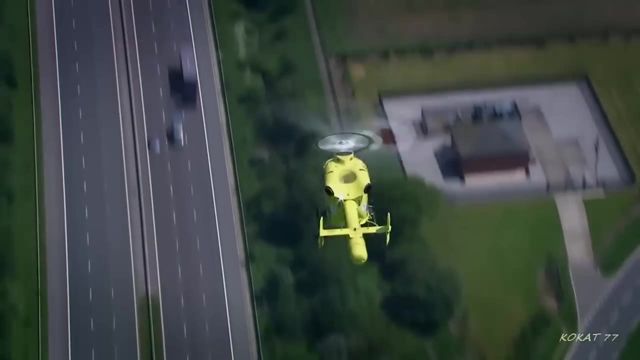 Cheers, Bye, then. Bridlington is at least half an hour from a major trauma centre, But the most important part of that is coming to her. The second Yorkshire Air Ambulance, Helimed 98, is carrying a consultant who will be able to anaesthetise Linda. 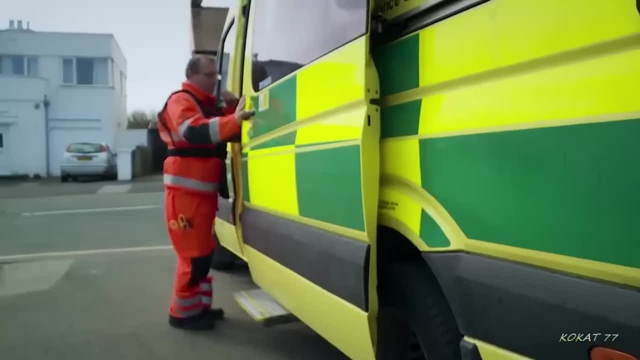 and help her Before her flight. Can you set up a kit for an RSI please? Sir John's setting up for an RSI, so as soon as they arrive, hopefully we'll be able to pop her off to sleep. 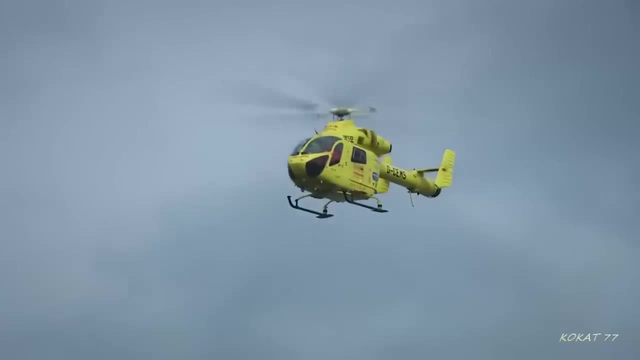 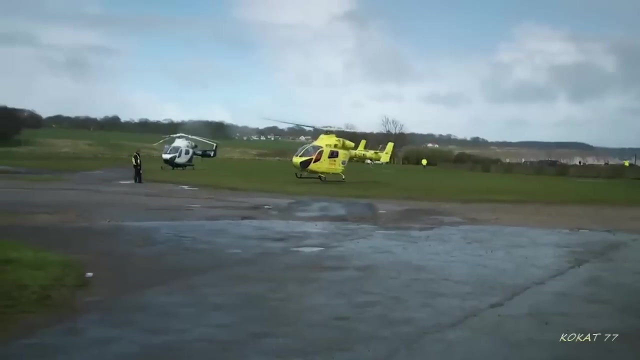 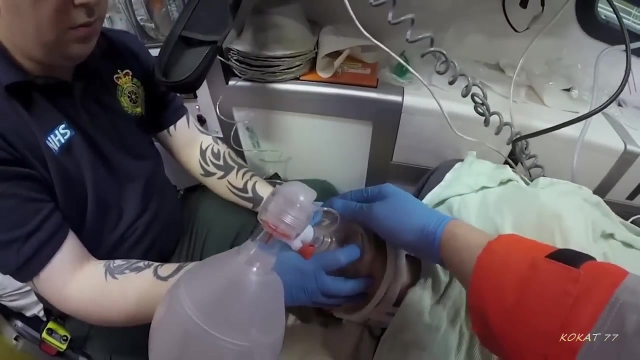 Yes, Linda, Relax, sweetheart, All right. Two helicopters, eight paramedics and one of Yorkshire's most experienced trauma consultants are now focused on saving Linda's life. Linda, can you squeeze my fingers for me? She's just making that constant groaning. 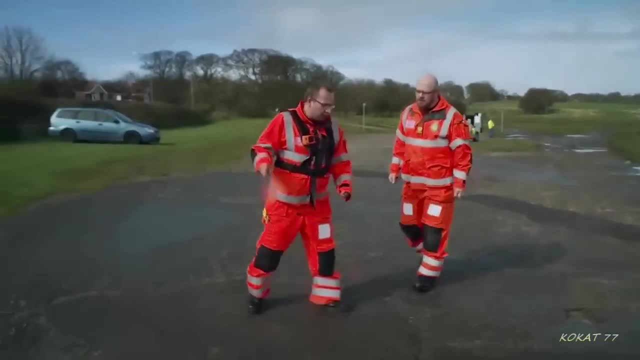 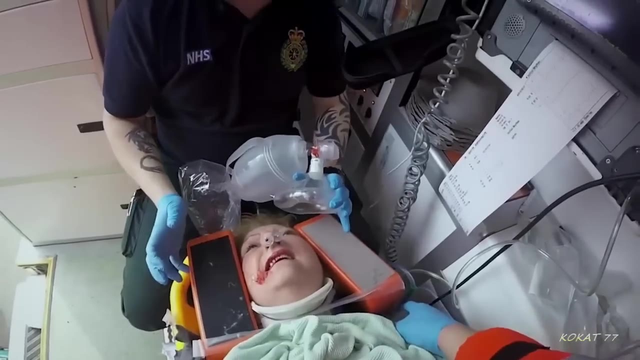 Hello Andy, How are you? Dr Andy Poutney is arriving to perform a high-stakes medical procedure that's risky even in hospital. Her survival will depend on its success. At the side of the road in the seaside resort of Bridlington. 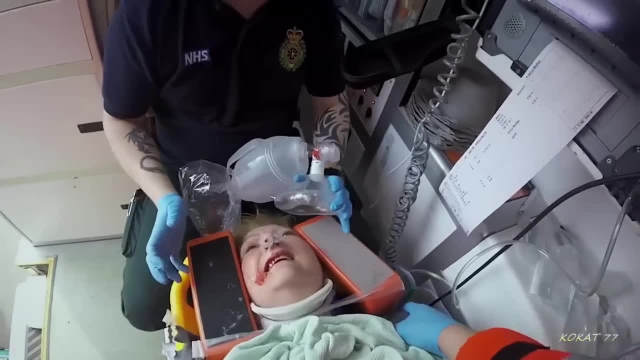 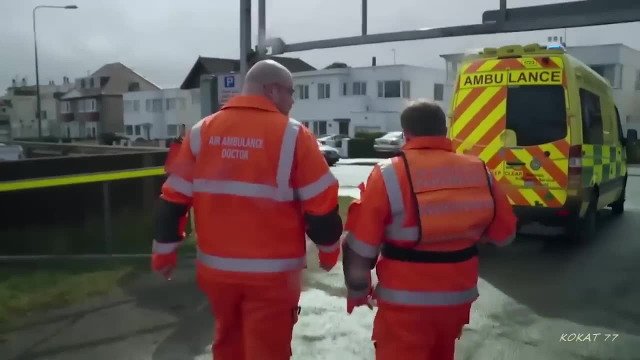 a medical team is preparing to anaesthetise Linda Parsonson. She's been found at the bottom of a ladder. We're not really sure if she's fallen or not. It's less than half an hour since Linda was found unconscious in her garden. 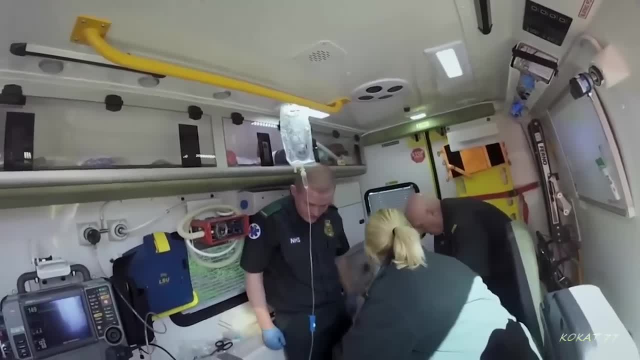 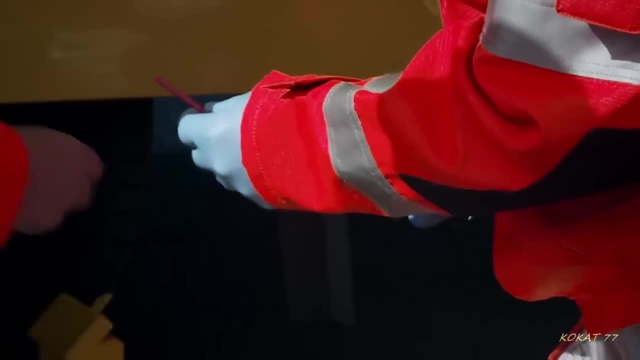 It's feared she may have a massive brain. We're going to pop her to sleep in the street out there, just where it's a bit more easy. Just grab a 20ml syringe for us. We've got size 6,, size 7,, size 8 ET tubes. 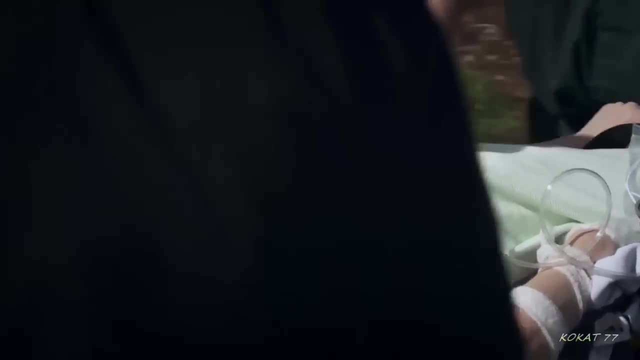 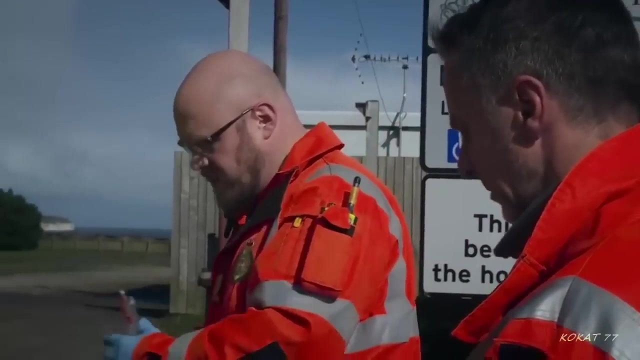 The whole team will assist in the procedure called an RSI or rapid sequence induction. John, are you going to be the assistant for this? OK, Yeah, so we'll actually go to the. We'll get the nasal O2 on it for Kat. 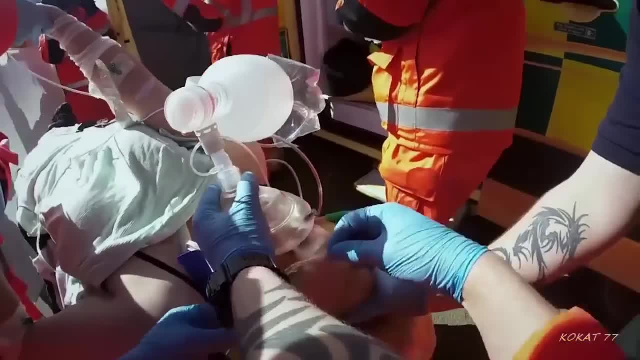 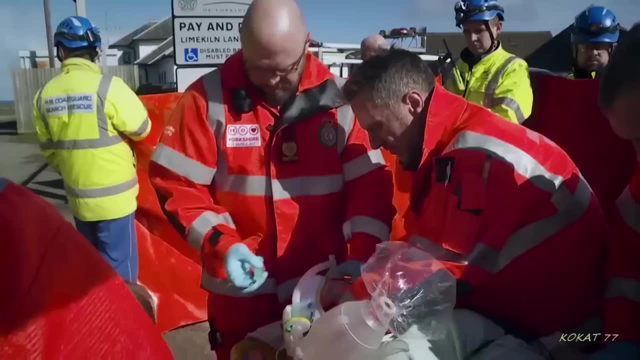 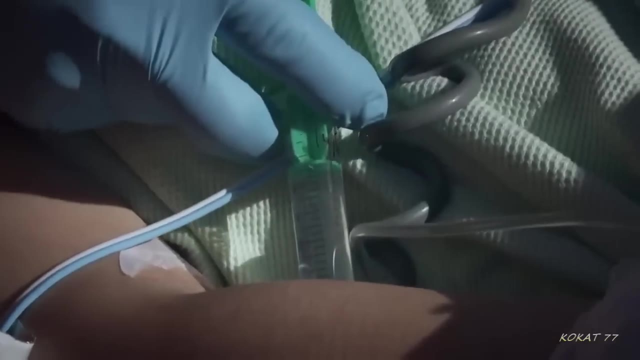 Linda. OK, Nice and relaxed Linda, Well done. I'll give the drugs Bag her gently during that time. OK, is everybody ready? All good, Everybody happy? Yeah, Linda's being paralysed with drugs, so they can take over her breathing. 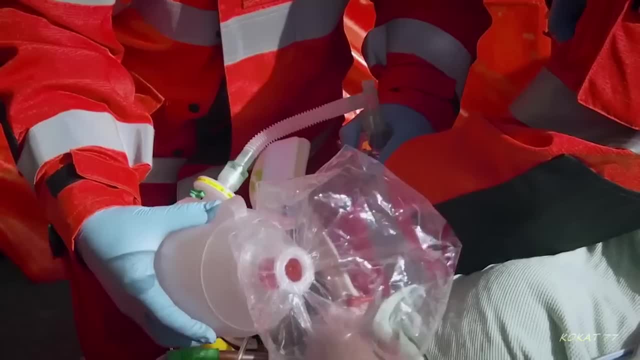 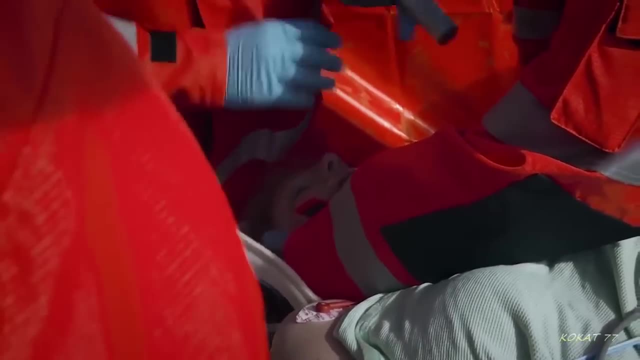 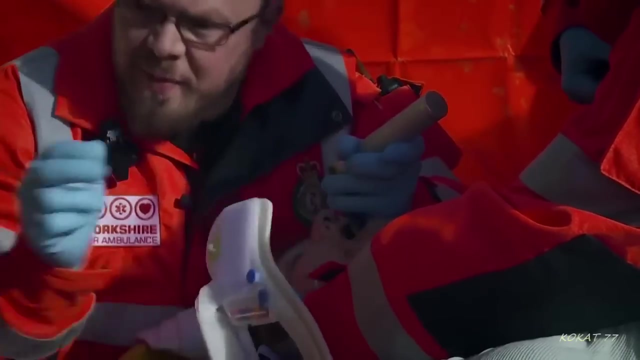 Nice, nice, Nice, One minute. Thank you very much. We've got a good view of the epiglottis Bottom end of the cord. bougie, please, thank you. A tube is being slid down her windpipe. 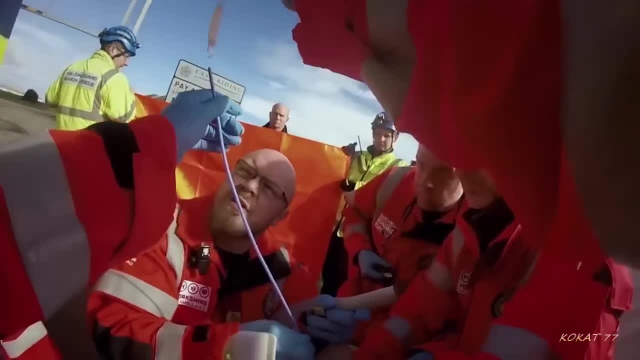 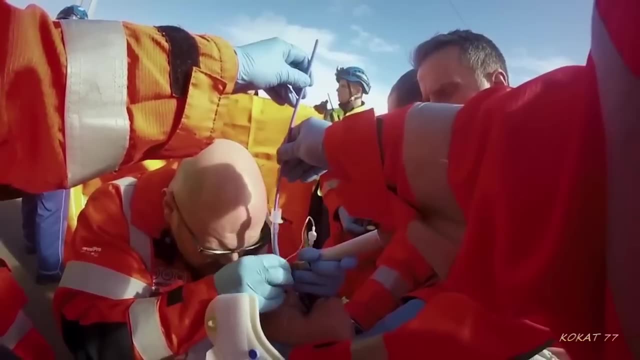 It's a difficult operation. I'm happy that's through the cords And it's being performed on a footpath. Thank you, Happy. the tube's through the cords, Bougie out please. Thank you, We've got a sling here. 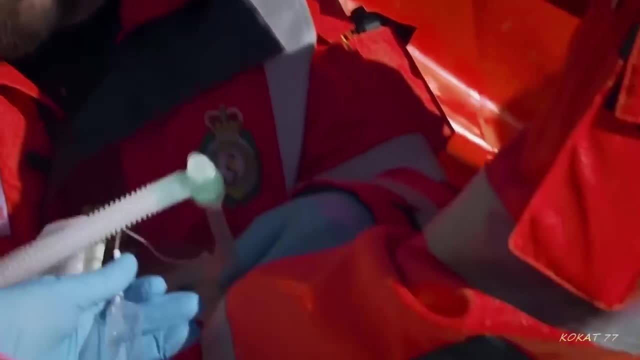 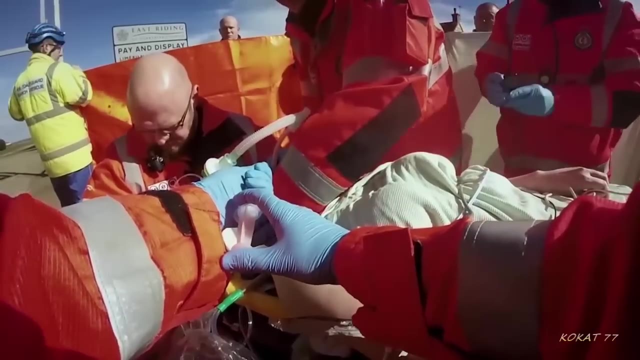 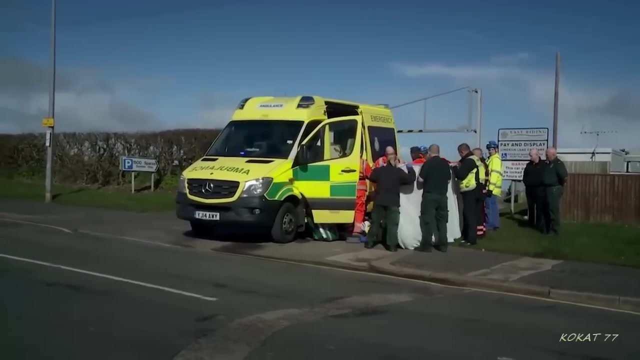 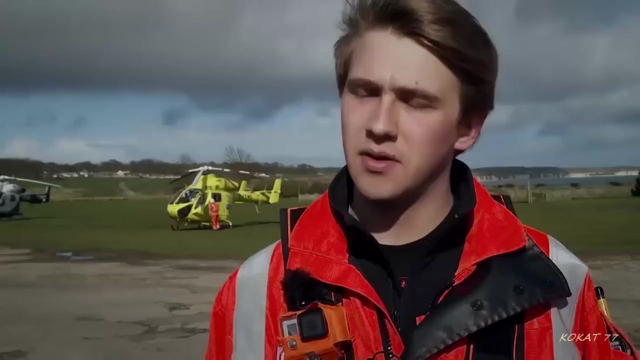 And we'll reattach it on. Thank you very much. We've got good CO2 coming back and good SATs at the minute. still, The team's successful. Linda's brain can now rest, But her condition is very serious. The race is now on to get her to hospital 30 miles away in Hull. 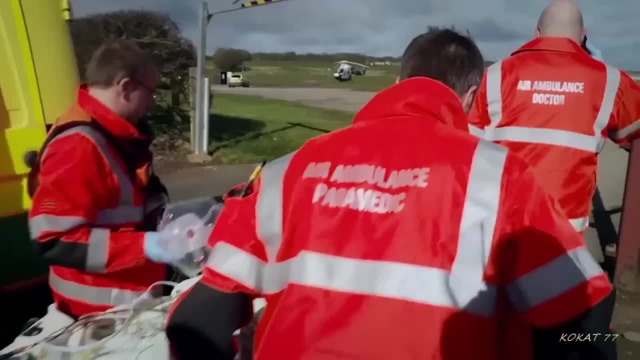 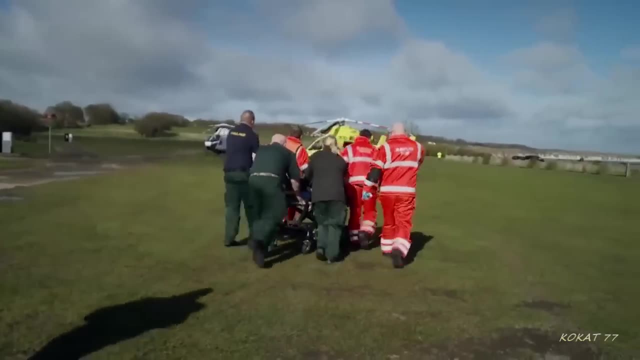 So we're not entirely certain what's happened to Linda. It's possible that she's fallen off a ladder and injured her head, which has caused bleeding which is inside her skull, which is making her very, very agitated, Ready, steady, lift. 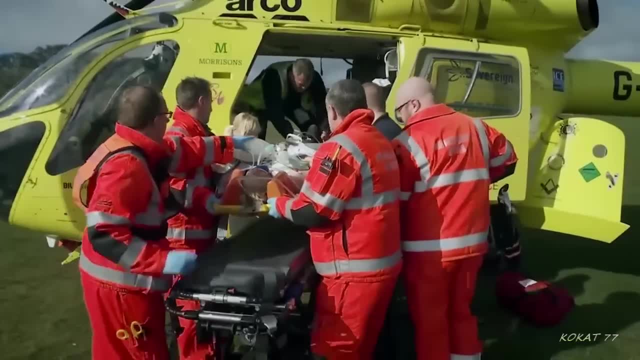 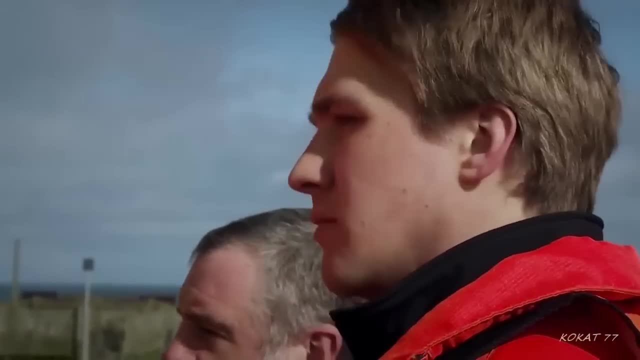 Another possibility is that she's had a stroke or bleeding on the brain as a result of a medical problem And that's caused her to collapse in the state that she is now. Just leave this down at the side, so it's there for when you're at hospital. 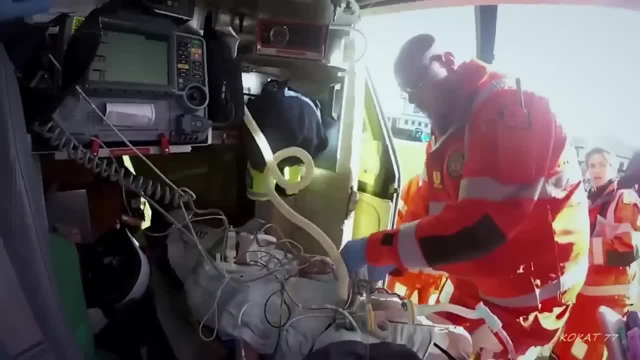 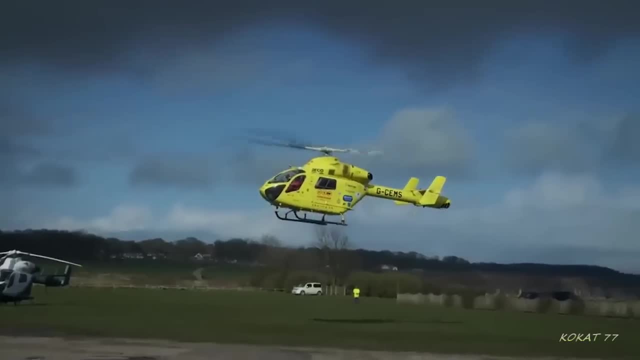 And we use it, then Shall I swap this fluid over? Kit's got another bag here. That would be really helpful. Is it this side, Kit? Yeah right, Helimed 98 will have Linda at the hospital in just over 15 minutes. 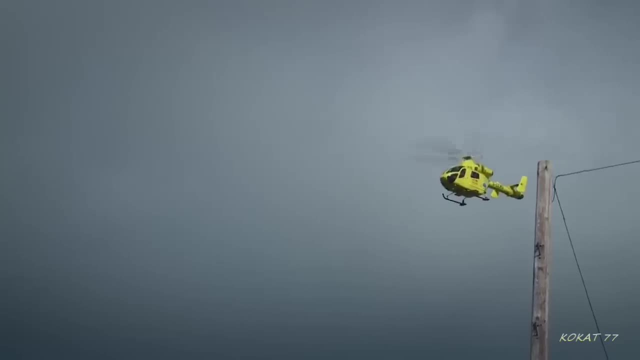 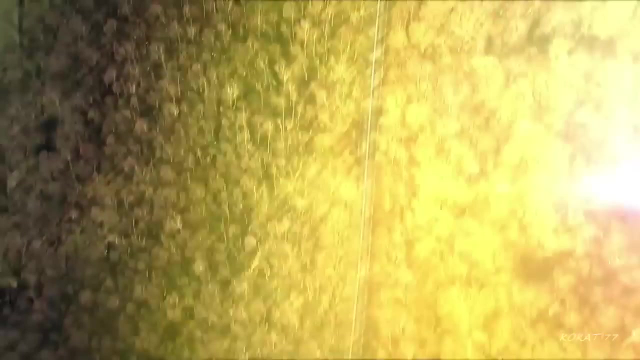 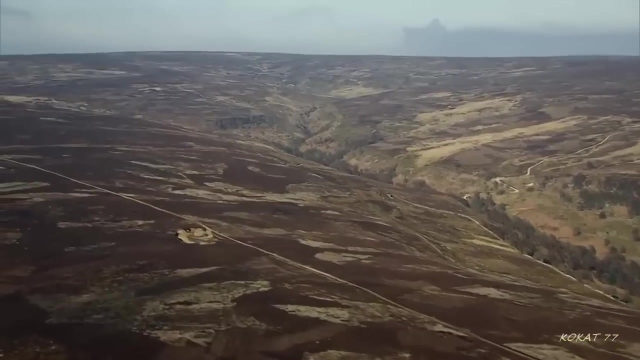 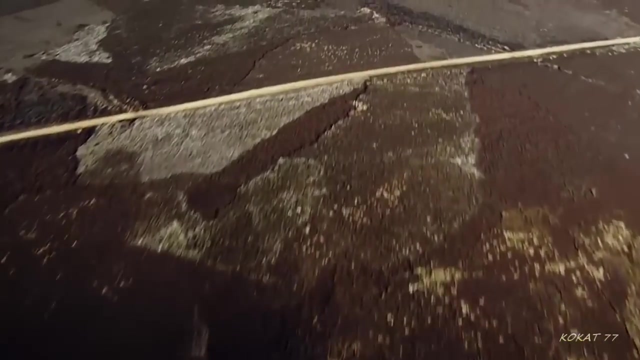 But even that might not be fast enough. It's uncertain whether she'll survive. On the remote Yorkshire moors even a routine medical emergency can become life-threatening, And a child with an asthma attack is especially urgent. In the market town of Helmsley a worried mum has dialled 999.. 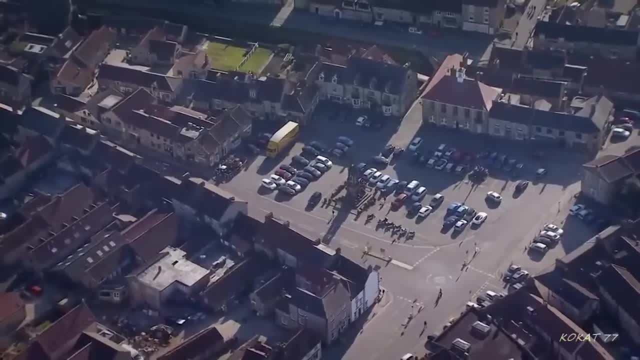 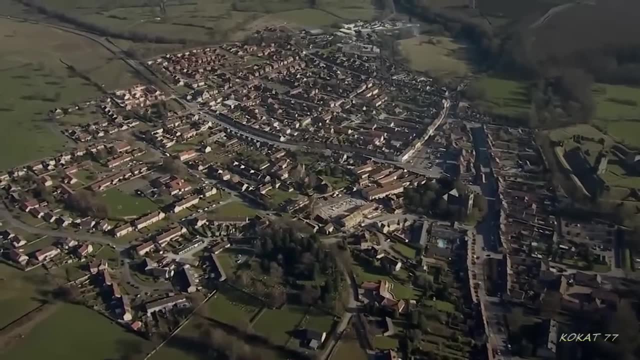 Can I take your name please, Kyle Williams? And are you Mum? I am, yes. I would advise you to try and use that email now, OK, OK. Air ambulance dispatcher Al Day is listening in. Are you sure that the help is being arranged? 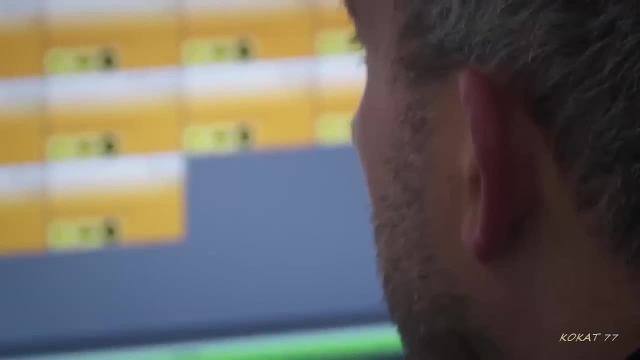 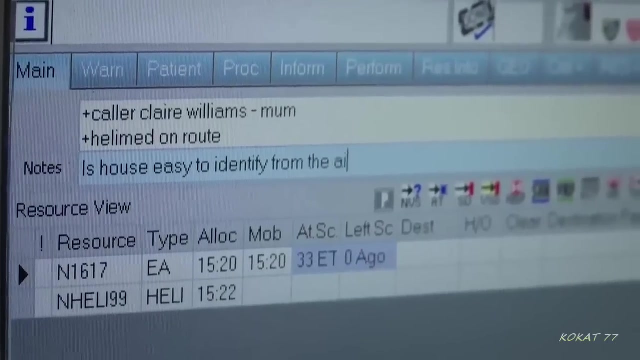 Yes, I am OK. Thank you, Help is being arranged. This young lady is really struggling to breathe, Really, Because we're so busy. the nearest ambulance is about half an hour away. It's only a five-minute flight for the Topcliffe aircraft. 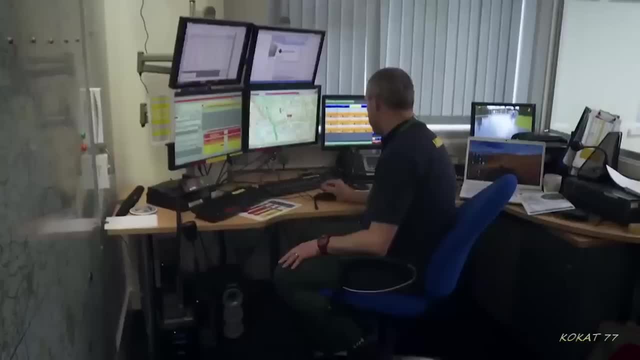 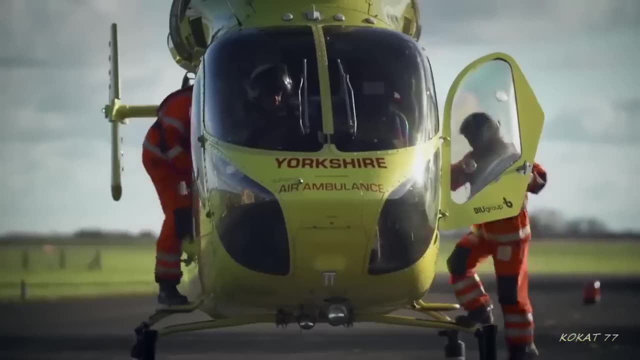 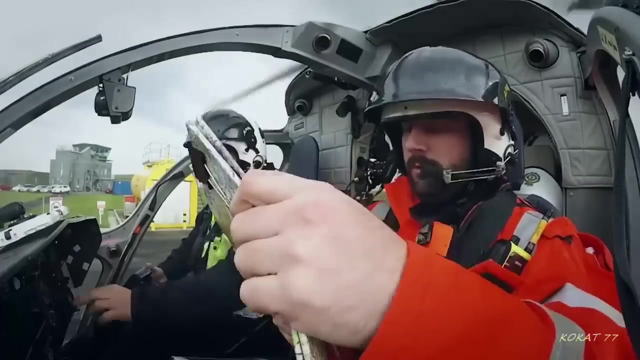 although it is in the town centre of Helmsley. 40 miles north, Helimed 99 is being scrambled from its base at RAF Topcliffe, That's 070.. OK, I think we'll find Helmsley, all right. 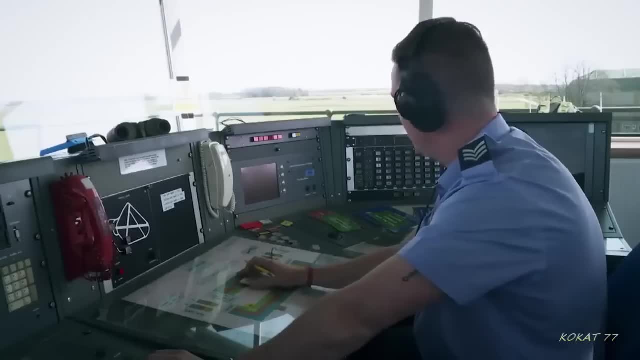 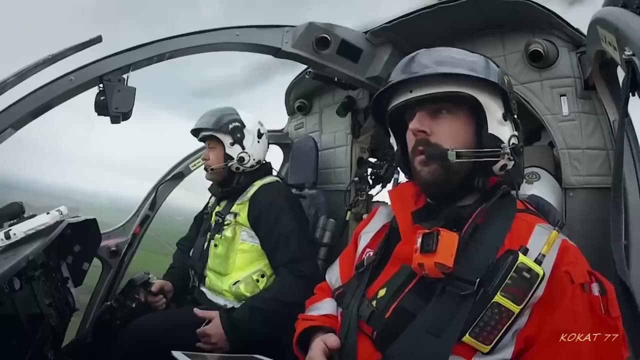 Yeah, OK, Helimed 99, take off for discretion. Present position surface 20-0-0-1-1.. Cross over to us. Stay on the left, Good right, All right. Paramedics James Stopley and Andy Armitage. 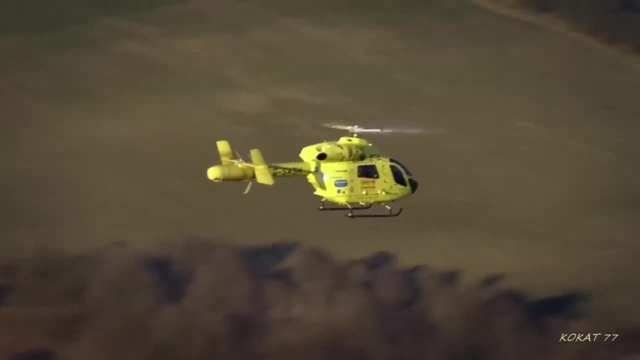 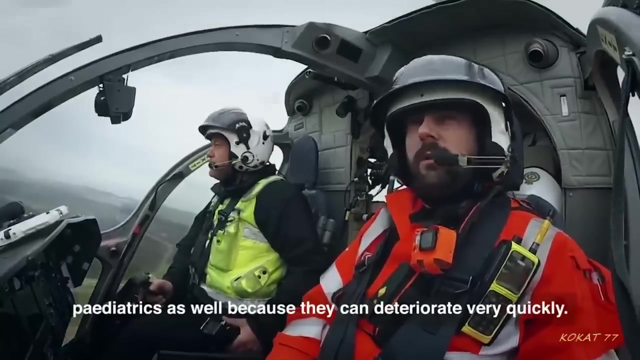 know that in asthma attacks seconds count. I mean, an asthma attack can be serious in any age. It can be life threatening. Time is of the essence really, particularly with paediatrics as well, because they can deteriorate very quickly. 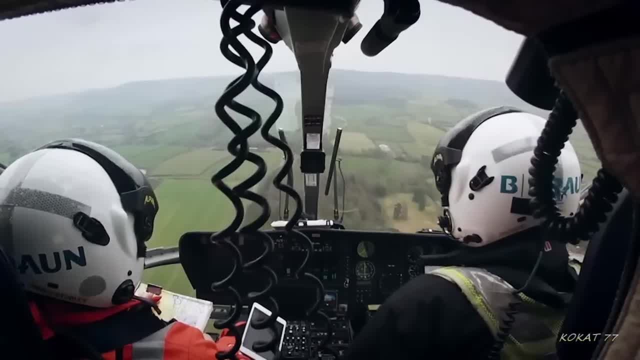 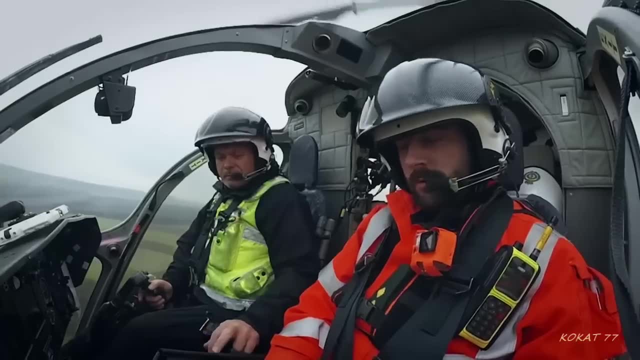 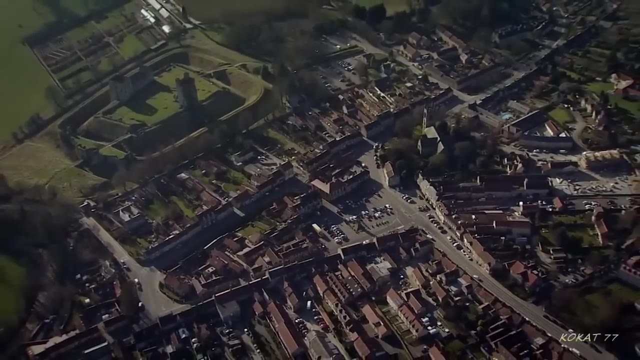 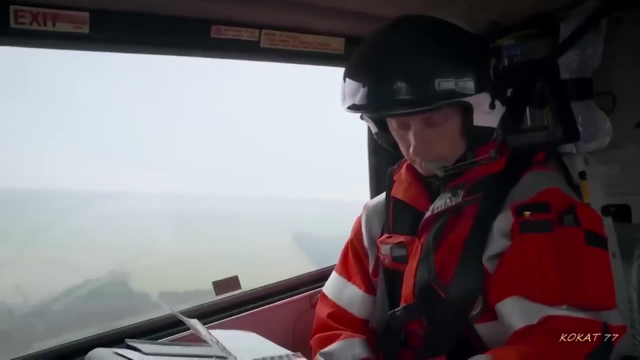 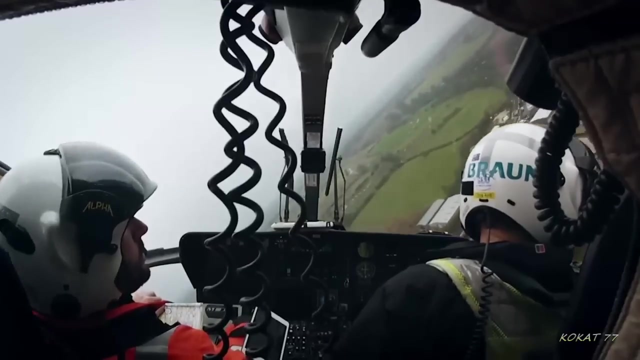 The right drugs could save the little girl's life, but in children, doses are critical. 2.5 minutes are beautiful. Helmsley streets are tightly packed, but the team know a landing place. just five minutes after the call-out, help is circling the rooftops. 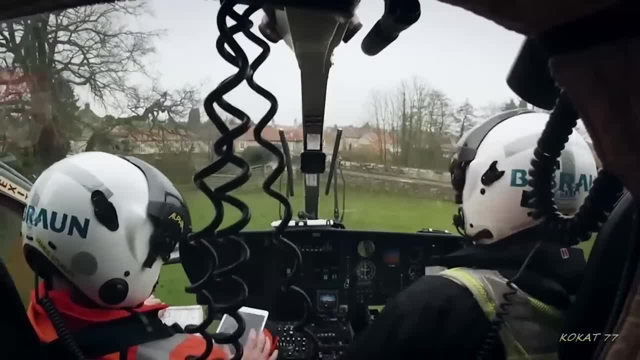 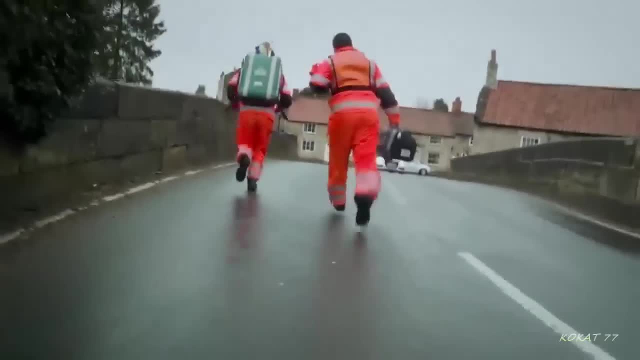 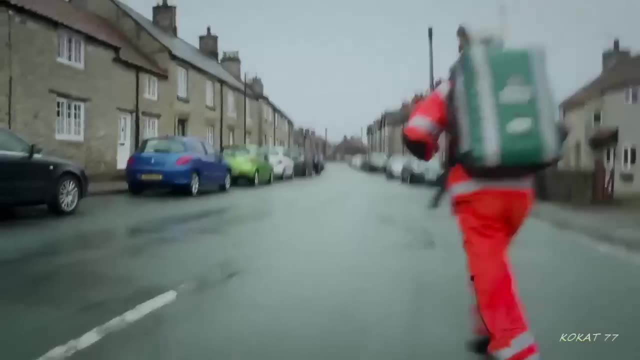 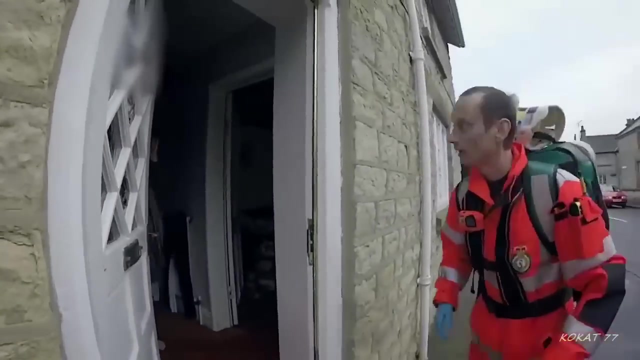 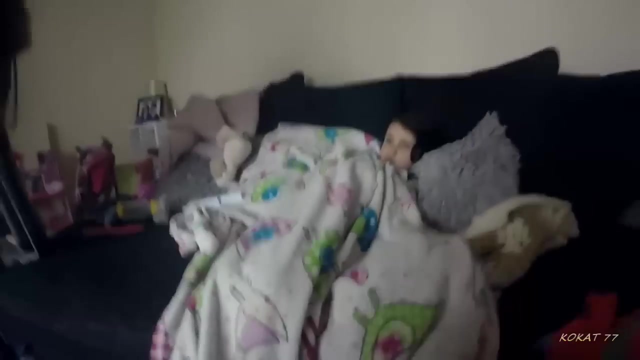 there's no time to waste. the team undergo annual fitness tests for a reason. what are you, mom? Claire Williams is still on the line to the 999 operator. all right, thank you very much. thank you, it's a long, fiery three and Ruby is fighting for breath. yeah, I got a message from the childminder. yeah, 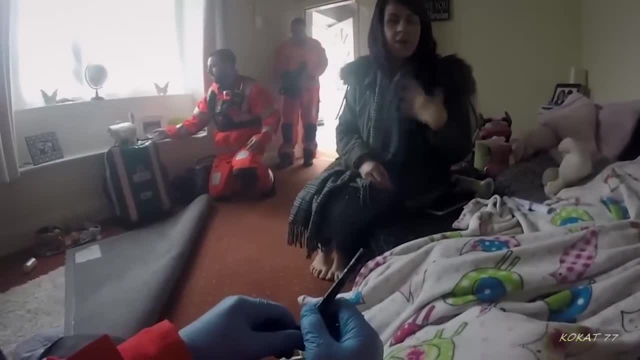 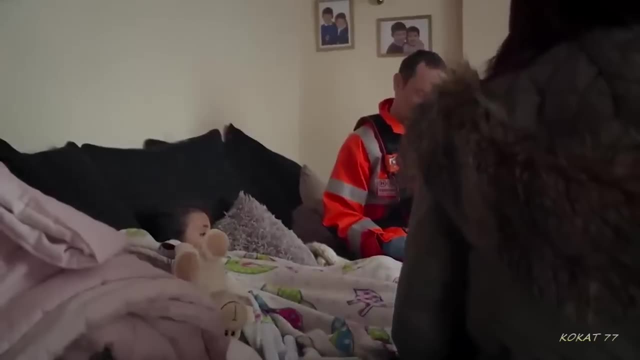 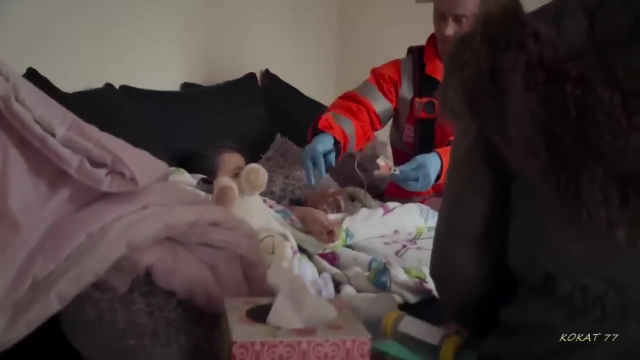 saying that she'd gone really downhill. so I went to pick her off and I noticed a breed. that's much I can breathe. it's been a bit difficult with breathing it. yeah, the family is used to coping with her asthma, but it's still worrying. you know it's coming, don't you? and I put that on your finger. do be there, you go. 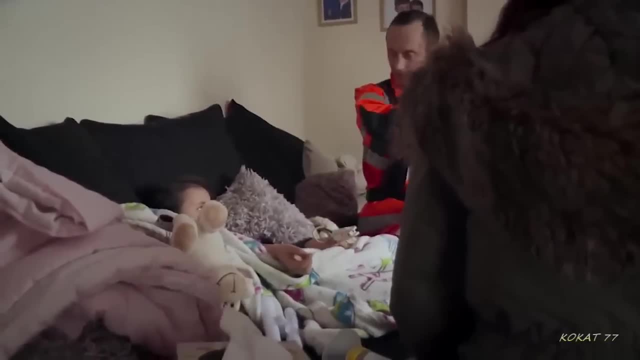 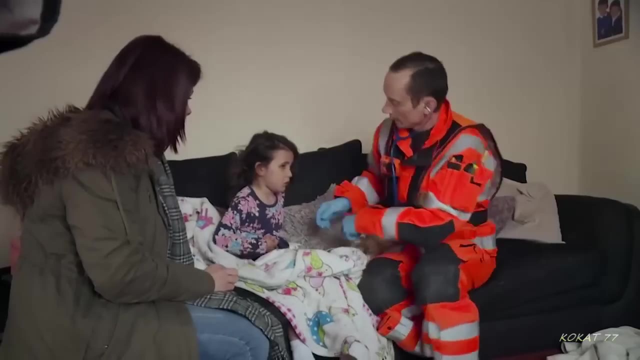 see if we can get a good reading on that and I'll have a little listen to your check. okay, so normally she's on an inhaler. she's taking them numerous times, not work. okay, can I lift that t-shirt up? is that okay? asthma kills three people a day. 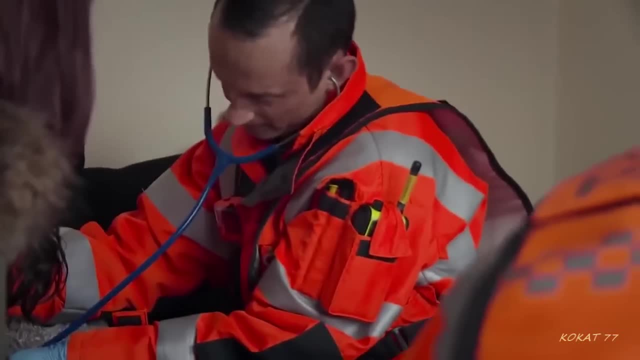 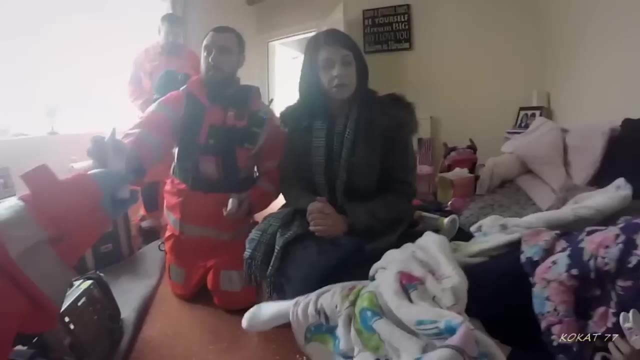 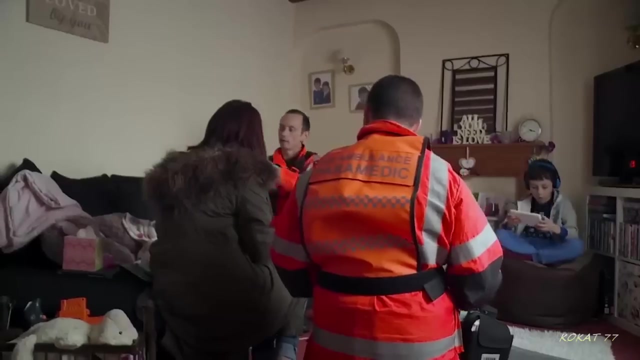 in the UK sounds all right. no, no, wheeze, breathing's up a little bit, so normal for it for Ruby's ages, say 20 to 25, and it's a 36, so that's up a bit. three temperature just goes in your ear: 38.2. I thought you felt like you were going to die. 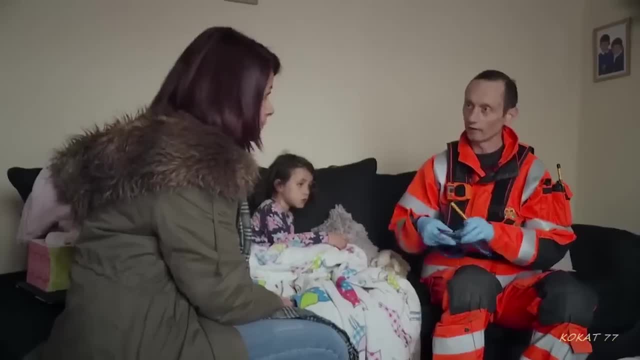 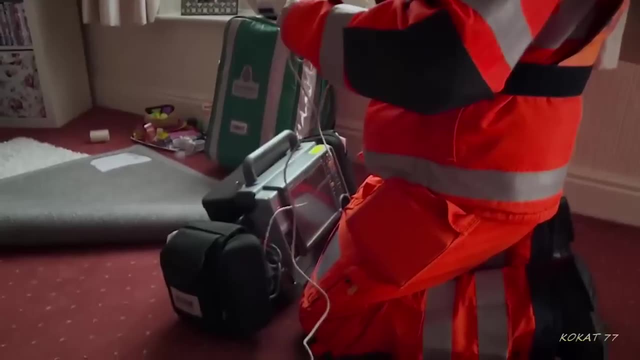 a little bit warm. yeah, breathing is up, so she's gonna need a check over in shit. to be honest with you. I mean, normally a pulse rate would be around about maximum of 120- 148. at the moment some are going to miss inter and he suspects an. 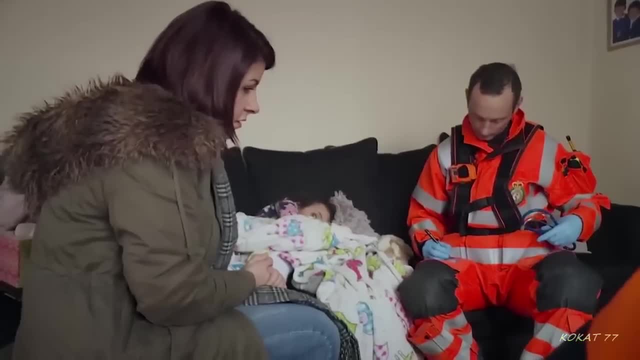 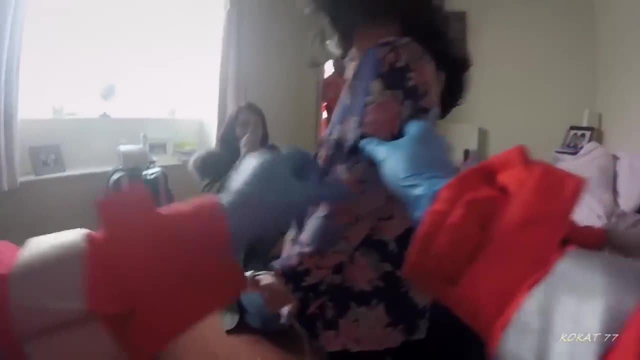 infection could be at the bottom of this and he wants to rule out meningitis. you've not noticed any rashes on the body. will just stand you up if you just have a look at a body, mum. I look at back and numbers are a little bit raised. I'm 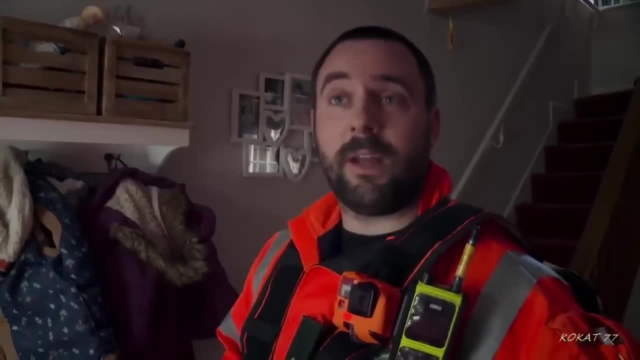 but not too concerned at the moment. She's obviously alert, she's orientated and interacting with us normally, So it's just a matter of she's got a temperature. so there may well be an infection somewhere. So we just need to try and sort out where that's going to be. 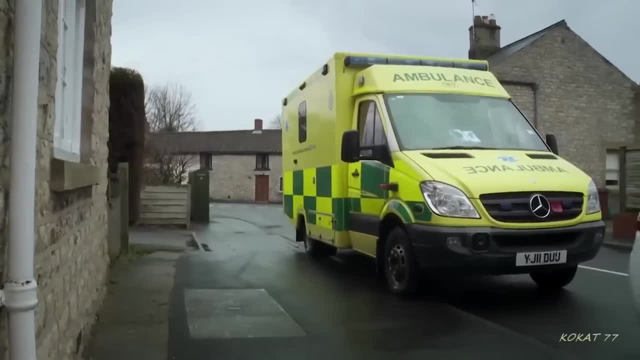 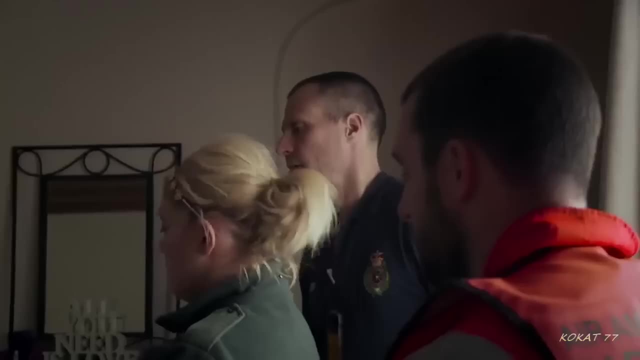 Crown paramedics have arrived after a long blue light run over the moors. There's no rashes, so increased pulse, increased rest and warm. Ruby's breathing has improved so it's decided she doesn't need to go to hospital. So I think, with it all in mind, probably just a check-up really. 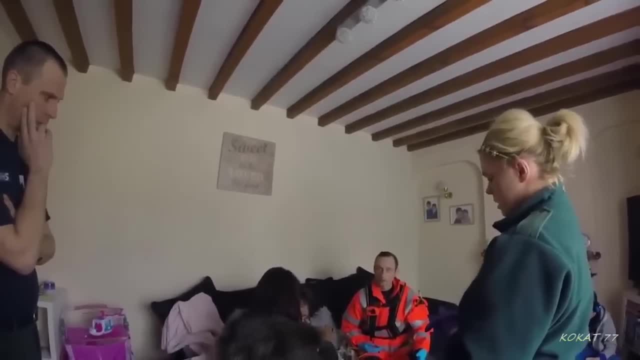 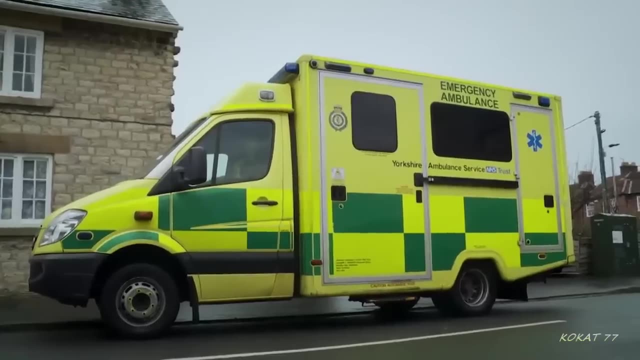 That's probably going to be the option, isn't it? With her being so young as well? Claire's GP practice advised her to ring 999.. Now Andy's satisfied. a GP is the best person to treat her and he's making sure she gets an appointment. 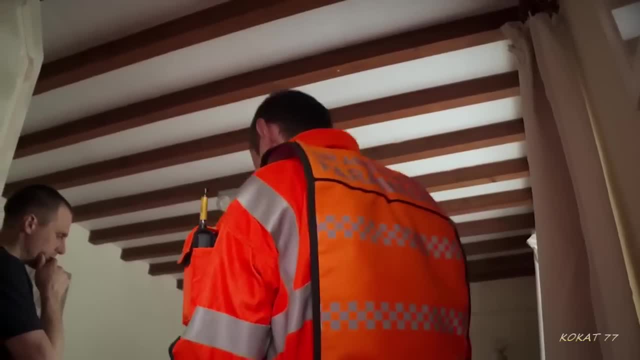 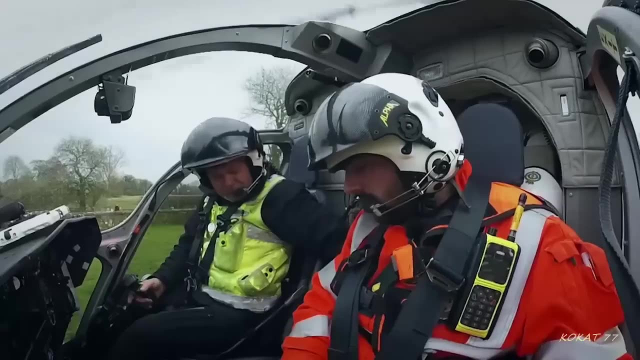 All right, Doctor. thank you, Bye, Here you go, Mum. I'll give you your phone back About five o'clock For the helimed team. it's time to return to base Engine controls. Back to flight. Top air flight airwaves. 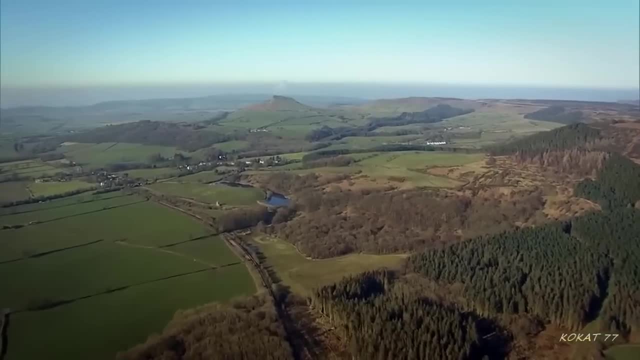 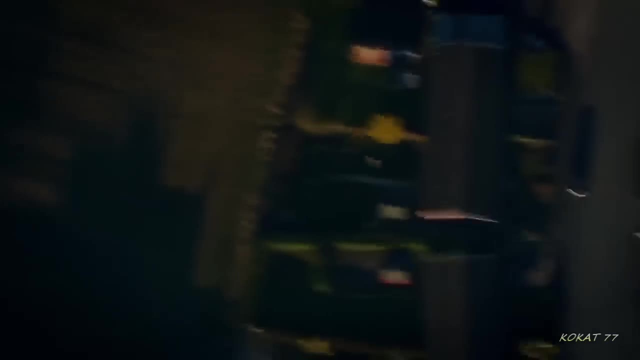 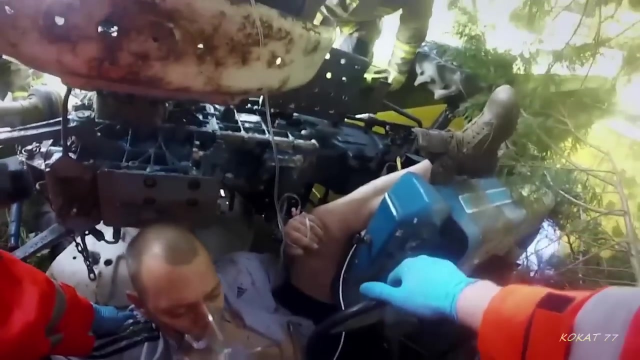 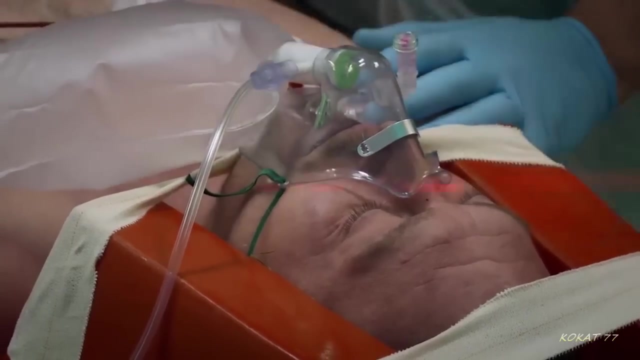 But the crew like nothing better, Better than a patient who doesn't need their medical skills. There's good news, too, for Sam, the tractor driver trapped in a lake. Against all the odds, doctors found he had no significant injuries, apart from severe bruising. 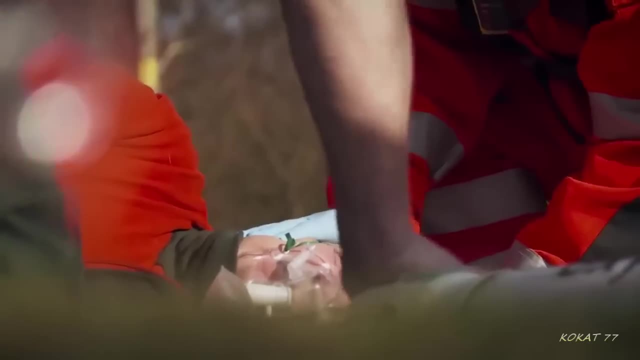 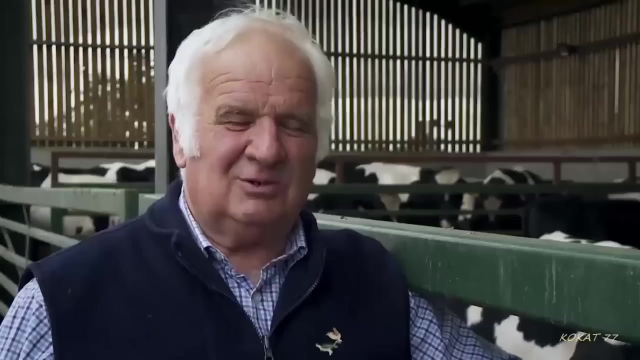 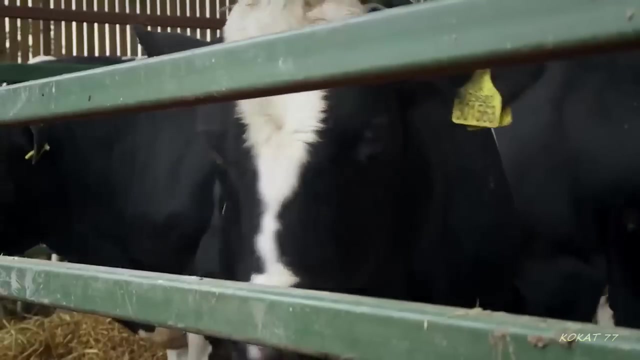 Kenny, the veteran biker who hit a deer, suffered a major fracture and was unable to walk for several months. Farmer Tom was off work for more than a week. Two and a half broken ribs and maybe some fluid on my lungs. The ringleader of the attack is no longer in the herd. 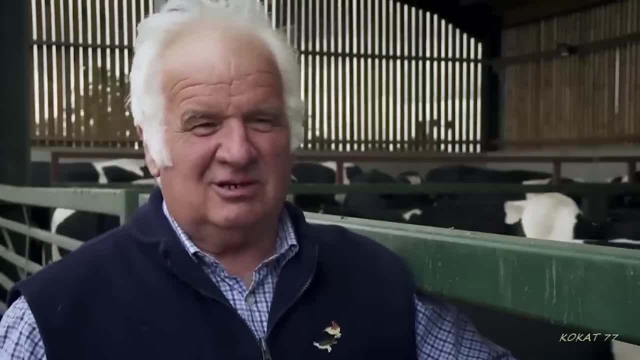 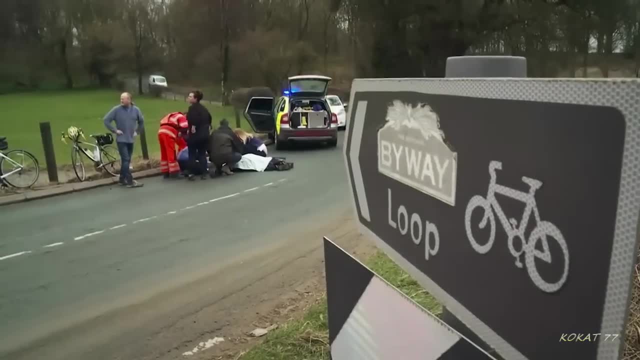 They've looked after livestock for 60 years and they can just turn and get you. Bull went to Selby Market and they made top price of that day of what we sent. Karen the cyclist spent several days on life support at Leeds General Infirmary. 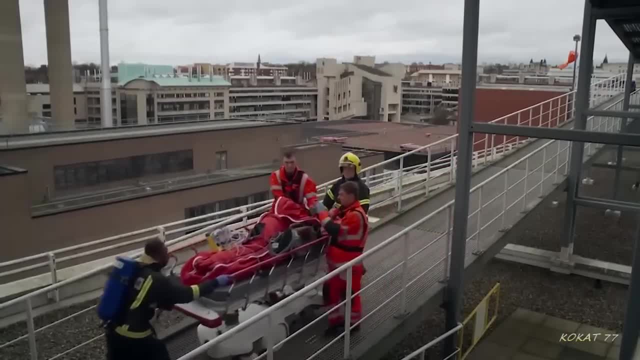 and is still slowly recovering from a fracture. She's been in the hospital for more than a year now, and she's been in the hospital for more than a year now. She's been in the hospital for more than a year now, and she's been in the hospital for more than a year now. 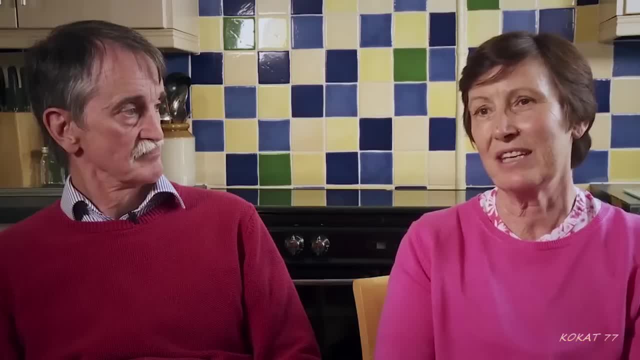 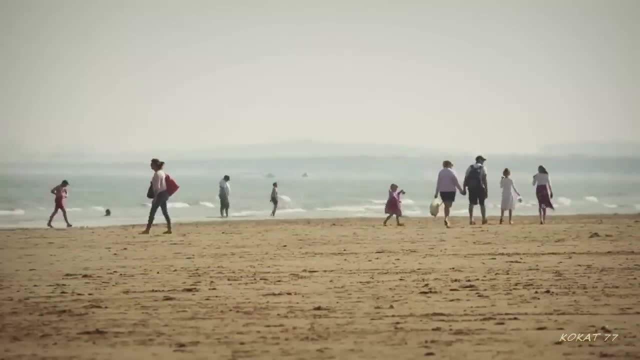 Previously, if you hurt, say, a leg, you knew that within days it would be, you'd see improvement. But with this it's been weeks, months, And Linda, the woman found unconscious in her seaside garden, had no idea. her rescue involved so many people. 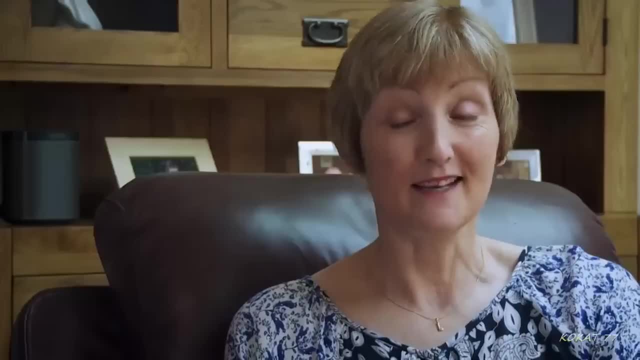 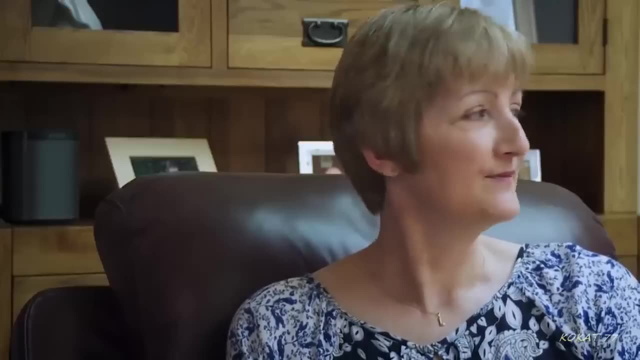 I don't remember anything for the first few weeks. It's amazing how many people come together just for one person, It's you know. Yeah, You feel slightly honoured. A bleed on her brain was found to be the cause of her collapse. 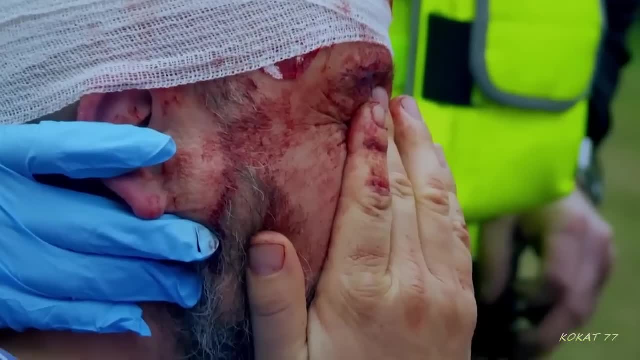 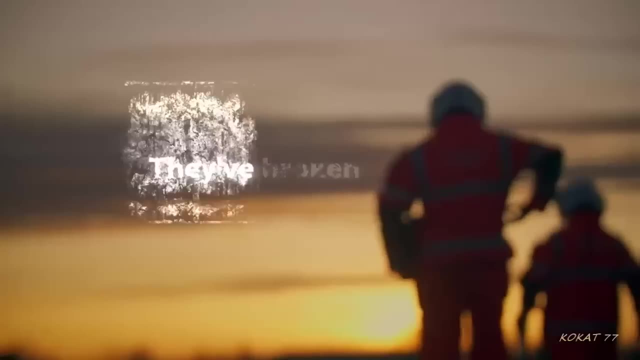 but she's no medics. Is there any serious bleeding? Yes, there is. yeah, Calm, ill legs anything below my neck. We're in a remote location. in the middle of a woodland. There's broken a bike. 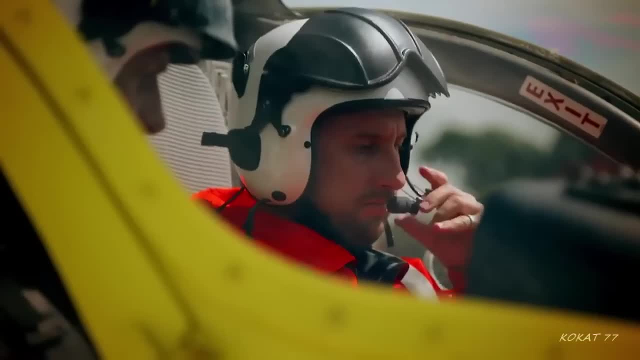 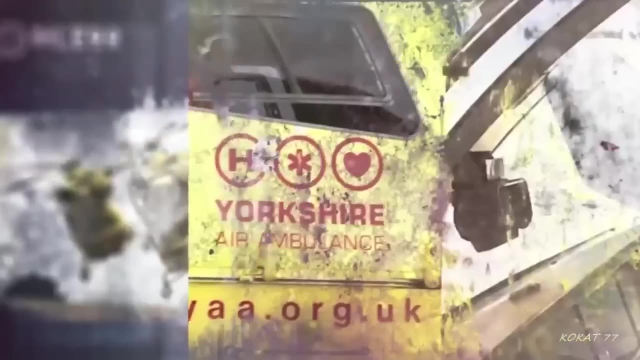 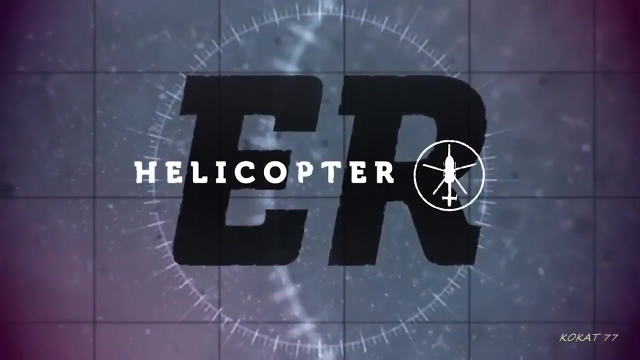 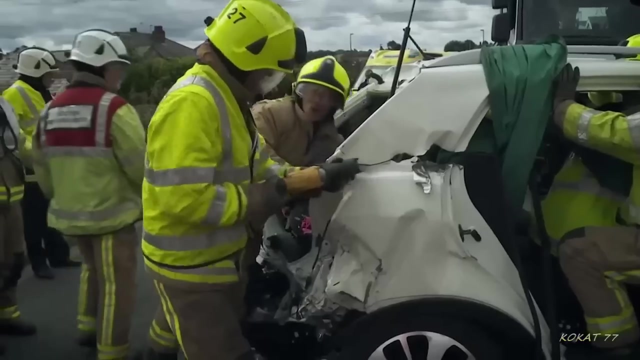 The speed of the Yorkshire Air Ambulance can make the difference between life and death. Your discretion to take off. There's no name listed. MUSIC PLAYS Today. there's a high-speed crash. The driver is trapped, but one victim is missing. 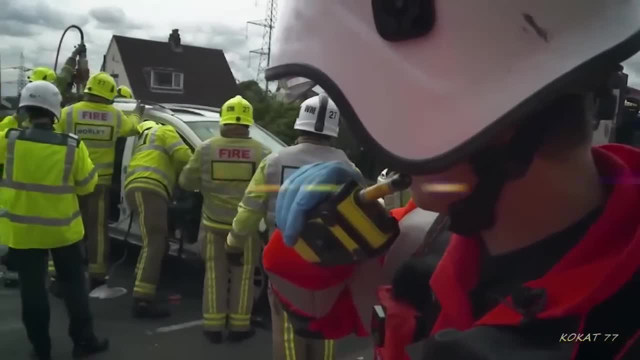 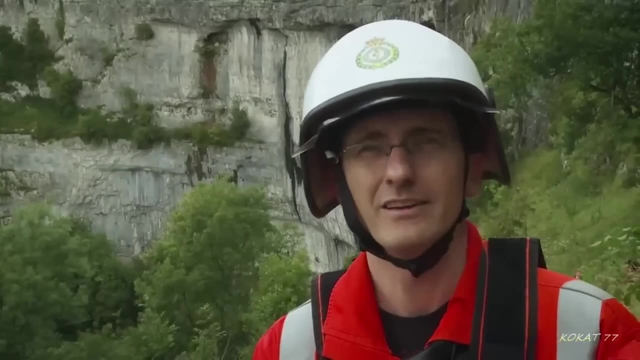 We believe there may have been a child in the rear car seat. A climber falls off Yorkshire's biggest landmark. He's become unconscious. He's had some jolt on the back of his head. The team call in the coast guard for a dramatic report. 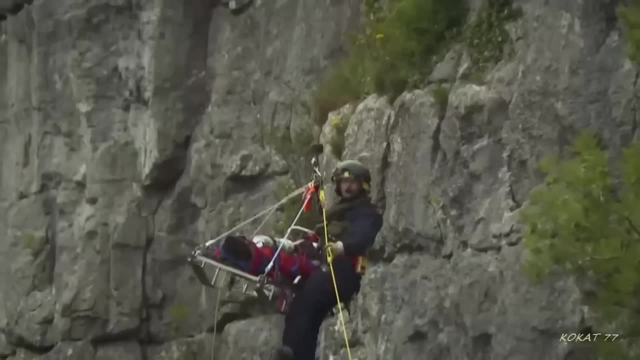 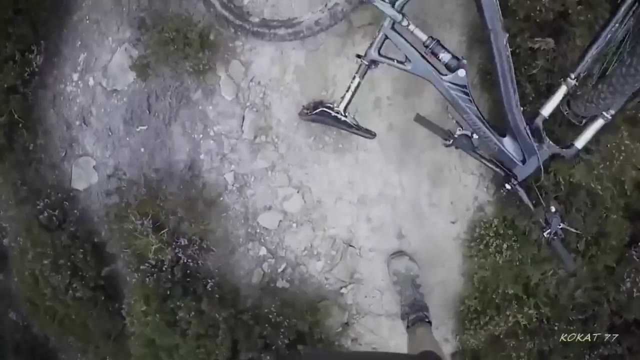 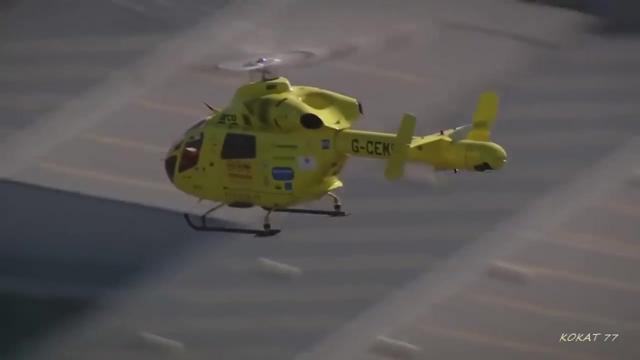 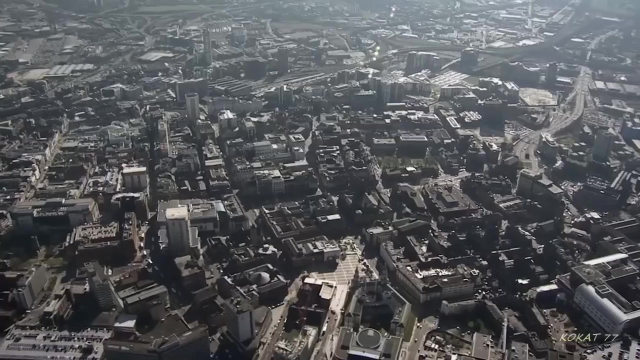 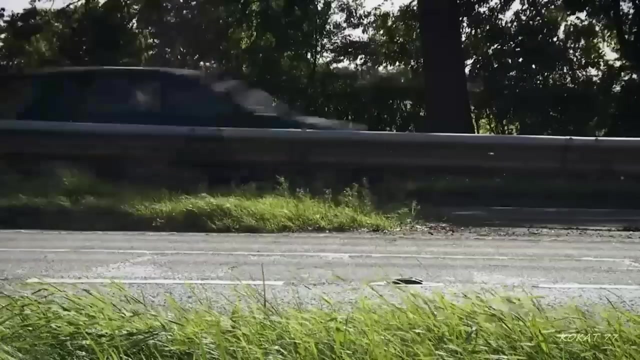 rescue and a cyclist takes a tumble in the middle of a mall with painful results. it's mid-morning in Leeds and a lorry driver's dashcam is about to capture a devastating accident. it's a 40 mile an hour limit. the hatchback is 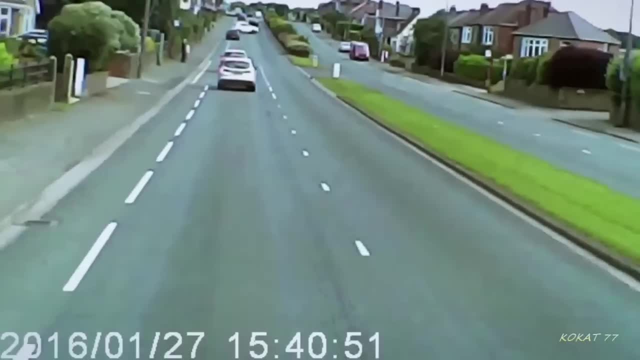 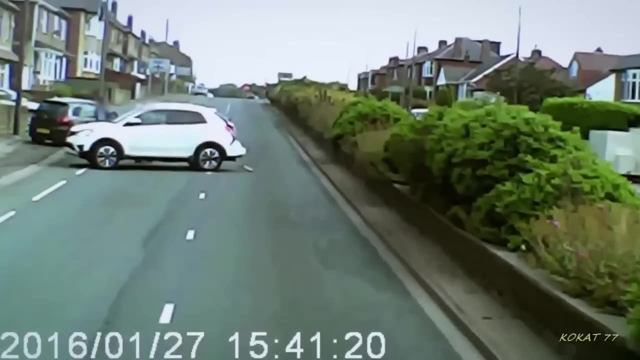 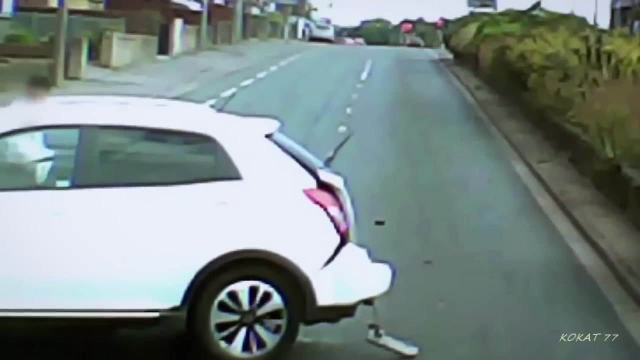 doing 80. as the white 4x4 reverses into a drive, the black car smashes into it. inside the 4x4, the female driver is trapped. the occupants of the high-powered hatchback, capable of a hundred and fifty miles per hour, appear. 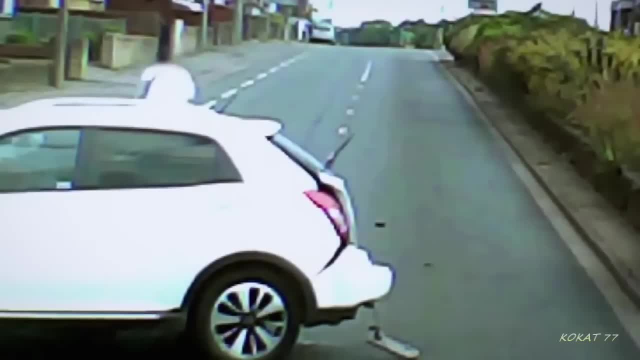 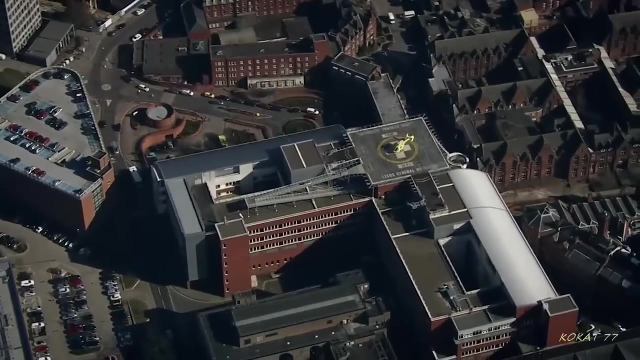 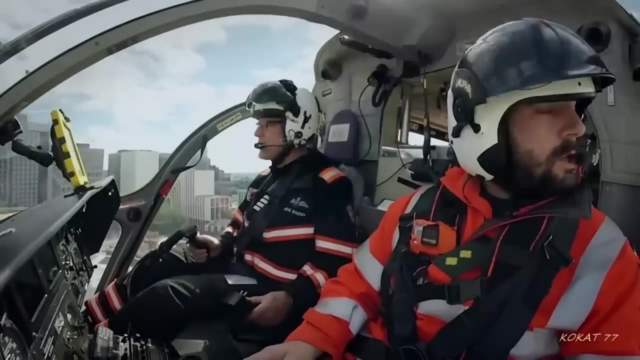 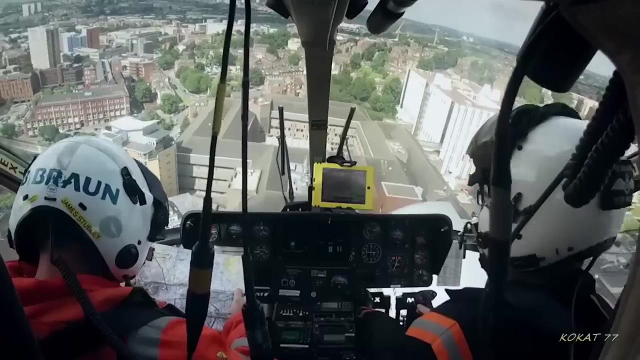 to stop to help, but then they simply walk off, leaving their victim who is seriously injured. five miles away, on the rooftop helipad of the Leeds General Infirmary, Helimed 99 is being scrambled to her rescue paramedics James Stubbley and Andy Armitage have few details of the crash. 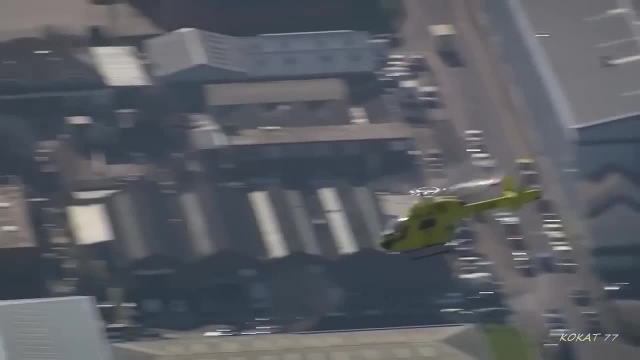 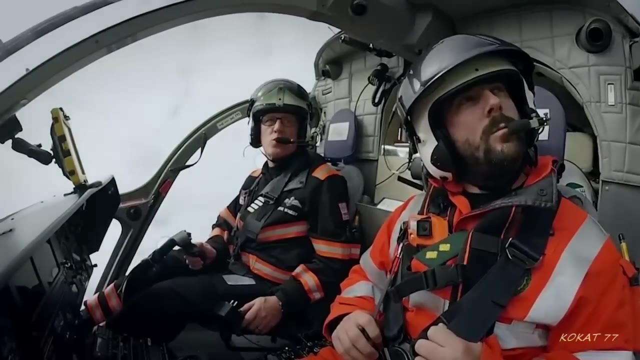 what is the crash we're attending, please? it's an RTC 2 car with a patient who's trapped on it. why is he coming round visual? we'll go just the other side of that and let him go slowly down towards the road from there. it's happened on a main route into Leeds. 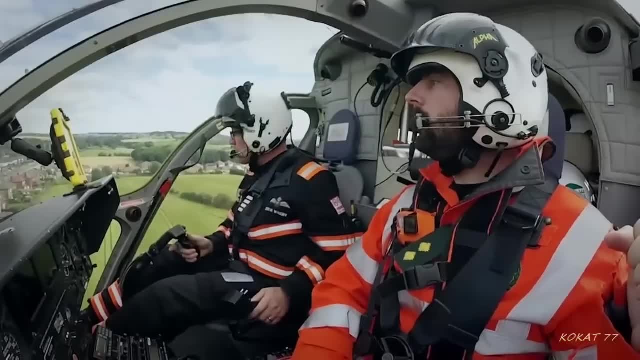 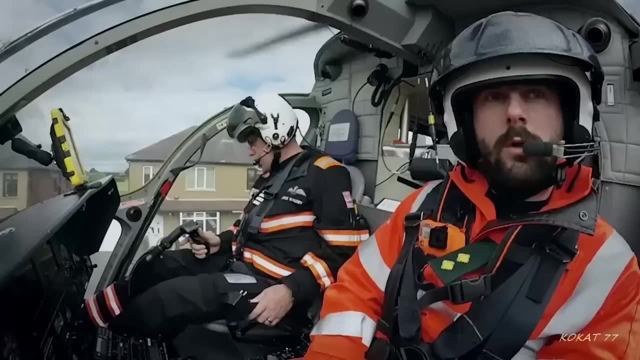 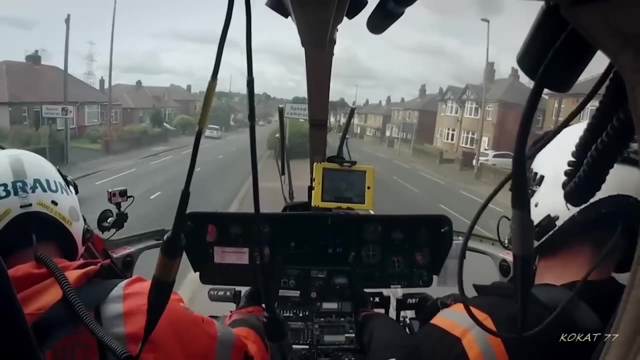 I need somebody to close that road off early. yeah, the police one coming up to clear the road. he's doing it. air ambulances have strict limits on the size of landing sites over the domestic. thank you, And this is big enough. Get out of the rear now. I'll be good there, guys. 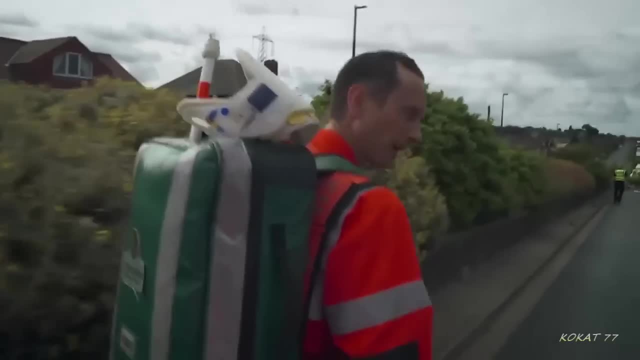 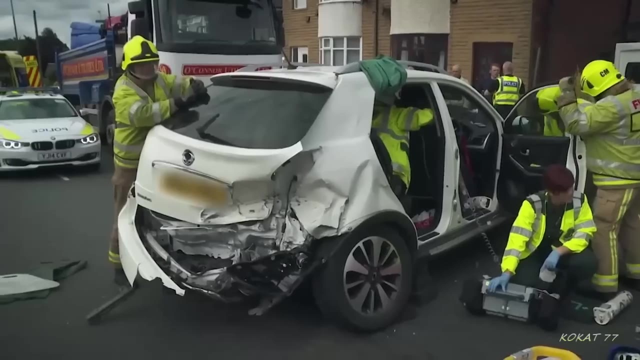 It's a road traffic collision, Dual carriageway, so a bit of speed. We've got somebody trapped, apparently, but we'll see when we get there. Tracey Scadden is 32.. The damage to the cars shows the force of the impact. 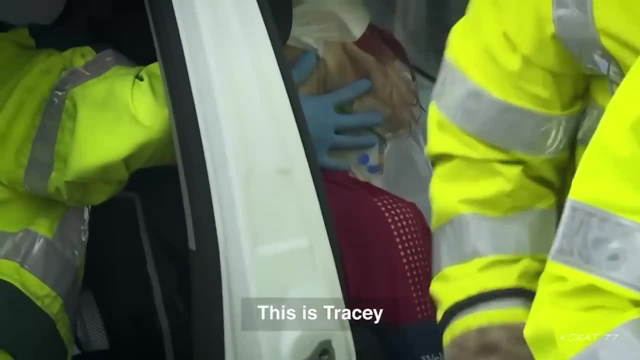 Hiya, you all right. How are we doing? All right, Tracey, Tracey, Tracey. you've got a nice lift today, don't you Tracey? Lacerations to the forehead, Lacerations to the forehead. 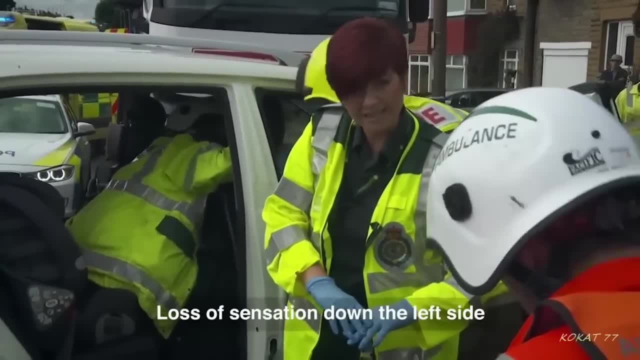 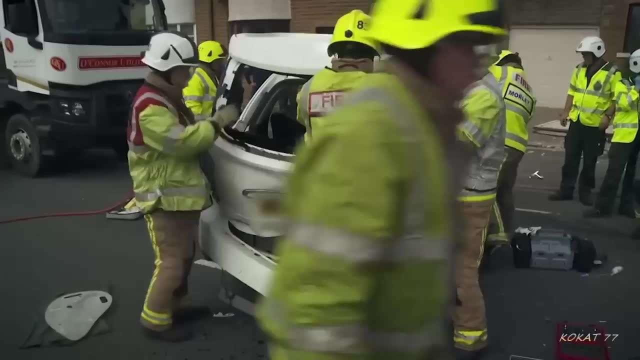 Yeah, Lots of sensation down the left side of both the arm and the leg. She feels numb. Feels numb. It's feared. Tracey has a serious spinal injury as well as the head wound. It looks like it's been quite a significant impact. 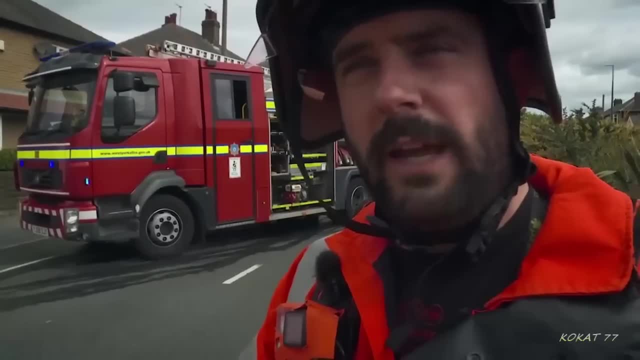 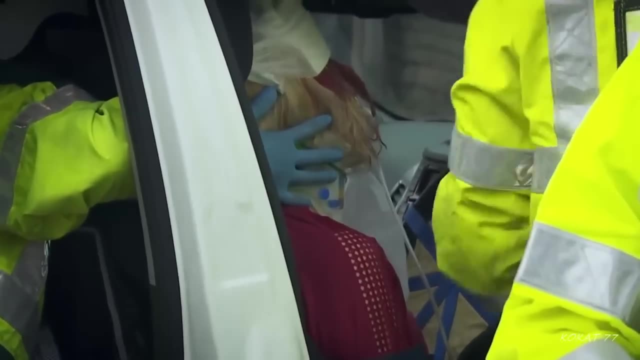 approximately 80 mile an hour is what's being said. The car's done at least a 180 from where she's been going in a driveway, so it's a significant impact. Five milligrams on the 1024.. All right, She's had some undones. 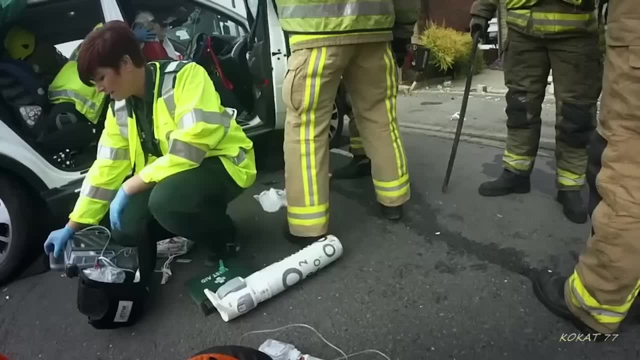 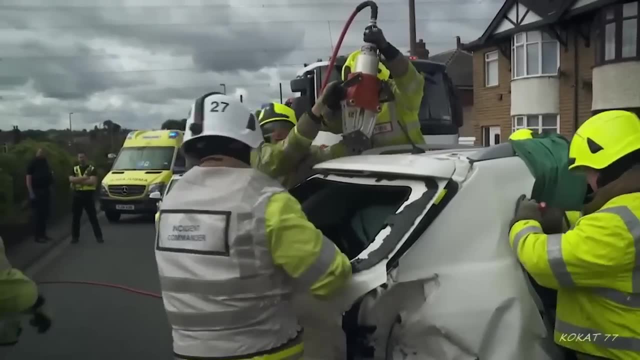 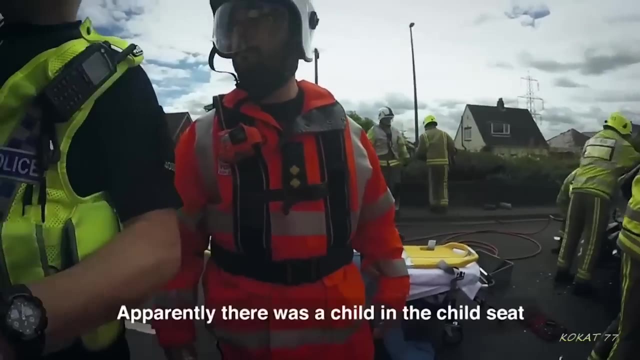 She's had some undones as well. Tachycardia 119. Blood pressure. at the moment Tracey's heart is racing, Her blood pressure soaring And she's complaining of numbness down one side of her body. And now there's more worrying news from the police. 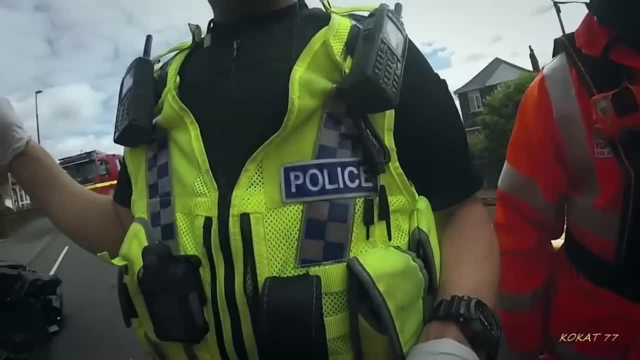 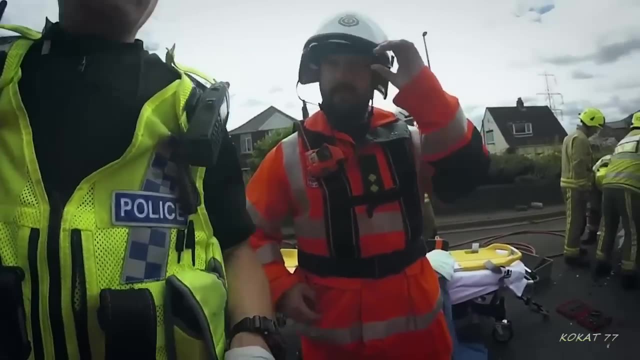 Hello, Apparently, there was a child in the back of it. All right, It's in that house. I've only just found out, so that's right. All right, There was a child apparently in the car. It's in the house. 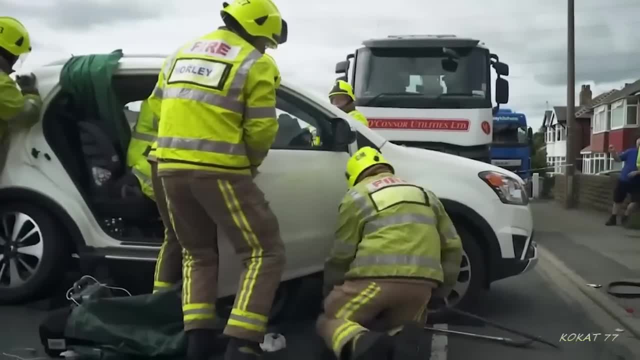 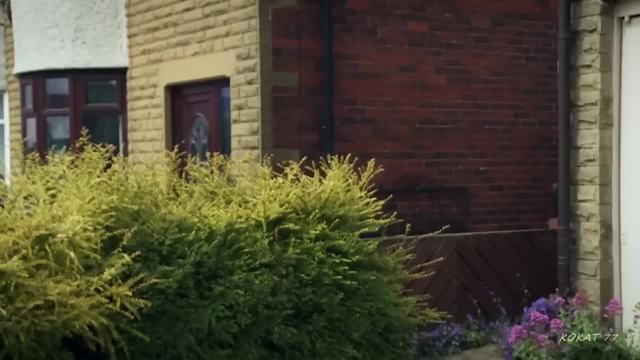 In that house. Oh well, Thank you. In the confusion no one realized Tracey's daughter had been taken in by relatives living nearby. We believe there may have been a child in the rear car seat and we'll get back to you about that one. 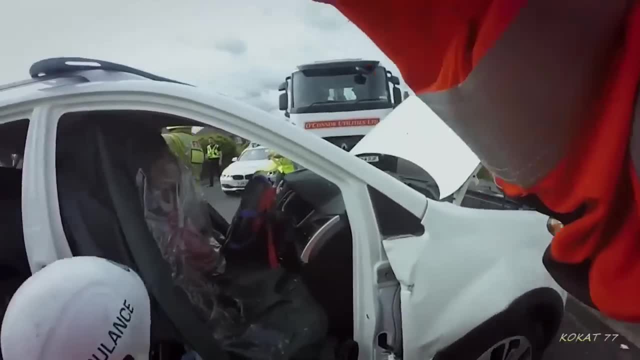 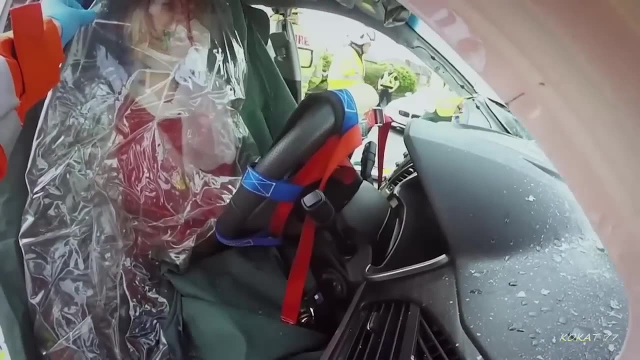 Tracey's, wrapped in a plastic shield designed to protect her as firefighters cut her free. All right, Tracey, You've had better days a bit, haven't you? The rear end shunt means Tracey's airbag didn't go off. 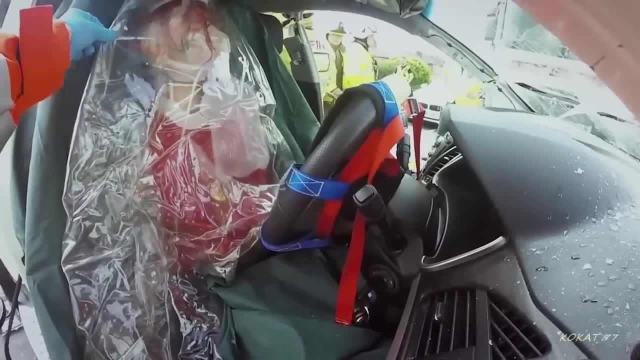 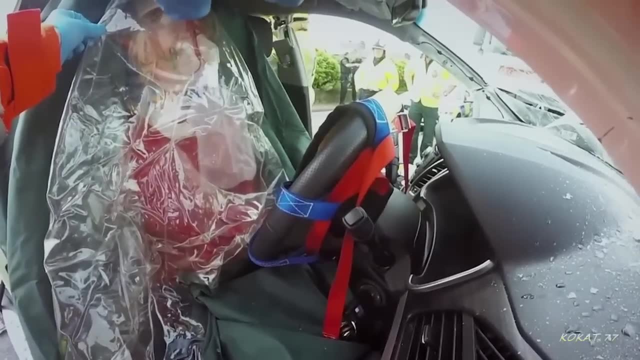 Now it's in the car. Now it's a danger to her and her rescuers. Would you like some more morphine? Yeah, We just need to be steady with you, though. Were you banging your head and that All right? 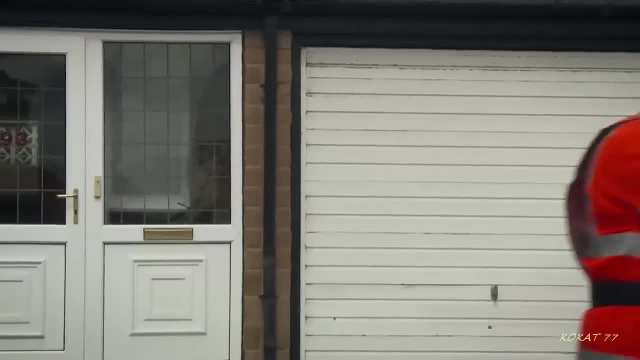 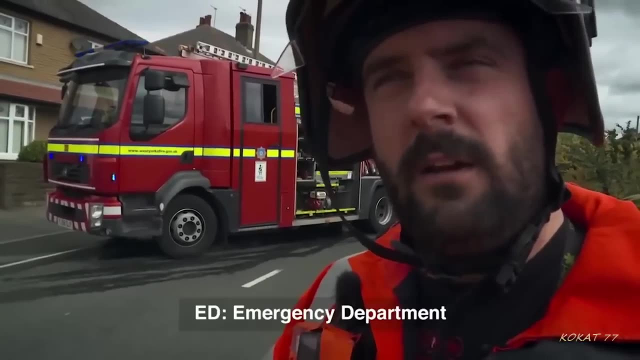 At least there's good news about the other victim of the crash. I've just been in and checked over the little girl and she appears to be fine, But obviously because of her age, what we'll do is we'll get the crew to run to the local ED and Grandma will come here and there while we 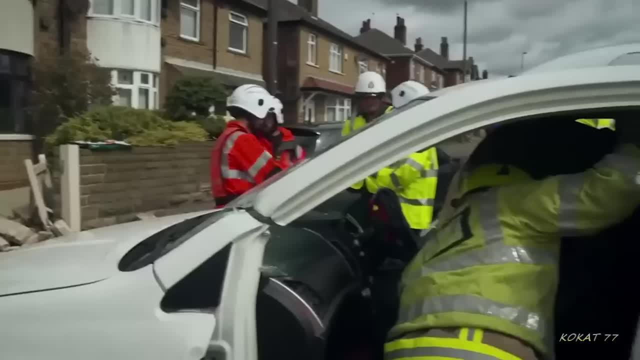 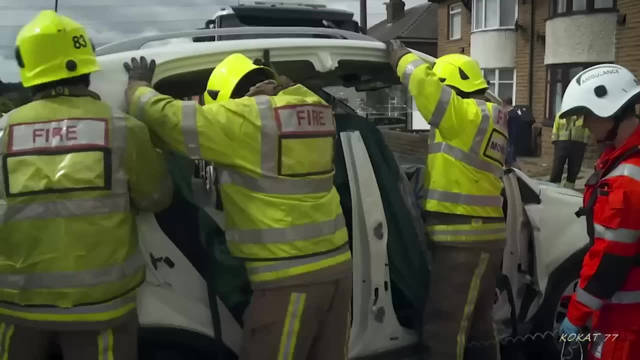 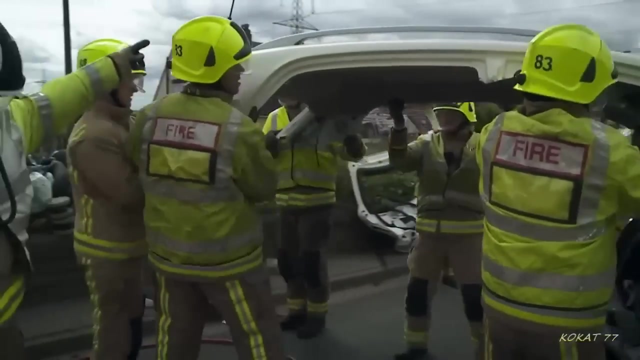 obviously can convey more. Firefighters are starting to cut her car apart. Just watch your foot mate with that. All right, we're ready for lifting. At last Tracey can be freed. How we doing. Yeah, We're going to get you out in a second. 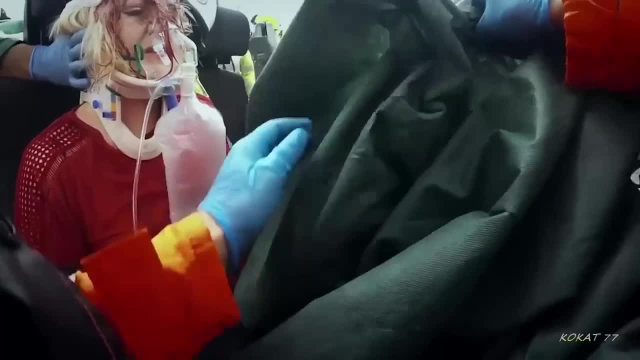 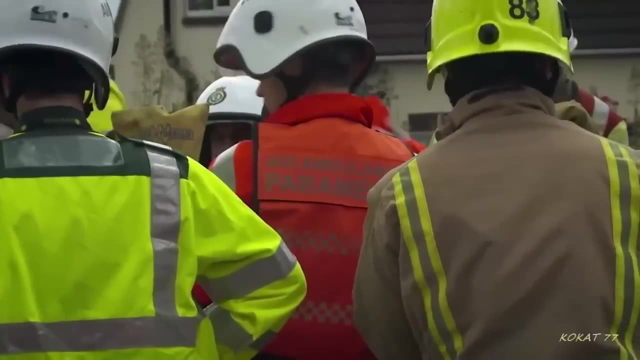 so we're just going to put a board down the back of you. All right, Are you the same as what I asked you a couple of minutes ago? Yeah, Yeah, The numbness she's complained of could be a sign of a spinal injury. 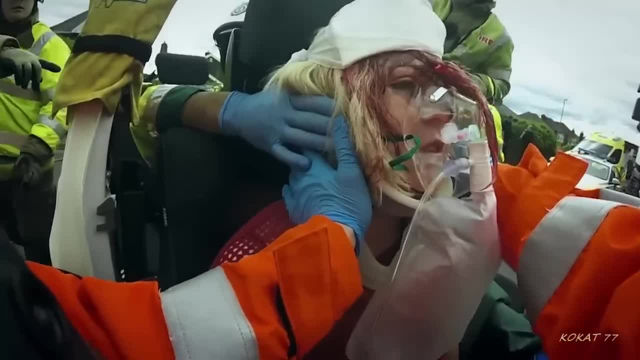 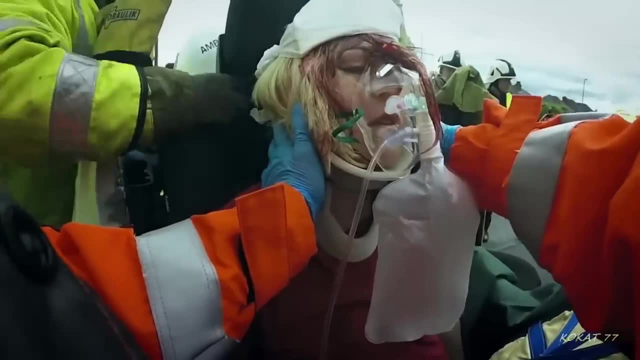 Yeah, Yeah, I've got control, mate, Have you? Yeah, OK, Right, We're just going to get you out, We're just changing over. Yeah, Get her in that headrest first. Tracey's back will be kept rigid throughout her rescue. 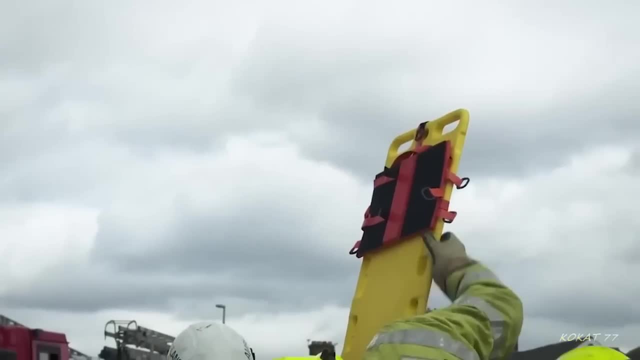 Tracey, you just feel this board going in that back of you. all right, You know you're complaining of that lost sensation. Yeah, We just need to make sure you've not done up to your back at all. OK, Nice and steady. 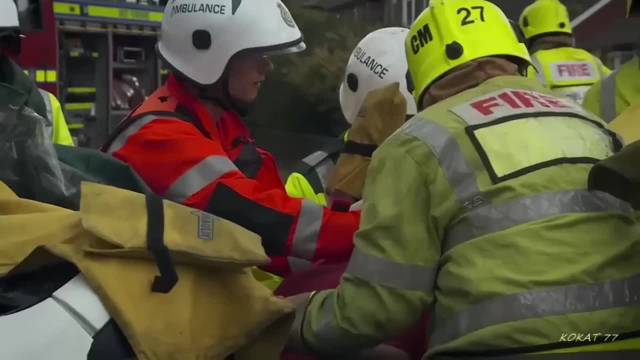 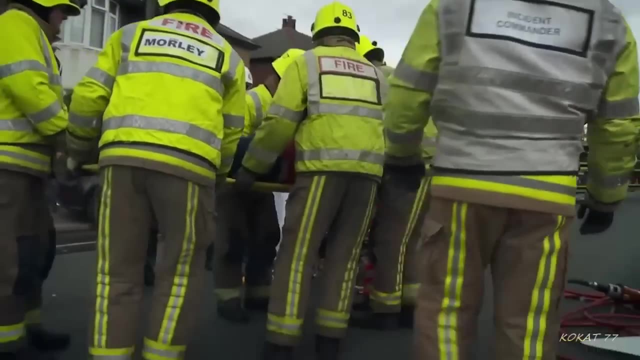 Go with it. Go with it. Let us know. if it's hurting. As far as you need to go, guys, We're going back as far as we can. The loss of sensation down her left side is just one symptom worrying the medics. 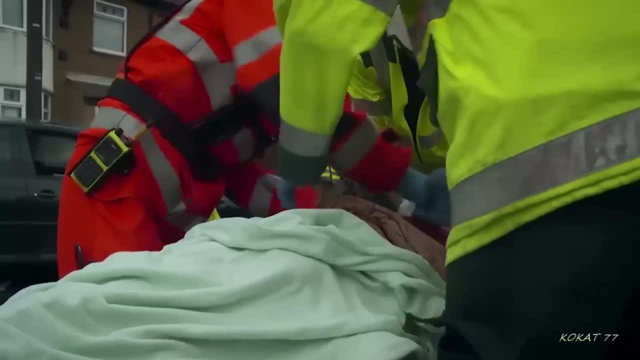 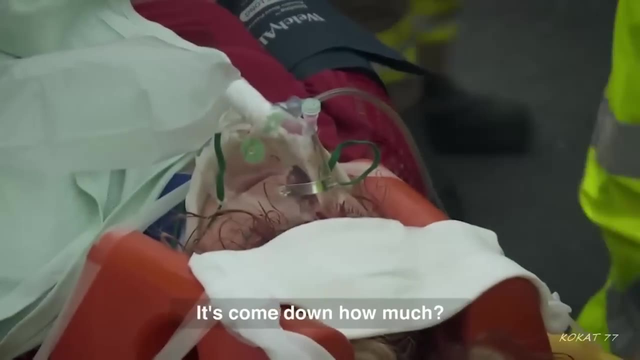 Does your breathing feel OK? Yeah, Can I have a feel of your belly? Does that feel OK? Yeah, Blood pressure's come down now. It's come down how much? 110.. Hmm, Their patient's blood pressure is dropping. 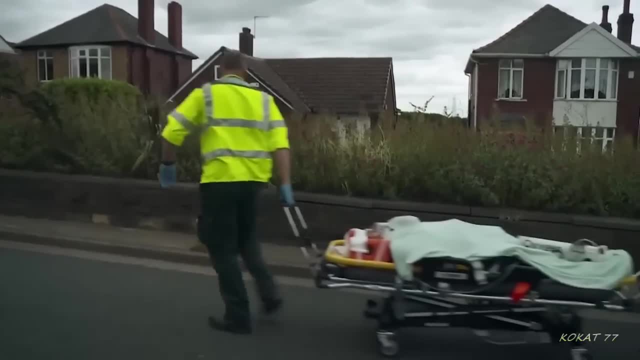 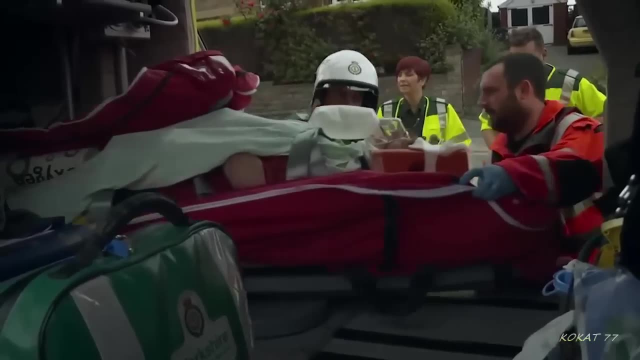 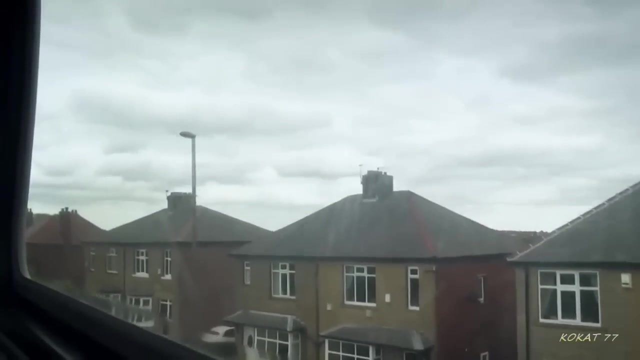 She could be bleeding internally. She's going to be flown to the LGI. It's just 20 minutes since Helimed 9-9 left its landing pad. It looks clear all round, Still clear, left, Clear to the right. They're leaving a scene of devastation on one of the main roads into Leeds. 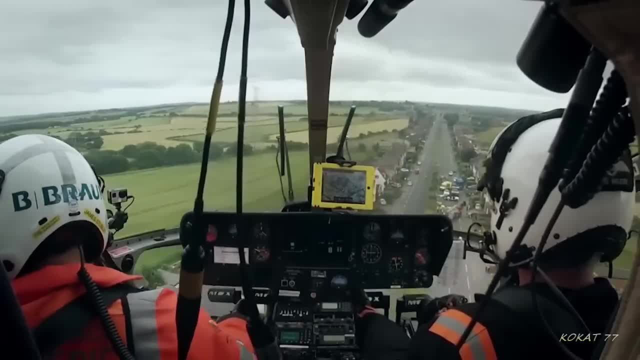 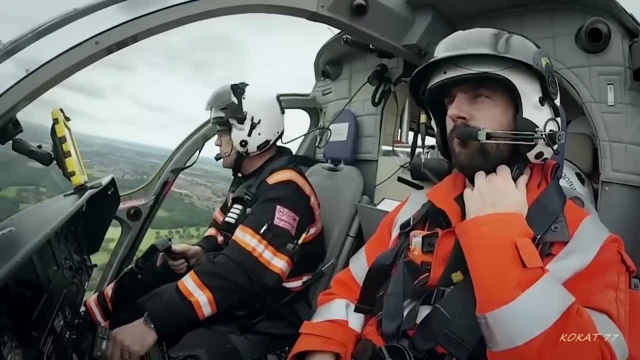 and a major police hunt for the occupants of the black car. 2655, the number is down to me. OK, man, Talk to you in a minute. All right, Cars aren't designed to withstand the kind of impact Tracy's experienced. 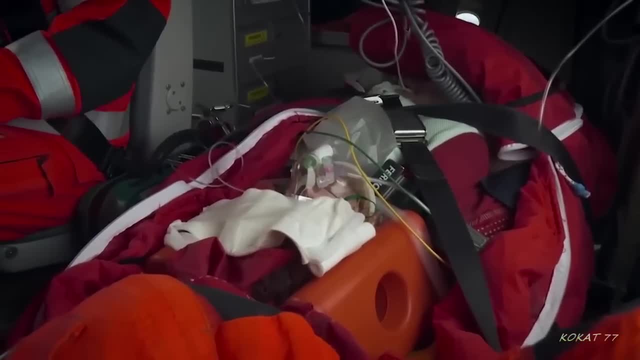 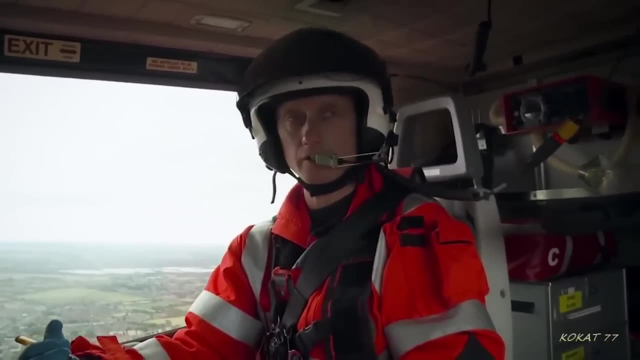 Her daughter's escape was down to luck and modern safety equipment. Massive impact to a bucket car. It just goes to show that a good, strong car and a good car seat nowadays does its job and reduces the risk of injury. Helimed 9-9, Alpha finals- LGI. 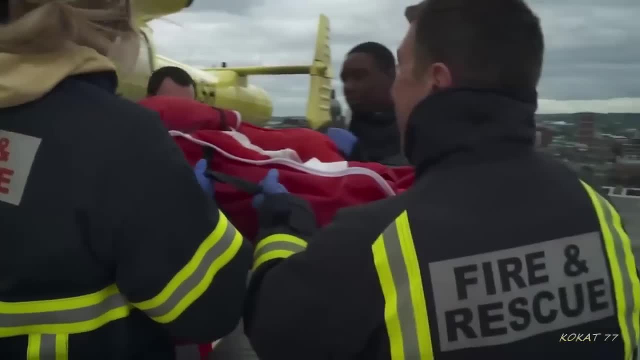 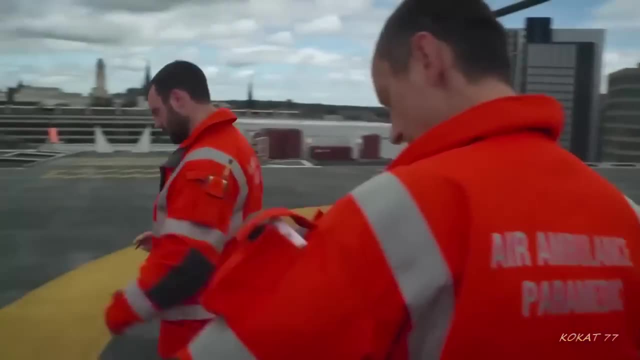 Helimed 9-9, London LGI. Tracy is being taken straight to resus for scans and X-rays and the first focus will be on her spine. It's not normal to have a lot of sensation. I would probably expect them to do a CT scan. 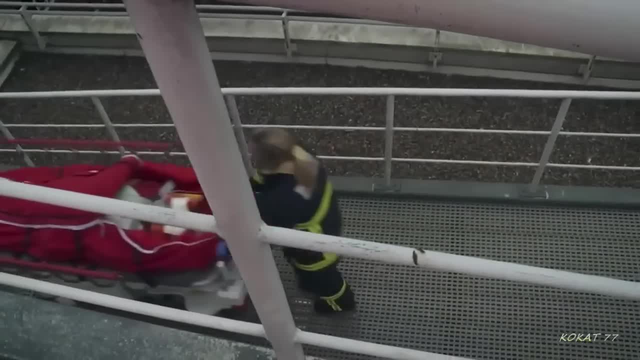 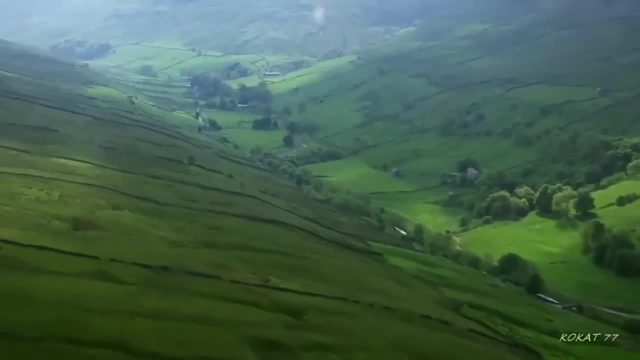 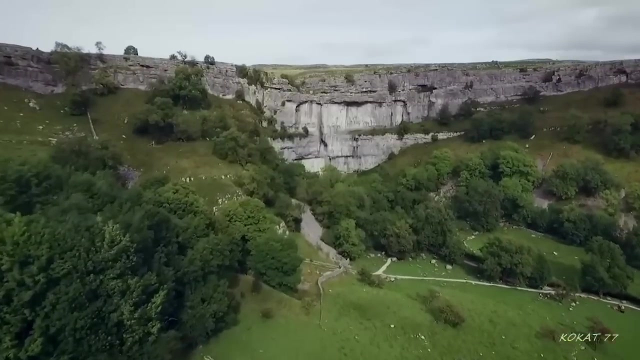 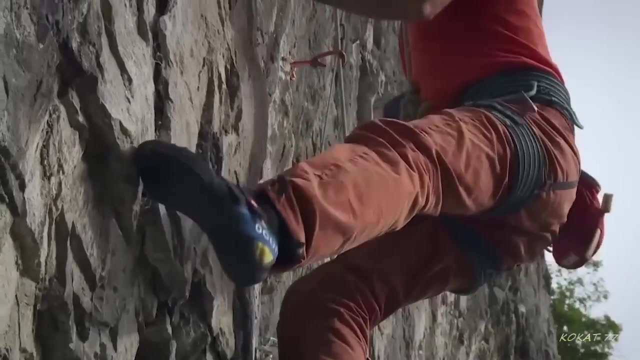 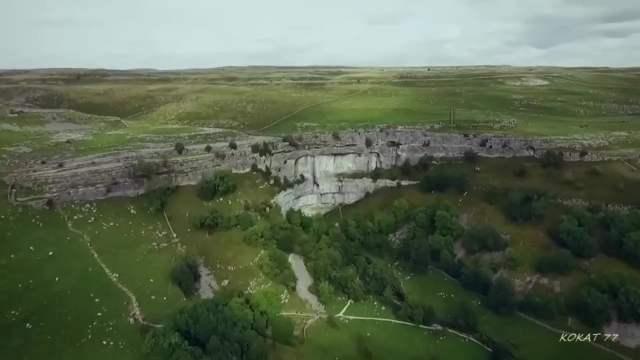 The accident could change her life. Malham Cove in the Yorkshire Dales is a prehistoric waterfall that was once bigger than Niagara. Now its limestone cliffs are an extreme playground for climbers testing their skills on a huge, 260ft high rock face. 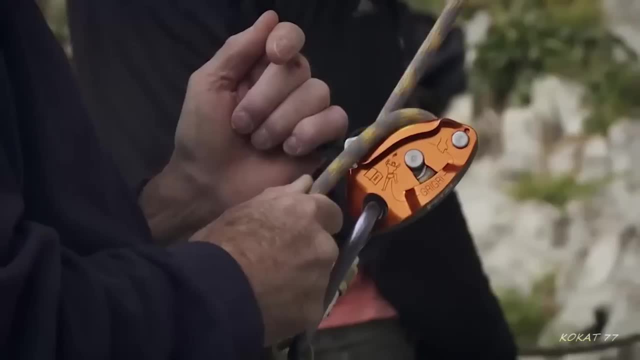 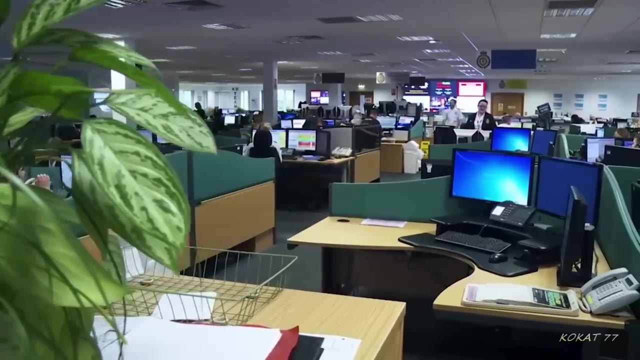 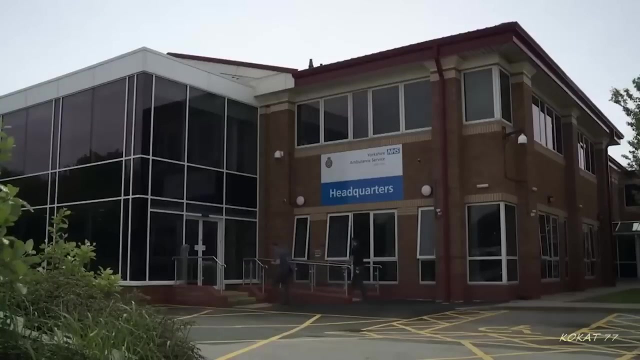 Ambulance service. is the patient breathing? He's making some noises like he's breathing. yeah, 50 miles away, reports of a serious accident are coming into Yorkshire's ambulance headquarters. And is the patient conscious? He's not conscious, Right. 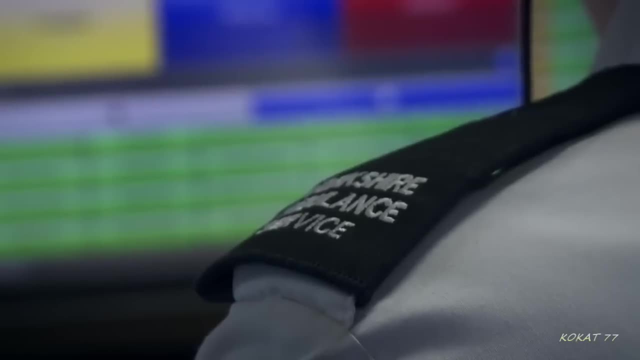 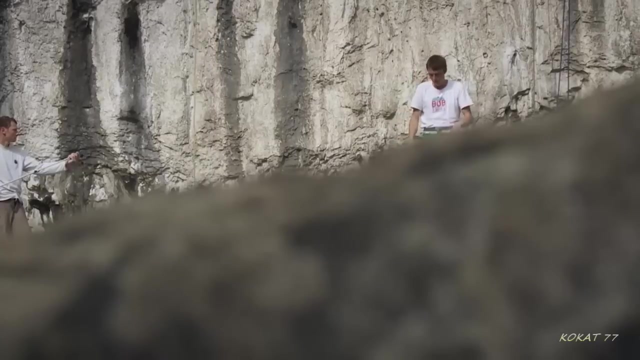 A climber's bad news. A man has been taken to Yorkshire's ambulance headquarters. He's not conscious Right A climber's, badly hurt and in serious danger of falling again. 999,, there's a job for you. It's Malham Cove. 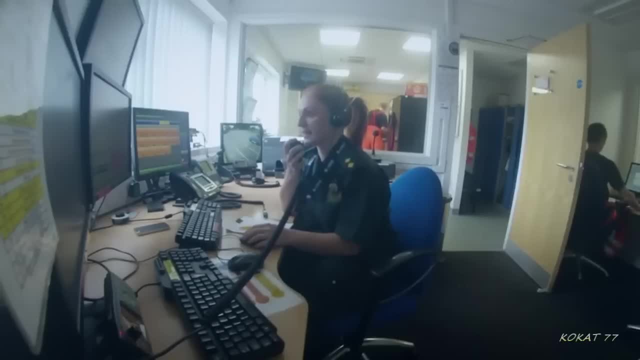 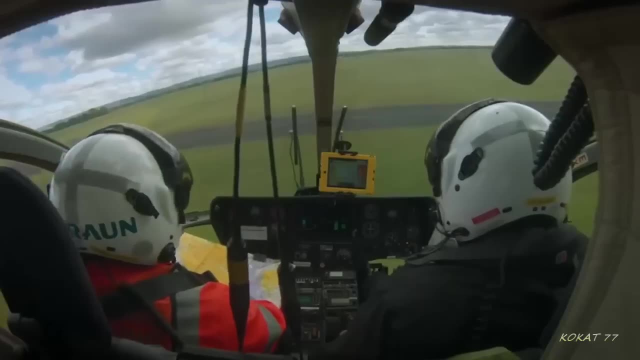 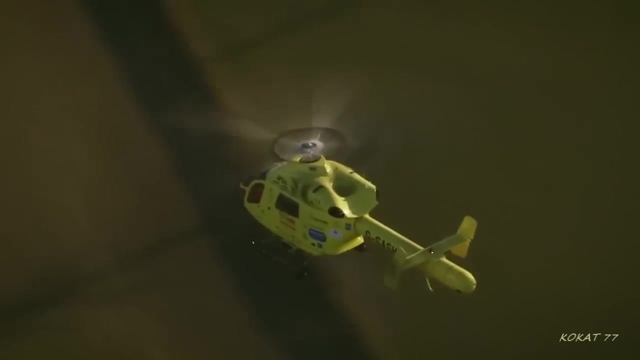 Someone is unconscious, fallen 10m head injured. Helimed 99 is his only hope of rescue. Top 5 traffic: Helimed 99 for lifting. departing to the south-west Malham Cove. Paramedic James is the leader of a mountain rescue team. 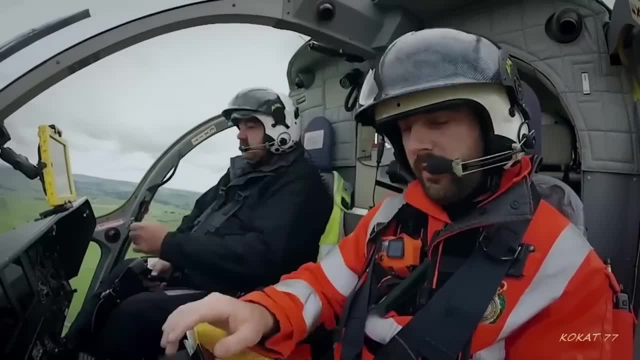 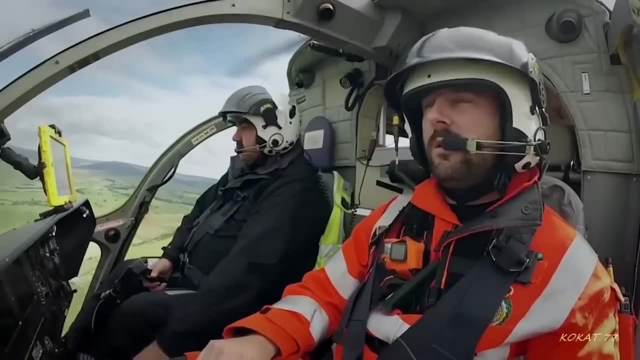 in his spare time, Right about 4 miles from his high ground. He's responsible for finding the patient today. If you're looking at the cove, it's the east side On the ledge And it's near the top of the cove. 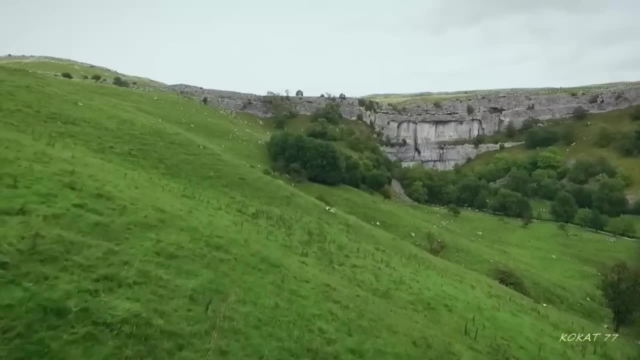 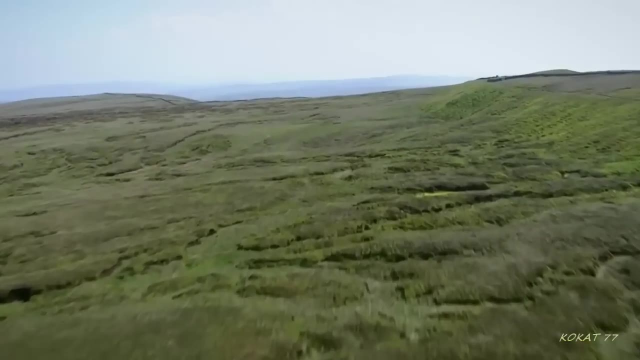 Yeah, The cove is one of Yorkshire's biggest natural landmarks and James knows it well. So we've got Malham, that's Gloucestershire, that's Malham. What we'll do is we'll approach to the right-hand side of the ledge. 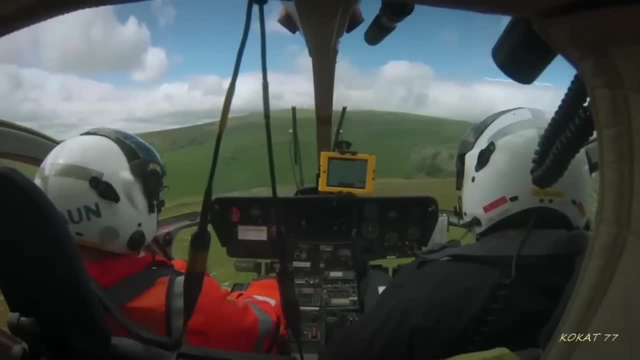 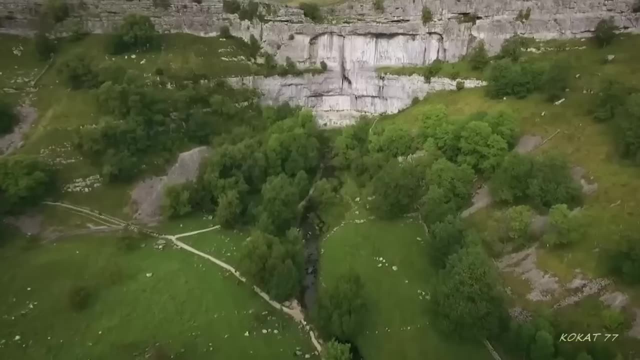 They're touching down in a lethal landscape. NS99. on the ground, The grassy slopes above the cove lead to a sheer drop with sharp boulders below. Paramedic Paul Holmes knows this terrain can kill. It looks like a bit of a precarious position. 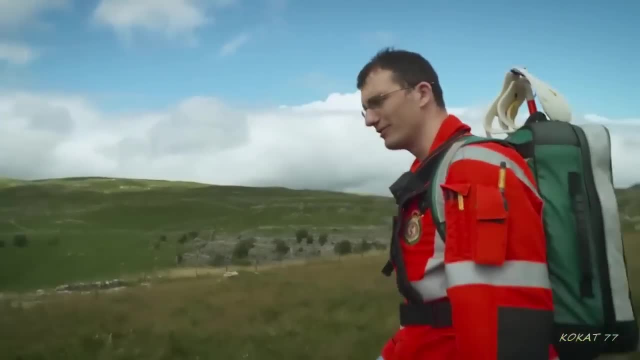 so we need to be careful making sure we don't actually slip and cause ourselves an injury. We've got mountain rescue en route, so off to wait and see when we actually get a bit closer to the edge, exactly where the patient is. 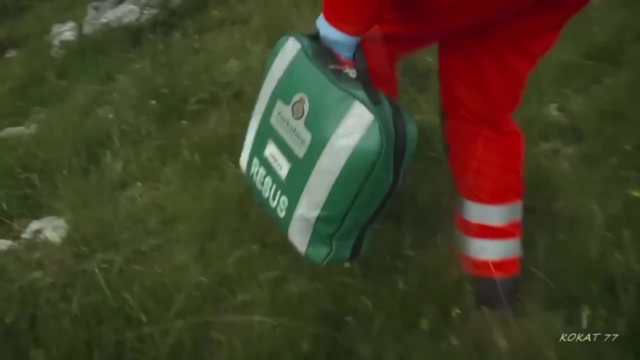 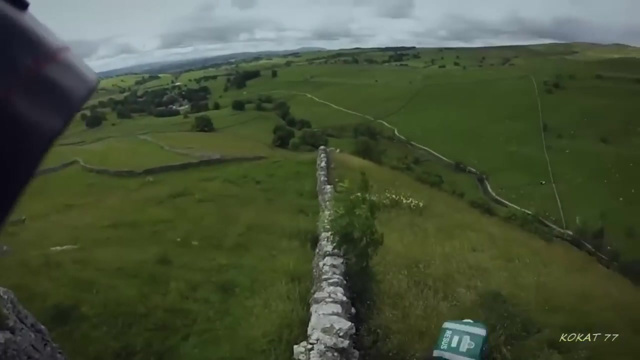 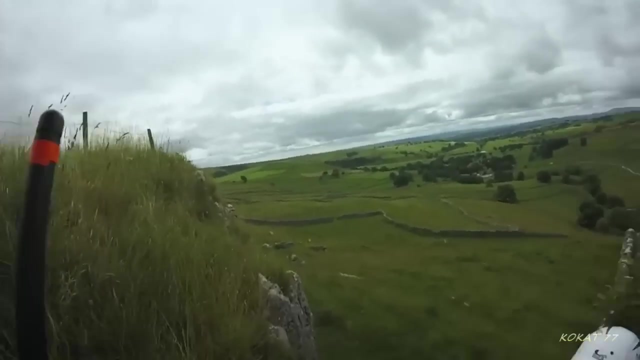 but it's a bit treacherous underfoot at the minute. really, You're in my territory now. Can I give you this, mate? yeah, Jeez, I've only got short legs, you know. Watch yourself, mate, all right. 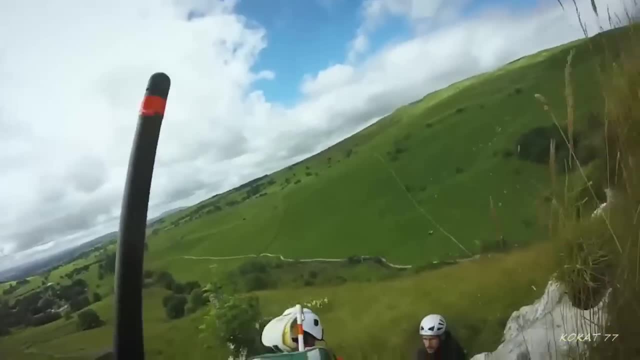 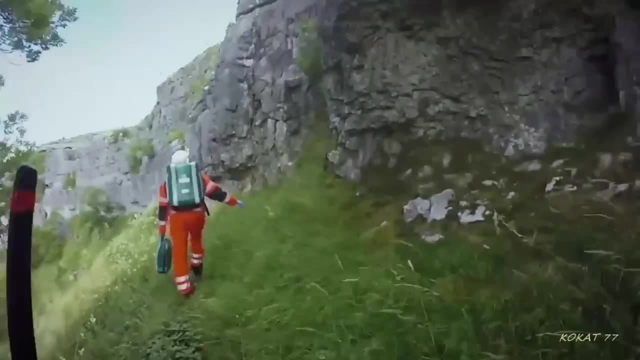 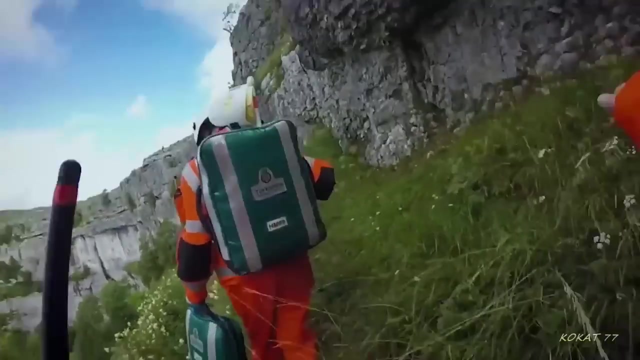 It's safer on your arse. Yep Cheers, mate. Unwary visitors have died after slipping on these slopes. Fucking hell. There's nothing between them and a treacherous 200-foot fall. Fuck me. Their patients lying in a precarious position on a narrow ledge. 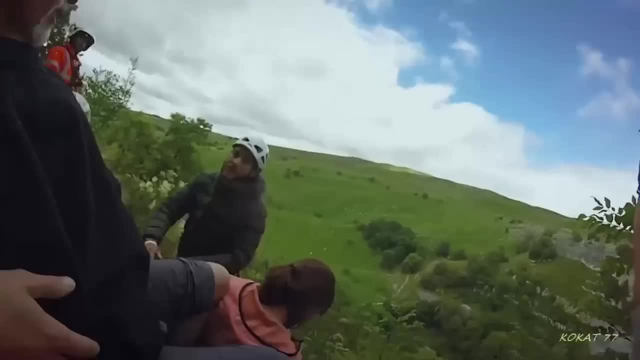 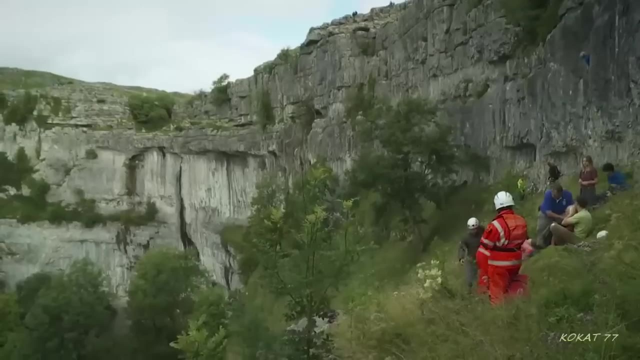 Hey, Hello guys. how are you doing? Victim and rescuers are one trip from a fatal fall. There's no obvious way of rescuing their patient. It's going to be quite a complex evacuation And all the possible methods involve a lot of risk. 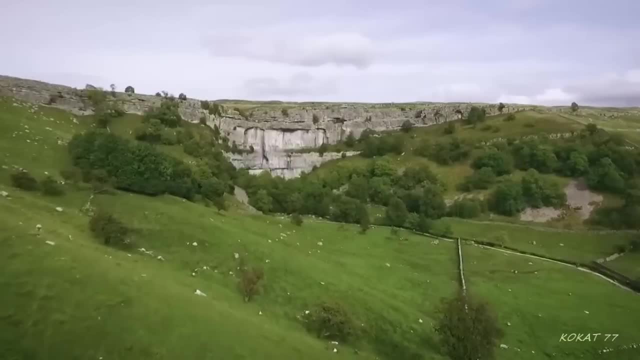 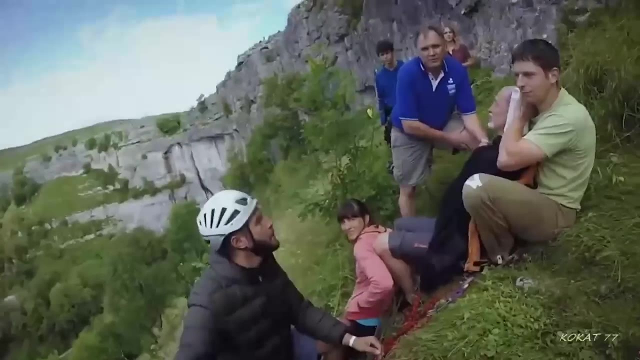 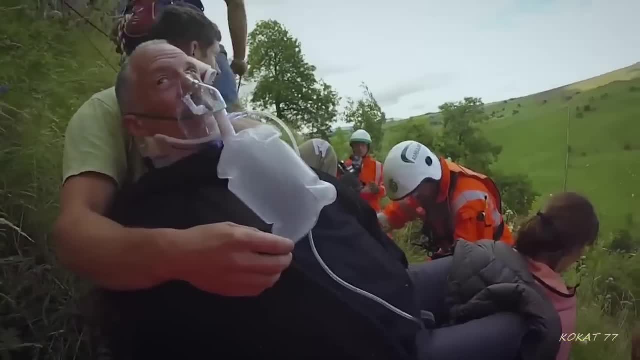 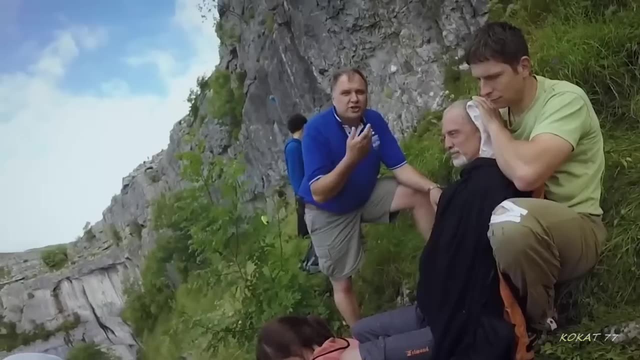 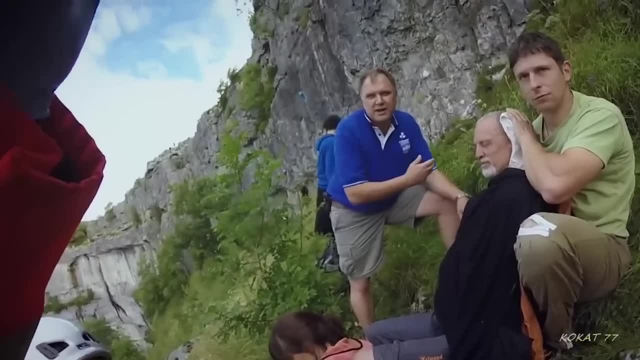 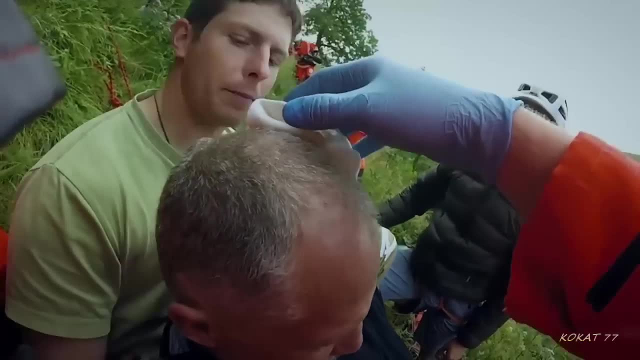 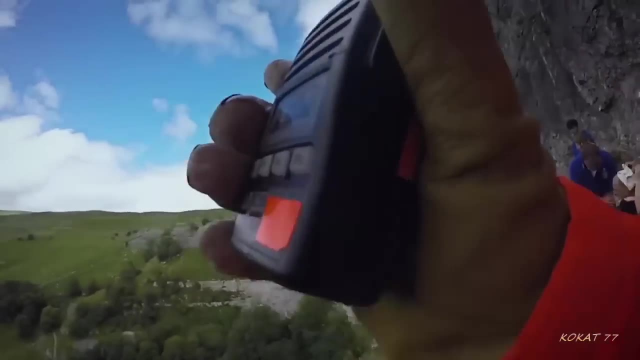 OK, we'll get you sorted. All right, can you remember falling? No, Can we look at that? It looks dramatic. Keep it on there, mate. Crow Andy, Crow Andy Helimed. 99. Search Dog Andy passing message over. 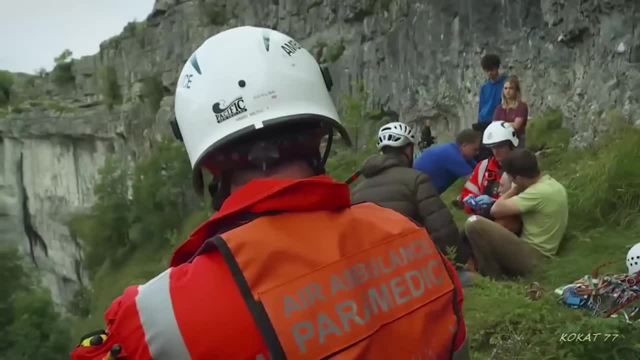 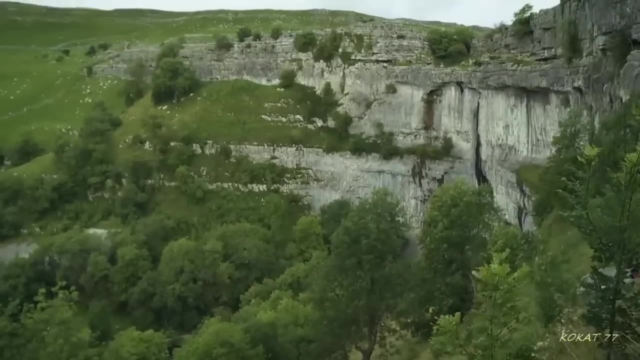 Yeah, Search Dog Andy Helimed, 99.. We're on the ground above. We've actually just arrived at the patient. now It's going to be quite a complex evacuation from here. I suspect we're going to need, obviously, a stretcher and ropes. 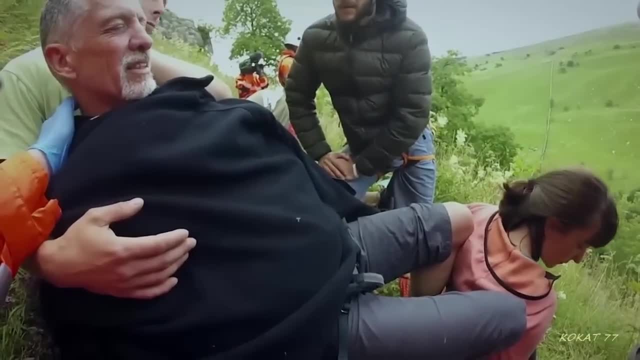 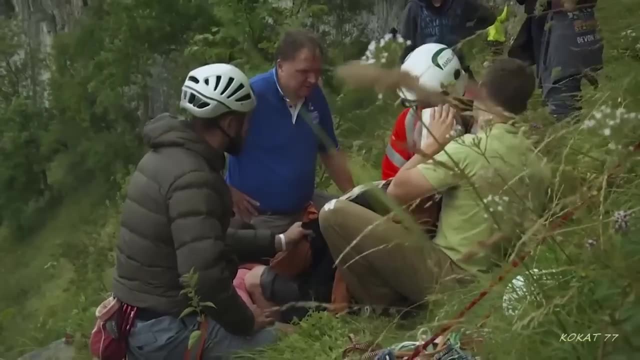 So if I just press down the back of your neck, is there any pain in the back of your neck A little bit, A little bit Centrally, or is it to one side? It's to where you've said, OK, no problem. 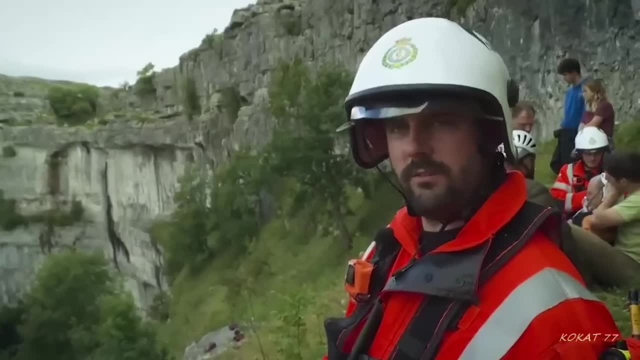 The working environment's not ideal. We're on steep ground so, as well as your own safety, we've got to be mindful that kit's obviously going to drop below. We've still got people climbing around us And then we're going to have to somehow get him onto a stretcher. 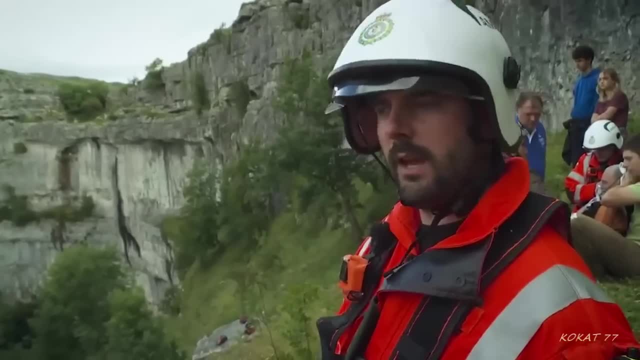 a loaded stretcher either up to the aircraft or down, for us then to relocate. So it's going to be quite a big job. It's going to be quite a big job. this James is concerned that one accident could lead to another. 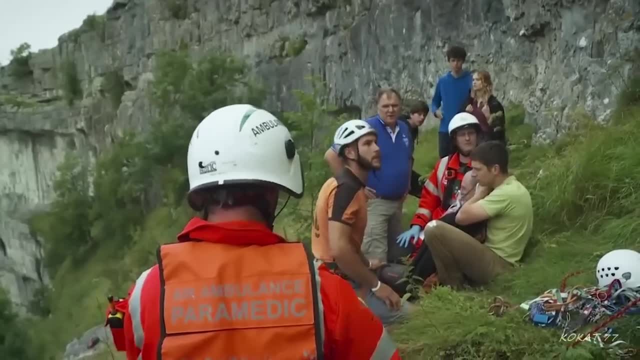 Is it just worth tying him into something, just so we don't all go? At least a couple of us I'm conscious of. I think we should be all right. yeah, Well, at the moment that girl's probably holding him up. 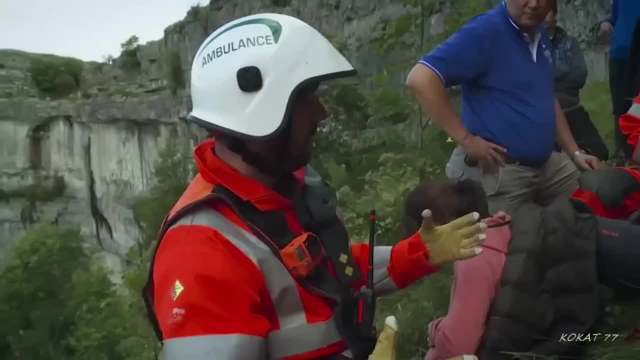 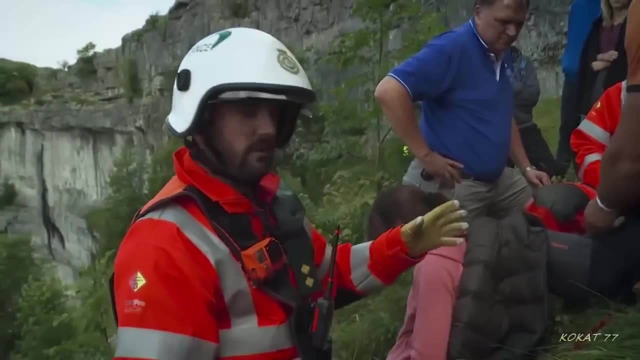 And if she slips, what's stopping you guys from going? But we're all in quite a precarious position. Everyone seems quite capable in this position, but if somebody slips, we just obviously want it as a bit of a backup. So we're just going to tie him in. 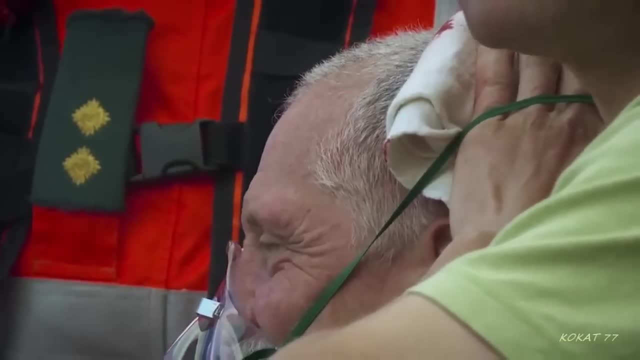 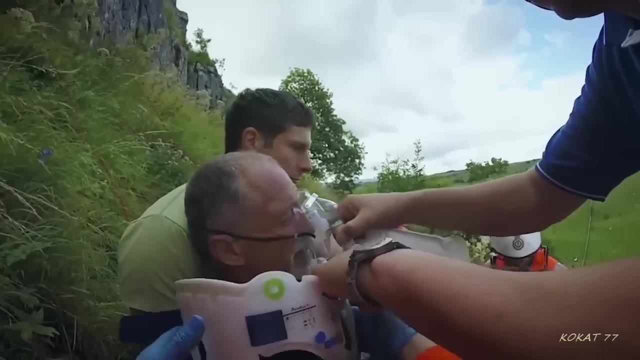 The team want to protect Rod's neck, but the slightest movement here is fraught with danger. I don't even think we're going to get this on. to be honest, Can you look at the chin? maybe? The thing is we don't want him to move his head, do we really? 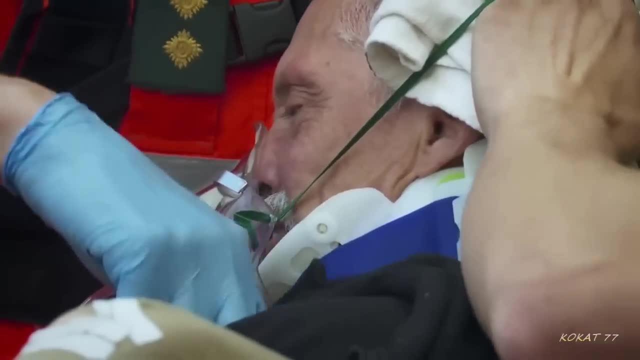 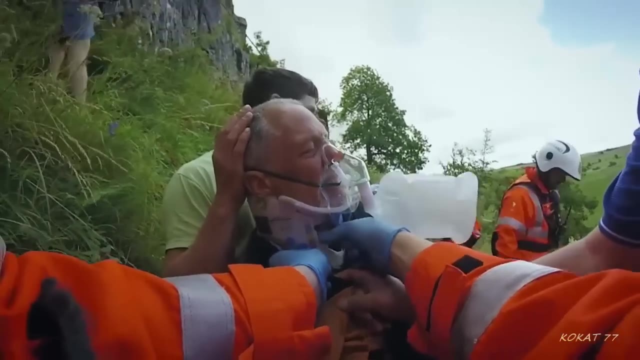 Yeah, You know what I mean. Rod's head wound looks superficial, but his growing confusion is very worrying. What happened? I've had a bit of a tumble, I think, off the rock Right. OK, I think you might have got a bit of a concussion. 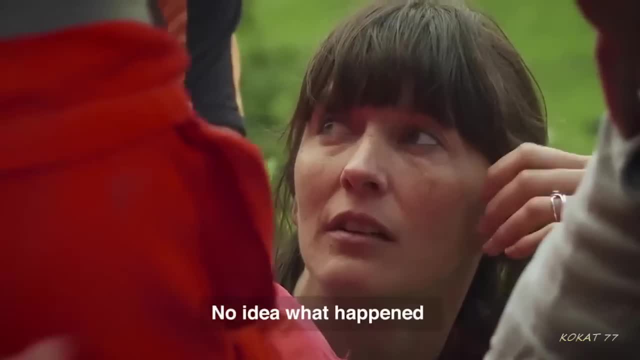 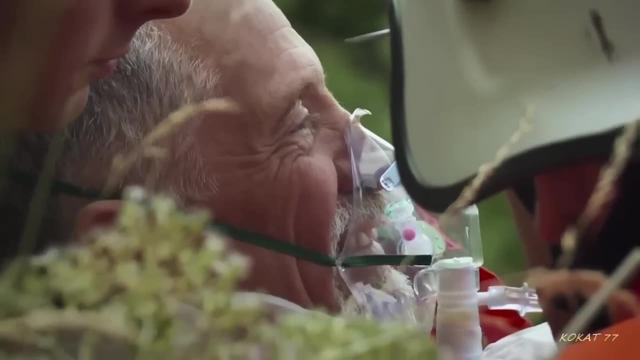 Oh dear, I'll get it in there. What happened? Any idea what happened? No, he's fell off while he was climbing. He's getting a bit repetitive, sir. It's becoming clear. Rod has several injuries, any of which could be life-threatening. 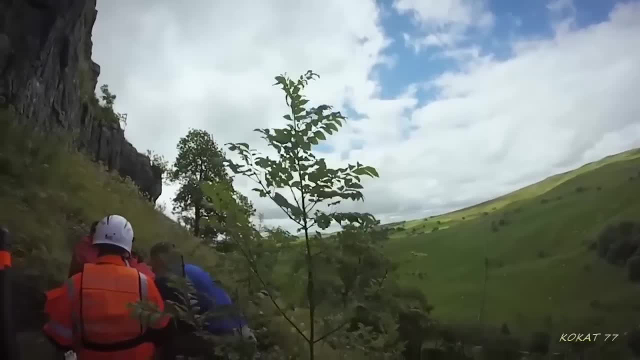 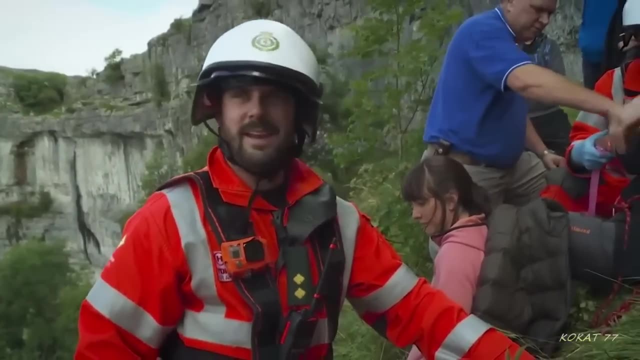 He needs an immediate evacuation, but that won't be easy. I think the plan is to probably sledge him down on a stretcher down into the bottom of the cove. So that's plan A at the moment. I'm sure B, C and D will come into it at some point. 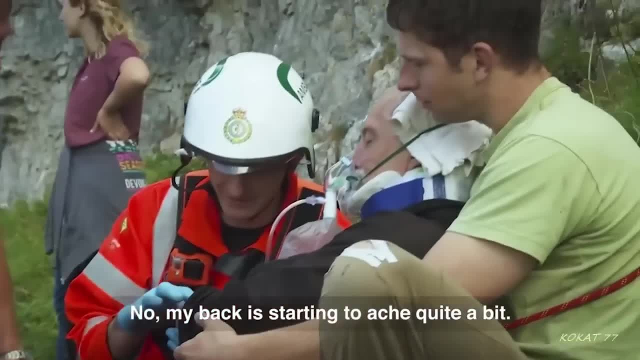 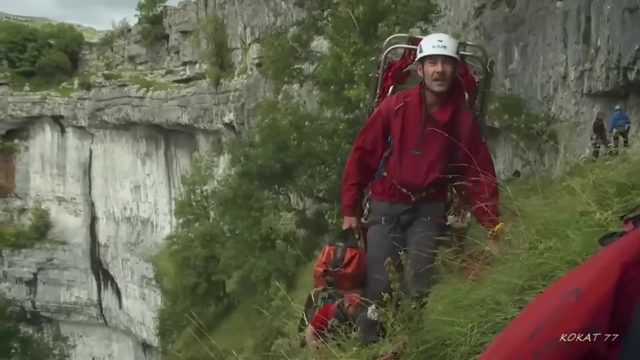 Are you and Rob all right? No, my back's bad and I'm going to eat quite a bit. It will do, mate, Do you know? I don't know what's up with your veins, mate? At last local mountain rescue experts have reached the scene. 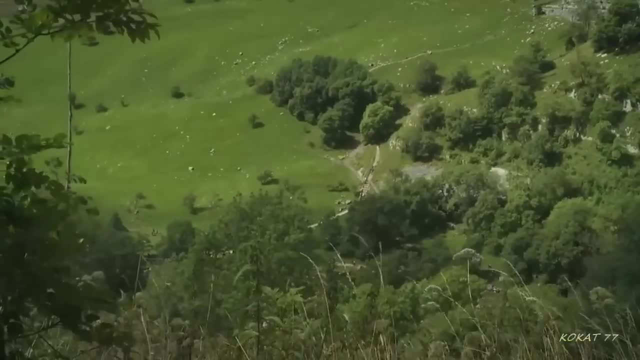 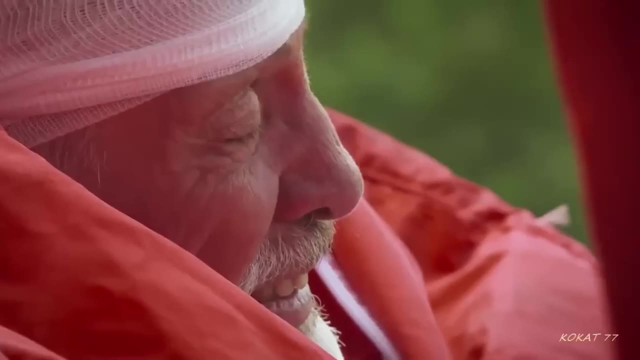 Are you all right? They're equipped to lower Rod down the rock face using ropes. How are you doing Good, thank you. Definitely slow and steady as opposed to anything in a rush, But it could worsen his injuries. What do you think about getting the coastline in and taking it out the top? 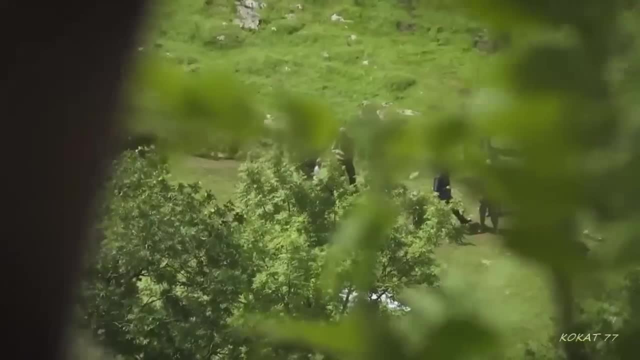 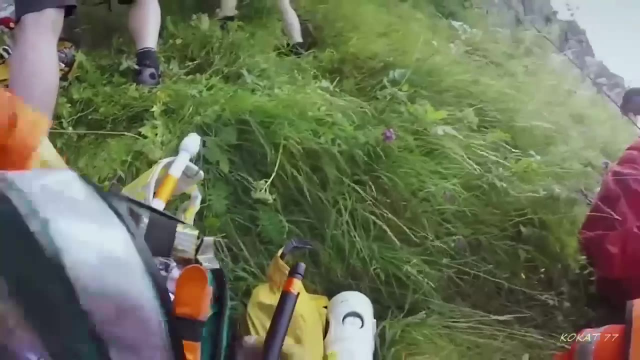 I said I'd leave it with you guys. really, I mean, we can request that anyway if need be, Because the smoothest would be up and out. Oh yeah, we're out of doubt. yeah yeah, Even minor medical treatment is difficult to deliver safely. 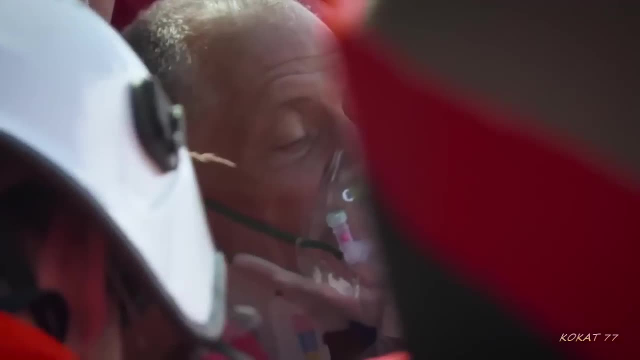 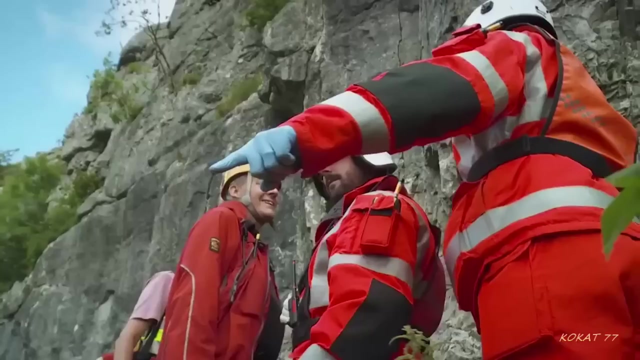 and Rod's showing signs of deteriorating. James is being forced to reassess the rescue plan. He's got no altered neurology but by the time he gets down there, if he has got an unstable fracture he may have, Let's just move the ride up if we can get it out. 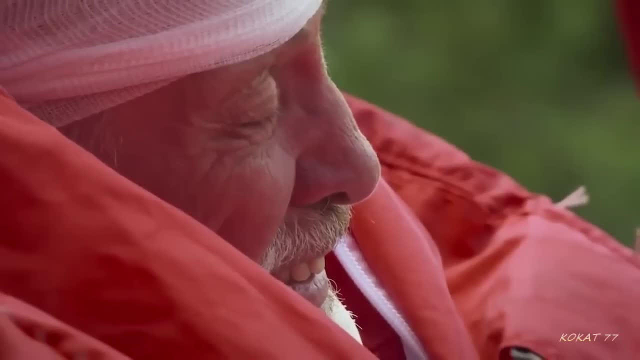 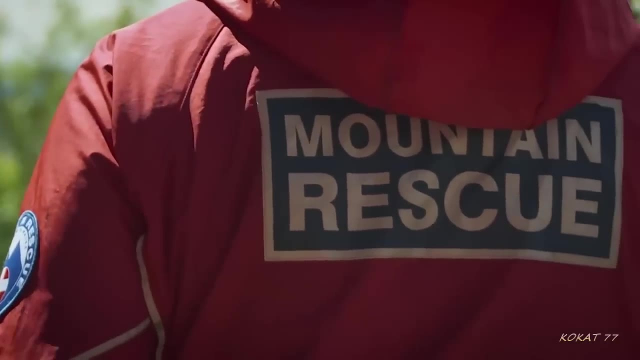 You know what I mean. They're calling in the Coast Guard to winch Rod from the cove. Three emergency teams, including £20 million worth of helicopters, are now on a mission to rescue Rod. We'll need to clear it and every bit of crap out of the way. 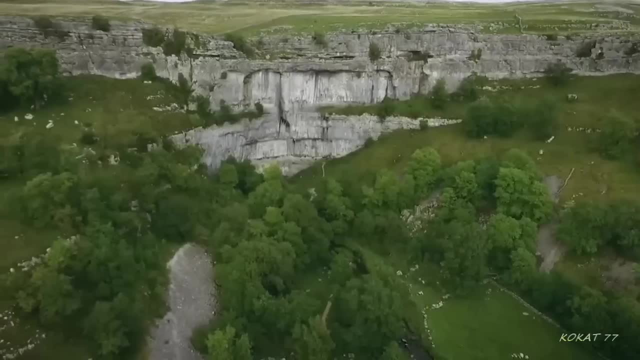 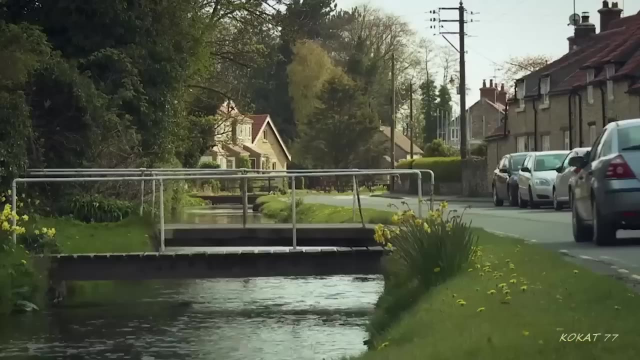 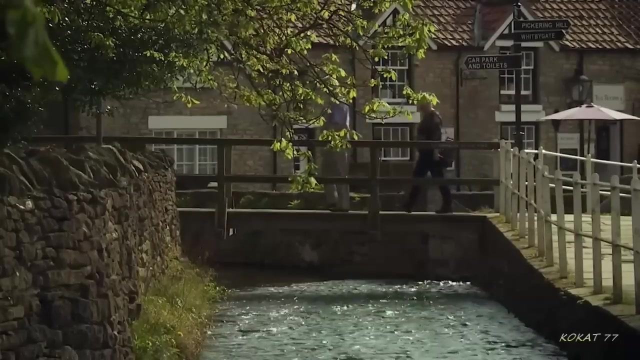 I'm going to say it'll blow us all to smithereens. The quaint towns and leafy lanes of North Yorkshire make it the perfect place for a romantic getaway, But today it's the backdrop to a serious car accident. Nice to meet you. 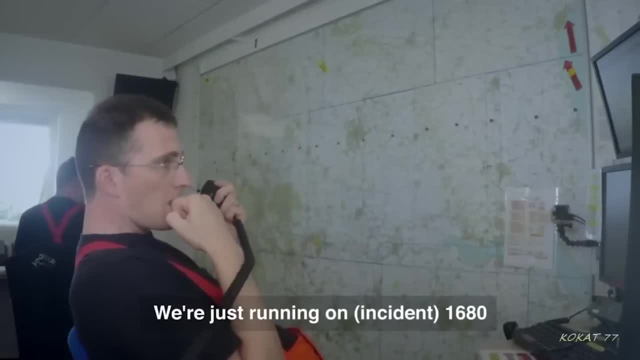 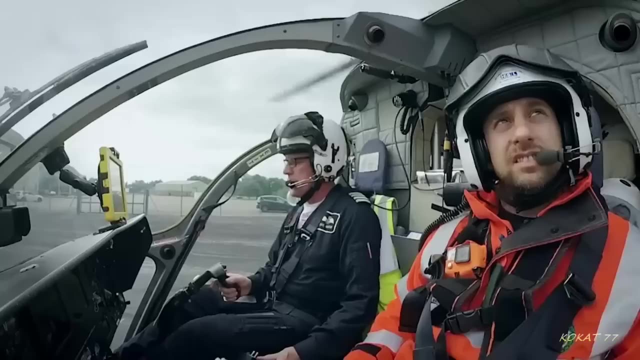 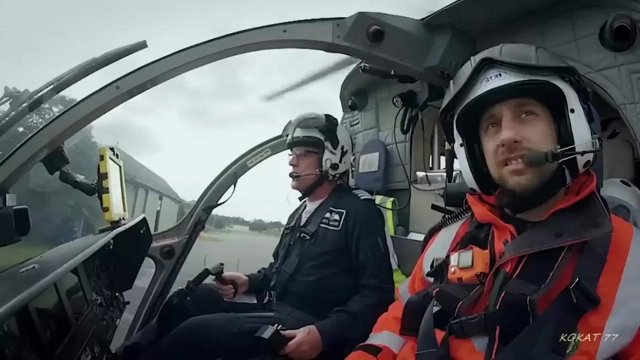 Nice, Dave. We're just running on one to 680.. Apparently we've got two. The victims of the crash aren't sure where they are. It's up to pilot Steve and paramedics Aidy and Pete to find them. The crash has happened near the famous white horse. 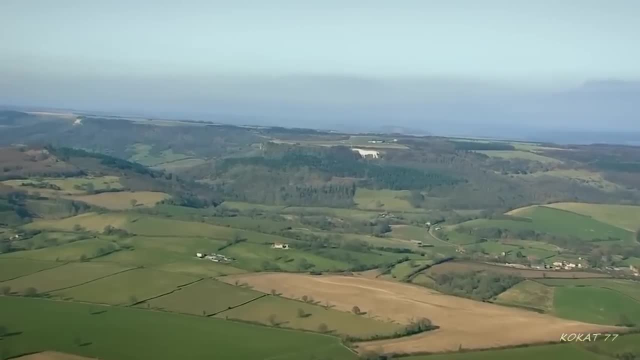 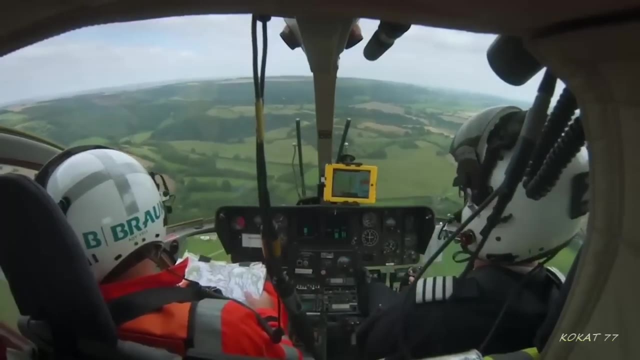 on the edge of the North York Moors We're going through a little bit of a sound that obviously calls Broxton for an old traffic accident. Now we don't actually show it's in Broxton, It's just a general area at all. 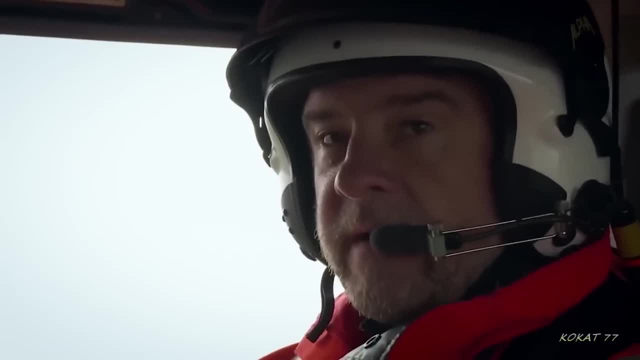 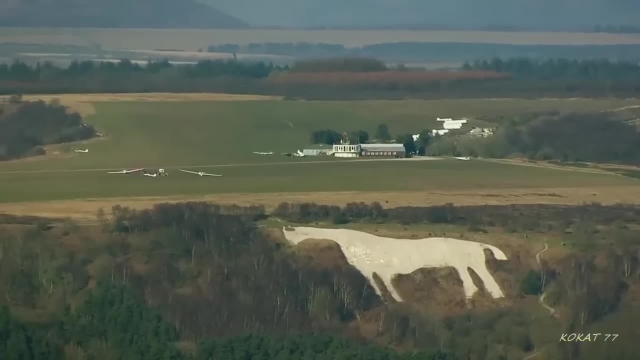 so it could well be that that's where it's at. That's just the nearest mobile phone mass that's pinged the 999 call. There's your incident, now half past 12.. Yeah, I've got the DCA approaching. 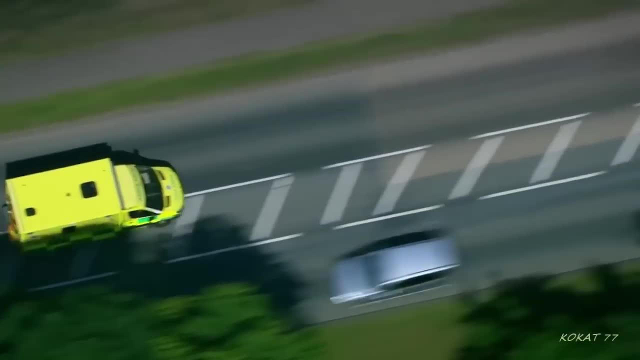 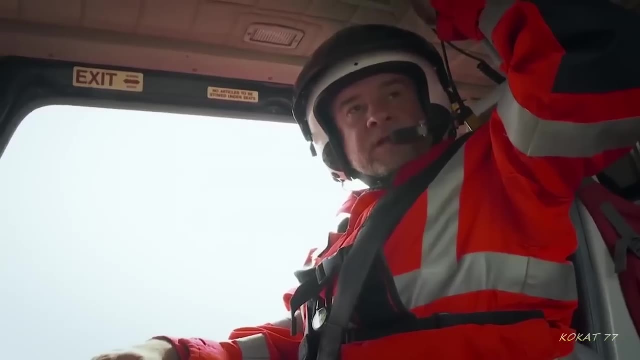 The team find the accident at the same time as ground units. Oh, dear Edison 999, visual scene there Also got visual on the DCA racing to it, haven't we? A car carrying An elderly couple has rolled over, hitting a dry stone wall. 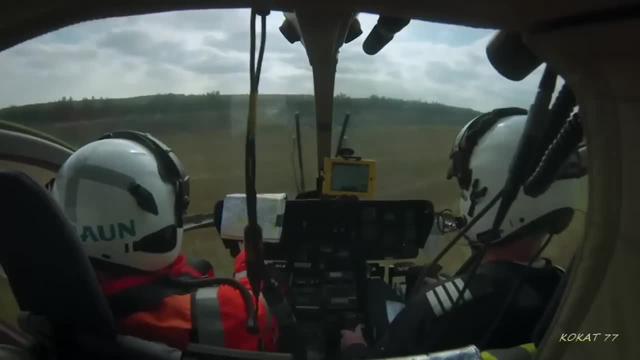 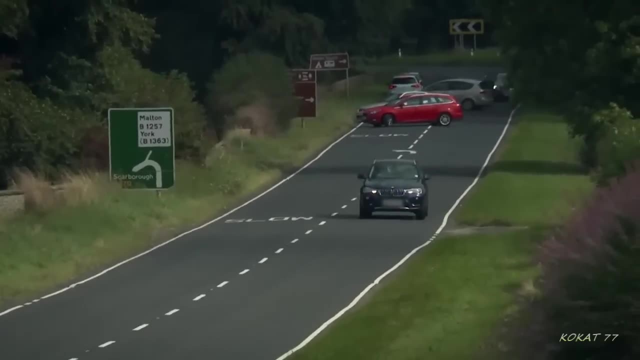 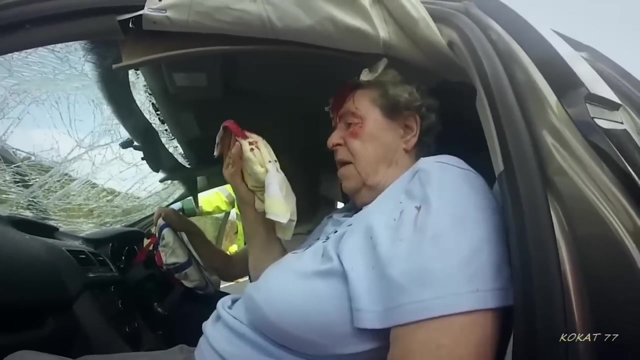 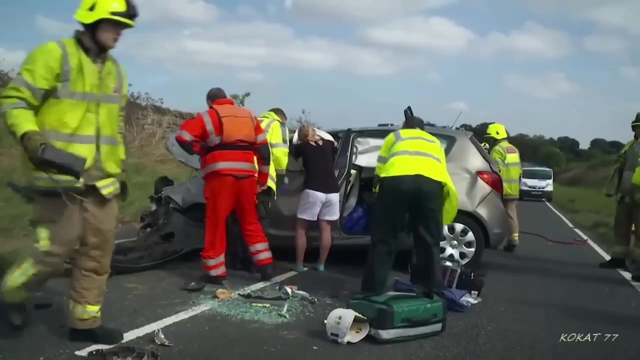 I'm going to put you in the field this side of the broken wall, Broken wall of the cliff. Bill and Ruth were on a break to celebrate their golden wedding. Now they're trapped. A passing GP stopped to give first aid. This is Ruth. 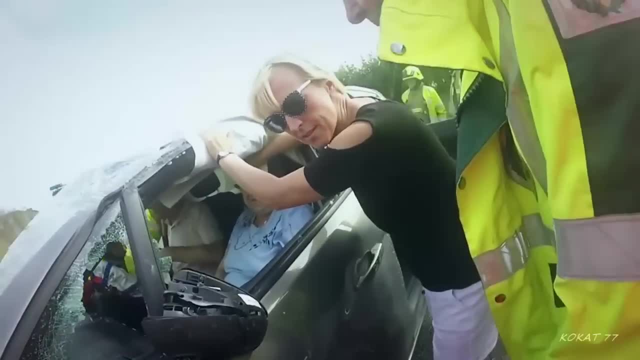 Hello Ruth, Hello Bill, Hello Ruth, Hello Bill, She's only on statin, She's on simvastatin. She's got no other health problems So roughly. do you know what injuries we're dealing with at the moment? 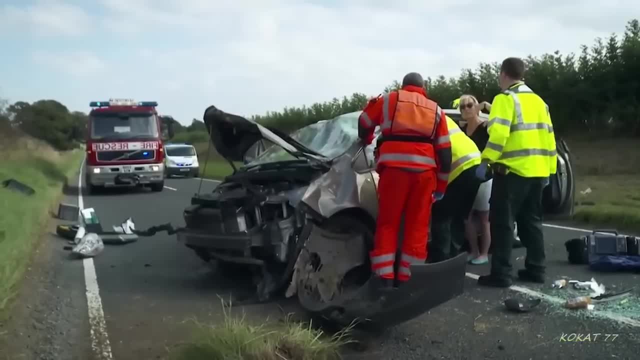 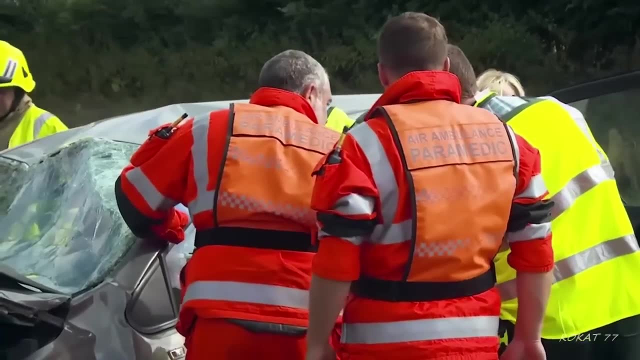 You just happened to hit that wall, hasn't it? Yeah, turn sideways on double turn. Yeah, She has a head injury. He's in shock. OK, Get a. You're on a cock. Yeah, get a dressing pad. 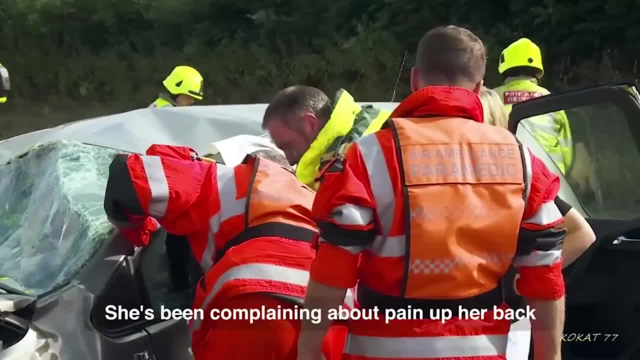 Test it out as well, mate, so we'll have a look at that, Right? so that seems in a bit. She's been complaining of a very pain in her back, Yeah, Beyond her ribs. OK, What's happening with this gentleman over here? 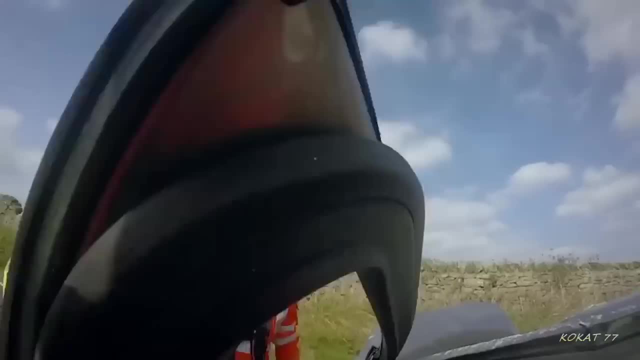 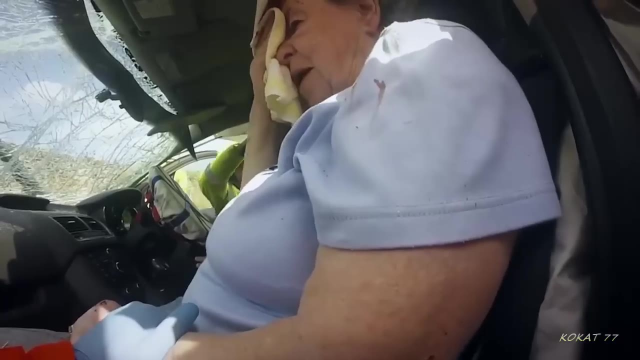 He seems quite moving about. Have a look with him. Cheers, Eddie. Hello Ruth, Hello, How are we doing love? What's up? Sorry, sir, This is Bill. I'm not so bad with my back, Whereabouts in your back. 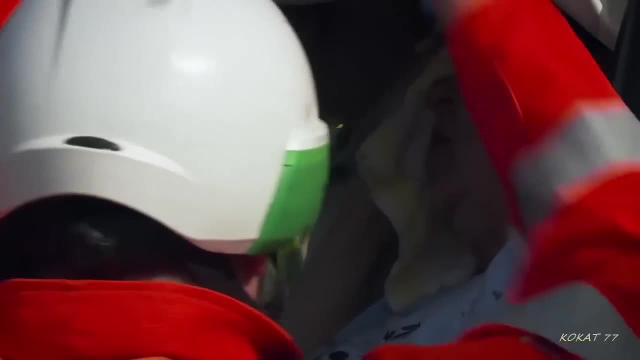 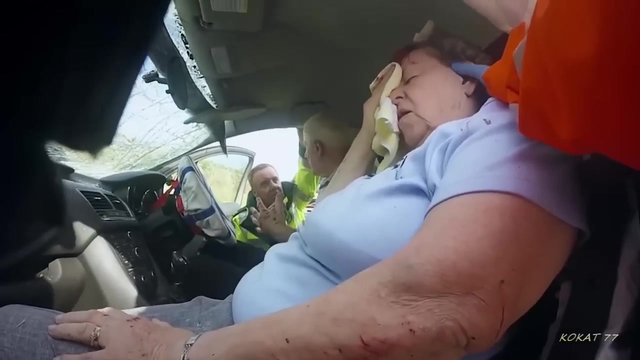 Oh sorry, In your side, Ruth could be describing a spinal injury. Let's do one. Let's have a quick feel of your neck. all right, Have you got any pain on the traction there? How are you doing, Dave? 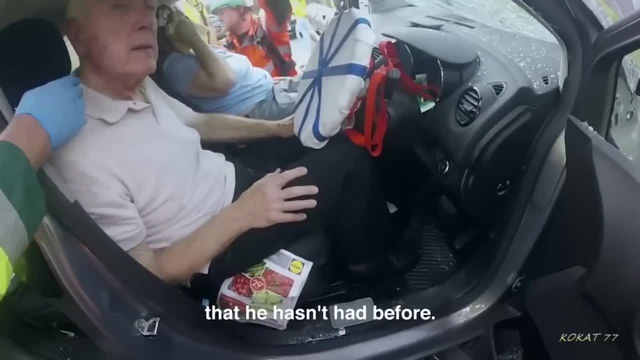 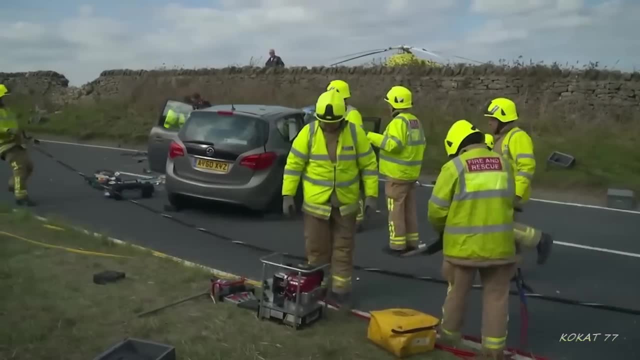 It's all right, He's not much back. Hello, He hasn't had it before. He can't do his aim, which we think is the glass. Yeah, But no other pain anywhere else. OK, How do you want to take this lady out of the car? 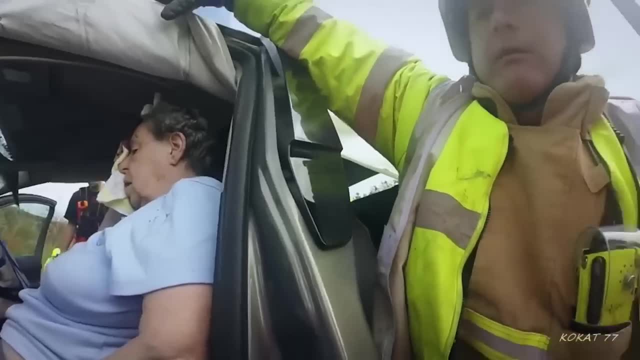 Do you want the roof off? or I think, at the way we're looking at the moment, we should be able to just get her out the door, because we've got the door moved right over there, so it's going to be all right on that one. 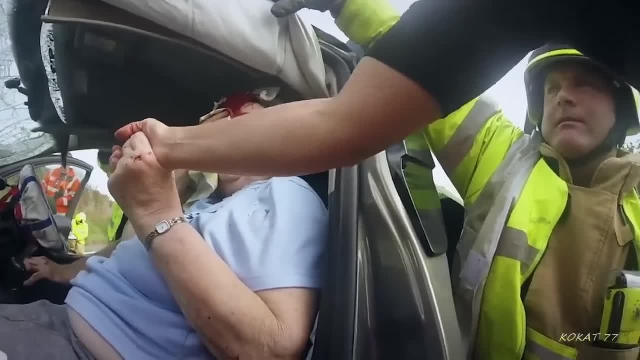 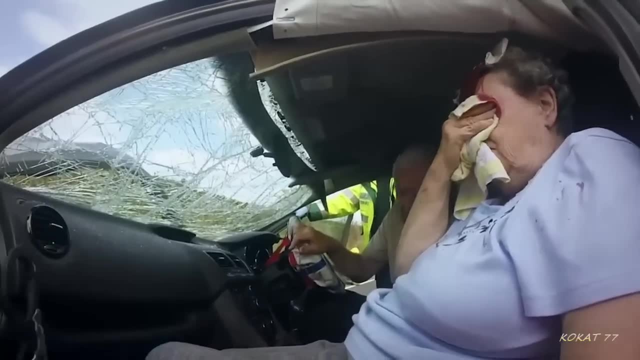 I'm sure everything will be fine. OK, All right, You're very welcome. The local GP narrowly escaped the crash. I was coming down the road and this car had to pull in to actually avoid me And as we went past, luckily we didn't collide at all. 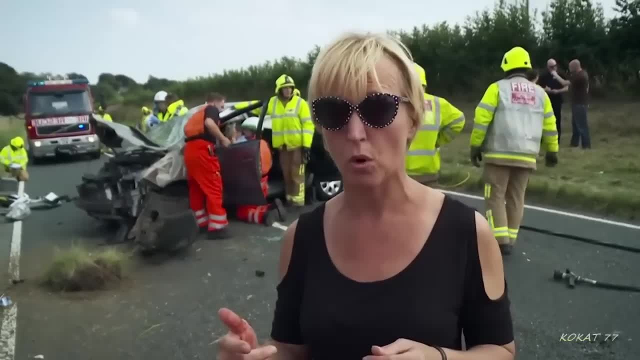 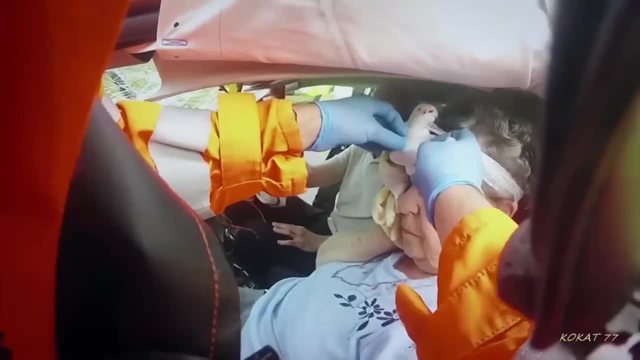 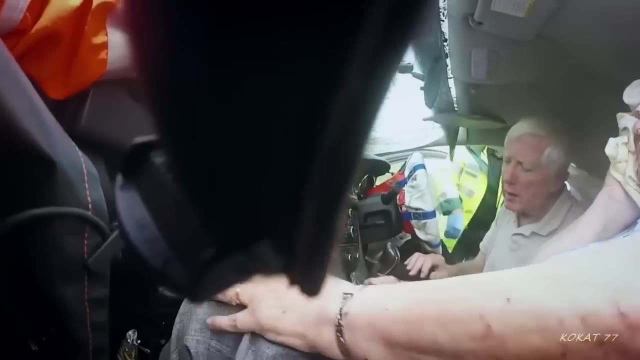 I saw in my rear-view mirror the car overturned a couple of times and hit the wall. How old are you, love? 77. 77. Elderly people are more likely to be permanently disabled by a road accident. The team's worried about both of their patients. 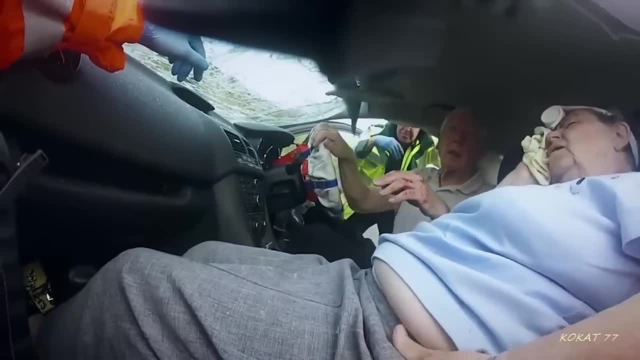 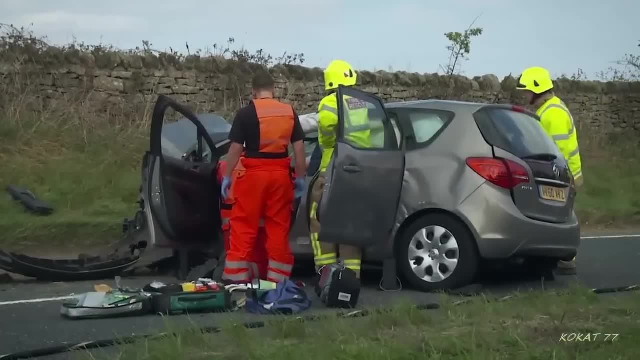 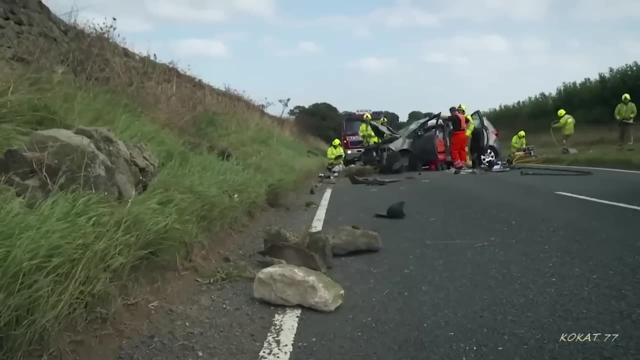 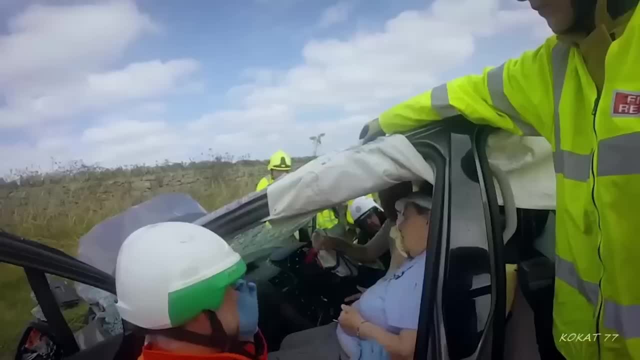 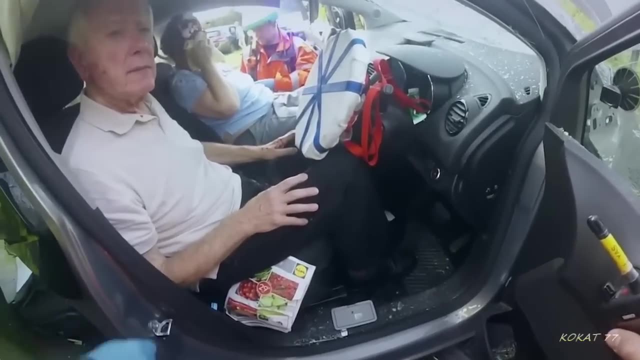 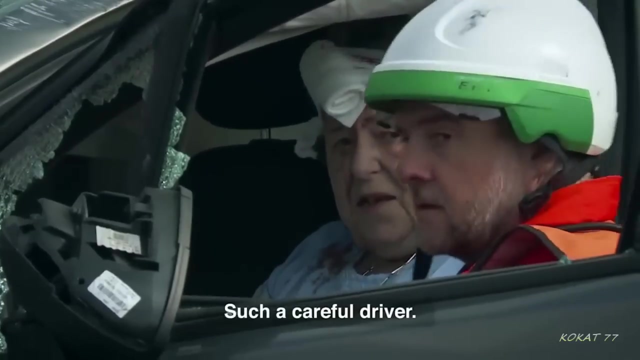 Any pain when I'm pushing you on there. How does that feel, Ruth? Not so bad. Not so bad. After a lifetime of driving, this was Bill's first accident. All he cares about is his wife. You're such a lovely man and you're such a careful driver. 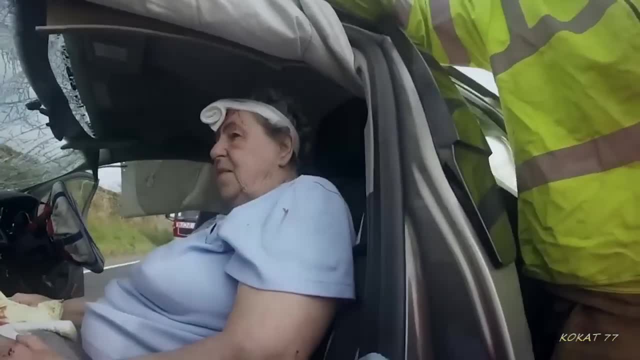 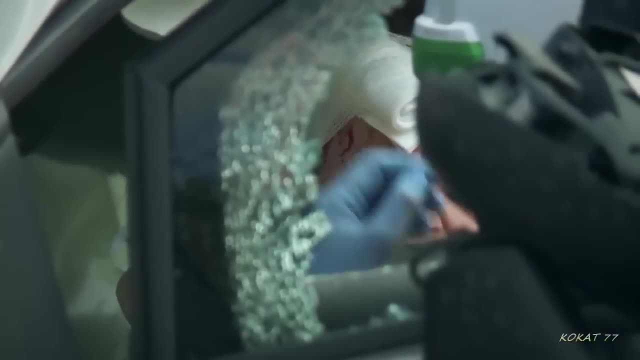 Well, he's obviously not. He's obviously just one of us, and what actually happened then, I don't know. Hmm, All right, then You've got a great big whacking. You're going to have a big bruise on your head, though. 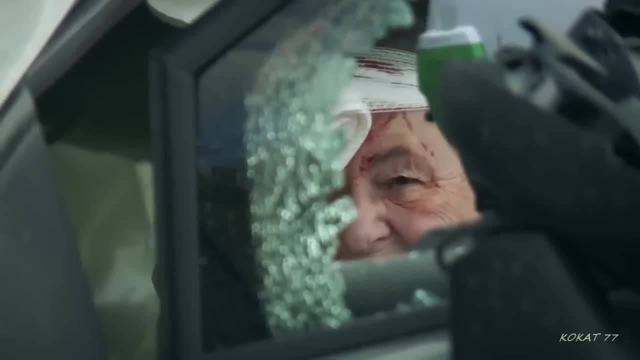 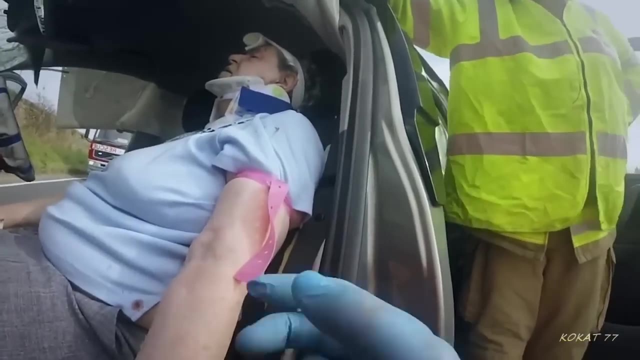 All right. Yes, You look like you've been cage fighting, So I'm just going to pop a little needle in your arm. It basically means if anything starts to hurt that we don't know about at the moment, we move you, I can give you some painkillers, all right. 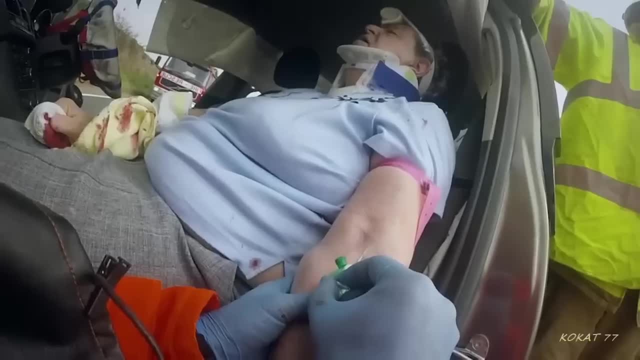 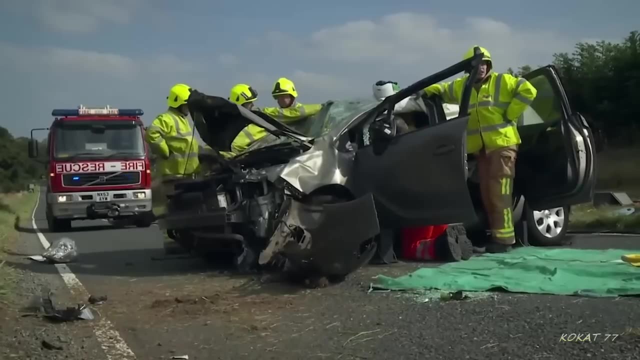 She's got a big haematoma and lack to her head just because of the head injury and her age and there's some sort of force. We're going to fly her to James Cook. Yeah, You come round here, Ray. I'll just guide your legs. 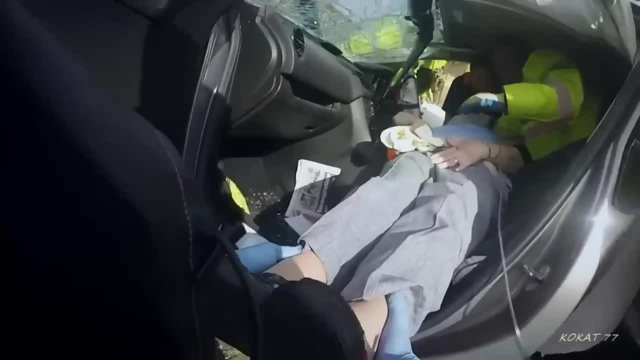 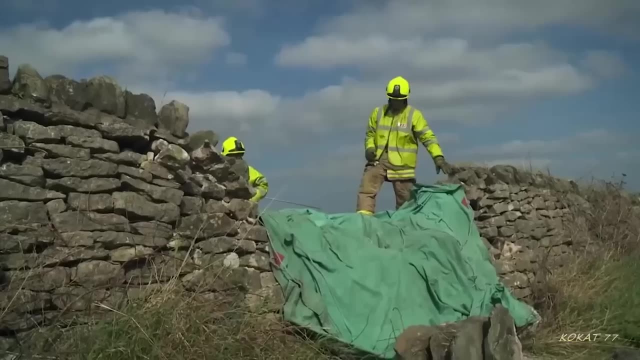 Yeah, I've got You. all right, Ray, That's it. you just lay down, We've got you. You've got your head: Wonderful, Ready, steady, move. That's enough. They'd booked this break as an anniversary treat. 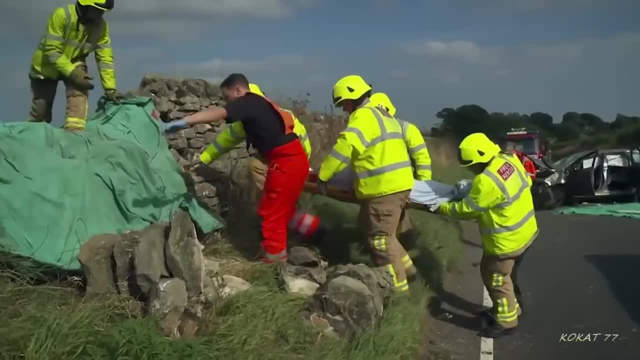 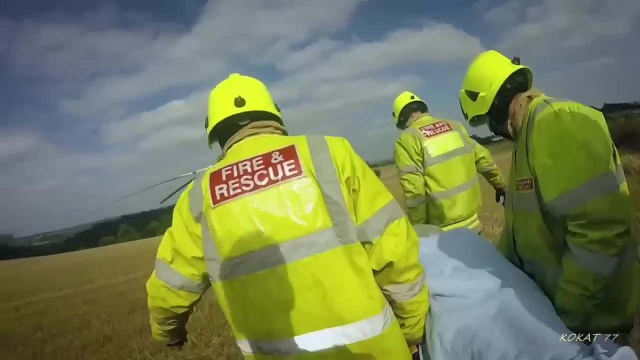 Now she's leaving him for a flight to hospital. We all ready, Ready, steady. lift, Here you go. Yeah, OK, you all good. So she'll need to go in feet first. Bill is being driven to the trauma unit. 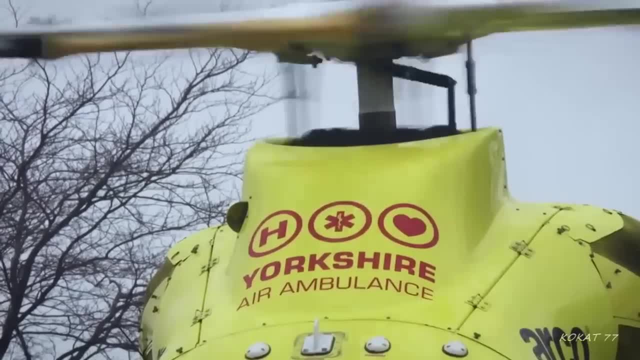 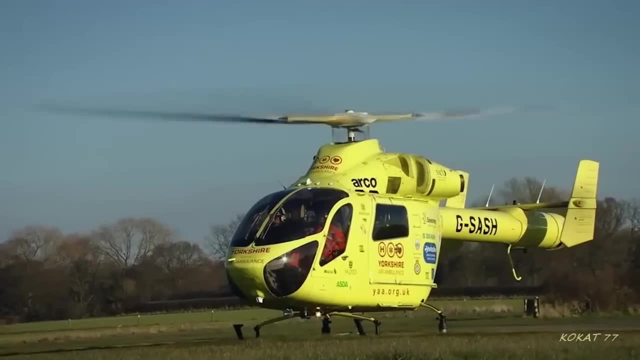 of the James Cook Hospital in Middlesbrough, Ruth, will be there first. Lucky the pair of them. Very, very lucky indeed. How did it Nine, nine, Lifted, didn't James Cook ever? She's a 77-year-old lady. 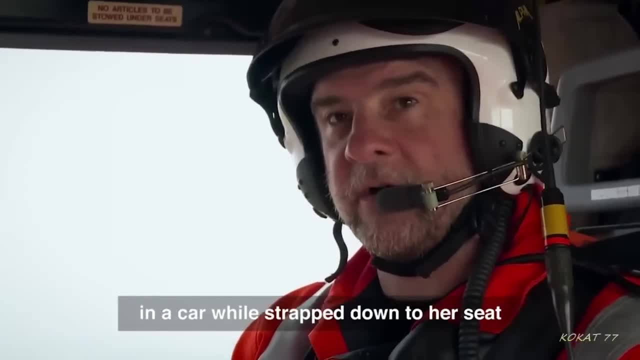 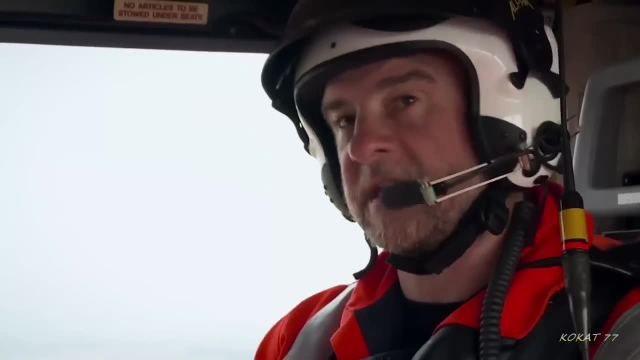 She's been thrown around at probably best about 40 miles an hour in a car, while strapped down to a seat. Looking at the amount of blood and the amount of hair that's stuck in there, there's every chance that could have actually gone through. 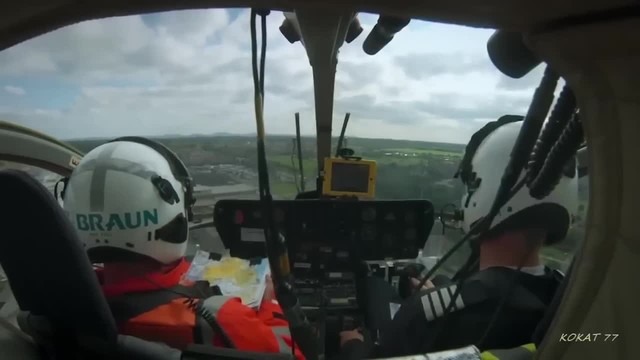 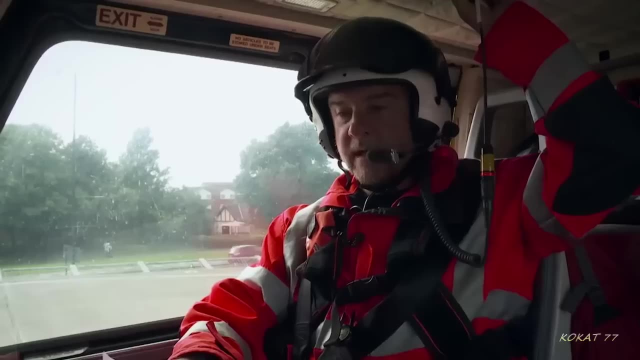 to the bone and that could be an athlete's infection risk. Look through the light station. The couple hoped that this would be a happy day in the countryside to celebrate 50 years of marriage. Nine nine on the ground. Now Ruth faces several weeks in hospital. 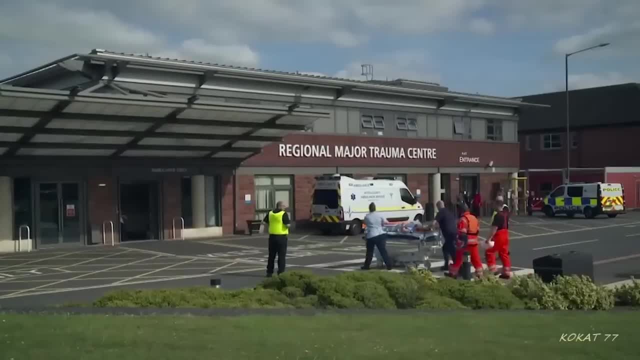 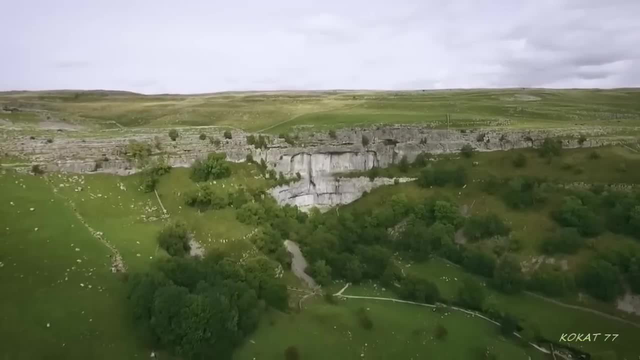 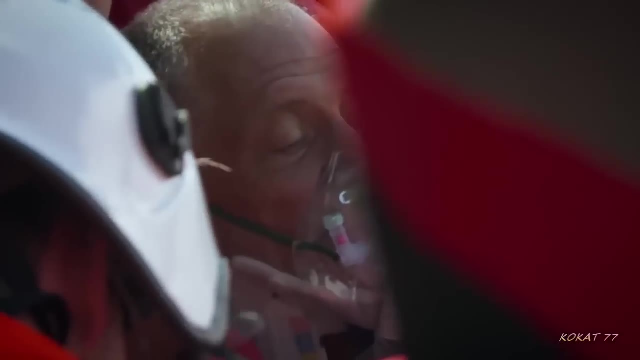 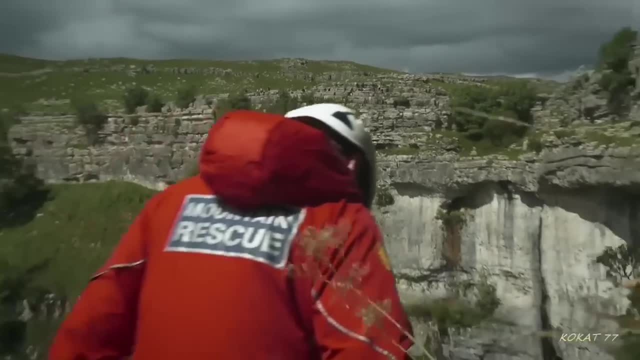 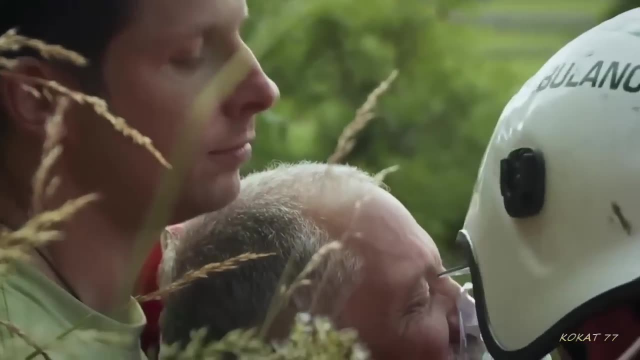 The team's clinging to a steep slope above a 200-foot drop. We're going to get the Coast Guard aircraft to come and winch you, so we do need to try and get you as comfortable as we can. Right, I'm just going to use my hands a minute. 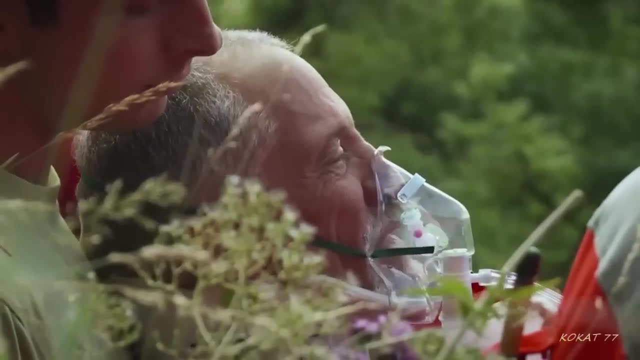 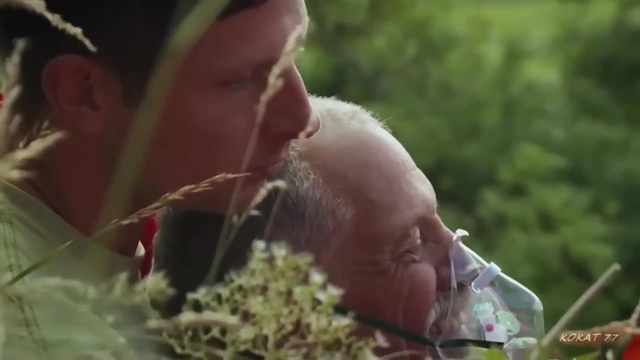 My back is really starting to um go into spasm, Right, OK. Climber Rod's pain is getting worse. He has powerful arms and his fitness is making it hard for Paul to get a cannula into his veins. Come on, this is ridiculous. 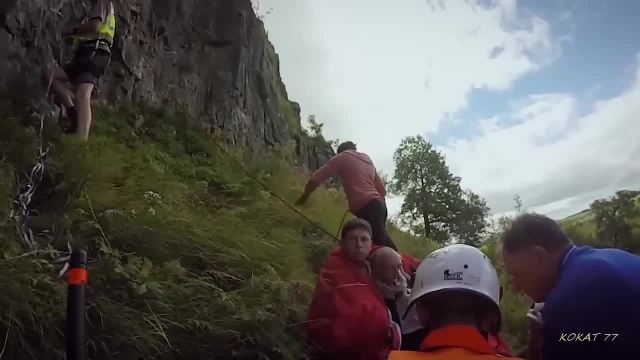 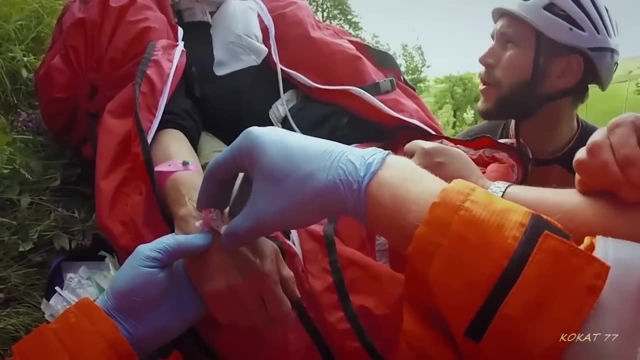 Without a needle, they won't be able to give Rod the strong painkillers he needs. You've got veins like rhinoceroses. have What happened, Roman? Hey, Rob, you took a fall. You slipped, Yeah, and then you took a fall. 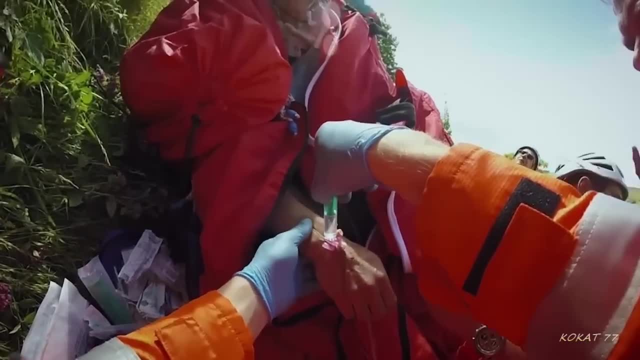 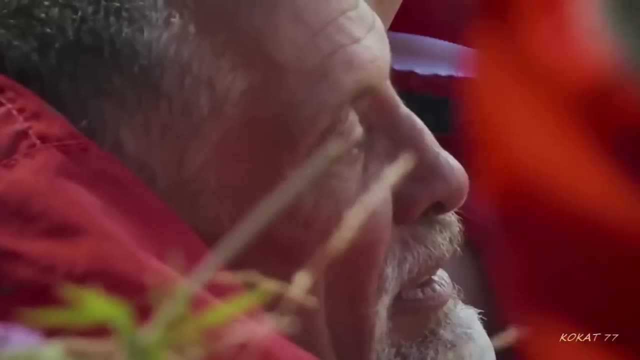 Oh, come on, this is I'm getting frustrated with myself now, Rob, But Paul's forced to give up Right plan B. Rod will have to make do with an oral form of morphine usually given to children Right. open your mouth. 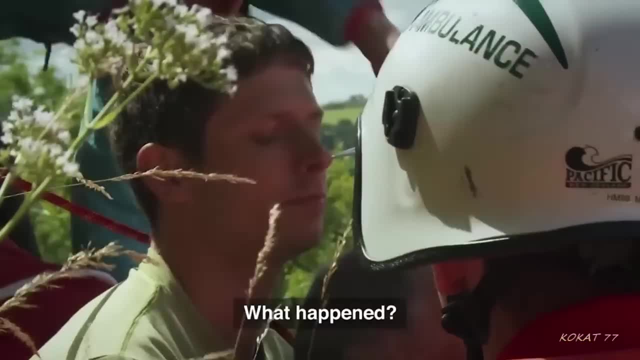 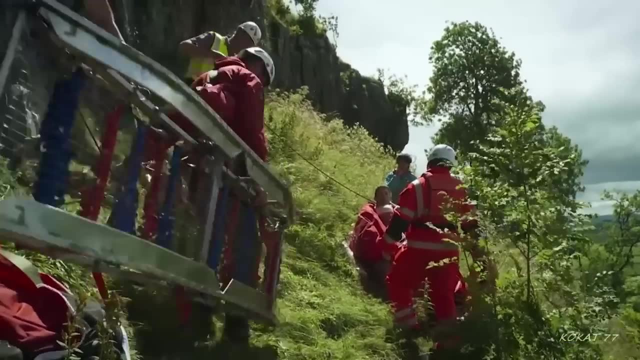 There's concern his condition is deteriorating. What happened? You fell off while you were climbing, Rob. He's repeating himself, and that's often the sign of a serious head injury. He's had a helmet on, so a helmet and still become unconscious. 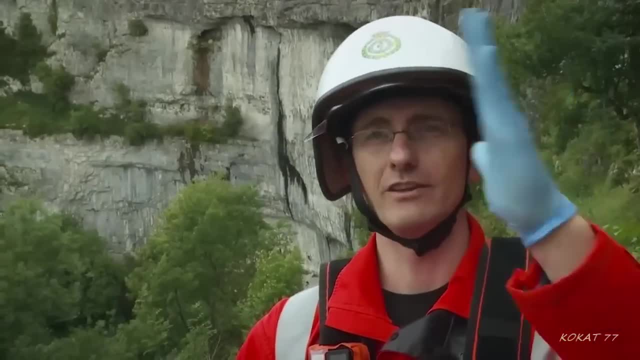 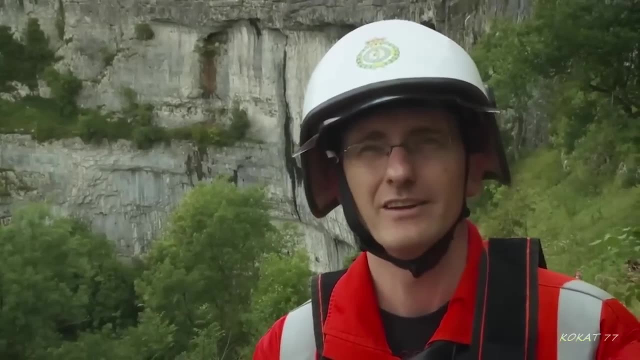 It's quite a blow The way the rope apparently has caused it. it's basically caused him to flip down that way and obviously bang the back of his head, So he's had some jolt on the back of his head. What's the timescale? What's the plan now? 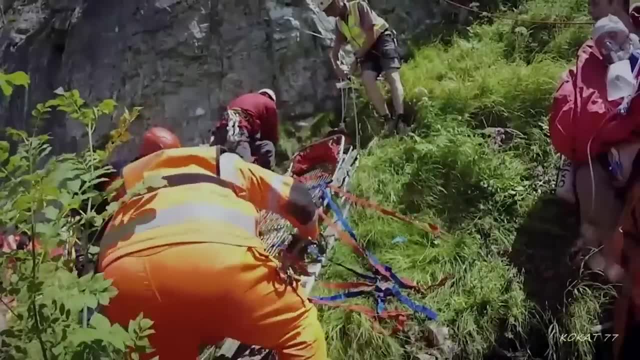 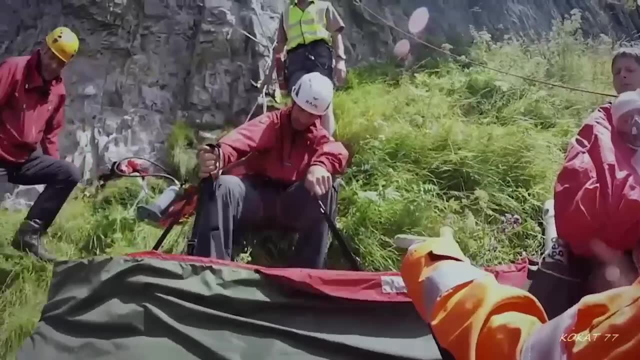 The plan, As you can have a little ride in a helicopter, Vacuum mattress alongside him. We'll transfer him onto that. You happy with that move? Yeah, All right. you need to trust us. Yeah, yeah, All right, We won't drop you, I promise. 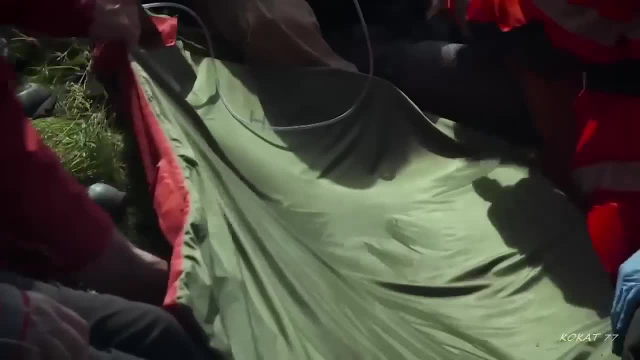 It's a delicate task. so what we're going to do, fella, we're going to swing your legs around, we're going to pivot you on your bottom. All right, You're going to be all right, holding him, supporting him there. 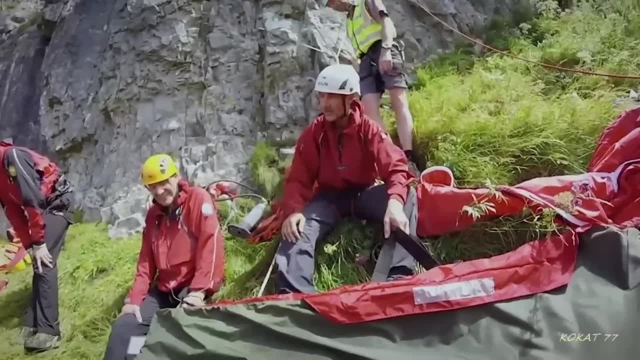 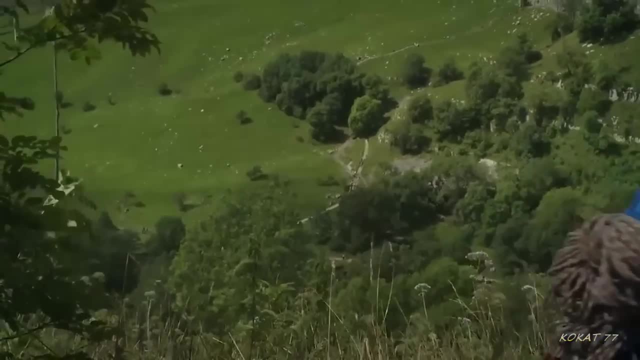 Keep your head nice and still as best you can. You all ready on the vacuum, guys, We're all ready. One wrong move now and a fatal fall could be the result. So we're going to lift your bottom up. Keep his legs up as well. 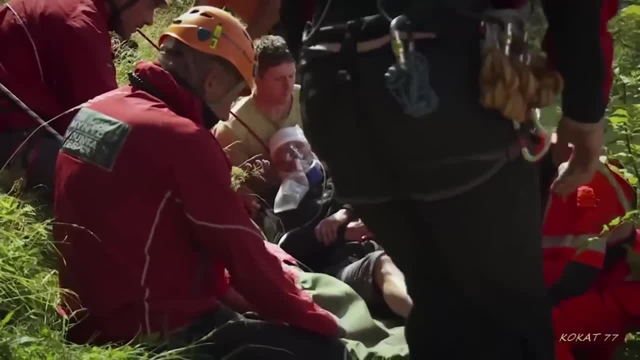 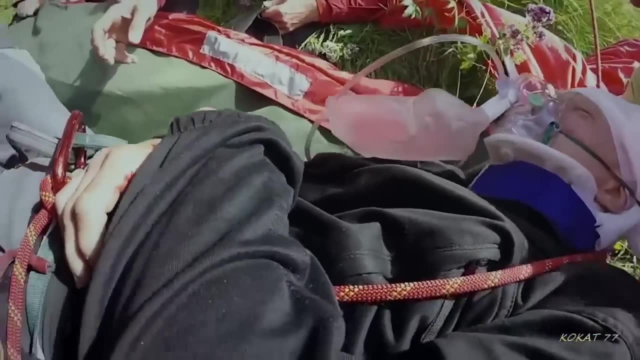 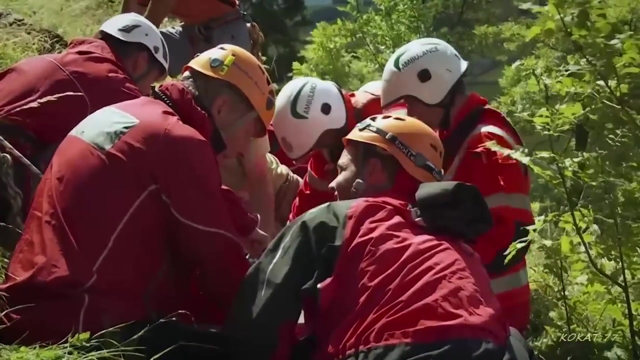 Vacuum mattress. Okay, Okay, Can you slide him down a bit more, mate? Yeah, Where's that Your back? I know, mate, We'll get you sorted. Everybody on the vacuum, ready, Yeah, Ready, Steady. 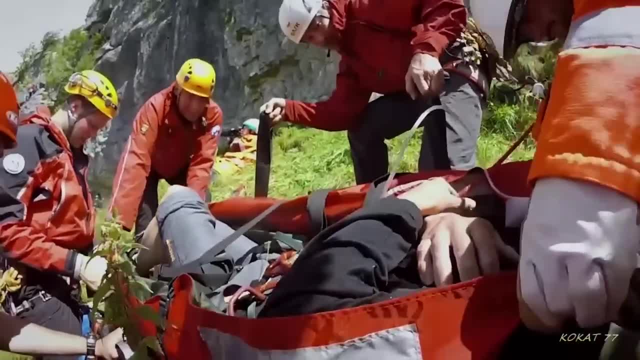 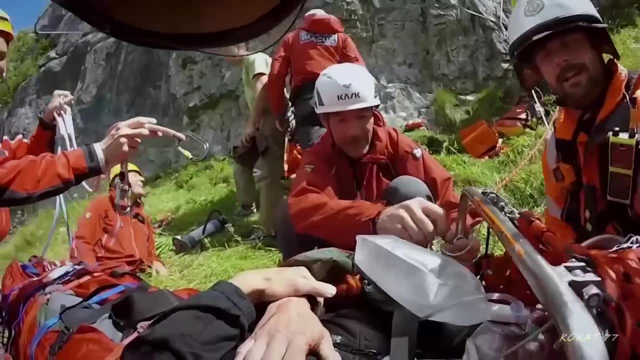 Lift. We're just going to put some air back in there and then we'll mould it round you. It should be a bit more comfortable. Hey, aren't any of this splitting in? Yeah, Yeah, there's a little arm that comes up. 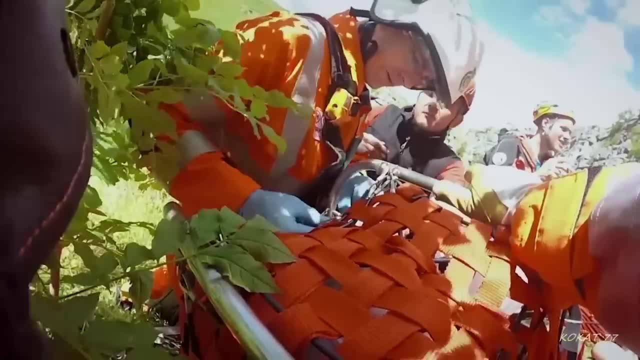 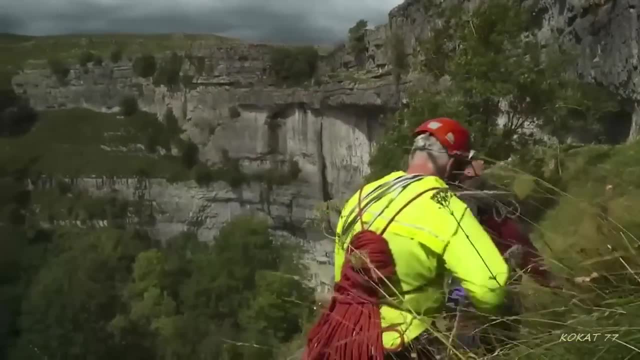 and then just clips onto there just to keep it. Oh, does that go on there? Yeah, It's on there first, is it? Oh, okay, yeah, The team's going to evacuate the cliff face for the Coast Guard chopper. 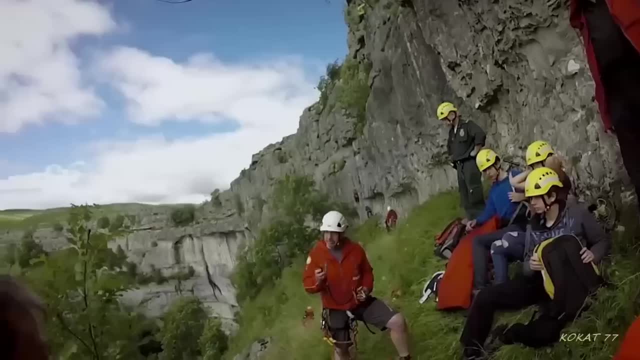 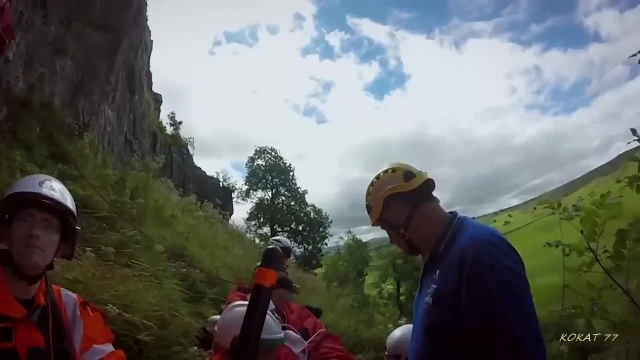 that's been called in from its base 60 miles away. We need everybody that's not needed on here to go. All right, Thank you. So all these are going down, All these are going yeah, because we need to get rid of all this kit. 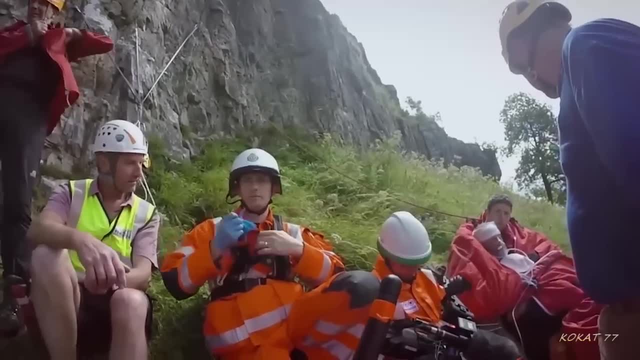 We need to get it all tied down. No, I've not done the job yet with the Coast Guard. Seriously, when it comes, you'll have to put your visor down and everything. It'll blind you and it's just deafening. 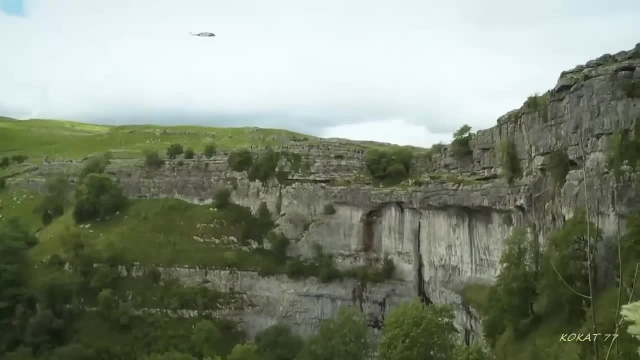 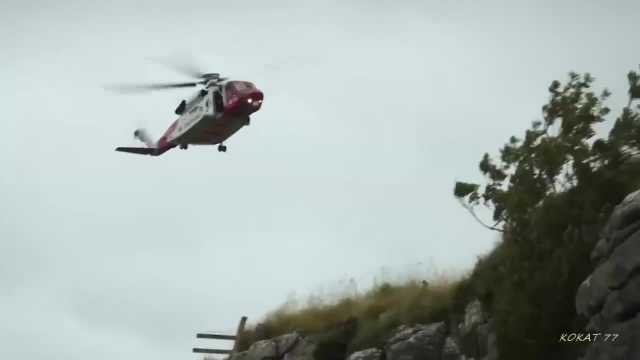 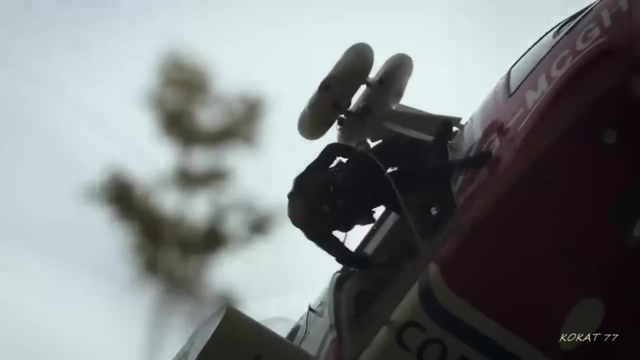 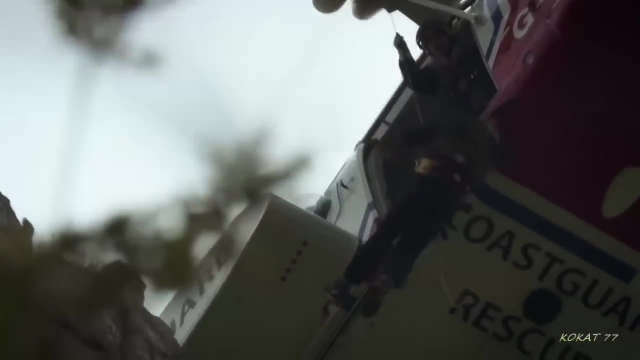 The rescue helicopter weighs 10 tons and is big enough to airlift entire ship's crews. It's downwash is enough to blow a grown man off his feet. Malham Cove's a major tourist attraction and Rod's rescue is being watched by hundreds of visitors. 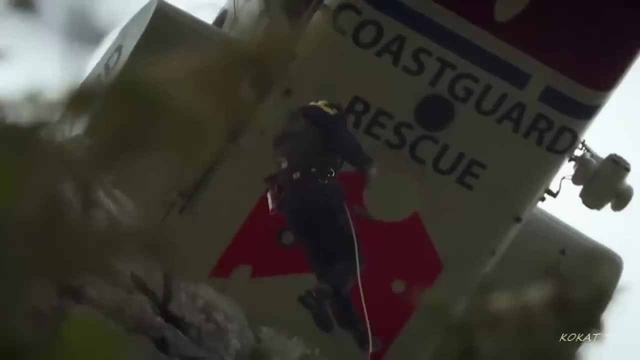 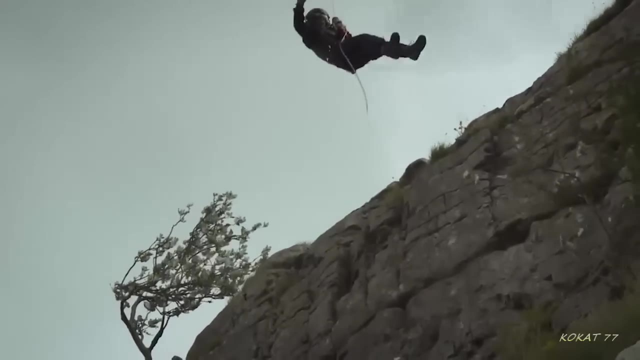 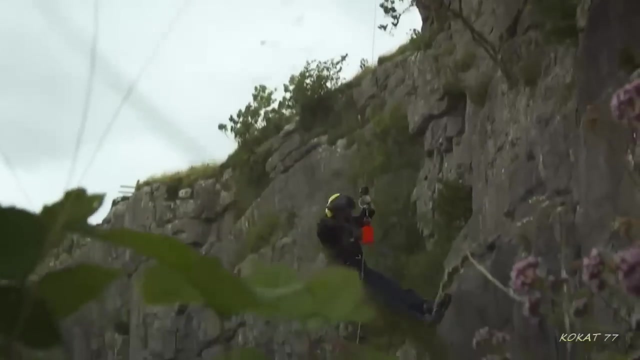 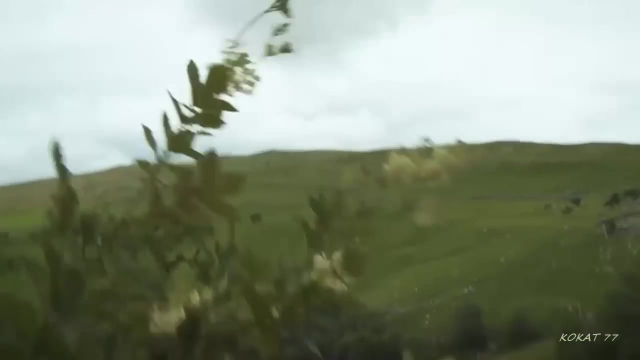 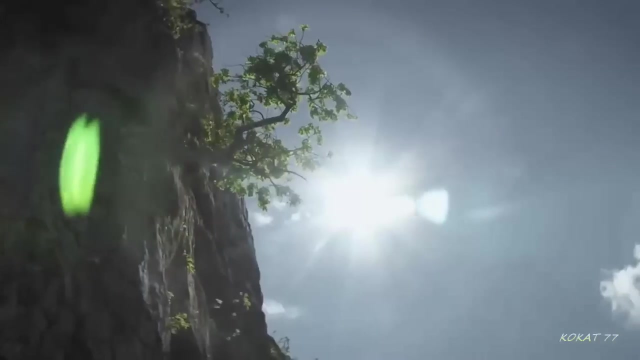 It's a great place. The winchman's aiming for a ledge barely three feet across, But thanks to the skill of the Coast Guard crew, Rod's rescuer is now by his side, James pause, Paul patient. Basically, it's fallen from that ledge just below that tree. 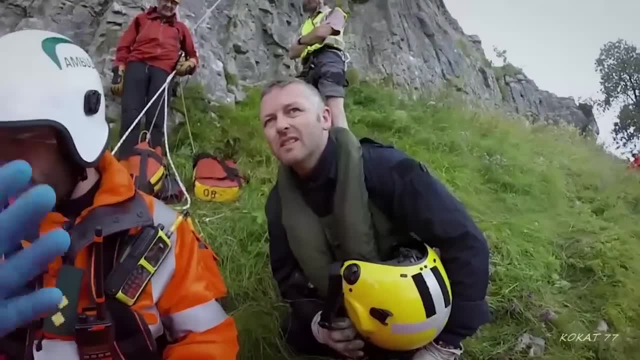 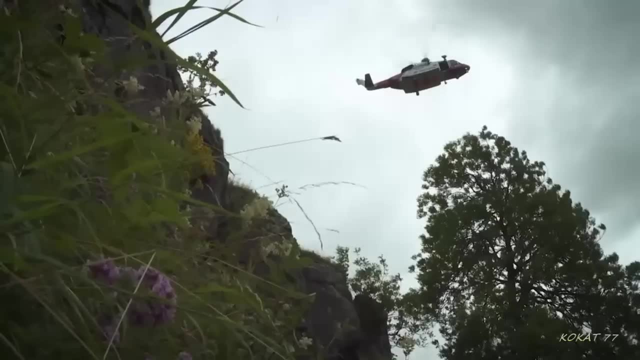 Fell backwards, got a head lack on his left-hand side. It stopped bleeding but it was immediate LOC for about five to ten minutes, Very repetitive post-incident. The plan is to pluck Rod's stretcher from the rock face and winch him directly up. 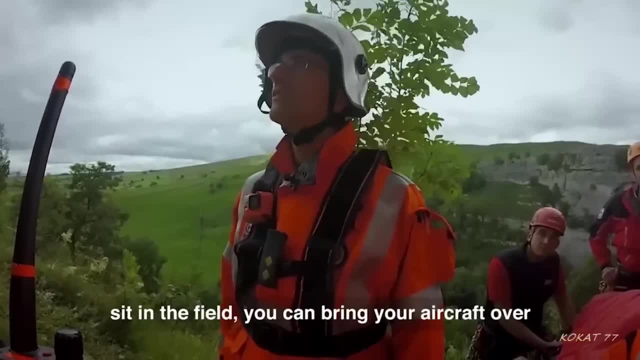 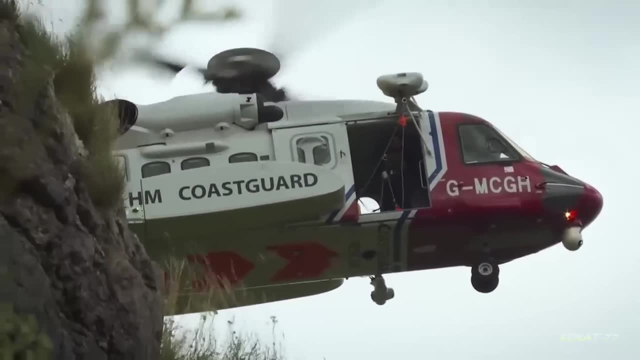 Well, what we're going to do is: I'll go up to the casualty, up to the top, sit in the field. You can bring your aircraft back in, OK, But the cove generates unpredictable turbulence and updrafts and it will be a difficult, dangerous operation. 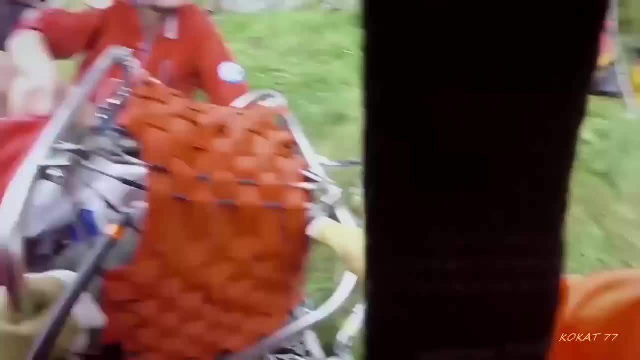 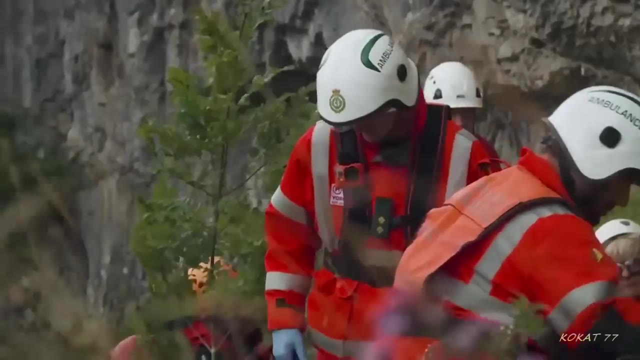 Rob, We're just going to take this sleeping bag off you now. It's going to get really drafty. The winchman's going to be with you all the time. We're going to see you on top, all right, It's time for the medics to leave the danger zone. 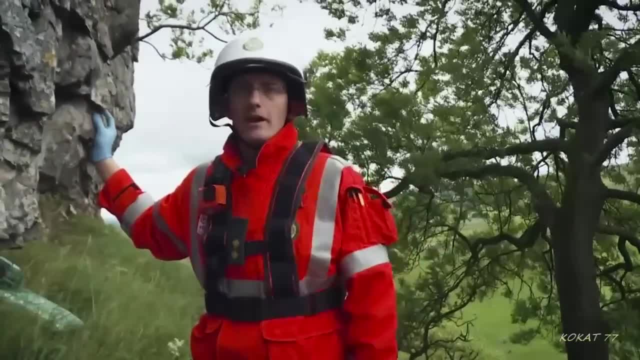 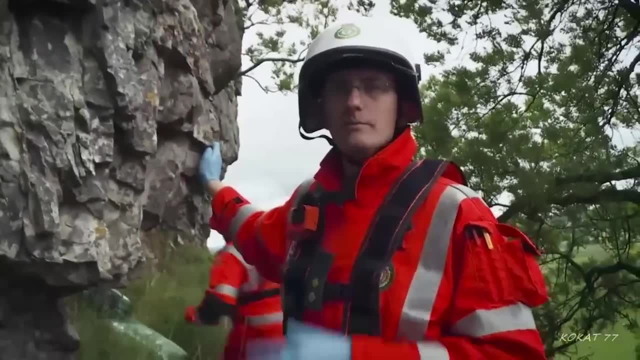 We're going to make our way back up to the top of the, to Mallon Cove. The winchman's down with him at the minute. We're going to be planning to land over. What we're going to do is we're going to meet him back up there. 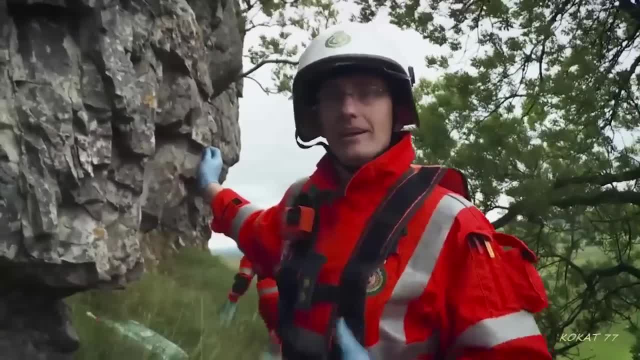 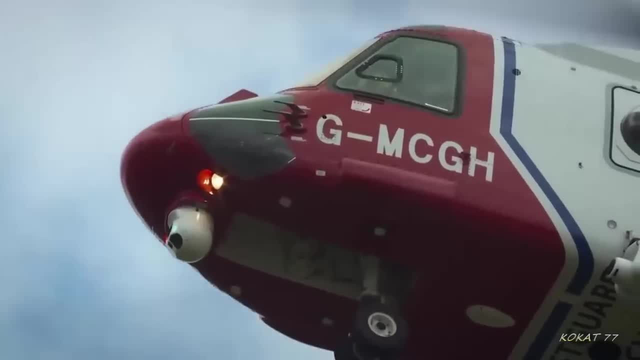 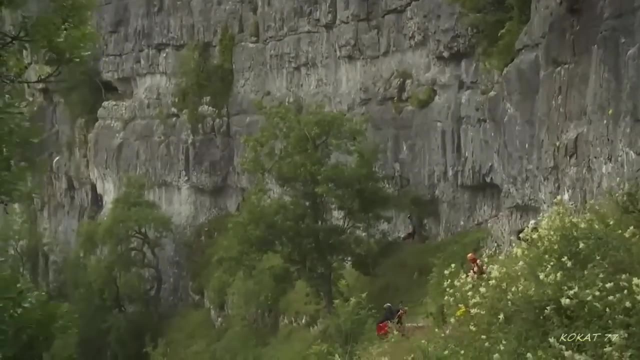 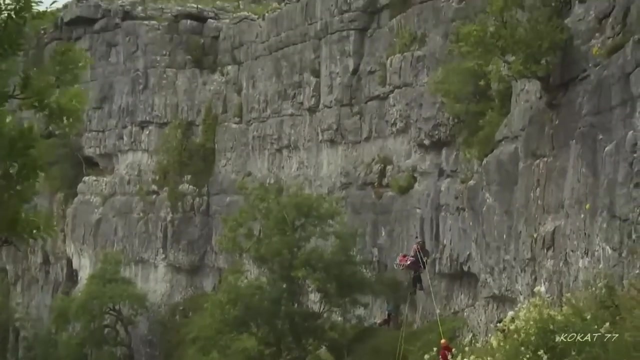 They'll lift the patient up here, We're going to take him back to our aircraft and then we'll take him to World Euro. All right. Rods dangling from a cable thinner than a man's finger. The stretcher is swinging in space 150 feet above the ground. 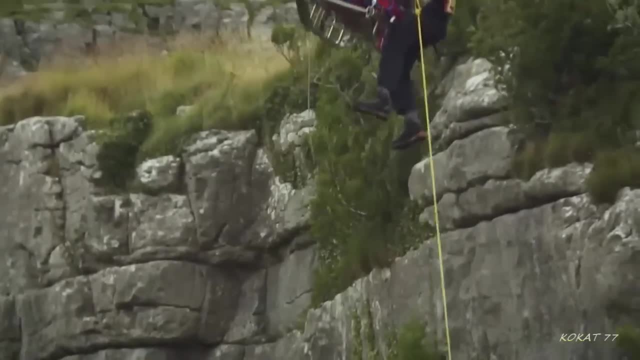 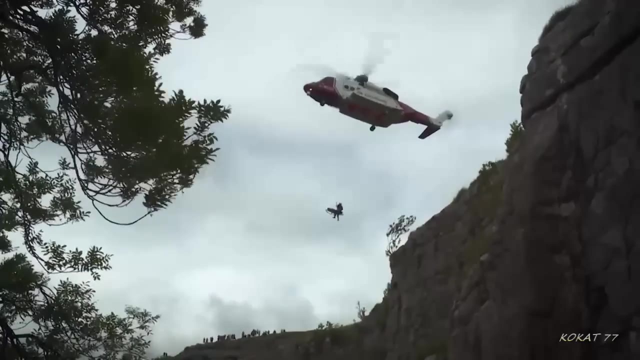 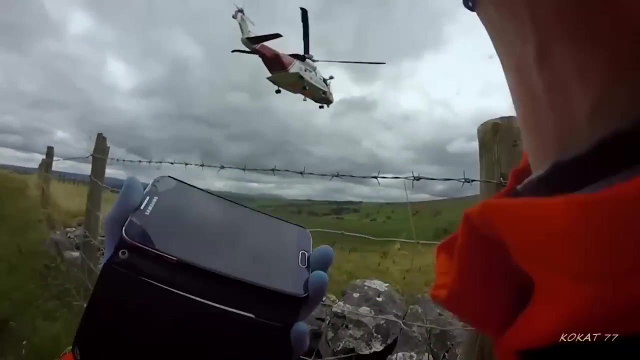 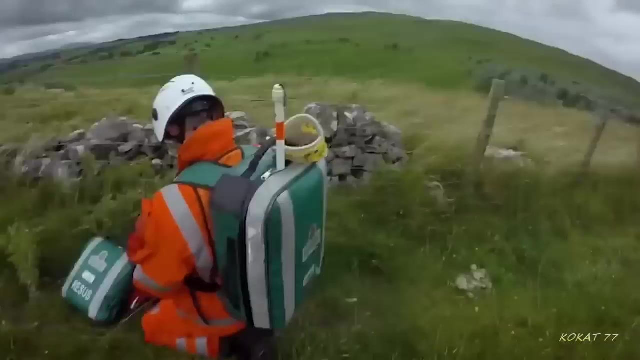 And yards from the sheer bare face of the cliff. This takes supreme skill. Thankfully the Coast Guard team have it. They train to rescue people from ships in raging seas. Paul can't resist a souvenir picture. Paul get it up. 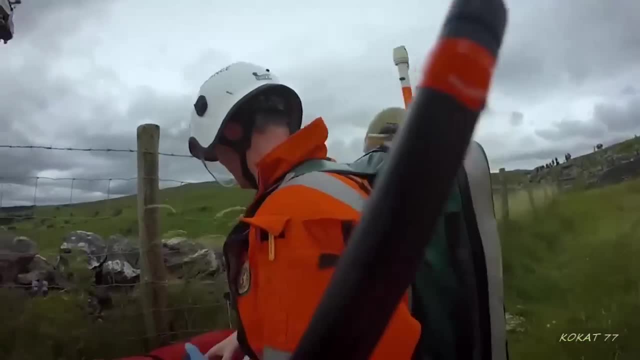 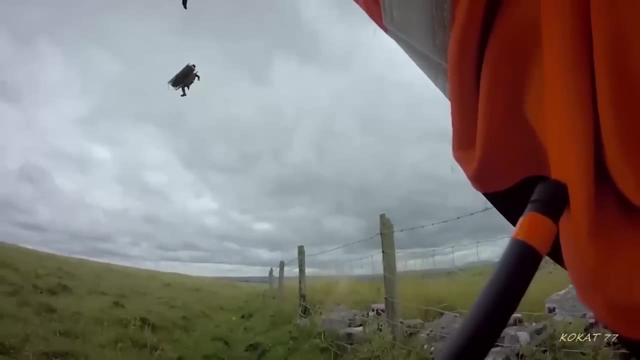 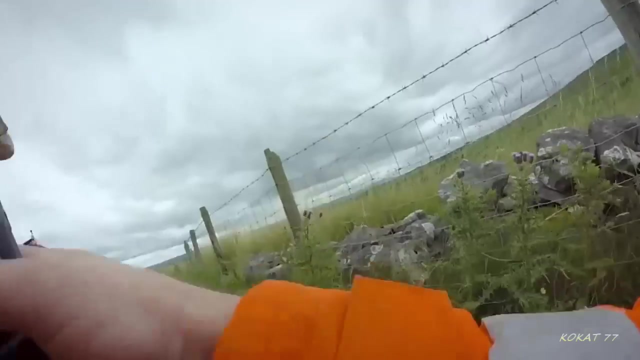 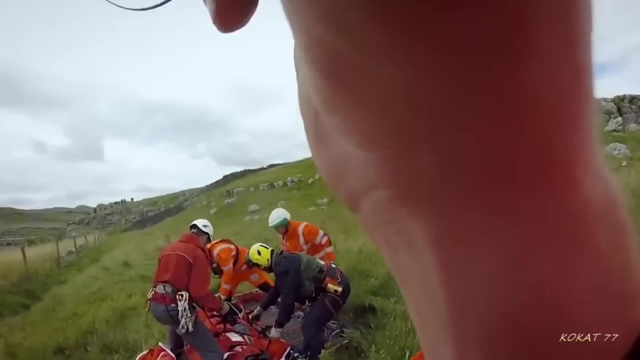 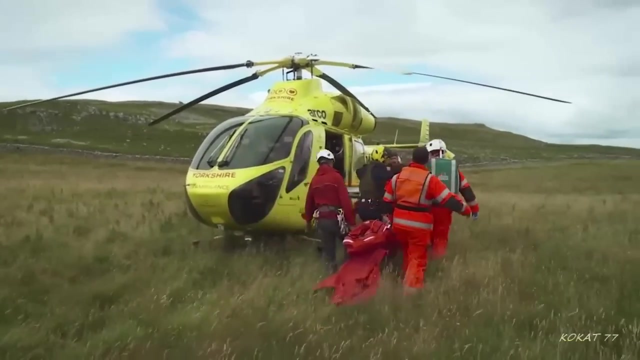 Get it up, Get it up. The expertise of the Coast Guard team is now about to deliver Rod back to safety. There he is: Everybody ready, Ready, steady, lift. Rod has coped well with his hair-raising rescue, But he's becoming subdued and his confusion continues. 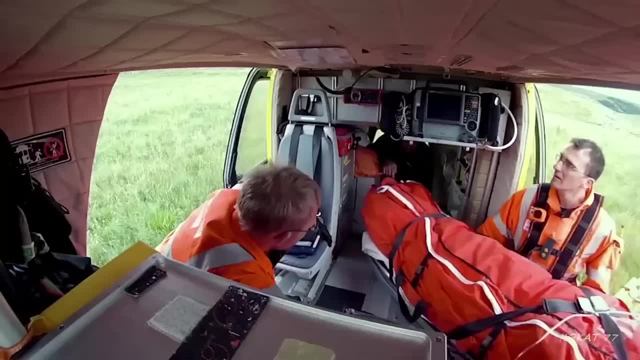 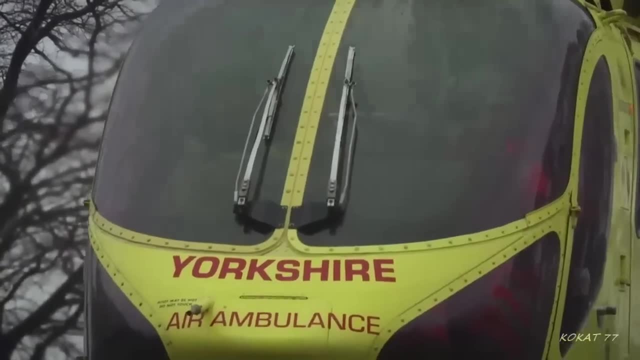 Off that mate. Yeah, we'll put that outside if you're all right with that. Yeah, yeah, It's a worrying situation. It's a worrying sign. Clear And number 560 on the field Rolls. He's being flown to Leeds General Infirmary 30 miles away. 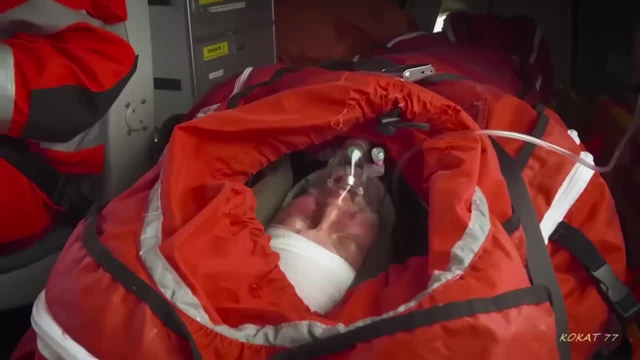 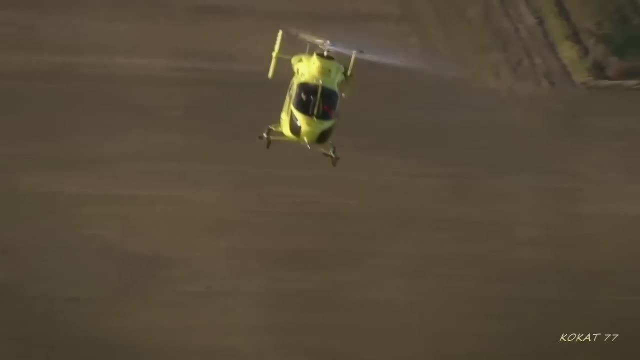 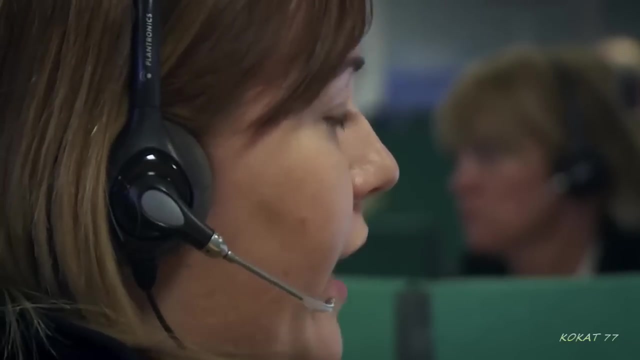 Get us right away, thanks. It's feared he has a serious bleed on the brain. The fall could still leave him with life-changing injuries Or worse. Ambulance is a patient breathing. 999 controllers Must rely on information given on poor phone lines. 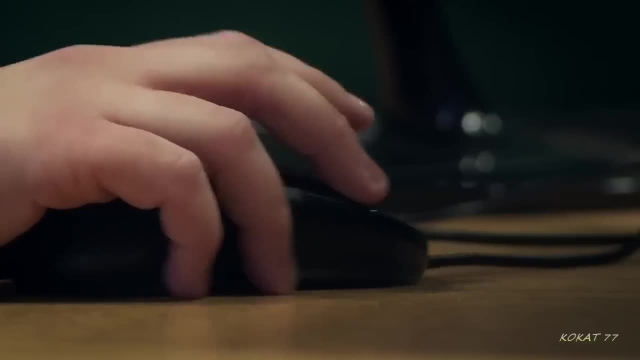 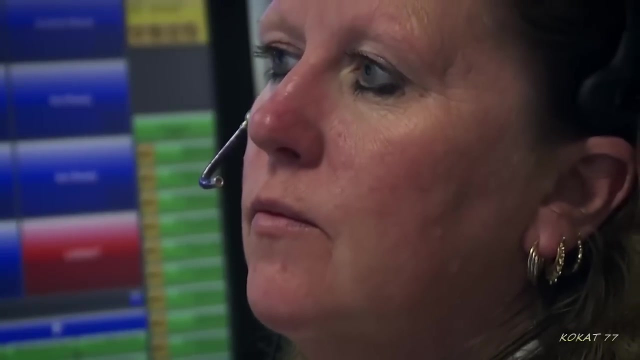 It's a very bad area for signal, so you can't get much out of here From people often in distress. He's just been knocked over by a car And sometimes what sounds like a serious case turns out to be relatively minor. 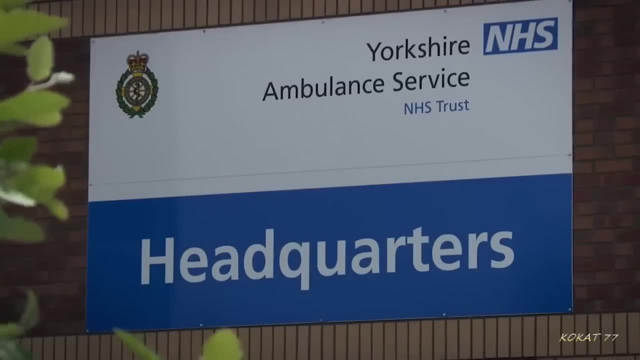 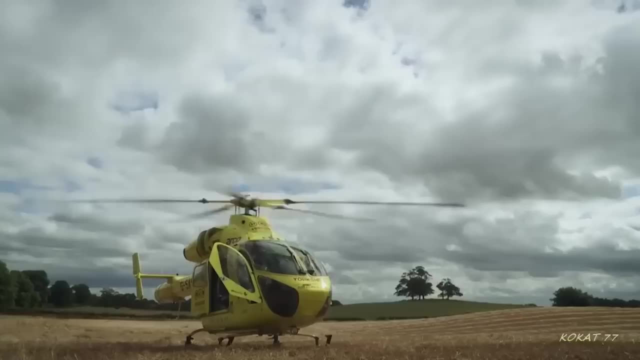 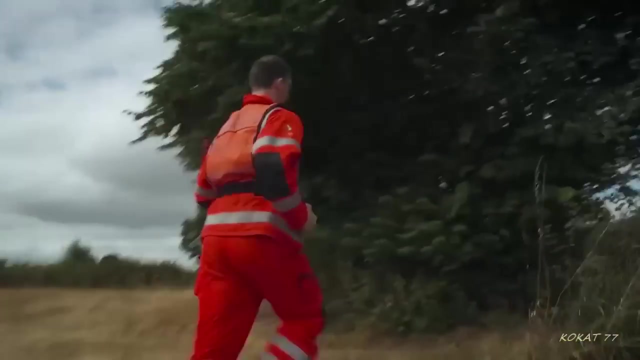 How's her breathing at the moment? Is that still normal? All right, take care, Bye-bye. It's a summer's afternoon in North Yorkshire And a hayfield has become an emergency helipad for two air ambulances responding to a crash on a country lane. 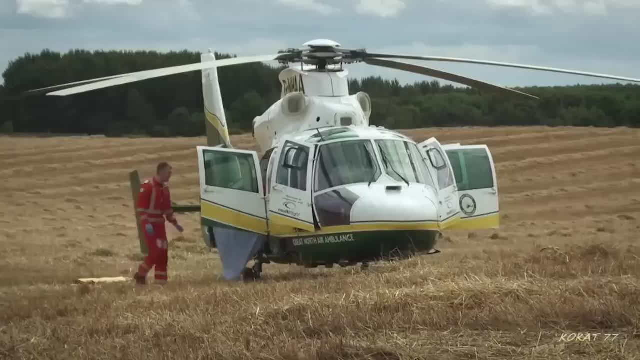 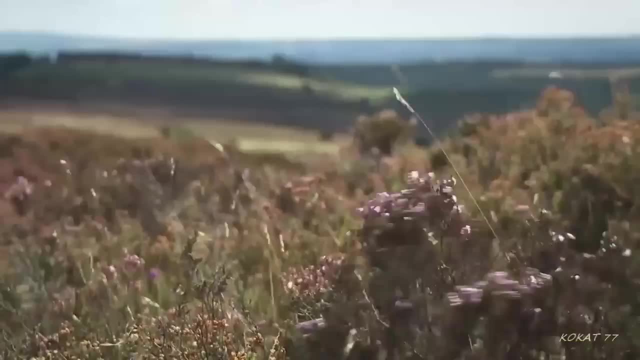 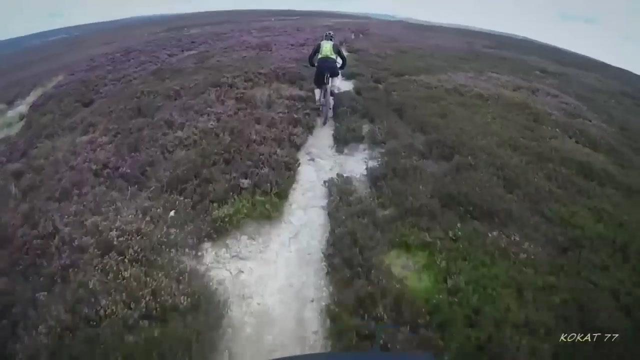 But it's not as serious as it sounded. Helimed 6-3,, the neighbouring Great North Air Ambulance, will carry the patient, But 15 miles away, in the purple heather of the North York moors, another man is about to be in greater need of an air ambulance. 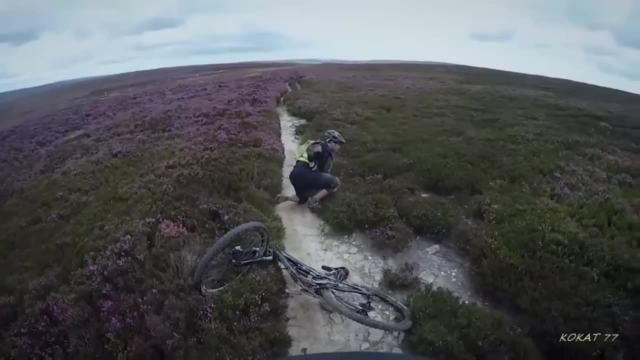 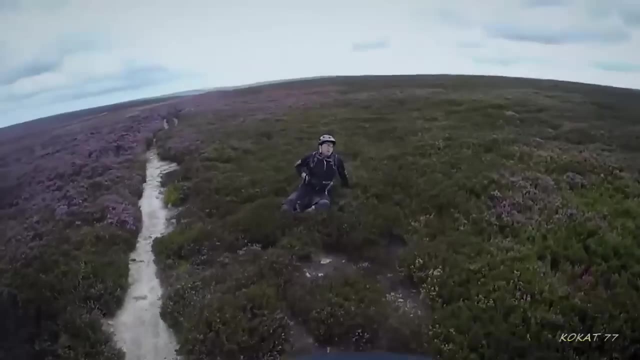 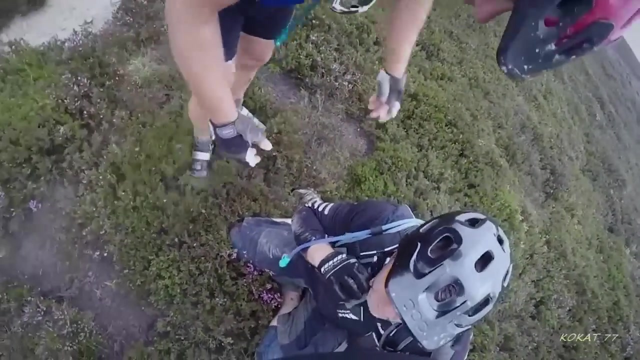 The accident didn't look too serious, But Sean Farrar landed on a boulder. He's in agony and finding it hard to breathe. Keep, still, keep, still, keep, still. His mates are dialling 999.. He's landing right on that rock. 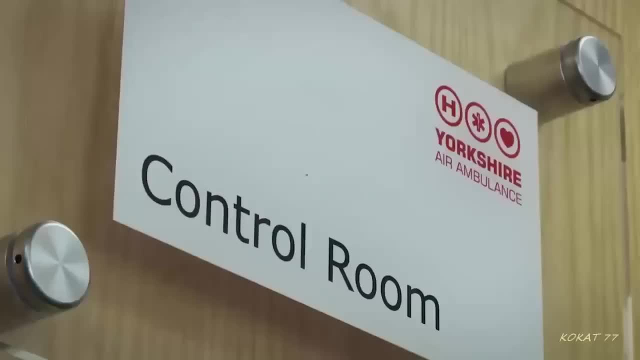 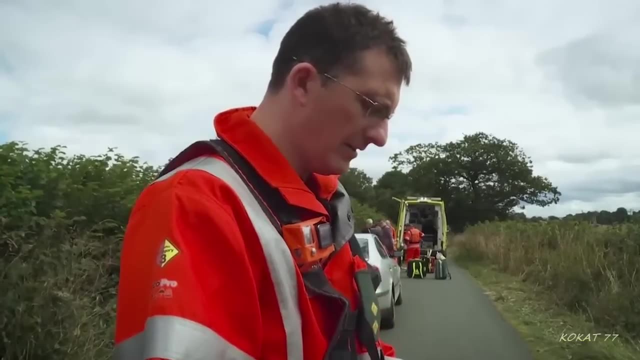 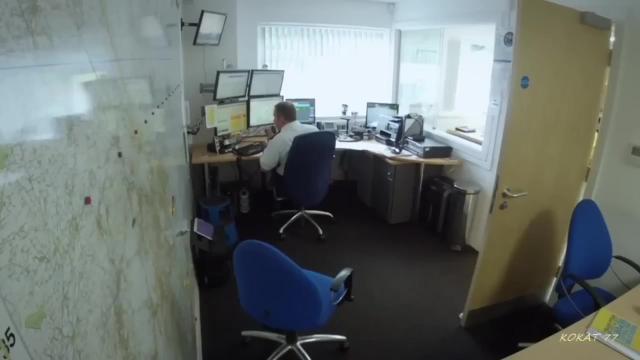 Paramedics Tony and Paul are being diverted. I've got another job coming in at the moment over at Gofland up on the moors And it's someone come off a mountain bike, Difficulty breathing And a note's just gone on. they will not get an ambulance to where he is. 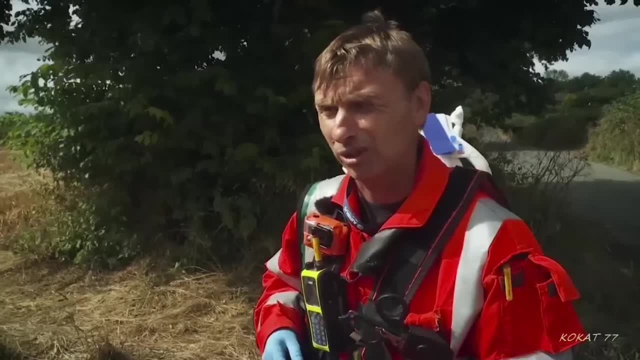 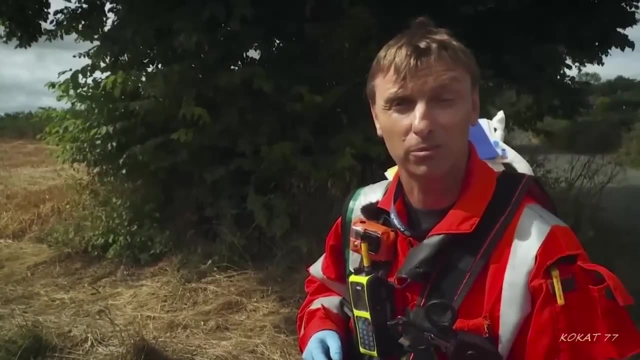 So I will need someone. We've just got another incident given to us on Gofland Moor in North Yorkshire. Apparently somebody's come off a mountain bike, difficulty breathing, possibly a chest injury. So we're just going to get ourselves together now get off to Gofland Moor. 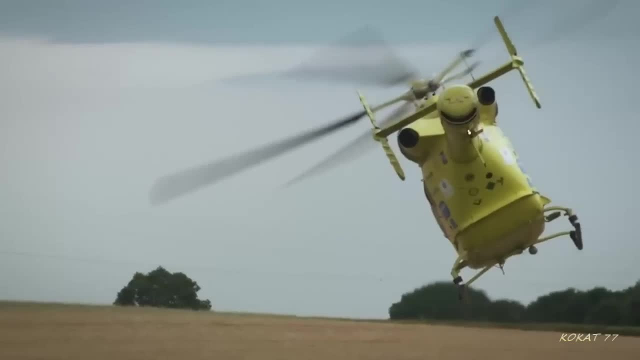 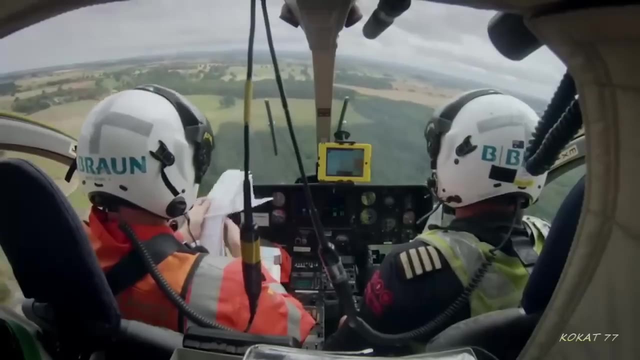 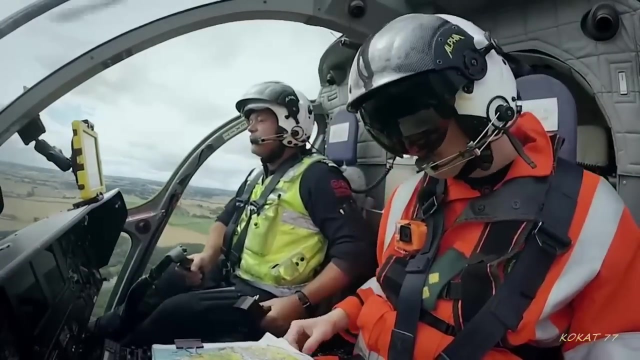 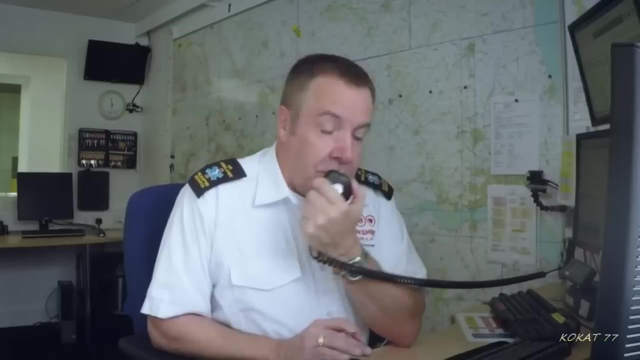 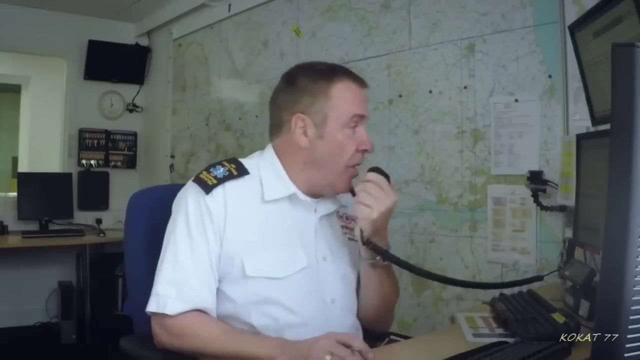 off the moor and leave 6-3 with his patients. I've just spoken to the caller. they've got a good signal up on the top of the moors. The actual grid isn't far out. Sierra Echo 830985, over. 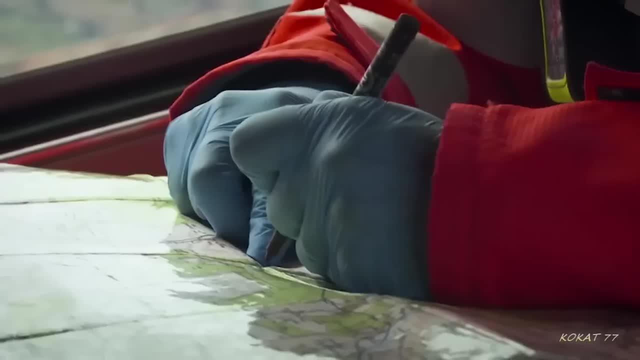 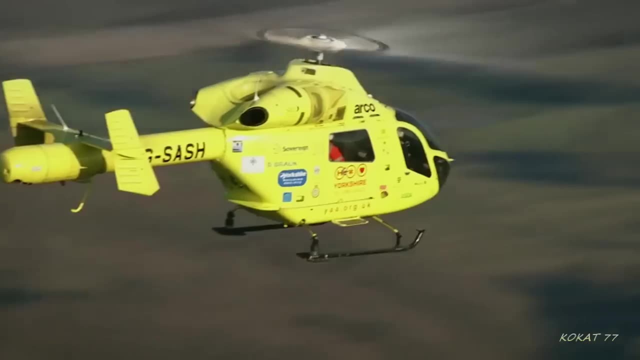 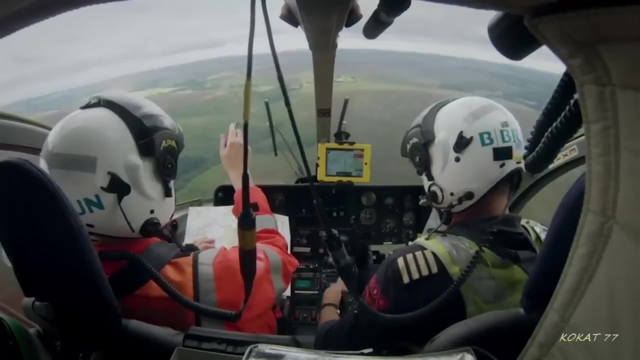 Having a grid reference means the chopper can fly straight to the patient. Finding someone on the vast expanse of the North York moors can be tricky, especially when the heather is out On the nose could be on a track, I'm guessing. 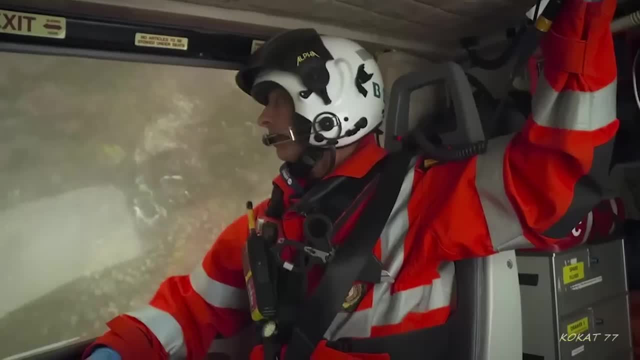 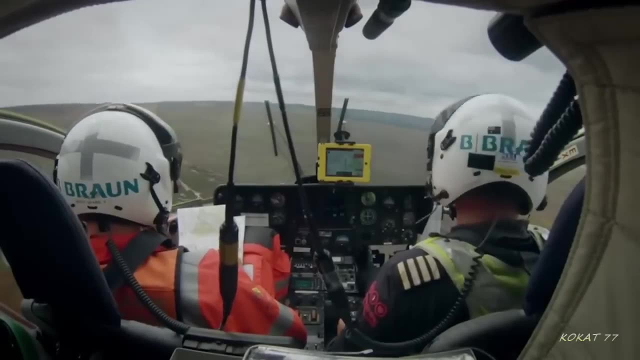 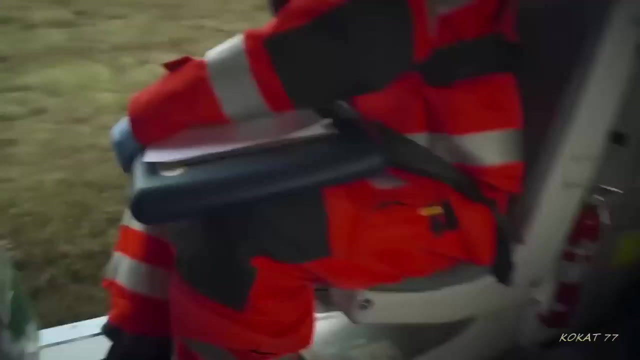 Is that somebody there with red tops? Yep, Addis 99, visual with the patient about to land? Got a little crappie rocks just underneath you, Chris. OK, I'm just looking. It's rough terrain. Tony's helping pilot. Chris land. 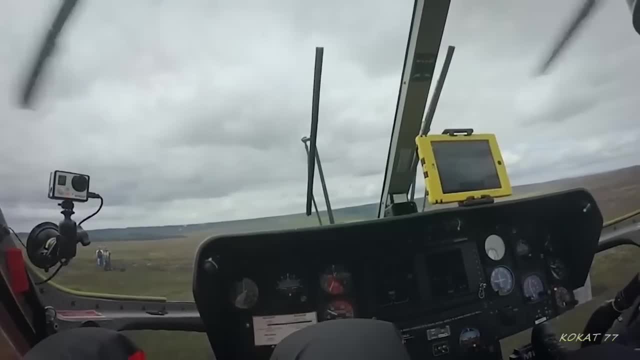 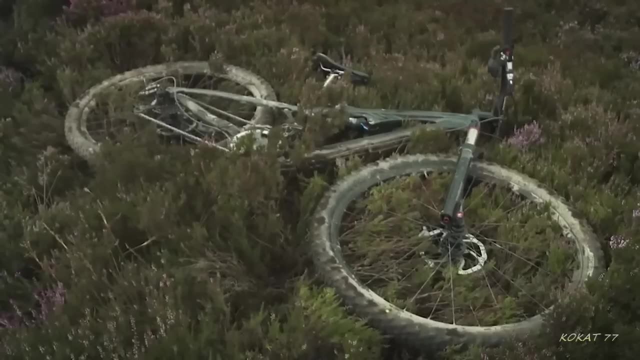 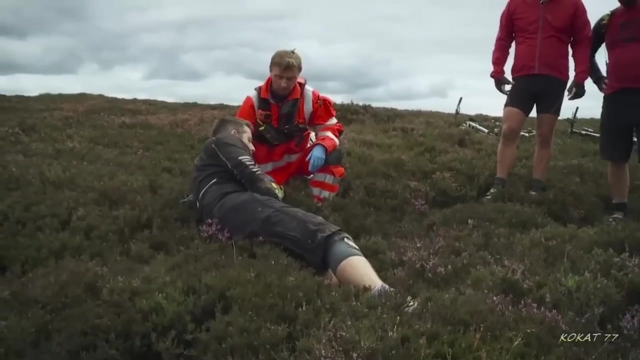 Yeah right, skid's. good Looking there guys. We'll stop here. Sean's still in great pain. He and his mates were on a day out from Leeds. I've landed on that with my ribs, With your ribs. Right on the side there's a hole in his jacket. 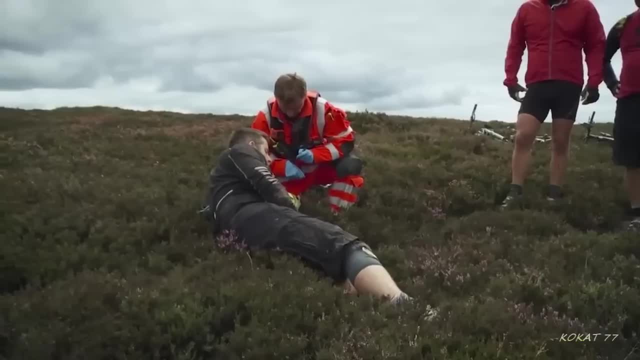 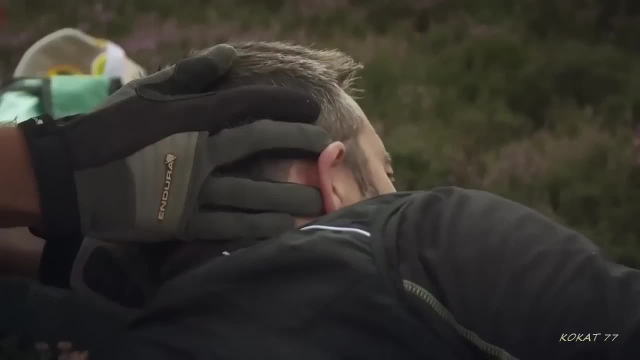 OK, So you've landed on your front. Yeah, OK, Right, so you've come off your handlebars, landed on your front. rock under your right chest. Have you got any pain? I've seen my ribs Right. Any pain anywhere else? 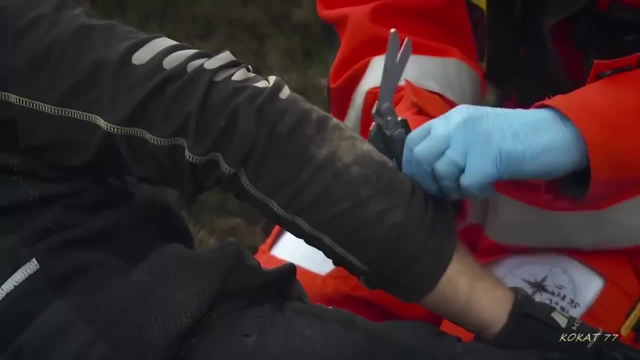 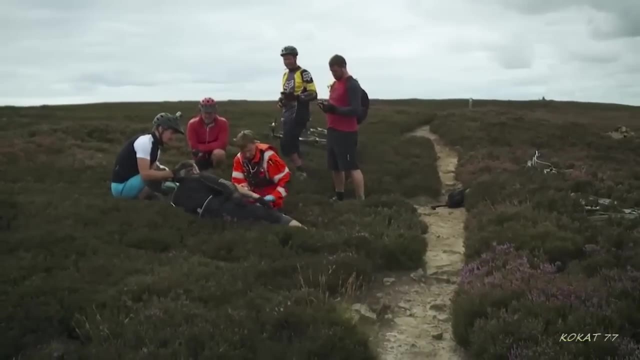 Just breathing. OK, I don't want to cut any more off than I need to do, maybe. No, This one's cut anyway, ain't it? Tony's patient is showing worrying signs of a collapsed lung and it looks like he could be bleeding internally. 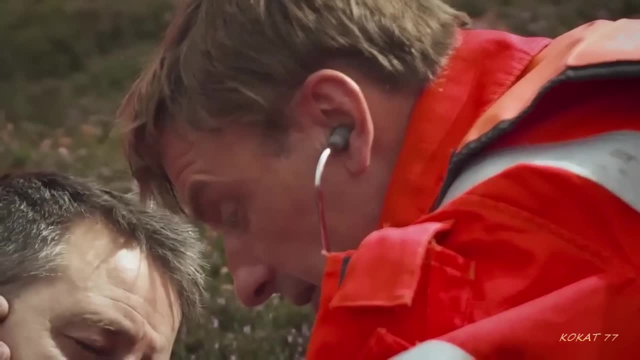 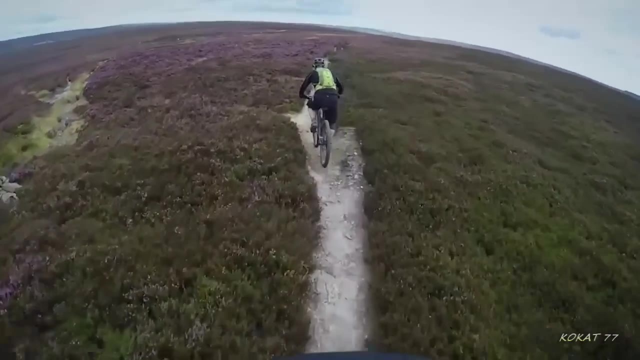 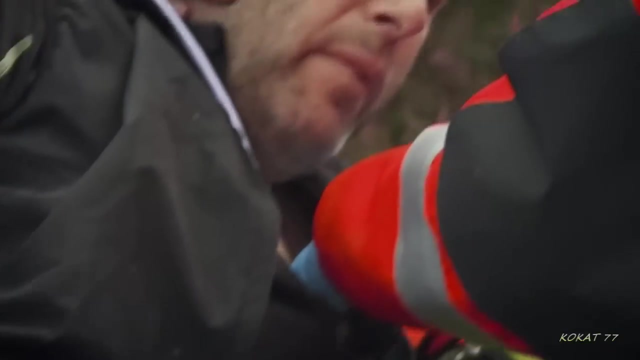 Time is not on his side and the clock is ticking. It's 20 minutes since mountain biker Sean Farrer did this on a moorland track. His mates are surprised by the apparent seriousness of his injuries. He's obviously lost it. He's gone over handlebars. 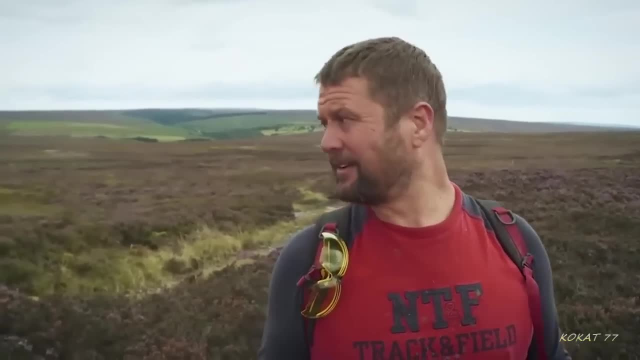 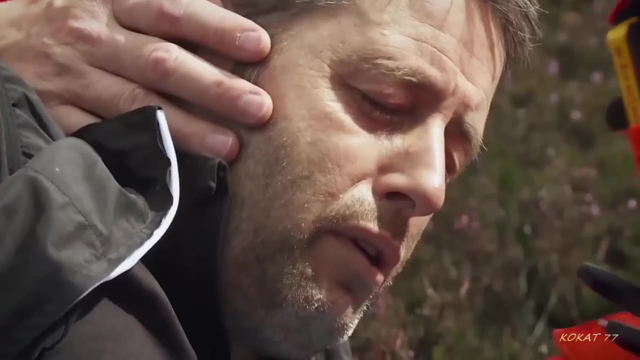 Which wouldn't be a problem, because there's heather everywhere, But he's landed. One of the lads pulled the rock out. He's landed on a big rock on the side of his ribs and he's not done himself any favours really. 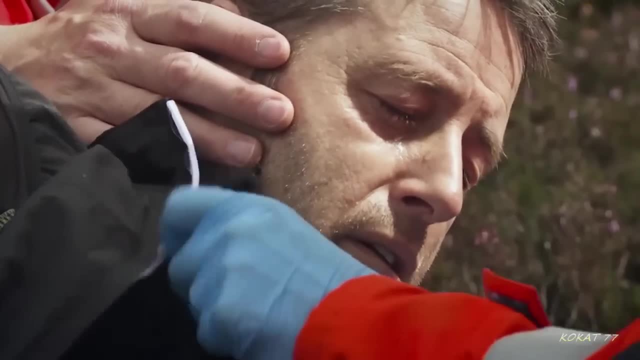 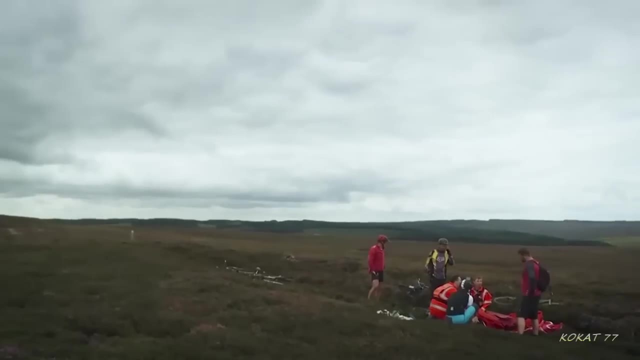 You normally fit him well. Yeah, Got no allergies to anything. No, OK, He's not the first rider to fall victim to the treacherous tracks of the moors today. We set off, we ate First, downhill we hit, went over handlebars and we think he's broken his wrist. 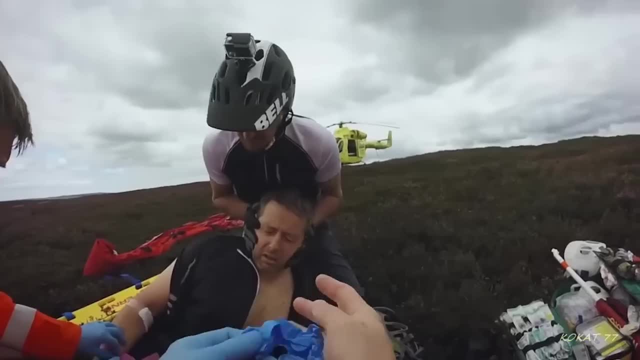 He's sat up now in Levesham waiting for us. OK, mate. And then we've done seven and a half miles and we've lost another one. So I mean, there's still four of us left, isn't there? 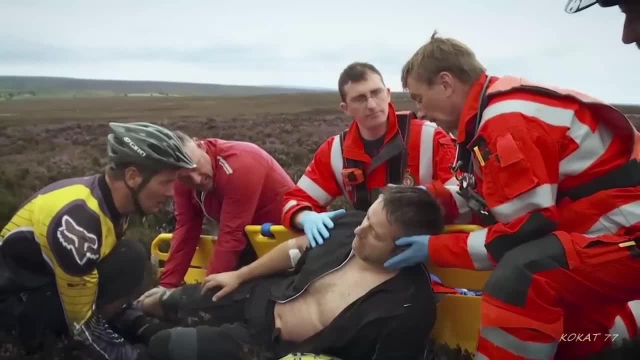 Yeah, still plenty to go at, so I'm sure we'll be all right. OK, Right, buddy, Just relax your back. We're just going to roll you onto your back. Are we all ready, Ready, steady roll. 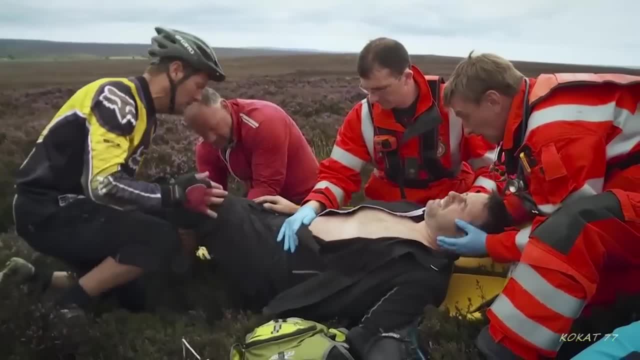 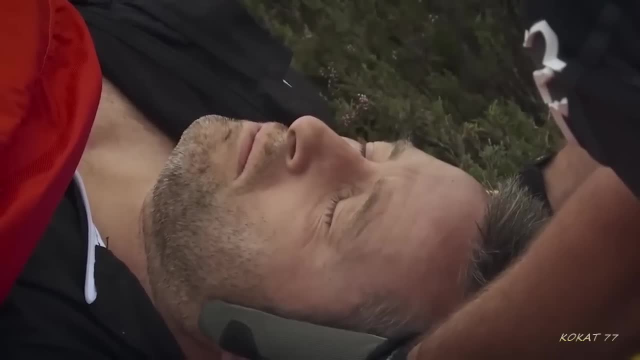 Let yourself come over. The team's taking no chances. They're treating Sean as if he's broken his neck and injured his spine as well as his chest. He's in a bit of discomfort. I'm lying on the rock, So we'll give him a bit of morphine. 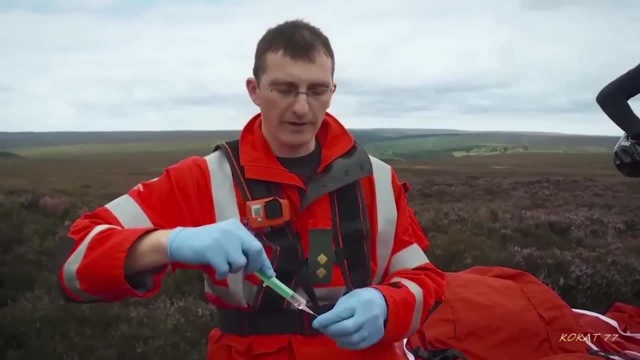 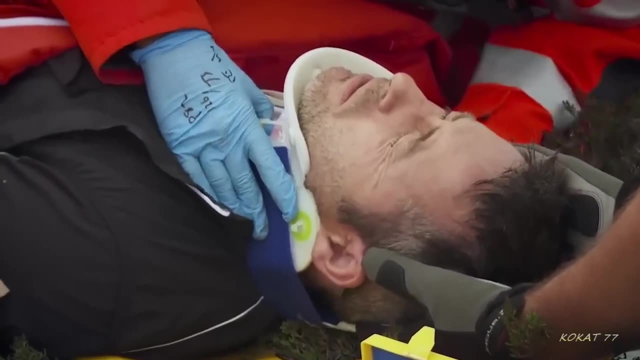 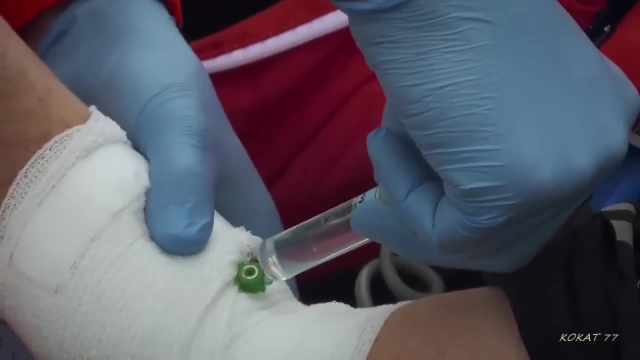 We should take about 15 minutes or so to start having some effect. Sorry, bud, This is going to be uncomfortable. All right, That hurts when I cough. All right, well, don't cough then. All right, Sean. So once you've had this extra bit of morphine, OK, we'll get you fully strapped up. 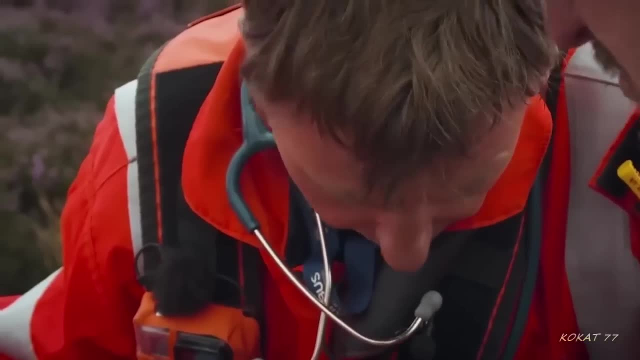 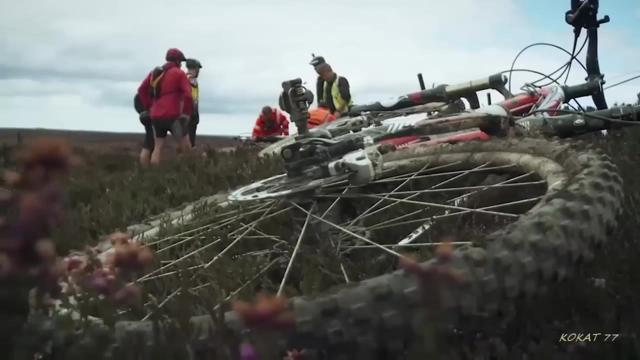 We're going to get you in a sleeping bag properly and then get you onto a helicopter out at cold. All right, All right. Time is of the essence. The sooner Sean is X-rayed and scanned, the better. I'll phone James Cook first. make sure they're happy to take him, and I'm sure they will be. 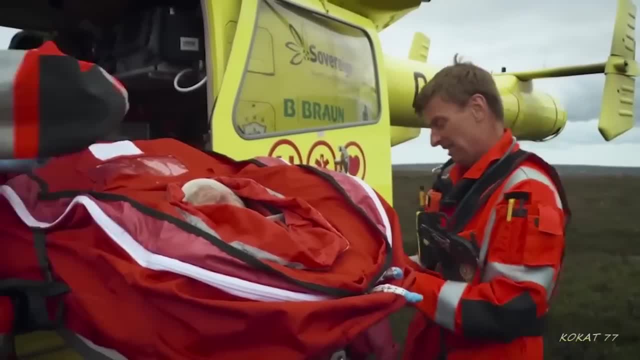 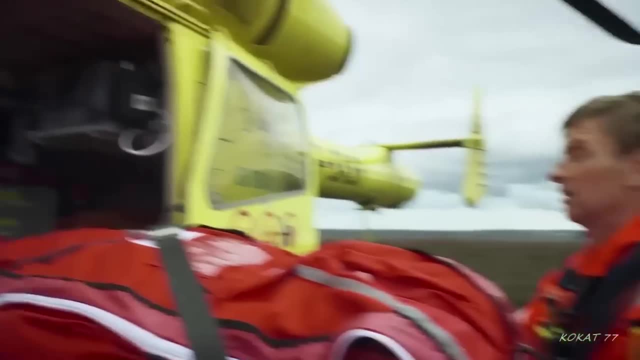 He's going to be flown to the major trauma unit in Middlesbrough, 20 miles away. Just get you on, Sean, Then we'll give you some more morphine mate. We'll get you off to hospital. His mates aren't exactly sympathetic. 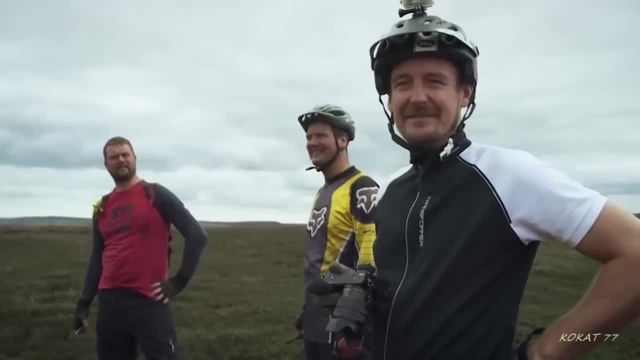 He doesn't have to cart his. That's it. yeah, We've got to cart his bike, haven't we? now, It's It's us that want sympathy. I think isn't it. I think it is Yeah. 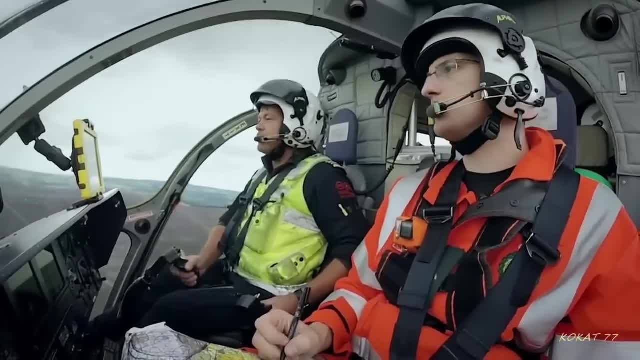 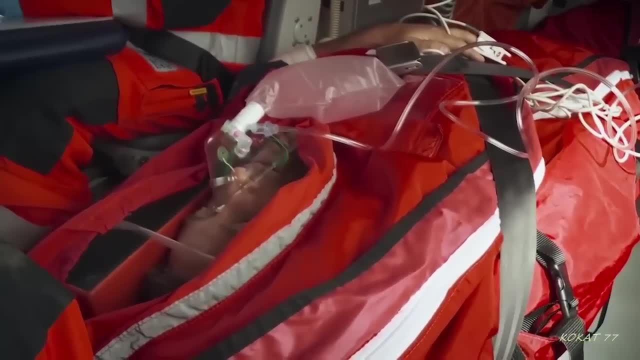 Don't tease Helmet 9-9, Alpha's lifted from near Ghostland On route to James Cook. We'll call again closer in. Paramedic Tony is optimistic. Sean's blood pressure and other vital signs are holding up well, But the impact was very severe and no-one can be sure. 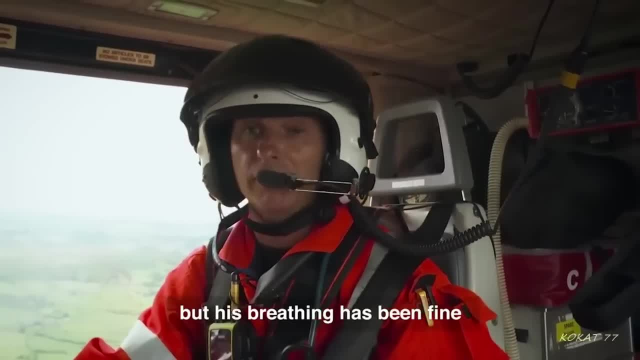 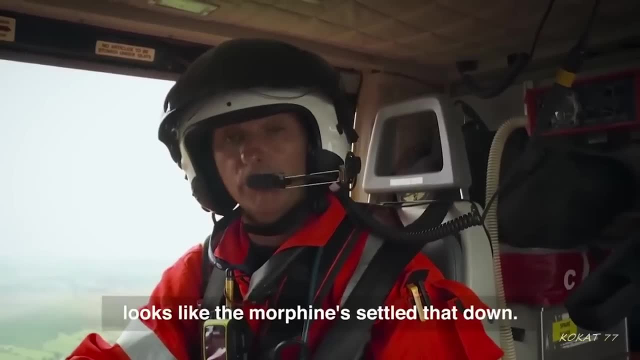 The main concern. in this case It's been fine. All his observations were at normal limits. He's obviously been in quite a bit of pain and discomfort- 7-0-3-1-1-0-2-1.. So fingers crossed he'll be fine. 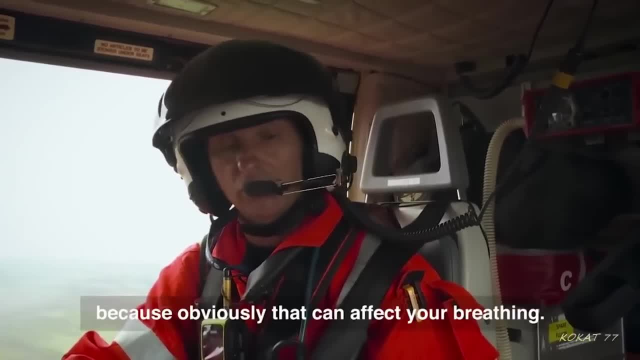 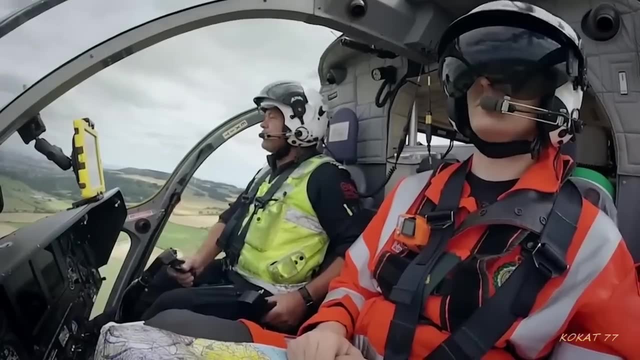 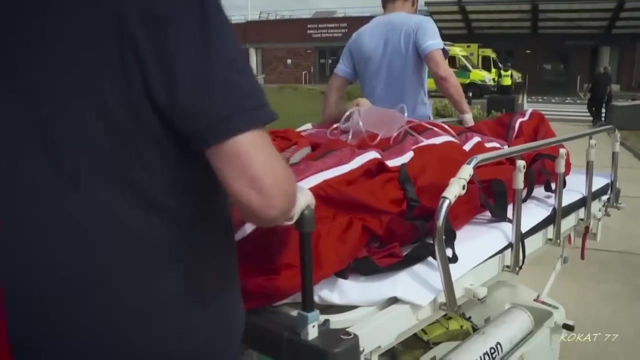 But any chest injury always gets slightly wooded initially, because obviously that can affect your breathing. Don't tease. Helmet 9-9, Alpha, Surely loading down James Cook, We'll call again in a bit Injury-wise. he has got some bruising down his chest wall. 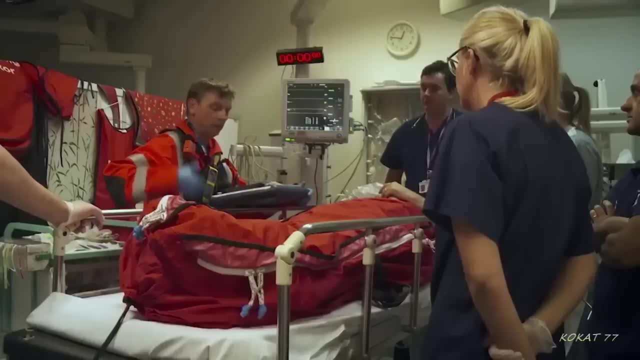 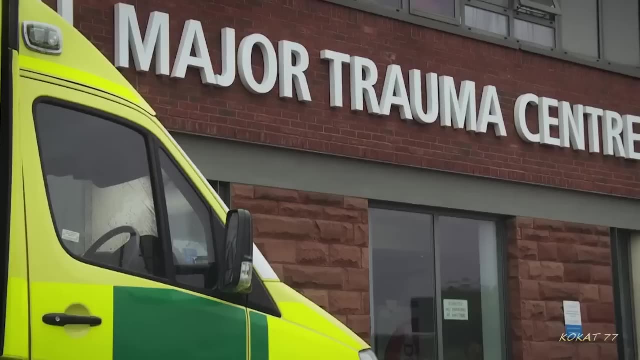 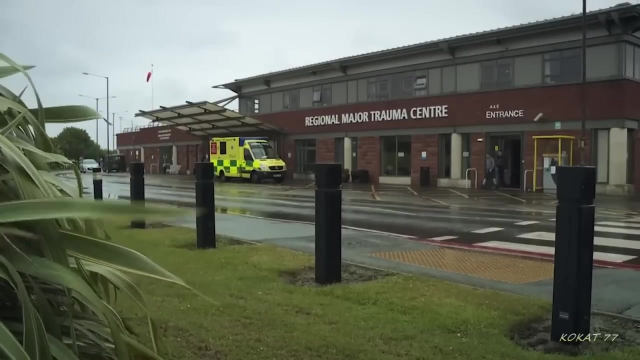 and on his upper abdomen as well. He's got localised pain all round there Clearing right side of chest upper abdomen problems. Sean won't be leaving the James Cook hospital until a battery of tests is completed And the results will prove the team were right. 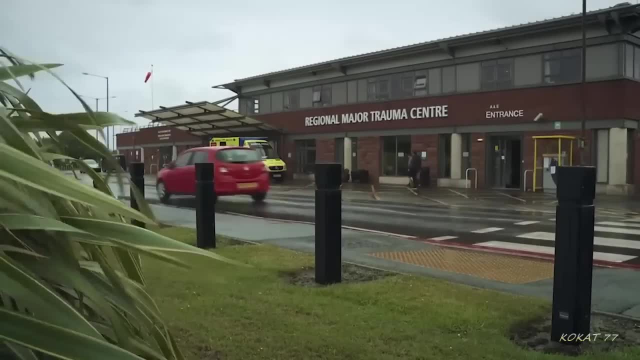 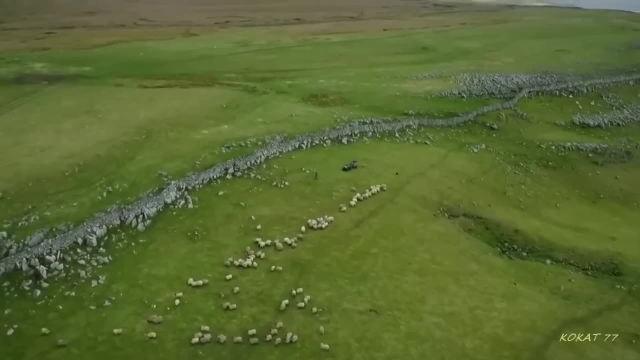 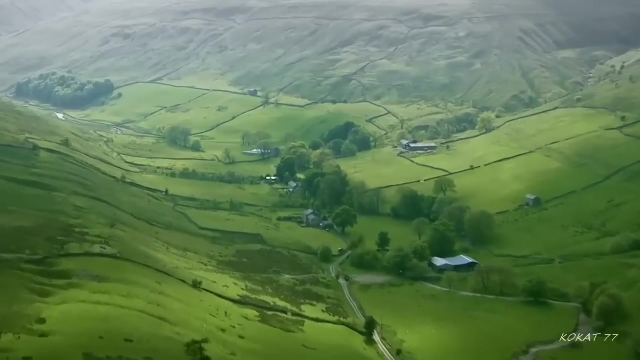 to take every precaution with his care. A critical illness can make Yorkshire's hills a dangerous place to be. High in the Dales above the village of Grasington, a man has collapsed with chest pains. Hiya, it's Pete on Airdess. 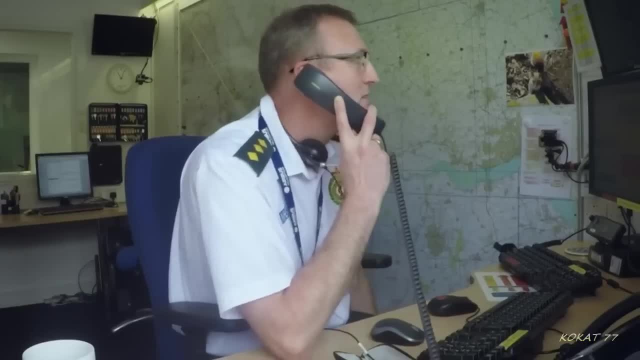 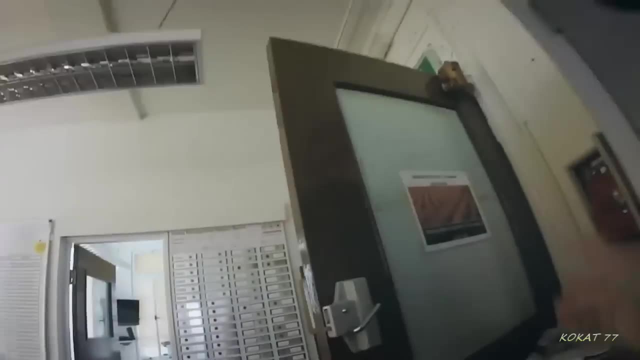 Hiya Dee, They're still trying to track this guy down. It is Grimwith Res. It's a bit sounder. It says it's about four mile away from the path. It's definitely Grimwith Reservoir. Yeah, Helmet 9-9 is being scrambled from its base at Topcliffe. 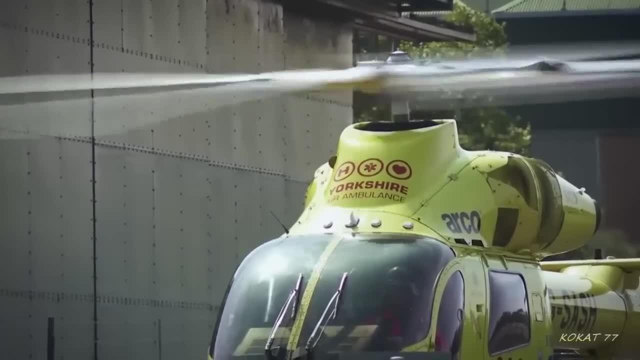 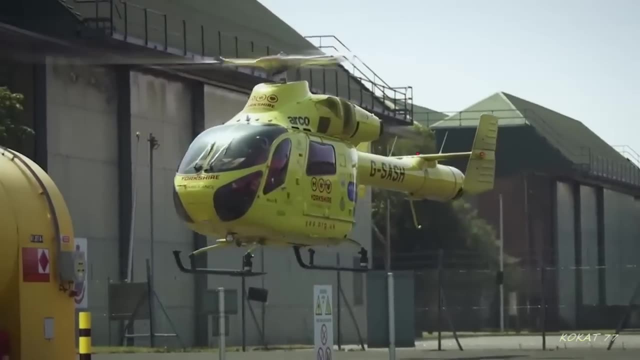 25 miles away. It's the same track as before. Yeah, there's Grimwith, Topcliffe Tower. Helmet: 9-9, alpha lifting. we're calling to the south-west Airdess 9-9, lifting, 11-0-9-0.. 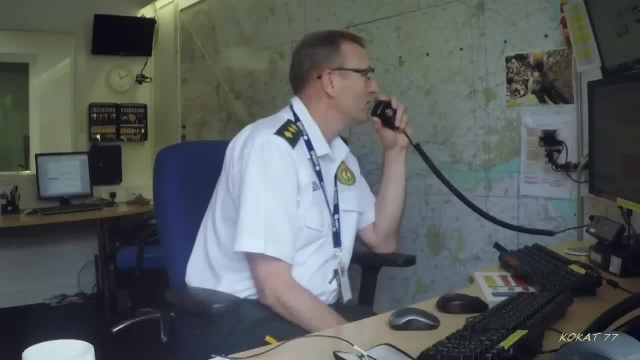 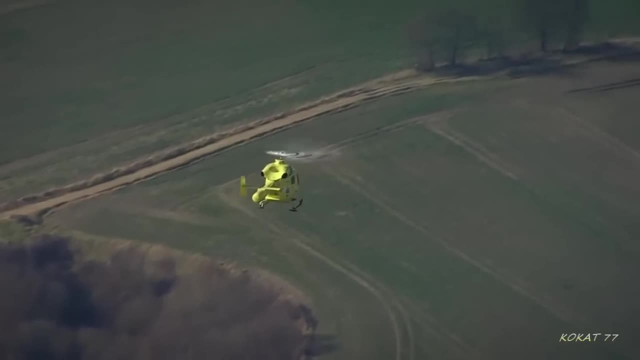 That's received. It does sound like it's more an access issue. Query CVA, Query cardiac cover. It sounds like a walker has had a stroke or heart attack. Paramedic Pete and pilot Steve must find him on the moors below. 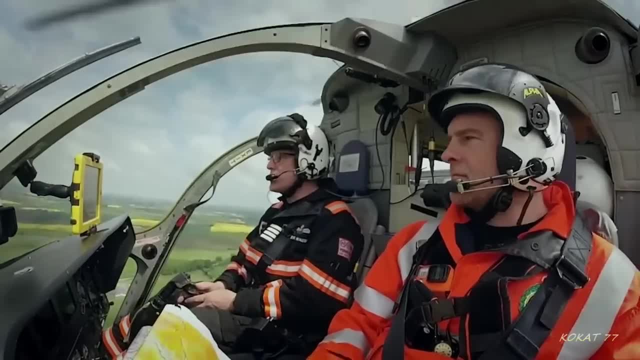 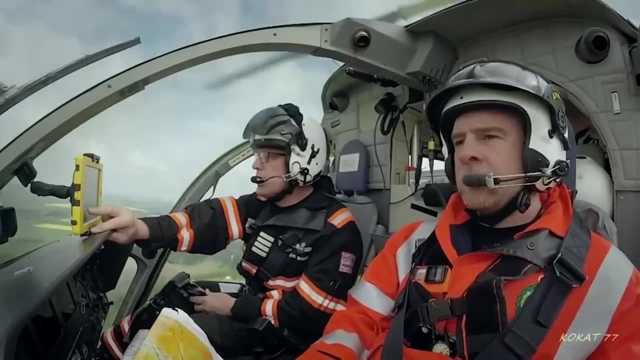 Did he get a rough one, Or is it just Grimwith Reservoir? I've got a grid reference for the reservoir, so it could be anywhere in the vicinity. Oh good, All right, well we know where Grimwith is anyway. 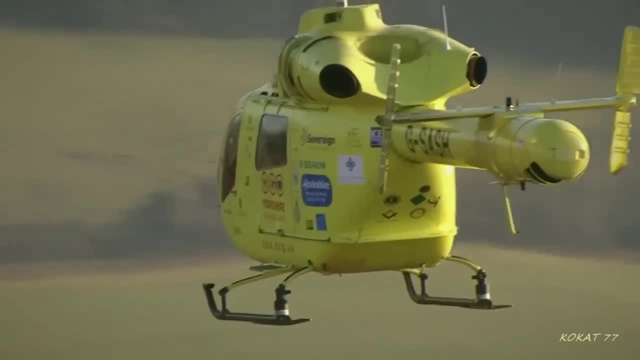 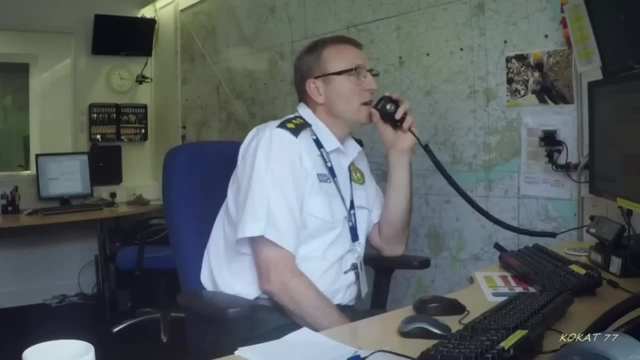 Yeah, The patient's having chest pains. His life could depend on the team's eyesight. Ground paramedics are hiking to the rescue. They've headed about a mile to two miles to the west on the bank in there. We are aware Helmet's attending. 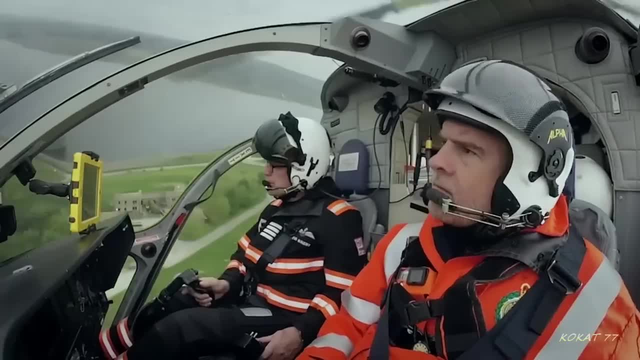 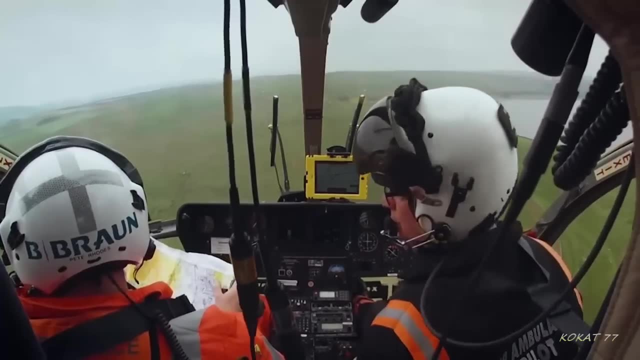 so hopefully someone will look out for you. There's someone in a red jacket on the corner behind the trees on the nose: Steve. Yeah, visual Pete's eagle eyes pick out three people on the banks of the reservoir. Help is now seconds away. 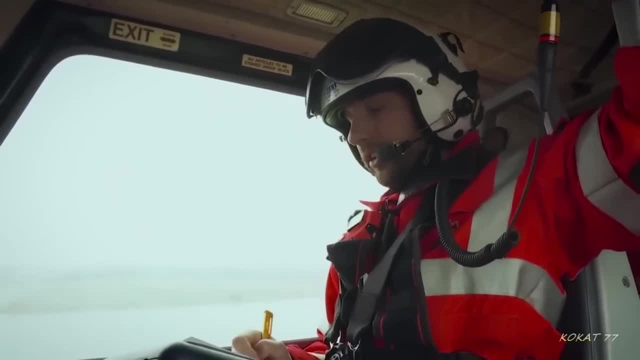 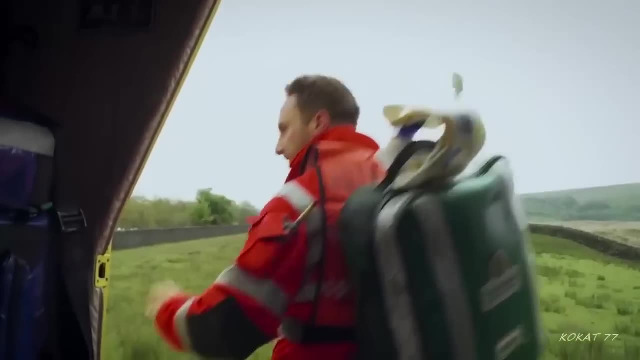 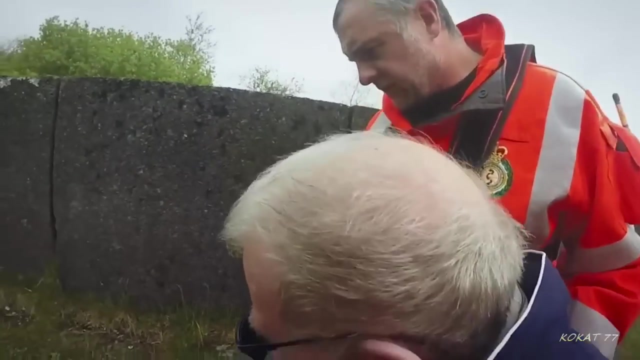 You've got visual on scene over there. That's a roger. Pray to land over. Paramedic Aidy will take over the man's care. Are you all right sitting up Or do you want to lean against the wall? Can you shuffle yourself over here, John? 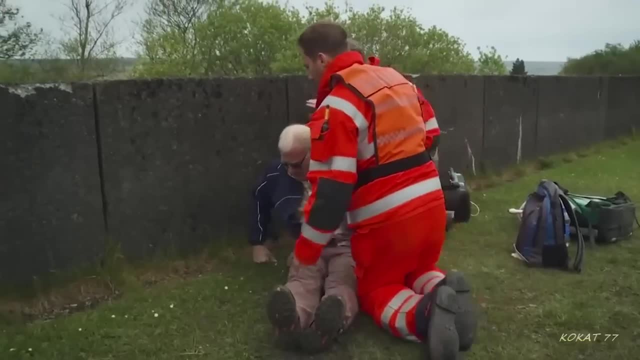 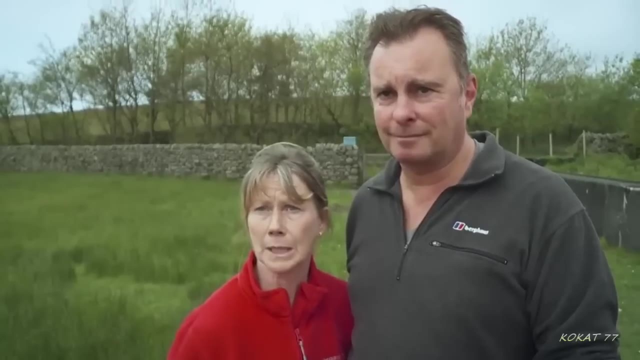 George into it. George George Ray was on a day out walking when he asked other ramblers for help As we just crossed each other's paths. he says: do you know where the nearest hospital is? And we said we don't. 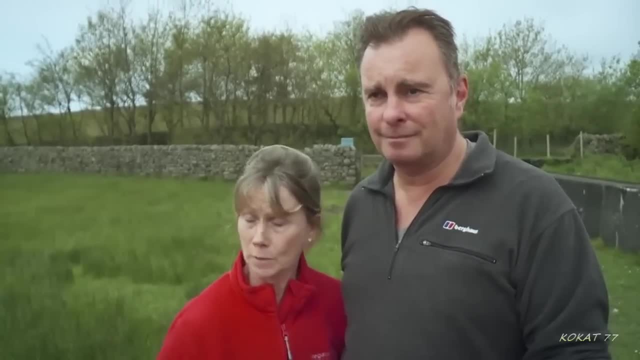 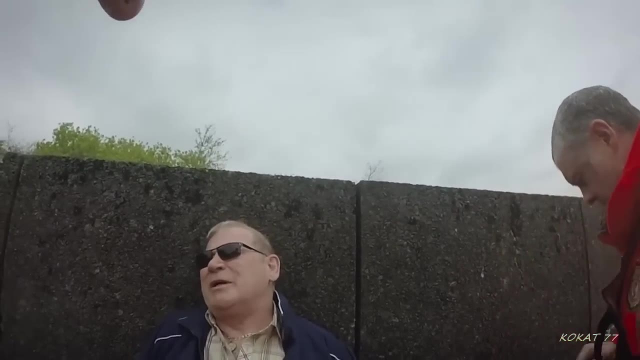 We don't really know the area that well, And he just fell to the floor Right then. George, Are you normally this out of breath? No, Can you give me a big smile? Aidy is testing George for the telltale clues of a stroke. 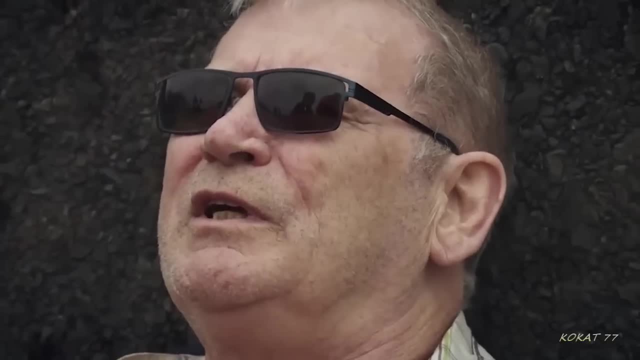 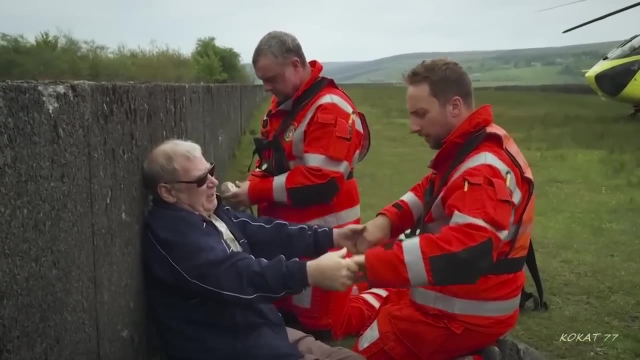 As best you can. His smile is thin. You grip my hands and squeeze really tight. Go on, try and break my hands Really tight, But his grip is strong. The signs are pointing to a heart attack. Try and stay as still as you can. 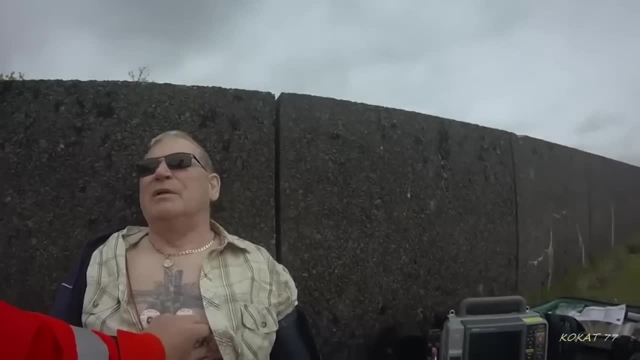 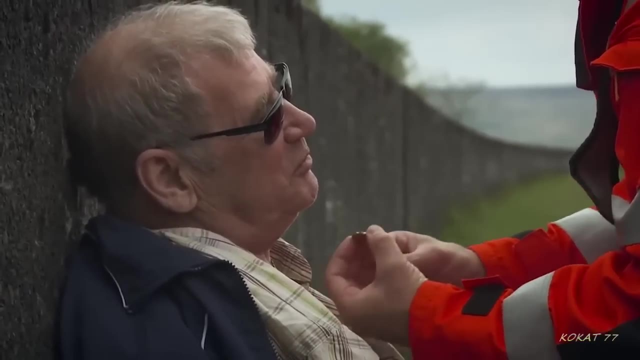 Just going to take a quick picture of your heart. So still, you are about the picture. All right, George is being wired up to an ECG machine. Not only will it help Aidy pick up the signs of a heart attack, but if George goes into cardiac arrest, 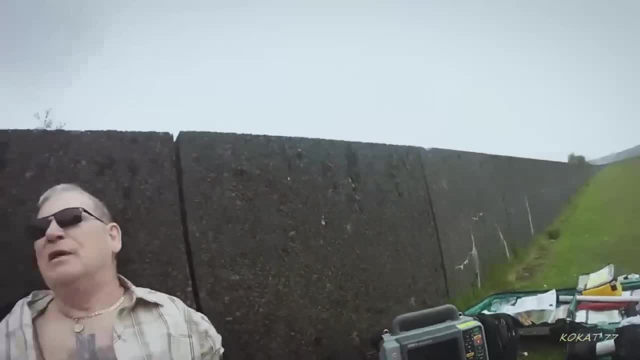 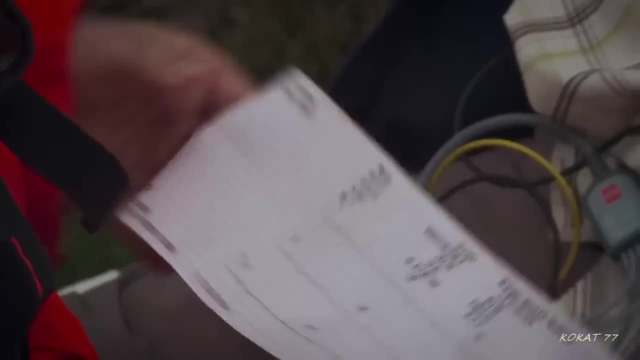 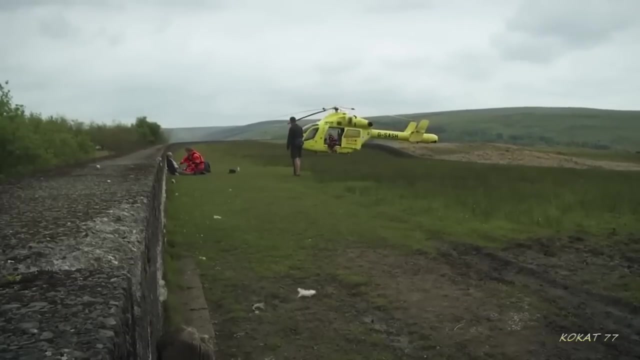 it'll allow him to shock him His heart back into rhythm. Very exciting in there. There's nothing really acute showing on your ECG, But the tests draw a blank. It's looking like George's collapse was caused by an illness or a minor cardiac event. 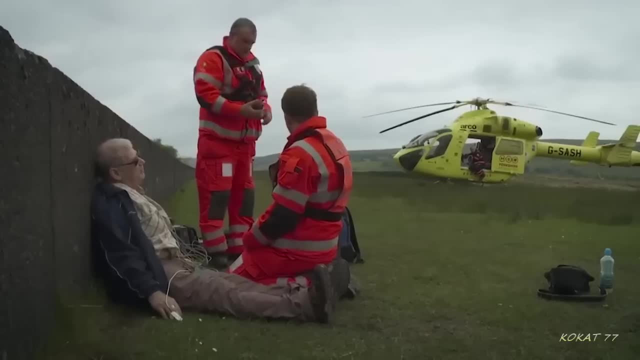 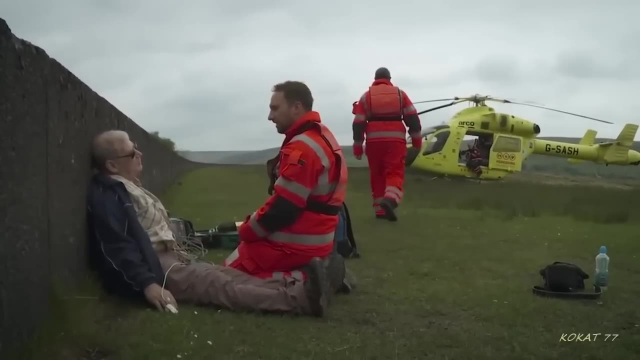 Right then, George. The plan of action is: we'll fly you to the ambulance, OK, And then they'll take you to the local hospital. The local hospital doesn't have anywhere that we can really land. Hello, is that Karen, Getting all mixed up? 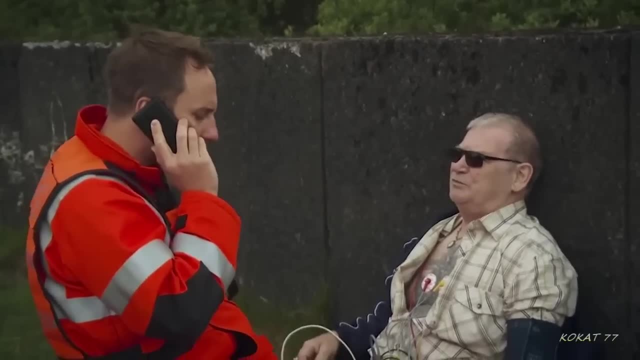 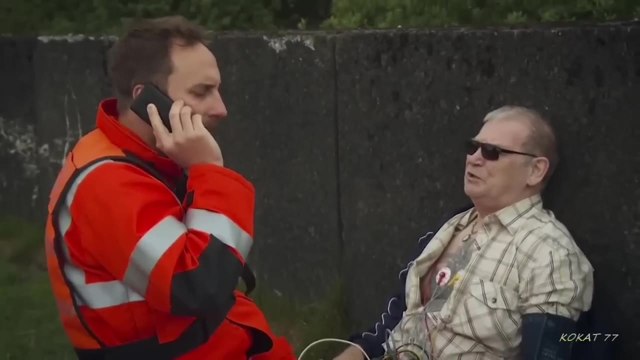 Hello, My name's Aidy. I work for the ambulance service. We've come to see your dad. Don't worry, He's OK, He's at Grimmouth Reservoir, Grimmouth. yeah, And he's been out walking and he's had some chest pain. 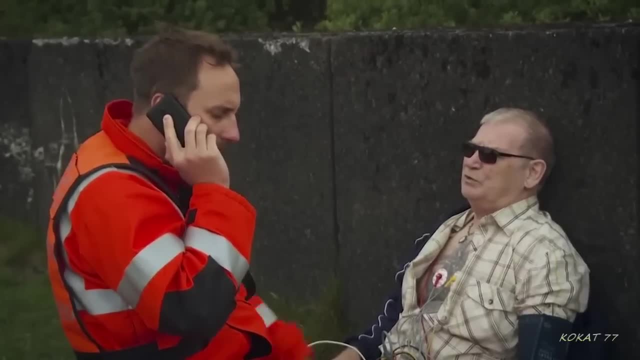 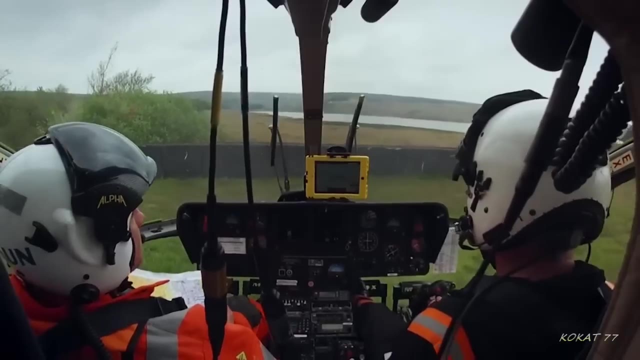 which we've dealt with and that's kind of gone. So he's not having a big heart attack or anything like that, but he does need to go to the hospital to see the doctor and just have some investigation. There's the DCA now. 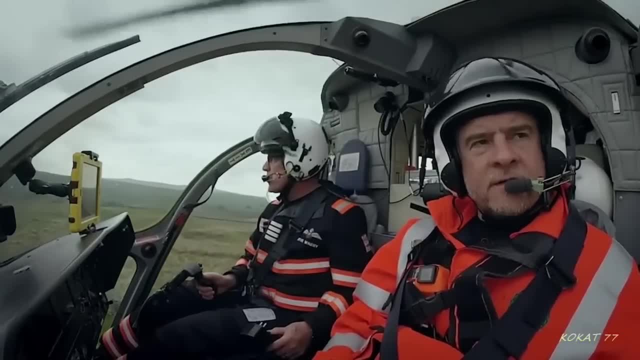 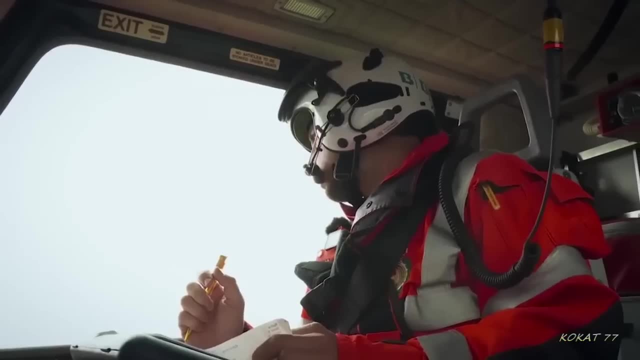 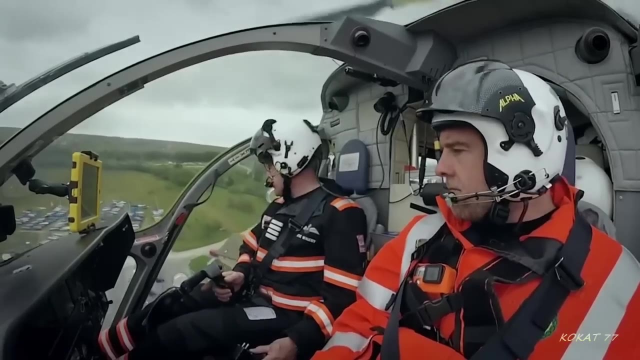 Got it. There's nothing to match air ambulances for speed, but paramedics will find it much easier to monitor George's condition in a road vehicle. Just watch out for any sails or maps which are out and about. Yeah, Tent at the far end there. 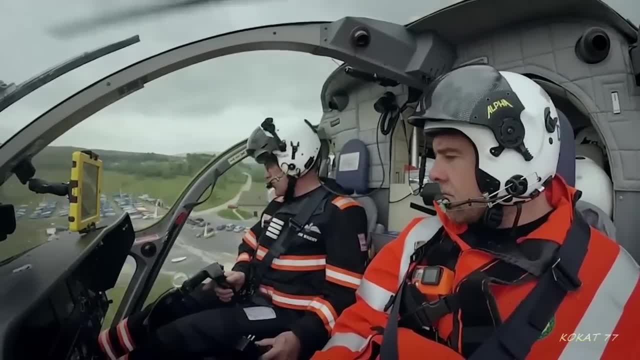 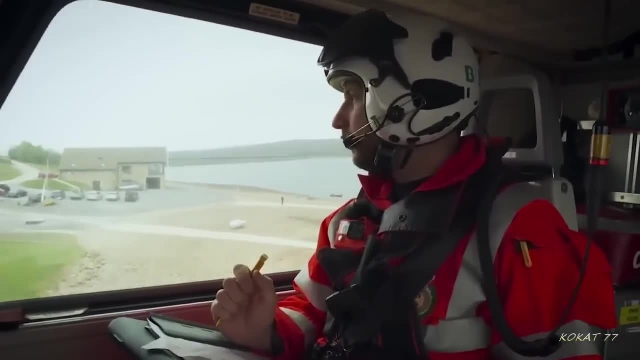 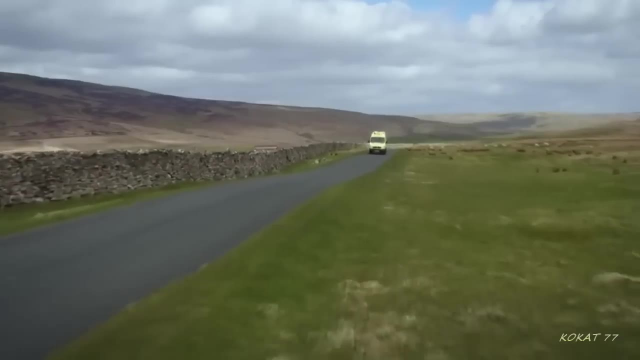 Yeah, got it All right. I'll just come to a little low hover here and then we'll reposition to the car park. That'll be fine there. George is off to hospital in Lancaster for tests They eventually revealed the cause of his collapse. 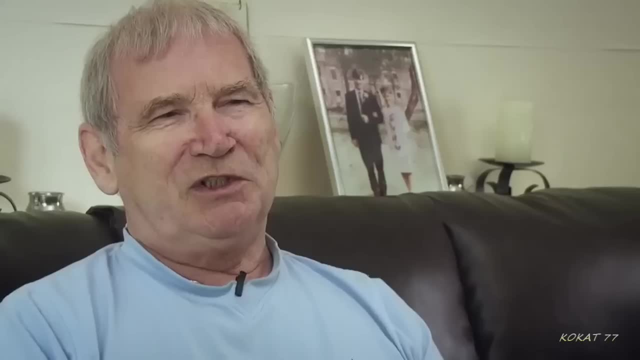 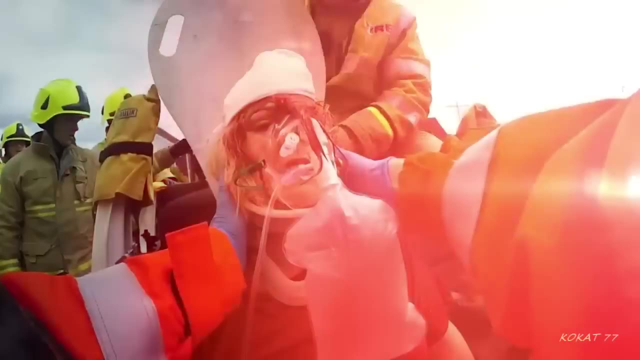 Consultant came, gave out tests and stuff and he said: basically I think you've had a small heart attack. George is now on the mend, As is Tracy, the motorist trapped in her car after it was hit by a high-powered hatchback outside her home. 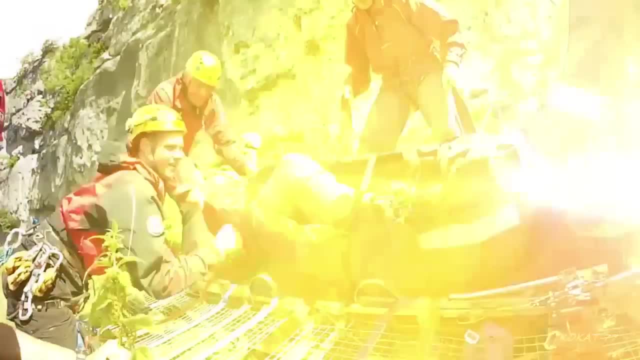 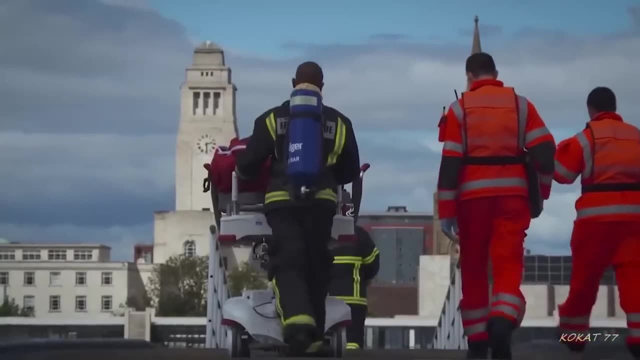 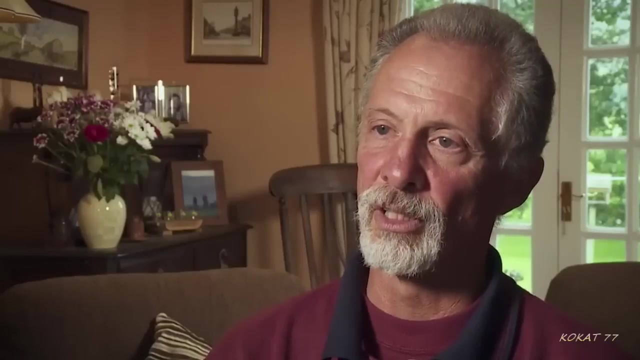 Police are still investigating. Climber Rod's dramatic rescue from the wreck could have saved him from lifelong paralysis. X-rays in hospital revealed the extent of his injuries. After the fall I had two fractured vertebrae, a fractured thumb and quite bad concussion. 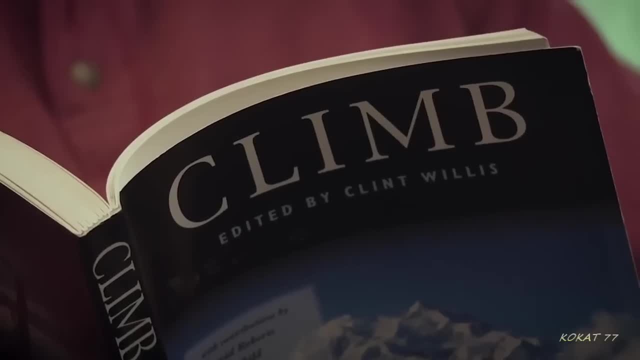 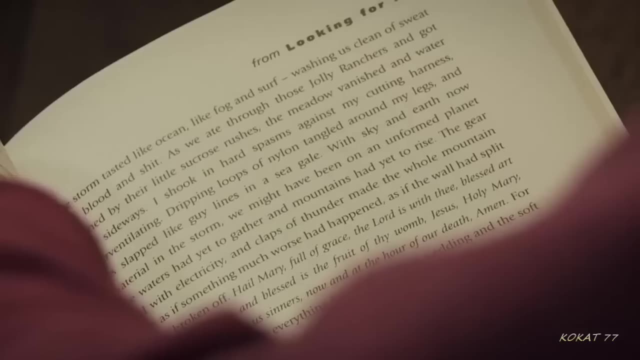 He's just glad he wasn't alone. Climbers end up in remote areas all the time and we very much rely first of all on ourselves to look after our climbing partner or whoever's with us, And other climbers and other walkers and members of the team. 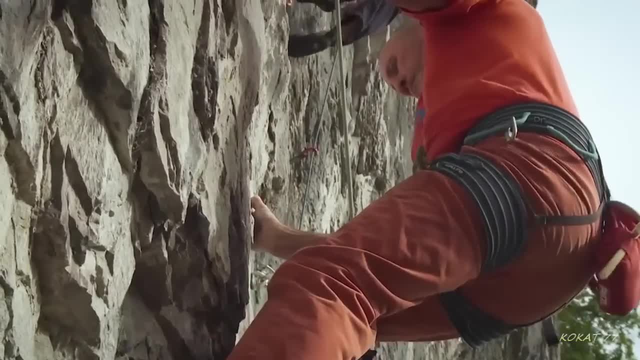 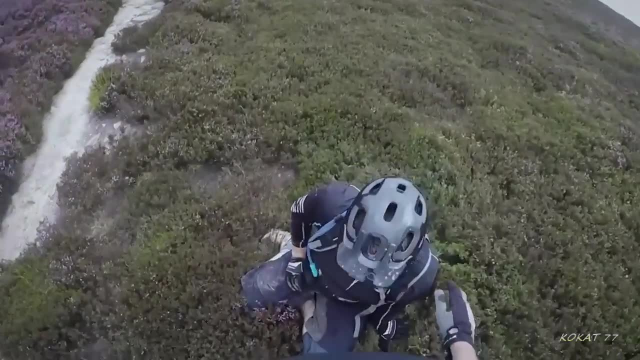 to help us out Climbers and other walkers and mountaineers. there's no question that you'd help someone else. Whatever you were doing, you'd drop everything to go to help them. Sean the mountain biker who landed on a boulder. 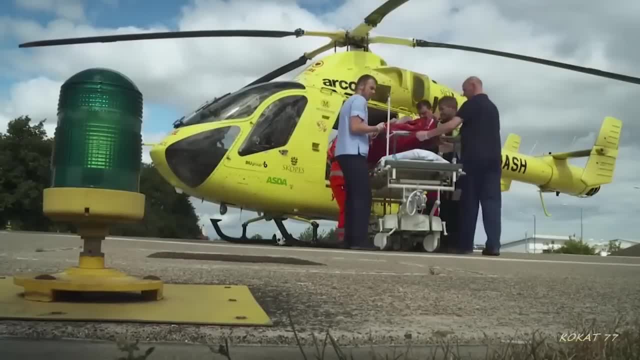 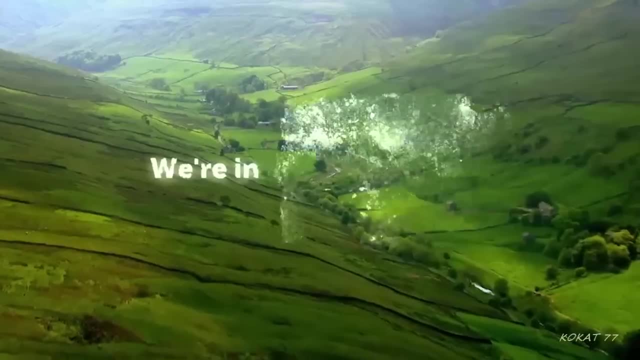 was found to have three broken ribs, a collapsed lung and two lacerations to his liver. He's recovering Hill legs anything below my neck. We're in a remote location in the middle of the woodland, The speed of the Yorkshire Air Ambulance. 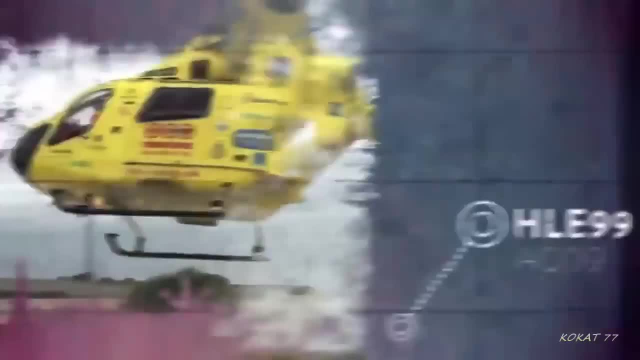 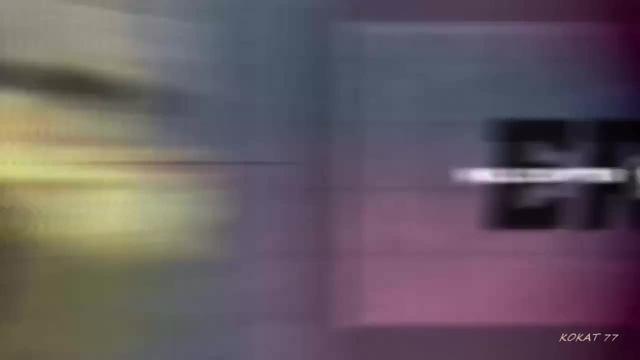 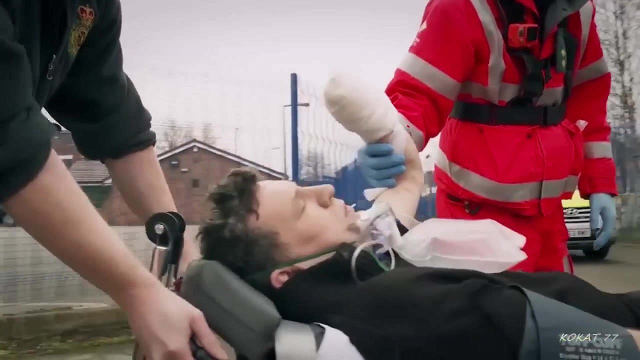 can make the difference Between life and death, At your discretion, take off. Today the team's been called to an industrial accident after a factory worker loses his arm. Where's the other part of his arm? Ice puts the skids under an elderly motorist. 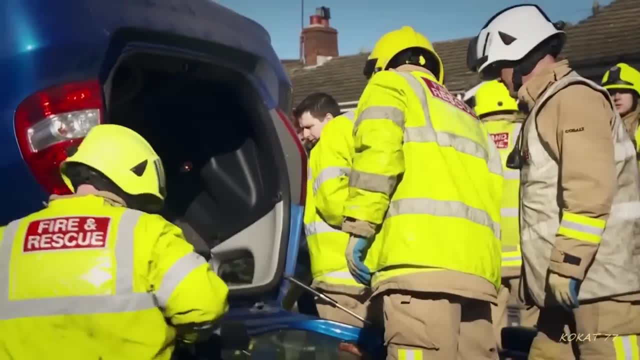 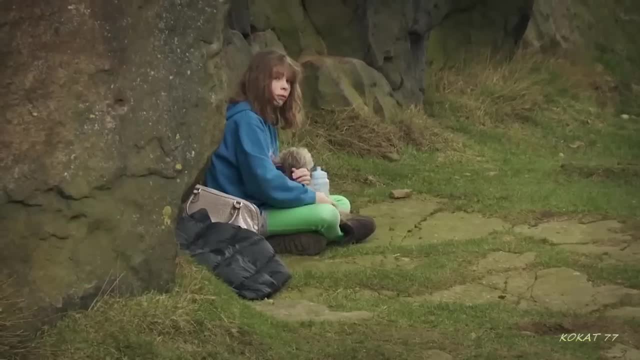 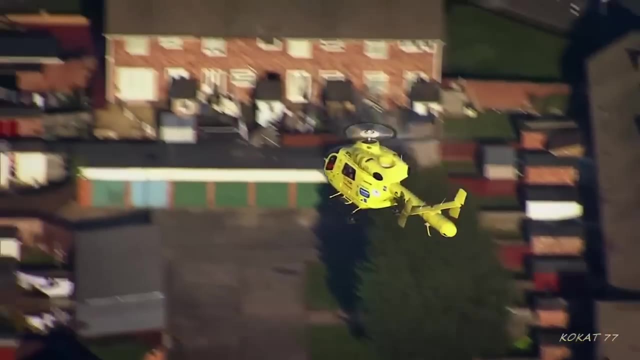 and his wife is trapped. I love you. I love you. And a man's fall from a famous Yorkshire landmark is witnessed by his wife and daughter. Why don't you not listen? Hello ambulance service. Is the patient breathing? He's struggling to breathe. 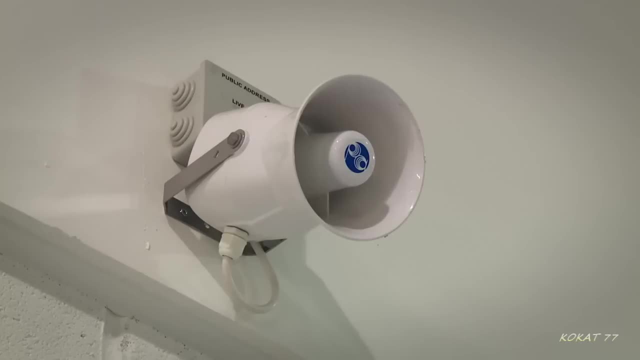 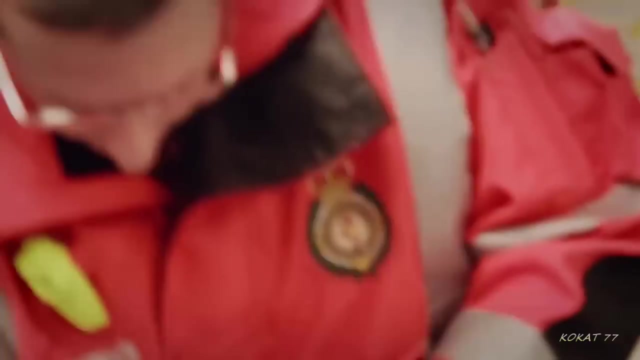 Tell me exactly what's happened. He's breathing OK. I've called an ambulance earlier. I've got a job for you. This happens more than 1,000 times a year at the Yorkshire Air Ambulance Bases. The mission is to be in the air. 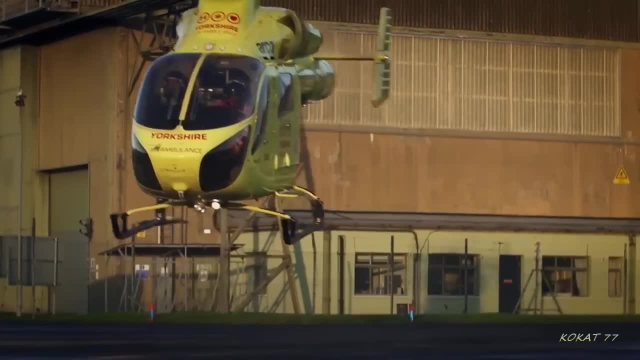 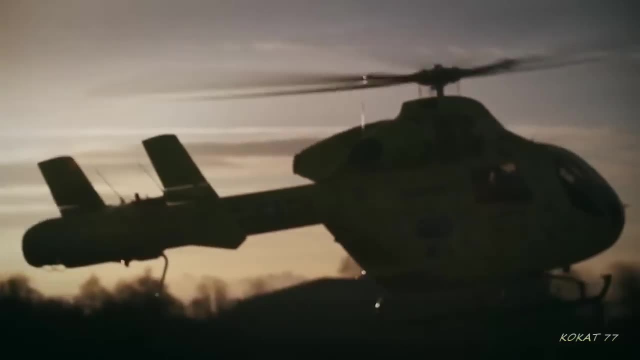 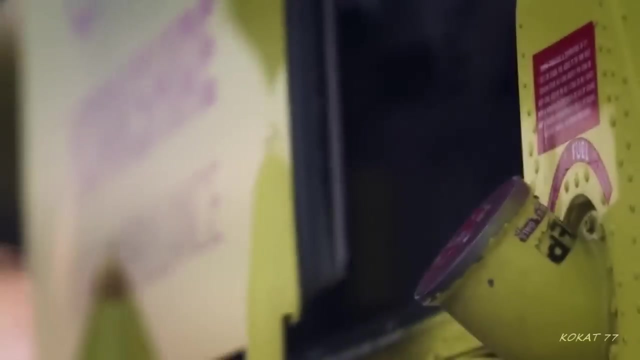 within two minutes of the scramble siren. Speed saves lives in this business And even when they've just delivered one patient to a trauma unit, if another case comes in, they must be ready for take-off at any moment, And today at Sheffield Northern General Hospital. 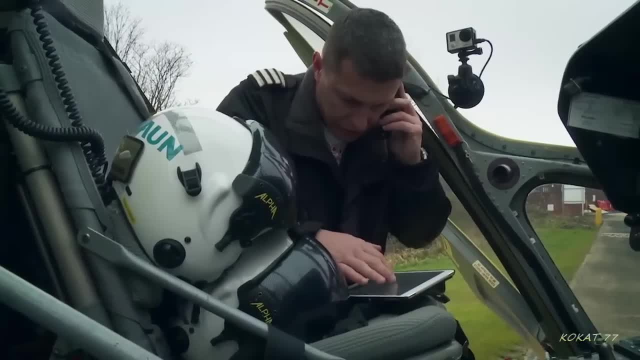 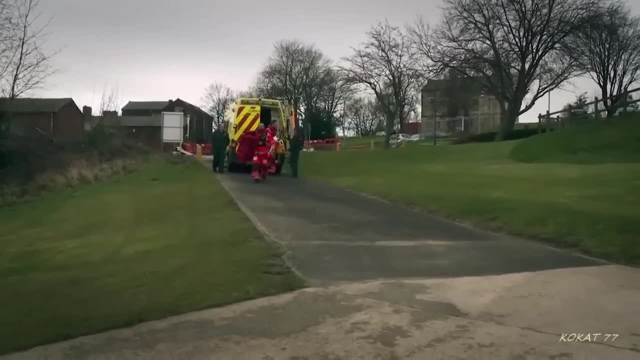 that's exactly what's happened. OK, no worries, mate. yeah, It's an industrial site. yeah, OK, mate. See you in a minute. Cheers, mate. Pilot Gary Brasher and his crew are being scrambled to a bad accident ten miles away. 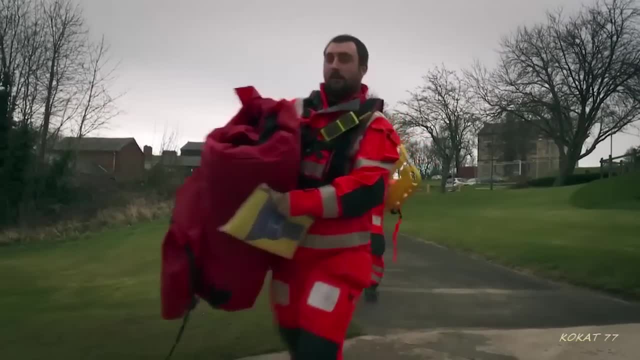 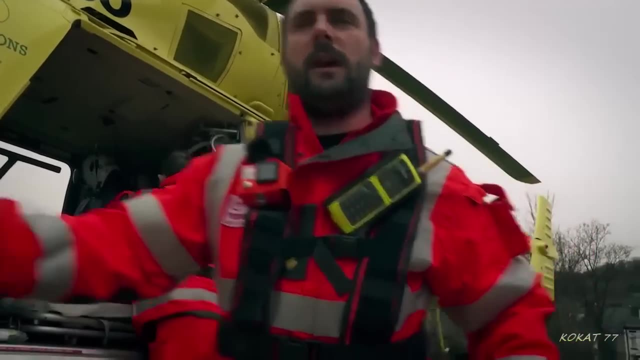 Have you got the job? Yeah, Got it great. We've just been alerted to another job in Mexborough, in the local area of Rotherham, Possibly a traumatic amputation. so obviously we're just going to make up quickly now. 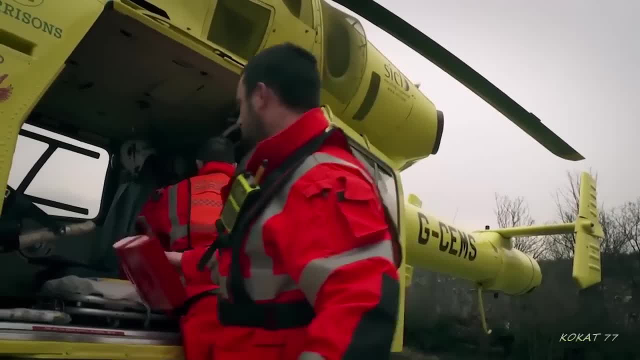 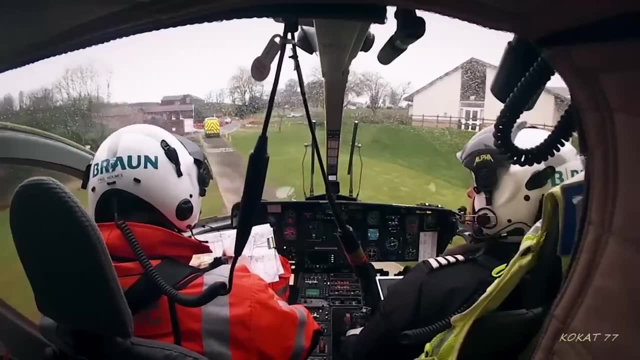 and then get on our way there. More details will get out in the flight. so Just control switches, Flight flight confirmed Flight airwaves off- Clear left. We'll be there in five minutes. Yeah, Roger, thanks for a quick turnaround. 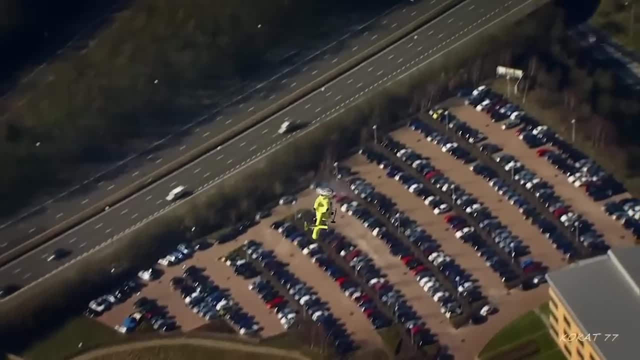 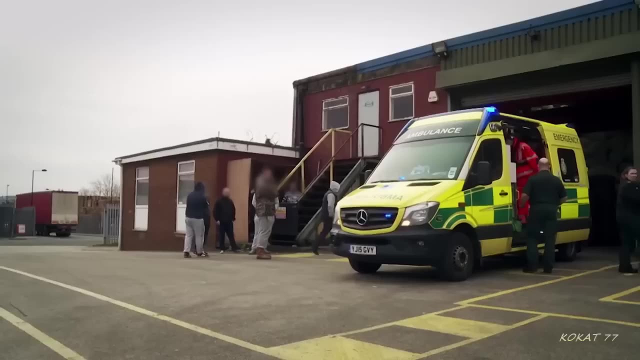 Paramedics James Stubbley and Paul Holmes are on their way to a factory where a worker has had an accident with a shredding machine. An ambulance crew are currently working on him. It's unclear why he had his hands near the machine. A bit of confusion. 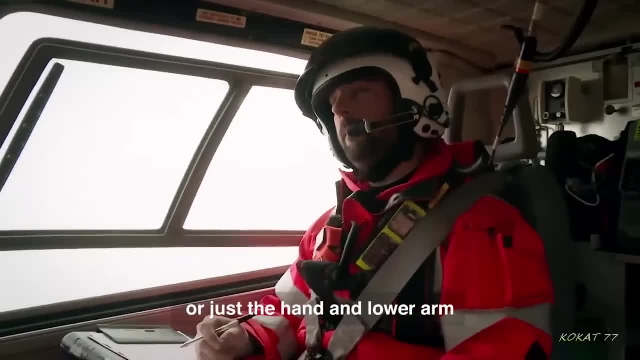 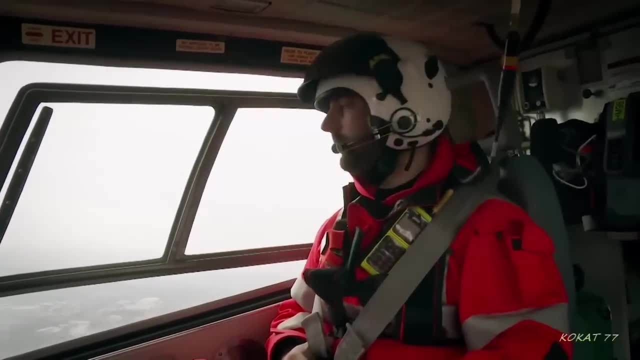 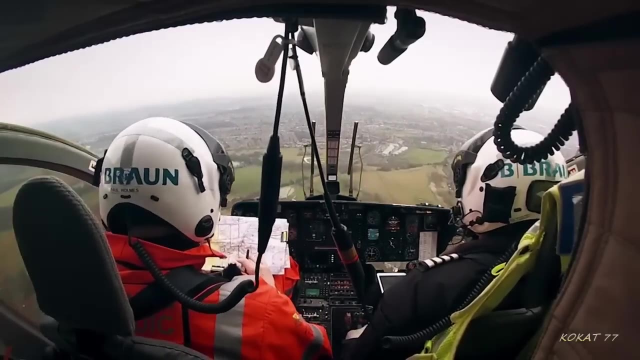 whether it's the whole arm or just the hand and lower arm of it. No, We just need to remember to bring both bits with us from this. Yeah, Body parts can be reattached even a few hours after injury, but there are often complications. 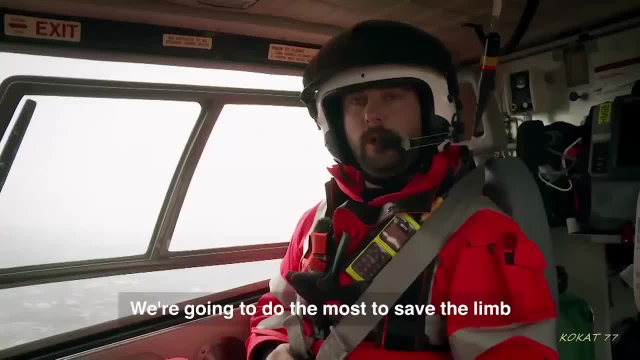 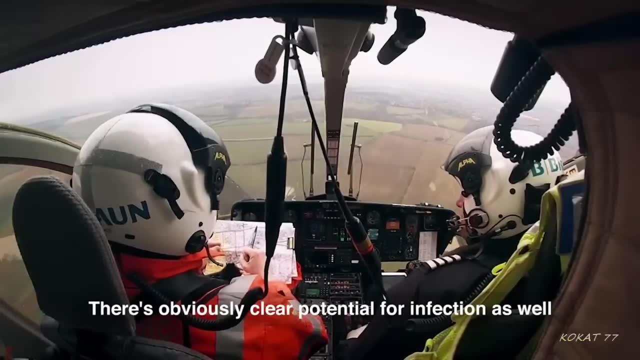 There's significant potential for blood loss, so we're going to do our best to try and save the limb, but it just depends on the degree of the severity of the amputation. There's obviously clear potential for infection as well, which then cause problems further down the line. 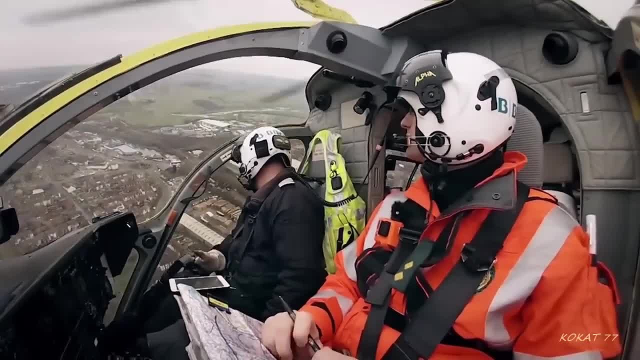 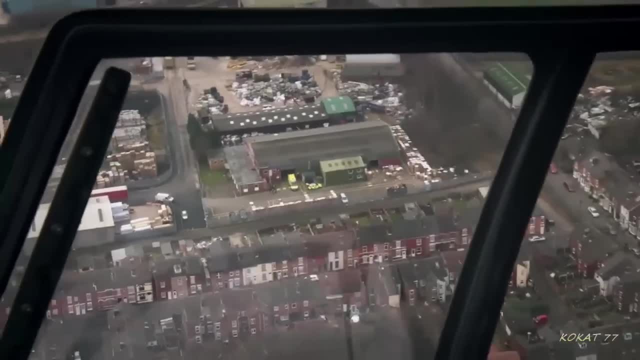 Ambulance down low 3 o'clock. They're on final approach, but it's a built-up area That's a bit of a frigging nightmare to land, isn't it? It's too dangerous to go into the yard. 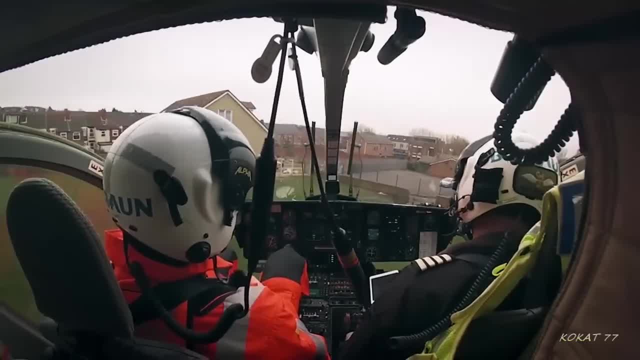 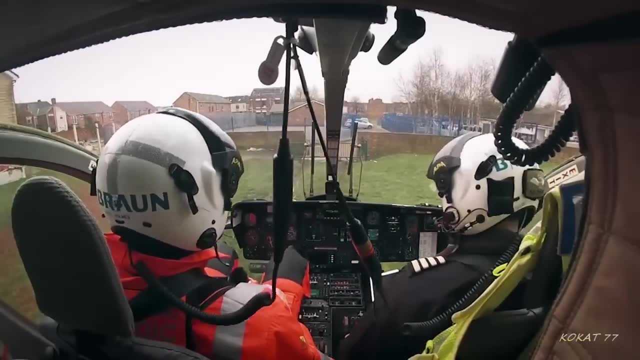 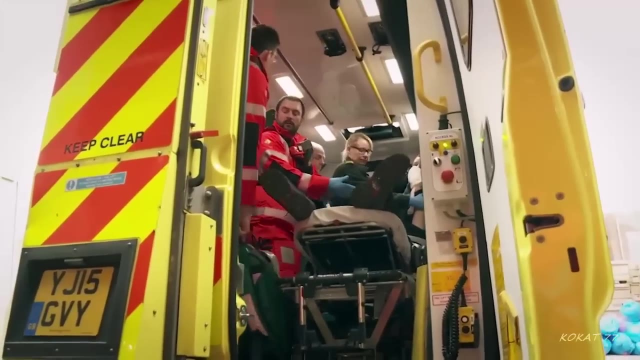 Gary chooses a nearby playing field instead. Bag blowing away, one going up. Yeah, it's going for the disc. I'm happy. Yeah, that's nine-eight apologies on the ground: 55-year-old Tony Davison is still in the back of the ambulance. 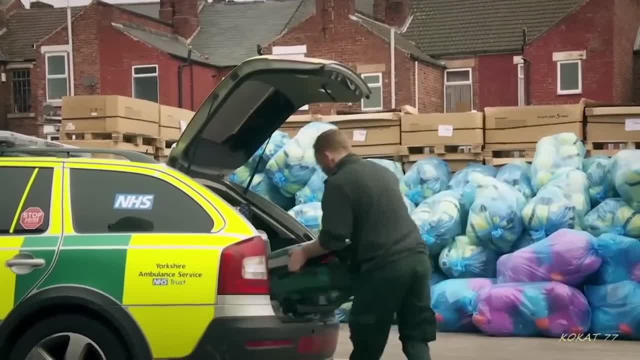 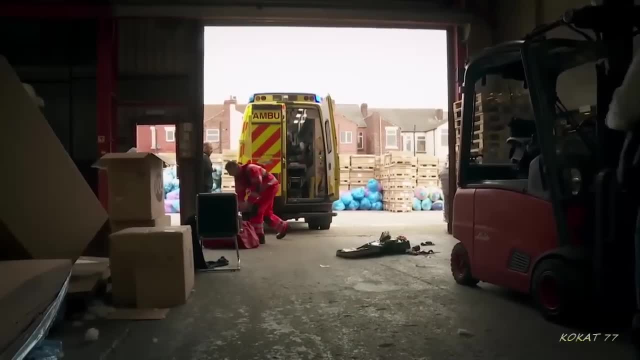 when Paul and James arrive. His arm is bandaged and he's stable, but it's a devastating injury. The crew's done a good job. It looks like he's amputated it, probably from round about there, so his hand's obviously missing. 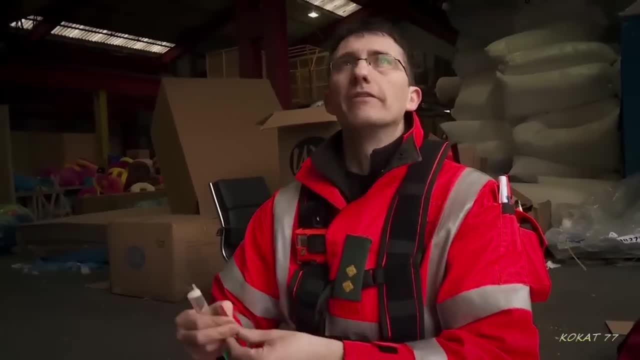 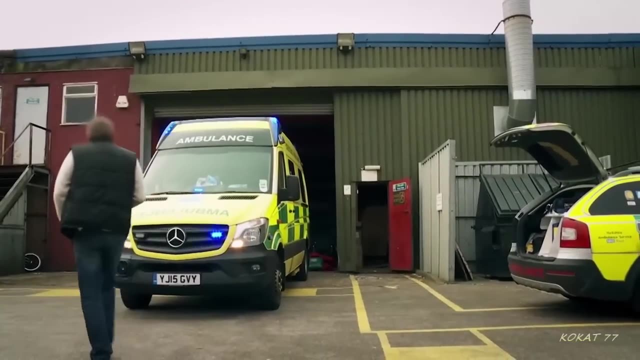 but he has got obviously part of his forearm, So it's just above his wrist. I think A combination of shock and nerve damage have kept Tony's pain levels surprisingly low. but Paul isn't taking any chances. He'll be administering the strong painkiller ketamine. 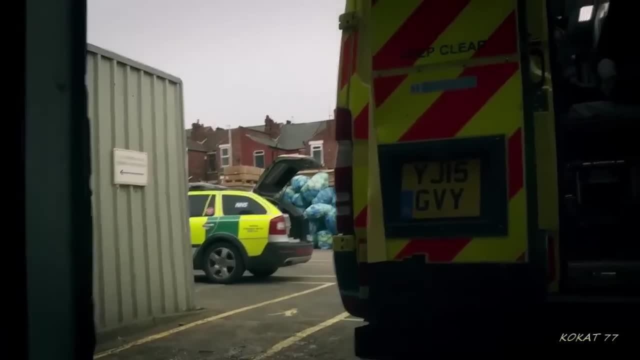 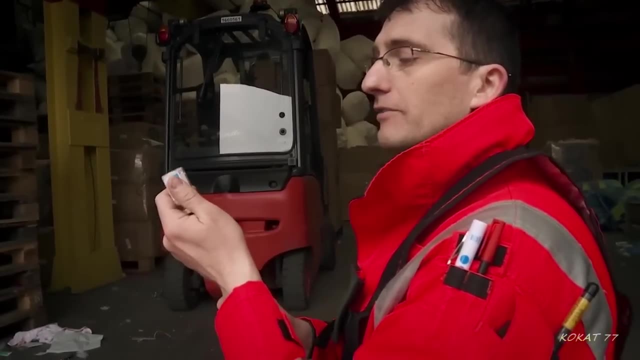 So we're going to join some ketamine up, which is obviously a bit more strong analgesia than morphine and paracetamol. Give him some of this. It's not actively bleeding at the minute, so we've got a cat tonic here. 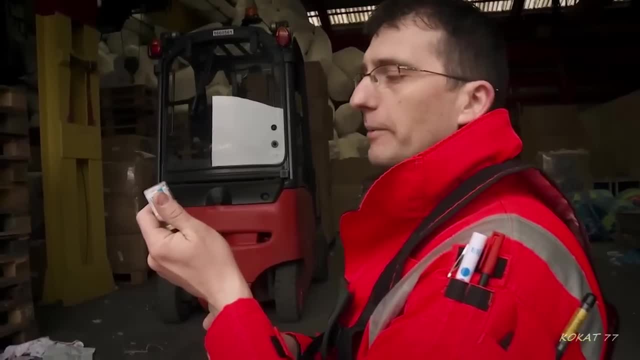 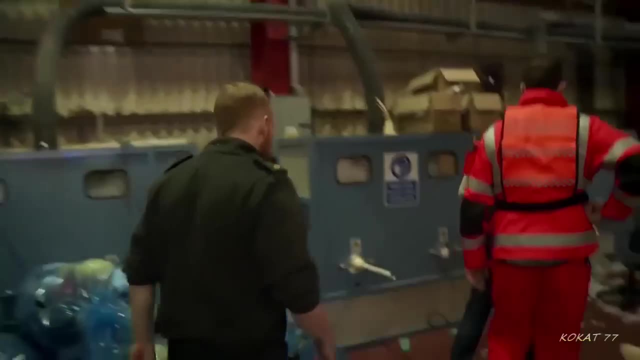 and the crew's done a good job of stopping the bleeding. So we're going to give him this, Get him on board the conveying back to Northern General. Understanding how it happened, what medics call the mechanism of injury, will be important information when they get to the hospital. 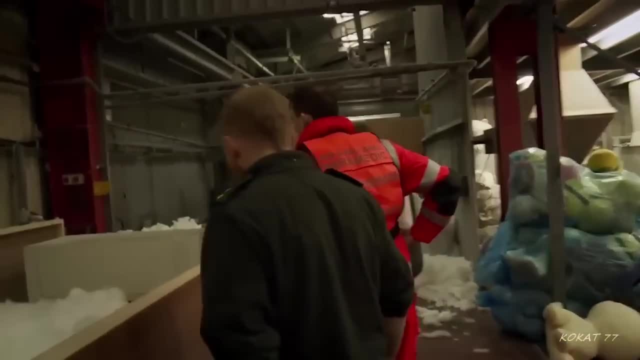 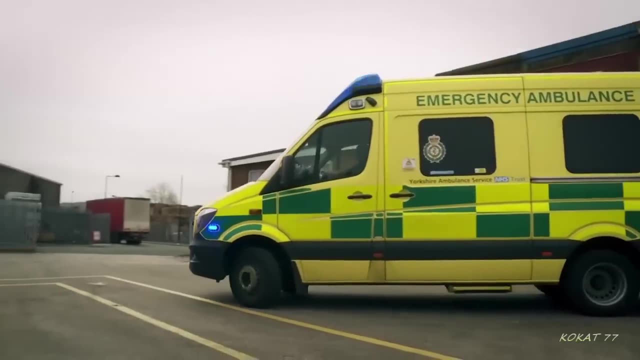 There's also an important unanswered question: Where's the other part of his arm? I don't know. Even after a thorough search, the missing hand and wrist is nowhere to be found. Just take it over that way a bit, Dave. It's a bit bumpy. 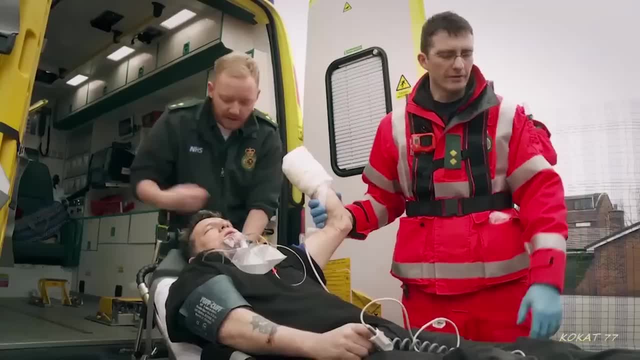 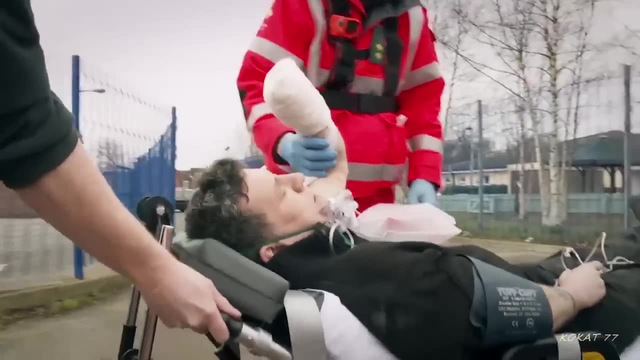 It's a bit bumpy. It's a bit bumpy And we'll scoop him. It's just. it's easy for us to try and support him on the scoop. that's all, Yeah. What have you been doing then, Tony? 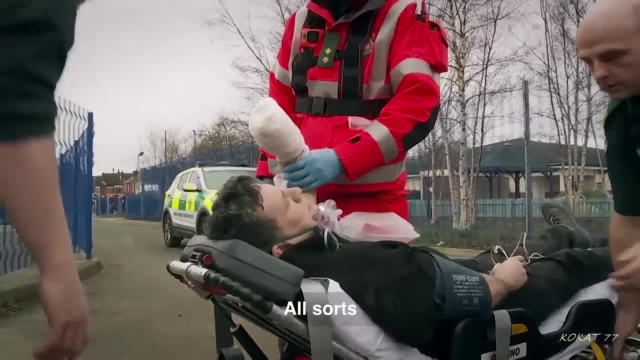 What do you do at work? All sorts. You find loads of stuffed teddies. Yeah, How long have you worked there for This new place? we've only had it, we've only got it for 15 months, Oh yeah. 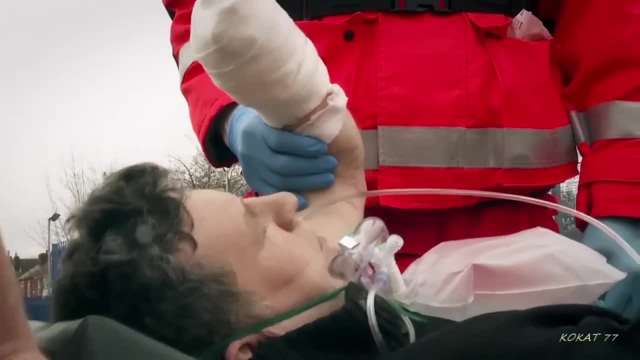 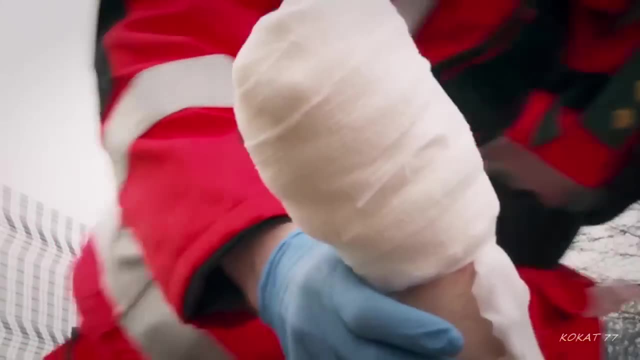 We haven't been there that long. Just relax back, will you? Yeah, We've only been there since the 4th, And it may be a while before he's there again with this injury. He's got to be careful. He's got to be careful. 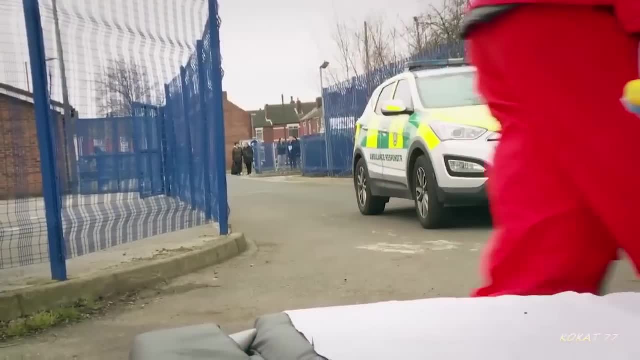 There you go. All right, mate. Once we've got him settled down, sorted out and wired up on the aircraft, we're going to fly him to Sheffield Northern, off to the Regional Trauma Centre. The team's already waiting for us. 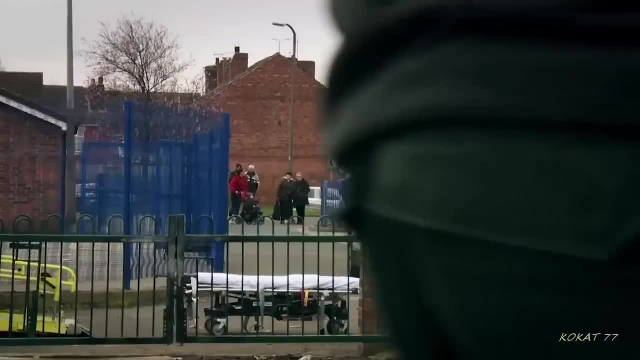 So once we've got there, they'll be able to quickly give him assessment and then get him into whatever treatment course they need to do. Confirmed perfect flight Airways are stooped or off, or whatever you want to do. Yeah, Yeah. 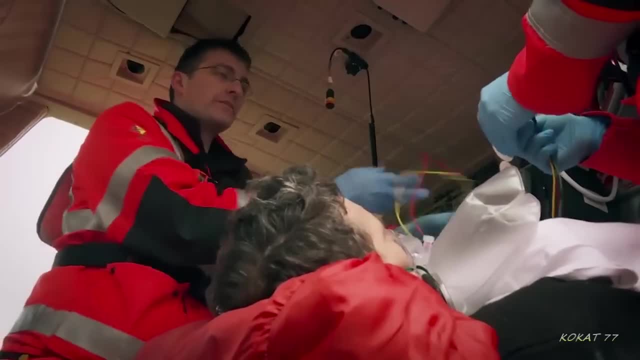 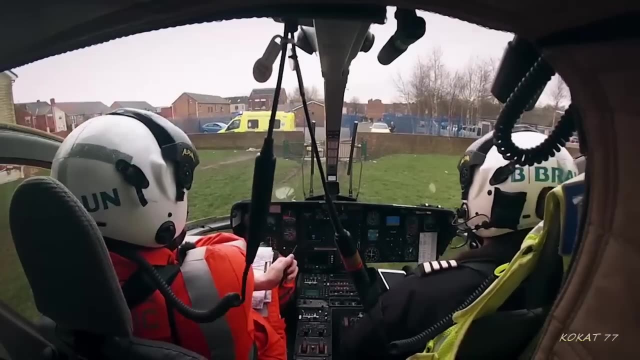 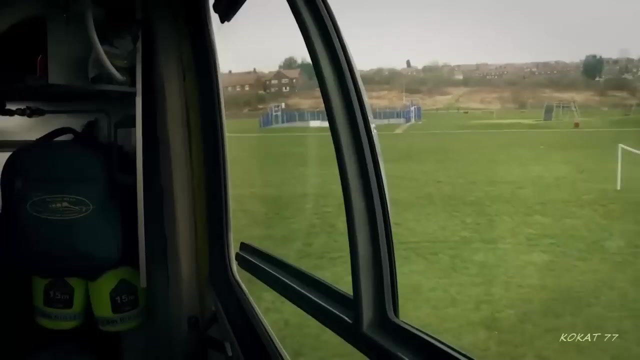 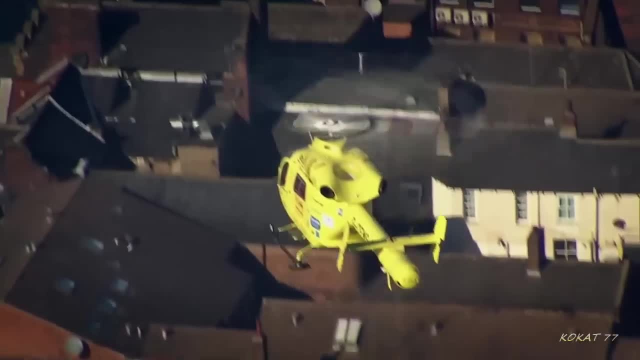 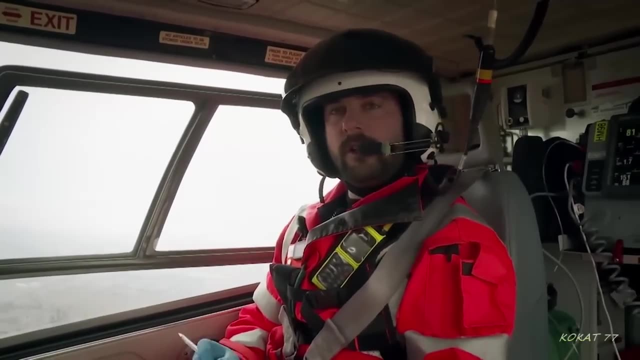 But his injuries are extensive and the prospects for rebuilding his arm look bleak. What they've described is that mid-forearm has been. It looks like it's been shredded from what they've described. rather than an actual clean amputation, They have described that it is still attached. 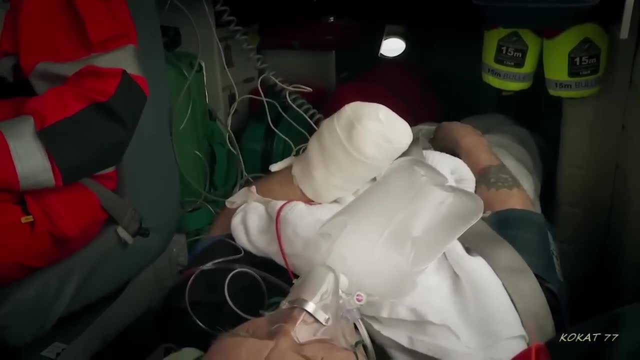 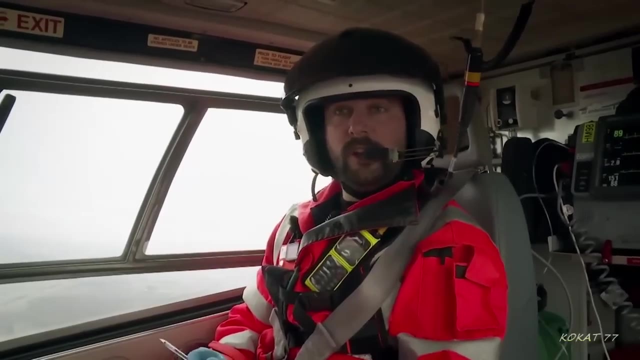 If surgeons can save even part of his hand, Tony's quality of life will be much improved. Yay, The specialist people at the Northern General. that's the best place to take him to. so if there is any chance, then he's going to the right place. 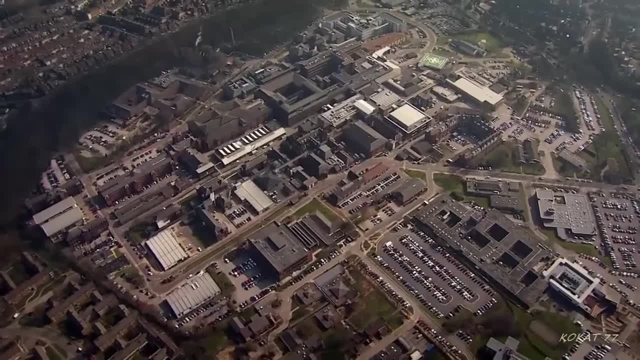 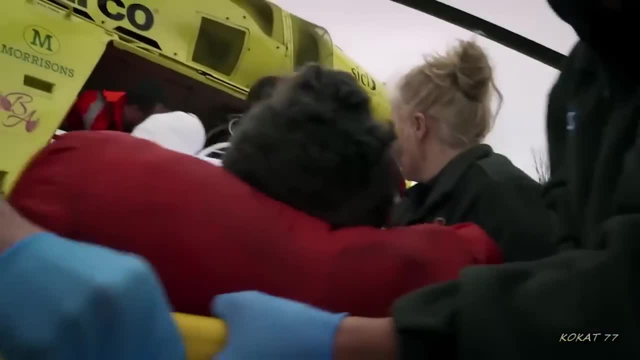 It's amazing what they can do, but it just depends once they've done a full assessment here with the specialists. An ambulance awaits their arrival in Sheffield In the next hour Tony will find out if part of his hand can be saved or whether he must learn to adapt to life with only one hand. 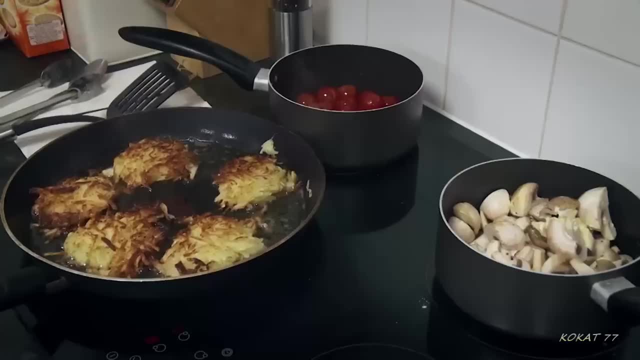 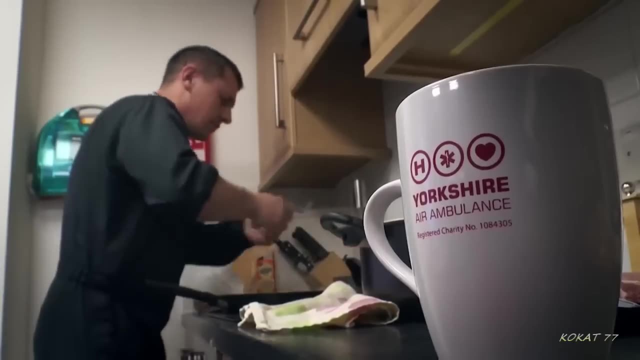 Every day's an early start at Helimed headquarters and there's no argument who's in command of breakfast. When you're a pilot, it's like a helicopter pilot. You have to do a lot of things at once, a lot of complicated tasks all in one go. 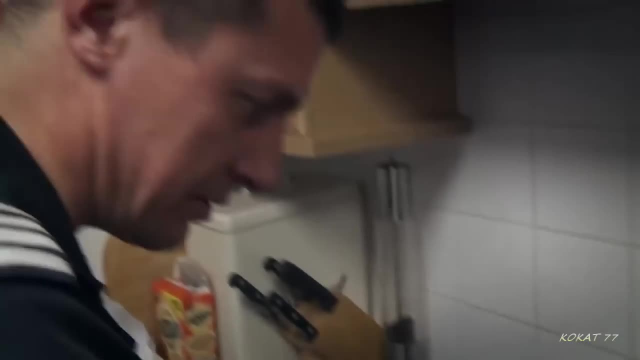 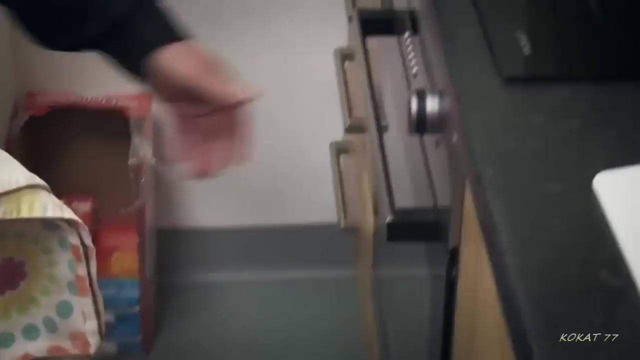 And making a good breakfast requires you to do something quite similar, because you're juggling all the different things. You've got things in the oven, things on the go. We're nearly there. we're nearly there. Pilot Gary is an army veteran. 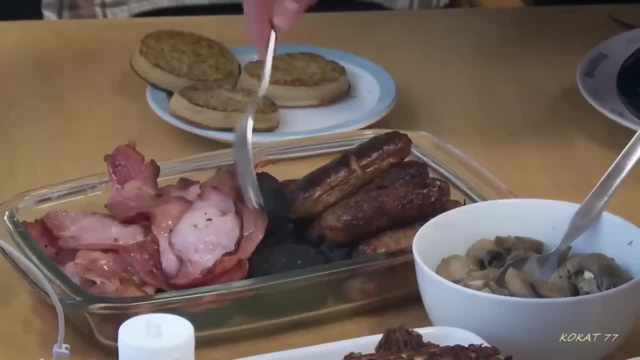 and he's been in the military for over a decade. He's a man who insists on a great British breakfast to set his crew up for a day saving lives. It makes sense, really, If anybody's going to make the breakfast out of the crew. 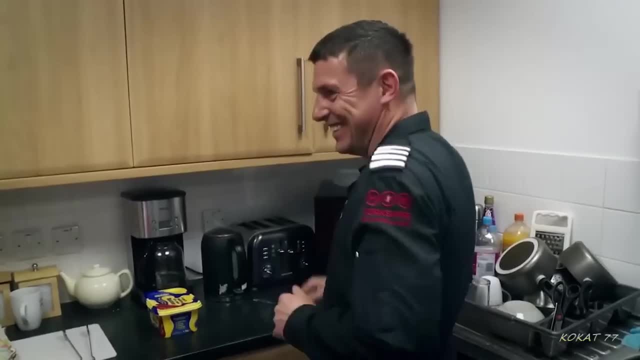 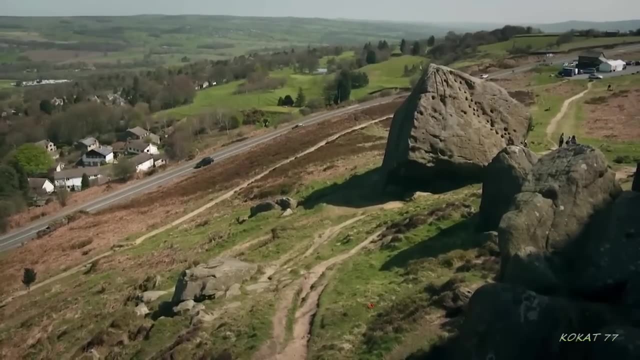 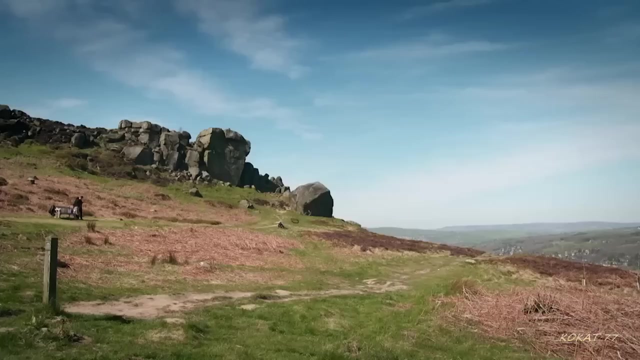 it should be the pilot, because they're going to be the best at it. But 30 miles up the road, on the edge of Ilkley Moor, someone else's morning has had a terrible start. Reports are coming in about a serious fall. 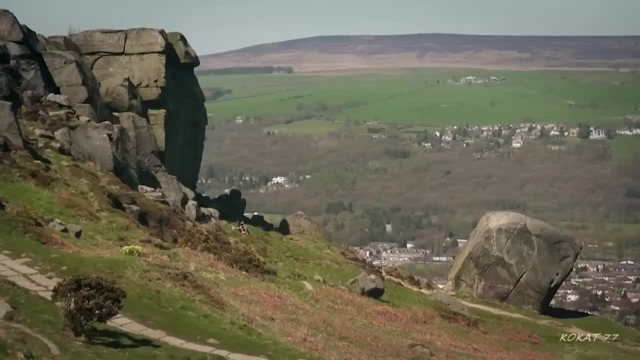 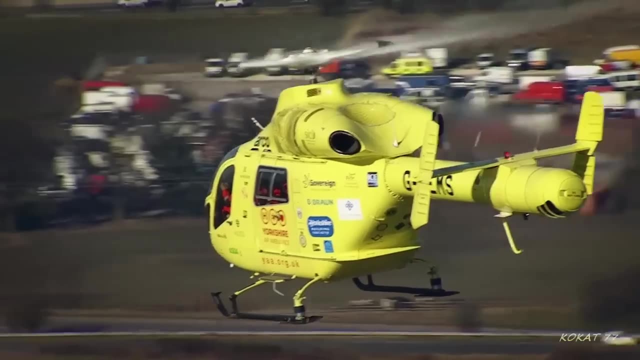 on the huge boulders known as the Cowan Calf Rocks. How far did he fall? Probably about five metres. Is there any serious bleeding? Yes, there is. yeah, And I have a flipper from Base 4 on board. 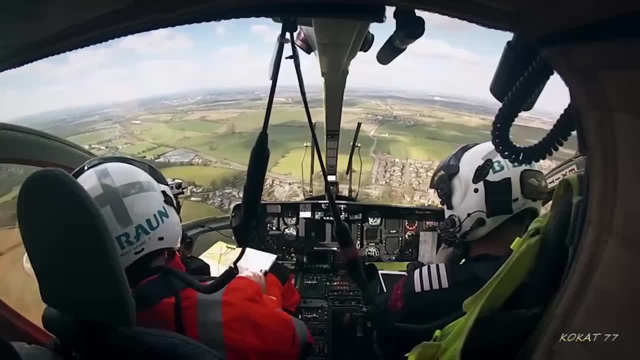 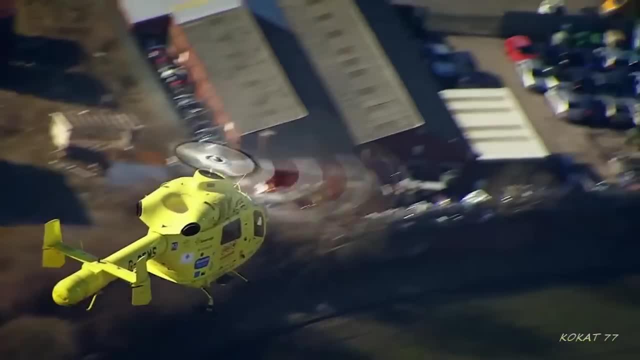 routing to Ilkley Moor on task. The base is servicing Clint through the zone. We're on the way to Ilkley Moor, to the quarry just behind the Cowan Calf- well-known sort of rocks on Ilkley Moor. 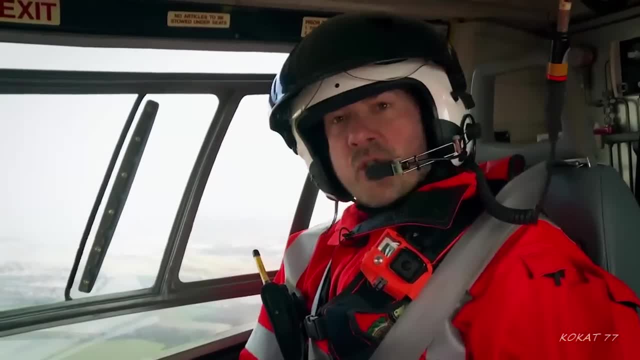 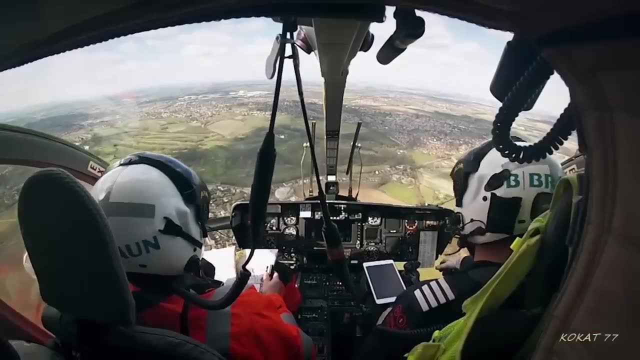 overlooking the town of Ilkley. This chap's fallen and has a head injury. We don't know for certain. it's a climb or a mire, just a spin Walk. remember the public's got too close to the edge and it's a little bit loose in places. 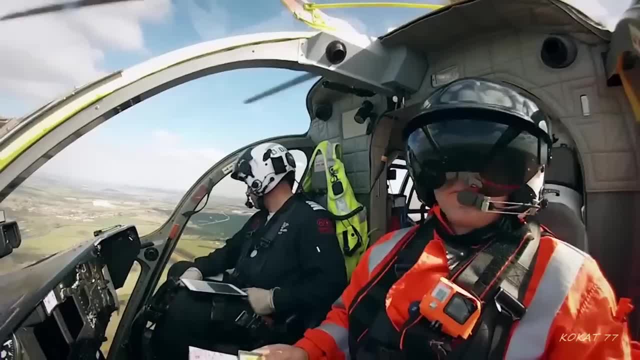 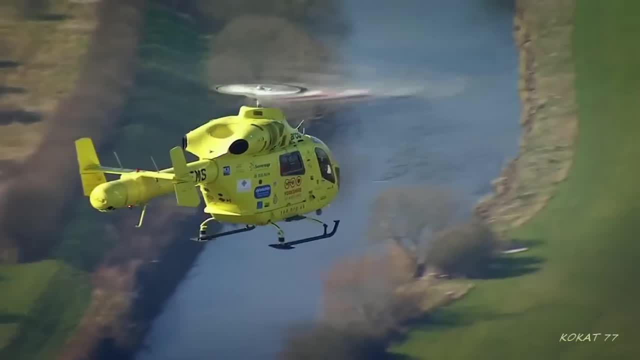 so people do tend to have mishaps there. Down the line, I'll tell you exactly what to do next. I'm going to tell you how to stop the bleeding and listen carefully to make sure we do it right. Pilot Gary's been there before. 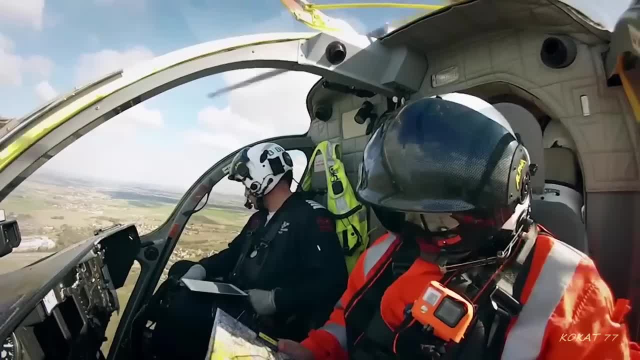 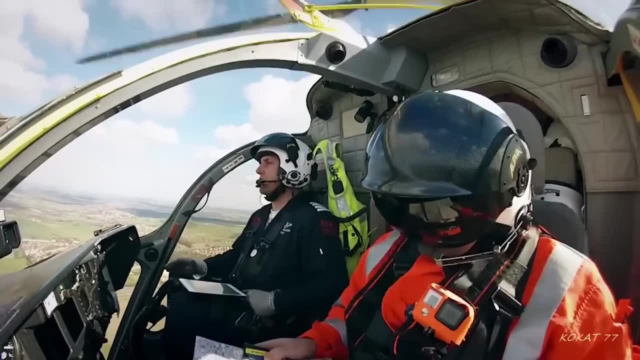 The accident has happened in a disused quarry. Your options are either on the top Gaz or down on the board near the car park. I've, actually, I've, actually, I've landed there before There's a crossroads of a trough. 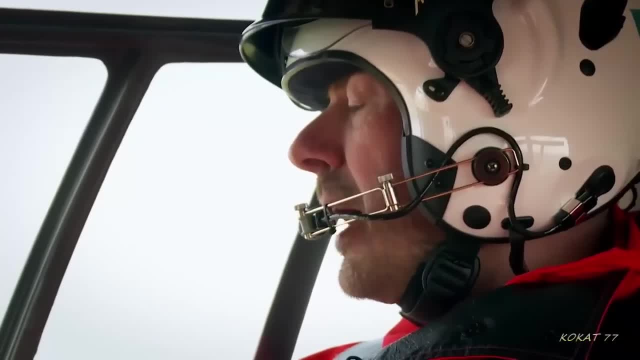 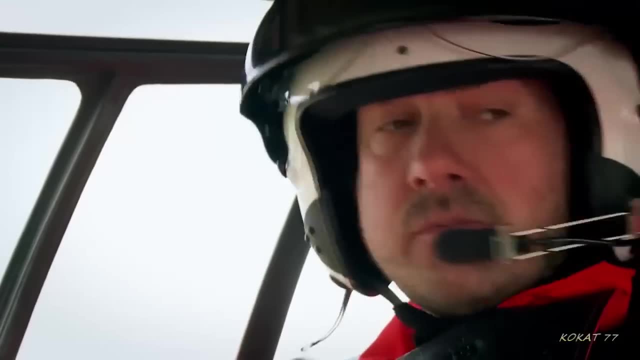 Just outside the quarry you can land them. Yeah, you might get in there. That'd be good if you could. Otherwise, on the top's- the probably next best option, Paramedic Al's a part-time mountain rescue leader. He knows the area well. 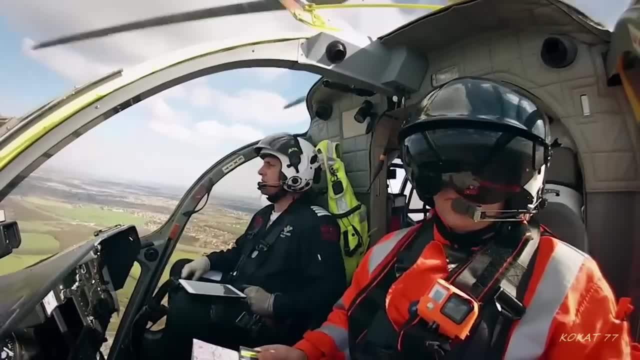 I don't think you'll get in that quarry, but Yeah, you can. There's loads of room. Ooh, challenge, Oh there we go. Challenge, Red rag bolt and all that. That was it, The heaviest build ever. 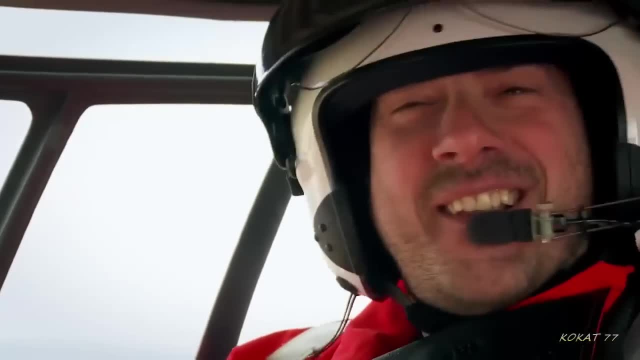 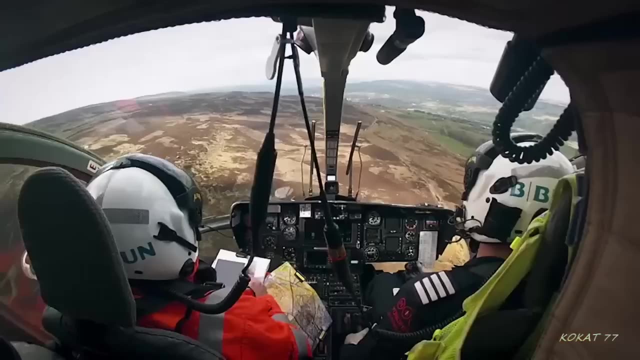 The gauntlet being thrown down. I will. Gary wants to land as close as possible to the patient. This is one of Yorkshire's most popular tourist attractions. Landing could be tricky, It's going to be heaving, And all them cars. 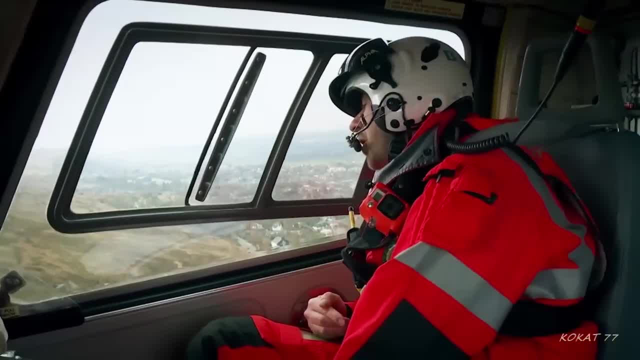 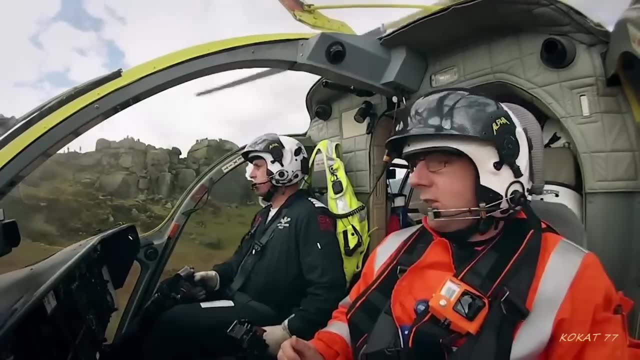 People on the People on the ridge. Do you want me to open the door and move them on? I don't do it. They're all tied together, Are they really? Yeah, They're on some sort of They're not criminals, are they? 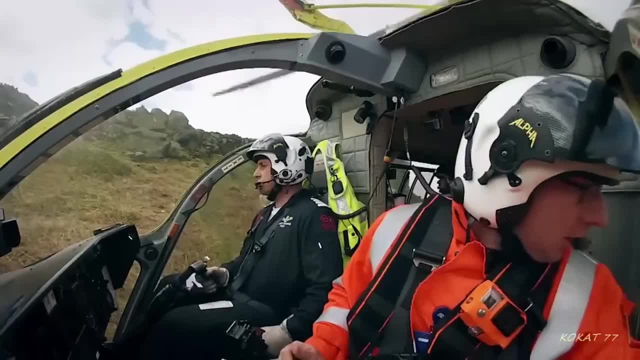 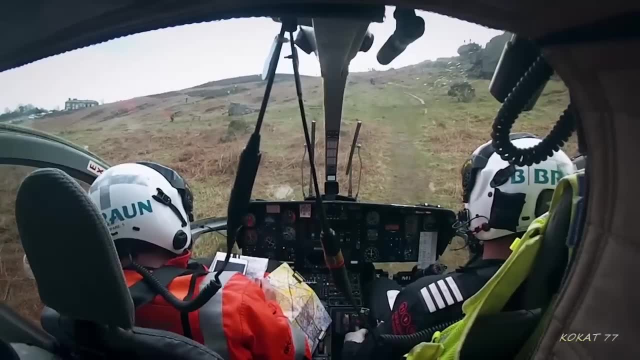 Last time I landed just here and it just worked out wrong. Looks OK this side. Gaz, You happy with this slope and your blades at the front? Yes, mate, yeah, Yeah, OK. Visitor Rob Anderson has a serious head injury. 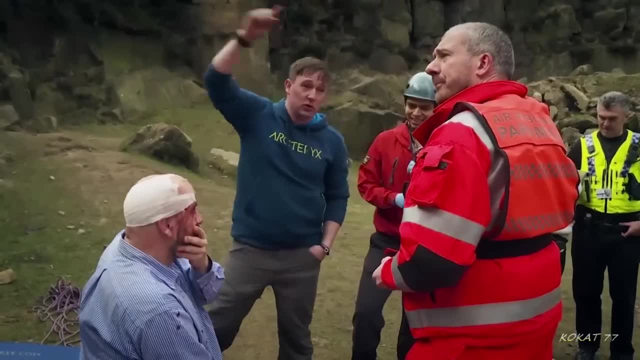 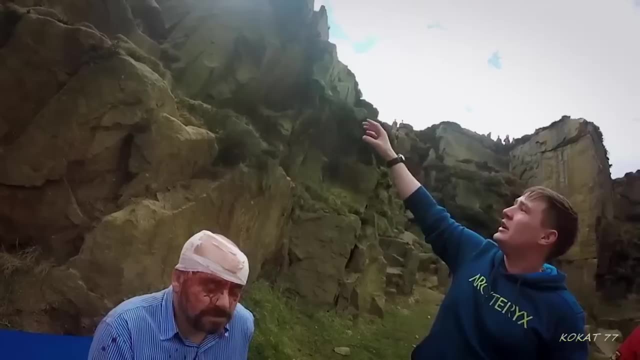 OK, Mountain rescue members are on the scene. We were called from the bottom with our first aid kit. He's falling down, Hit the middle ledge, hit the bottom ledge, so probably 15 foot and on. So he's slipped and bounced a couple of times. 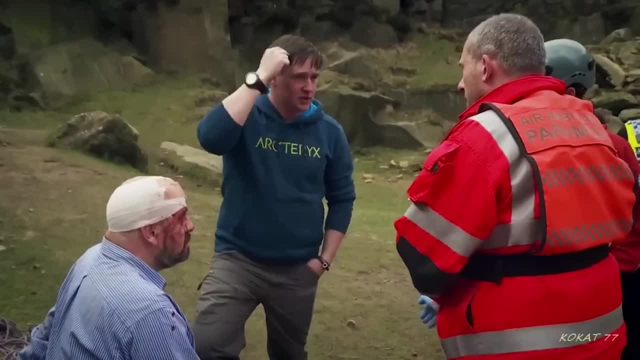 Yeah, he's slipped on his way down, bounced twice, He's got a good four-inch gash in the top of his head down to his skull. OK, We haven't cleaned it in any way, we've just put that on to try and stop the bleeding. 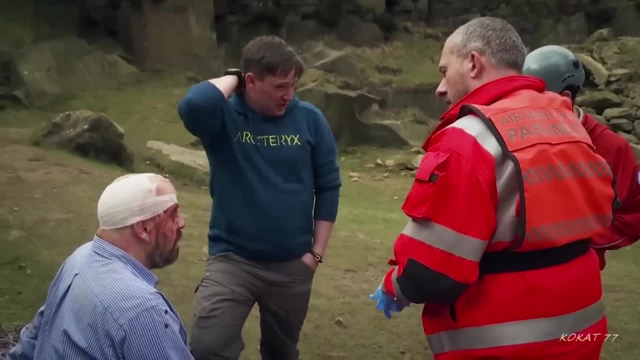 All right, But as you can see, he's bled quite a bit. You been knocked out at all? Doesn't remember being knocked out, but he's got a bit of memories. Was I knocked out? We don't think so. 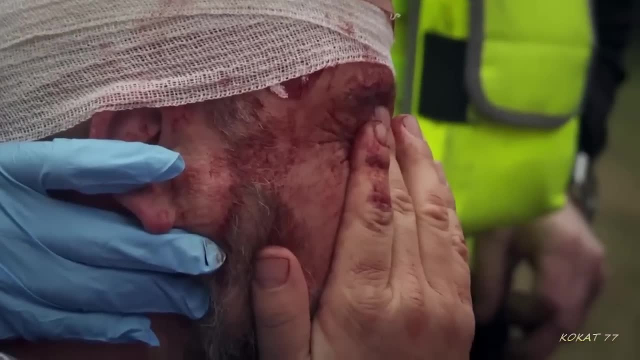 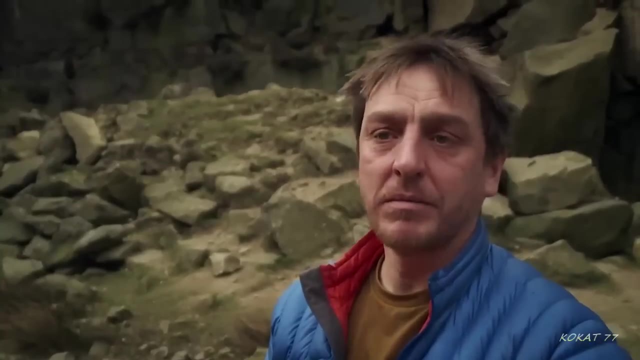 Just keep your head still. Climbers saw him fall As I turned round. he was rolling down the embankment and landed straight on his head. He was conscious, but he obviously was bleeding quite badly, so we just grabbed some tissues and things and tried to save him. 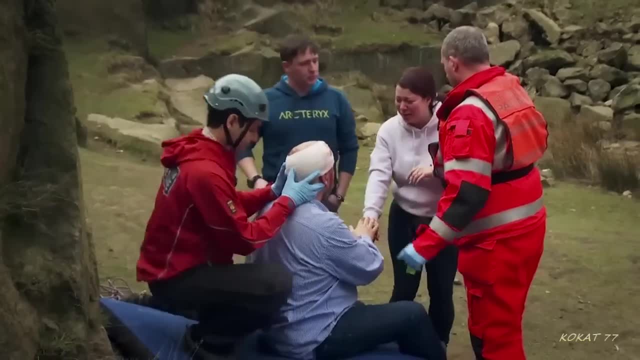 His wife, Melanie, is distraught. You've not fallen as well, have you? No, no, Well, there's no need to cry, He's going to be fine. He's just bumped his head, He'll be all right. 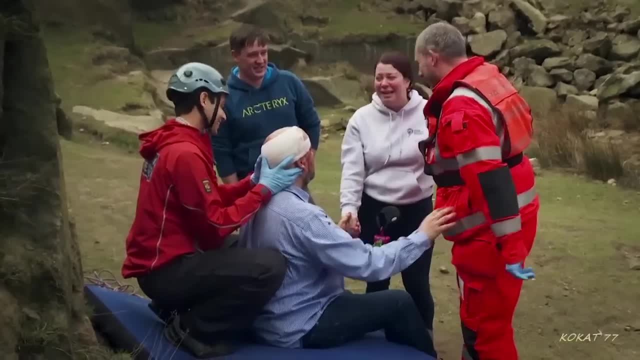 Don't worry about it, He'll be all right. Can I sit down here next to him? Oh, bless you. You all right? Yeah, I think so. Thanks for your help. That's all right. Listen, just keep your head still, sir. 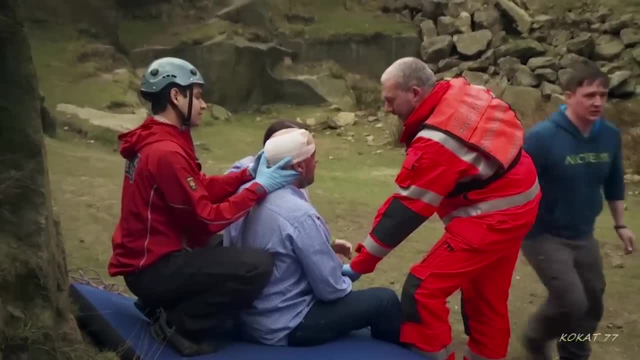 Just look towards me. It's been a terrifying experience. He just kind of like lost his grip and I was like There was no, There was no Hold on to it. That was the problem. Yeah, Were you going up or down? 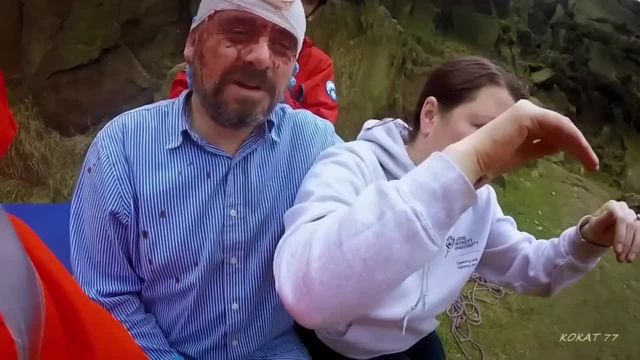 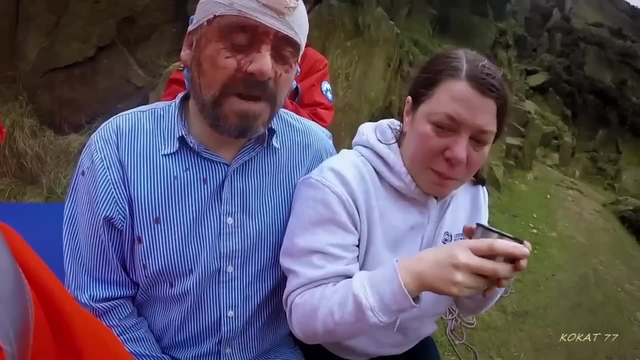 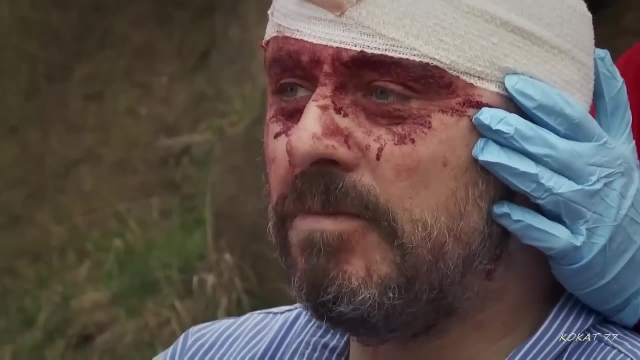 Down, Stupidly down. Thank you, Oh man, Oh Rob. honestly, What were you thinking? What were you thinking? Rob was on a family outing when a lapse of concentration on the rocks led to a fall that could easily have been fatal. 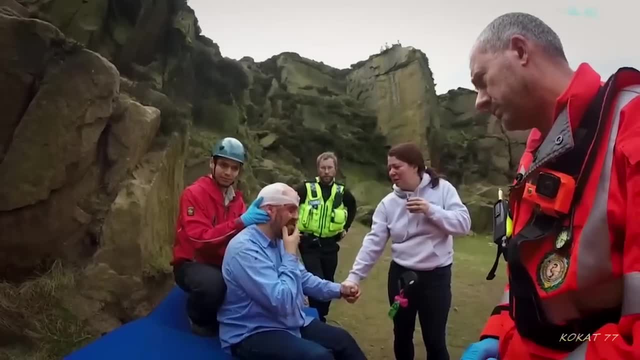 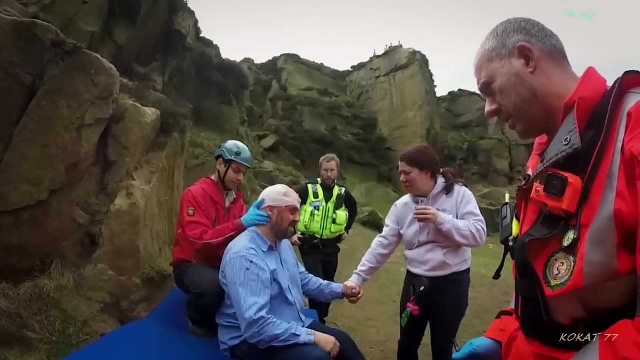 Who's the prime minister? A simple question. A simple question does little to reassure Rob's rescuers. Um is um. Don't tell me It's a sinister sign. That is odd, isn't it? Don't tell me. 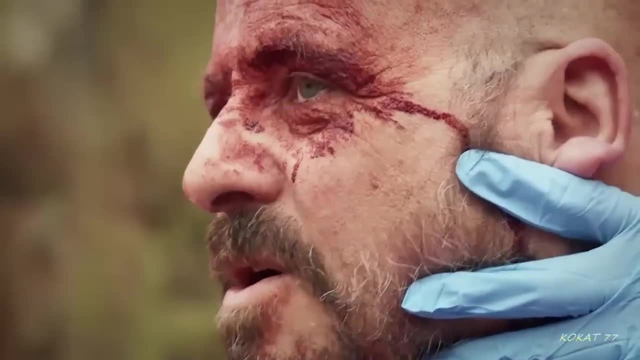 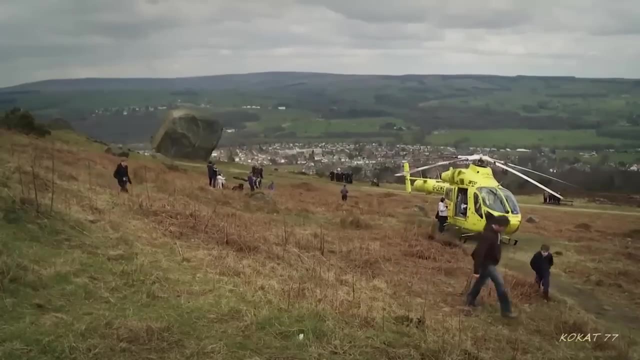 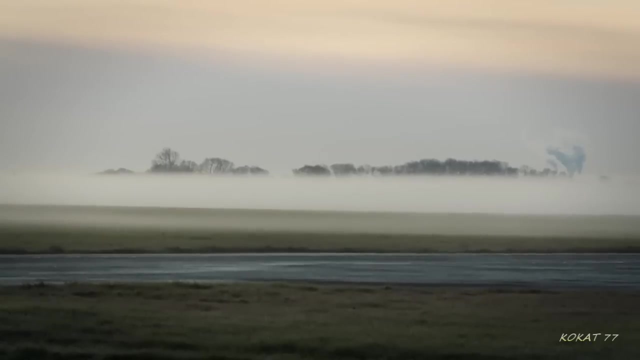 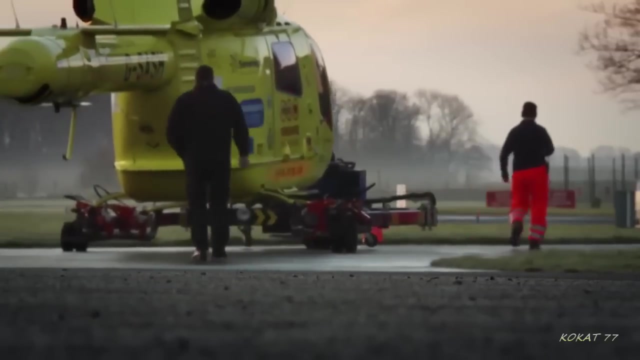 Okay. Al's beginning to suspect a serious brain injury. His patient needs an immediate flight to the trauma unit in Leeds At the Yorkshire Air Ambulance's northern base at Topcliffe. winter has the team in its grip. It's minus five. 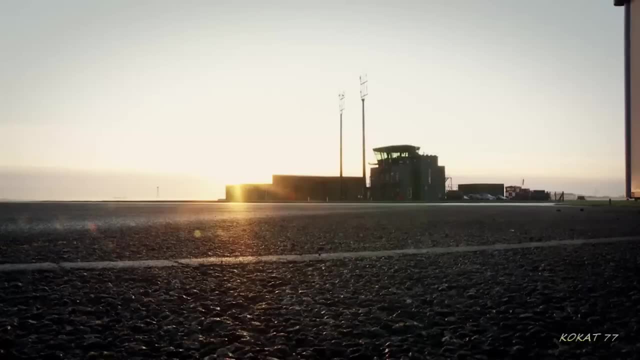 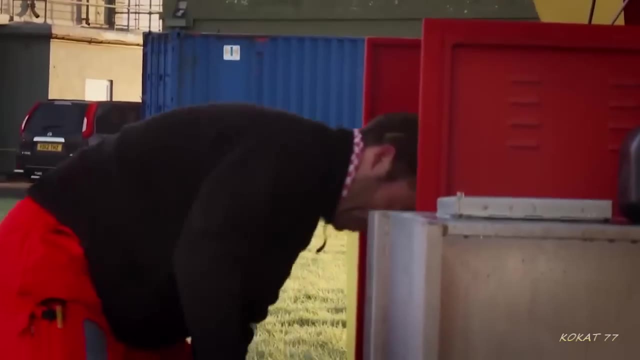 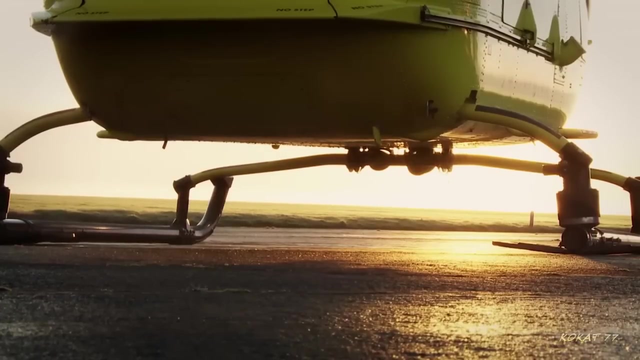 Master FM Today's weather. it'll be bitterly cold and struggling to get above freezing for much of the day, And paramedic Lee Greenwood knows from grim experience that accidents can often be weather related. There's lots of patches of ice, These roads don't thaw out and we could be called out to some unfortunate drivers this morning. 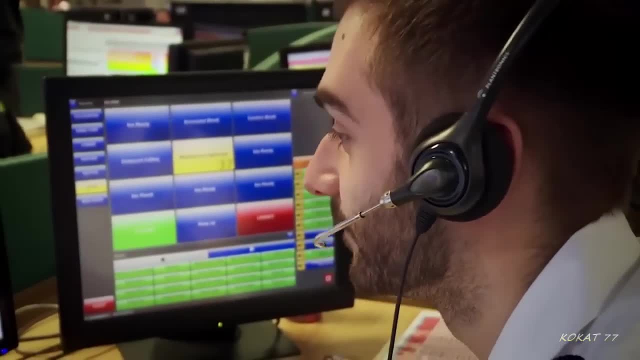 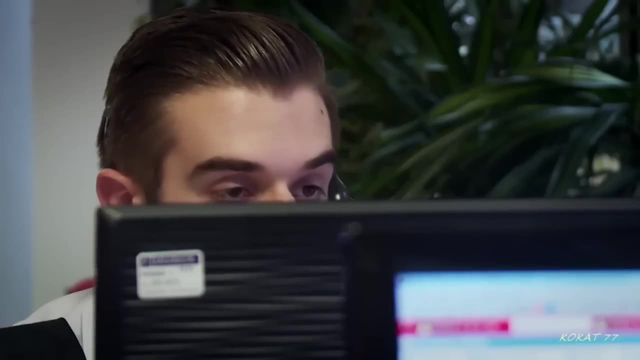 Ambulance service. is the patient breathing? There's been an accident just outside my house. There's a car turned over. Okay, Old view leaving him. Okay, is everyone conscious? Yes, there's somebody inside hanging up by the seat. 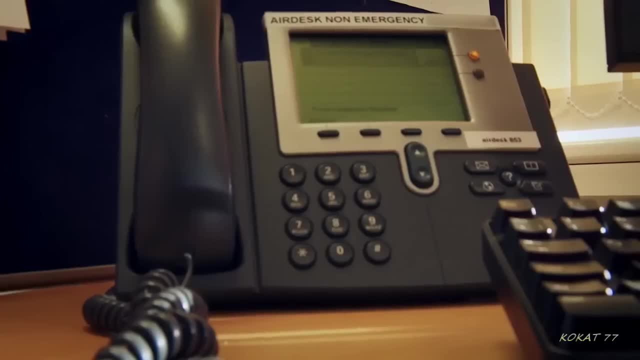 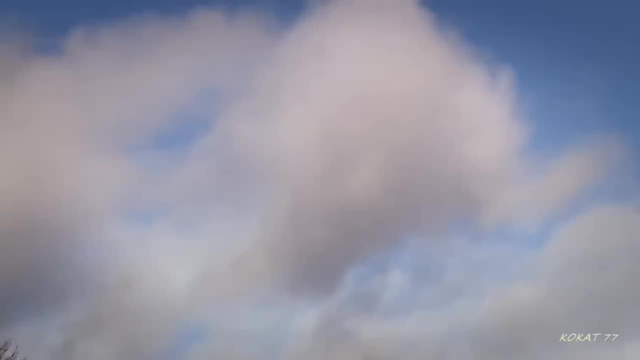 Right, Could you send somebody outside away? Okay, we're already getting the help arranged for you. It takes less than an hour before Lee's instincts are proved right. The emergency call comes from the bottom of a notoriously steep hill in the Yorkshire Woles. 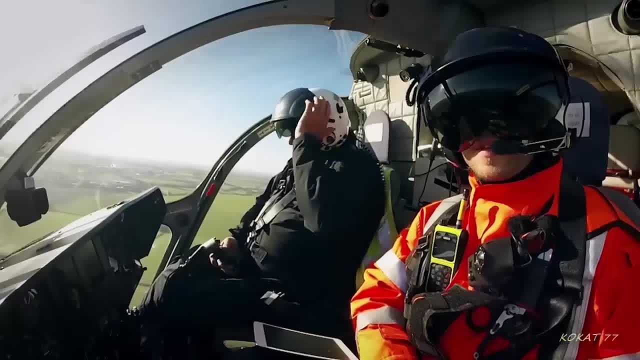 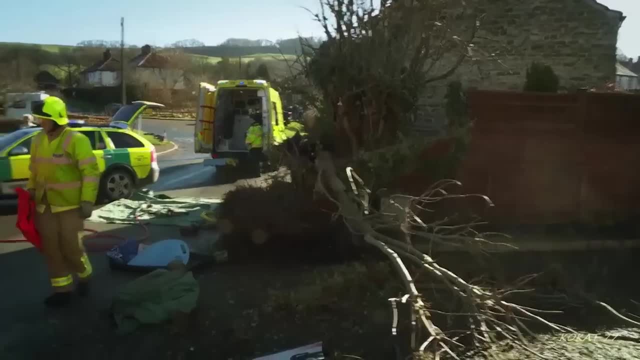 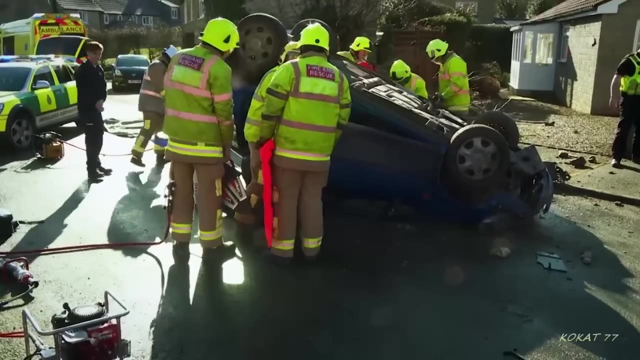 A rolling range of hills east of York, Linton town. good morning. In the small village of Levening a couple in their eighties along with their son are trapped in their car. Paramedic Tony Wilkes knows this could be a difficult case. 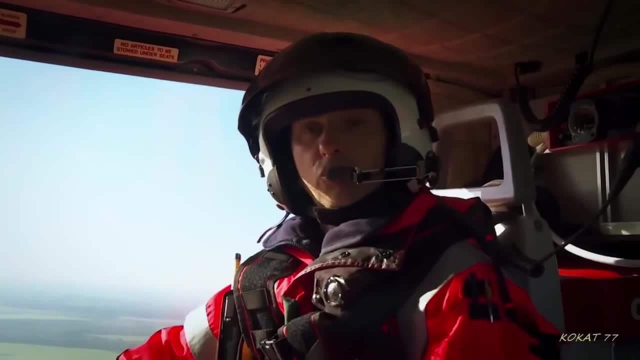 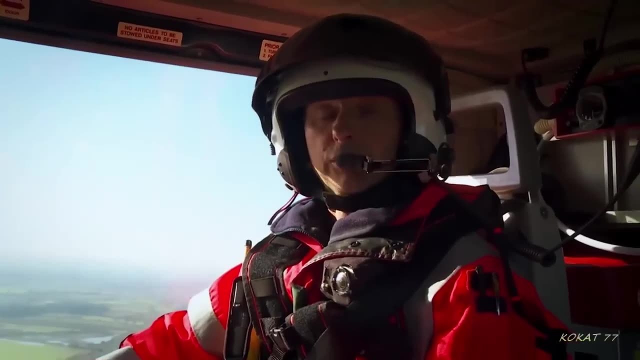 It's like all else with each of us. sometimes they may be trapped, physically trapped, because they can't get out, because they're just stuck or something. So putting these jobs away could be a very serious, life-threatening case. Fire and ambulance teams are at the scene. 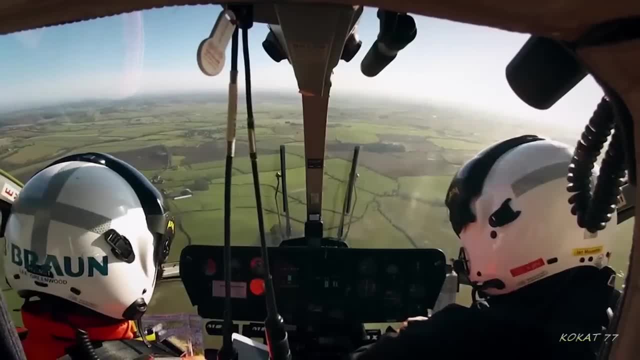 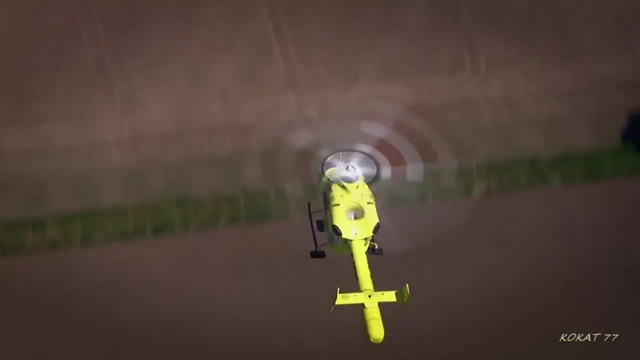 From this location. there's going to be a choice of two hospitals. they can fly the injured patients to: Yeah, Roger York showing at 12, nearest trauma centre Halls at 24.. Got the two lights Right? yeah, we'll get them to the scene on the nose in. 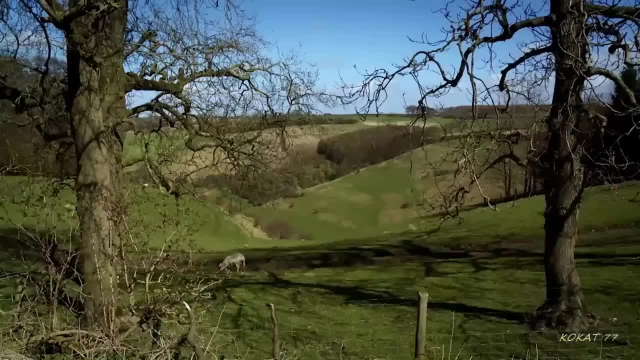 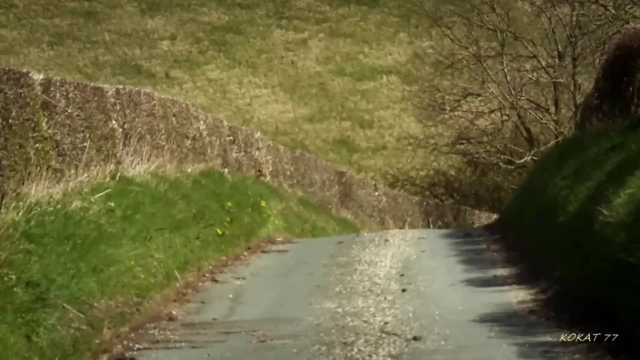 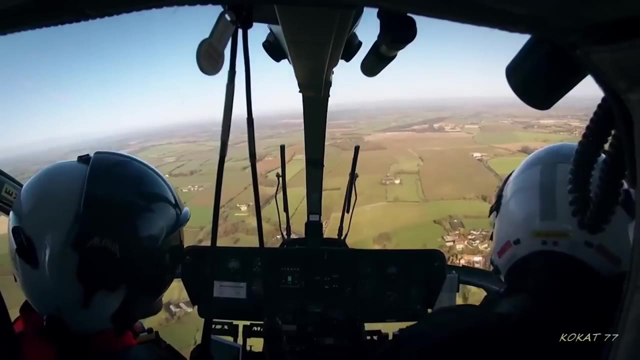 Got it, Yep. The hills are one of the hilliest areas in the county, and the slopes that seem to have contributed to the accident are now presenting a problem for pilot Ian Mouzet. The helicopter has to land on flat ground, The one field there is. it's got a heck of a slope on it. 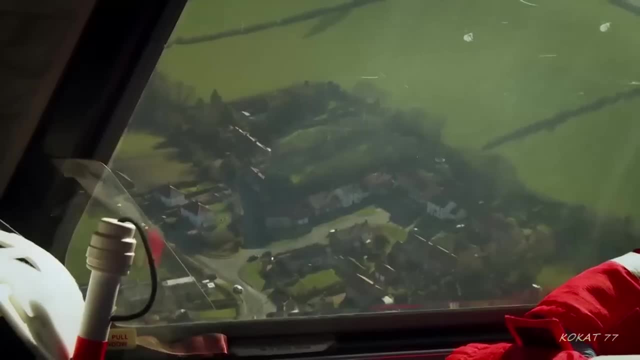 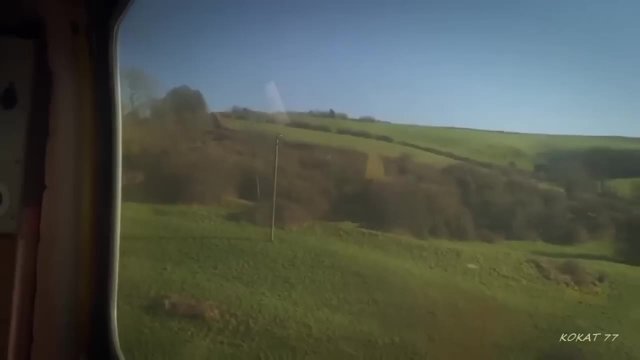 It is three o'clock now, Ian. like there's a little outhouse- The muddiest one, Yeah. yeah, It just looks wet. When a soggy sloping field with nearby power lines is the best option, the final decision to land will only be made after a close inspection. 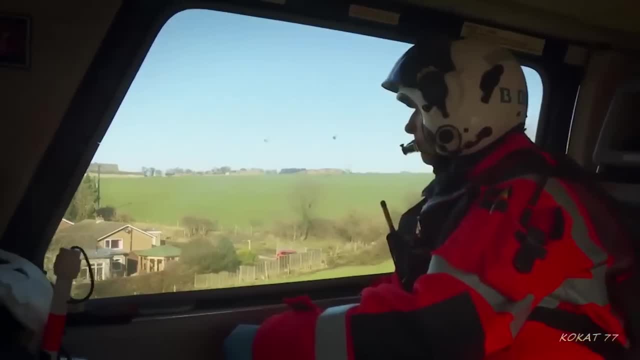 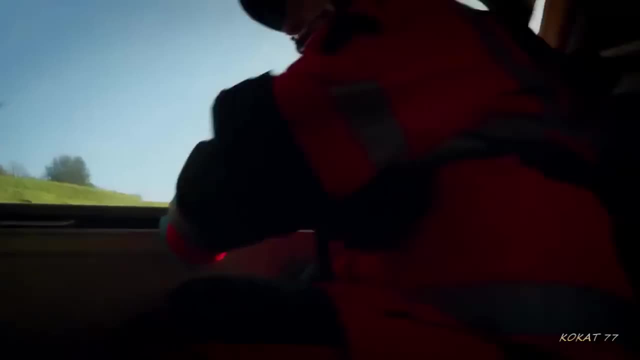 Just bear with me a sec As the helicopter hovers inches from the ground. Tell you what we'll bear. Tony, do you want to get out of here? I will do, mate, Right, Yeah, that's from Helibet 99. now on the ground. 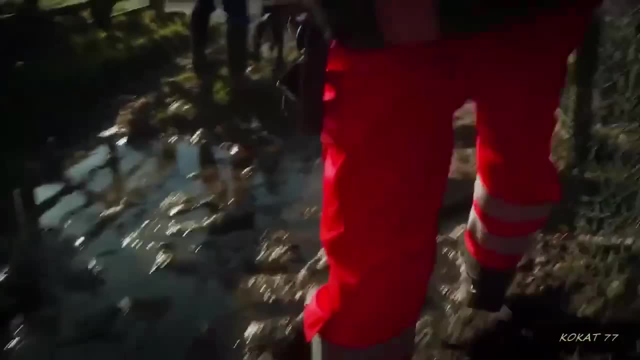 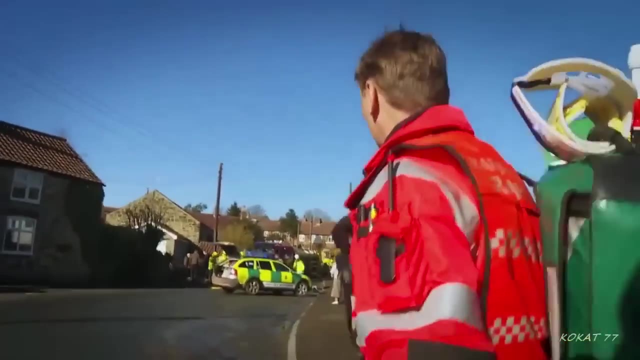 It's really foggy down there. It's all right, mate Spend his life walking through mud, Yeah, so just making his way to the scene. There's obviously an ambulance response vehicle here and an ambulance has just turned up, So we'll just get a quick handover from them. 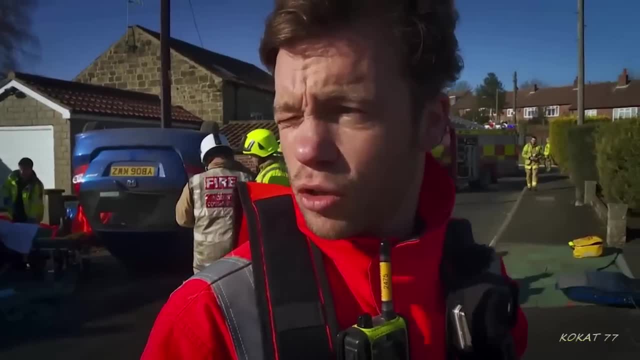 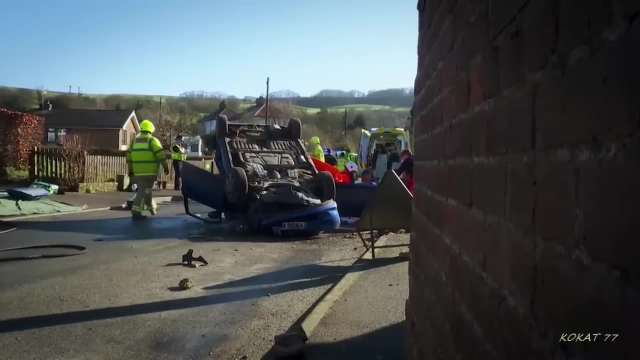 They've come down the hill. It looks like there's a sort of lost control right at the side of the wall which has just rolled the car over. The 80-year-old driver has managed to get himself out of the wrecked car. 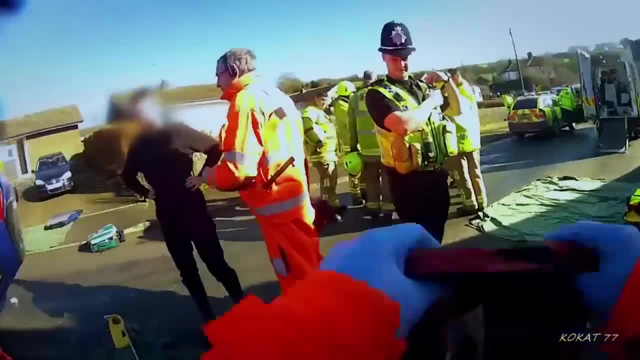 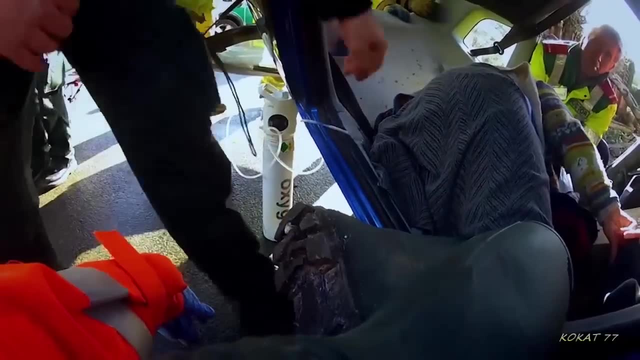 uninjured, along with the man who was travelling in the front passenger seat. But Elizabeth Carroll is in the world. She's in the worst state. I'm just going to have a look at your ribs, OK. She has severe pain in her chest and neck. 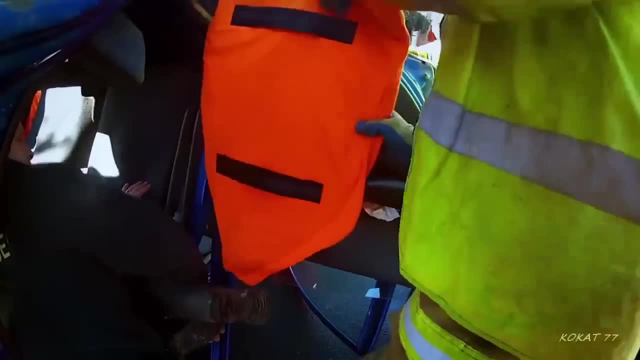 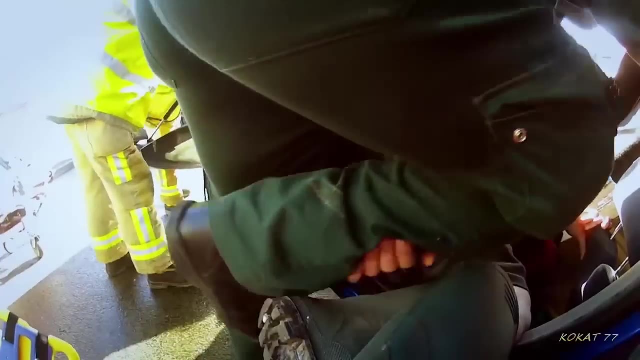 See your spine. That's all I've been told. Firefighters are cutting out parts of the car to make way for a spinal board. Here, mate, Start sliding the board under yourself a little. The size of the car and the way Elizabeth is lying. 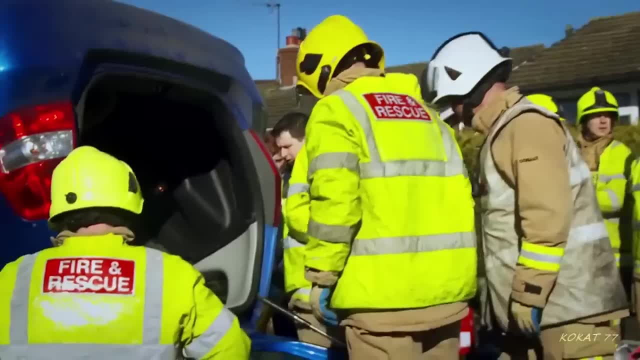 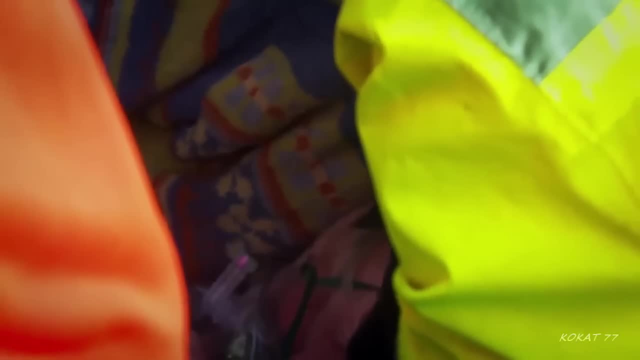 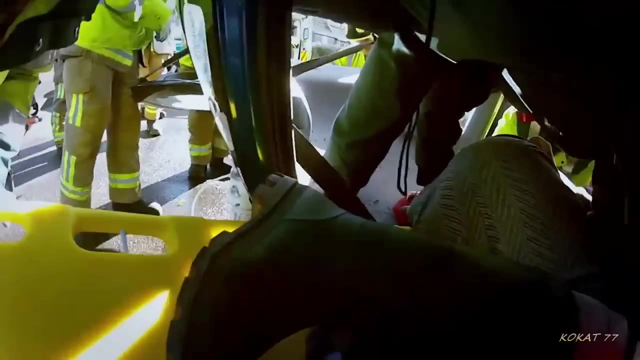 is going to make it difficult to get her out. It's not going to be easy, is it No? For Tony and the other paramedics, the solution is often a combination of dexterity and manpower. Right, I'm stuck on clothing now, mate. 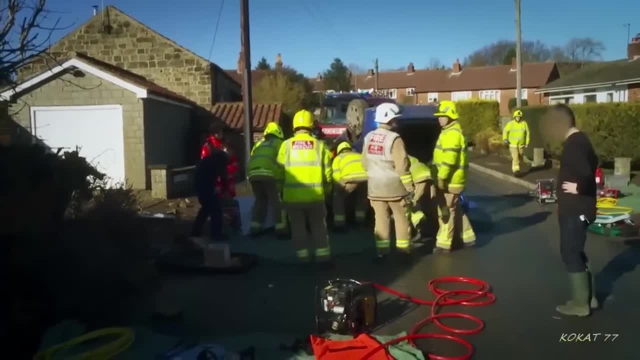 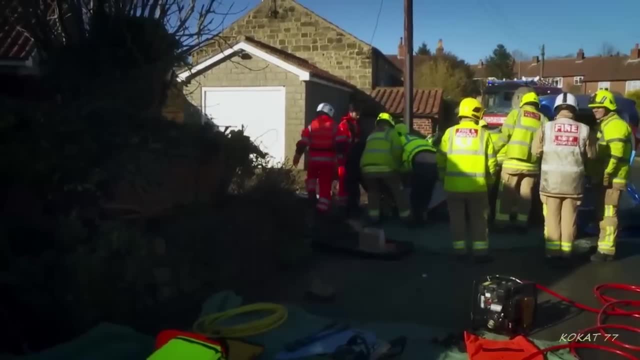 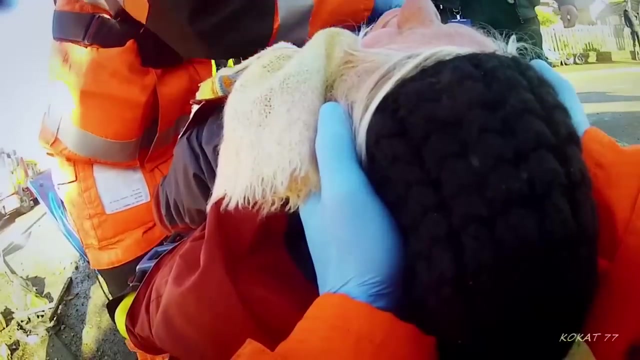 The main priority is to protect the spinal column and head. You got it: I can't breathe, I can't breathe, I can't. It hurts, It hurts. I tell you, Even a shallow breath is hurting. A shallow breath is hurting. 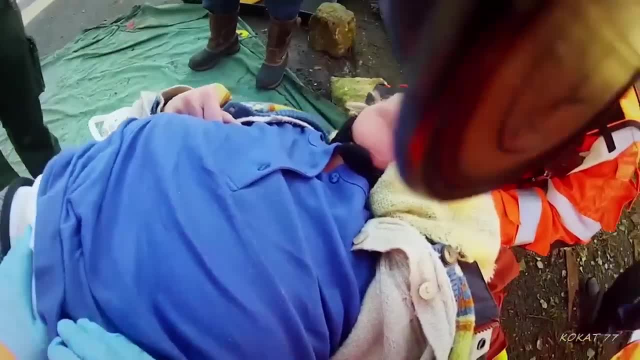 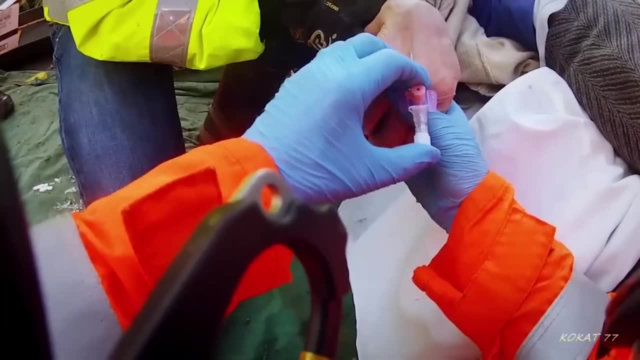 Is it where you're putting your hand? Yes, What about your tummy? That's all very uncomfortable, actually, Everything's uncomfortable. Shall we have staff coming up, sweetheart, Why? Just so we can give you some pain relief, Make you a bit more comfortable, that's all. 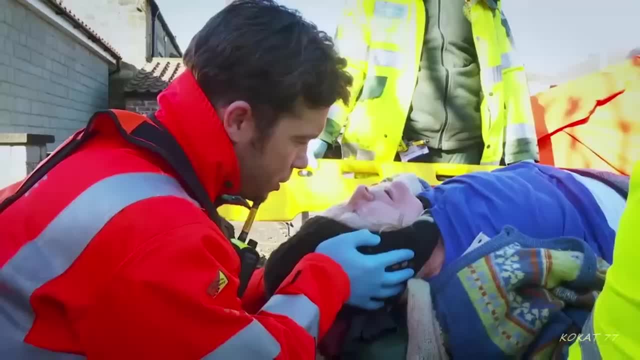 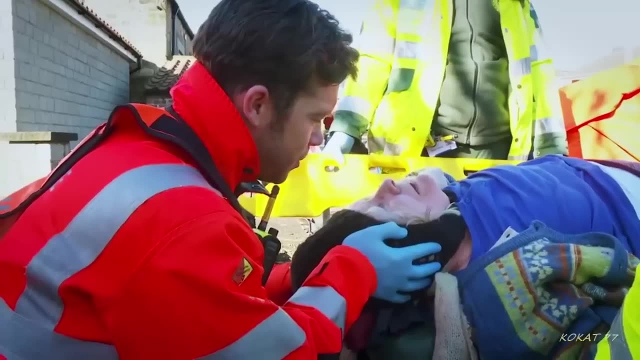 You're probably going to have to trip to the hospital to see some of the doctors. OK, Yeah, OK, The important thing is: you remember everything that happened, don't you? No, You don't remember anything that happened. No, What do you mean? I don't remember the accident. 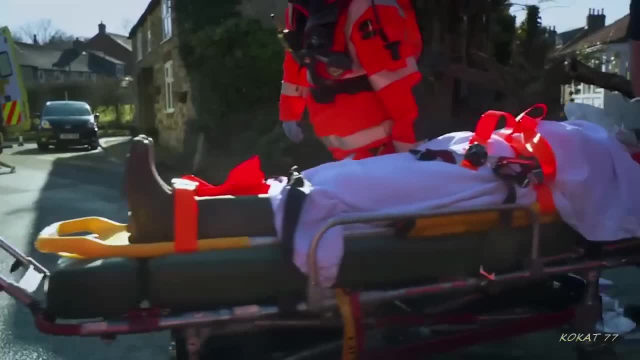 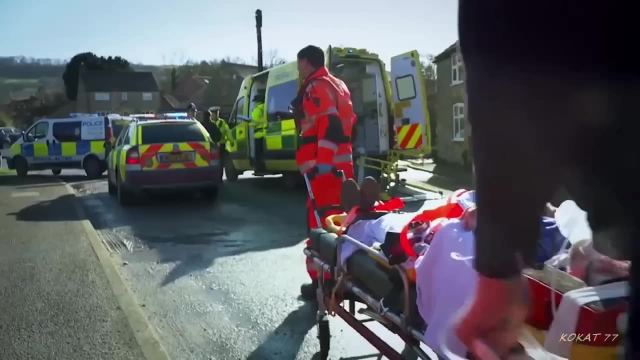 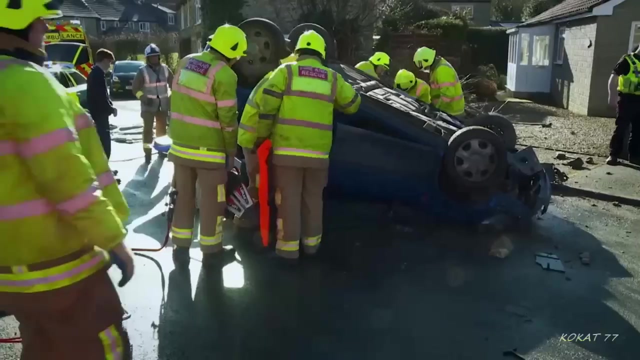 You don't remember the accident. No, Elizabeth has appeared lucid for most of her ordeal, but her memory loss means she may have a brain injury. She's going to be flown to Hull Royal Infirmary. It's a moment of relief for Elizabeth's rescuers. 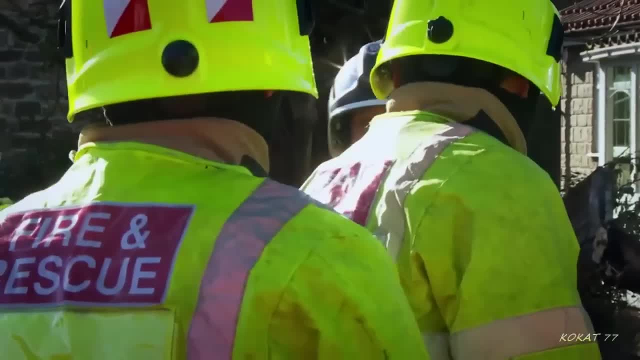 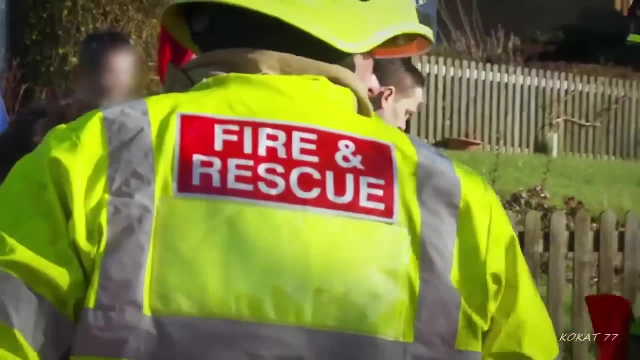 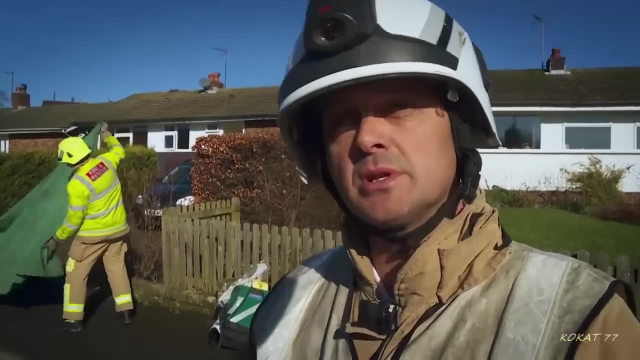 Many of the firefighters are local part-timers and this has been a tough rescue. A modern car, great safety features, but the old cars present different issues and problems. We've got all-time and routine appliances from mall to appliances. They use various cutting equipment, stabilisation equipment. 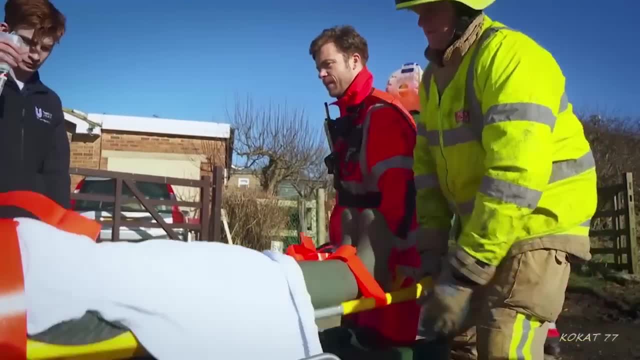 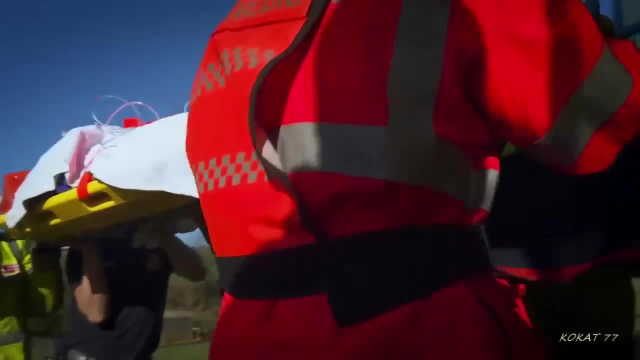 to extricate the casualty. We might need a few firemen to give us a hand, because it's like a club night up there. It's time for Elizabeth to say goodbye to the local paramedic who's been by her side throughout. Elizabeth, Yes. 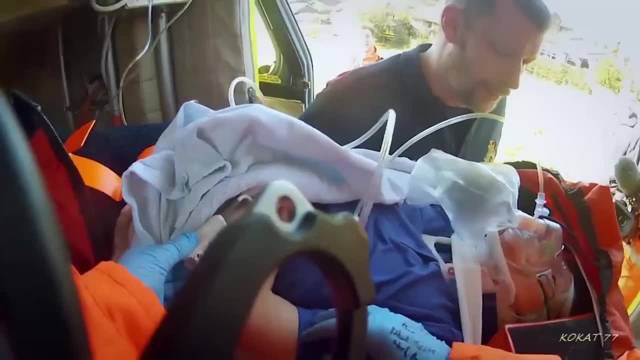 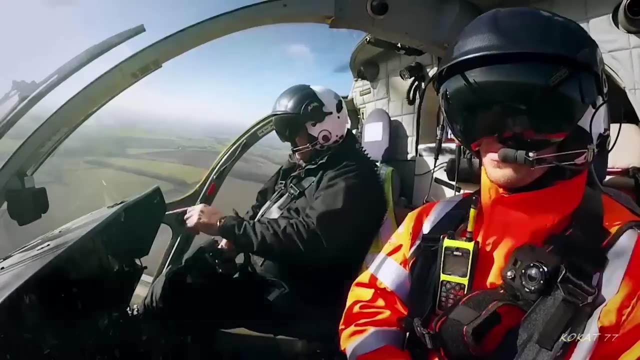 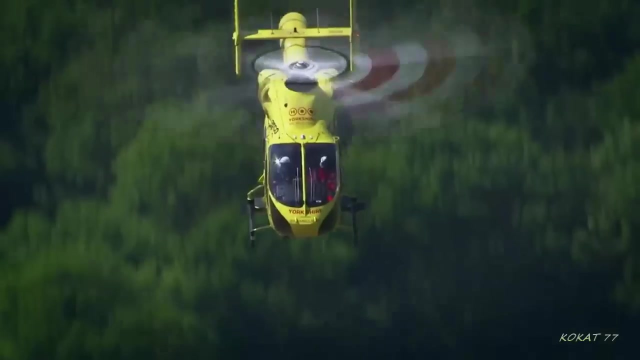 I'm going to leave you with these lovely flying boys now. Thank you for all your help. OK, You take care. Enjoy the flight. The trauma unit is already on alert for their patient's arrival. Elderly people are less able to recover from major injuries. 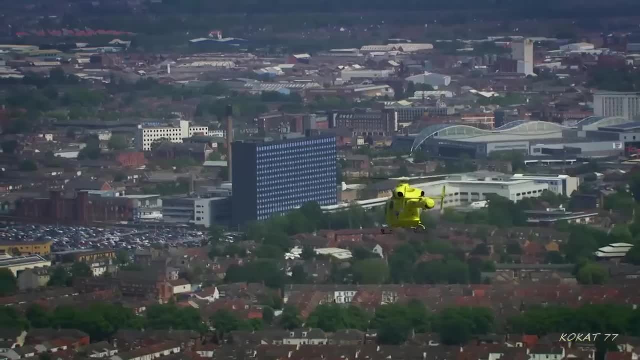 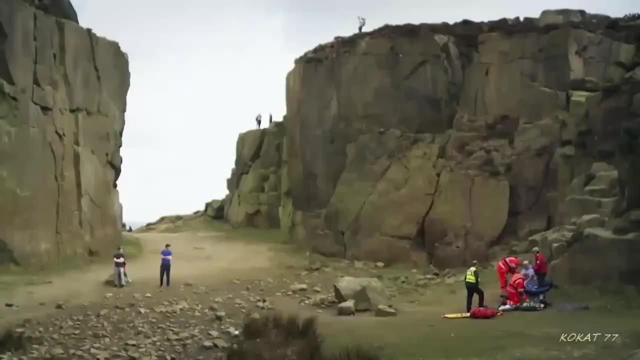 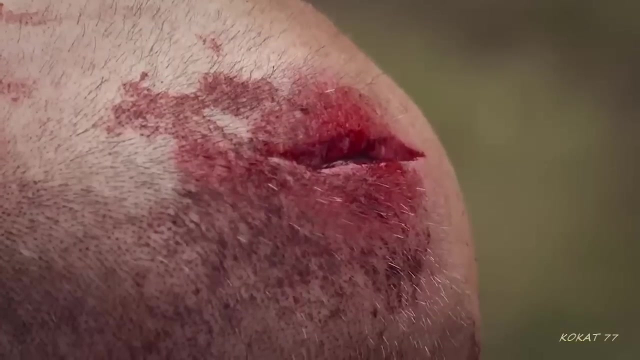 and more likely to develop complications. Elizabeth's will be a complicated case and the next 24 hours will be critical. Back at the Cow and Calf Rocks on Ilkley Moor, the team's patient is causing concern for paramedics- Alan John. 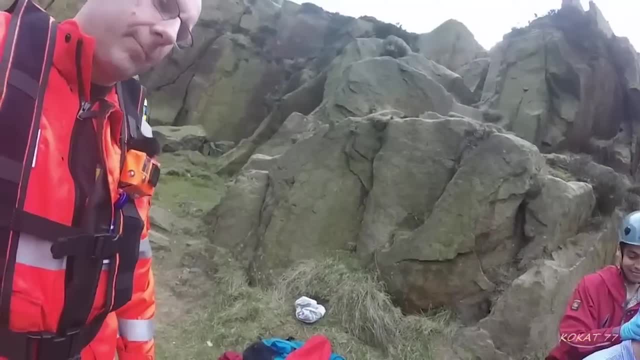 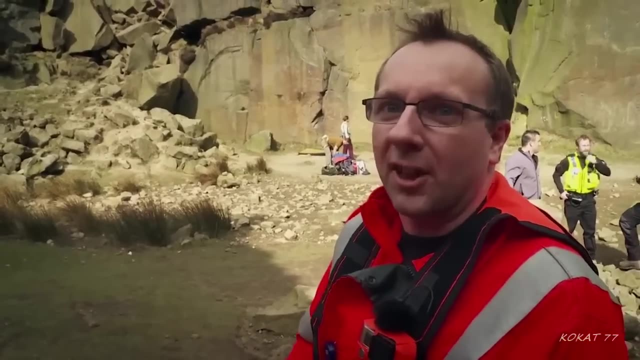 Don't worry about it, It's all right. Very good, I think A bit of concussing too Probably should have brought him somewhere. He can't remember that the Prime Minister's David Cameron, which I wish I couldn't remember as well, but I can. 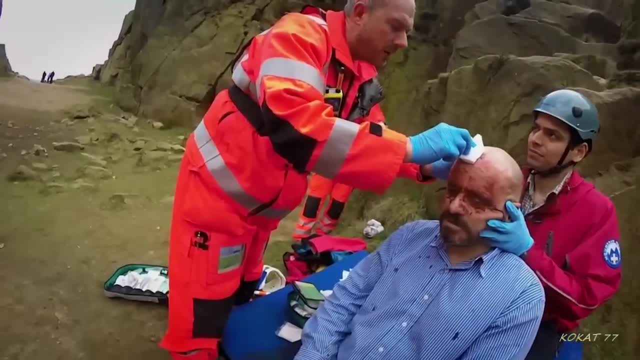 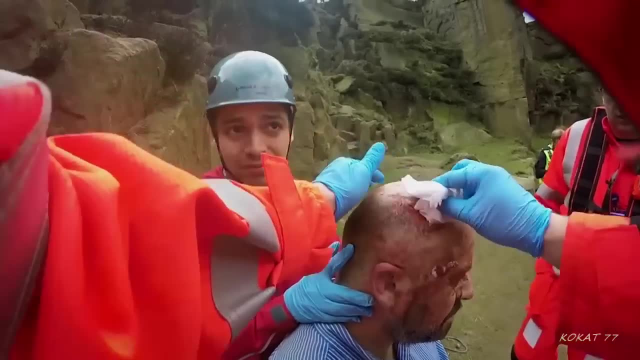 This is just Rob's head wound is through to the bone. I can see the skull there. It doesn't look like there's any. I'm going to be sick. Al is making light of the injury. Stop talking about your skull. 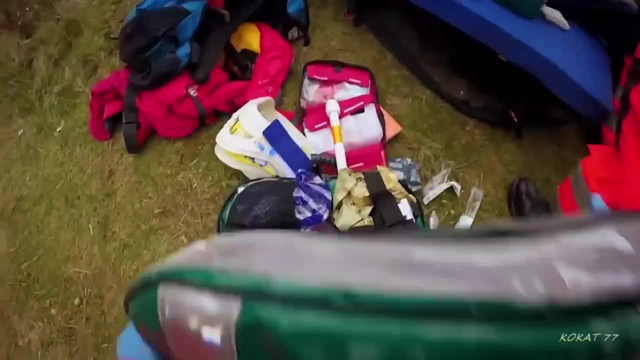 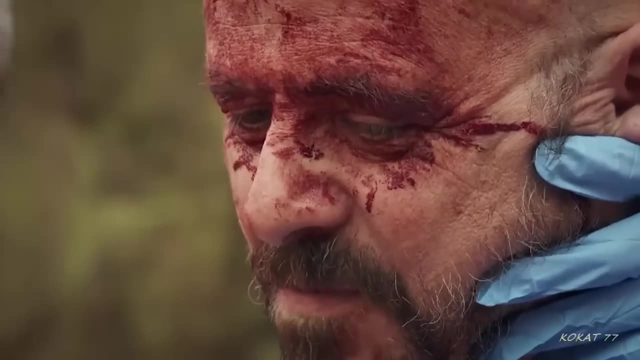 But it's potentially very serious. It's starting to hurt, My head's starting to hurt a bit And Rob's new symptom is very worrying. Did it hurt when you? No, I've heard more. now The pain's coming in. 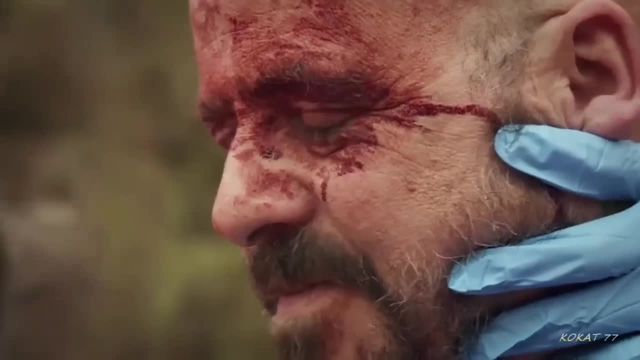 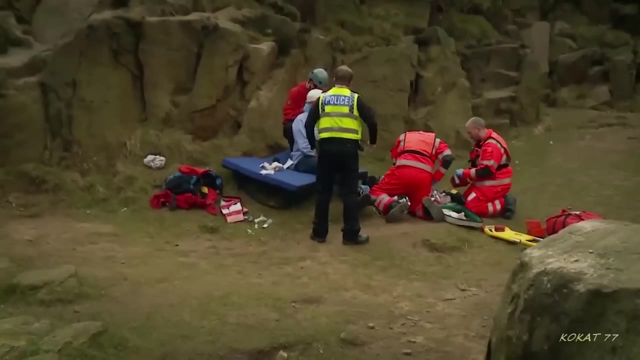 The team want Rob to undergo brain scans as soon as possible. Just relax your hand. Al's asking the police to conscript some helpers. Do you want to go and see if you can round up a few of them- army lads from down there to do the carry? 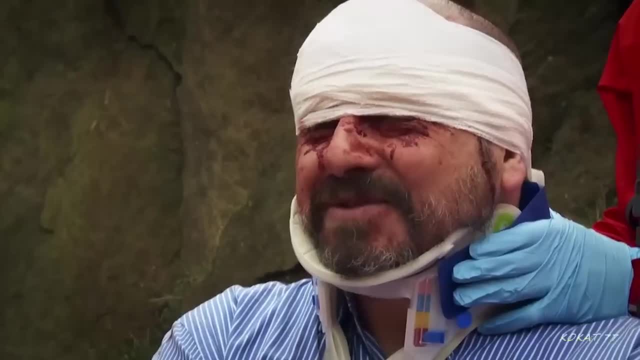 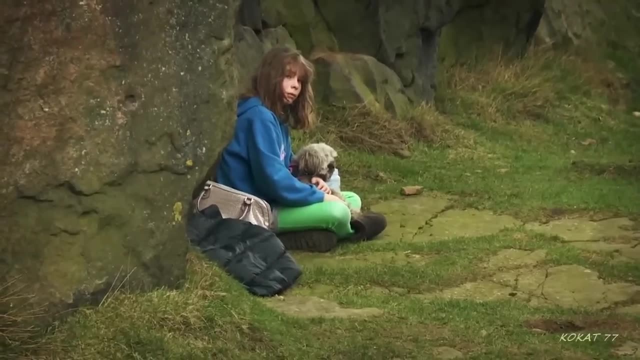 Yeah, Yeah. Well, it's a lovely day. I came up with my wife and ten-year-old daughter, Thought we'd go down to that cafe Rather than walk round. I was just climbing around the rock looking for a foothold. 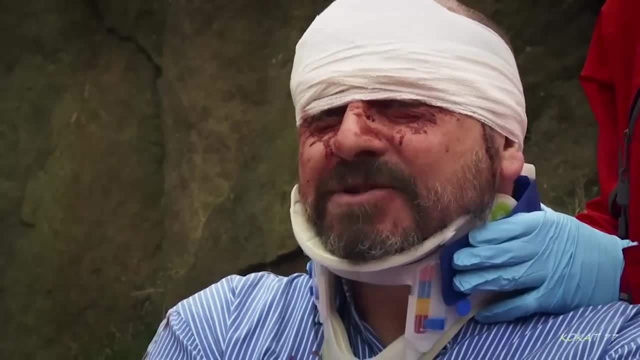 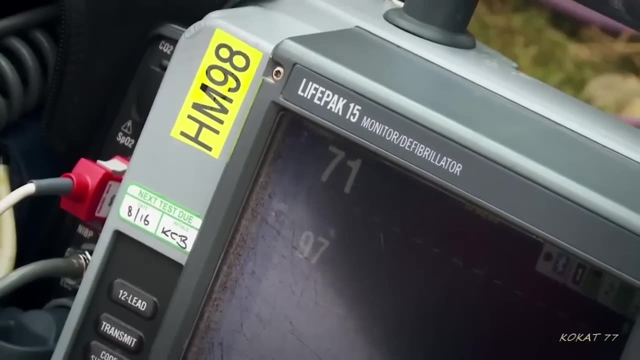 I put my hand out and there was actually something. there was nothing there to grab And I think I just fell backwards. I don't remember anything else. really, A day out from hell, really, it's turning into. It felt like he hit something at the midway point. 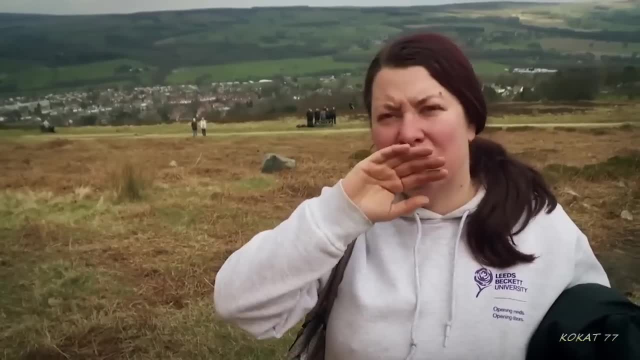 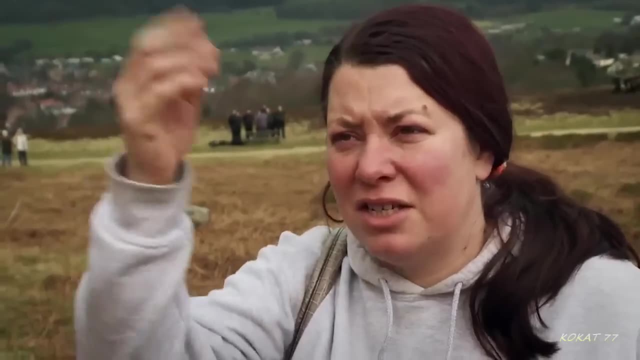 and then just ended up flat on his stomach And it was just, it was horrible, It was very shocking, It was just such a blur. It just happened so quickly, Because the immediate panic is especially when it's a head injury. 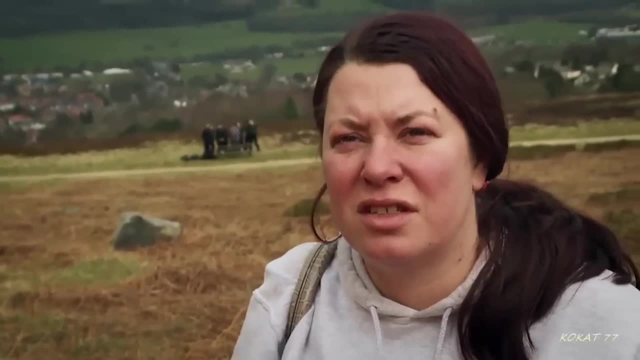 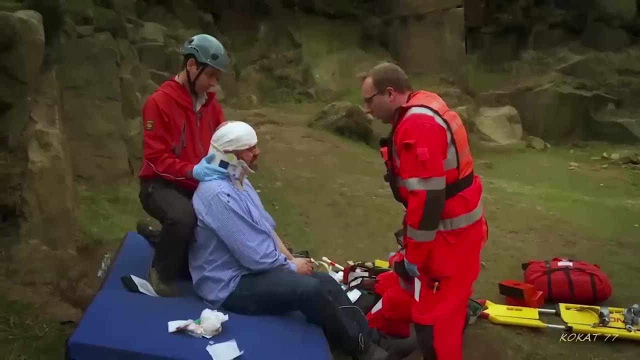 it looks ten times worse than hopefully potentially it is. So it was just a big, horrible shock. We can't really rule out whether you've hurt your neck. I don't really suspect you have, but just precautionary. I appreciate that, Thank you. 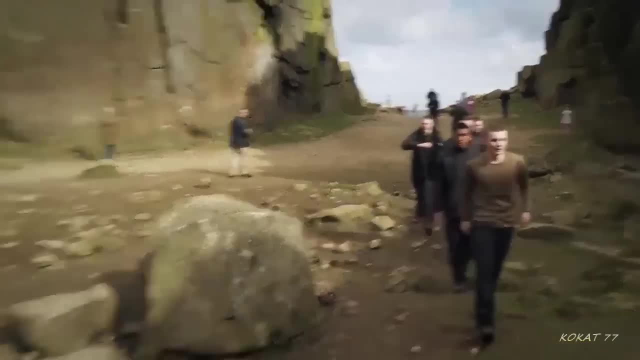 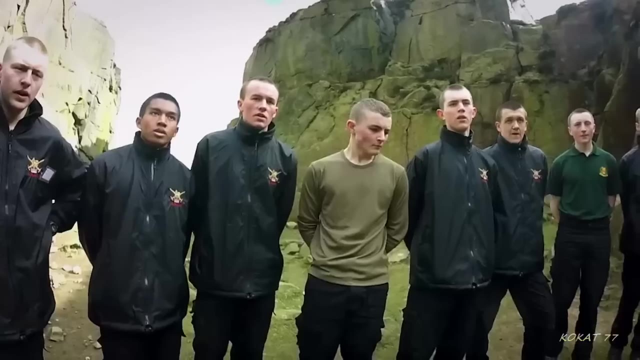 The army lads are getting their orders. Hey, what we're going to do is this: is Rob all right? He's fallen. We could do with your help to help carry him. Is that all right? Yes, sir, I'm not sir, You don't have to call me sir. 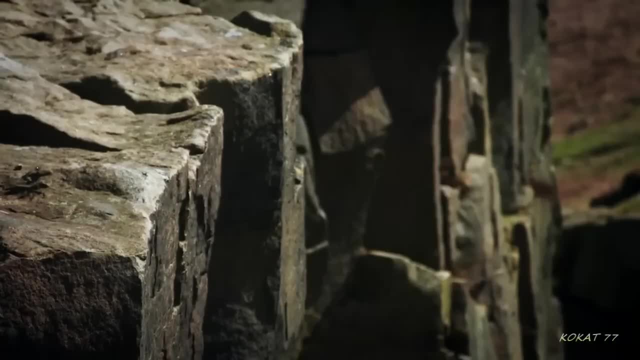 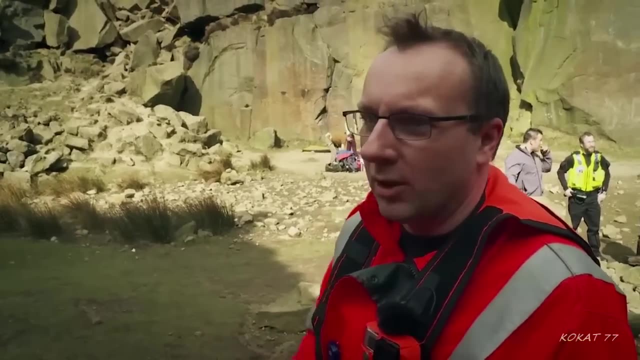 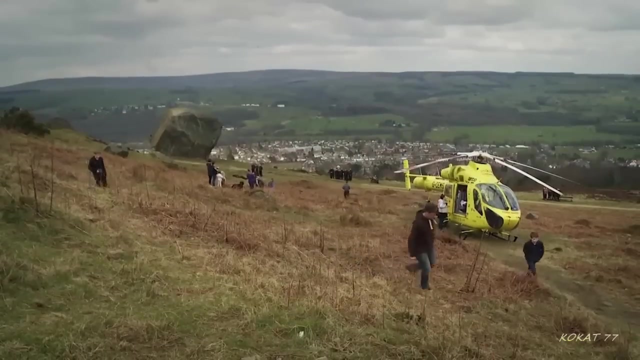 OK, But getting Rob through the rocks and down to the helicopter is going to be far from easy. Quite a crack to his head. So we can't rule out a neck injury and he's still not fully with it. He's still a long way from the hospital treatment he desperately needs. 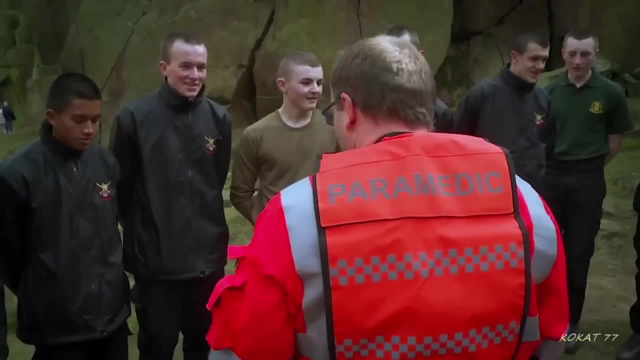 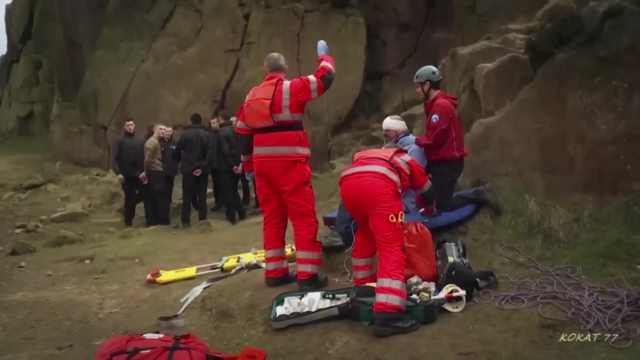 On the rugged edge of Ilkley Moor, the helimed team have enlisted the help of a squad of young soldiers in a difficult rescue. Can I borrow the tallest one of you lads for a minute? The army apprentices came here to learn the ropes of climbing. 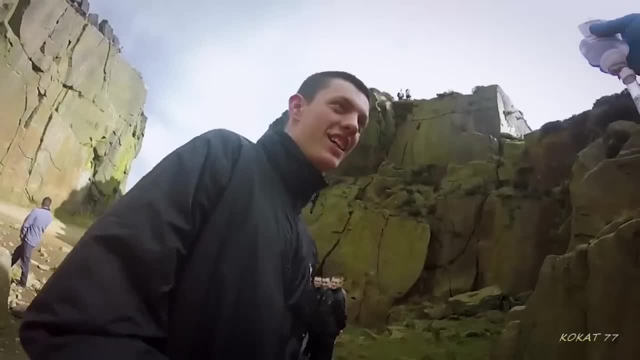 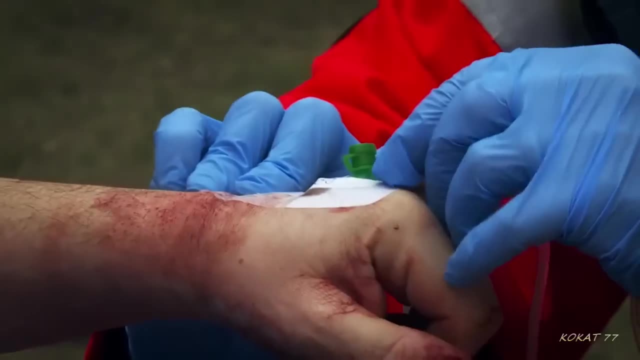 Right, you're Delta Sierra now. OK, That's drip stand. Now they could be able to climb. Now they could be helping save injured day-tripper Rob's life. We're just going to give him some pain relief and get him down onto our stretcher. 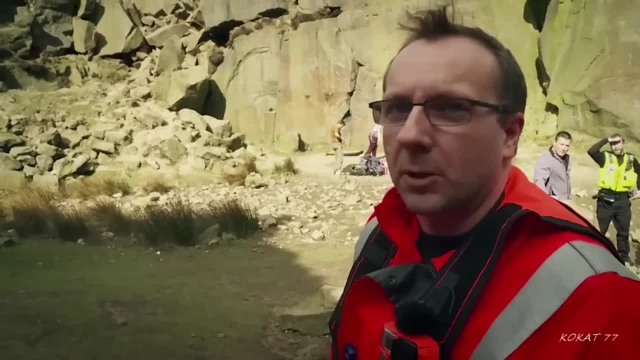 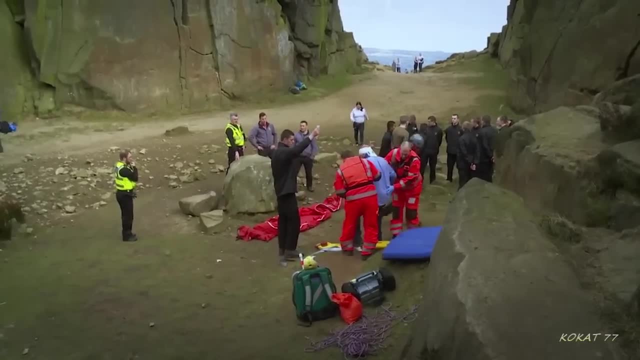 and carry him down to the helicopter and take him to the local hospital, which happens to be the trauma centre LGI. Now just sit yourself down, OK. OK, your head's going back down. We're going to lower you down, OK. 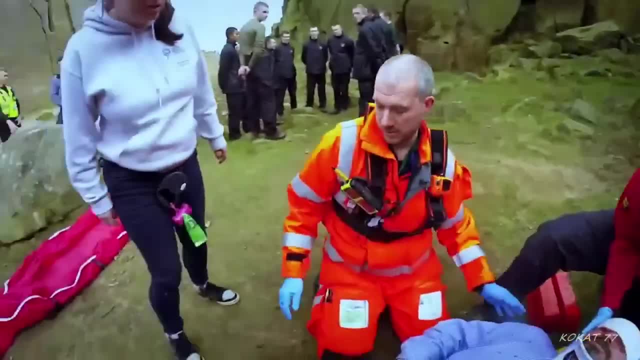 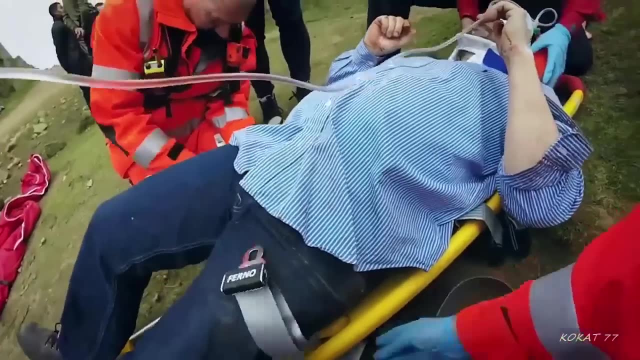 I'll do. you Just take your time. Yes, lovely, Well done, Doing all right, Great, Yeah, he's fine. No change, Nothing to worry about. You see, you'll never complain about paying for your taxes, ever again. 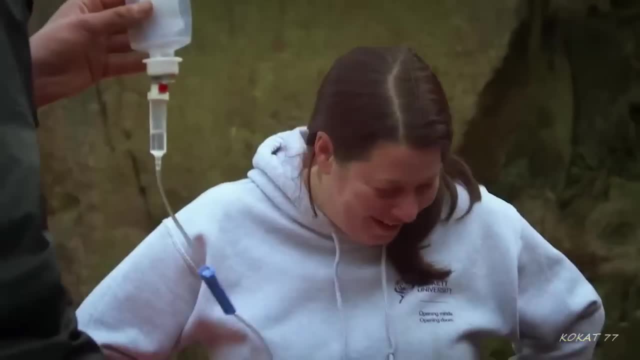 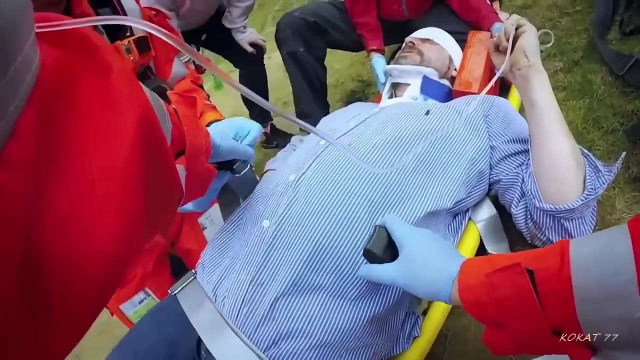 will you Just relax You all right. All right, see, I've got an outstanding tax bill. I'll pay it Monday morning. Yeah, Oh, look, you're causing them problems. love, You're a bit fat, No, no, it's cool, isn't it? 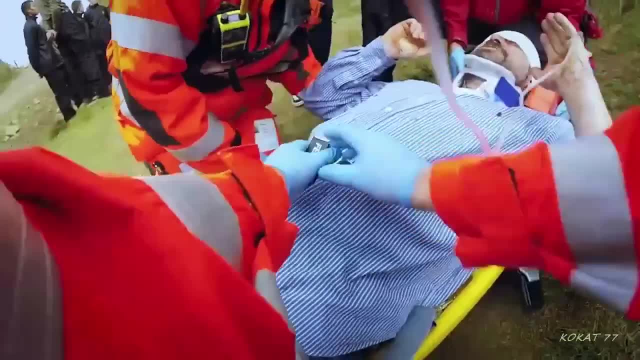 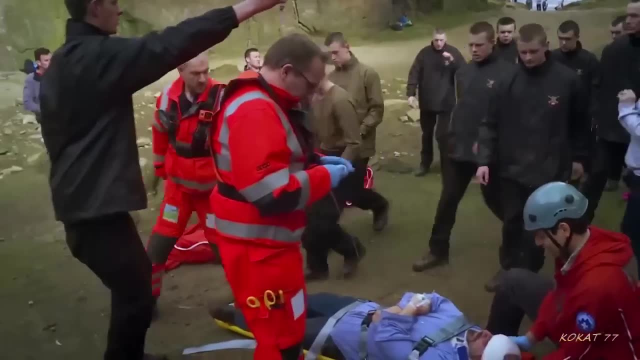 Yeah, don't listen to her, We're going to need a bigger stretcher. Right guys, can we get you round this yellow stretcher now? Six to six of you will probably be enough, Despite the banter. there's no time to waste. 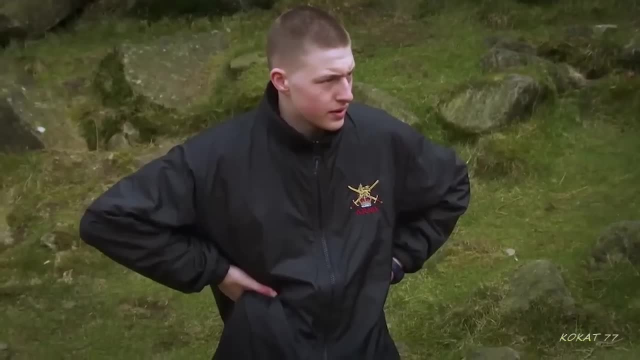 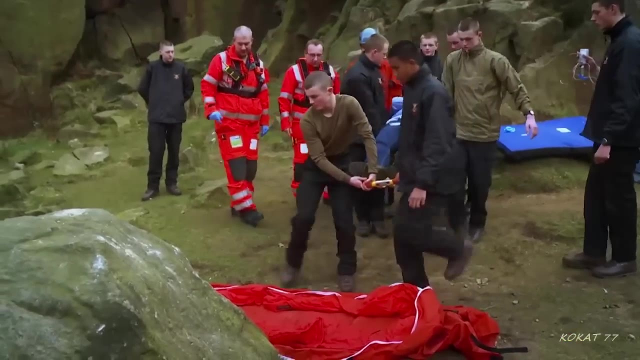 If Rob has a brain injury, speed is essential. All right on call, Ready, steady lift. This is all right. Can we underslung load for these all time? I'm 90% certain it won't be anything to be concerned about. 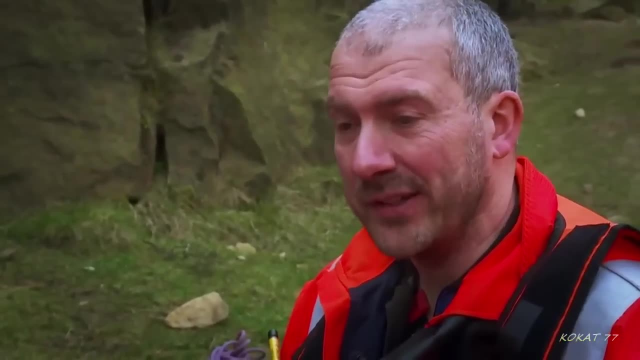 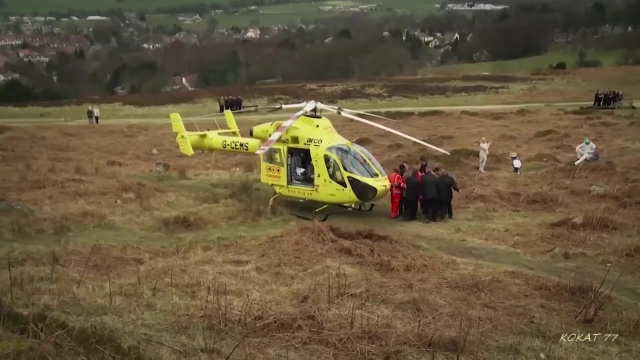 but he has fallen quite a long way and he has landed on his head. so we need to just be a bit careful, just to be on the same side. really, In we come. I'm just lowering him a bit now. That's high enough. 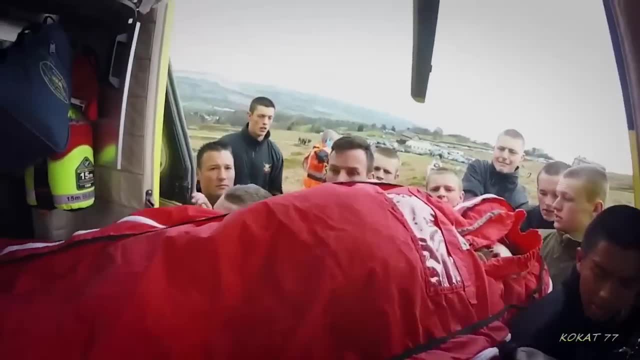 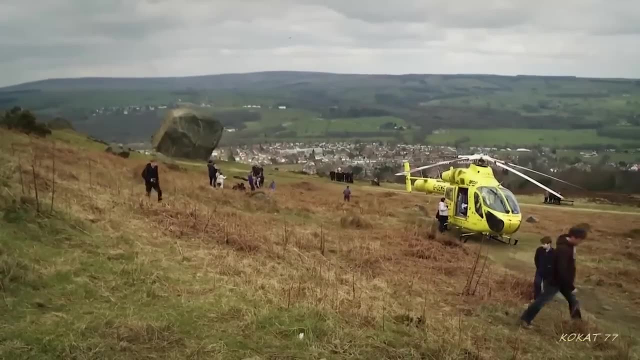 All right, Rob's going to be flown direct to the trauma unit ten miles away in Leeds. All right, Rob. Yeah, fine, mate, Yeah, Yeah fine. If he hadn't fallen for 15 foot, I'd have got some needle and thread out of the bag in the back. 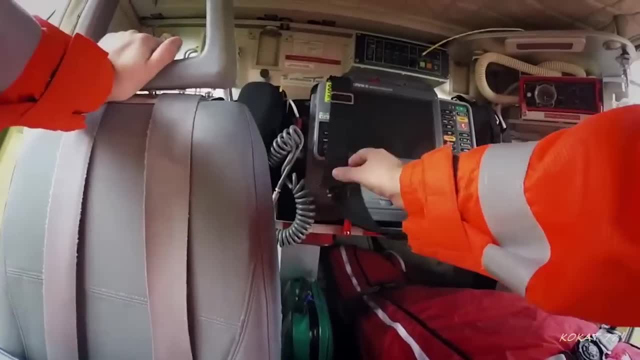 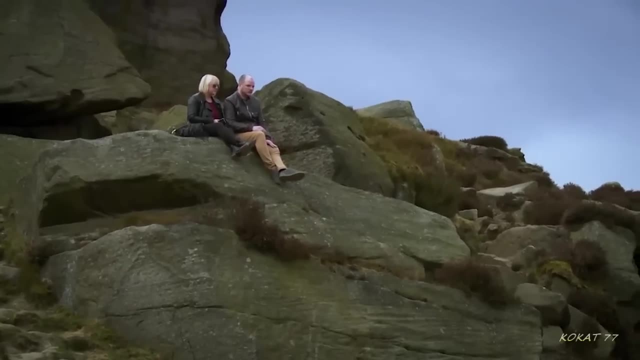 sewn it up and sent him home. I tell you what I've got nagging right now. You always have nagging right. The rescue's been seen by hundreds of visitors to the rocks. Cleared to land, Cleared to land. 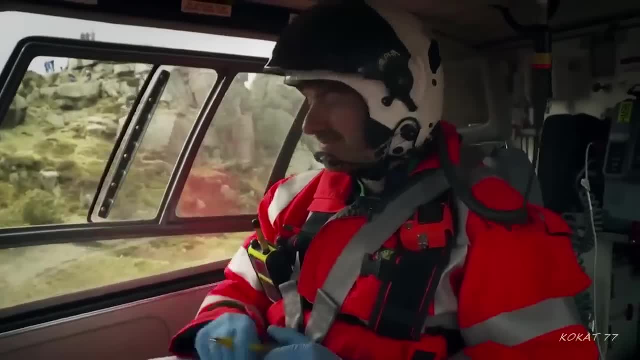 Hello. Helimed 98,. Hopper Helimed 98. South Leeds. good afternoon Helimed 98,. Hopper Helimed 98, that's us lifted from Caracopp, Hillclay 5 on board now. 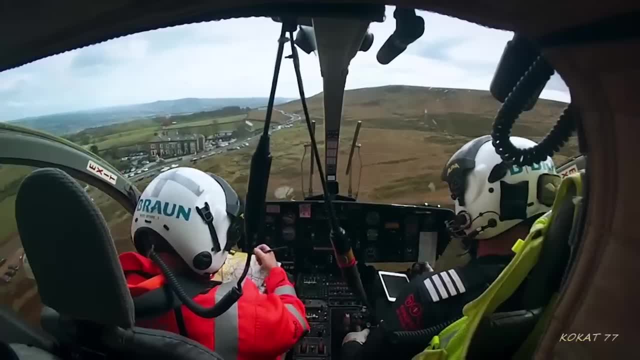 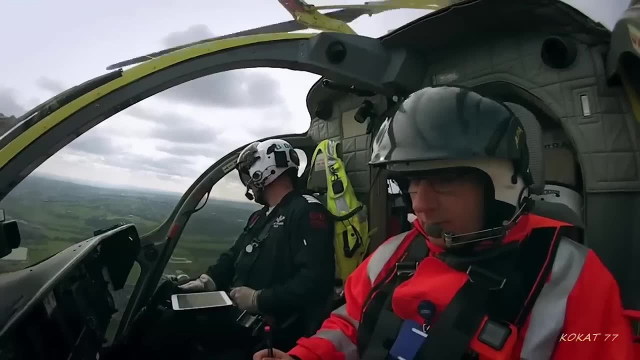 routing El Jai: Cleared to land. Cleared to land: Helimed 98 will be landing in the heart of Leeds, Helimed 98. That's us two minutes out from the North. Landing here is not without risk, Roger, that. 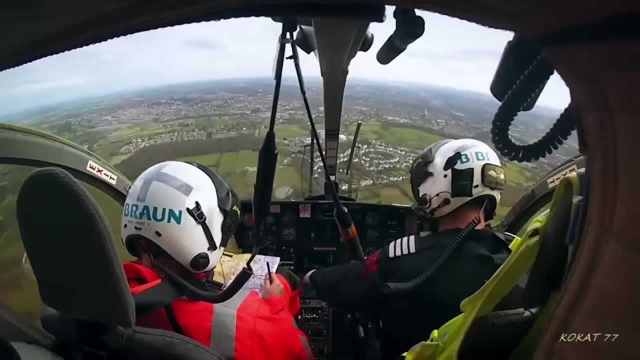 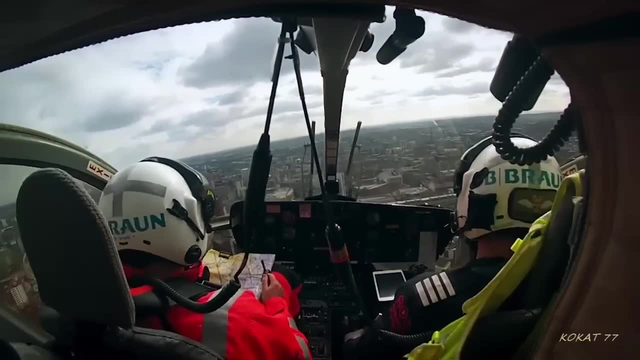 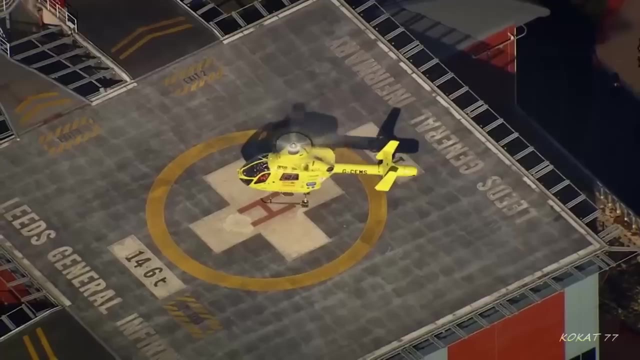 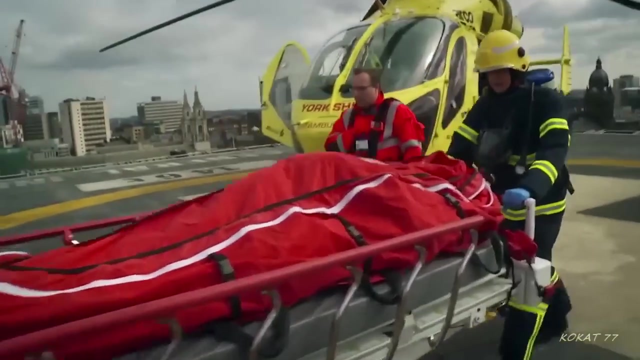 You're cleared to land Roger. Helimed 98, Hopper. Helimed 98, Hopper. Good afternoon. Firefighters are on standby every time a chopper touches down on the rooftop helipad. The trauma team is awaiting Rob's arrival. 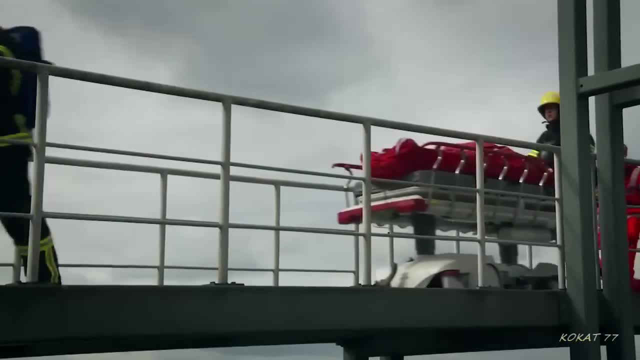 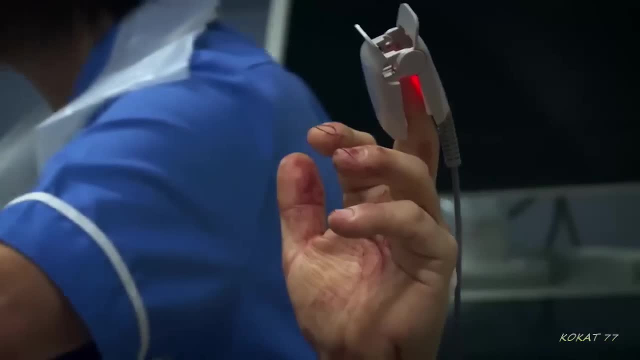 He'll be x-rayed and scanned before medics begin trying to close the wound in his head. OK, this is Rob, normally fit and well. About an hour and a half ago he's been at Ilkley Moor with his family. 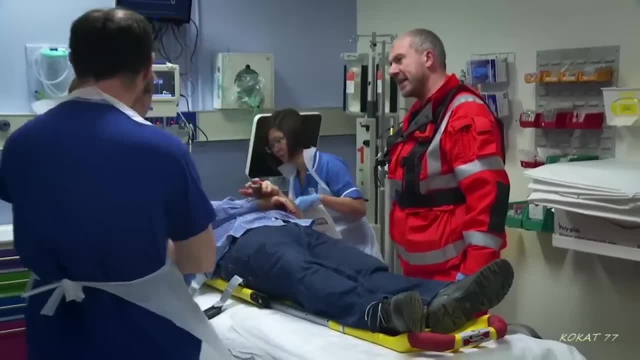 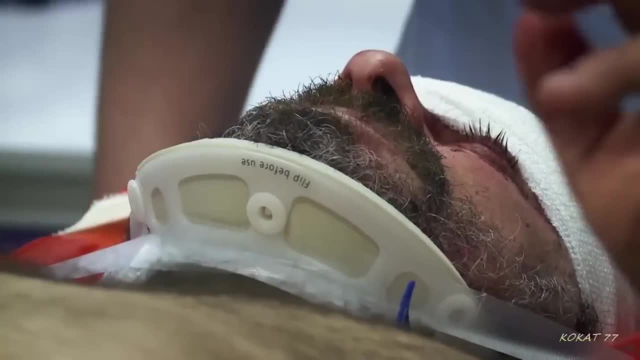 taking a tumble, really landing on his head, striking his head as he's landed. He's been a little bit confused. The scalp injury- you can see the periosteum of his skull through that, but it doesn't appear to have any damage to the skull. 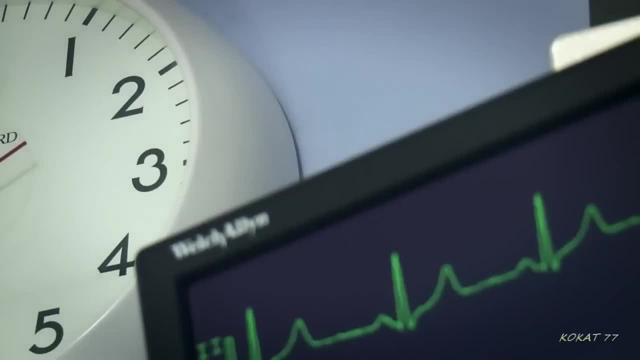 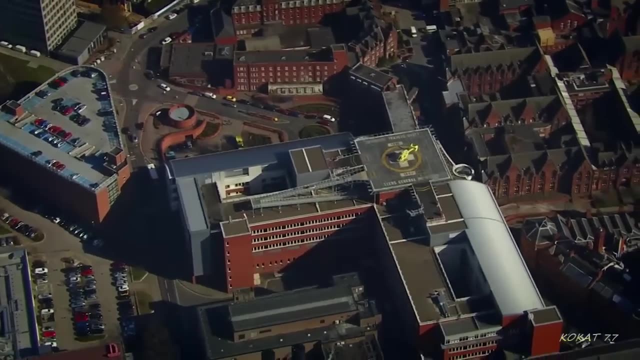 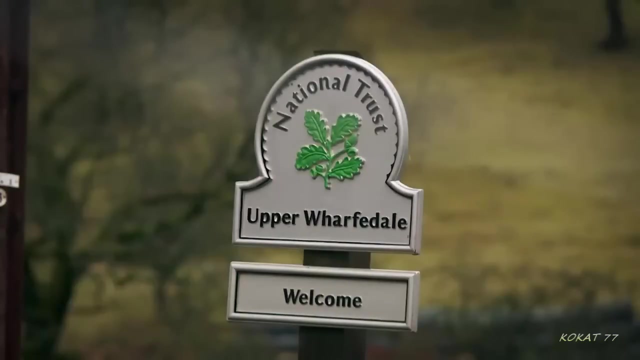 Within a few minutes, Rob will be wheeled into the hospital's body scanner. Only then will doctors be able to rule out a brain injury, And the result is far from certain. The Yorkshire Dales covers nearly 900 square miles, but only 20,000 people live here. 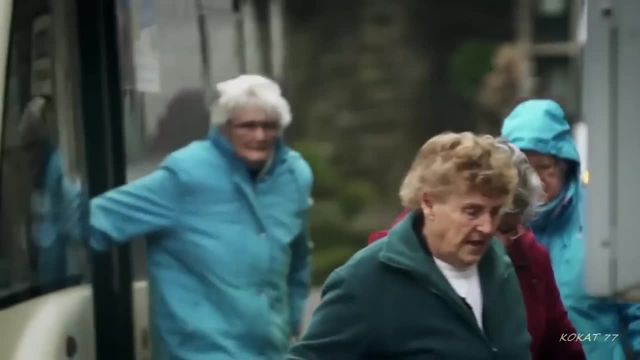 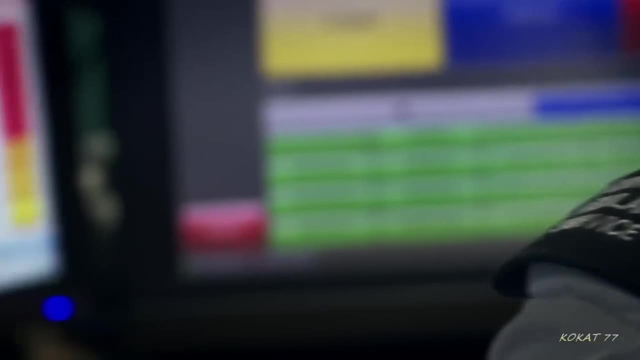 Some are a two-hour drive from A&E. It means that when families dial 999, the air ambulance is often the fastest way to send help. This is the ambulance service. Is the patient breathing? And at the airbase in Topcliffe? 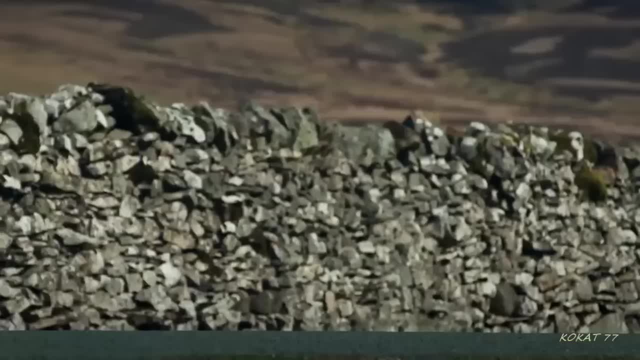 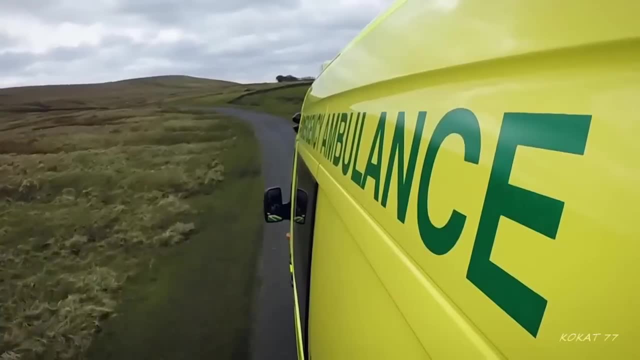 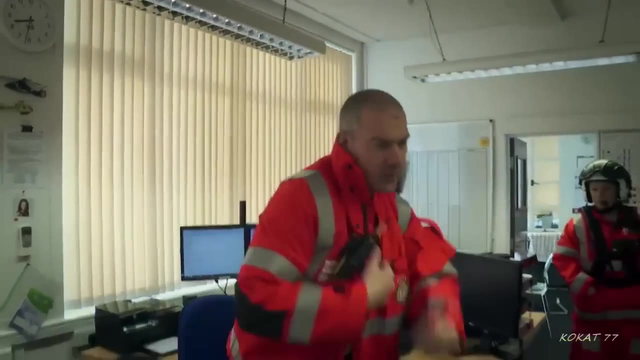 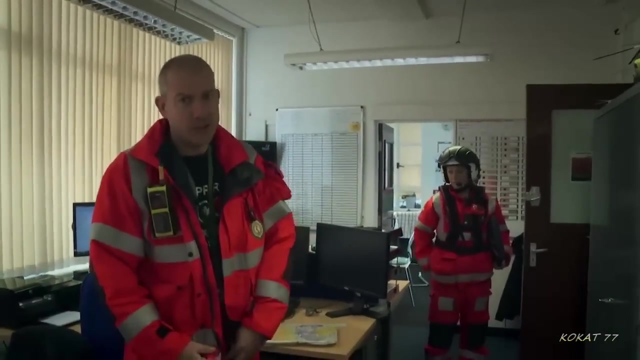 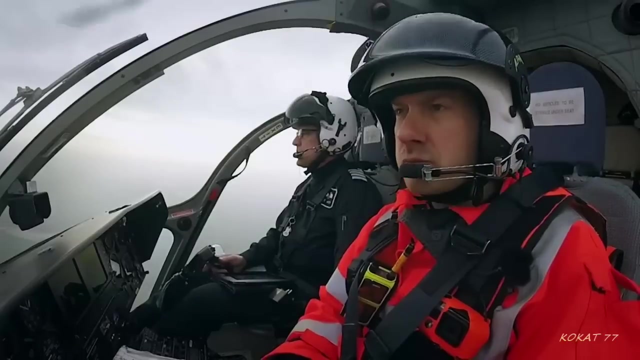 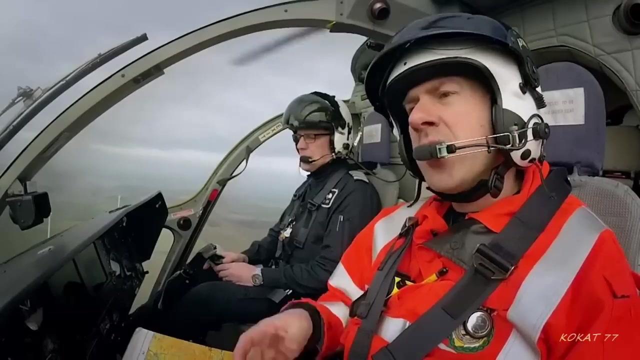 the call is just coming in. It's a child that's poured some hot coffee on themselves and the reported area of burns is quite significant. Paramedic Al is a new dad himself. This could be a difficult, distressing case. Quite common for kids to grab out at cups and pants and things like that. 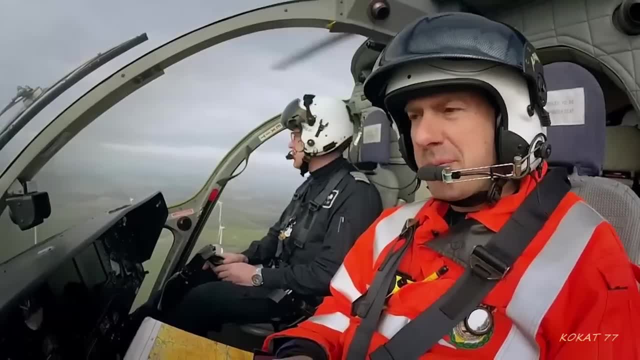 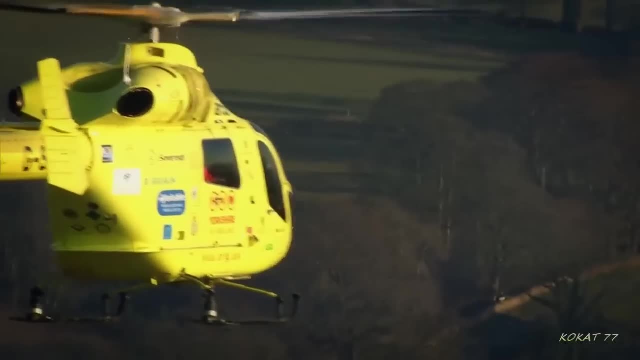 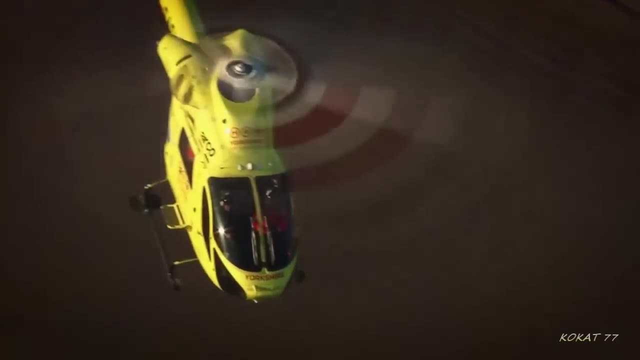 and skull injuries of that type can be quite common. They're always very painful and uncomfortable and very distressing for the child, unfortunately. Is he awake? Yeah, he's awake and screaming. He needs to try and cool the area around, So we are trying with cold tea towels and flannels instead. 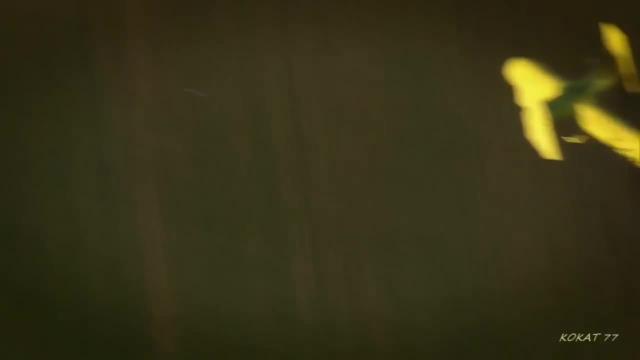 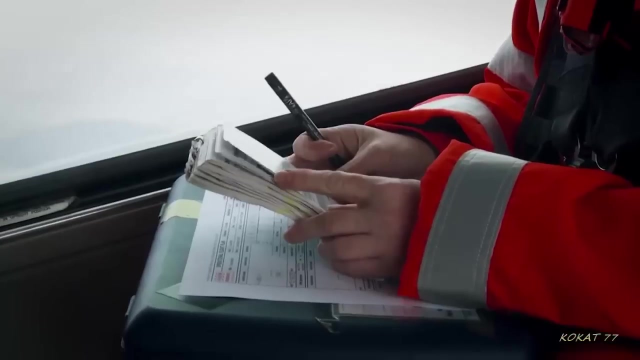 OK, well, just need to try and cool it with water there. OK, Lisa Raywood knows the child may require powerful painkillers. I'm just reading GR Calc. So an 18-month-old total burn surface area between 10% and 20%. 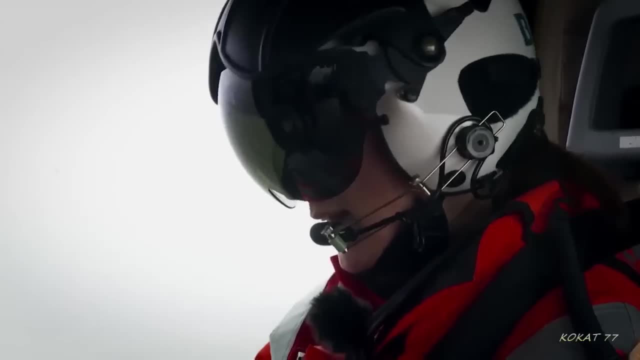 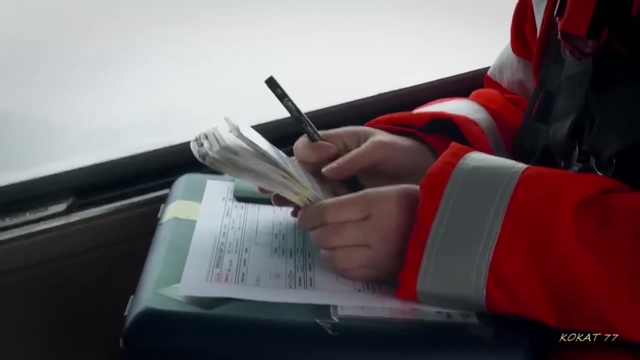 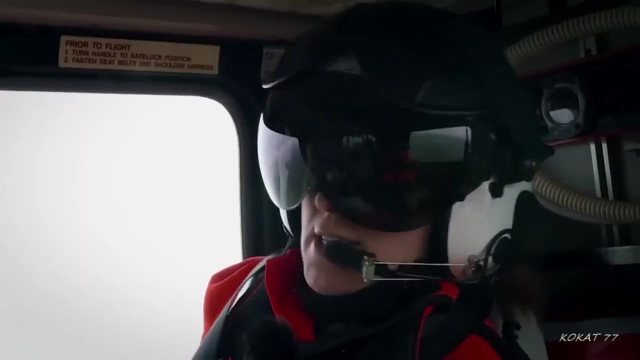 and time to hospital greater than 30 minutes. They get 10 mls per kilogram. OK, In a two-year-old dosages are critical. We're just starting. We're just prior preparation and planning looking at the fluid regime for a child with burn. 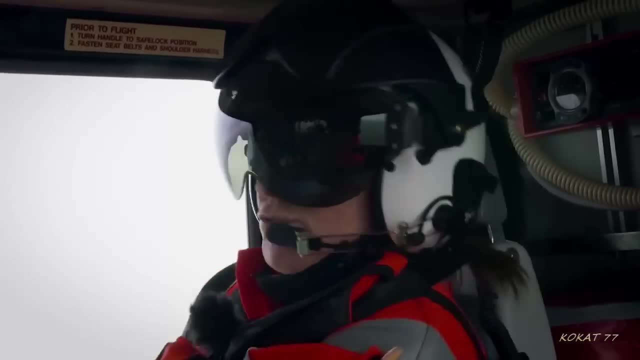 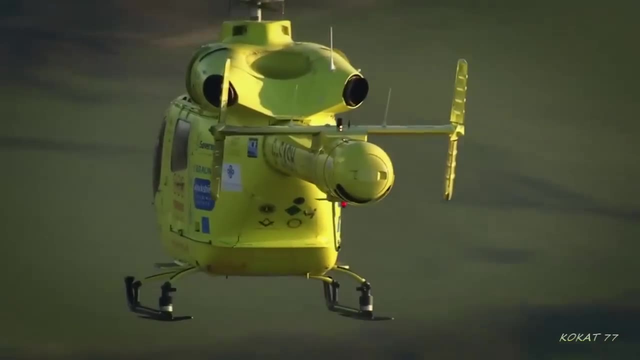 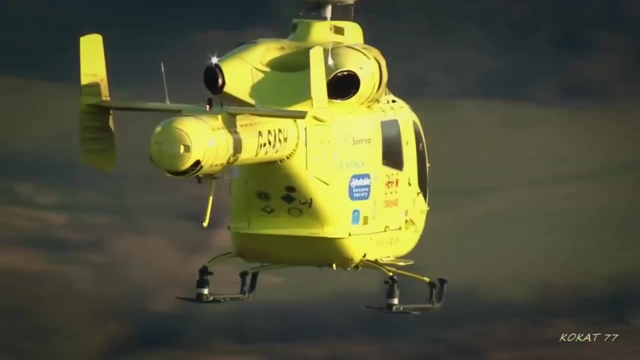 Looking at our guidelines, So we're just rehearsing, making sure that we're both up to speed. The patient's at home, on a remote farm near the market town of Leyburn, The child's parents, are being given first aid advice by ambulance control. 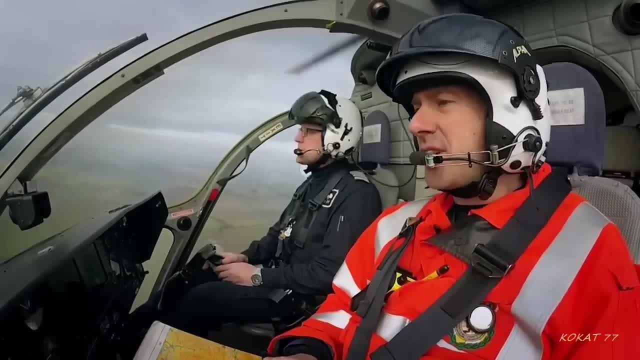 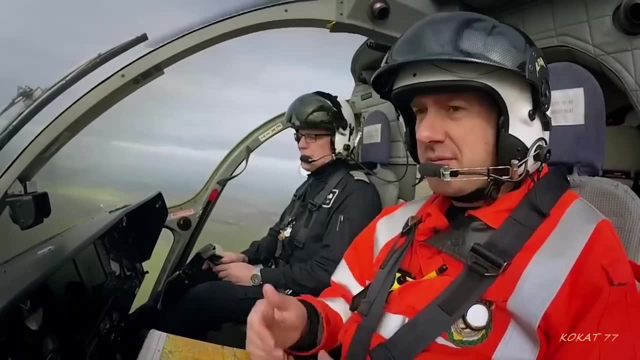 The parents always blame themselves, of course, but pretty much when anything happens to your kid you kind of always think it's your fault, So you're always. There's always an element of kind of guilt, as well as the kind of feeling the pain of your child as well. 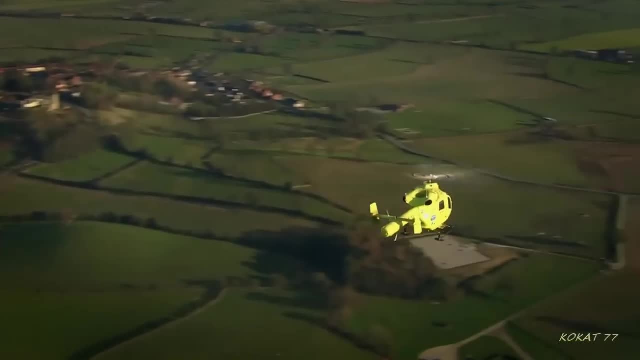 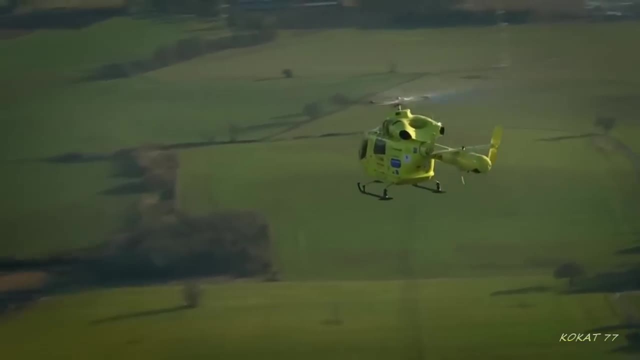 So it's a sort of- It's always very distressing for parents these sorts of situations. Right, we've got one and a half minutes to landing, OK, OK, I'm going to put it on the grass just beyond the track. 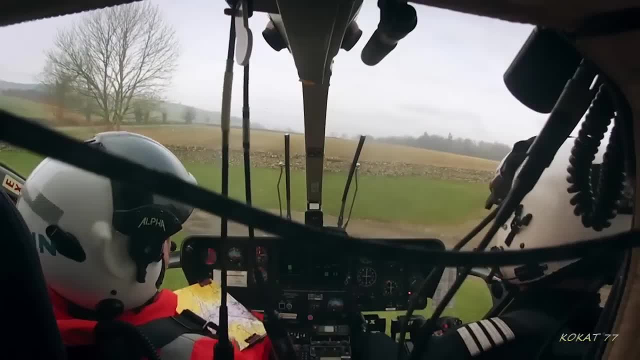 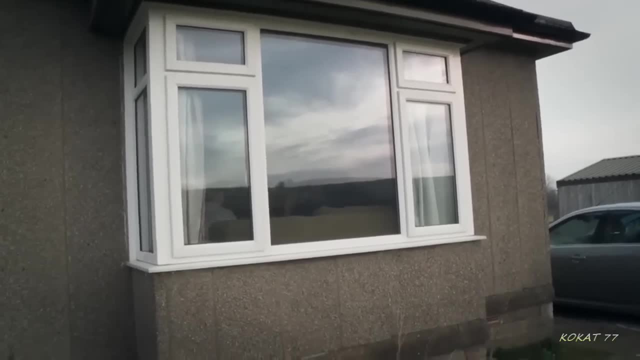 OK, You're looking good, my side, Thank you. We'll clear this side. The chopper crew are arriving at the same time as local paramedics. Lisa brings them up to speed. Hiya, you all right, This is Finley. 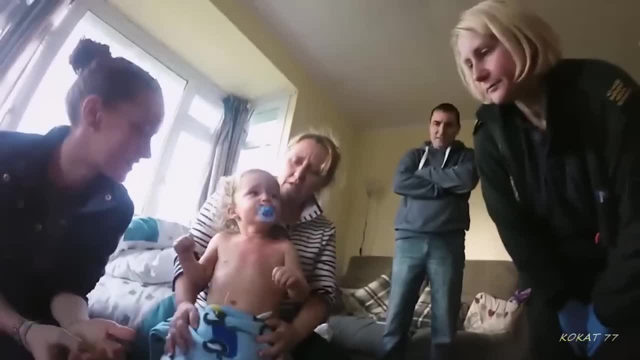 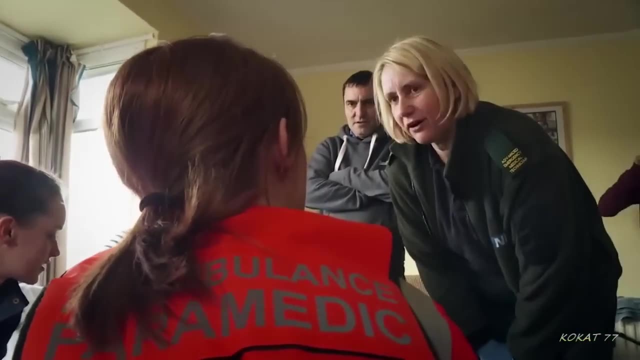 Hello, This is Finley, who's 18 months old. He's just been toddling around in his pyjamas Hot cup of coffee that had just been made on the side. I think he's gone to grab his milk but got the hot coffee. 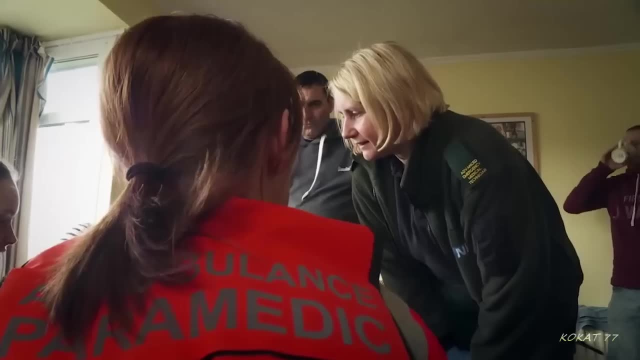 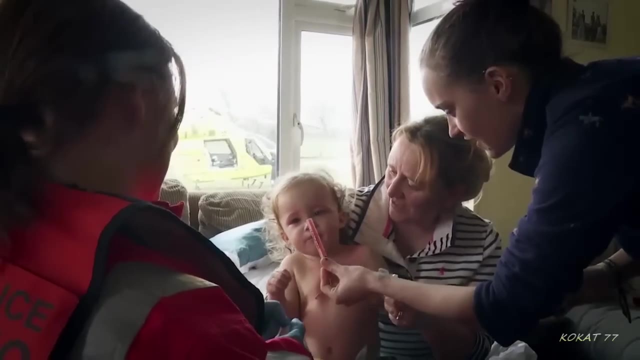 Just the tiniest drop of milk, so it would have been quite hot. It had just been made. Lisa's giving him a mild painkiller first. You like that, don't you? Yeah, That must be the first child I've ever met. 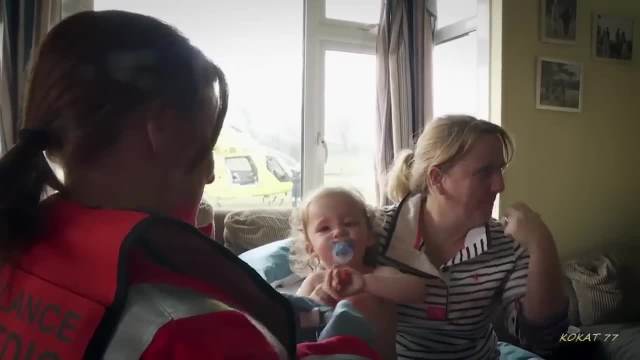 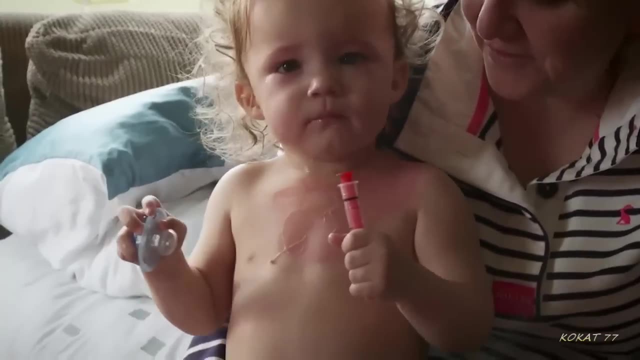 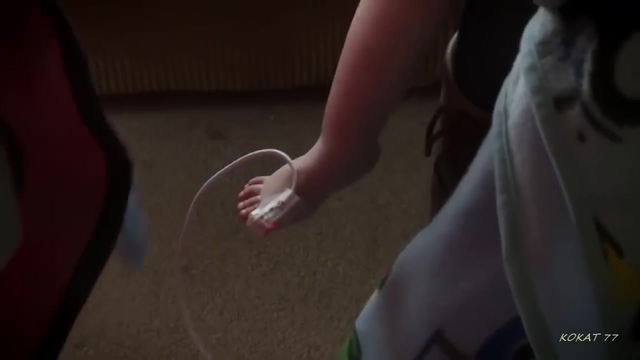 that he doesn't end up all over his face and up his nose Right. have we got a toe, Finley? Can I borrow one of your toes? All this attention is distracting Finley from the pain he's in. He's really wanted his medicine. 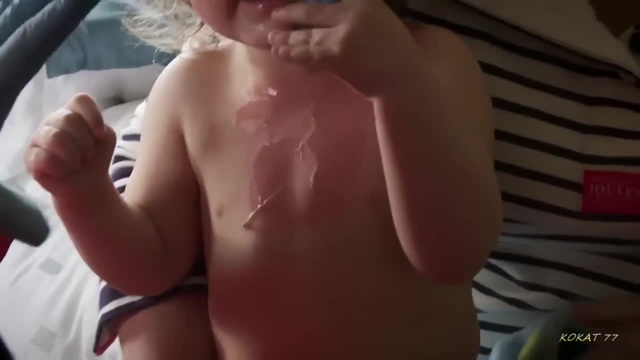 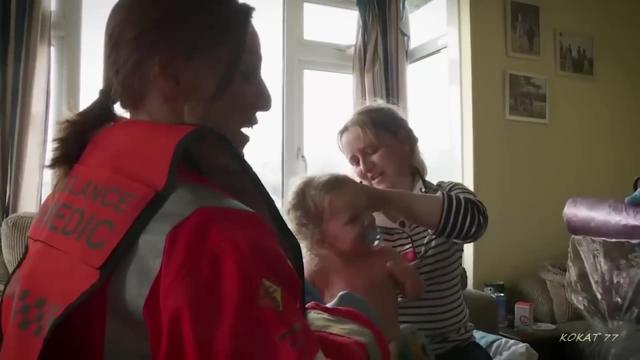 Yeah, What we're going to do is put some clean film on, because what causes the pain with burns is the air hitting the soap. We're not sure whether to put it on or not. Yeah, no, that's fine. Kitchen wrap protects the burn and prevents infection. 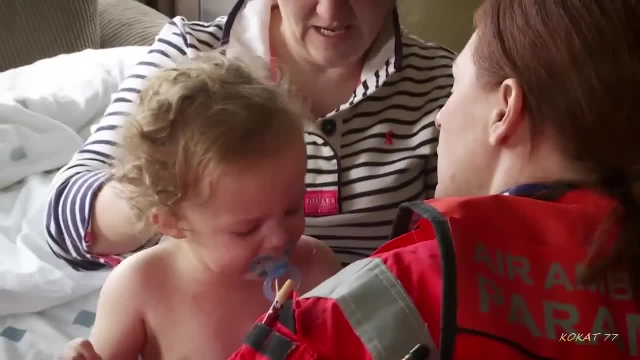 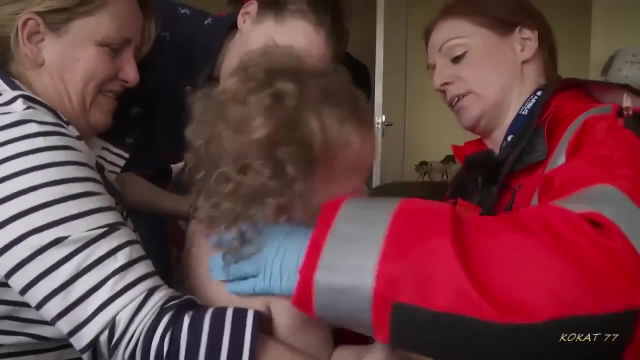 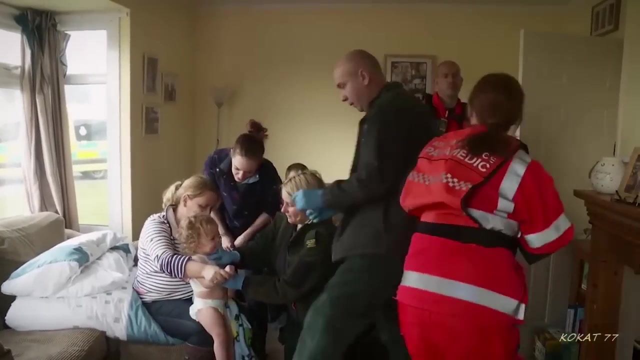 But it's clear Finley's still in pain. We could do with a bandage, couldn't we? Just to stop him pulling pain, Stop it from stinging, Or a maw, please. Yeah, we could do, couldn't we? 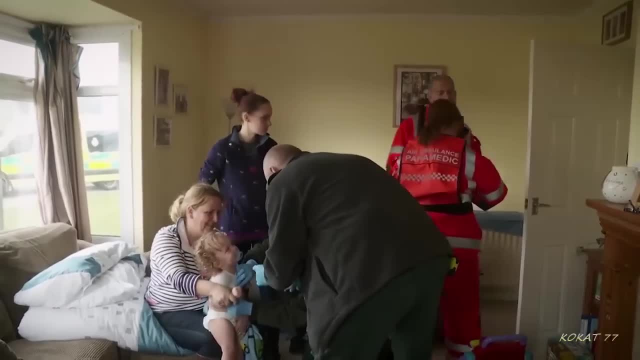 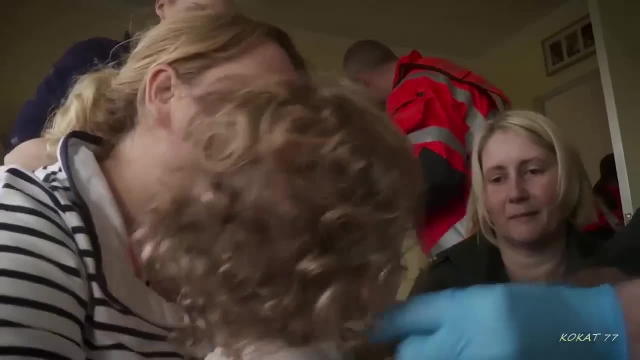 Two milligrams for a two-year-old. Can I leave that with you and I'll just give him a buzz? He's just had some proofing stuff. They're going to give him an oral form of morphine. It's much more powerful, with potential side effects. 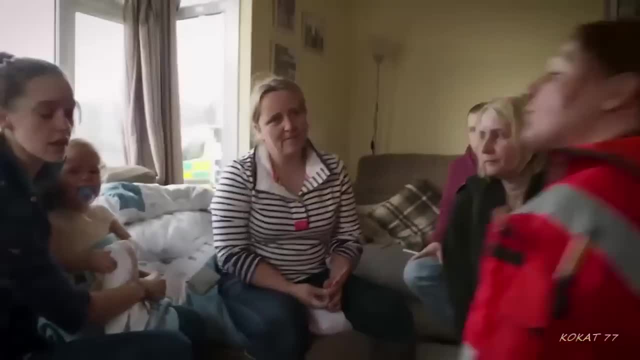 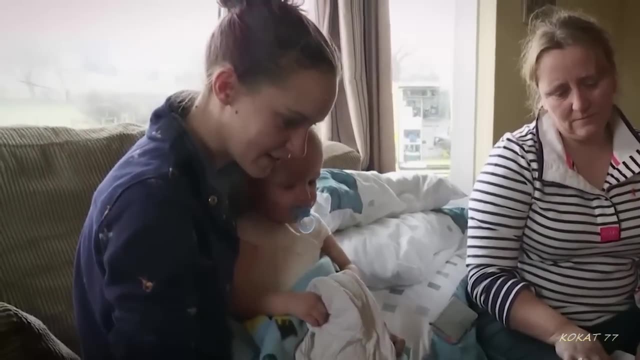 They'll need to monitor his condition closely from now on. We're going to take him to James Cook, All right, so we'll fly him up there. Ooh, how exciting. Finley's injuries urgently need to be assessed by specialists. 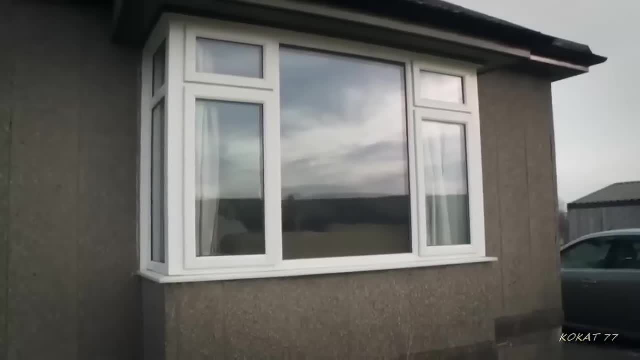 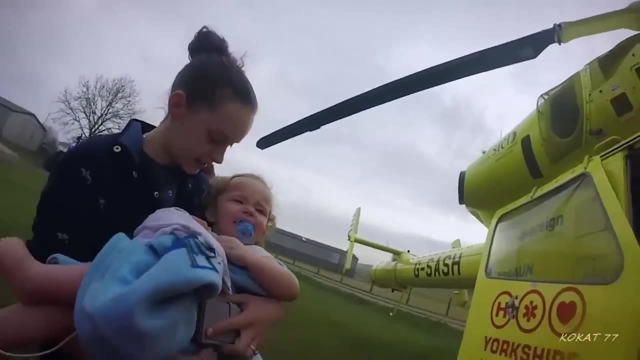 Childhood burns can scar for life. Speed counts in cases like this, and the family home is an hour's drive from hospital. Oh dear, It might upset him, but we'll just have to play it by ear and just roll with it. 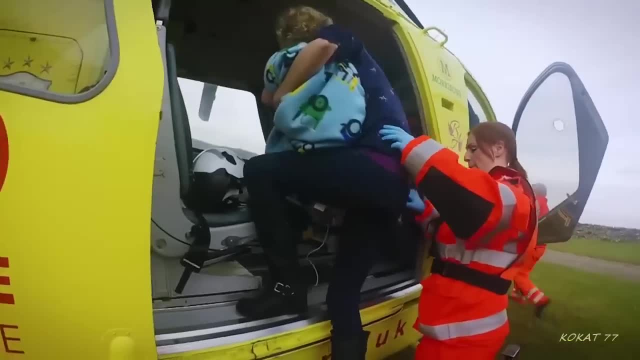 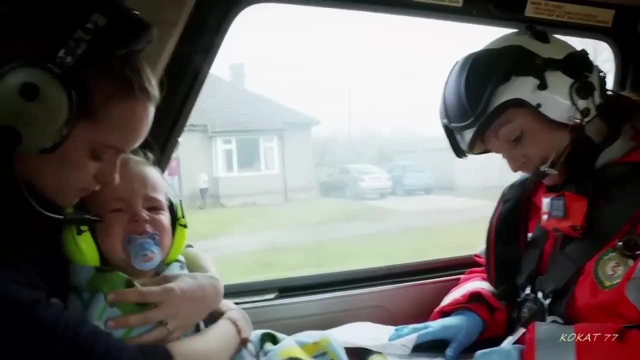 Mum's going with him. He's being flown 30 miles to the trauma unit in Middlesbrough. OK, if you're happy to start. Hair desk 9-9 is lifting for James Cook. OK, we'll lift. we'll turn tail right. 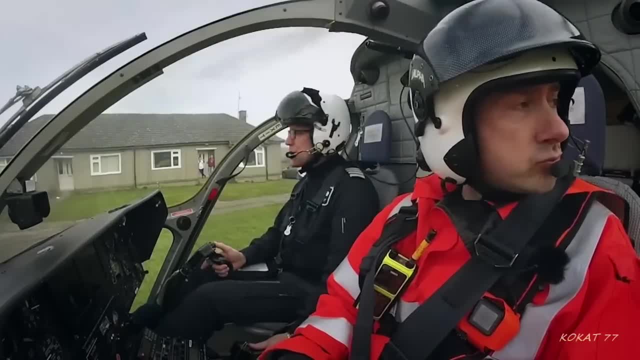 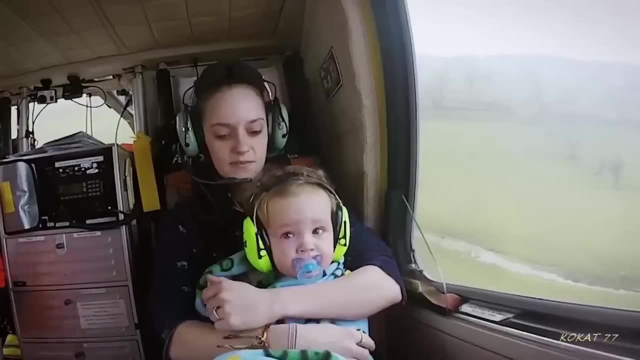 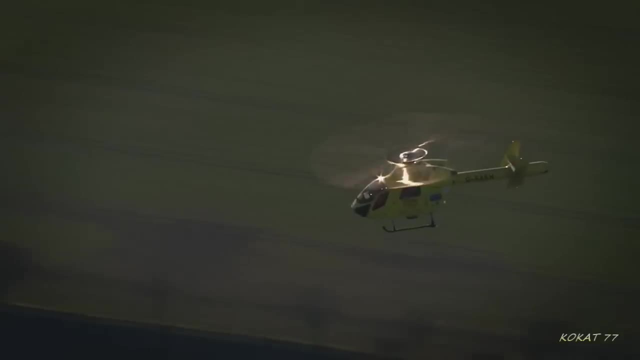 we'll go out into the 9 o'clock across the fence And out the opposite direction. Be good, right, I was quite impressed today. Good Helimad 9-9 is a familiar sight in the skies over the Dales. 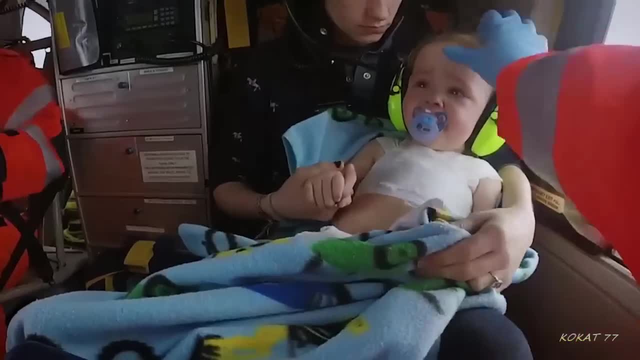 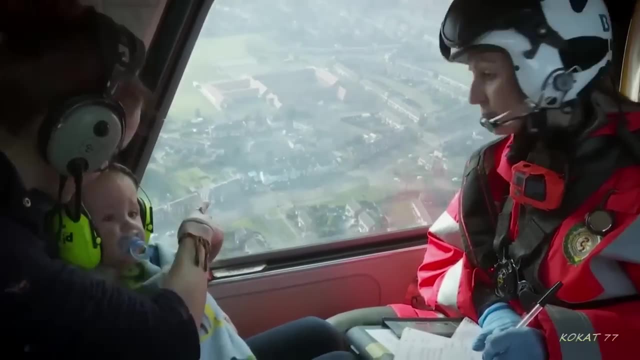 Taking Finley for treatment by road would have meant a three-hour round trip for an ambulance crew. Helimad 9-9, Alpha- finals for James Cook. Helimad 9-9, Alpha- surface winds. at Durham We're at minus 0 degrees watching. 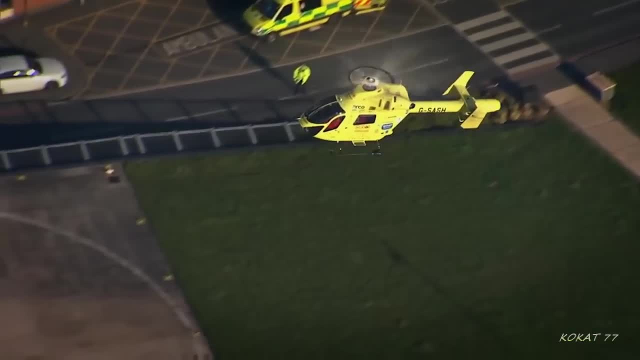 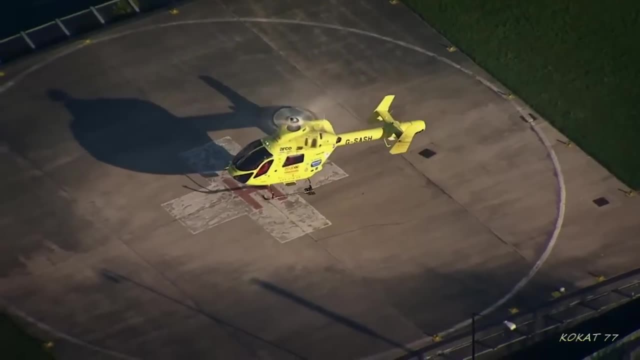 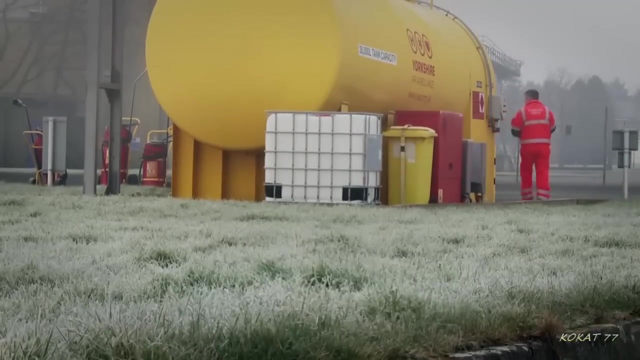 Thanks to the Helimad team, Finley will be undergoing treatment less than an hour after his accident. His mum is anxiously awaiting the doctor's assessment of his burns. It's yet another chilly morning at Topcliffe: Minus 3, pretty cold. 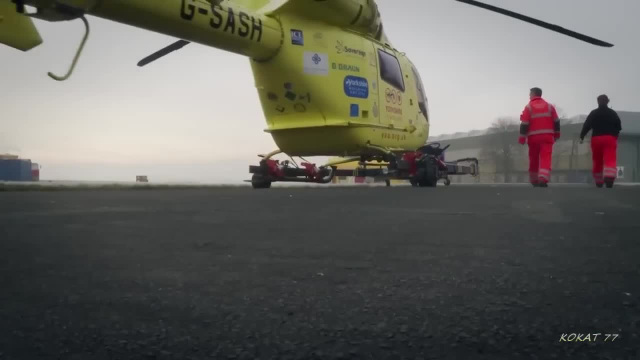 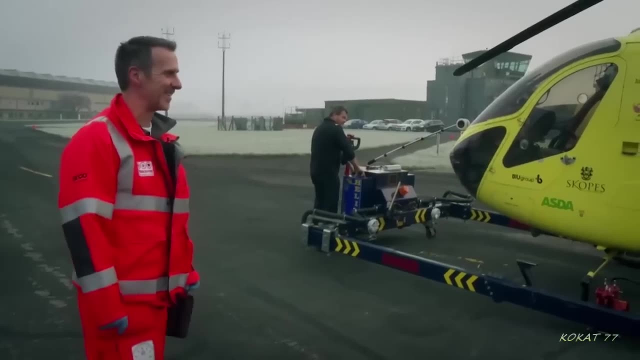 Paramedics Daryl Cullen and Lisa Rawood are used to it. It's always chilly up here, even in summer it's chilly up here, but we're going to wrap up warm out with ice. Yeah, we've got those sexy thermals on. 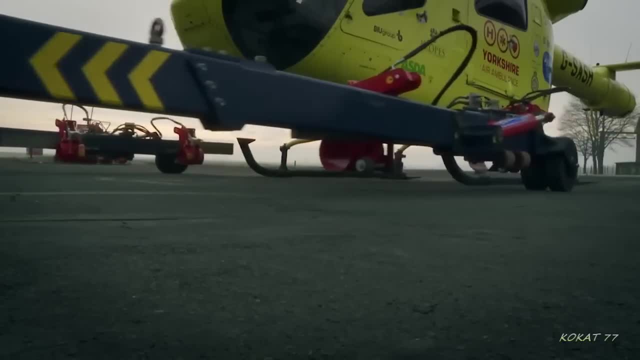 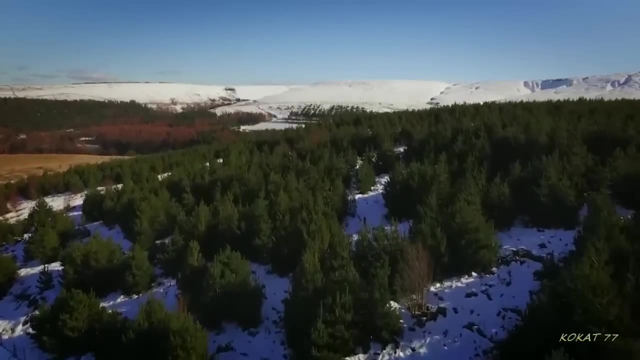 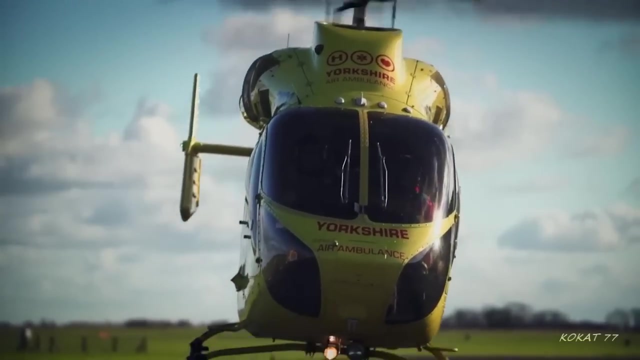 But over 250 more people per day in the UK die during the winter, and not just from acute trauma. Those with chronic medical conditions are at much higher risk, and many of these patients are frequent flyers in the air ambulance Helpliwinter. we're looking for a pilot. 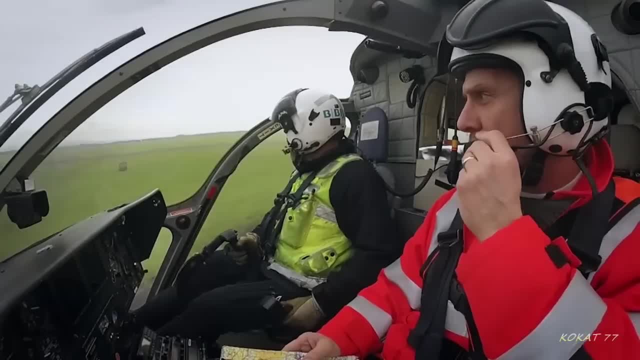 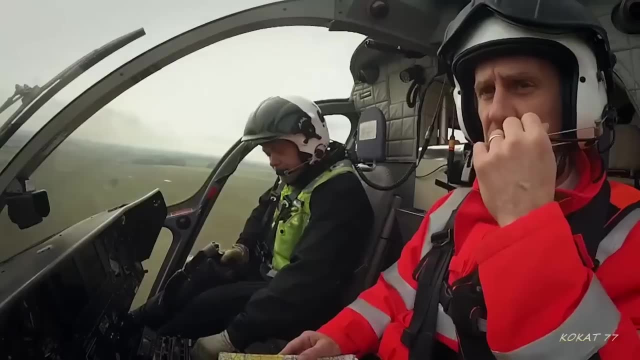 Thank you. Pilot Chris Attrell is responding to a call that's just come in, A call that's just come in from Formanby, a small village about 10 miles north of York. We're going to be first on the scene, are we? Lisa? 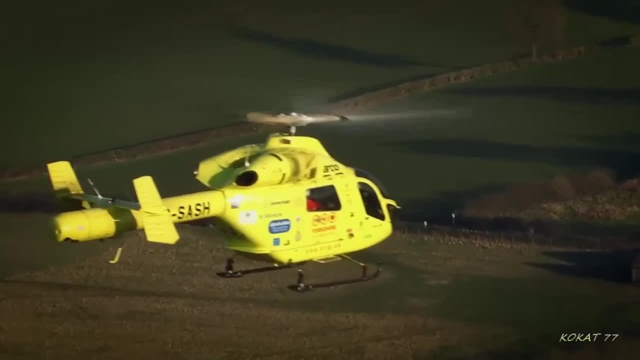 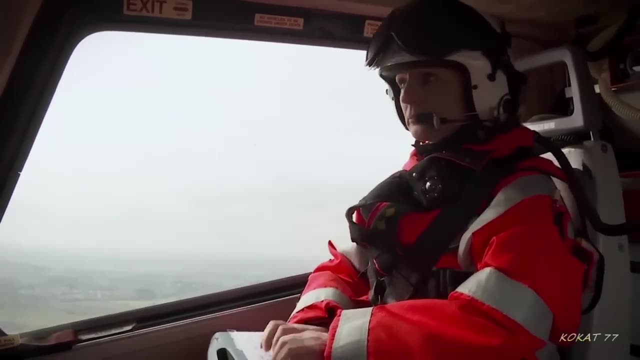 Yeah, crew's greater than 20 minutes away. she says: All right, A woman has gone into an anaphylactic shock, a potentially fatal allergic reaction. Lisa thinks she's met the patient before, So if it's the same patient. 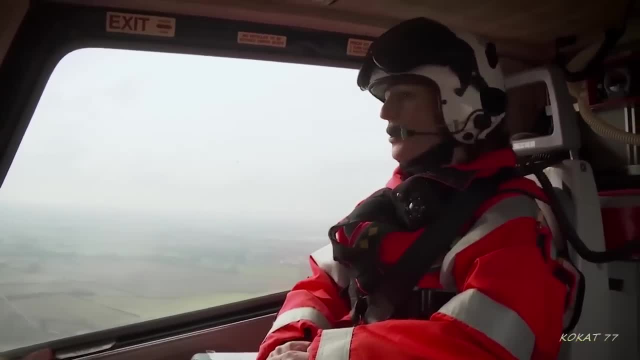 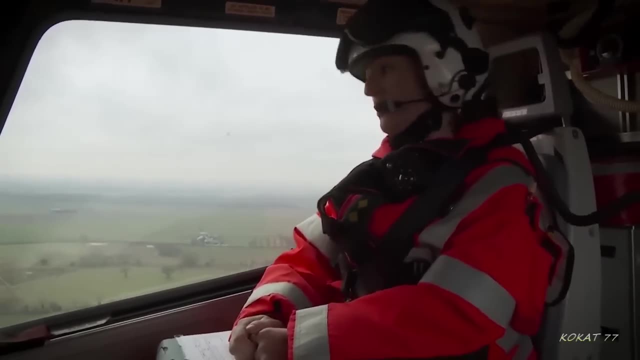 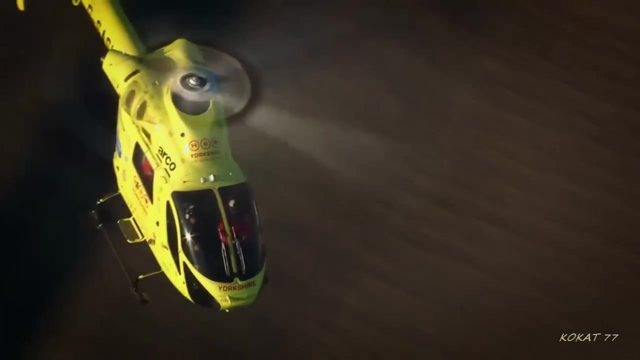 I went to this patient about three or four months ago. it can be a life-threatening situation and time is crucial really to get treatment into the patient to stop it progressing into quite a sinister event. Living just five minutes flight away from the base. 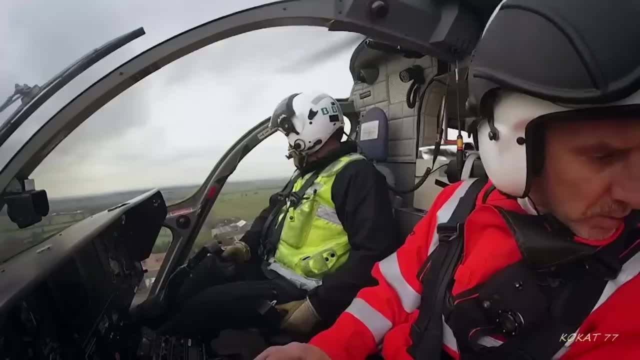 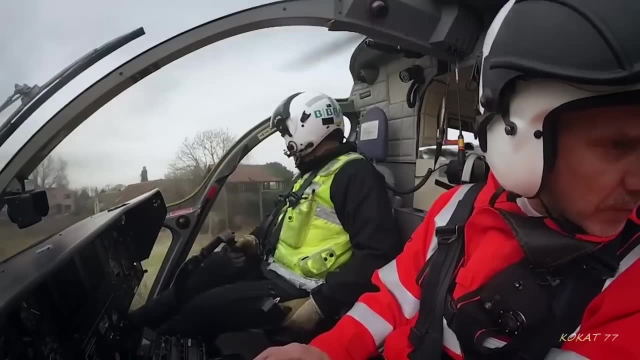 could make all the difference for this woman: Clear on the left, Receiving Clear of the tree. Got the domestics to the right. Chris, You're good my side. Yeah, no, I'm fine. Clear left, OK. 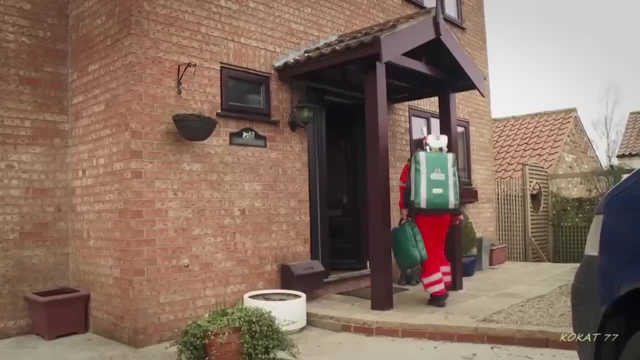 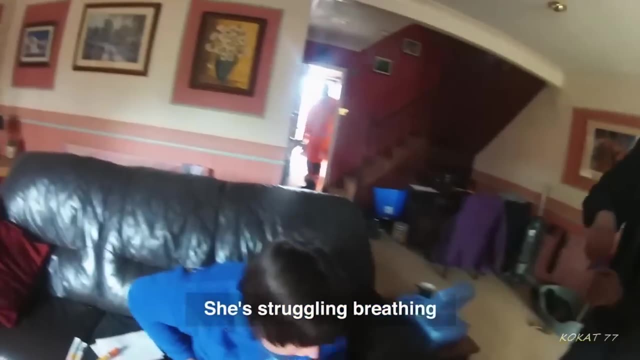 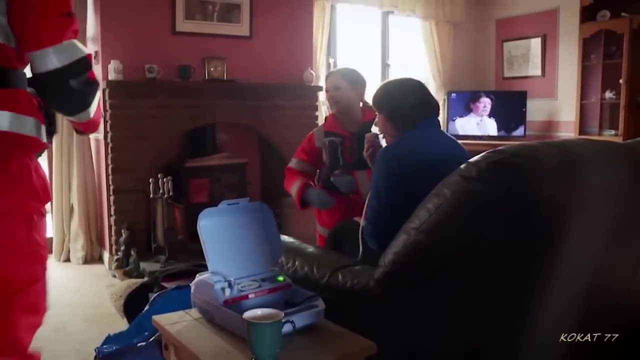 No, no, we're on the ground. Hiya, Just tell me what's been happening. I've given her three epithets. She's struggling breathing. She's been like sick all night. OK, Rachel Fyldes is hypersensitive to food colouring. 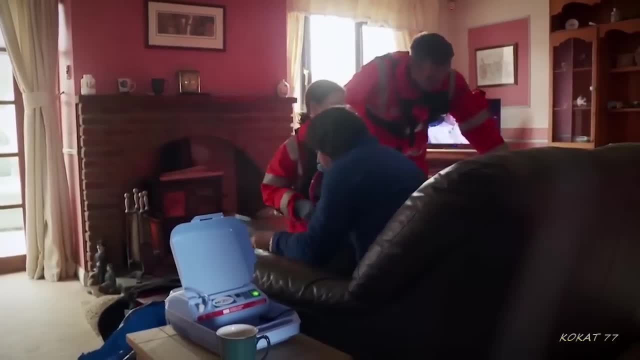 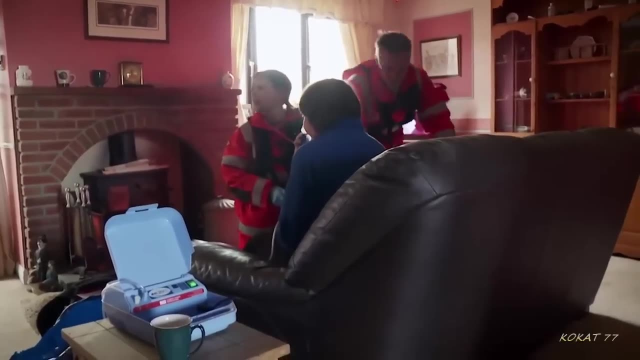 pollen and numerous other allergens, even antihistamine, the medication often used as first-line treatment for anaphylaxis. Her partner, Alan, has given her oxygen and three shots of adrenaline, but she's still in a bad way. 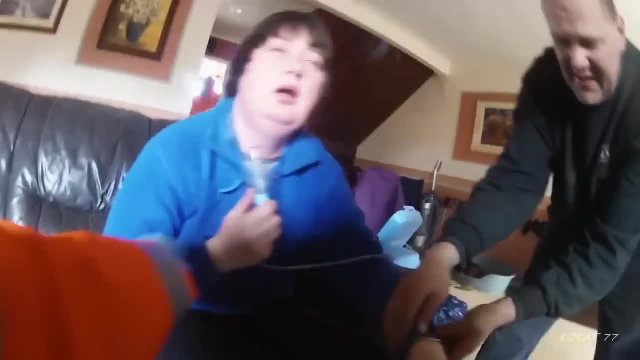 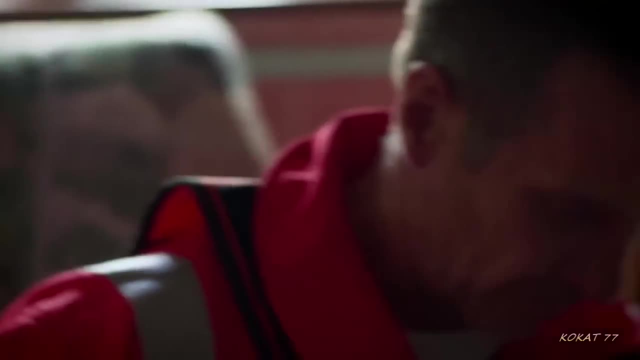 Is that anaphylaxis? Yeah, She's got a brace there. Rachel Daryl's just going to wire you up to a few things so we know where we are. OK, Monitoring is essential. Severe allergic reactions can cause a drop in blood pressure. 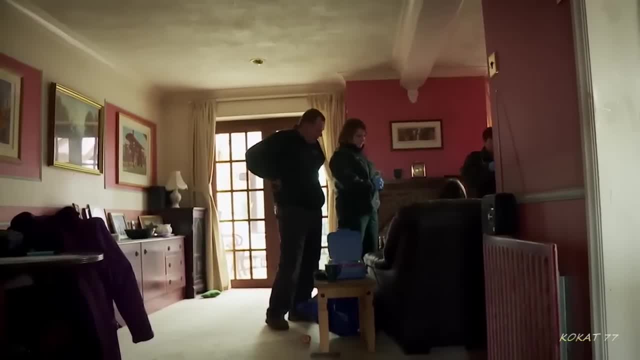 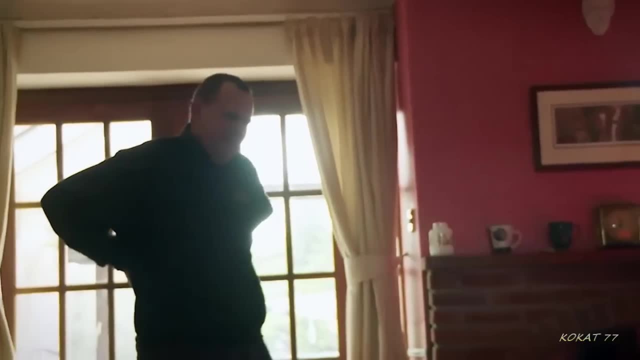 which can result in dangerously low levels of oxygen. Just get that held up to you a minute. Anaphylaxis kills 20 people a year in the UK and speedy treatment is vital. Are you able to tell me what's happened? I don't know. 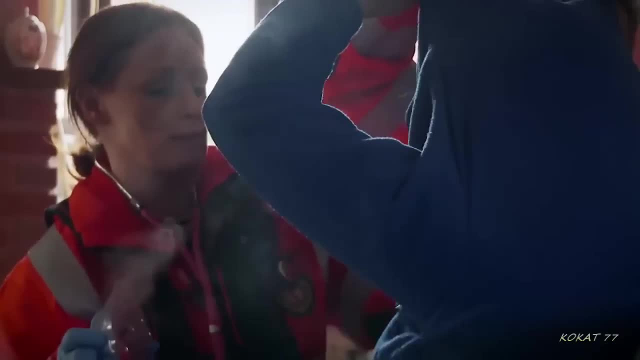 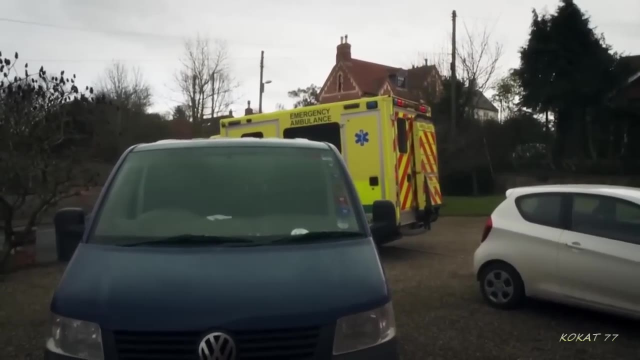 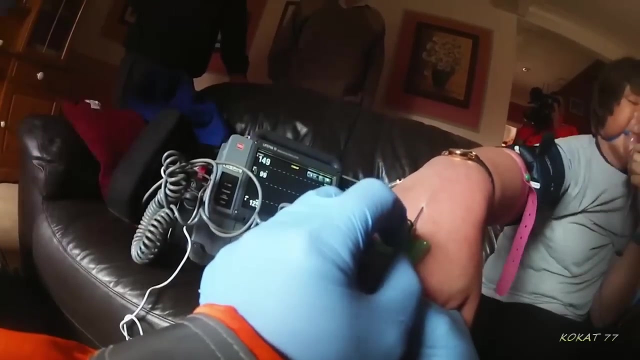 I've been having my infection all week- Chest infection. Apart from the chest infection, it's unclear what triggered the attack. Right, Rachel, sharp scratch. Just try not to flinch love. The cannula goes in, but Lisa can only administer drugs that Rachel is not allergic to. 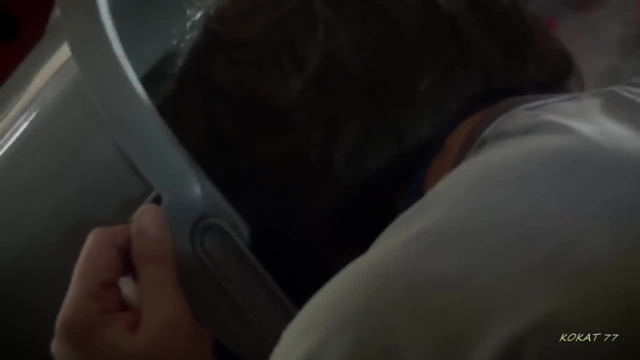 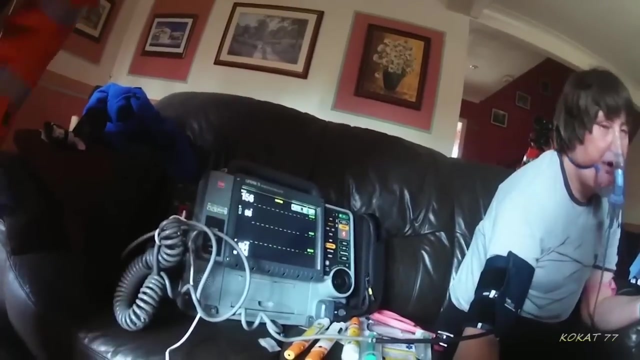 That one's already good to go. So I'm just thinking um. We can't give her any cloth anyway. she's allergic to antihistamines. No, she's allergic to antihistamines, yeah. Are you allergic to steroids? 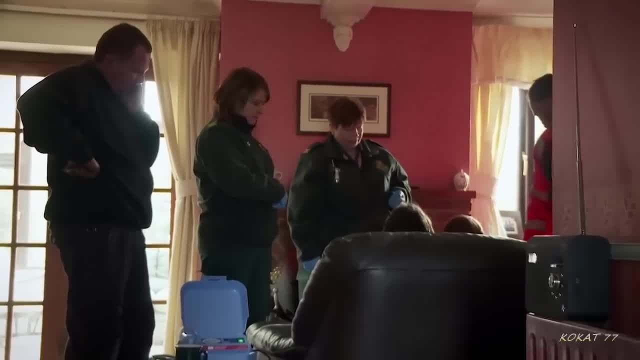 No, We could give her some hydrocortisone, couldn't we? Have you ever had hydrocortisone before? Yeah, they give it to me all the time. Were you OK with it? You didn't have a reaction to it. 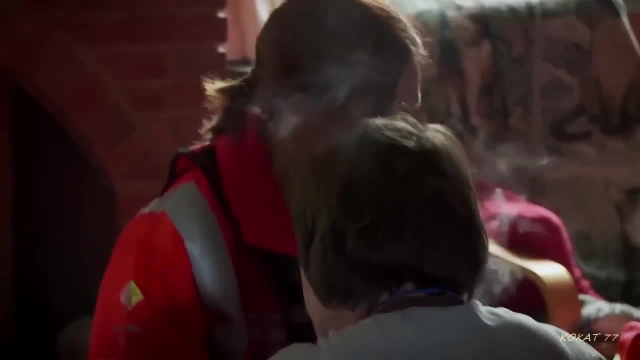 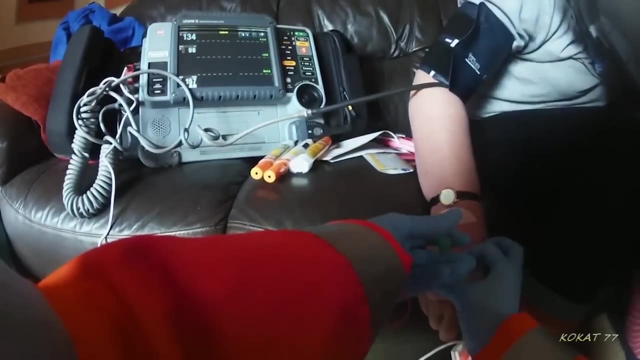 No, it's all I can have. It's all you can have, Right, we'll give you some of that. It's a powerful drug, but Rachel still only gets a few minutes between each attack. She may need a lot of help as she travels to hospital. 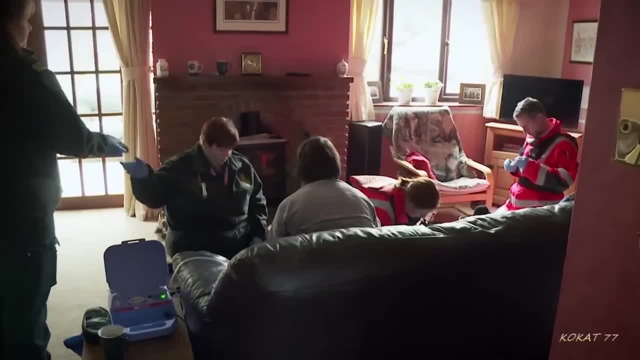 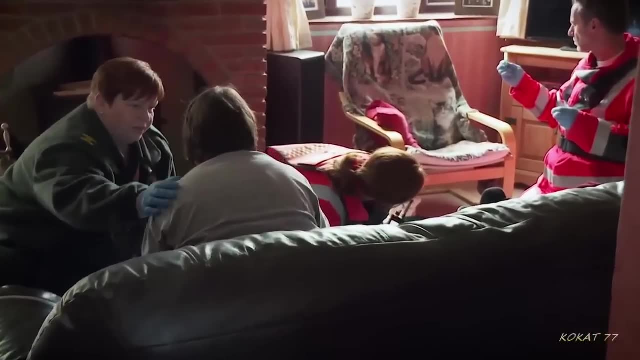 so a decision has to be made. Pass your message. Yeah, just a quick update. I'll travel down in the DCA with the patient of her. In cases like this it's safer to go by road. I know you will be. 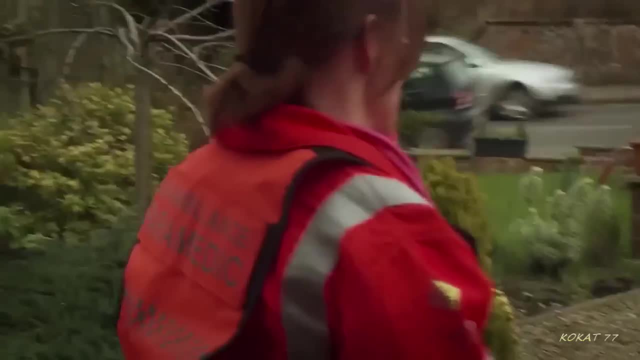 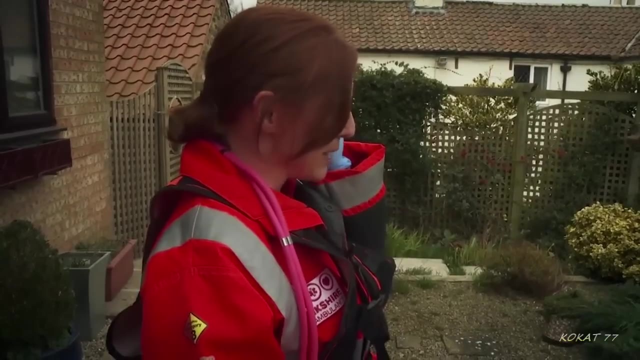 Don't worry, we'll look after you. It's Helimed 99 here. She's had an anaphylactic reaction this morning. She's had three of her own EpiPens before Helimed arrived. It's a worrying time for Rachel's husband. 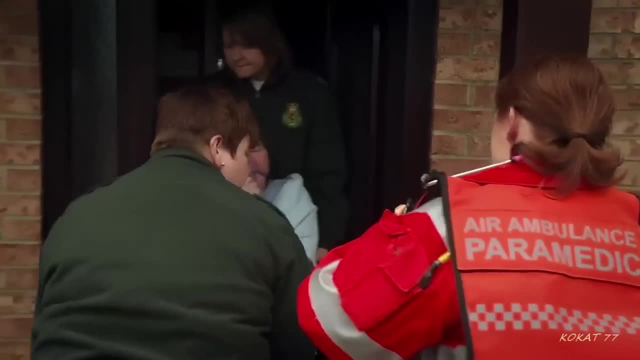 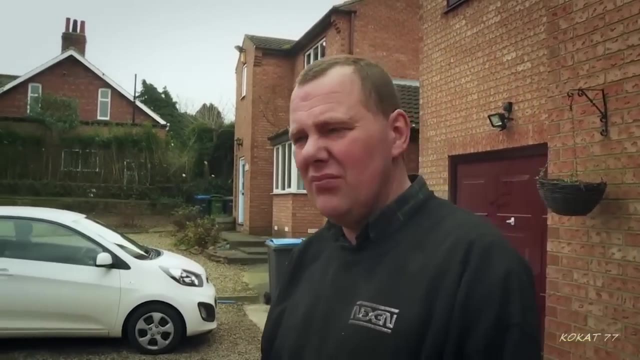 He's no idea what caused this. I know she's been to her artist. at 9 o'clock this morning She went to work today. Sometimes it just triggers it and then that's it. But she knows what food to eat and stuff. so 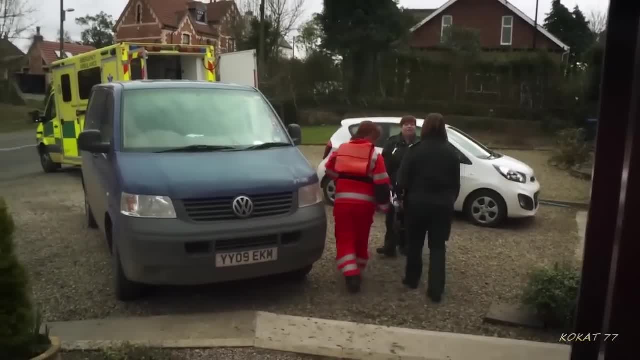 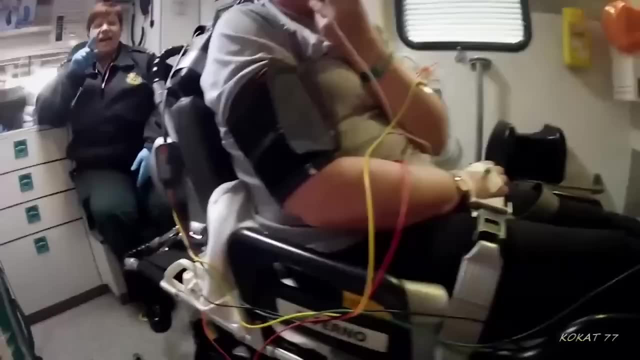 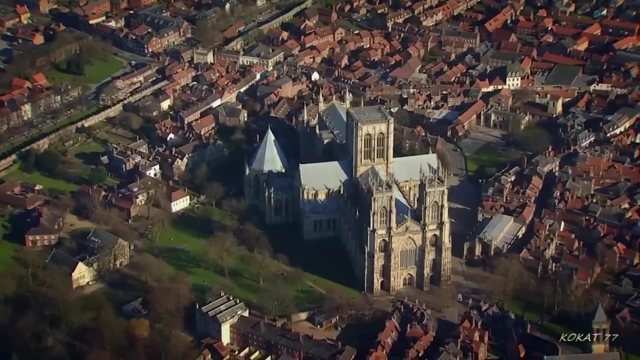 How are you doing? You're looking a bit better. This is the 12th time this year Rachel's been taken to hospital. Lisa will be keeping a close eye on her patient throughout the 20-mile journey to York. Rachel's life could depend on her skills. 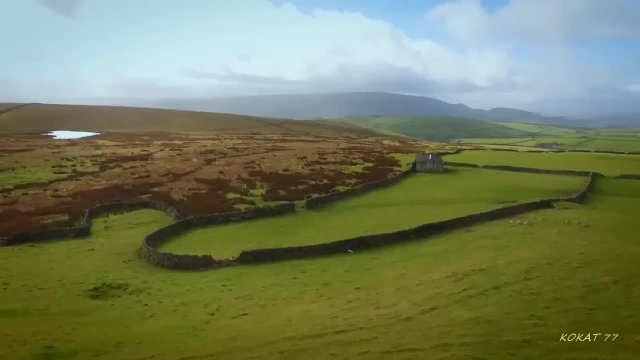 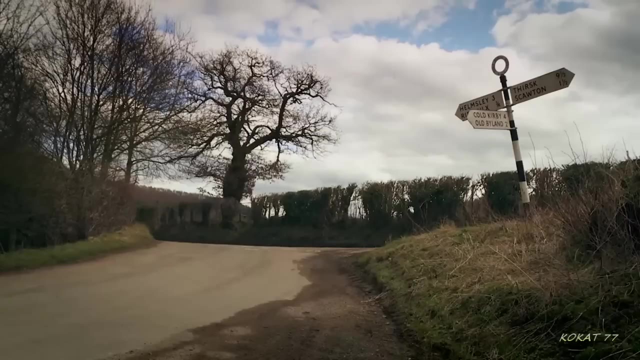 She's been in the hospital for over a year now. When the Helimed teams are called to provide emergency medical care, finding the patient can often be the trickiest task. You've got to come up Pepper's Lane. You can't get to us down Grove Street. 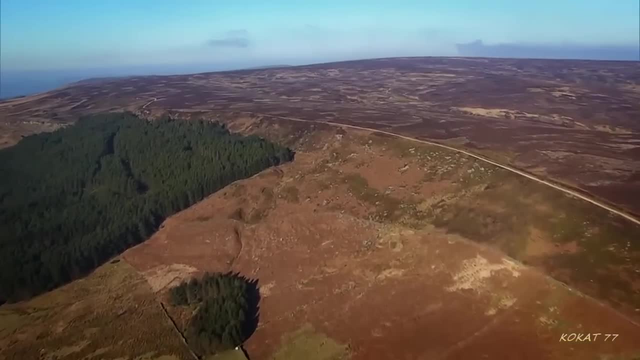 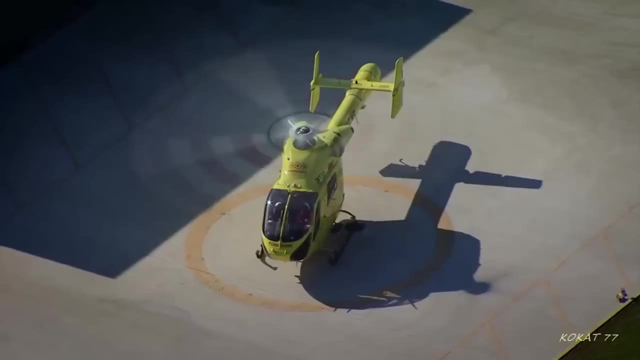 OK, not to worry. Yorkshire is a big place, so the accuracy of information provided by those on the scene is of paramount importance. But the next job for paramedics Pete Rhodes and Al Day should be the easiest one. They've got a grid kit. 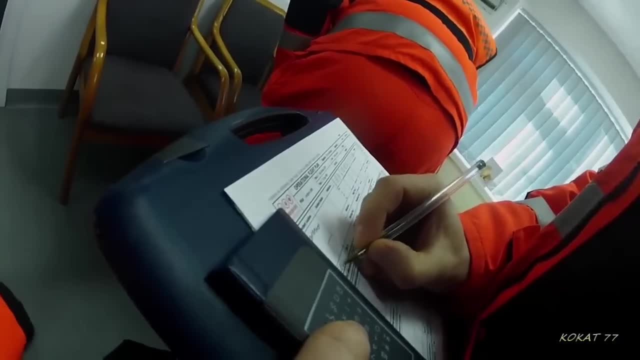 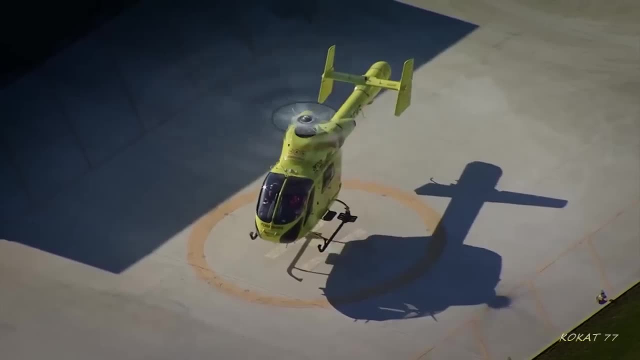 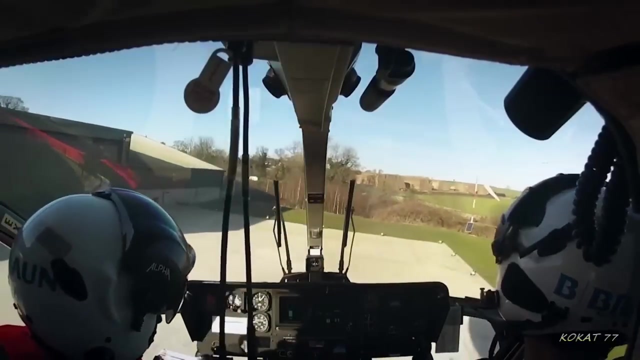 Is there an echo 424204.. That's Featherstone railway station. They could practically walk there from the base here at Nostal Priory. Estimated flight time: one and a half minutes. In theory That's about the shortest hop you're ever going to get. 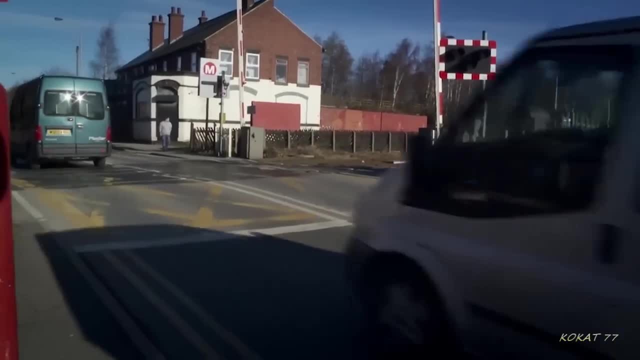 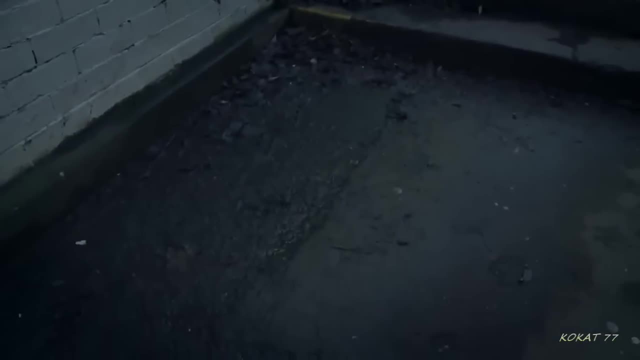 The job itself also seems like it might be straightforward. A man has fallen down some steps- 25 of them in fact- But it's still a common accident. Is it the railway station or the level crossing The railway station? This might be as local as it gets. 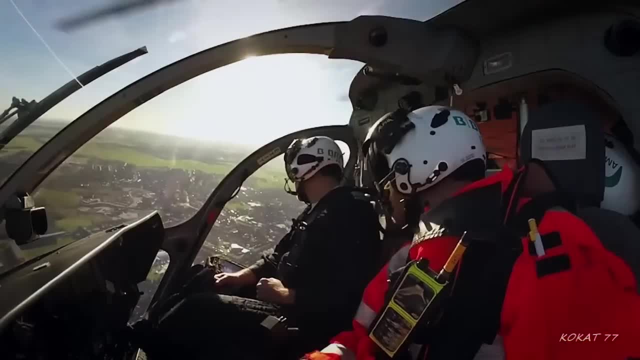 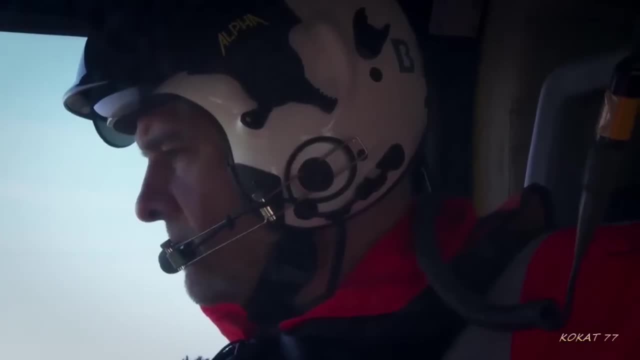 but something doesn't add up for pilot Andy Lister. It doesn't look like there's 25 steps anywhere. 992, I'd ask. 992, I'd ask for a message. Yeah, can you just confirm? is it Featherstone railway station? we're going to. 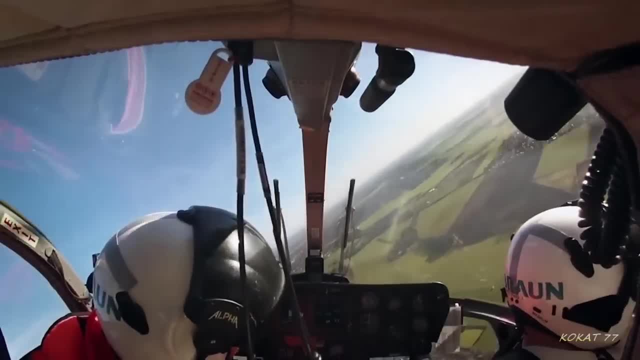 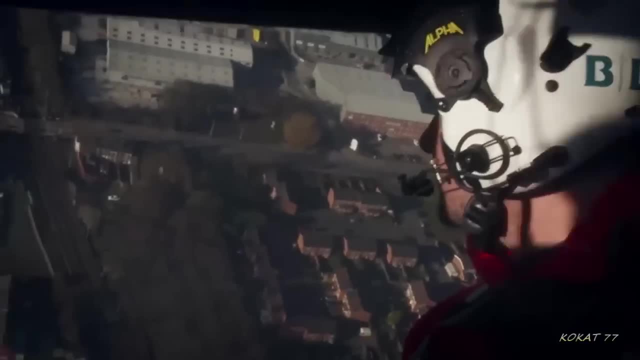 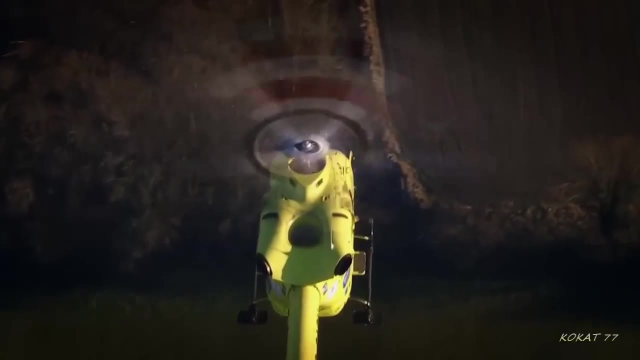 But then a breakthrough. Hang on. there's some steps going down, There's a slipway, There's an underpass Right Where, Underneath the railway, Andy puts Helimed 9A down in the nearest available spot. 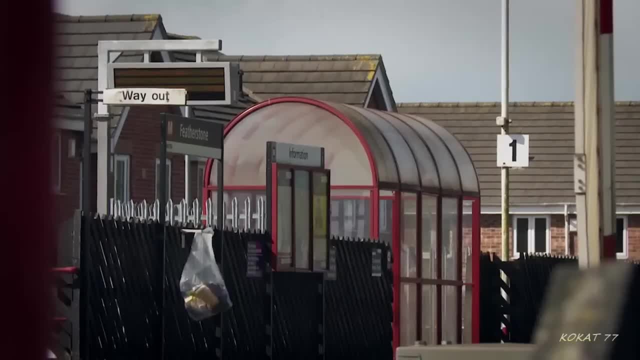 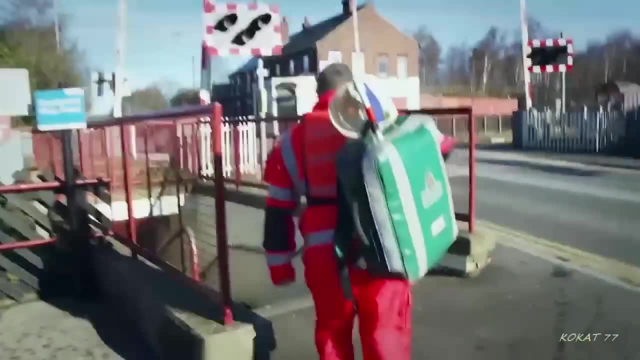 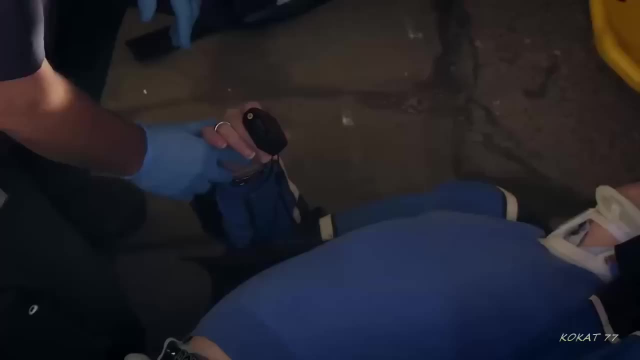 but it's a hike to Featherstone station. Hey, mate, you all right. As Pete finally gets a view of the steps in question, it's clear how far the man has tumbled. Hey, mate, You all right. Knee gave way coming down steps. 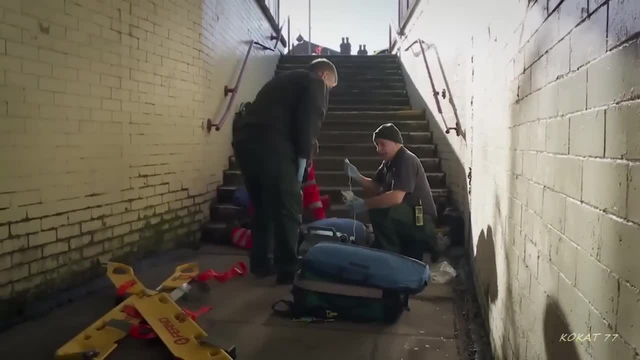 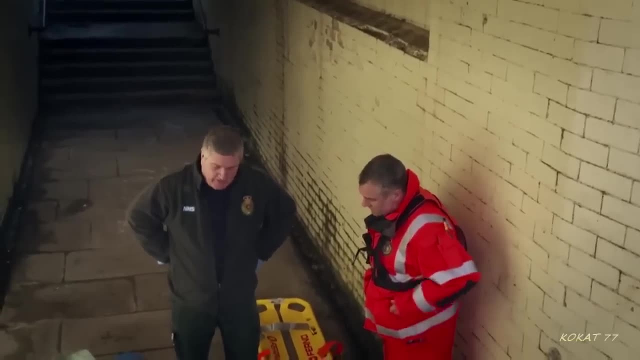 Right, He says he's actually rolled all the way down, but there's quite a gap in between. Yeah, No, epileptic diabetic. Yeah, Compain of pain, cervical pain. What's your name, fella John Tom? 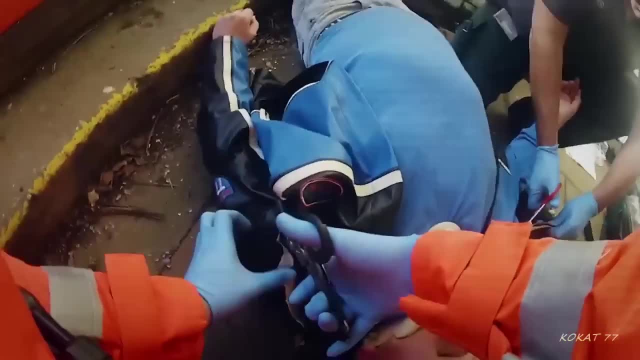 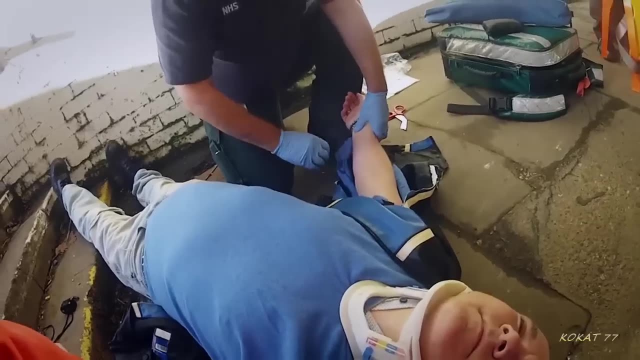 John, John, Sorry, John, I'm Pete. All right, All right, John. where's it hurting west at the moment? Mainly lower back, Your lower back. Yes, Sorry, fella, We're going to be coming at you from all angles, I'm afraid. 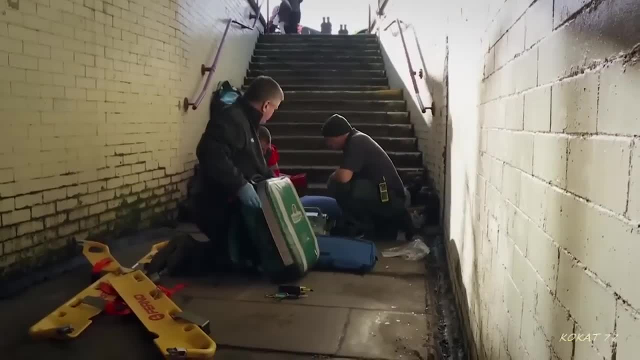 Yeah, no worries, Someone chuck us some cannulation stuff. I'll get a line in for you while you're doing your bits. Yeah, Right, so you're all right with morphine? yeah, Yeah, Okay. Have you had any alcohol or drugs today? 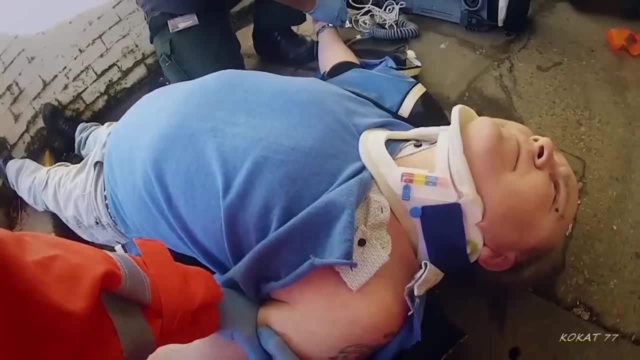 No, Right, so let's have a quick race, or so? Oh, he's fine, Breathing, reasonable. You happy with his chest, It's clear? Yeah, Daff, question This pain at the bottom of your back, Yeah. 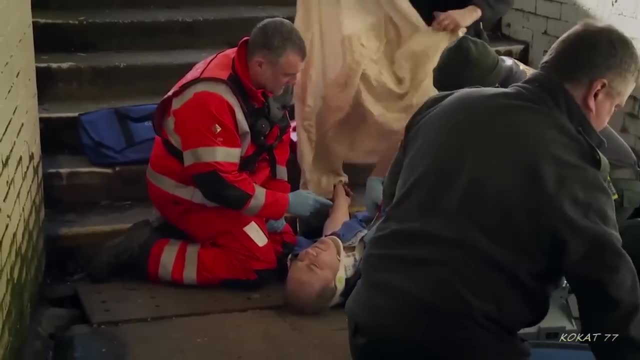 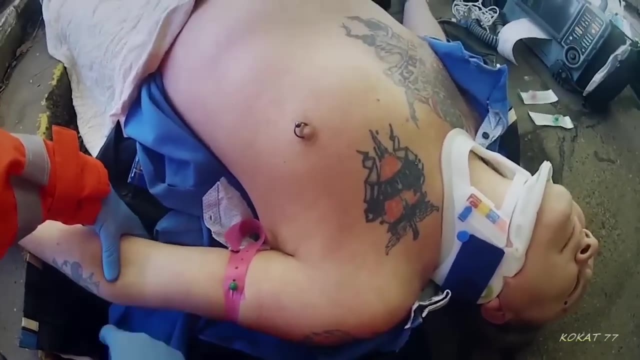 Give it a number between one and ten. What number would you give it About an eight? About an eight. Yeah, Okay, Tom, can you wiggle your foot? Yeah, Yeah, Yeah, Yeah, Yeah, Yeah, John, can you wiggle your toes, mate? 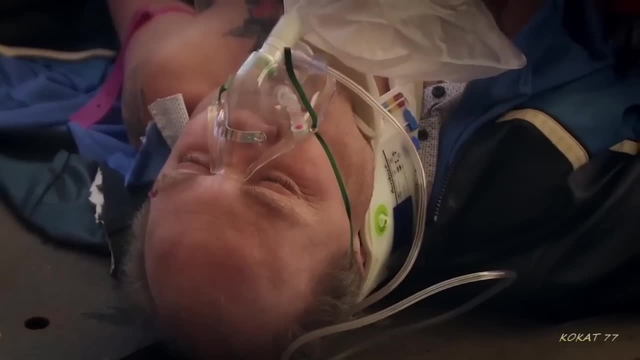 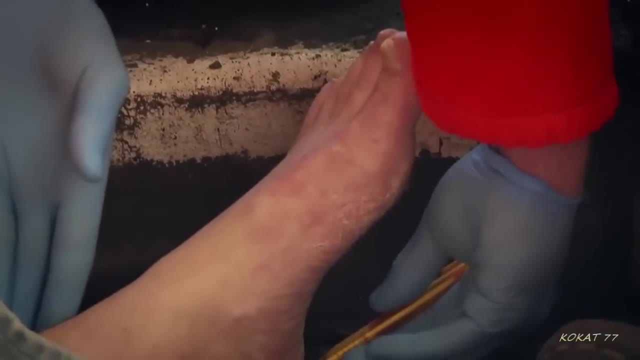 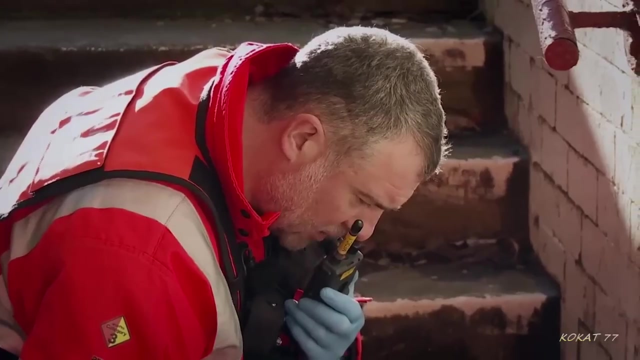 Can you feel me doing that? No, No, Just going to rub your foot, mate, All right, Do you feel that? Oh, okay, It's a worrying sign. this might not be a straight forward tumble. We've got negative Babinski's at the moment, so it's going to be a further assessment. 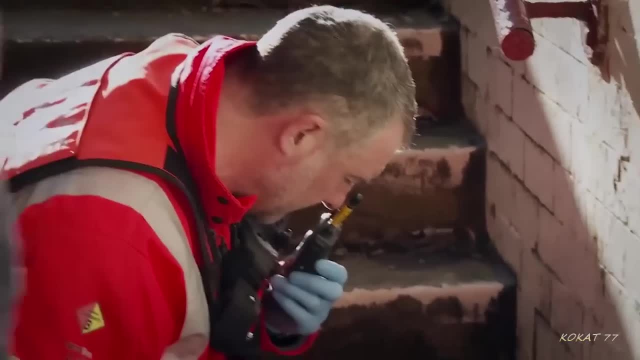 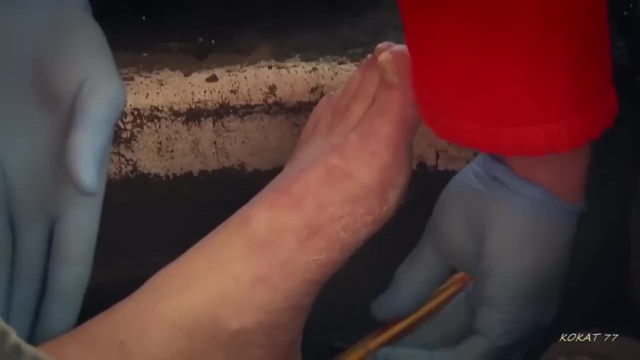 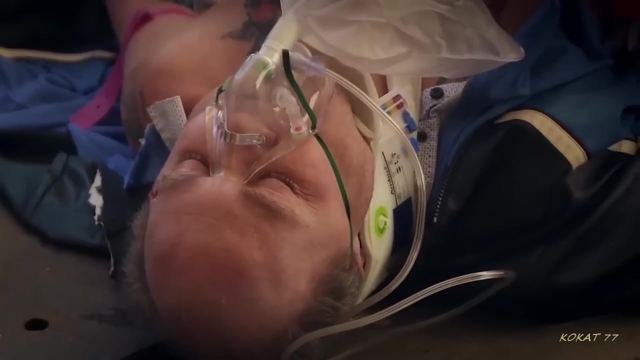 get them packaged up and I think Roud's probably gonna be better. I hope Testing the Babinski reflex is a way of seeing how well the nervous system is working in adults. toes down are good, toes up are bad. John's response could indicate damage to the spine, but then he reveals a crucial piece of information. 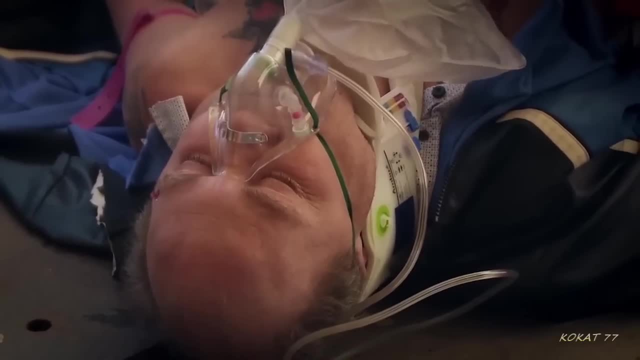 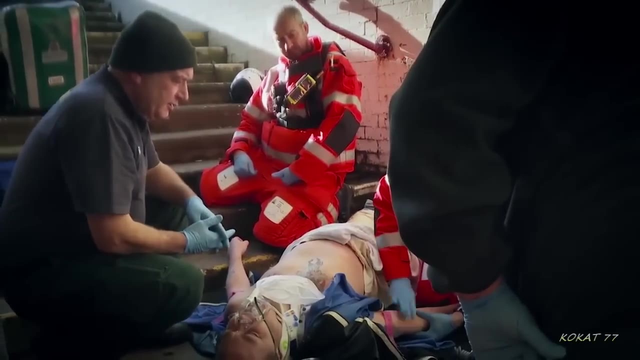 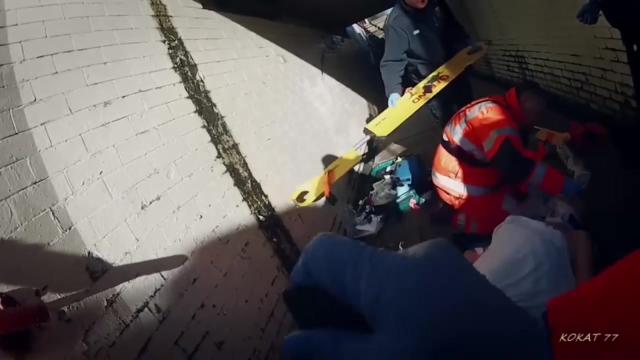 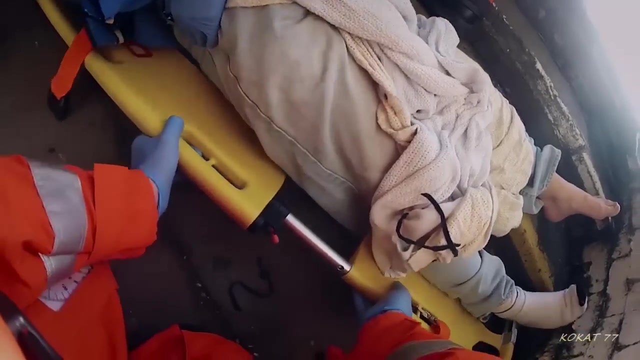 John has a muscular condition which alters his sensitivity to pain. it could also explain why he fell down the stairs after a dose of morphine. John's ready to leave the less-than-hygienic environment of the subway. even now, paramedic Al is not certain about. 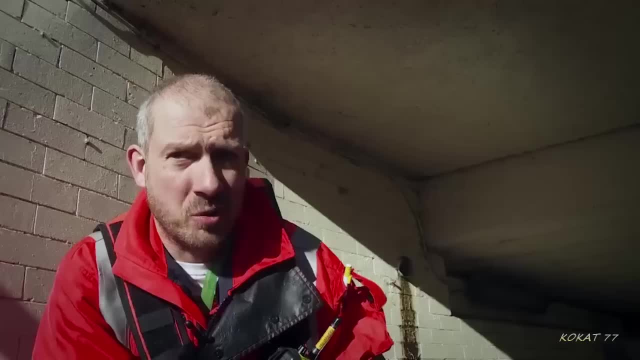 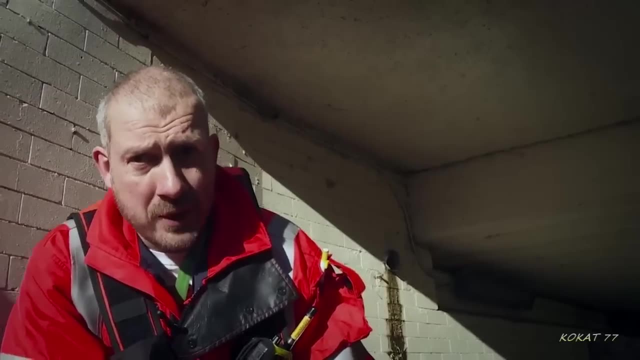 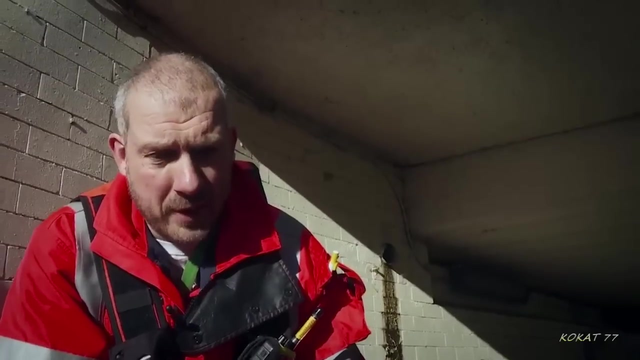 his patient's condition. there's a little bit difficult to assess as to whether what he's experiencing is a result of the fall and an injury to his back, or whether it's just his normal kind of medical problem that he has. so, just to be on the safe side, we're going to immobilise him and then he'll probably go up to LGI. 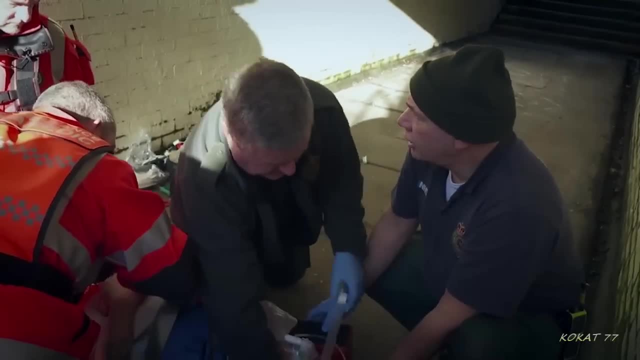 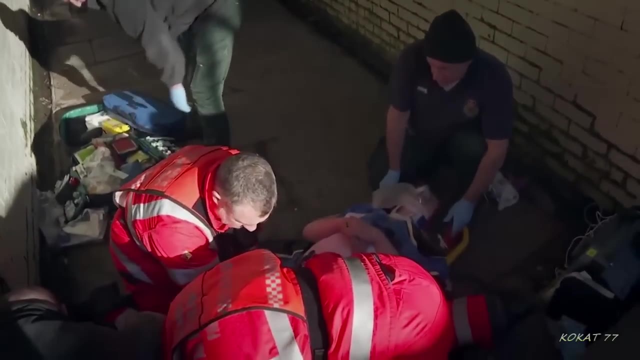 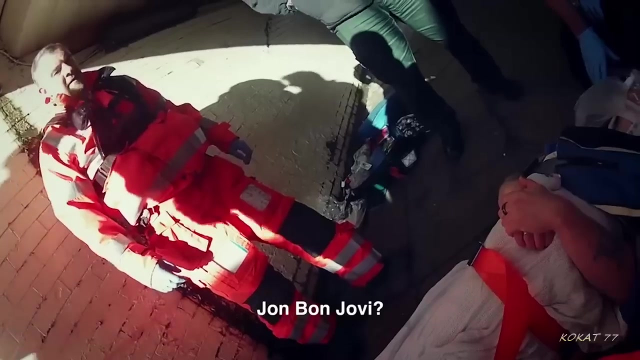 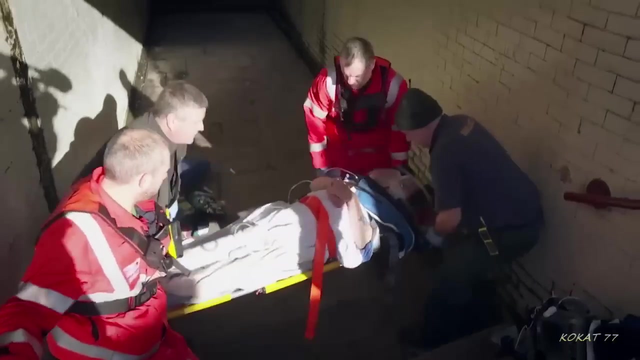 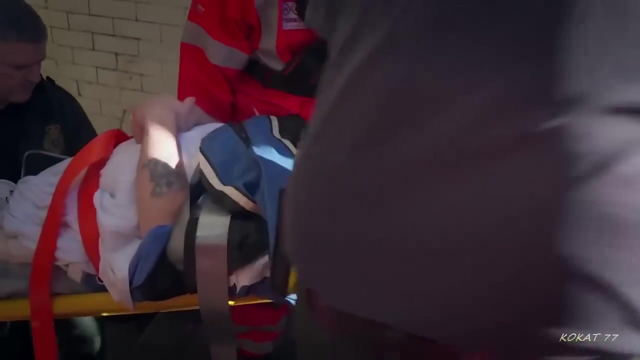 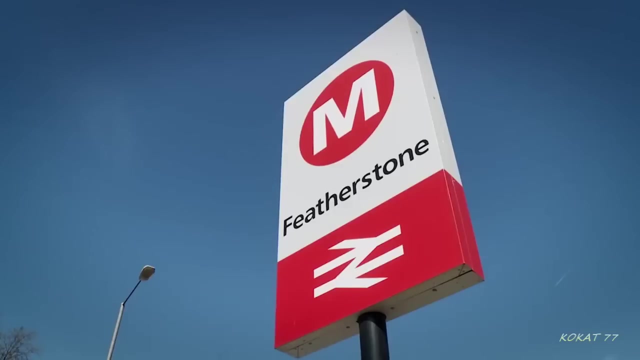 despite his trip to hospital. doctors are sadly unable to pin down the precise cause of John's fall, but he's leaving the medics in no doubt about one thing, and that's John's devotion to his favourite band, as proved by his full name, John's very이트. 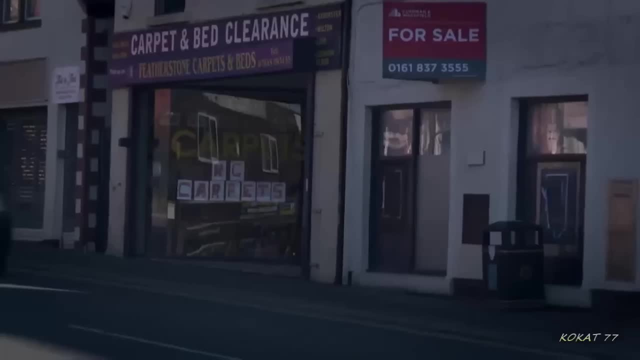 so this is quite renowned for its celebrity areas. I think Obamas busy later on today to go to the chip exe. yeah, I'm glad you got me at the end of a long day. great to see you then. I'm thinking we're off to do another run, though, but you've And it's not every day you get to rescue rock royalty. Don't worry, we're halfway there. You've got so many Rollers. Fennyson is quite renowned for its celebrity areas. I think Obama's visiting later on today to go up the chipby, so I can't довere a get some of the stuff we've got. You've got two people in this room here, Right about two or three people too. 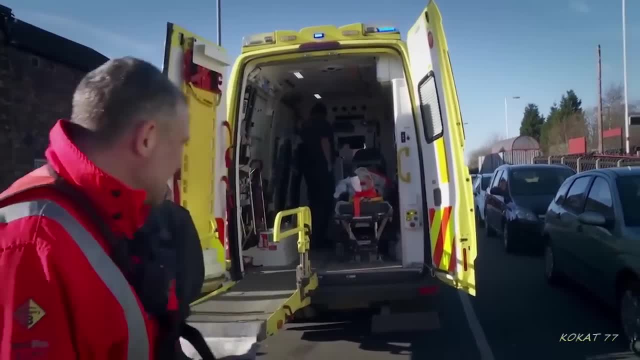 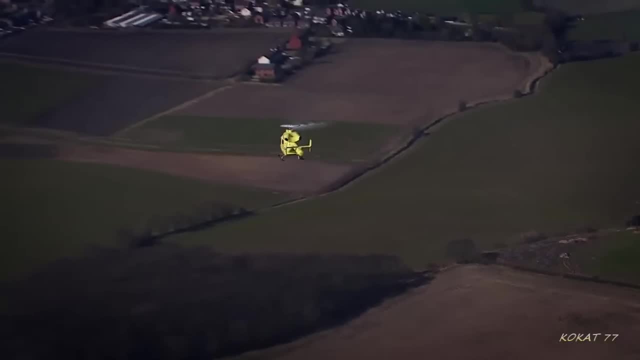 Mixing with a high life. again, Helimad 98 leaves without a patient. It's quicker for him just to go by land to leave, so it's a lot better for the patient. And Al and Pete are on a roll with Bon Jovi's back catalogue. 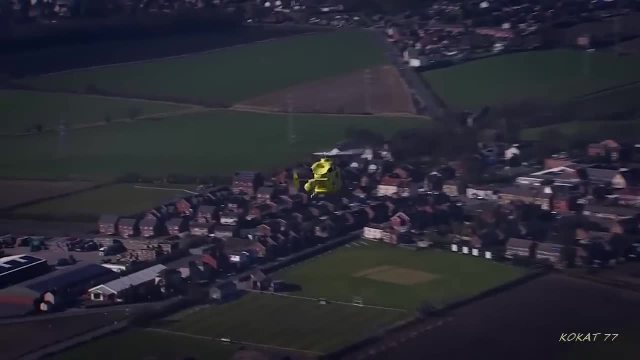 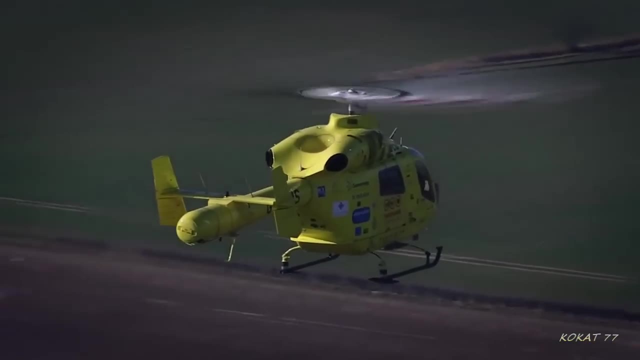 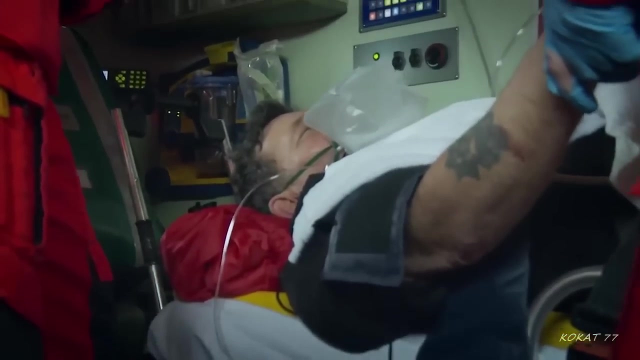 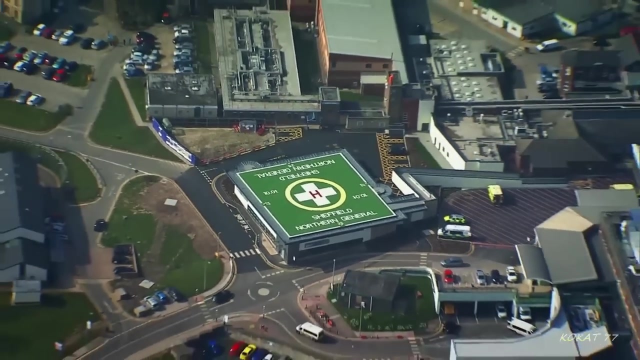 Keep the faith and hopefully he'll be all right. Well, you know what, Al? I will always love you, HE LAUGHS. Factory worker Tony underwent surgery on his left hand at Sheffield Northern General Hospital, But doctors were unable to save it and it was amputated. 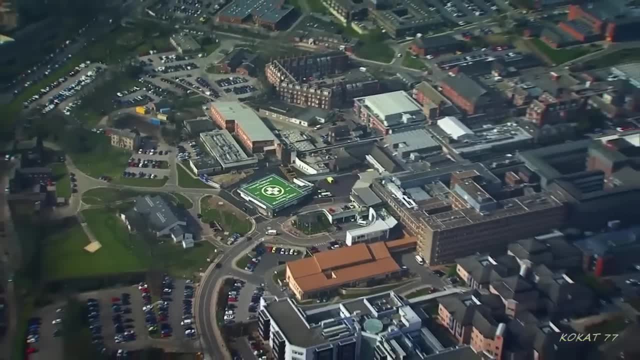 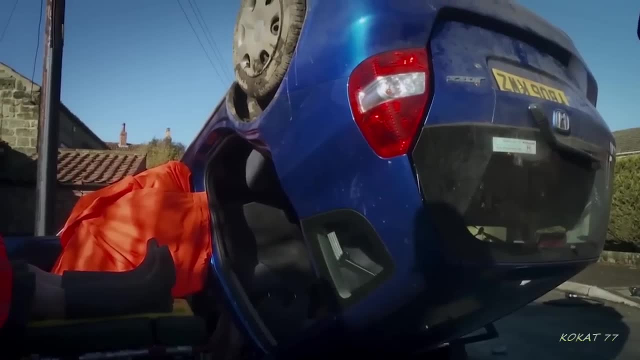 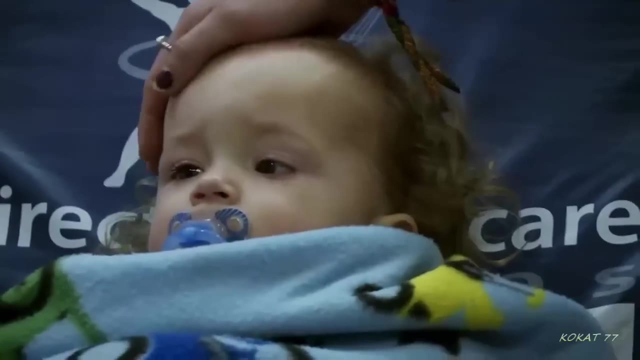 He's now returned home and is adapting to life without it. Elizabeth, the elderly passenger trapped in an overturned car, spent more than three weeks in hospital but recovered well and is now back home in York. He's had 50mg of blood. 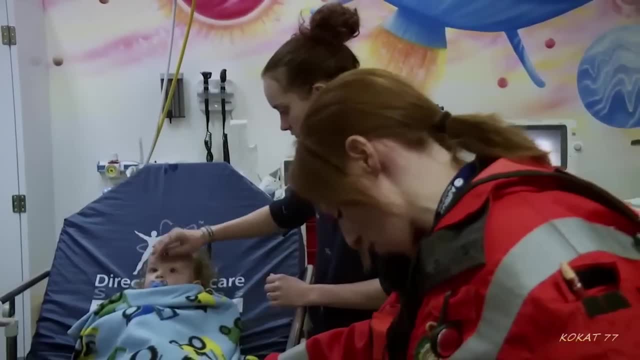 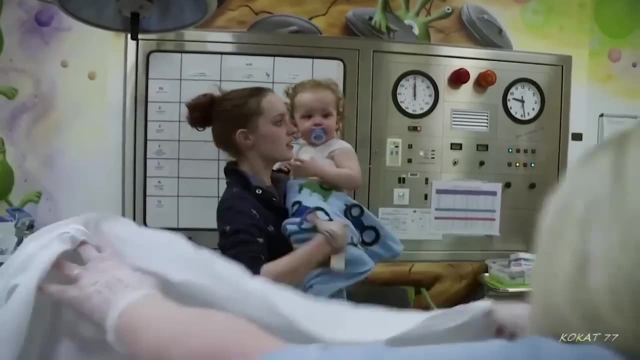 He's had some ibuprofen given by Mum and he's had 2mg of Oromath by us. Little Finley, who spilled a cup of scalding coffee, was found to have only superficial burns and he's now back in the Yorkshire Dales with his relieved Mum. 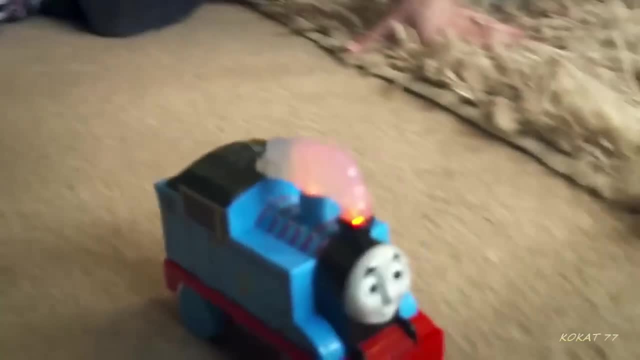 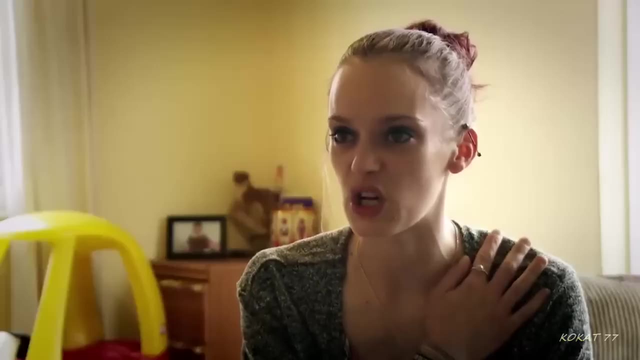 Ready. One, two, three Coming through. It looked awful. I think it looked a lot worse than it was. We thought it might have hindered him a little bit, cos it's on his shoulder, but no, he's still climbing the furniture. 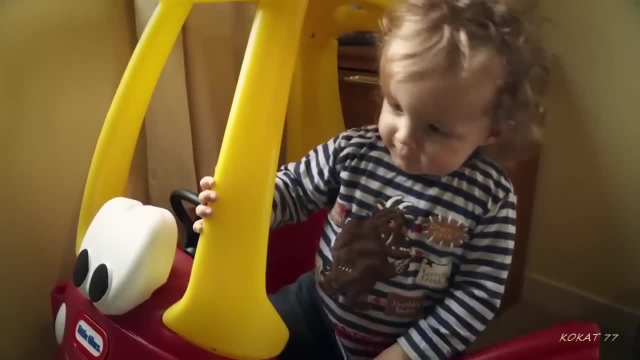 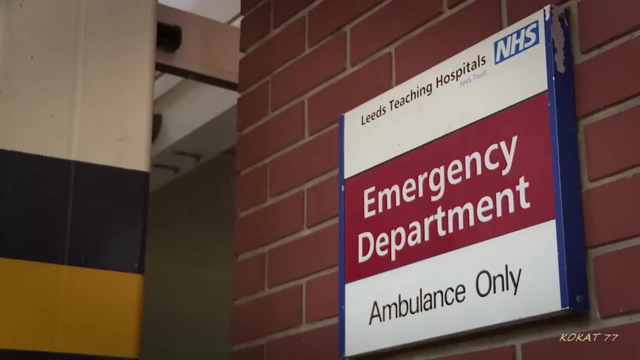 he's still, you know, trashing things. He's not at all fazed by it. Scans at Leeds General Infirmary revealed that day-tripper Rob escaped serious injury when he fell from one of Yorkshire's most famous landmarks. 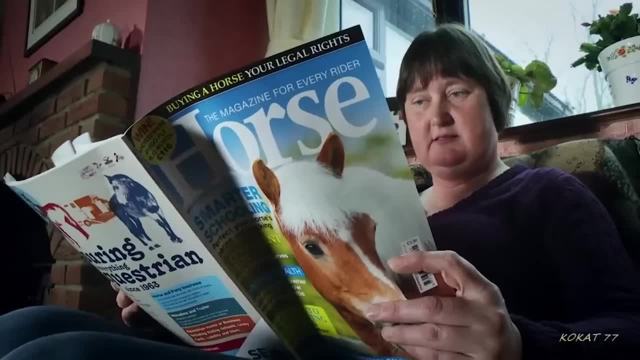 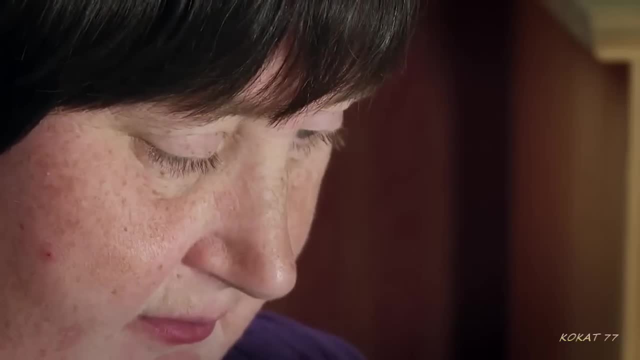 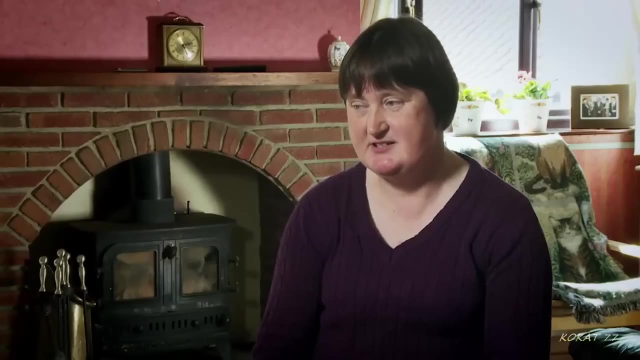 But it was a close call And Rachel, whose allergies have landed her in hospital a dozen times, was put on a two-week course of powerful steroids. The cause of her anaphylactic attack is still a mystery. It's difficult. It's obviously difficult for friends and family. 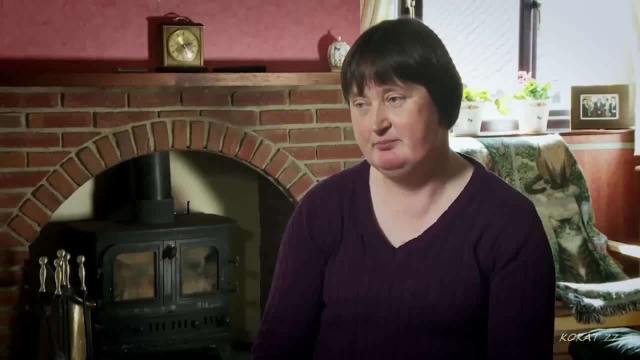 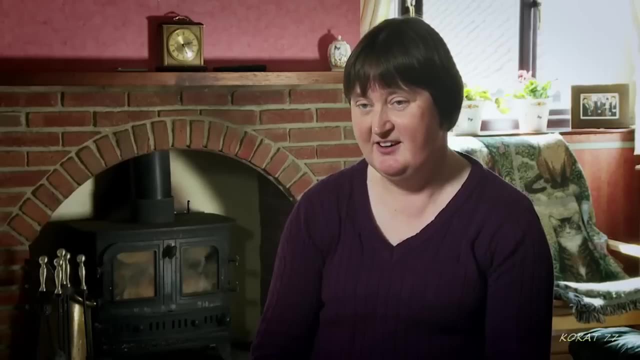 Close friends and family have got used to it. But for onlookers it's quite frightening to see suddenly somebody just swell up and go and can't breathe. It tends to be the onlookers that panic. If I panicked I wouldn't be here. 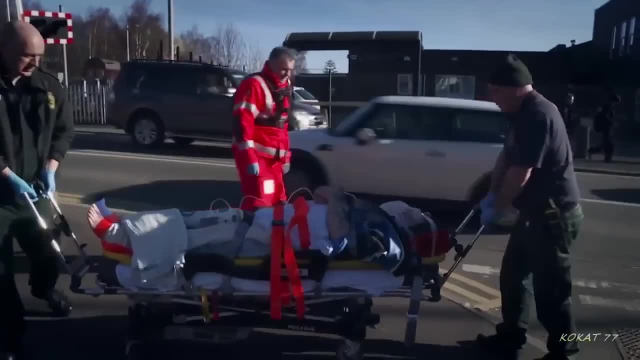 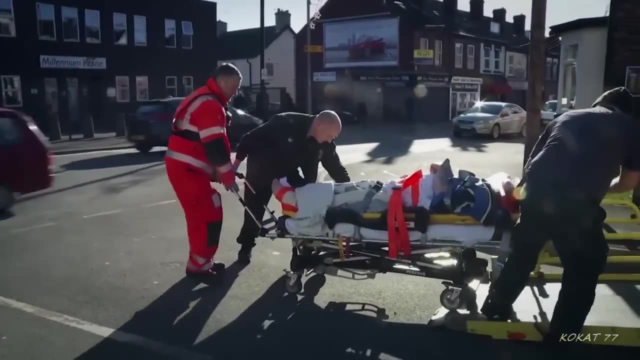 The other, John Bon Jovi, lives in sheltered housing in Featherston and uses a wheelchair following his fall, But he's still a rocker at heart. He's a very possessive and talented man, and a godly man. He's a womanizer. 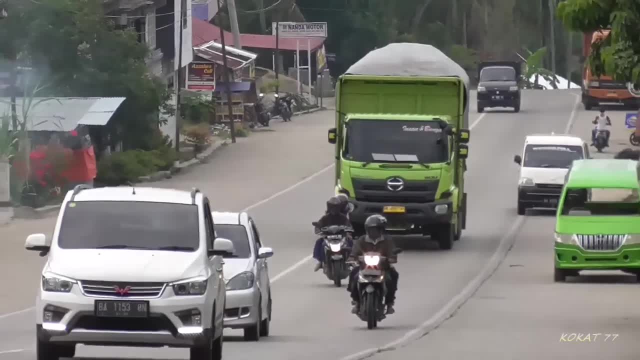 He's a shrewd man, He's a nice guy And he's a great man And he's a great guy. He's not a bad guy, It's just he hasn't got the ability to do a good job of it. 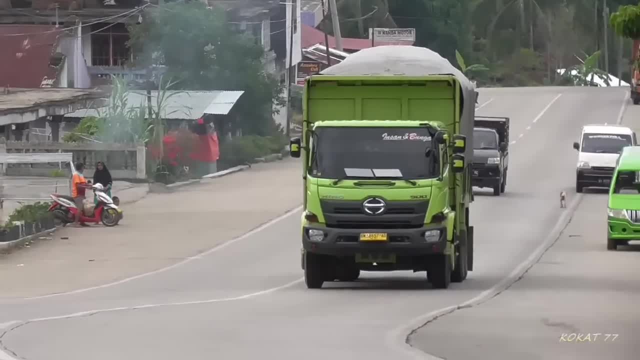 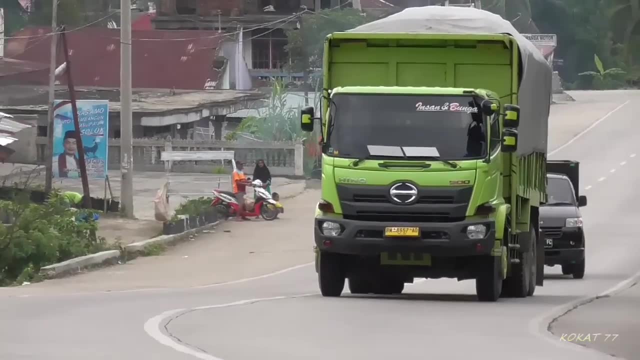 He could have done better? Is this the only time you've heard him say that? If that's possible, I guess he's a little more comfortable. So the main thing is, if you do care, it's actually not something you're interested in. 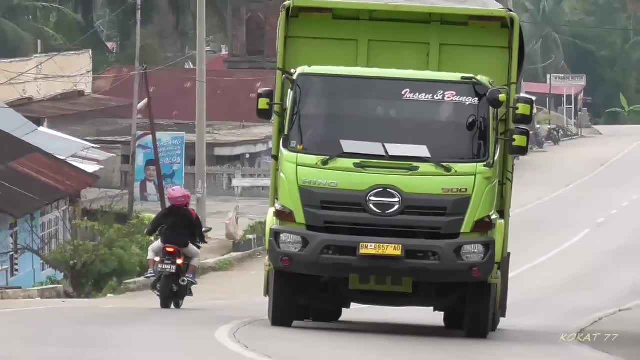 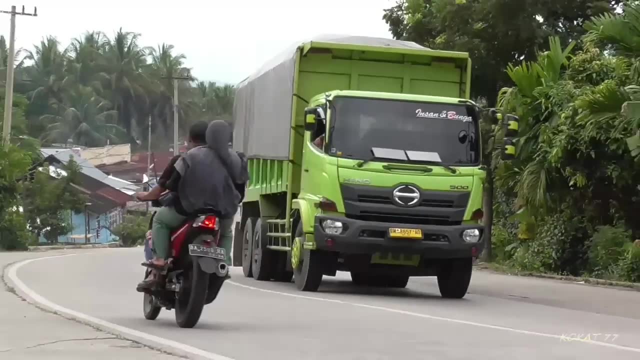 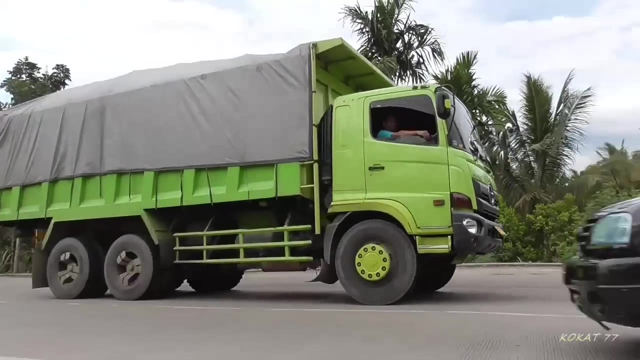 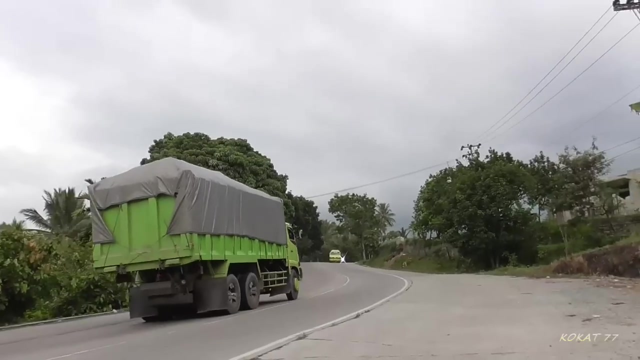 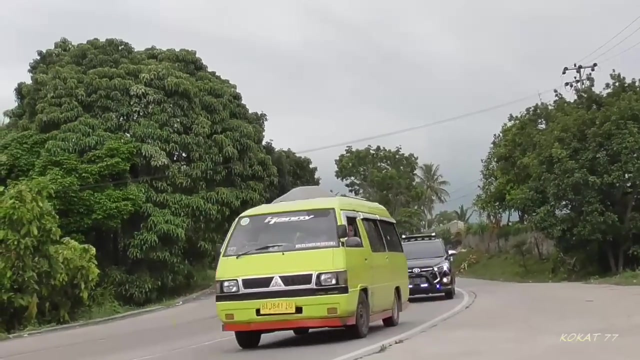 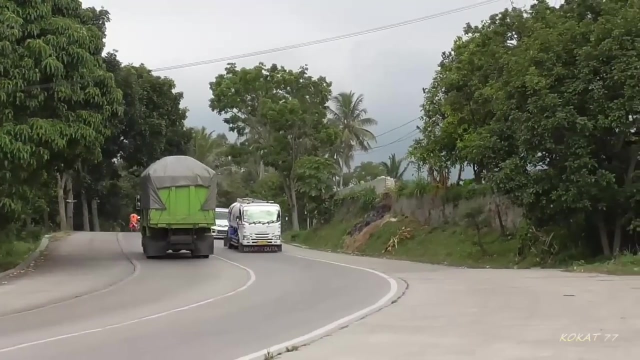 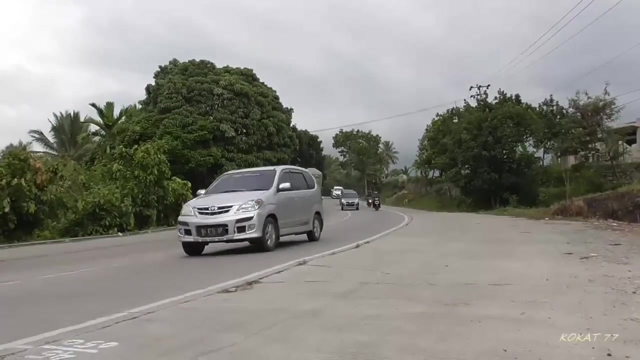 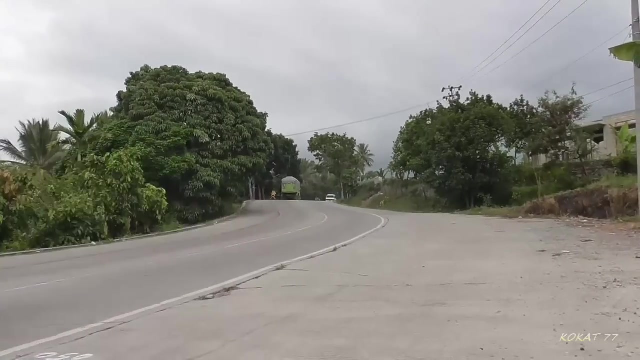 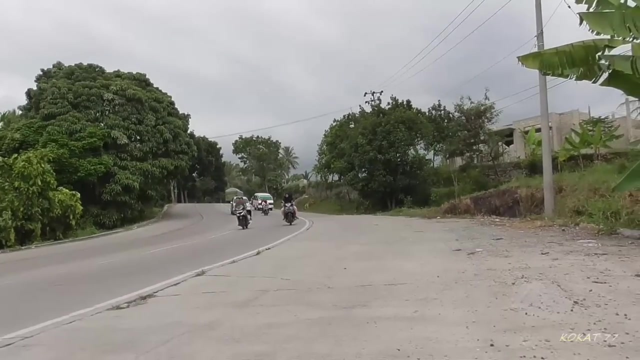 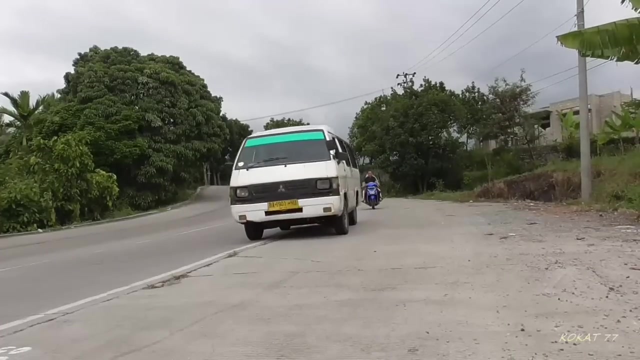 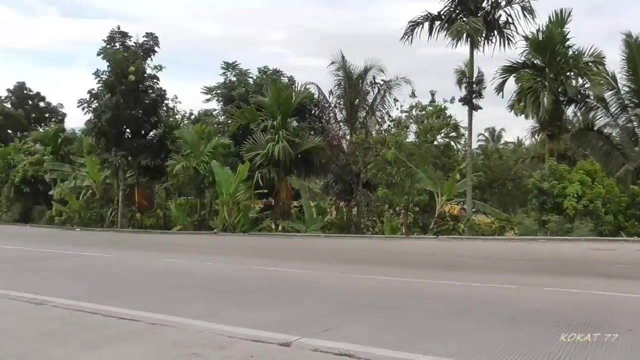 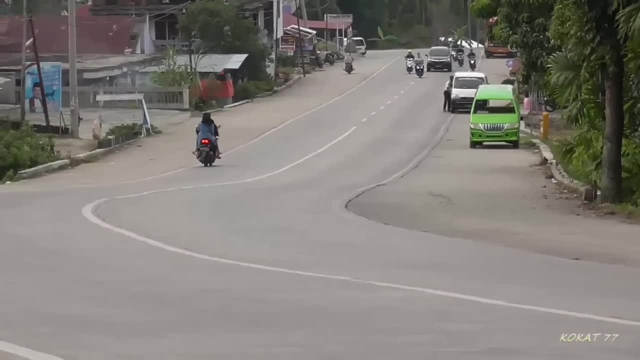 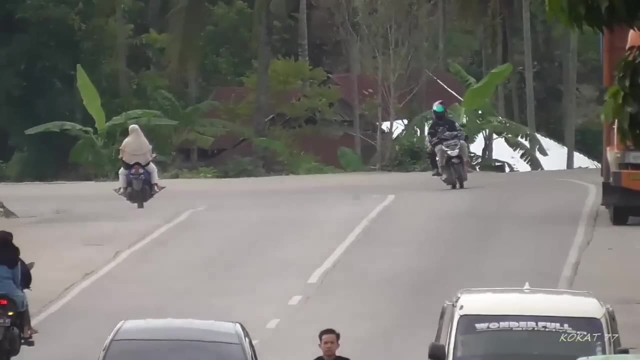 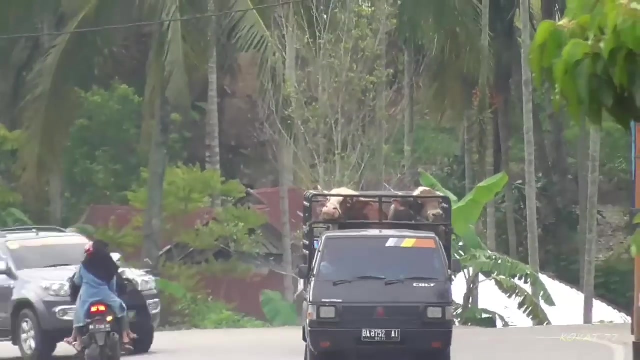 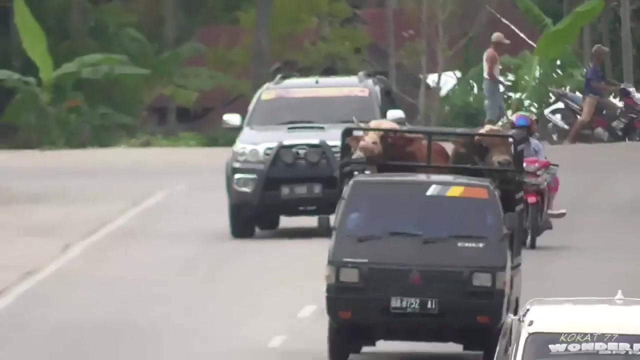 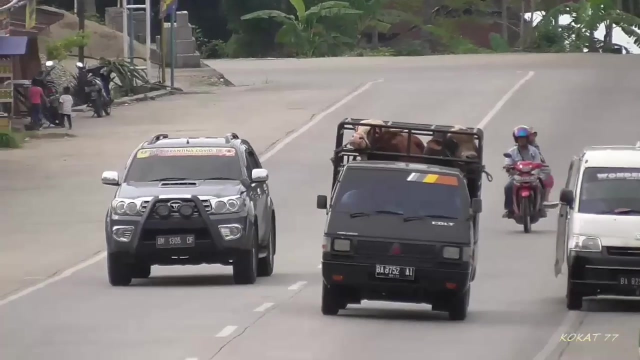 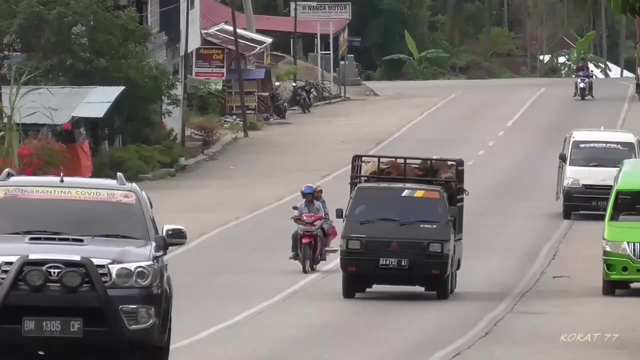 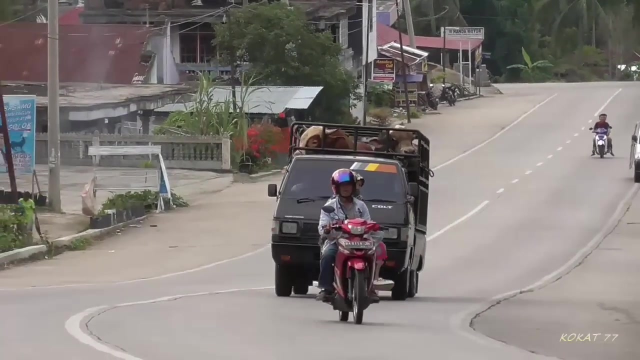 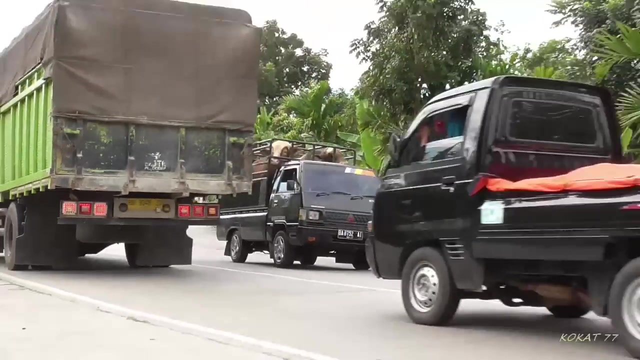 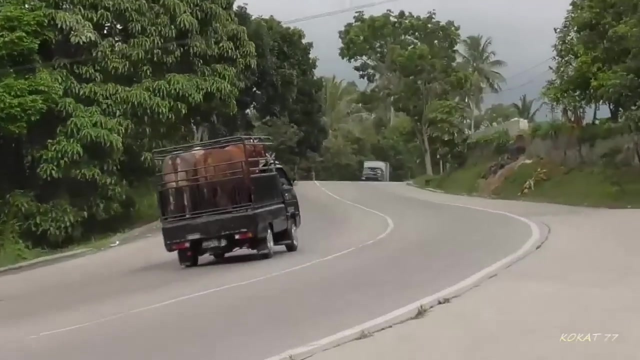 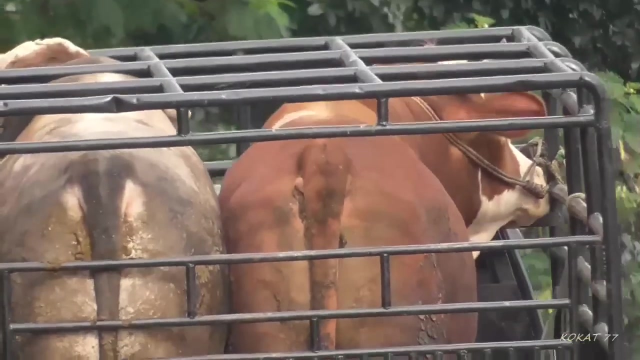 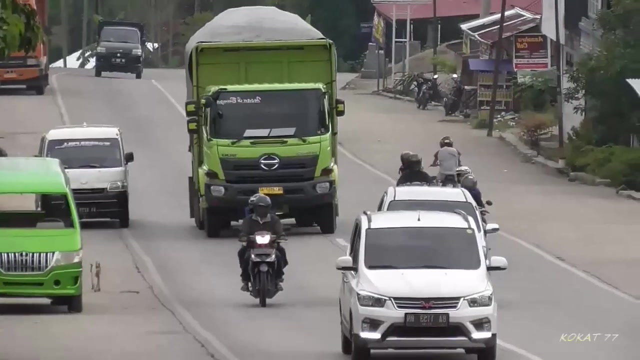 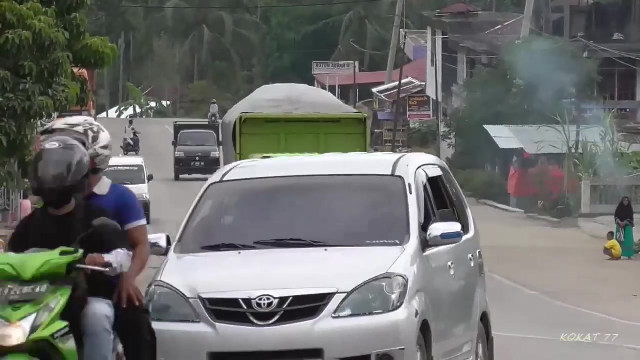 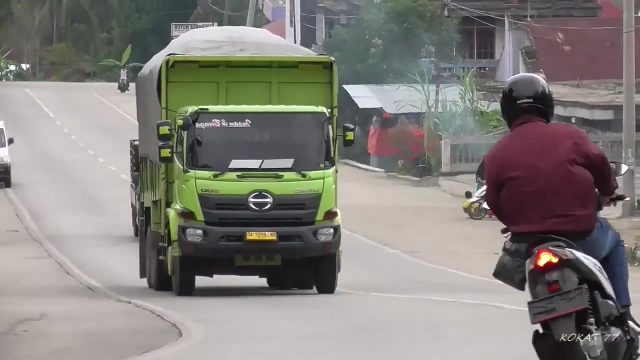 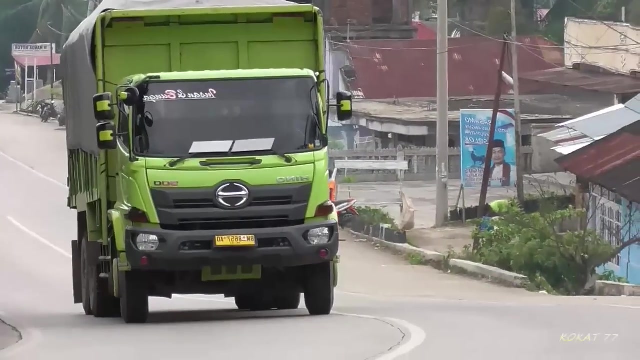 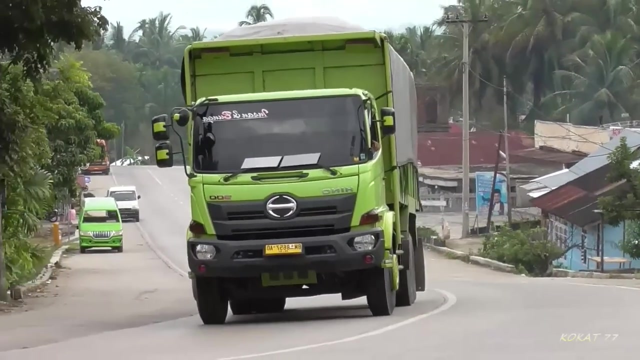 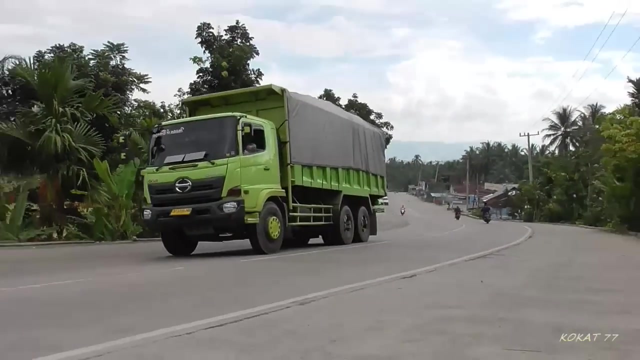 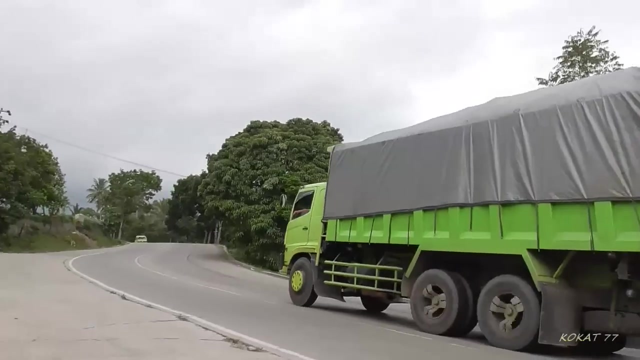 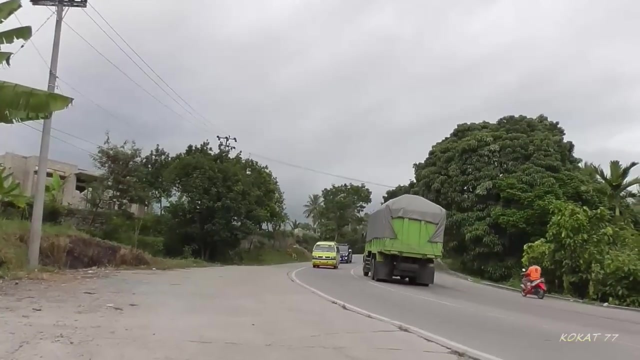 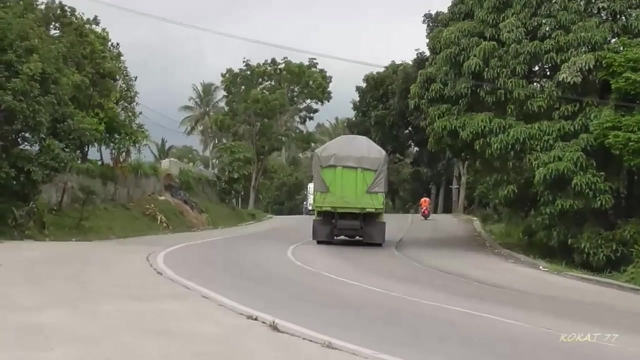 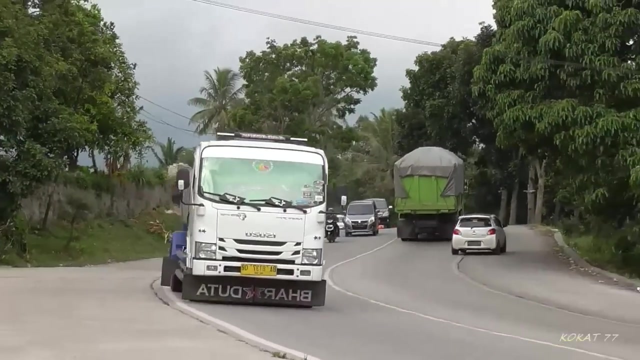 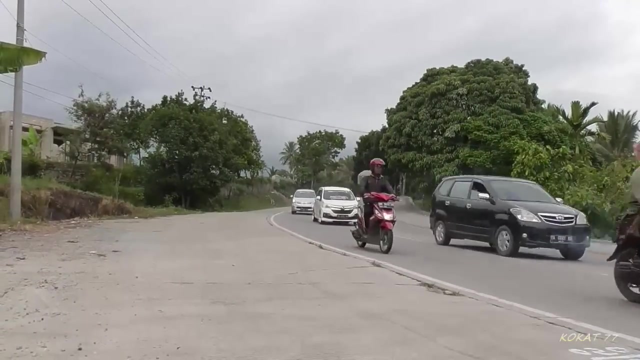 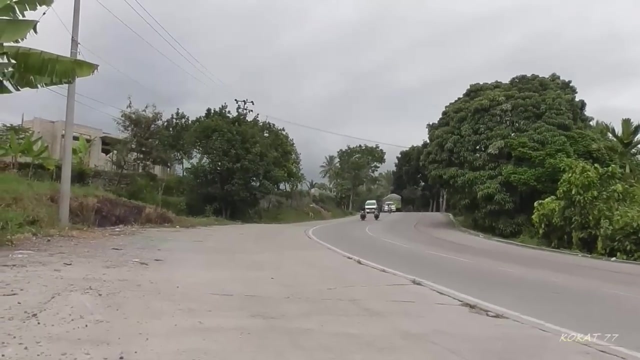 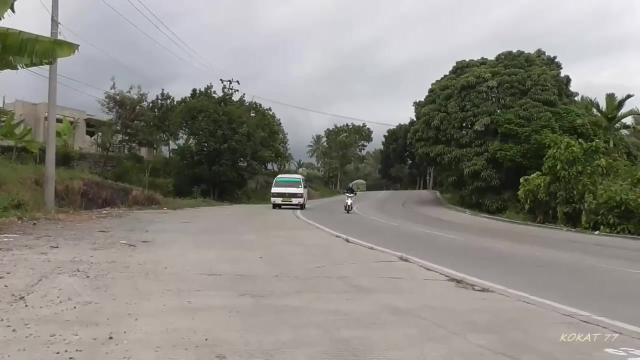 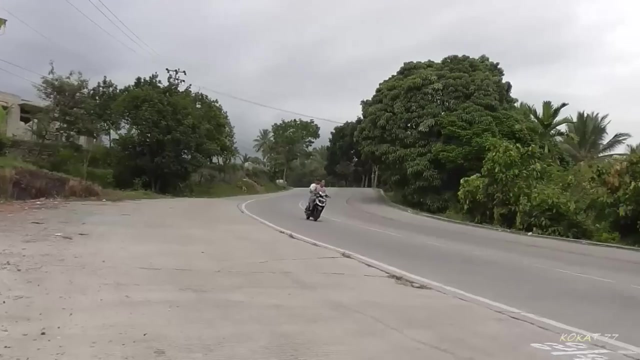 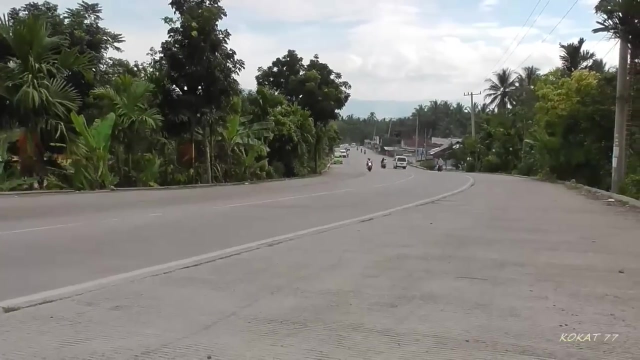 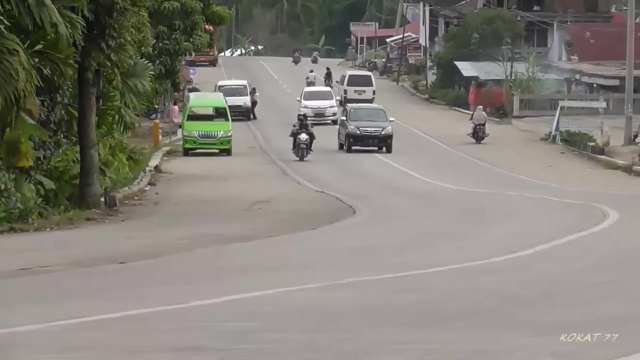 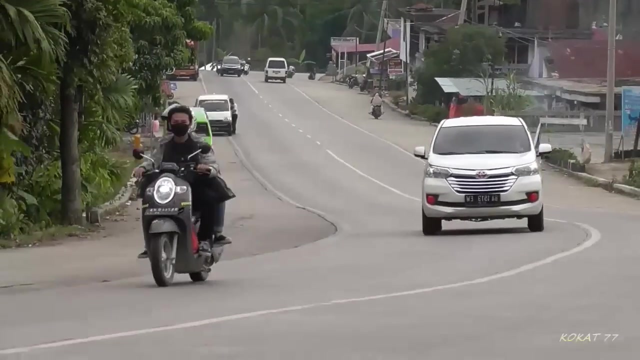 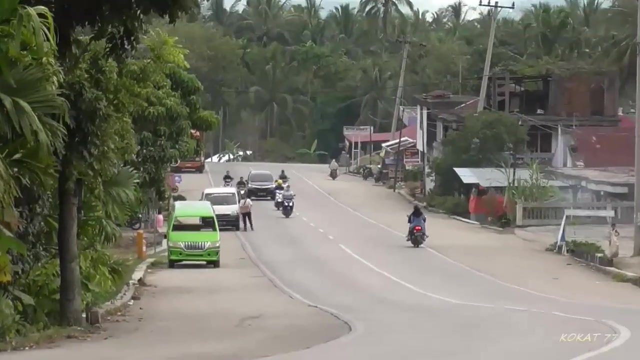 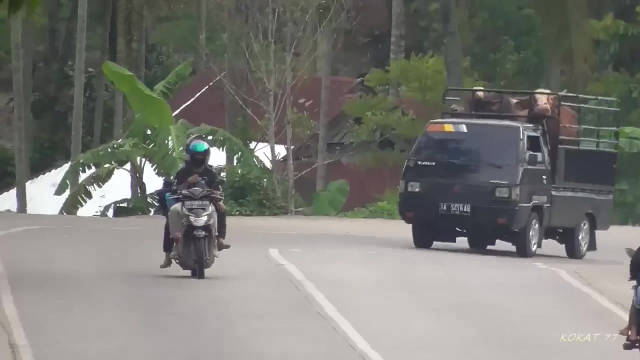 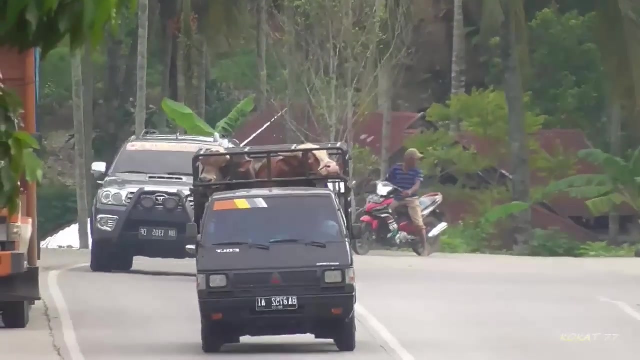 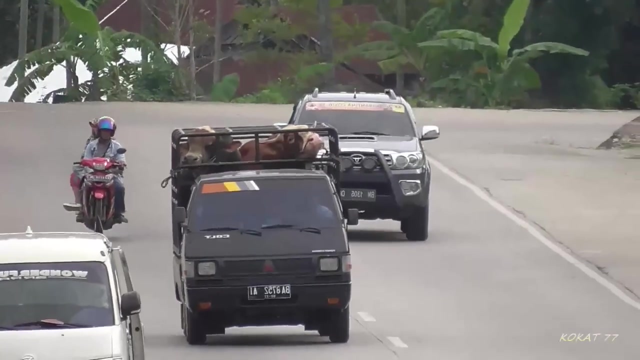 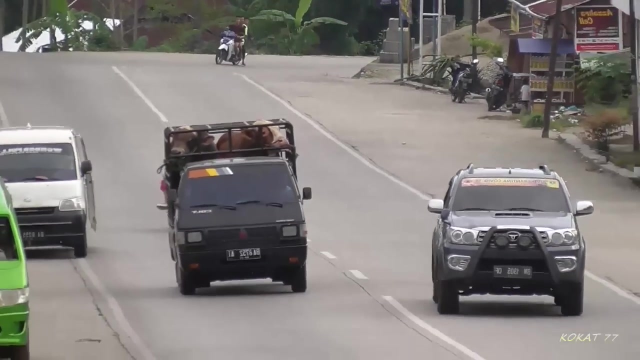 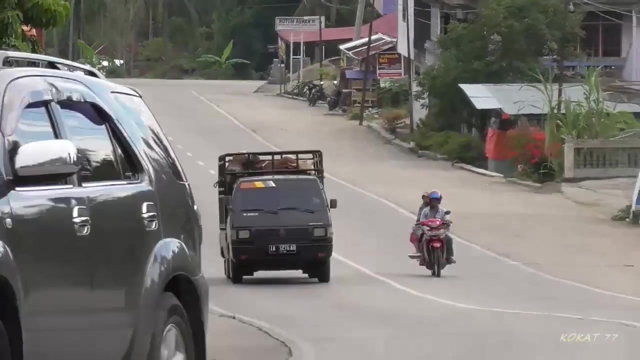 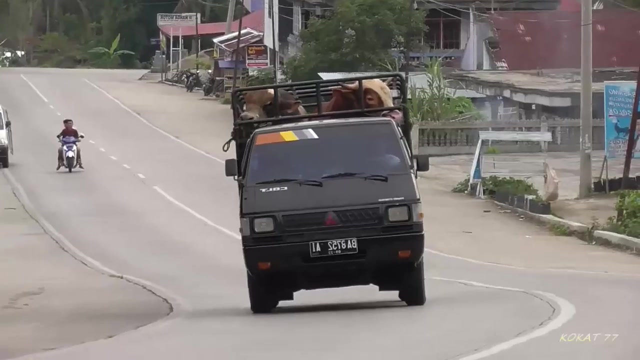 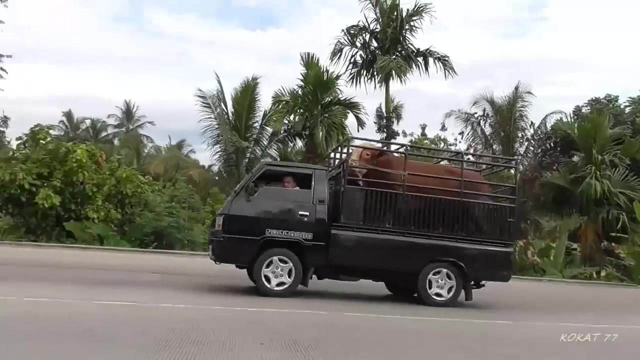 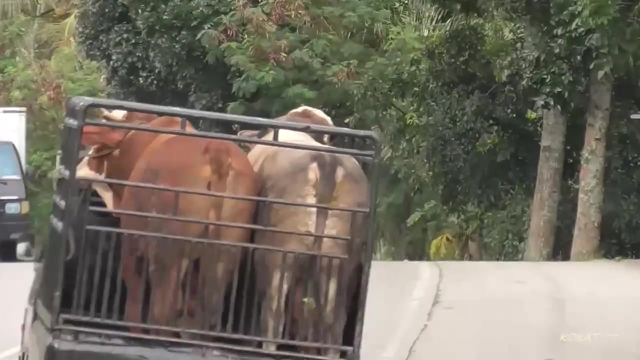 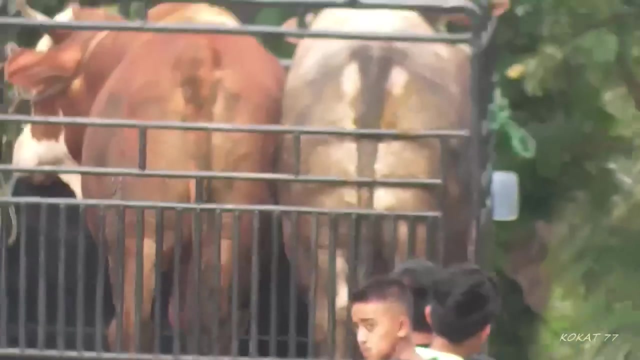